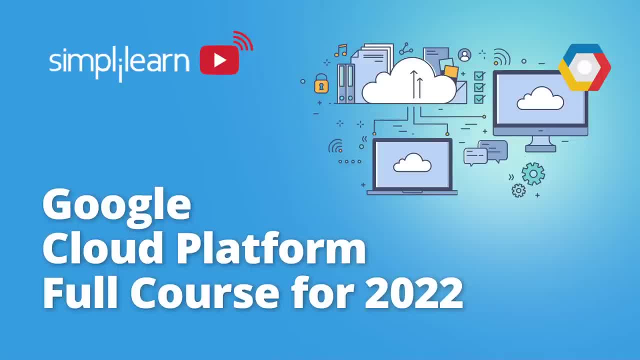 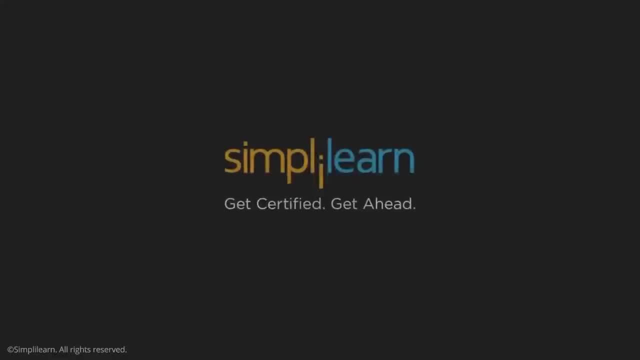 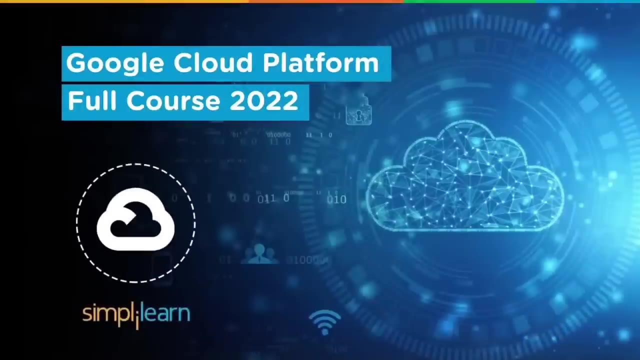 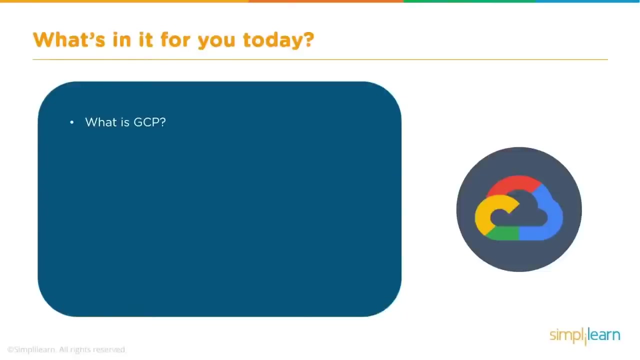 Hello everyone, welcome to this interesting video on Google Cloud Platform full course. In this video, we will explore and understand all the important concepts revolving around Google Cloud Platform, starting with the basics of what is GCP and its following concepts, like GCP domains comprising various services like compute, storage, networking, IoT, etc. 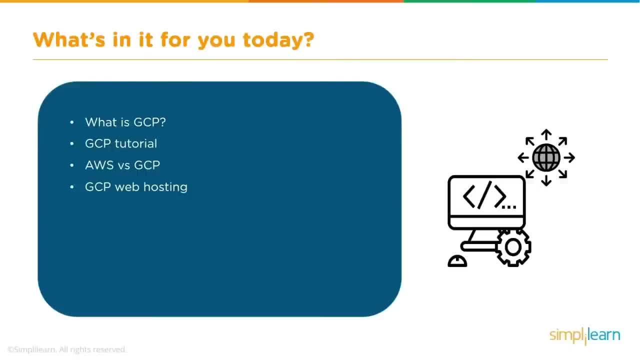 With a proper hands-on demonstration on these services. Following that, we will have a comparison between GCP, AWS and Azure and we'll see how they differ from each other and how they hold their individuality, And then, at the end, we will understand some of its depth. 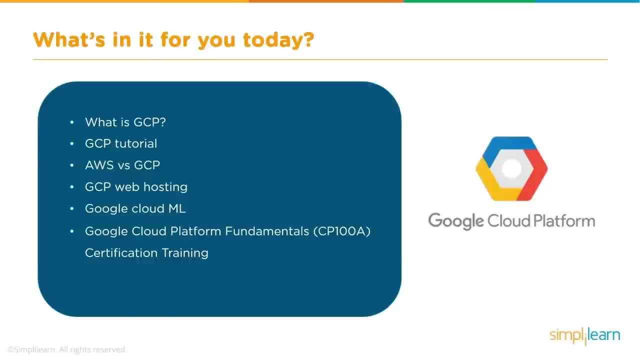 concepts like GCP web hosting and GCP Cloud ML, And towards the end, we will take you through GCP fundamentals and certification training that will help you gain this certification. So for this training, with me I have our experienced GCP specialist Together. we will take you. 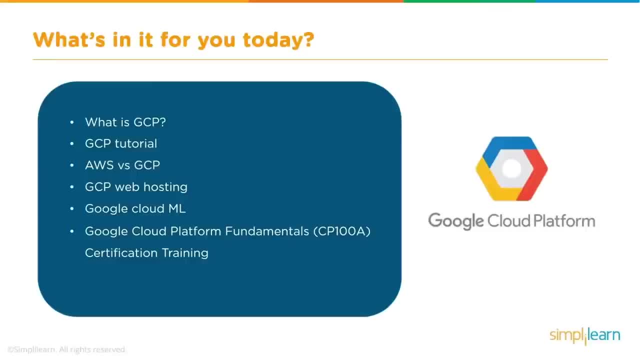 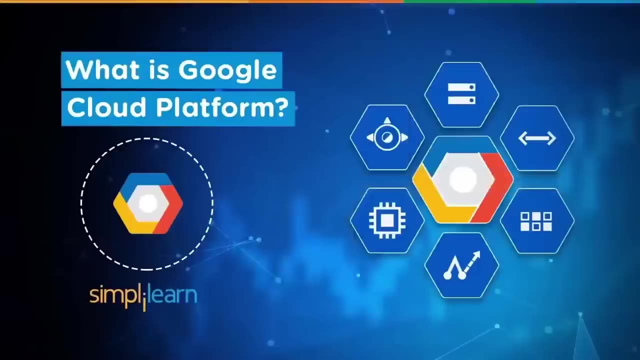 through the various important keynotes. So let's start with an exciting video on Google Cloud Platform full course. Before we begin, make sure to subscribe to our YouTube channel and hit the bell icon and never miss an update from Simply Learn. Good morning and good evening everyone, So welcome to this session on Google Cloud Platform. 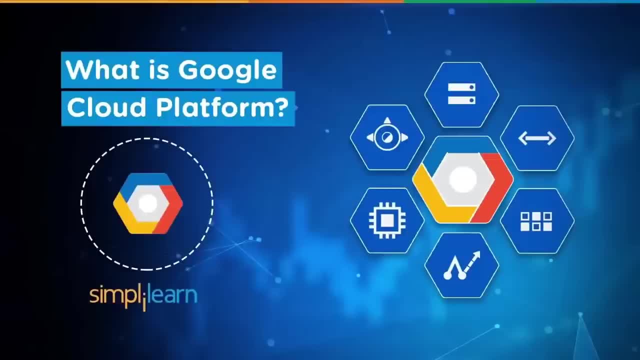 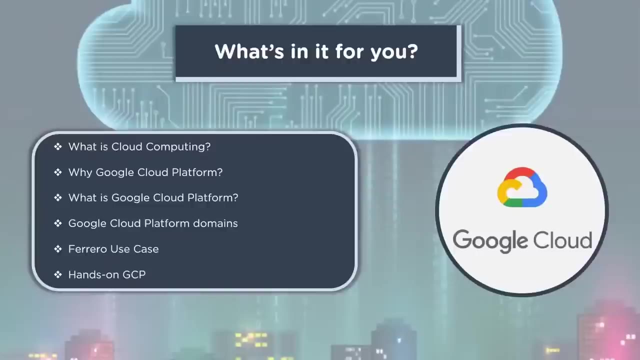 My name is AJ and I'm an instructor with Simply Learn and also working as a big data and cloud architect. We have various clients across the globe. In this session, we learn about Google Cloud Platform, wherein we will learn about: what is cloud computing, why Google Cloud Platform, what is GCP? that is Google Cloud Platform. 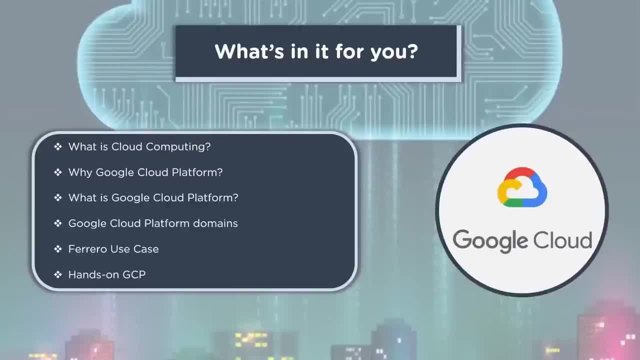 Google Cloud Platform domains, about a use case- that is, Ferrero use case, and also a quick demo on using services from Google Cloud Platform. So when we talk about Google Cloud Platform, we also need to know about GCP. We need to know what is cloud computing. 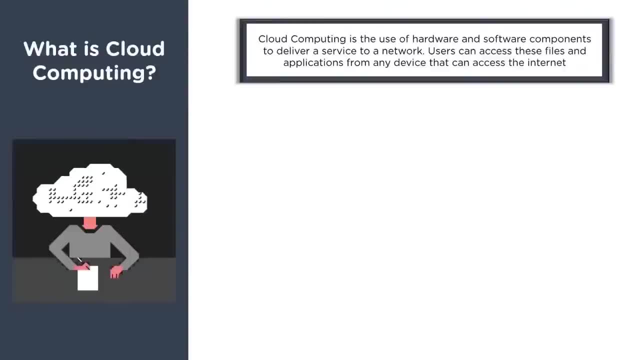 So cloud computing is the use of hardware and software components to deliver a service to a network. Users can access these files and applications and services provided by a cloud provider from any device that has access to internet. In short, cloud computing is a way where cloud provider provides access to different services. 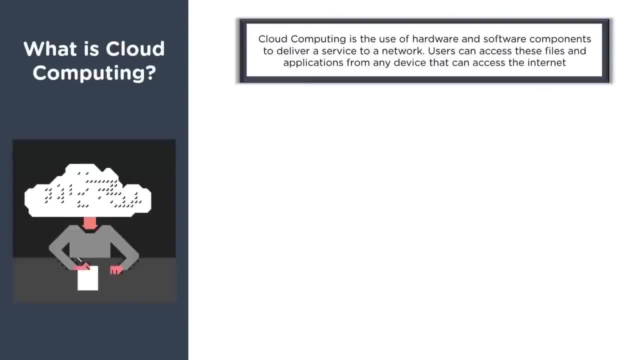 such as resources, And when we talk about resources here, we talk about computing, we talk about memory, we talk about processing power, we talk about storage and we also talk about different services which cloud providers make available for the users. Now that allows us for automatic software integration, backup and restoring data unlimited. 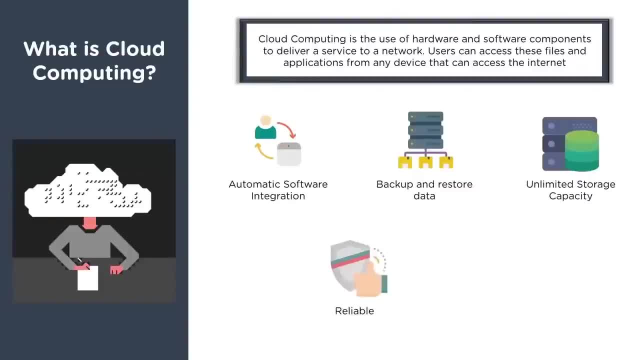 storage capacity, having a reliable use of different data. So that's what we're going to talk about today. Thank you, Thank you Bye bye. And also some organizations build their own private clouds using open source, open stack. Let's focus more on Google Cloud Platform and what it has to offer and how it is gaining. 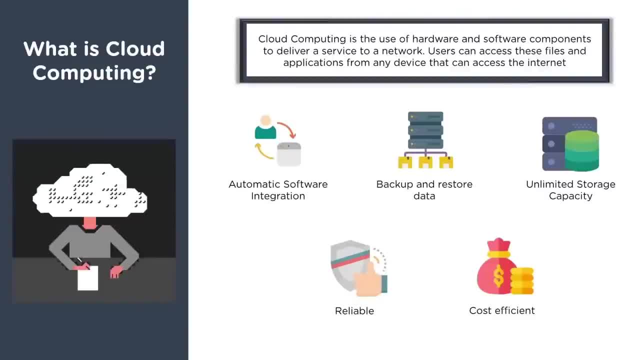 popularity in the market, with different organizations which would want to work on a cloud platform or which would want to work on an infrastructure which is modernized. So when we talk about cloud computing, this is one of the approach which organizations can take to instantaneously benefit from modernization using different services, different platforms. 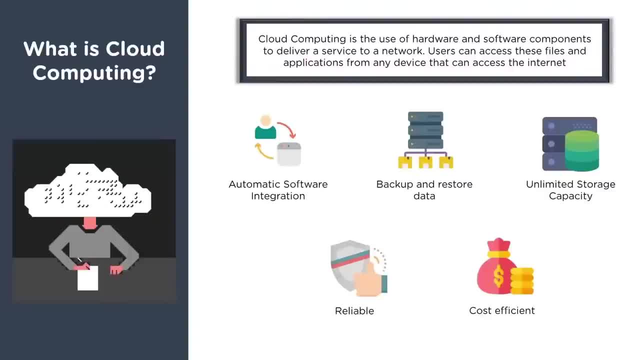 and also newer technologies for their various requirements, such as scalability or dynamic businesses. Before we get into Google Cloud Platform, it is also good to understand where you can find some useful resources. So let's talk about Google Cloud Platform, And here you have a website which is from your Google Cloud. 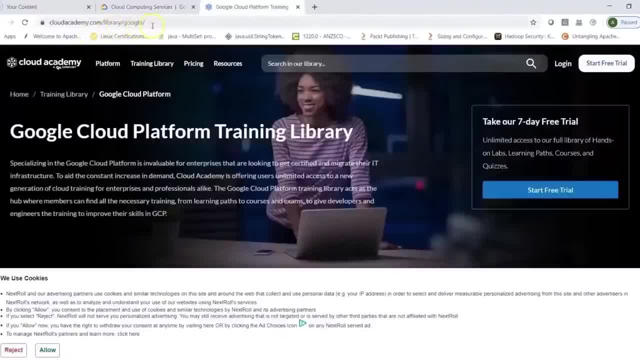 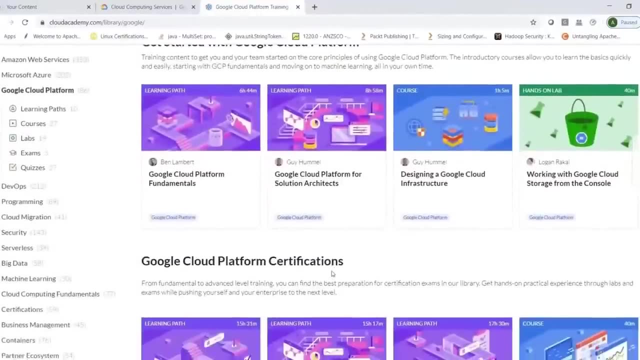 So this is cloudacademycom slash library, slash Google, And here you can create a free account Now. that would give you just seven days trial, but that has a lot of videos which talk about your Google Cloud Platform and essentials, and it has various certification related videos. 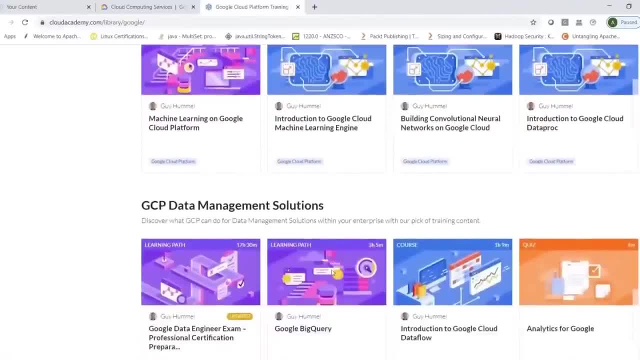 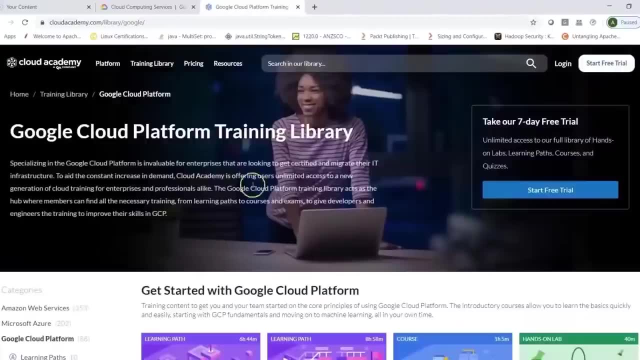 which you can access, And then, after seven days, you can create a free account, And then, after seven days, after you have tried, you can obviously go for a paid account where you can take detailed learning from here. Now. this is your training library, which shows your different cloud providers, such as Amazon. 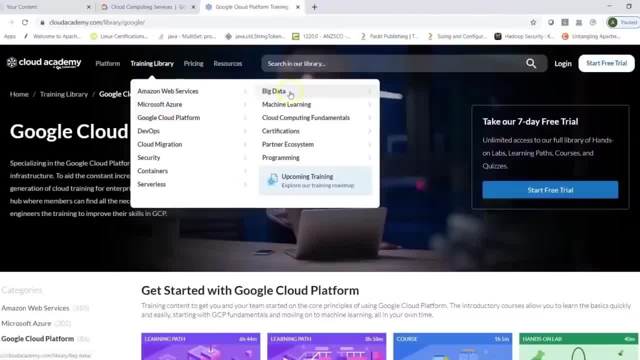 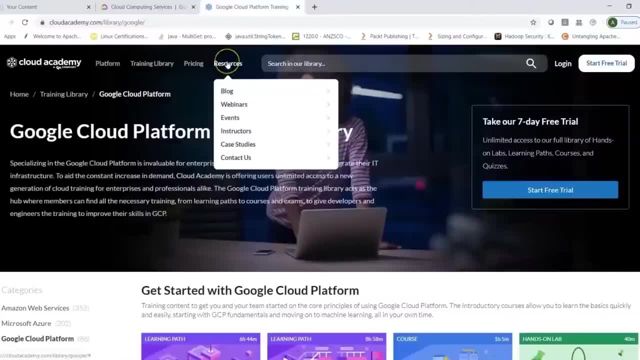 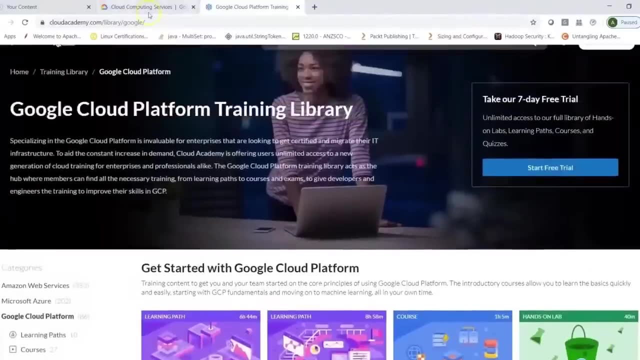 Microsoft Azure, GCP, and then you have various other topics which are specifics to organization. You can obviously look at the pricing and you can also look at resources which will give you a good experience in learning from Google Cloud Platform. You can also create a free account, which I will walk you through later. 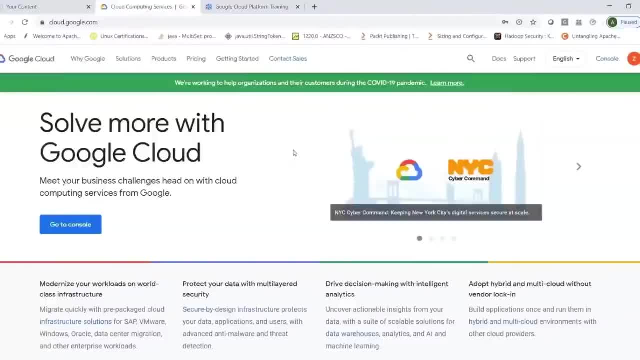 So you can create a free account on cloudgooglecom. Now, when I say free account, that basically means it allows you to create an account, and every user who creates an account gets a 300 dollar free credit which can be used to practice. 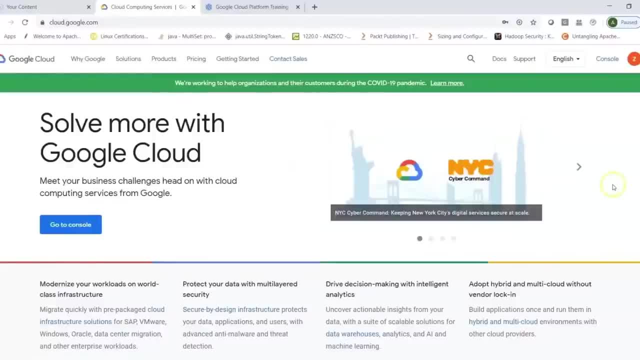 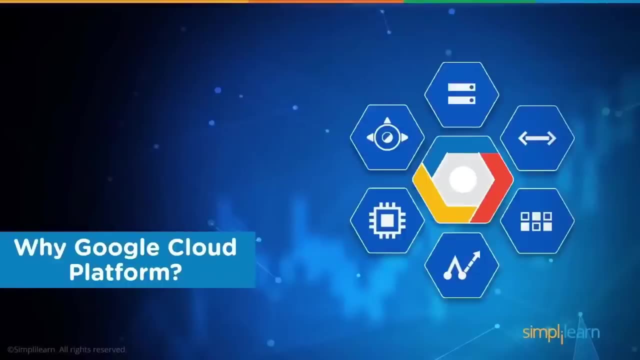 brush up your skills and also explore and learn about your cloud platform- So this is a free account- and learn about different Google Cloud products which are offered by Google. Now coming back to our Google Cloud Platform, let's understand why Google Cloud Platform. 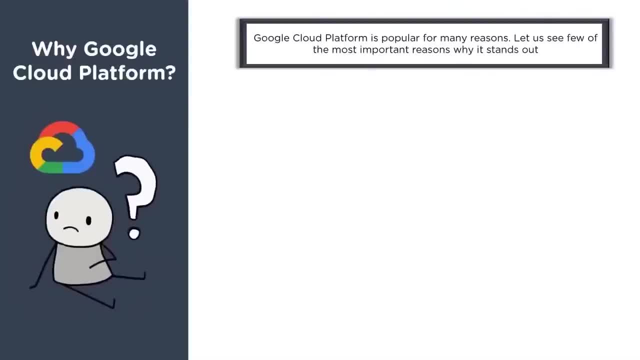 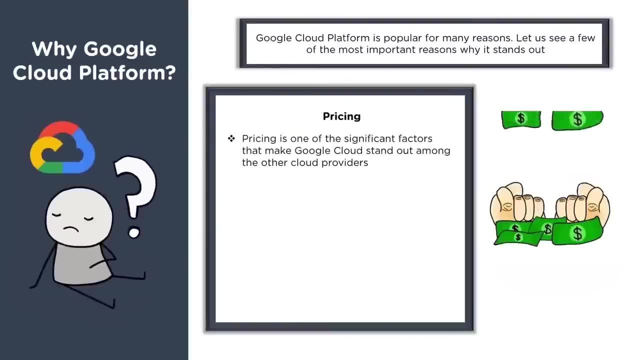 So Google Cloud Platform is popular for many reasons. Now let us see few of most important reasons why it stands out. When you talk about pricing, pricing is one of the significant factors that make Google Cloud stand out among the other cloud providers. It offers a monthly pricing plan which is billed according to monthly usage and when. 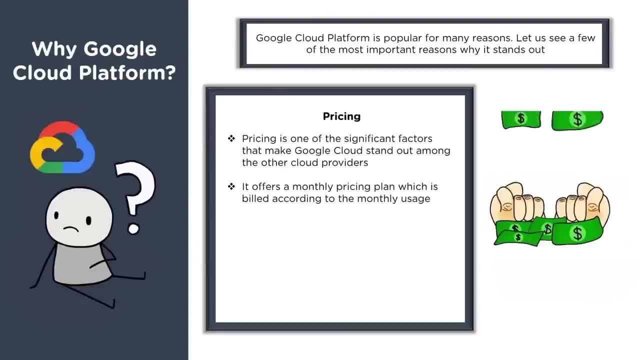 we talk about billing here. the billing can be in hours, it can be in minutes and it can also be in seconds. There are different options when you talk about your pricing, which can be found from your Google Cloud web page. Now, pricing could be based on pre-employment. 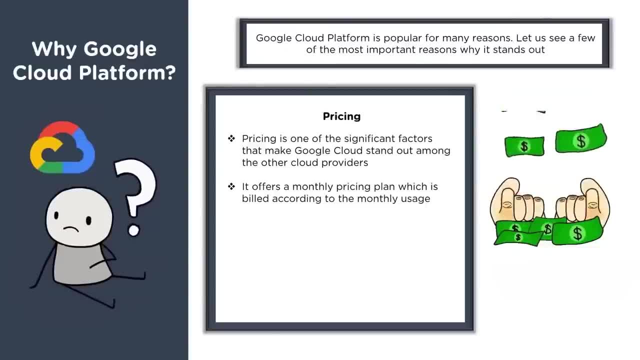 Preemptive machines. pricing could be based on reserved instances or reserved resources. I'll show you the link where you can find more details on pricing part of it. So Google Cloud really has various pricing options which help customers in their different requirements, whether they would go for any of the service models, such as infrastructure. 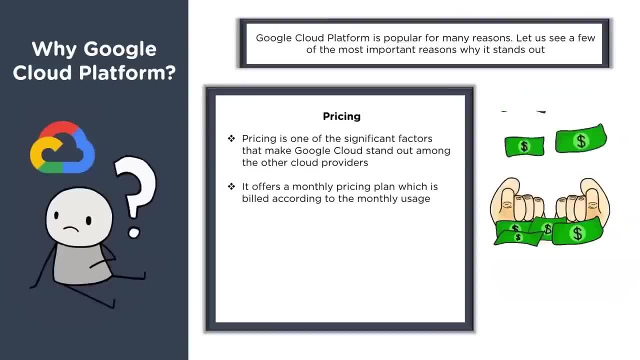 as a service, platform as a service or even software as a service. One more attractive thing About Google Cloud pricing is that it provides committed use discounts. For example, under this scheme you can purchase a specific amount of virtual CPU cores and memory for up to 57% discount off regular prices if you commit usage for either one. 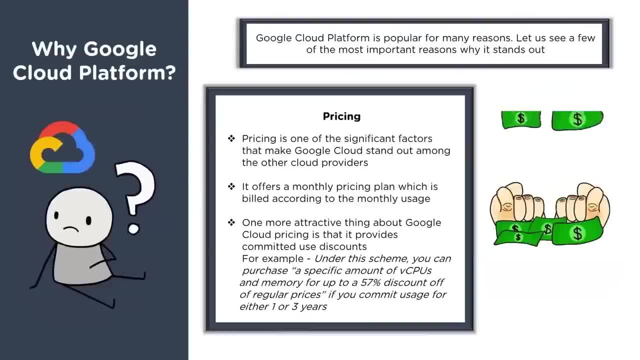 or three years. Now, this is just one option. There are various such options which you can learn about from the Google Cloud's page, and that really suits different customers for their needs. Now let's talk about pricing. Let's talk about pricing. 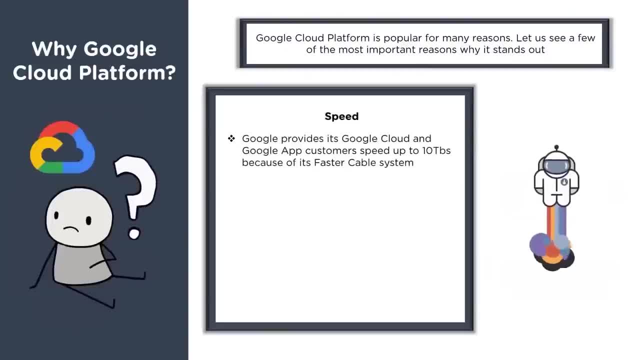 Now, when we talk about cost, we're talking about volume of the app and staging and such. So with Google Cloud, it provides three different options. One is speed. With Google Cloud, it provides speed and schedule. So those are the three different options for you to choose from for your business. 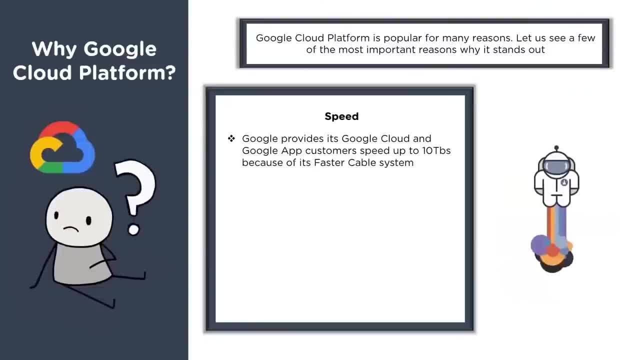 The second option is speed. Now, when we talk about speed, we don't need to really challenge this aspect when it comes to Google services. So Google provides its Google Cloud and Google app customer speed up to 10 terabytes because of its faster cable system. 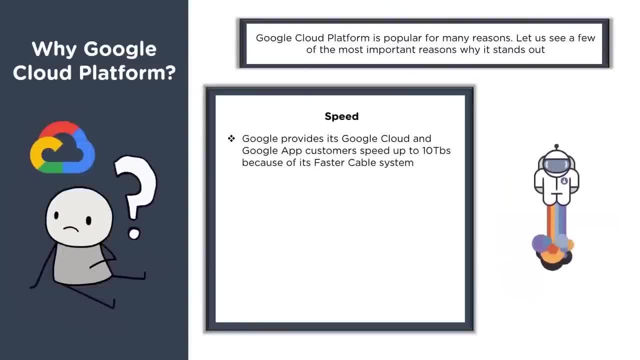 There are different kind of machines which can be used if you're talking about computation, if you're talking about memory-hungry applications or even storage-intensive workloads, So you can take advantage of the different components. It's easy to use. It's easy to use. 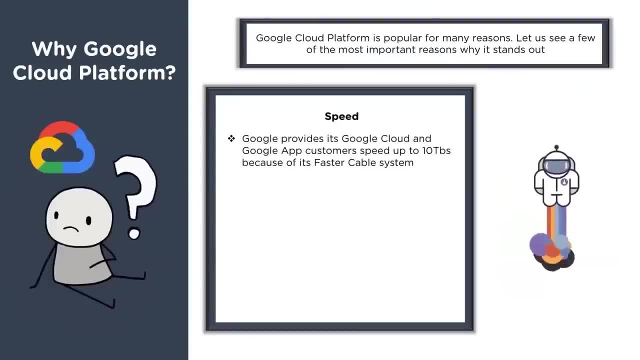 You just have to do a really good job of using Google Cloud workloads. All in all, speed is one of the defining characteristics of Google Cloud services. The cable has connections over US West Coast, main cities in Japan and even major hubs. 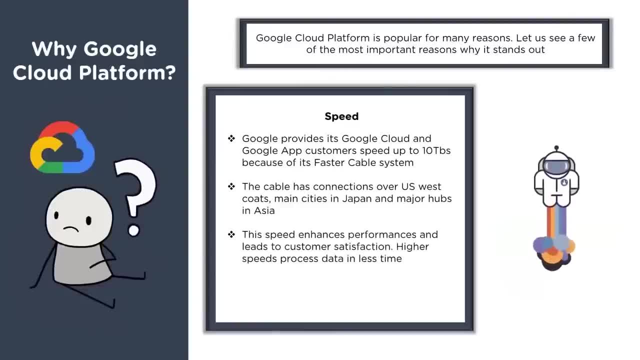 in Asia. This speed enhances performances and leads to customer satisfaction. Now, when we talk about customers, any or every customer would prefer to have low latency, high throughput based services. They would want to use higher speeds to process their data in as less time. 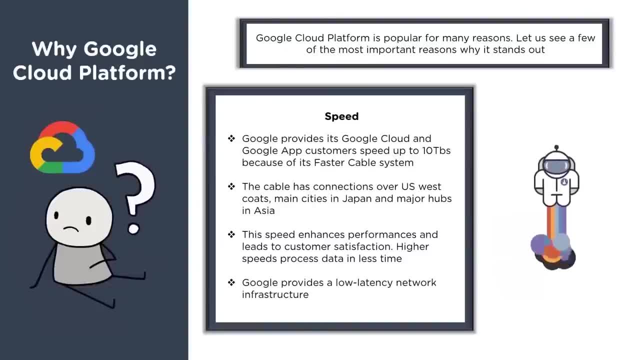 as possible. Google provides a low latency network infrastructure. In fact, you can say that when you are using Google Cloud services, you are using the services from the same infrastructure which Google uses for its popular services, such as Google Search or even YouTube, which. 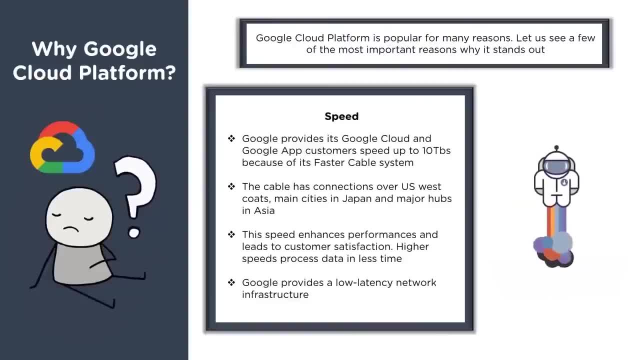 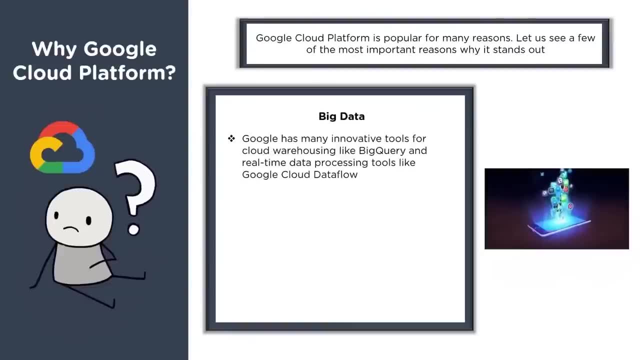 is one of the second largest services, just repository- which can be accessed for videos. Now, when we talk about big data, big data is data which is very complex, has a lot of other characteristics, such as your volume, you have velocity, you have variety, you have veracity, validity, volatility, virality and so on. So if 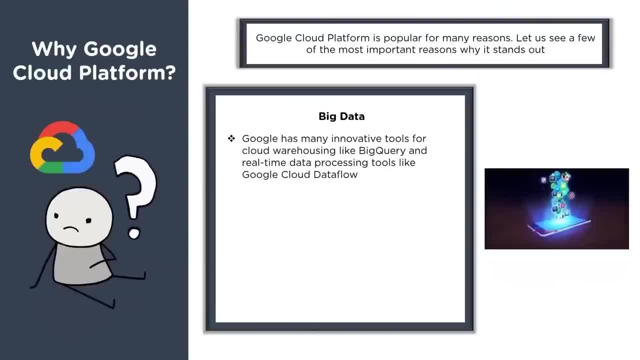 an organization is working on big data, Google Cloud can be a better choice, because Google has many innovative tools for cloud warehousing, for example, such as BigQuery, and even real-time data processing tools such as Dataflow. BigQuery is a data warehouse that allows massive processing of 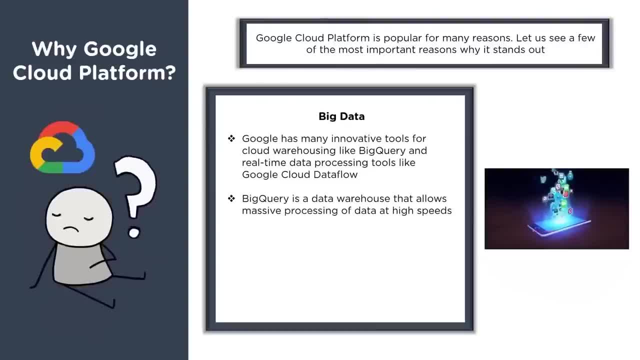 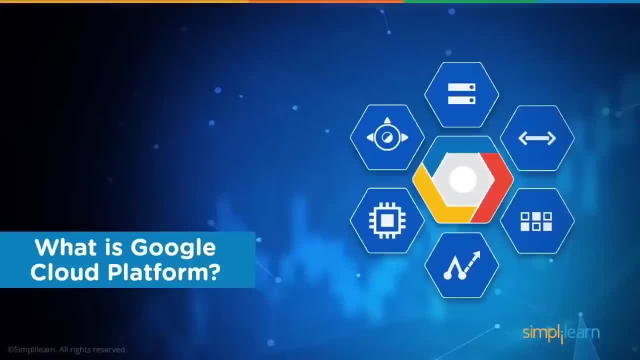 data at high speeds, basically working on your structured data. Google also has launched some new machine learning from Google Cloud. Google Cloud is a data warehouse that allows massive processing of data from artificial intelligence tools. Now there are various other services which we can, which we can use from Google Cloud platform. but let's understand what is Google Cloud platform. 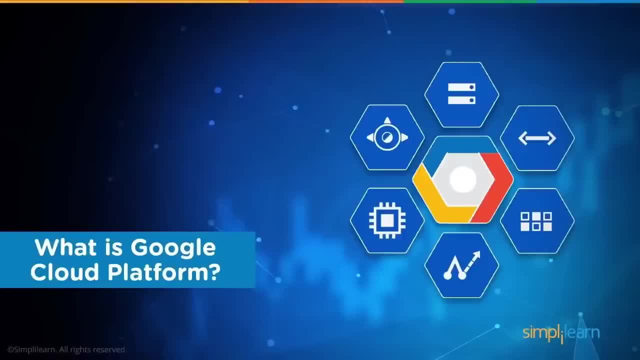 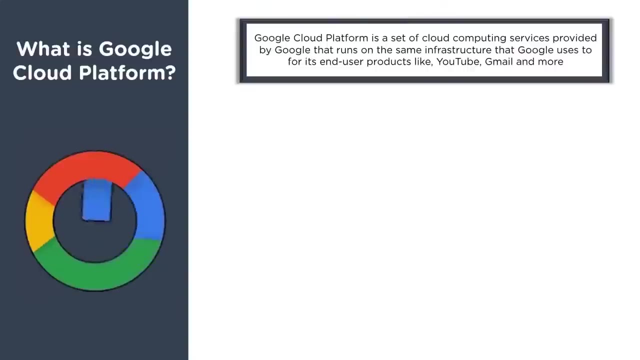 and what are some of the services? Even the services which are not listed here can be found in your console from Google Cloud. So what is Google Cloud platform? GCP? It is a set of cloud computing services provided by Google that runs on the same infrastructure, as I mentioned. 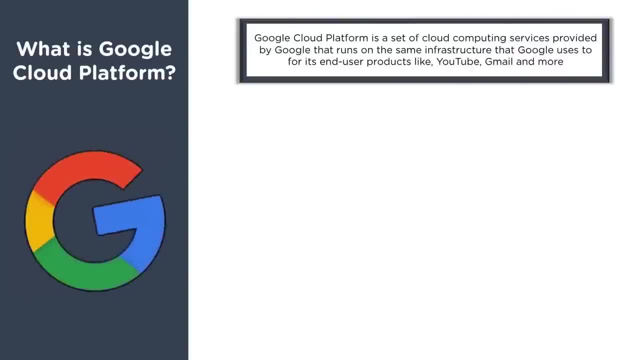 That Google uses for its end-user products like YouTube, Gmail and even Google Search. The various set of services offered by Google Cloud platform are. so you have services which are specific to computing requirements and again, in computing, you have various different options available. You have machines which are compute optimized machines which are memory optimized machines. 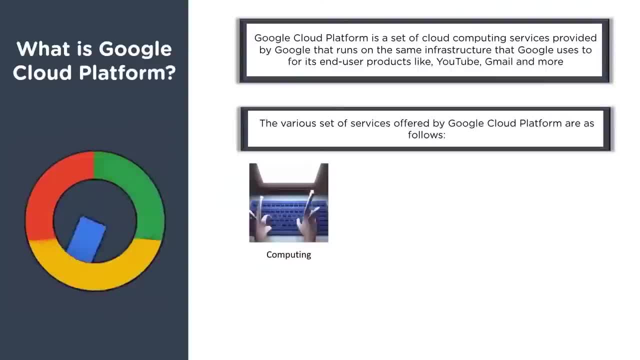 which are storage optimized, and also we have certain machines such as pre-emptive, which basically means that you could get a machine to work on at a far lesser price than any other machine. But when we talk about pre-emptive, these are the machines which can be requested on demand, and 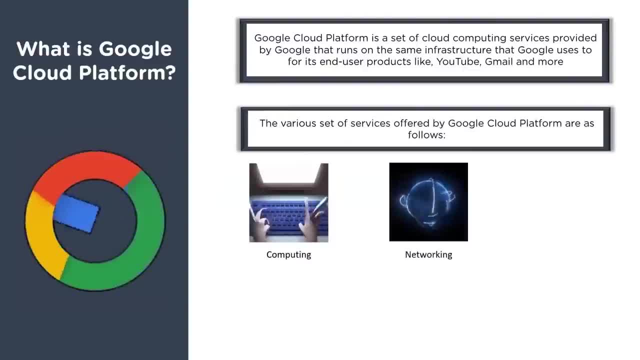 they can be taken back by Google at any time. You have networking related services, which can be very useful when you are working on a project. You have the ability to work on a project, that is, when you are setting up your applications or your services across globe. You also have different 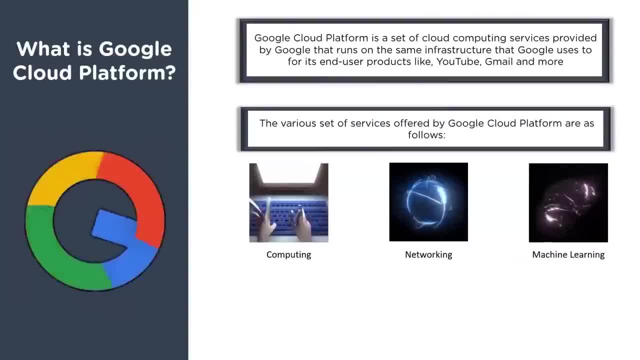 services which are specific to machine learning, and organizations which would be interested in working on machine learning or artificial intelligence would be really interested in using these services. There are also innovative solutions to work on big data and big data related technologies. Now when we talk about Google Cloud platform domain. 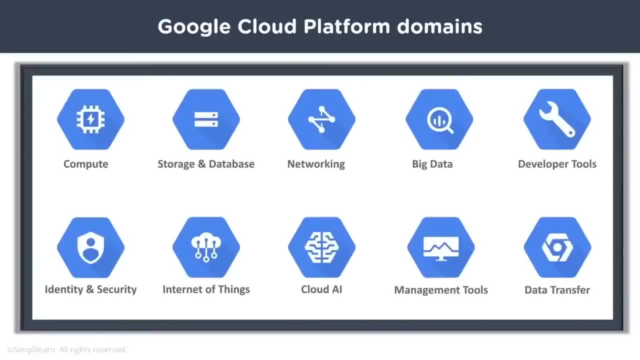 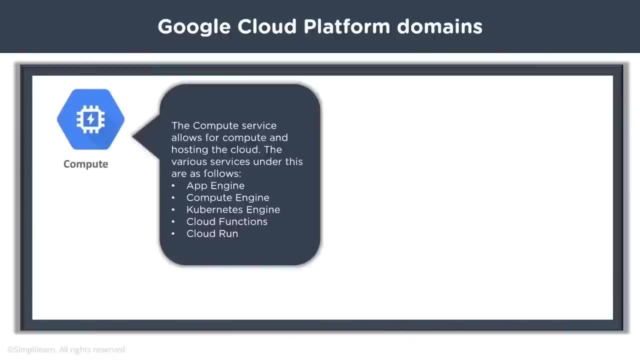 so we can break down these services into specifics, such as: you have compute. Now the compute service allows for computing and hosting the cloud. Now, when you talk about computing here, there are different services, such as App Engine. you have Compute Engine. you have Kubernetes, you have 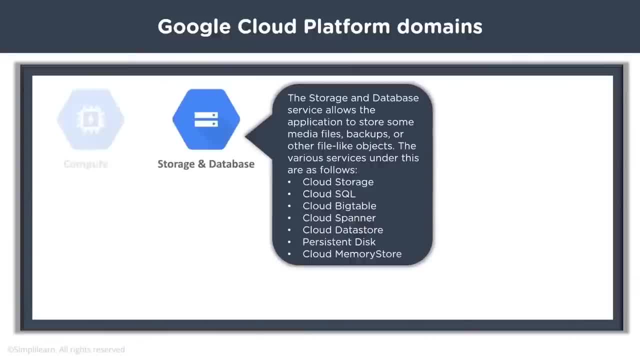 Cloud Functions and Cloud Run When you talk about storage and database. so the storage and database service allows application to store media files, backups or other file-like objects. Now, various services under this are as follows. You have Cloud Storage, Cloud SQL, Cloud, Bigtable for unstructured 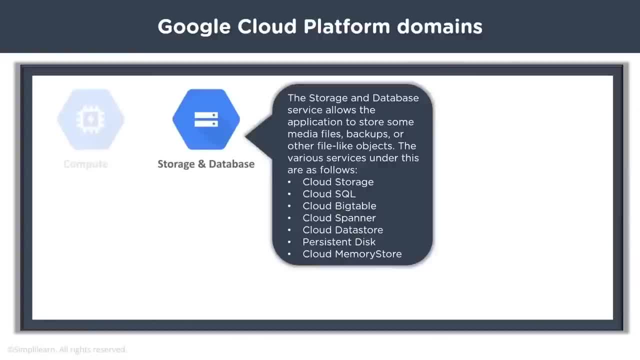 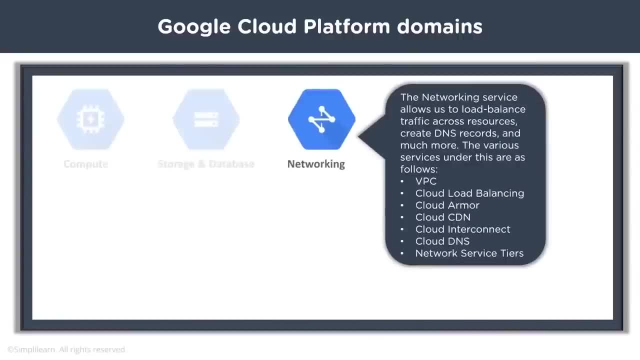 data. You have Cloud Spanner, Cloud Datastore, Persistent Disks and Cloud Memory Store. When we talk about networking, the networking service allows us to load balance traffic across resources. Now, as I said, you can also use the cloud storage service to store data. You can also use the cloud. 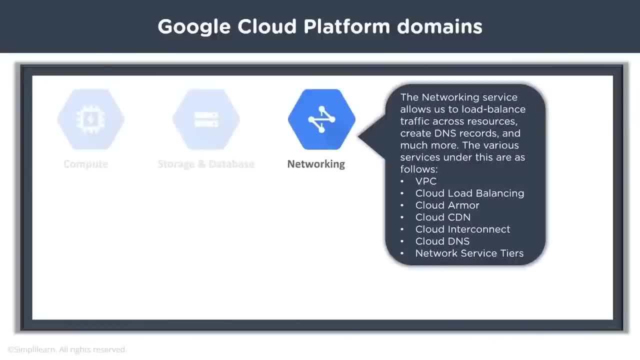 storage service to store data. Now are some others services, as I mentioned earlier. resources could be your different resources which you would be using from a cloud platform, such as your devices, your instances, memory optimized or CPU optimized instances, or other resources creating DNS records. 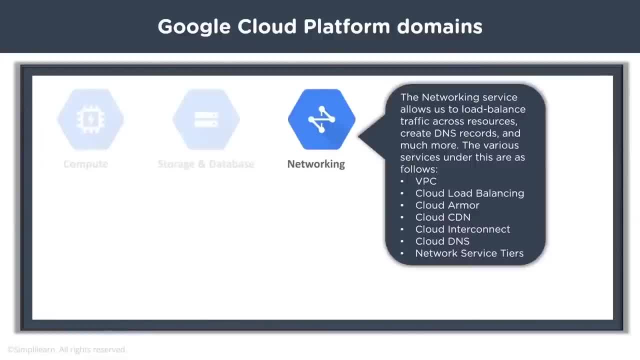 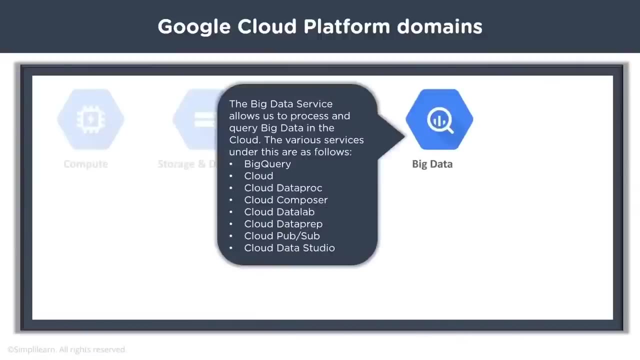 and much more So. various services under this are VPC- that stands for virtual private cloud. You have Cloud Load Balancing, Cloud Armor, Cloud CDN. You have Cloud Internet. you have Cloud interconnect, DNS and network service tiers. When we talk about the big data service, 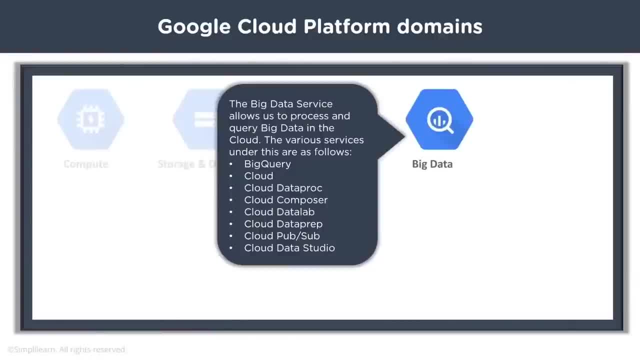 this allows us to process and query big data in cloud. Now, various services under these are as follows. You have BigQuery Cloud Cloud Dataproc Cloud, Composer Cloud, Datalab Cloud, Dataprep, Cloud, PubSub, which is publish and subscribing system. 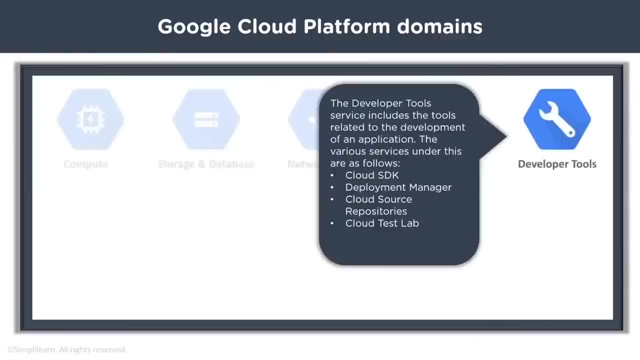 You have Cloud Data Studio. Now you also have the developer tools, and developer tools service includes tools related to development of an application. Now, various services under these are as follows. That is, you have Cloud SDK, Software Development Kit, You have Deployment Manager. 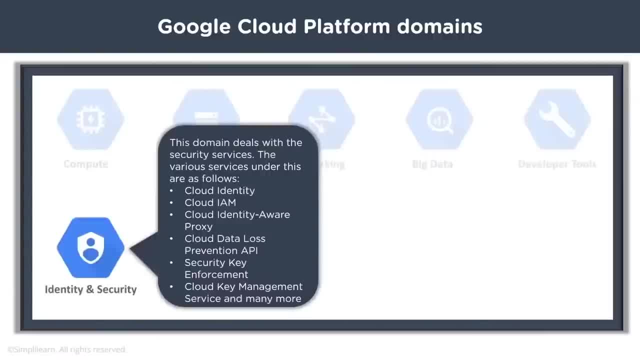 Cloud Source Repositories and Cloud Test Lab. When we talk about identity and security, which is one of the primary concerns for any organization or any user who would be interested in using a cloud platform, Google Cloud really has taken care of this. So, when you talk about identity and security domain, 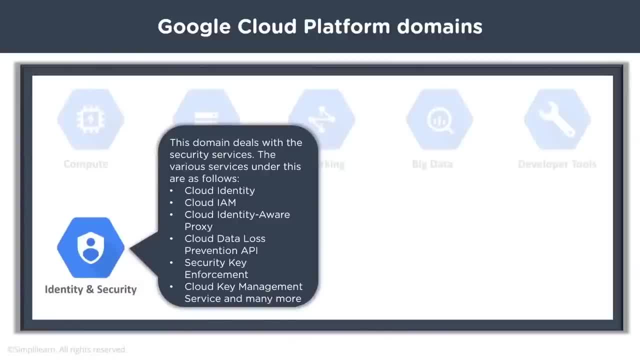 this deals with security services. Now. various services here are Cloud Identity- You have Identity and Access Management, that is Cloud IAM. You have Identity Aware Proxies. You have Cloud Data Loss Prevention, API, Security, Key Enforcement, Key Management Service and many more. 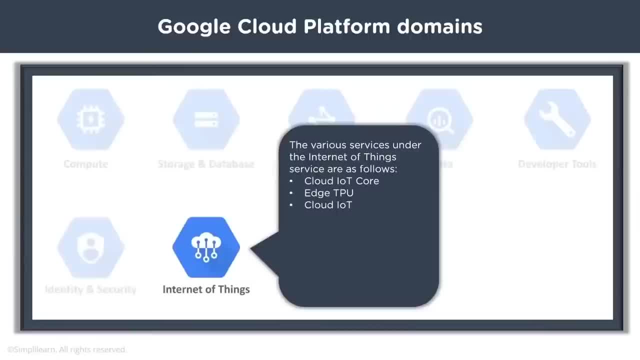 You also have Cloud Services which are related to Internet of Things, So very much would be used by organizations who would be working on IoT devices or the data generated by these devices. So various services here are Cloud IoT Core. You have Edge, TPU and Cloud IoT. 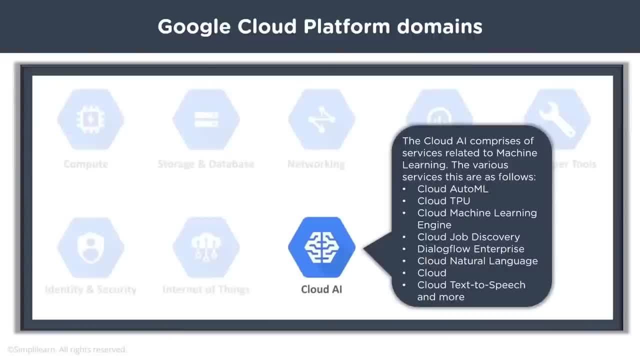 Also when we talk about Cloud AI, that is, Artificial Intelligence. this comprises of services related to machine learning and much more, So you have Cloud, AutoML, Cloud, TPU, Cloud, Machine Learning Engine, Job Discovery, Dialogflow, Enterprise, Natural Language Cloud. 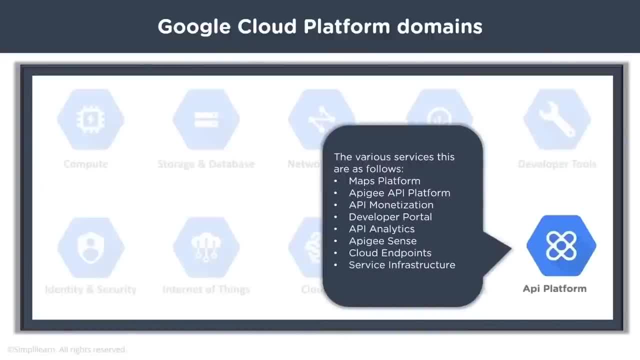 Text-to-Speech and much more. If you would be interested in services related to API platform, then there are different services under this category or this domain. So you have Maps Platform, you have APG API Platform, Monetization, developer portal. 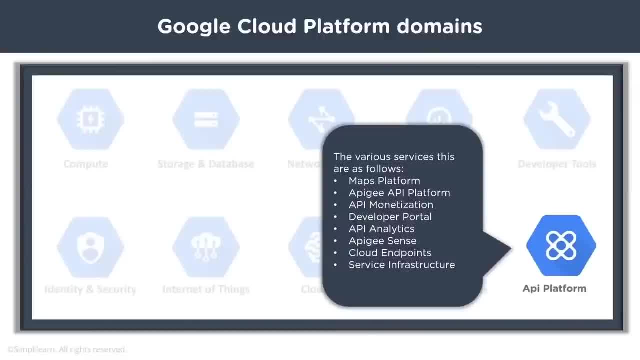 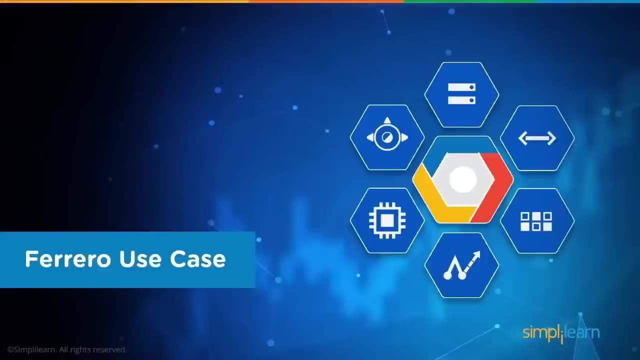 Analytics, that is, API Analytics, analytics, APG sense, cloud endpoints and service infrastructure. So these are some of the listing of services under each cloud platform domain. Now let's look at Ferrero use case and let's also understand what was done here. 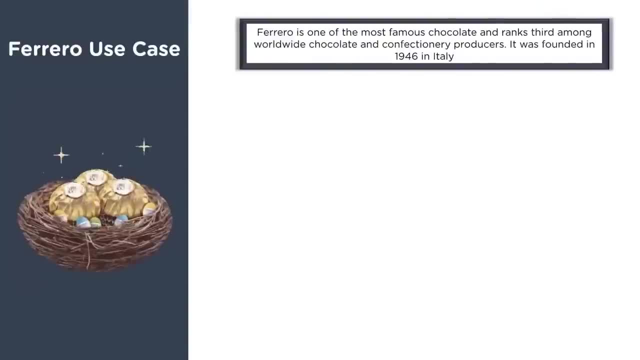 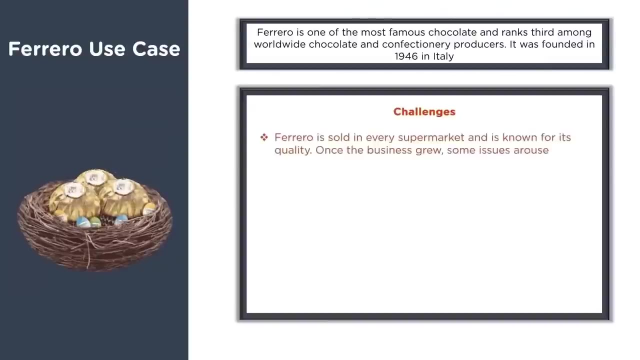 So Ferrero is one of the famous chocolate and ranks third among worldwide chocolate and confectionery producers. It was found in 1946 in Italy. I'm sure you would have seen the Ferrero chocolates when you would have gone out to buy some chocolates. 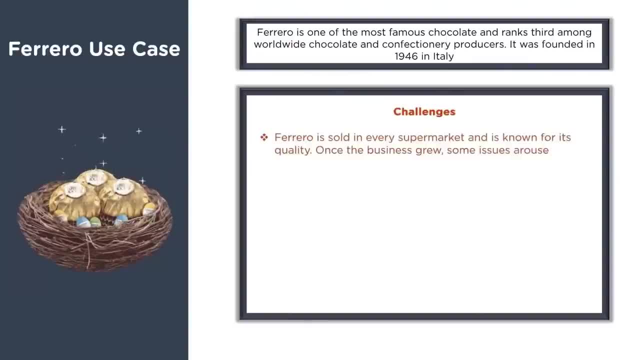 So the challenges here was that Ferrero, as we know, is sold in every supermarket and is known for its quality. Once the business grew, some issues arose. right, and that's what happens when the business grows. you have issues popping up which could be related to the volume of data, the speed, 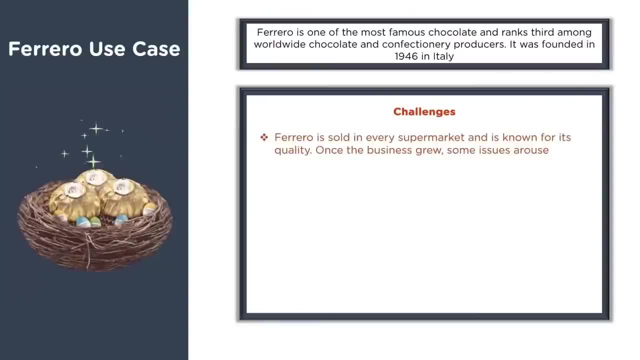 with which the data is getting generated, the variety of data, and also looking at your platforms, which support different dynamic applications, or your scalability requirements, performance requirements and so on. So it needed data storage, processing and analysis system for a wide customer database. There was a huge gap between the company and the people who bought its goods, because the 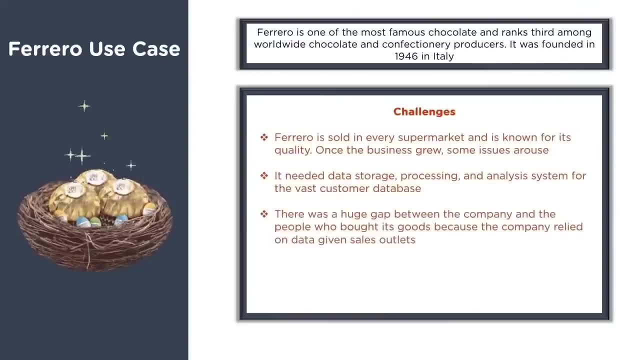 company relied on data given sales outlets. Now that's why Ferrero is so popular. So let's look at Ferrero. One of the challenge Ferrero wanted to create a digital ecosystem where there was a point of contact with its customers and also a foundation for an innovative data driven marketing strategy. 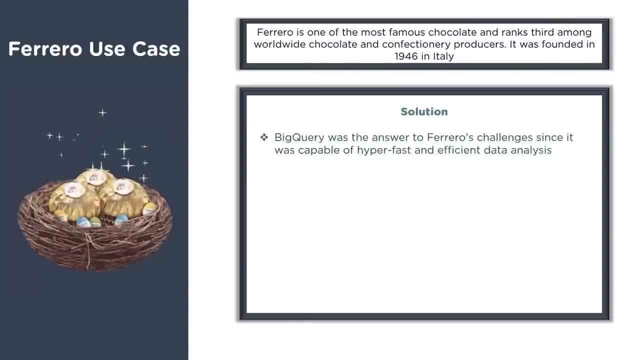 What was the solution here? So, one of the service of cloud platforms, or Google Cloud Platform, is BigQuery, and this was an answer to Ferrero's challenges, since it was capable of hyper fast and efficient data analysis. as a solution Now, as I mentioned, BigQuery is a data warehouse which allows you to store structured data. 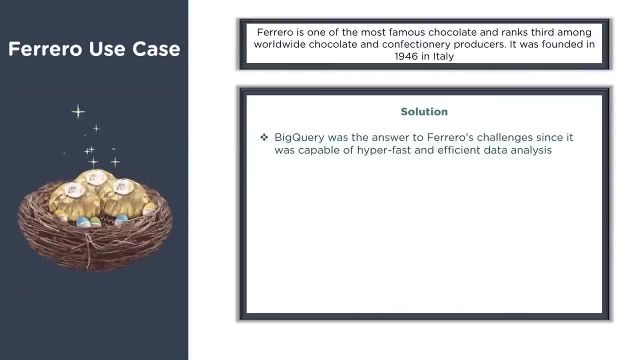 Now this could directly be used as a service where you could store in any amount of data and you would not be paying for storage. So there are different pricing models and for data up to 1 terabytes you would not be charged anything And if you would be accessing data, 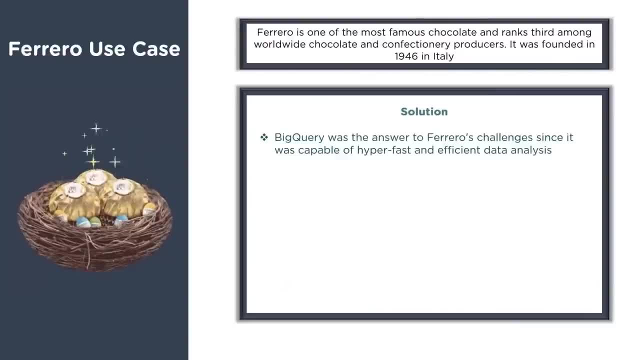 So there are different pricing models and for data up to 1 terabytes you would not be charging anything. So there are different pricing models and for data up to 1 terabytes you would not be charged anything. And if you would be accessing the data, that is, reading the data or processing the data. 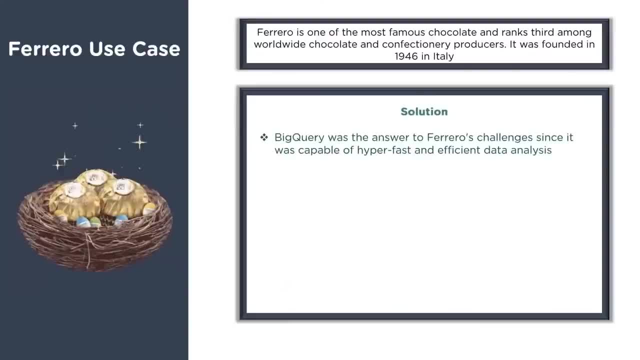 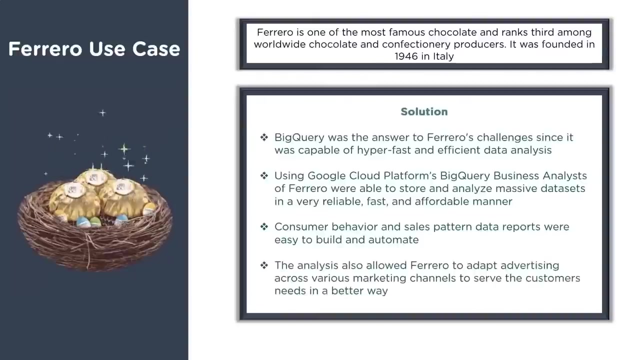 from BigQuery. that's where the pricing model kicks in Now. using Google Cloud's BigQuery, business analysts of Ferrero were able to store and analyze massive datasets in a very reliable, fast and affordable manner. Consumer behavior and sales pattern data reports were easy to build and automate, and the analysis 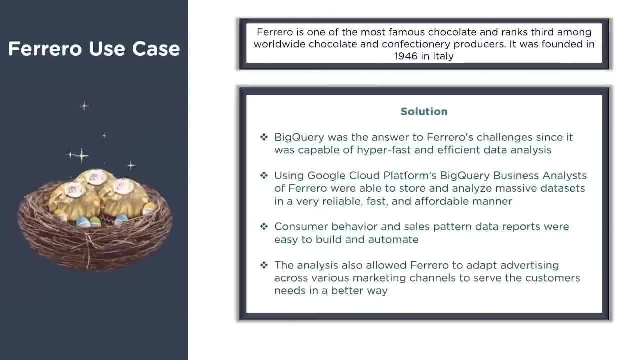 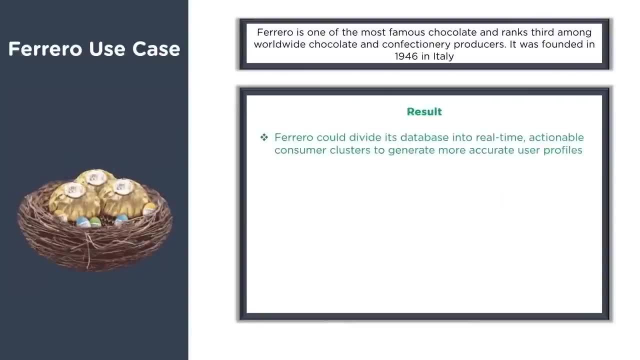 also followed Ferrero's data analytics followed Ferrero to adopt advertising across various marketing channels to serve the customer needs in a better way. What was the result? They could divide their database into real-time actionable consumer clusters to generate more accurate user profiles. Ferrero was also able. 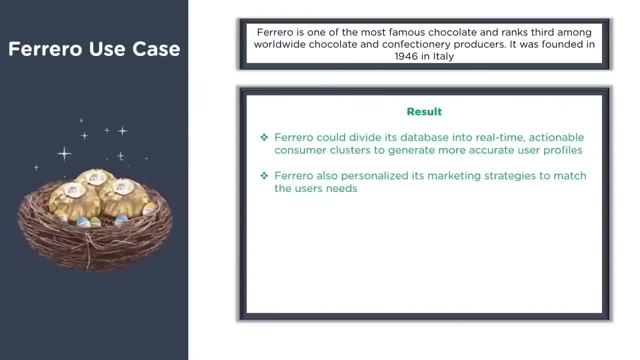 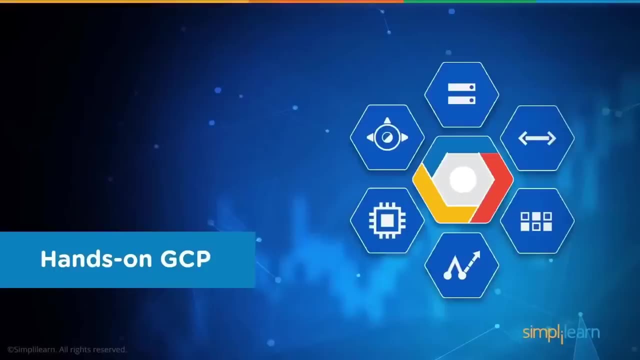 to personalize its marketing strategies to match the user needs. Now Google Cloud Platform completely tailored the website, mobile content and advertising, and created a very cost-effective media buy strategy. Now, these were some basics on Google Cloud. Now, as I said, you can always. 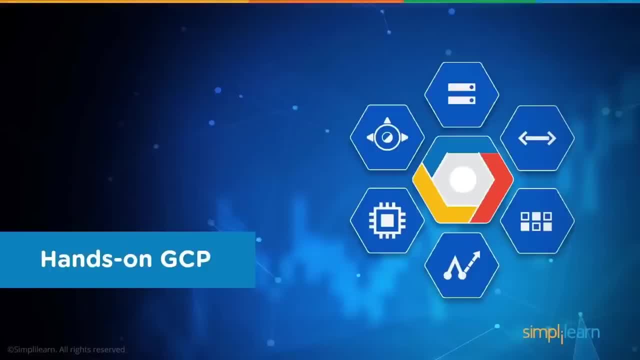 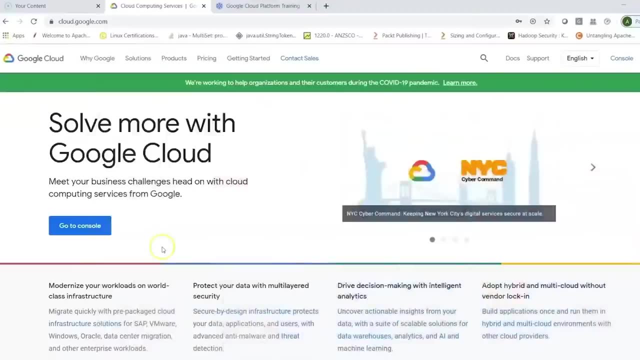 find a lot of details about pricing, about services, and also all the services are accessible in your free trial account. Now let me just walk you through here. So one is: you could always find details on documentation. Now let me just walk you through here. So one is: you could always find. 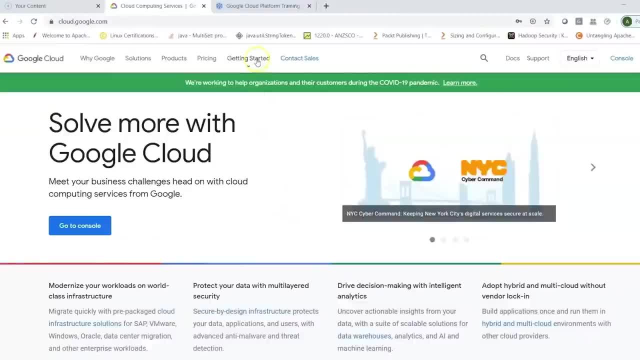 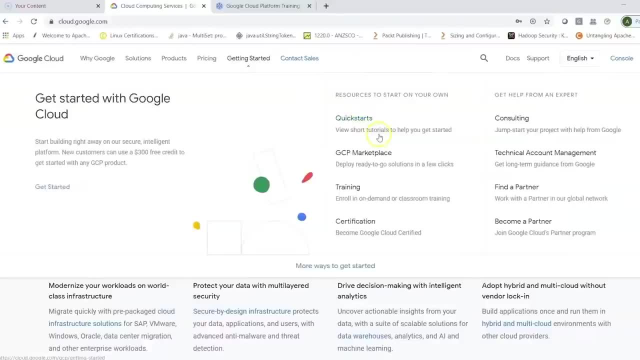 details on documentation. Now let me just walk you through here. So one is, you could always find documentation on each of these services. So if I would click on getting started, you have quick start, which basically shows you short tutorials. You have trainings and you have 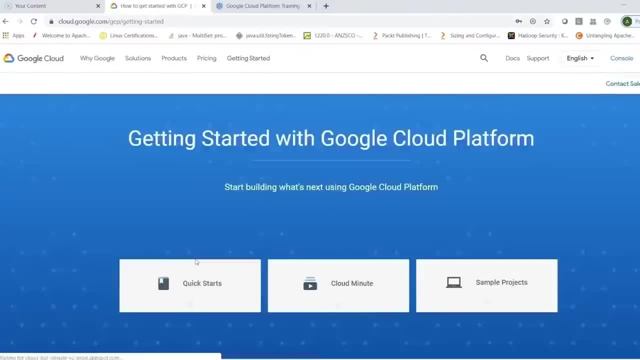 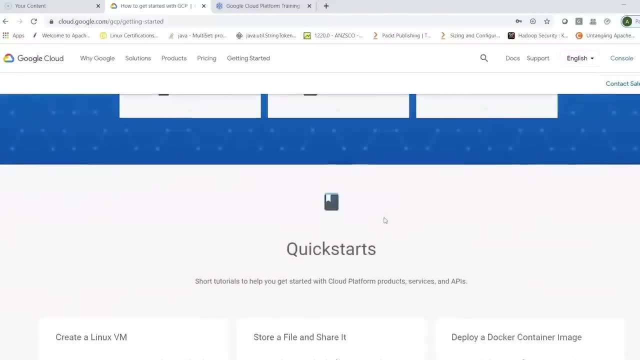 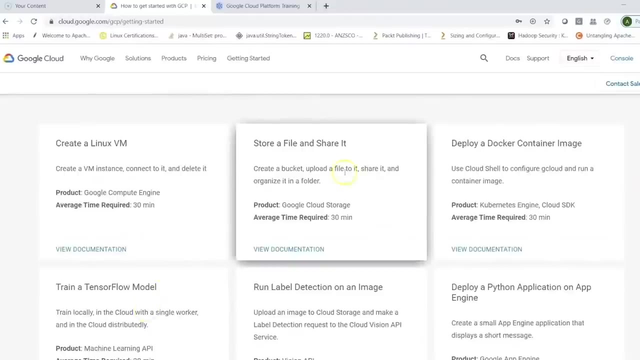 also certifications. Now, if we click on quick start- now that takes me to this page which shows me quick starts- or if you would want to understand about different projects, if you would want to look into the documentation of creating a Linux virtual machine. 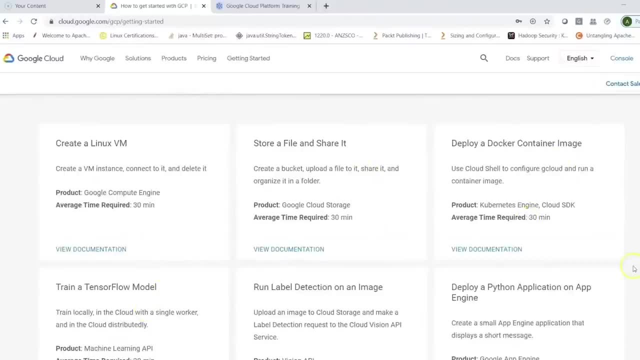 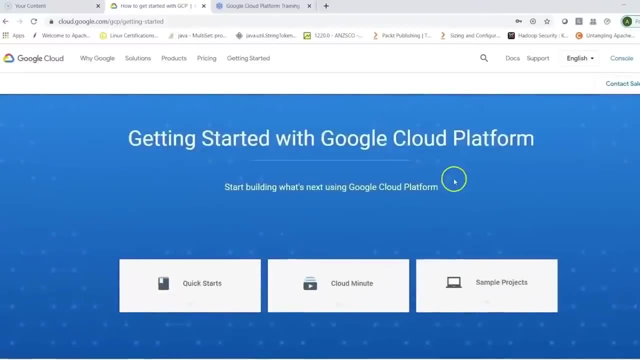 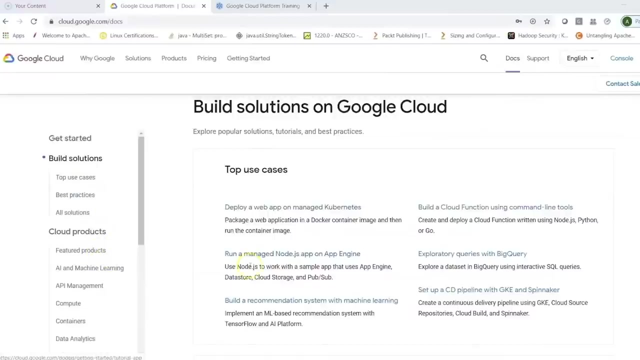 or storing a file and sharing it, deploying a container, Docker, container image and so on. So you have a lot of quick starts here. You can also look at Cloud Minute. On the same page, on the right side, you have Docs, and once you click on that it takes you to these links Now. 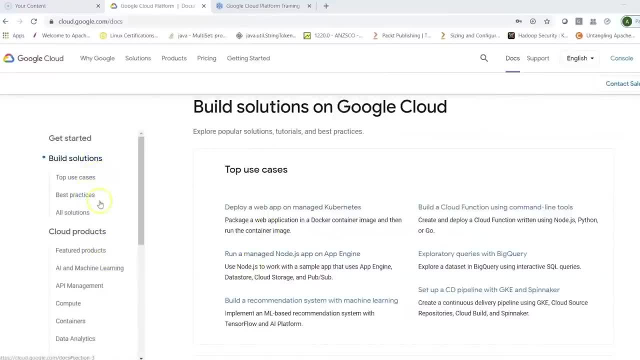 this shows you build solutions, which shows you top use cases, best practices, all the solutions. It's always good to learn from these use cases which are available And here you can see you have different featured products and all the different services which Google Cloud offers. 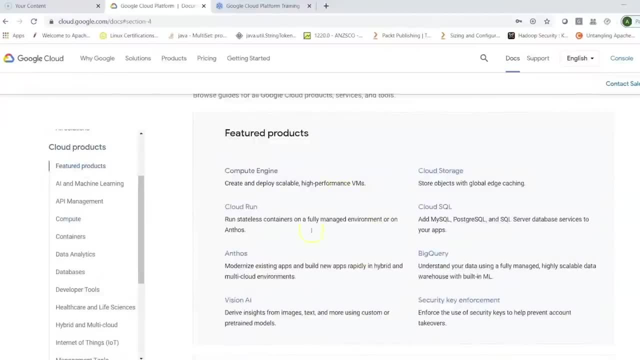 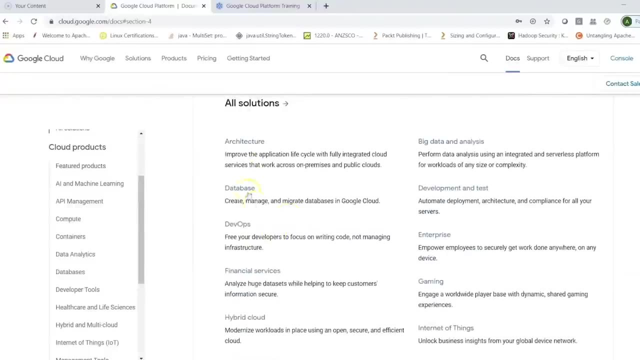 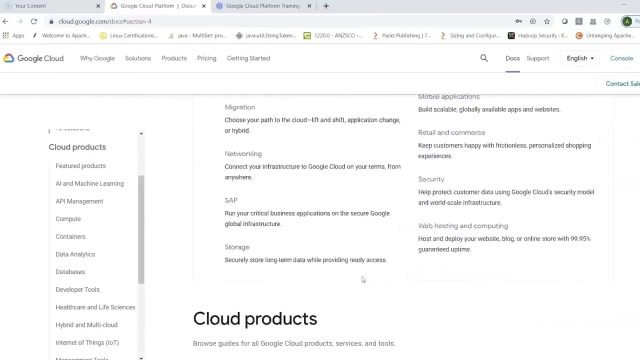 Now you can click on featured products and that basically shows you a list of these products. Now here we have all the solutions which you can look at: architecture, database, enterprise level, big data and analysis, gaming related, internet of things, and so on. Now, if you go down here, 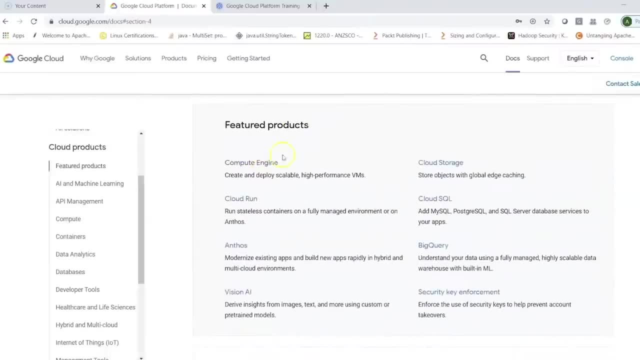 it shows you featured products and that shows you some of the important products, such as compute engine, which is belonging to the compute domain. you have cloud run. you have anthers, which is for migration, and basically cloud adoption, when organizations would want to move from on-premise to cloud-based solutions. 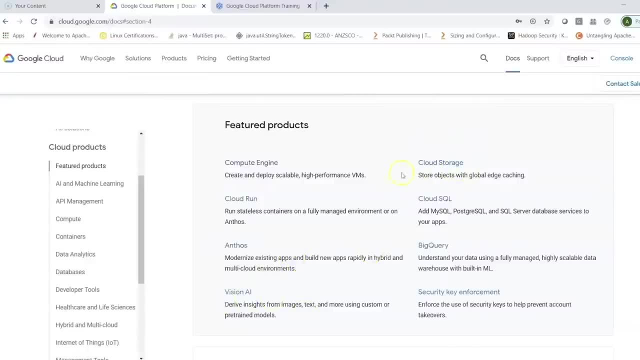 you have vision AI. you have cloud storage now. that basically allows you to store any kind of data, whether that's an object. so this is acting as an object storage. you have cloud SQL, which is basically a ready-to-use service where you would be using MySQL, Postgres or any other SQL Server database services. you 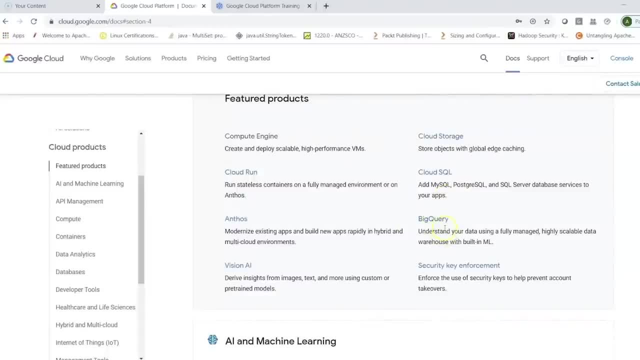 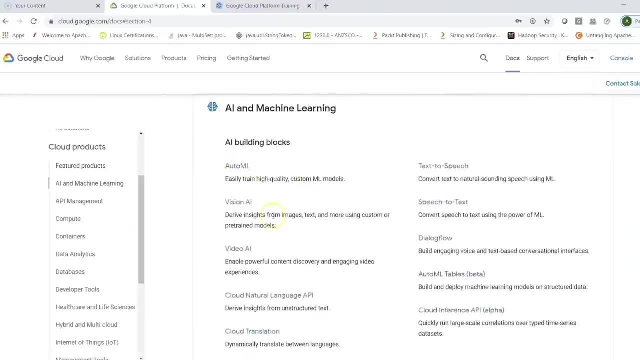 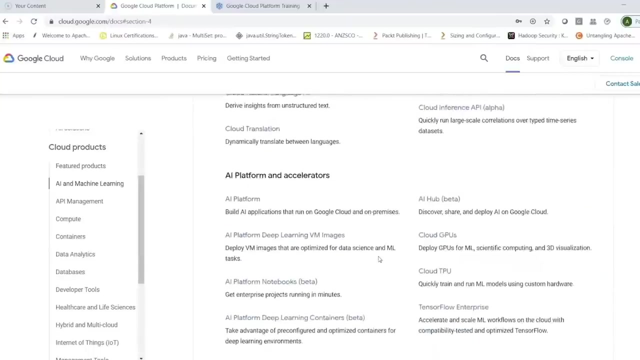 have big query, which is a data warehouse which basically allows you to store your structured data, and then you have your AI and machine learning related products. so you have AutoML, vision, AI, video, AI, text-to-speech, speech-to-text and so on. now you also have different. 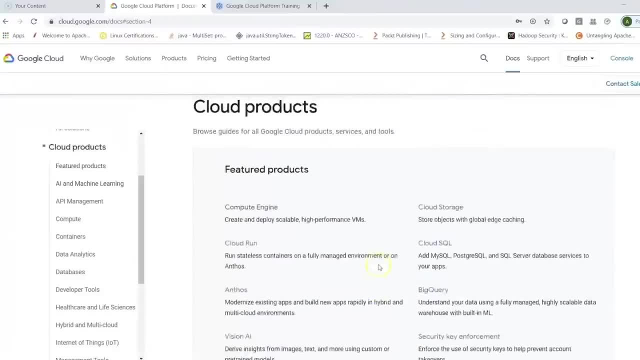 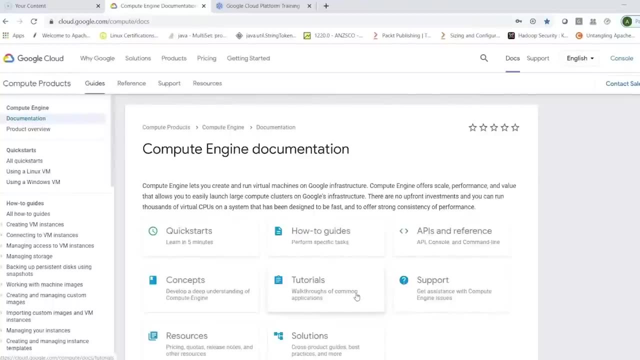 platform accelerators which can be used and in any of these cases, for example, if I would click on compute engine, which is a featured product from Google Cloud, now that shows you basically your quick starts using your Linux machines. how-to guides, which tells you completely working on a VM instance or working on 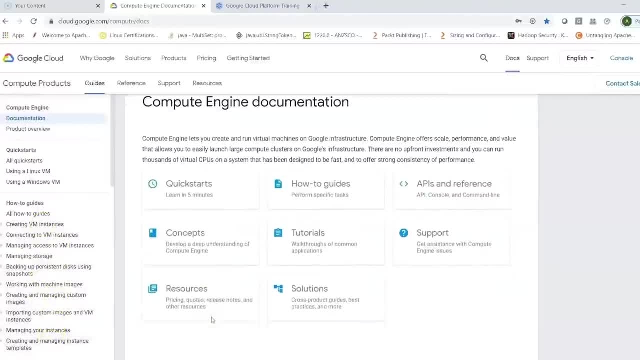 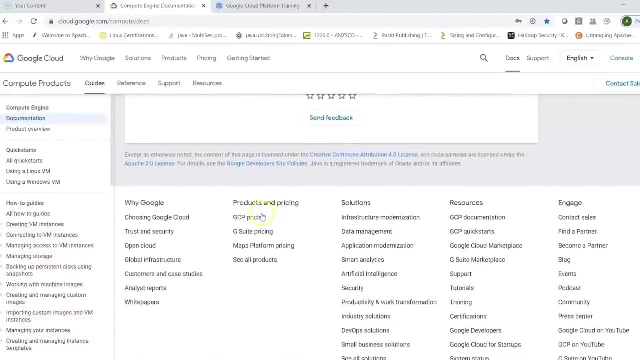 storage, working on persistent disks and so on, and it shows you the documentation here. now you also have products and pricing option which you can see for GCB pricing and you could straight away go to the pricing. you could be looking at solutions which talks about infrastructure modernization. now this is 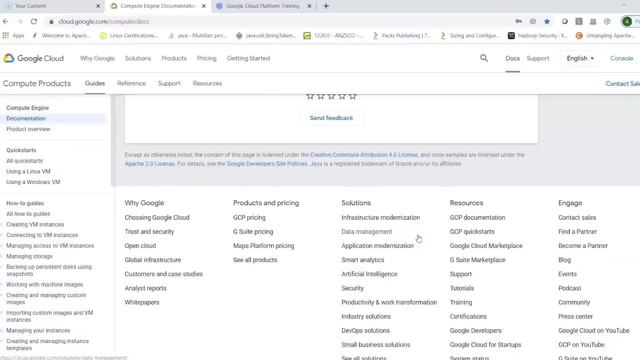 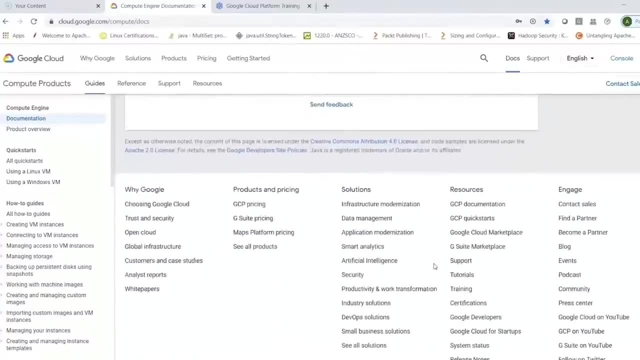 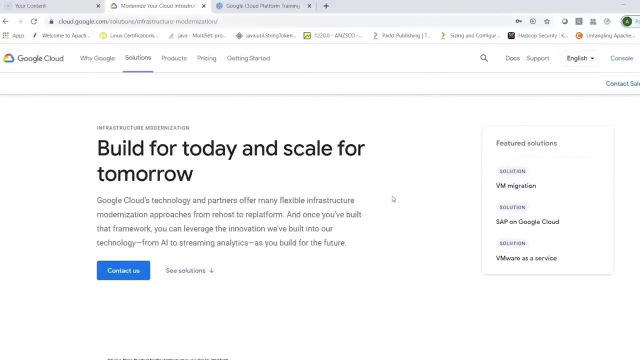 something which organizations are interested in when they would want to move from their on-premise solution to your Google Cloud. now, here I can say, for example, I click on infrastructure modernization, you can always find some case studies. what are the different solutions you we have here, right when you talk about? 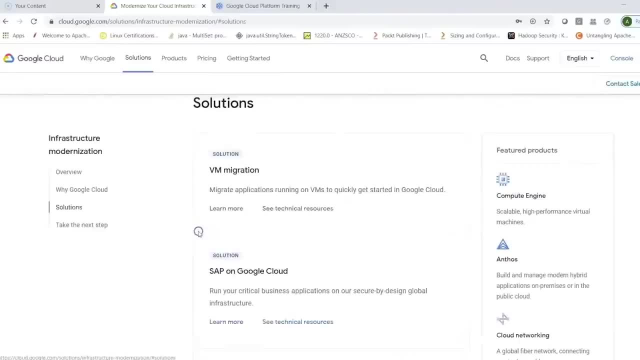 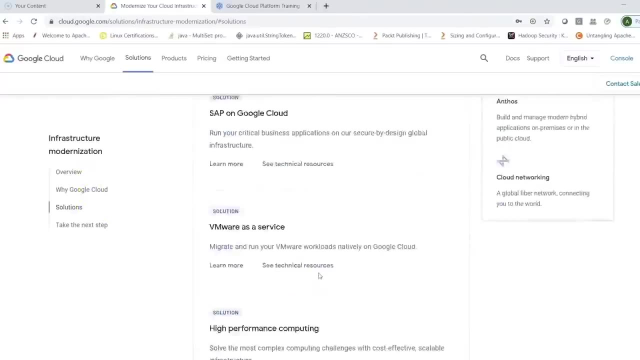 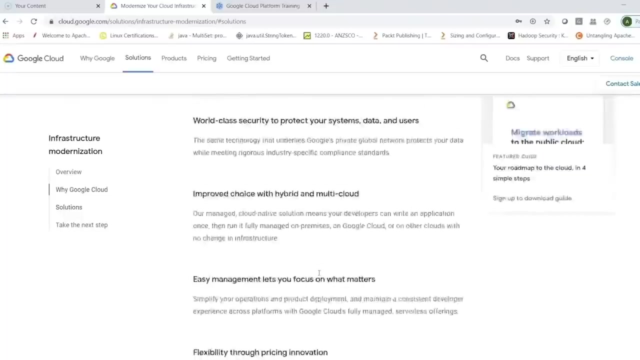 Google Cloud so you can always click on see solutions and you can look at VM migration or SAP cloud right by Google Cloud, what it can be used for- VMware as a service or HPC, that is, high-performance computing- and about these services we will learn in detail later. now I can go back on the same page. 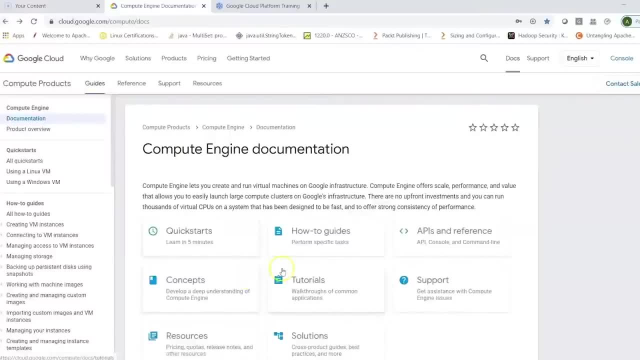 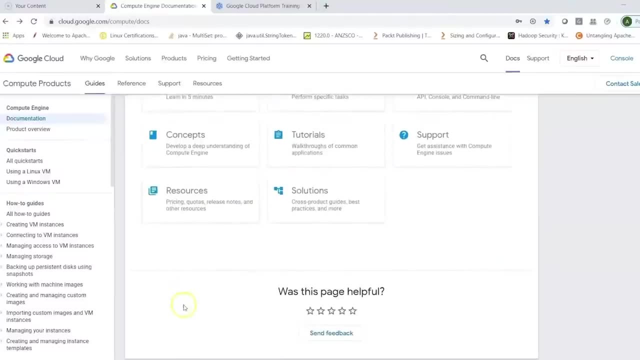 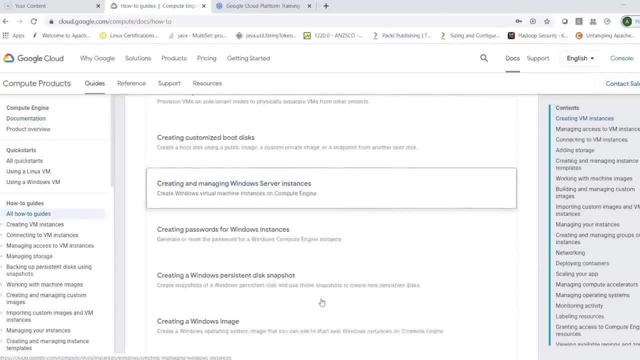 where I was clicking on the services. so you have quick starts, you have how to guides, you have deep understanding of different concepts, right, and here, if I click on all how to guides, so that shows me what are the different ways in which you can work with compute engine and working. 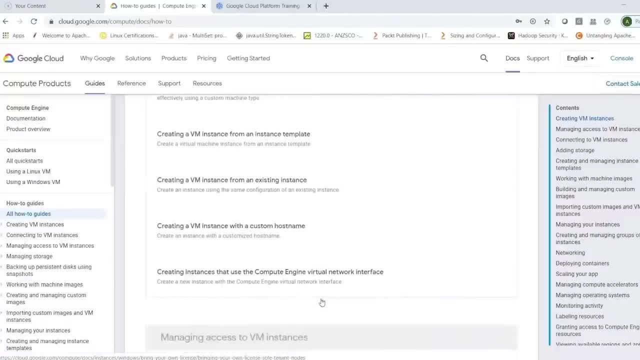 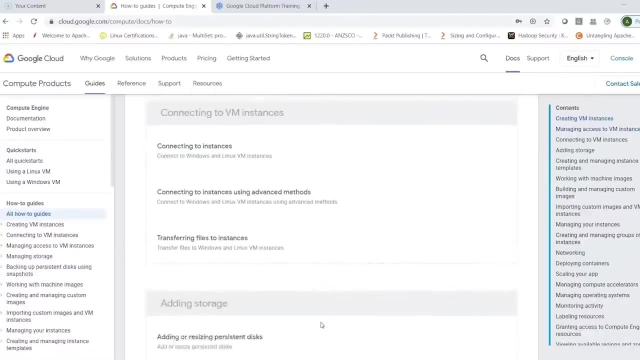 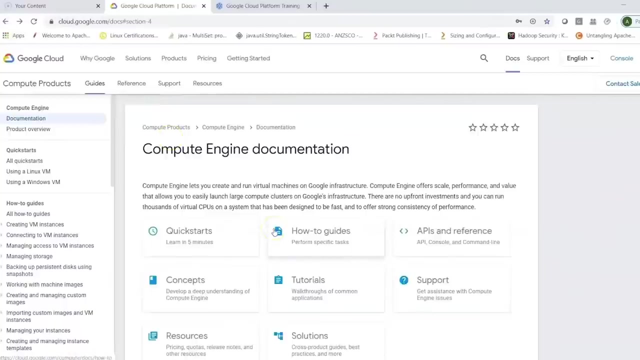 with different instances, although it's quite exhaustive content, but then if you follow steadily, then you can learn a lot about Google Cloud. now here I can just go back, so this is just the way it works here, so you can see that the process is. This is just giving you some idea on the different products which are available from Google Cloud. 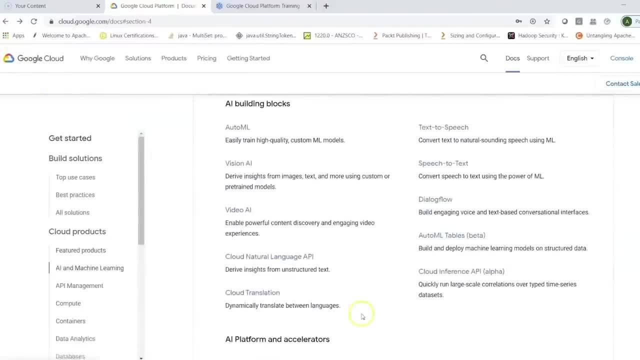 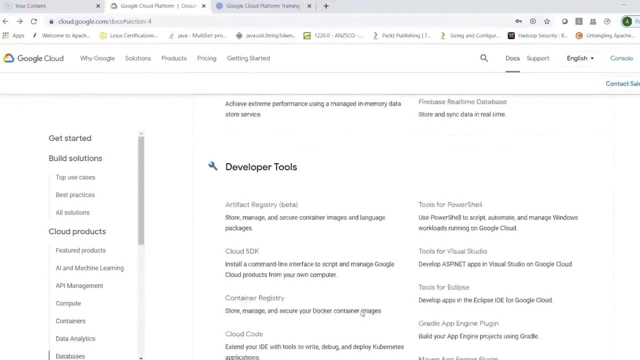 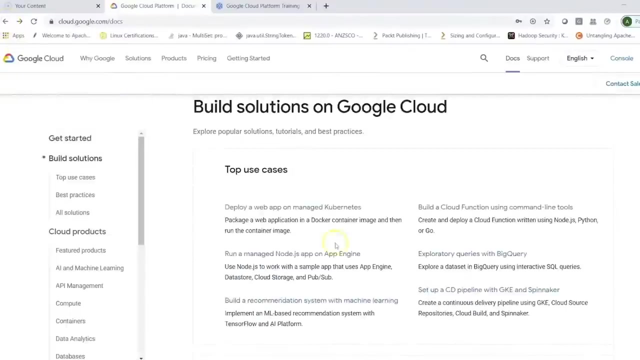 looking into different sections, finding documentation here, and you can always look into each one of these in detail for each product which Google Cloud offers. Now, if we scroll down, we could see all the options or all the domains which we see here. Let me just go back, because we got into Solutions. 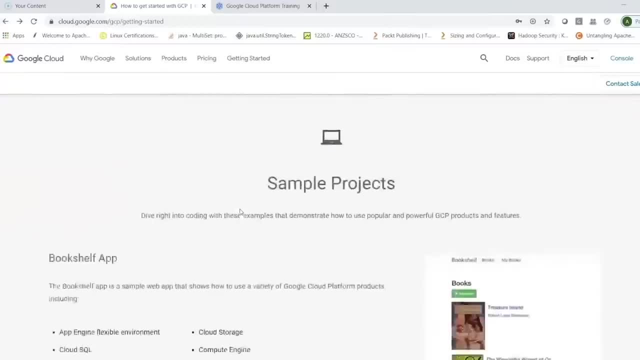 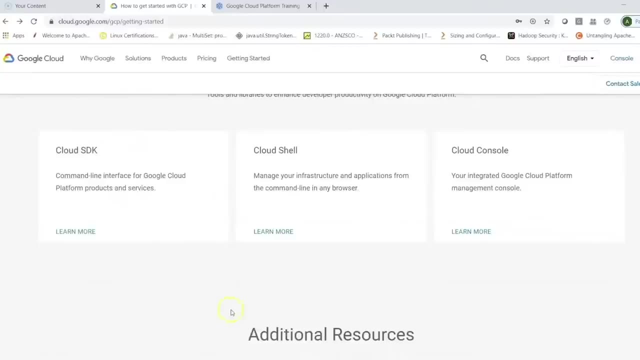 Now we have Quick Starts right, And then you can basically scroll all the way down to look at Cloud SDK, which can be set up on your Windows machine, like I have set it up on my Windows machine. Plus, when you use Google Console, you have a GUI which I'll show you in a couple of minutes. 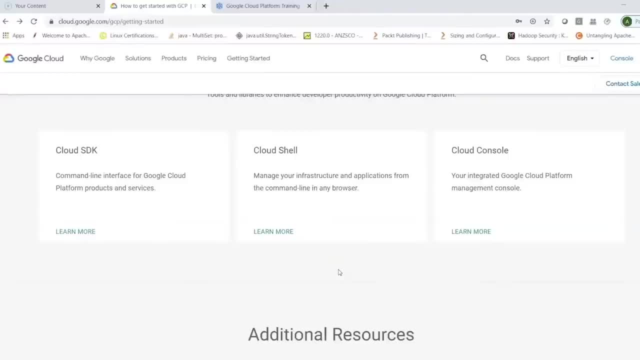 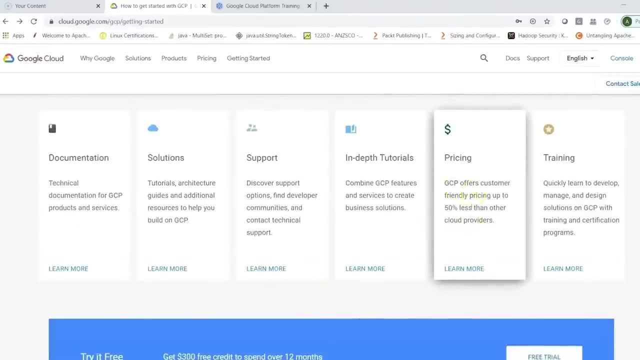 and also a Cloud Shell where you can use your command line options to work with Google. You have Google Cloud Platform. you have Cloud Console, which is nothing but your GUI to access your resources. Now you can also look at in-depth tutorials, pricing, and you have different other options. 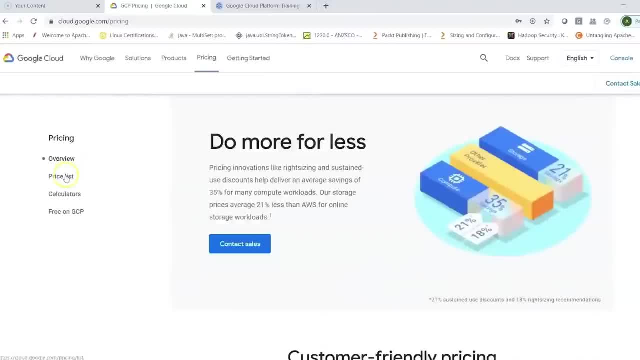 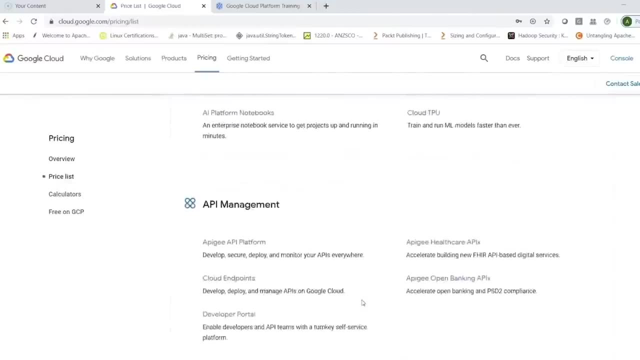 So let's just click on pricing here and then we have your price list, which basically gives you details of different services: what are available and what are the services or what are the prices. So, for example, if I click on Compute Engine- right, 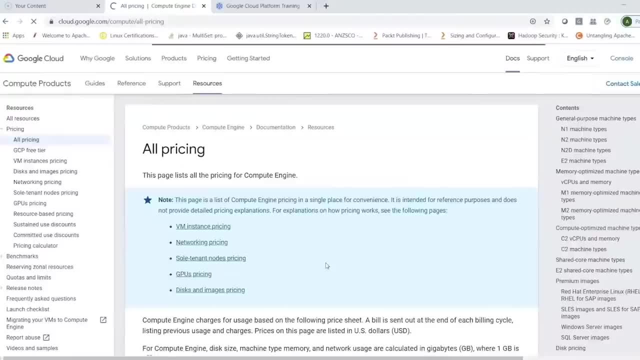 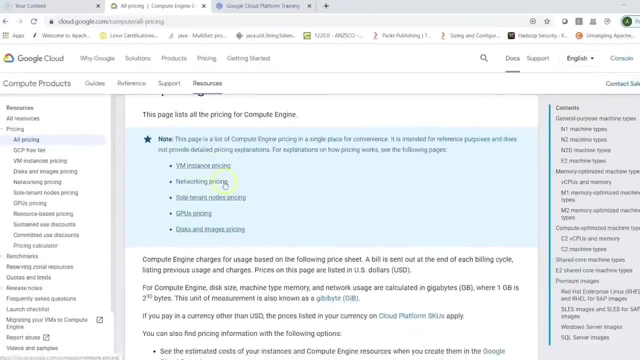 And this shows me the pricing aspect of Compute Engine, which belongs to Compute Domain, and here you can see: you have VM instance pricing, you have networking pricing, sole tenant nodes which are specific to particular organizations or if organizations would want to have dedicated nodes, you have GPU based pricing right. 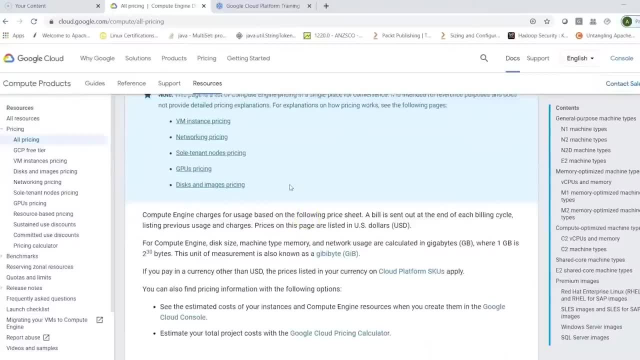 So general processing units. you have disk and image pricing and you can click on any of the links and you can see pricing which also shows you your pricing. So let's go ahead and click on pricing. So here you have different kind of machine types. 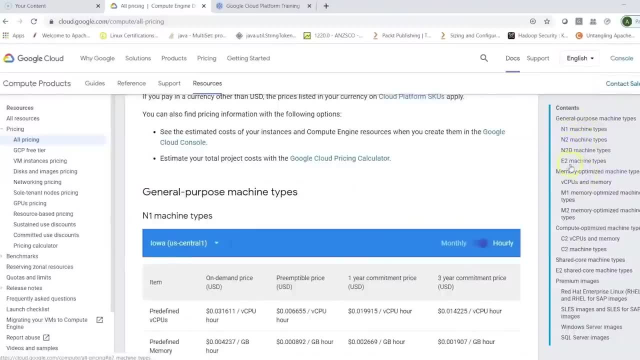 So here you have different kind of machine types, which says N1,, N2,, N2D, E2. You have memory optimized machine types, you have compute optimized, you have premium images and you can basically look at all the categories. You can look at disk pricing, which involves your persistent disk pricing for SSDs or HDDs. 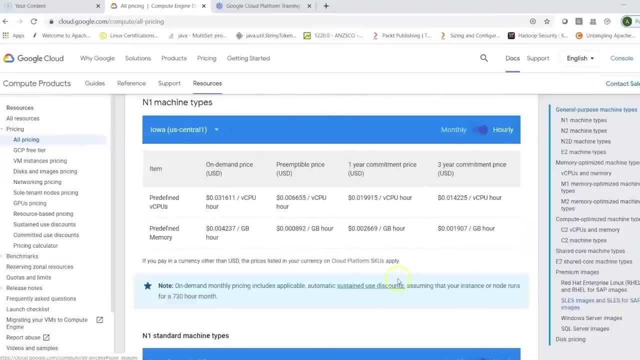 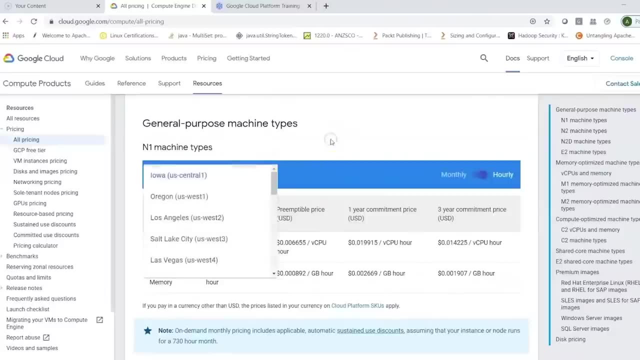 what are the kind of images? what are the different network services? right, And you can always look at Your machine types. you can choose a particular region- right, There is the concept of region and availability zones here and as per region you could look. 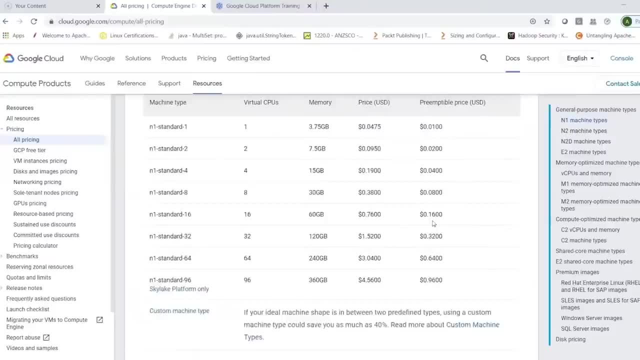 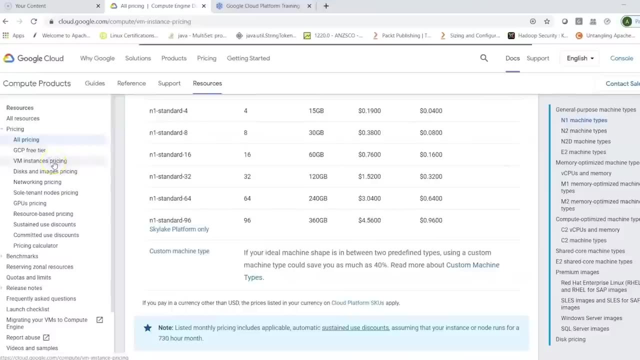 at the prices. You can also look at standard prices You could be looking for. what are the free tier machines? If I'm specifically looking for VM instance pricing, I can click on this one and that takes me to the VM instance pricing. What is the billing module? 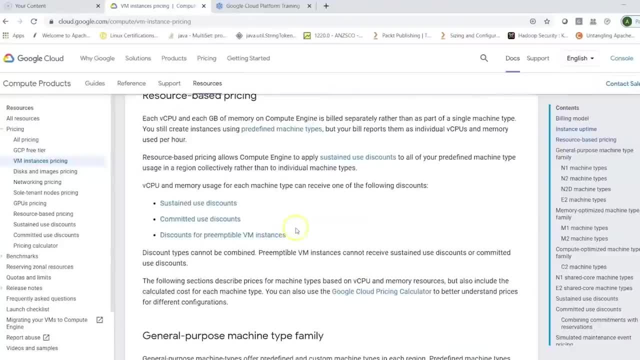 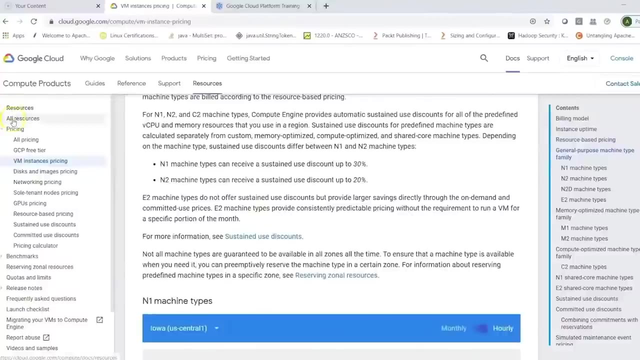 What is the instance uptime, What is the resource based pricing, And then you can also look at different kind of discounts, such as sustained use discounts, committed use discounts, discounts for preemptible VM instances and so on. And this is how you can be looking at pricing for all different resources and you can choose. 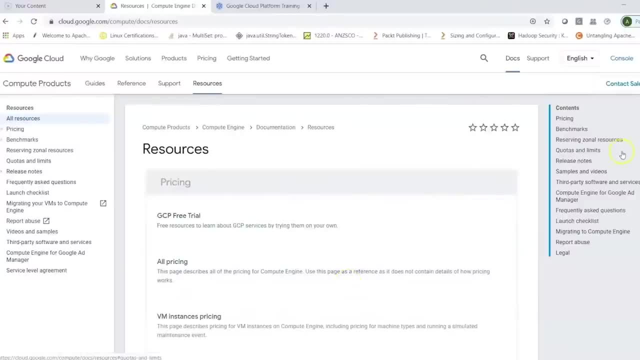 the resource which you are interested in and then look for the pricing, benchmarks, reservations if you would want to use and you would want to benefit, if you would want to look at what are the quotas and limits and so on. So please explore this link and you can find a lot of information when it comes to technical 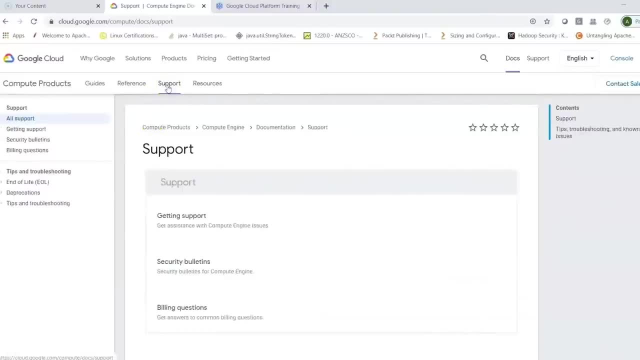 options looking at different Google Cloud products, which we briefly discussed when it comes to domains and what each product can be used for. You can always come back to the main page, where I was showing you different services. We went into pricing straight away, right? 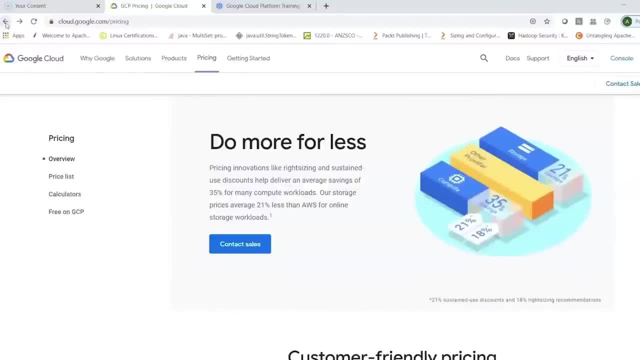 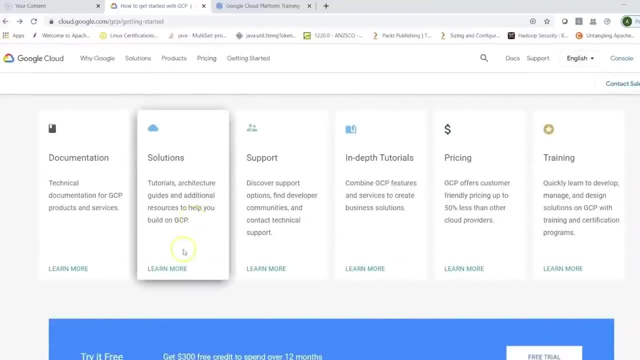 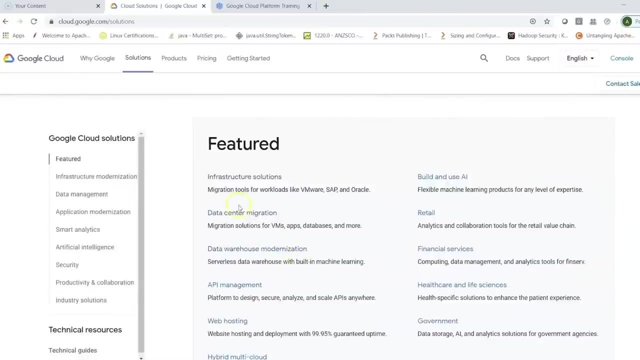 Now you can always come back to this page on your cloudgooglecom and then you have your solutions, Which talks about pricing, Talks about different products, right, And you can click on these or you can look into technical documentation. So this talks about your different featured solutions, infrastructure solutions you have. 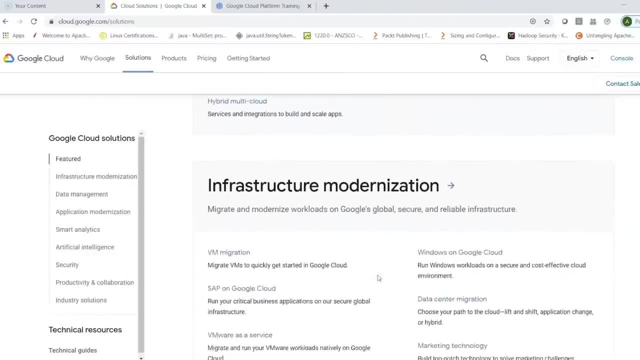 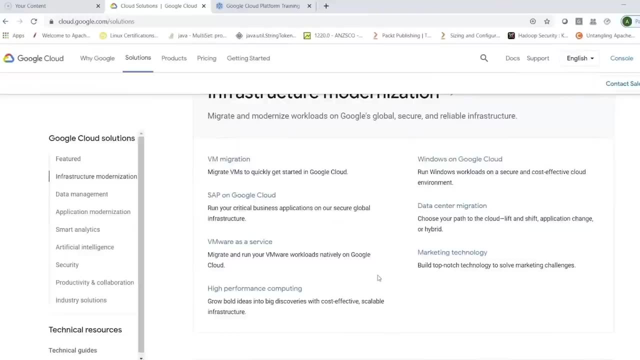 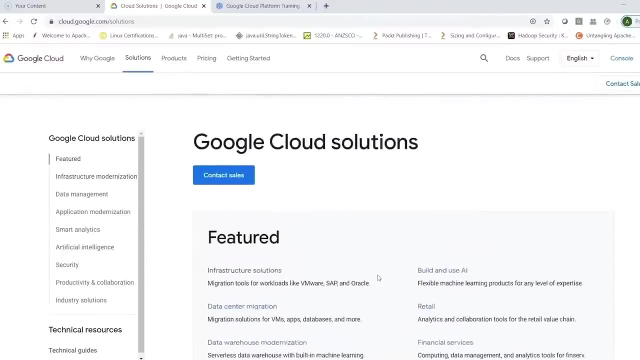 data center, migration related and so on. So I could be talking more and more about Google Cloud Platform. It's a ocean. It's a huge chunk of different services for different organizational requirements. So look into this link And also what you can do. 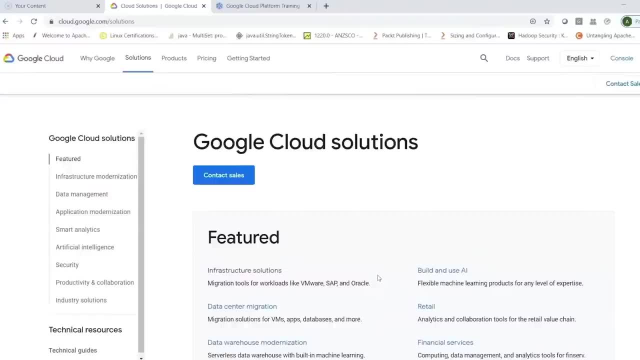 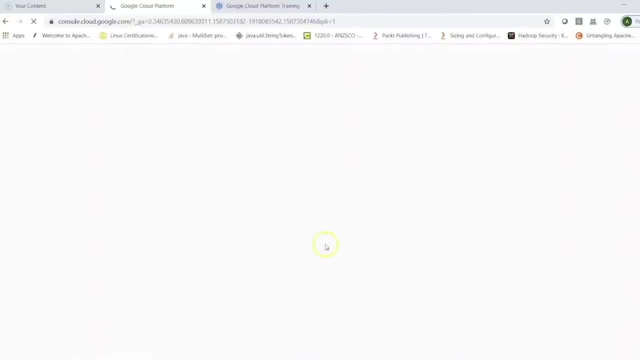 What you can do is create a account on Gmail- I mean you could create a free account- or you could go to cloudgooglecom and then you could create a free account, like I have created here, and I can just click on console. Now that's my GUI, or Google Cloud console, which basically allows me to work with Google. 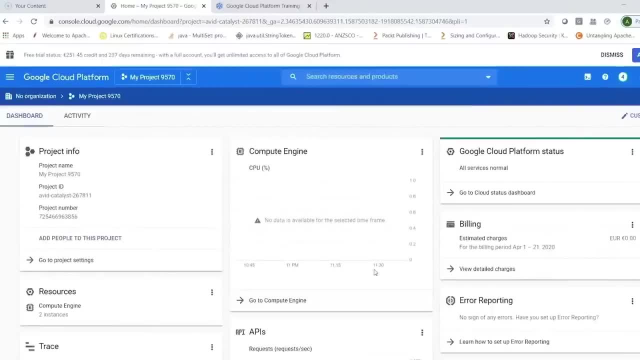 Cloud. Now there are a lot of options here by default when you create an account. Now, in my case, on the top it says it's a free trial account. I have $300 credit and out of that $251 is left and 237 days out of a year are left for. 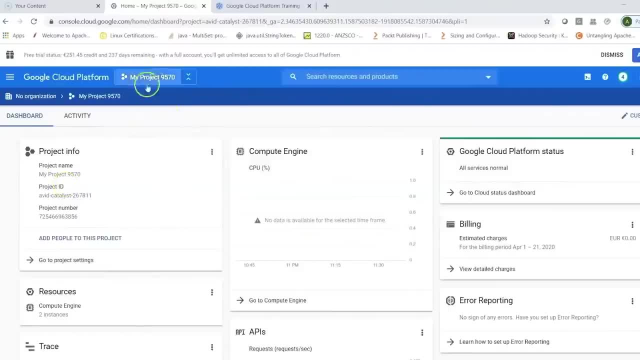 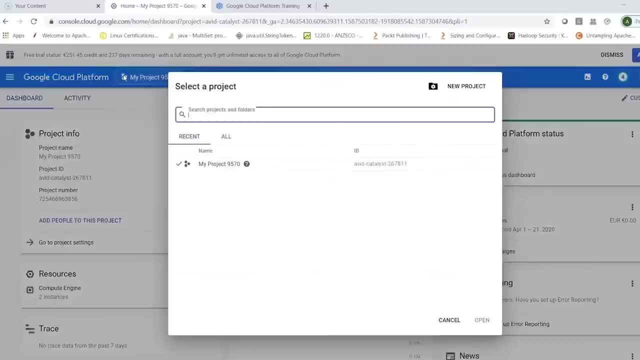 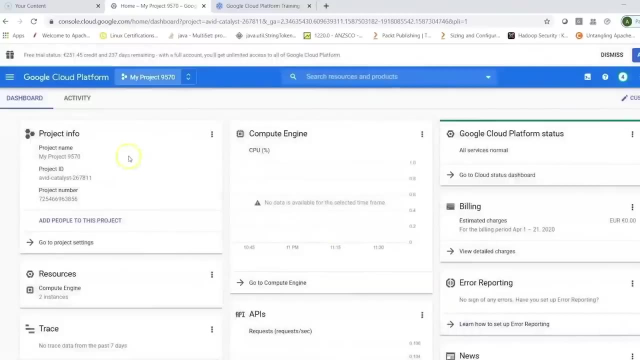 my account. Now here I can basically see the project right And by default we can create a project or by default there is a project existing for any user. So when you log in, it creates a particular project and you could create a new project. 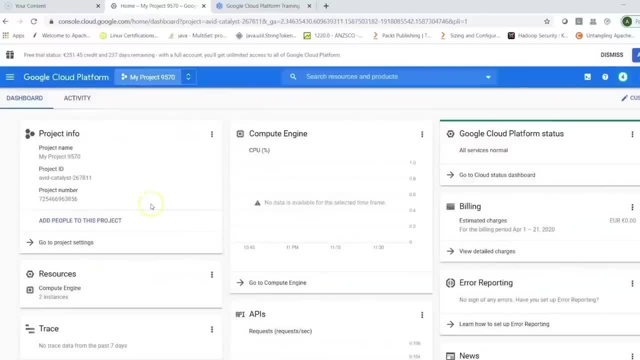 and project would be to dedicate your different services, So different resources, for different project. So this is your dashboard, which basically shows your project, which shows you a project number and a project ID which is always unique. Now you can click on this and this. if you would want, you can hide this information. 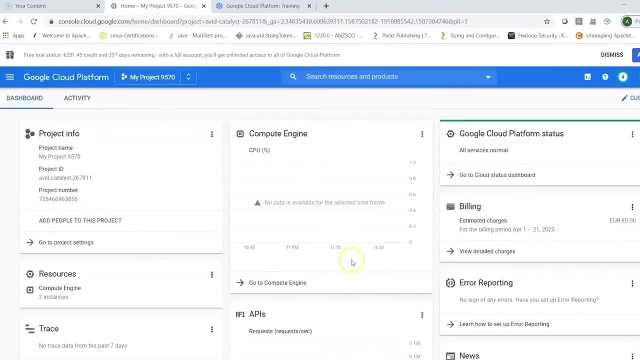 You can also look into the documentation part of it. Then it shows you the different services or a graphical information of services which you might have used in past. So you have compute engine which shows you How much percentage of CPU was used. You can always go to compute engine as a service. 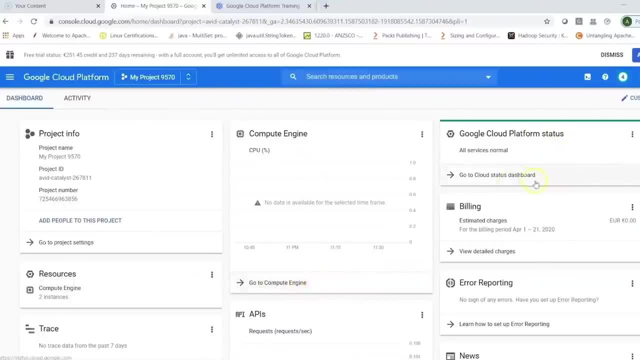 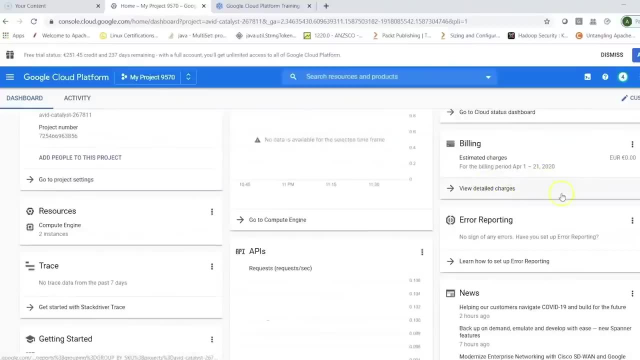 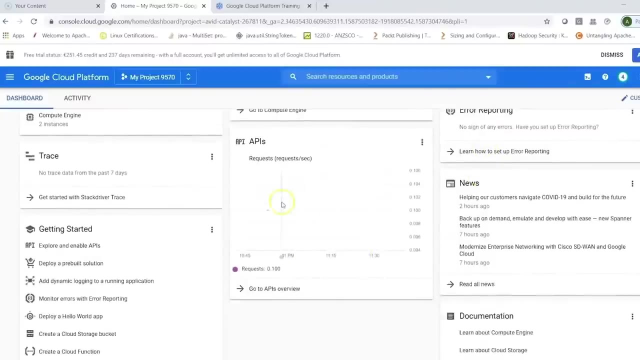 You can look at your Google road platform status and look at the Google cloud status. Now, this is billing Now, since this shows me the billing period for April month and I can always look at detailed charges. I can look at reporting. I can look at different API's which Google offers and for your different kind of work. 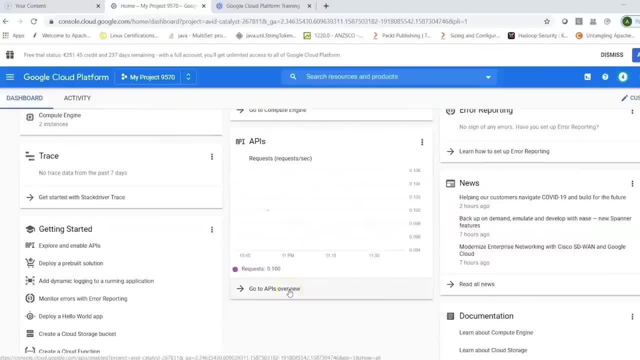 you can always go to the API overview. You can always go to the API overview Or the API link and enable or disable any API. Now, once you enable or disable any API, then you can use that. So you have new section, you have documentation and you have getting started guides, which 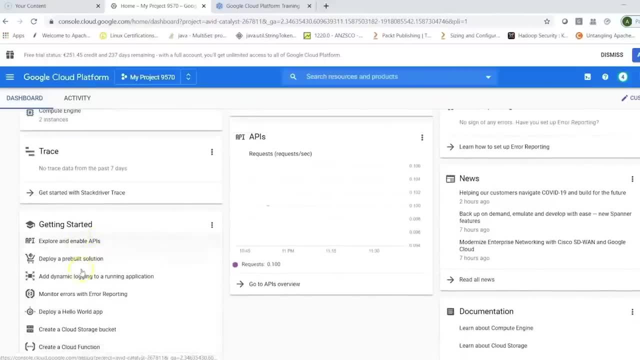 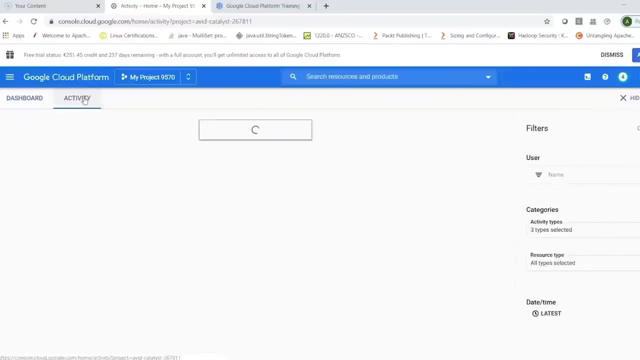 tells you how to work or enable different API's If you would want to deploy a prebuilt solution at dynamic logging, monitoring errors, deploying a hello world app, and so on. Now this is your dashboard. I can click on activity And that would show me what kind of activity I would have done in my cloud platform. 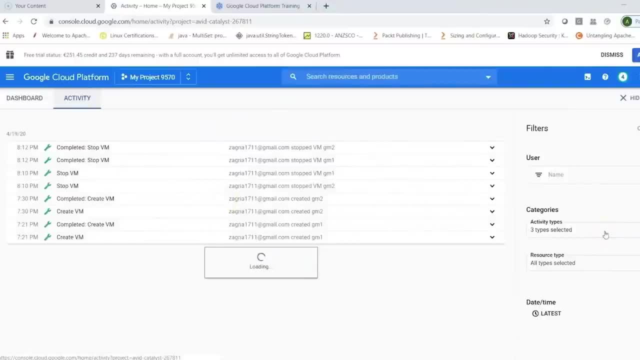 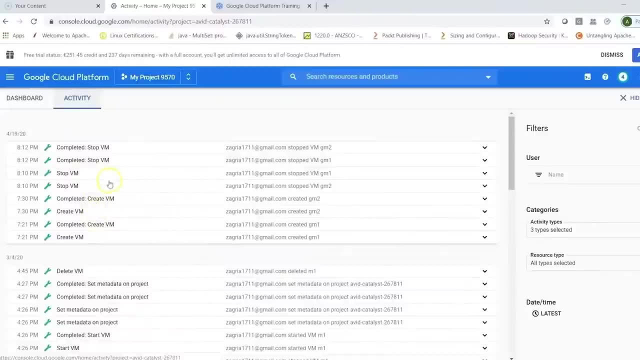 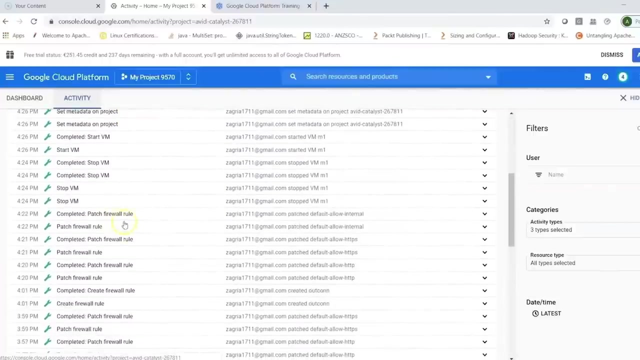 I can always choose the kind of activities. by saying activity type, I can choose the resources. Now it shows me that I created some VM instances. I deleted them, I updated some metadata. I basically worked on instances. I changed some firewall rules here. 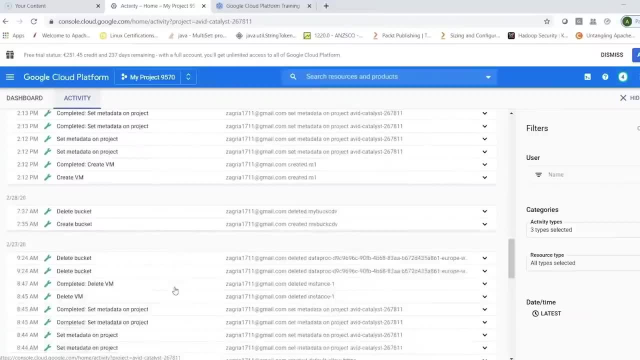 I have then also worked on some other things. I have then also worked on some other things. I have then also worked on some other things. I have then also worked on some other services or API. So I created some buckets, which is for object storage. 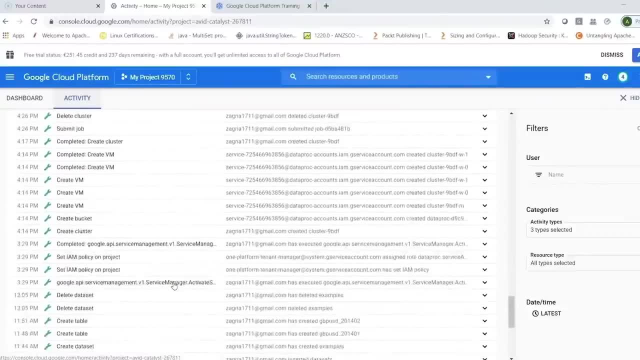 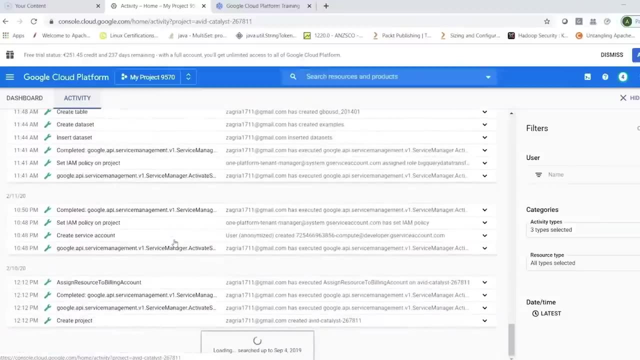 And again I have been working with some instances and creating some firewall rules. here I have granted some permissions, I am setting up a policy right. So this activity gives me a history of what things I have done over the past couple of months while working on Google Cloud Platform. 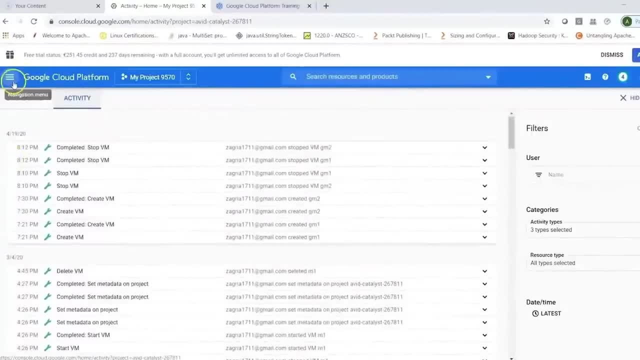 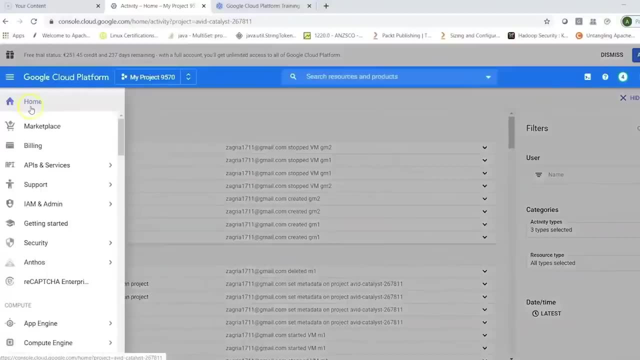 Now on the top left corner. Now on the top left corner, I have the hamburger menu, which you can click on this. So that's your navigation menu, And when you click on this, this shows you home. It takes you to the marketplace. 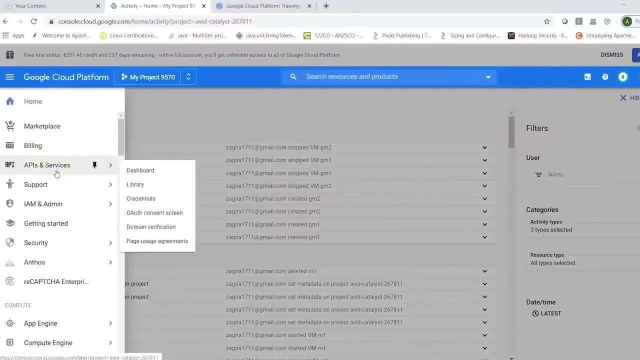 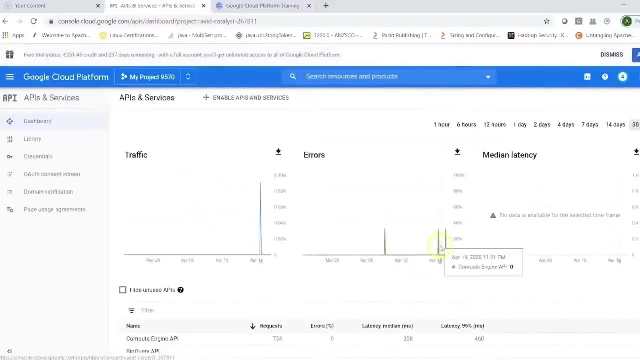 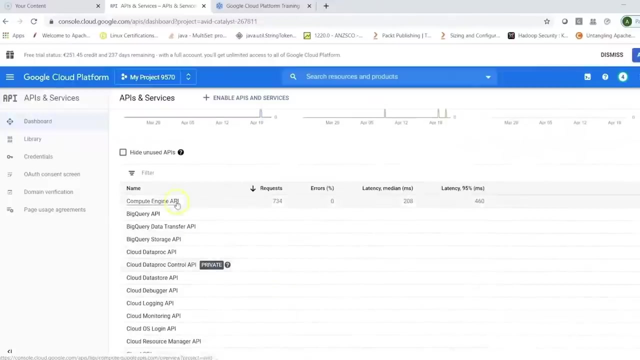 It specifically takes you to billing. You can always look at APIs and services. So here in API services I can pretty much go to a dashboard and I can see a report on the traffic or errors or latency and the kind of APIs which are available. 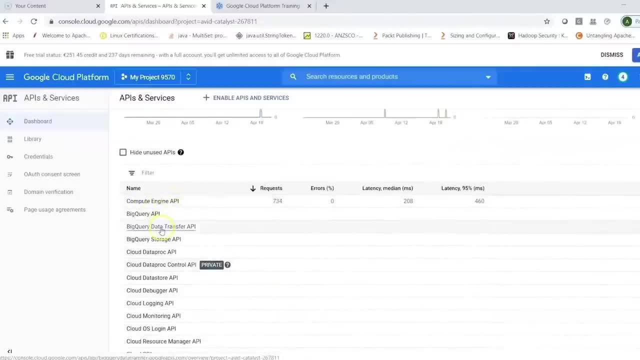 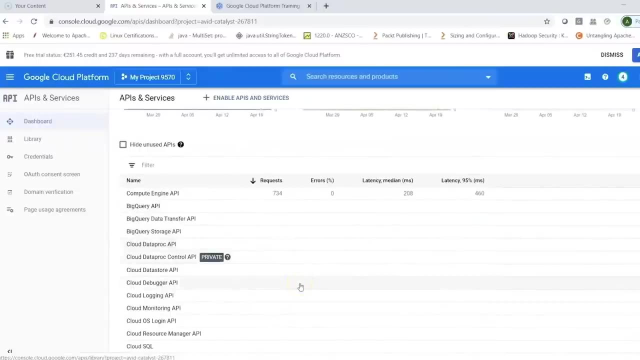 So you have compute engine API, You have BigQuery API, BigQuery data transfer API, BigQuery storage Cloud, Dataproc. So these are some of the APIs or services I've used in the past. Might be I was evaluating a product. 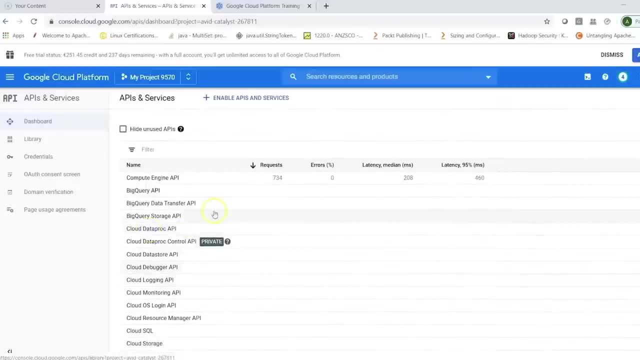 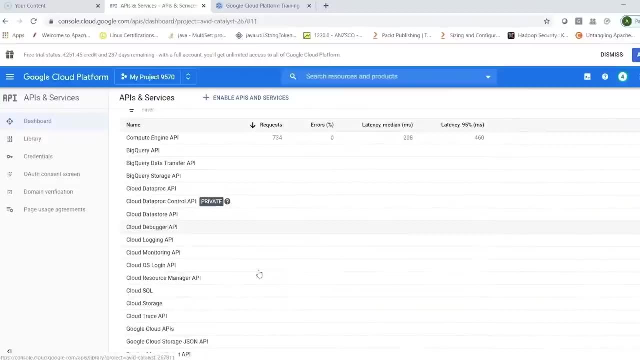 Might be. I was using a particular product, So you have, whenever you would want to use a particular service from Google Cloud Platform, you would be enabling these APIs. So here we see some APIs for Dataproc. You have logging, monitoring. 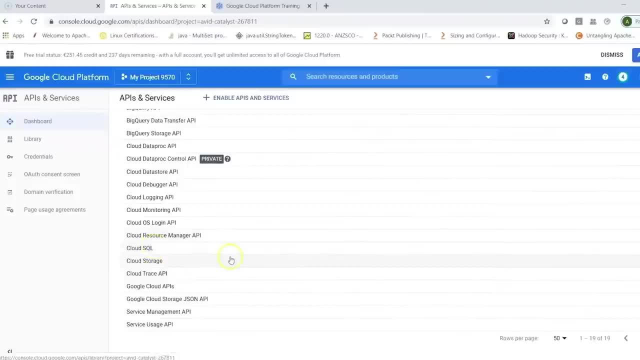 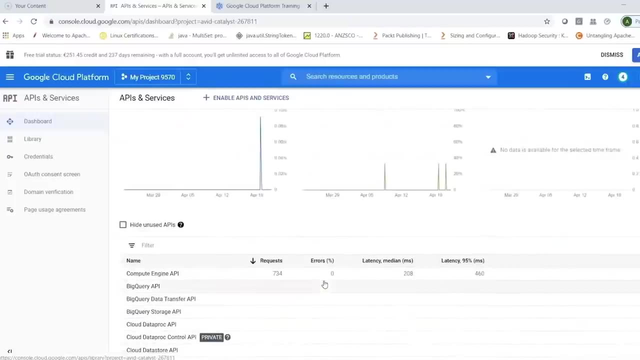 You have resource manager API, You have cloud, You have cloud SQL which allows you to directly use MySQL or Postgres, You have cloud storage right And so many APIs. So if I would want to enable a particular API, which is not right now required, but 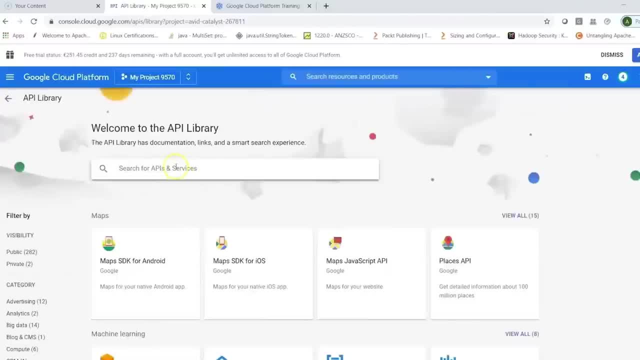 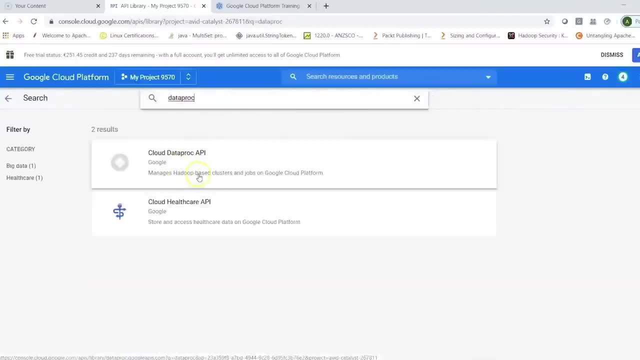 then it's good to know you can always click on this one. You can search for an API. So, for example, if I would say Dataproc, right, And that shows me the Cloud Dataproc API which manages Hadoop-based clusters and jobs on. 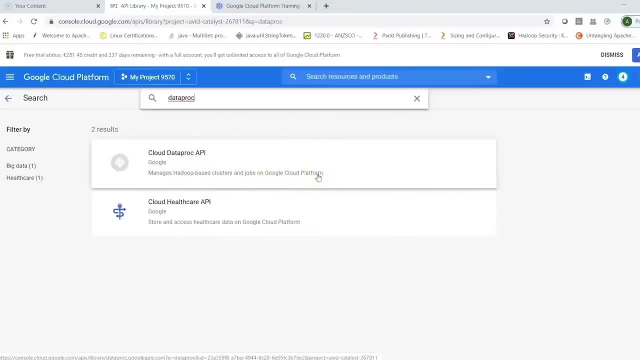 Google Cloud Platform. So I can spin up a Hadoop. I can spin up a Hadoop cluster and I can start running some jobs on a Hadoop cluster on demand And as I'm done with it, I can just get rid of it. 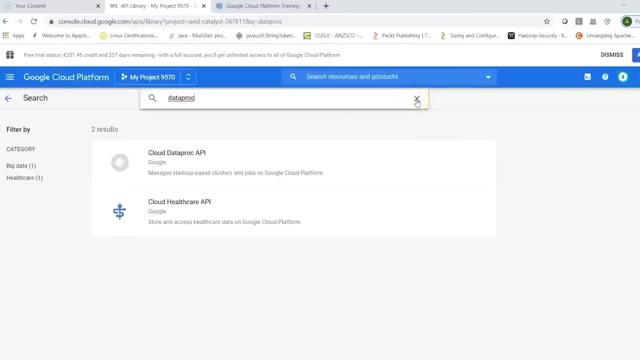 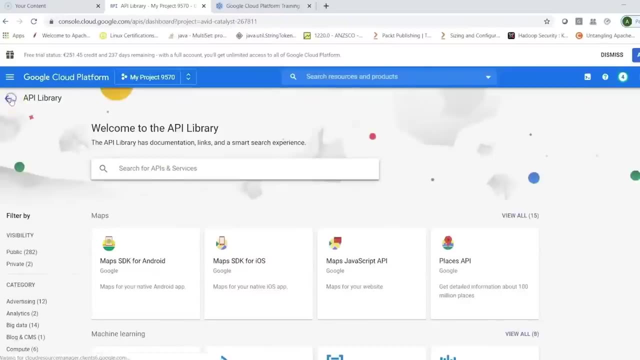 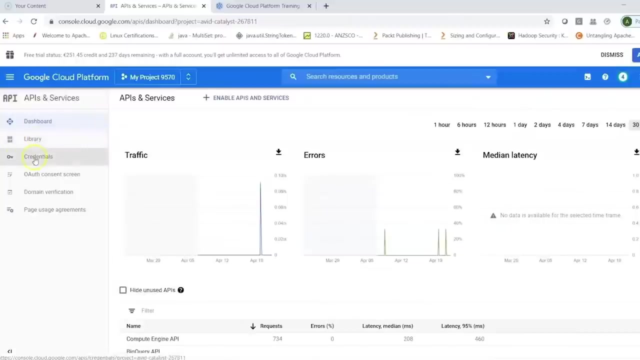 So this is an API which I would have to enable And then for every particular service, you also have an admin API which you would enable. Now, going back, so coming out from this API library, I got into API and services. Now there is, you can look into the library, you can look at credentials and you can also 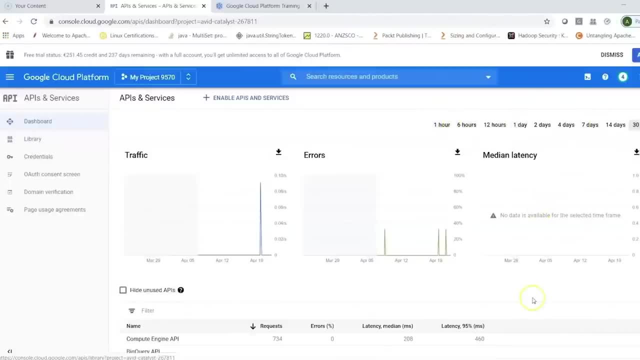 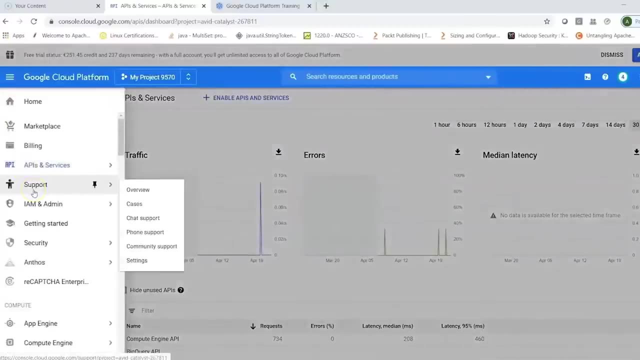 look at different time intervals for which you can see the usage of your different APIs. Now, going back to the menu, you have support, wherein you can always reach out to the Google support team. If you are using a paid version, even with free trial, you can try to reach out and you 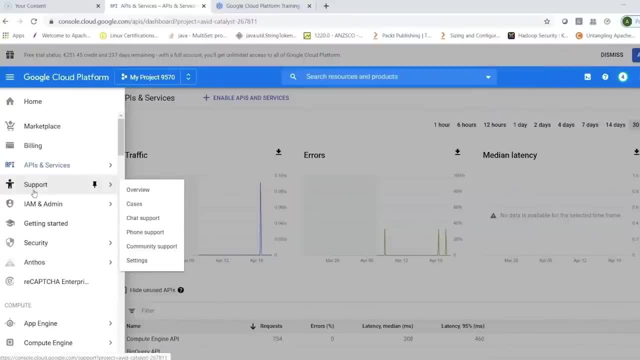 will find someone to help, But it is always good when you have a billing cycle reaching out the customer care. You have identity, access management and admin. You have security related options. you have Anthos, which is mainly for migration. Now, here you can look at your different domains, such as which we discussed. 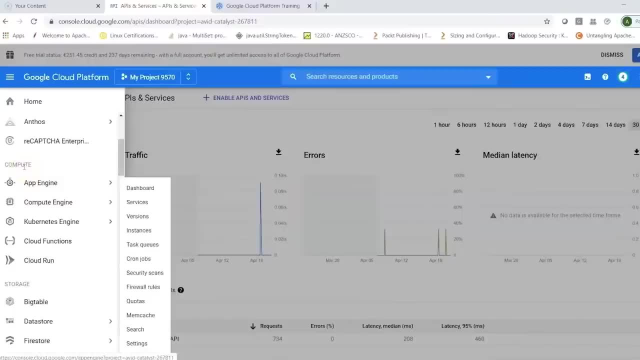 So you have compute and in compute you have different services. So you have App Engine, you have Compute Engine Kubernetes, you have Cloud Functions and Cloud Run. You can look into the storage aspect which shows you big table, which is usually and. 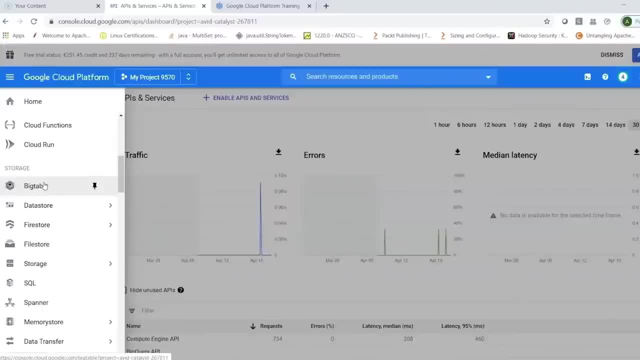 mainly for your unstructured data Big table, which is something which gave rise to popular NoSQL databases like HBase and Cassandra. You have data store which can be used. You have fire store, file store storage, which can be used to put in data of any kinds. 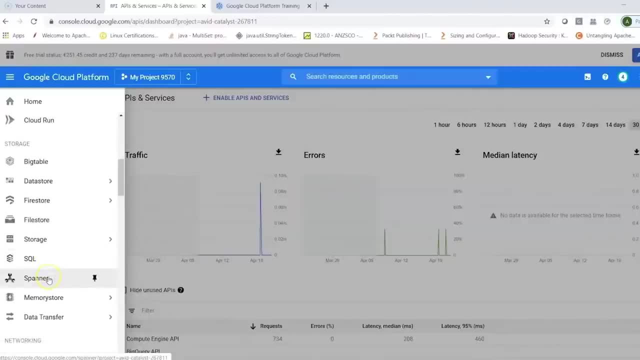 You have SQL for structured data, You have Spanner as a service, You have memory store And you have data transfer. Now, when it comes to the networking domain, you have all these services, such as VPC, virtual private network, network related services for your load balancing, for using a cloud. 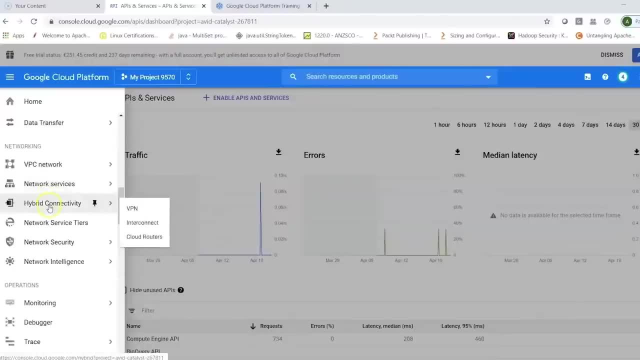 based DNS or cloud defined network. You have hybrid connectivity, network service, tiers, security and intelligence. Then you have other options for your operations which can be used, And here you have different other tools which can be used, such as cloud build. 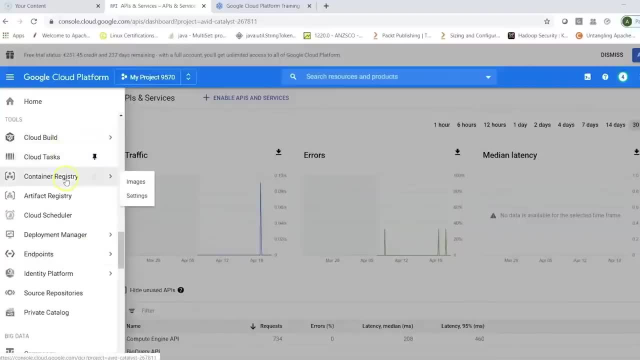 And here you have other options for your operations which can be used. And here you have other options for your operations which can be used, such as cloud build. You have cloud tasks, container registry, deployment manager and many more. Big data specific: you have the services here. 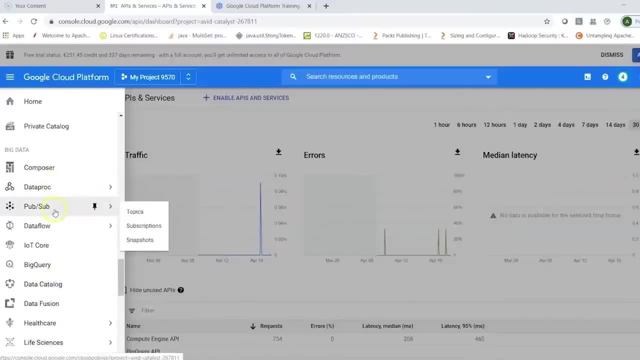 So you have Dataproc, which can be used to spin up your clusters. You have published subscribed messaging systems, such as now, Kafka, which you might have heard of, originates its idea from here, So PubSub. You have Dataflow. You have IoT Core BigQuery, which is a data warehouse package or data warehousing solution. 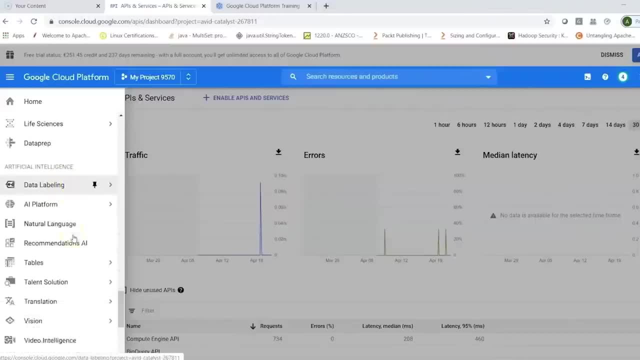 which is a data warehouse package or data warehousing solution. You have Google Cloud. Now then you have your artificial intelligence related services and other Google solutions, So you can always find a huge list of services or, you can say, at high level solutions offered. 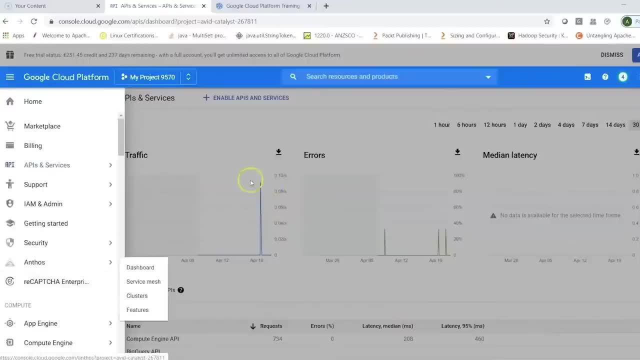 by Google Cloud And we can use these to basically test some of the solutions, use them and work on them. So I'll give you a quick demo on different services which can be used here from your Google Cloud platform. Now, this is your Google Cloud platform and this is your console. 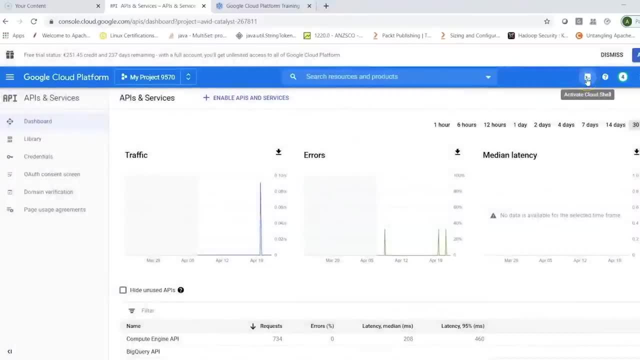 Now this also gives you a cloud shell which can be activated so that you can work from command line, And you can always find a lot of documentation on that. So you can also set up your cloud shell, that is SDK, on your Windows machine. 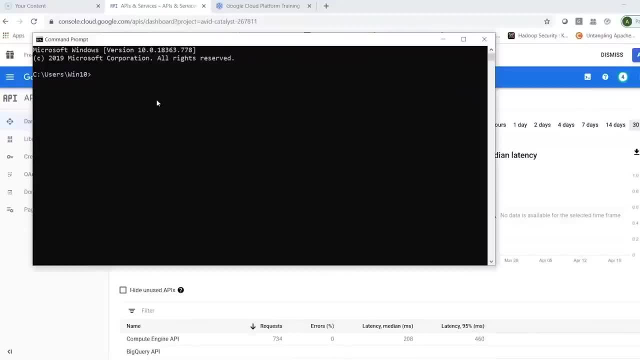 And if you have set it up, then basically you could be doing something like G Cloud, right, If the cloud has been set up. So in my case I had set up the cloud SDK and basically I can get into that by looking. 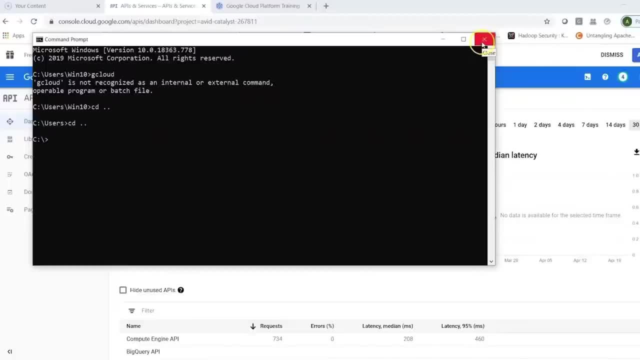 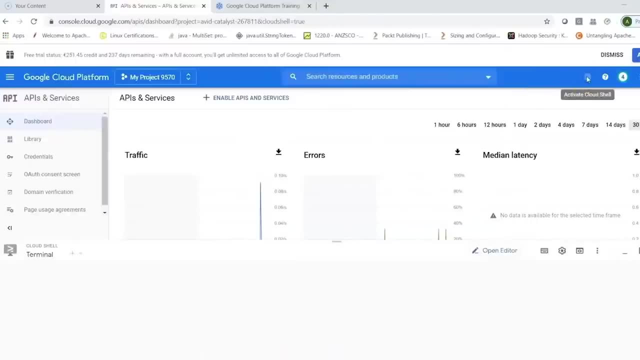 at what path I have set up So cloud SDK, and then I can be using it from my Windows machine As per my comfort. I can also activate the cloud shell here, which will basically open up a terminal, And at any point of time you can open up this one cloud shell in a different window. 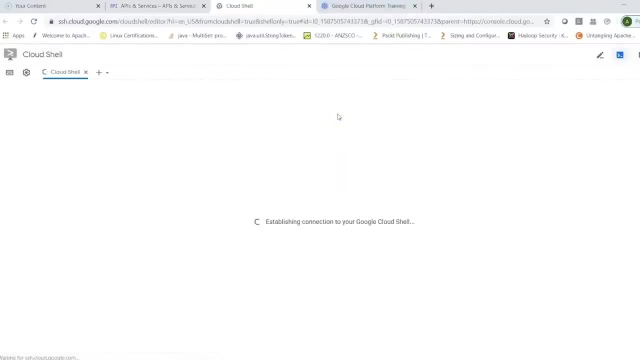 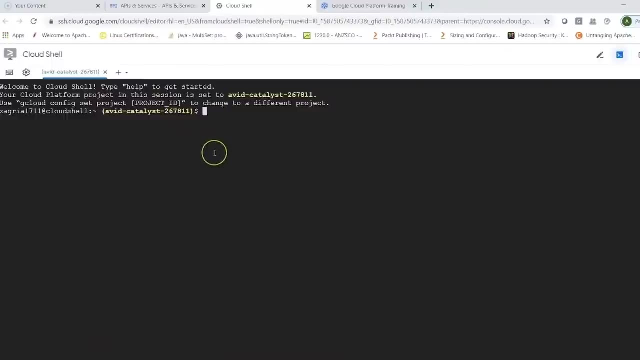 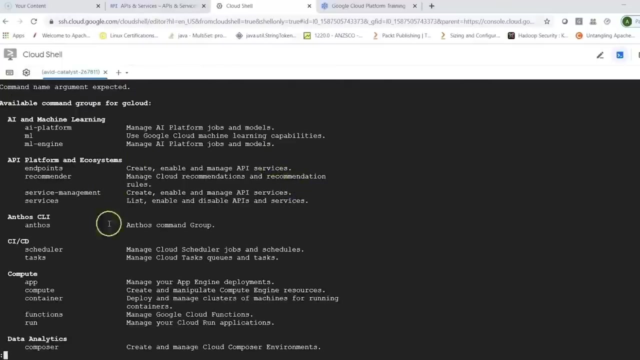 It is preparing the cloud shell, where it will by default set up your project. It will set up the metadata And now I am logged into my Google Cloud account from command line And here I can basically use G Cloud right, And that basically shows you the different options which are available, which you can. 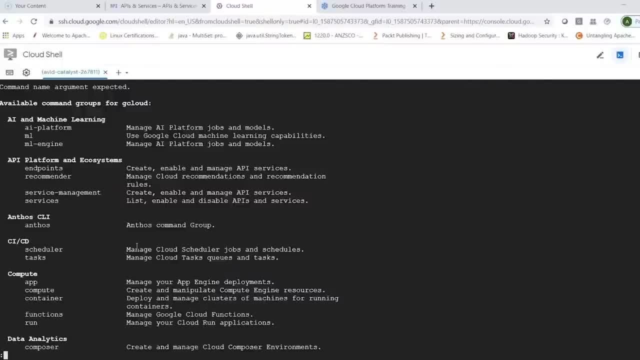 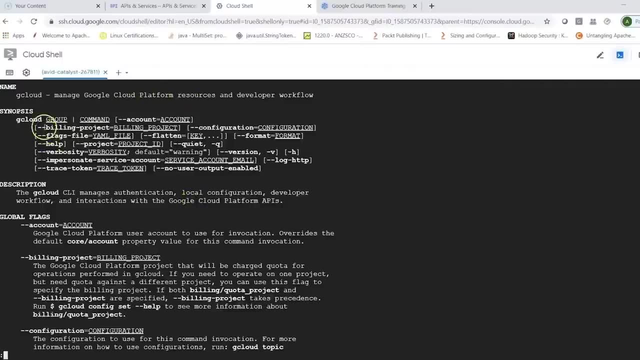 be using. So if you would want to use a particular service, you can also try giving a help And that shows you how do you manage your Google Cloud platform right. So you have different options for billing to work with your different services. 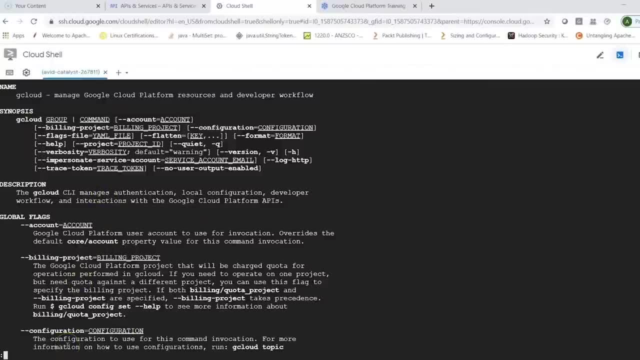 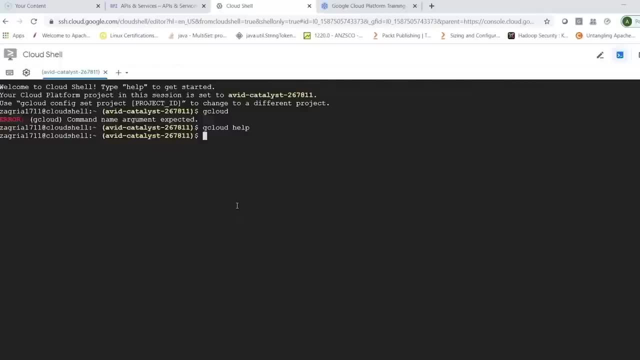 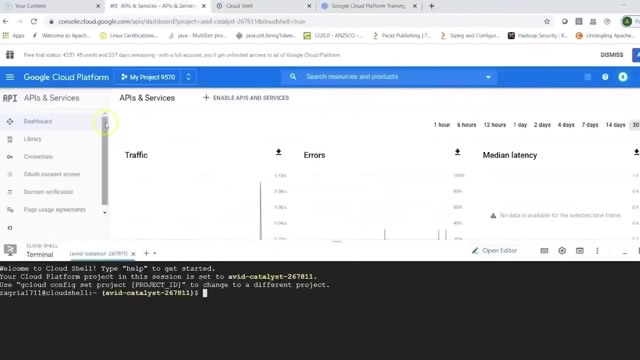 And that's it, And basically you could be working on Google Cloud using this cloud shell from your command line. Usually, for people who are learning Google Cloud in the beginning, it is always good to go for console and use your different services from here in an easier way. 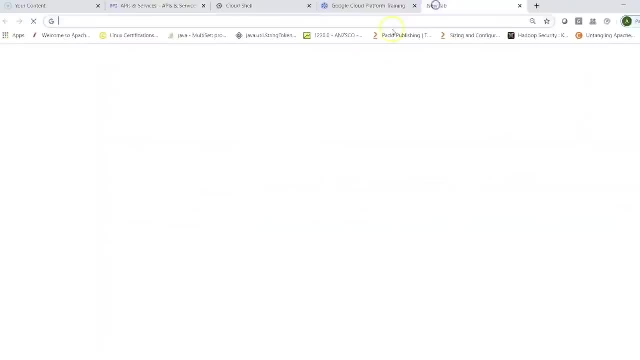 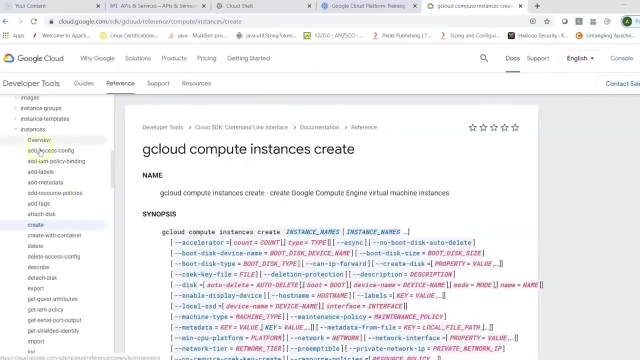 But, as I said, you can always use the command line. For example, if I would just go ahead and type G- Cloud- create instances, and that will directly take me to the cloud console documentation which shows you different options which you can use to work with instances. 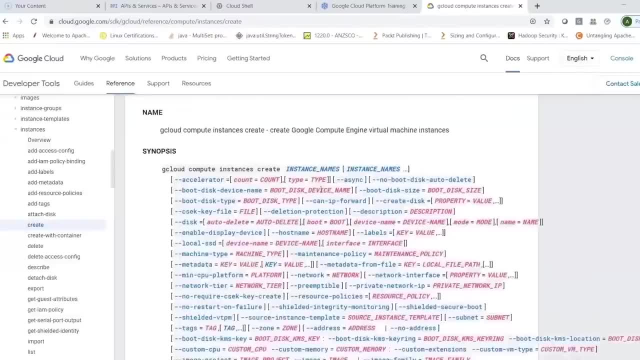 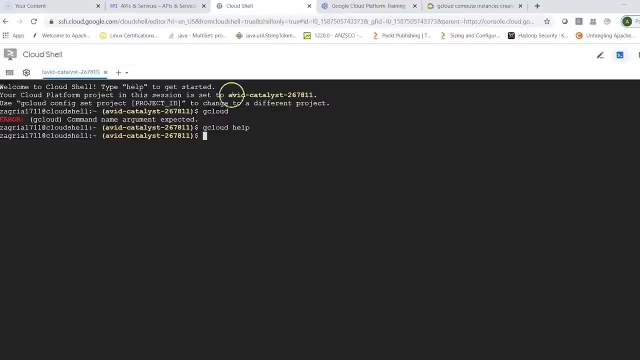 So I could do a G Cloud compute, instances create, and then I can give my instance name and so on, And I'll show you some examples on that So you can be using your cloud console. right, That is your cloud shell. 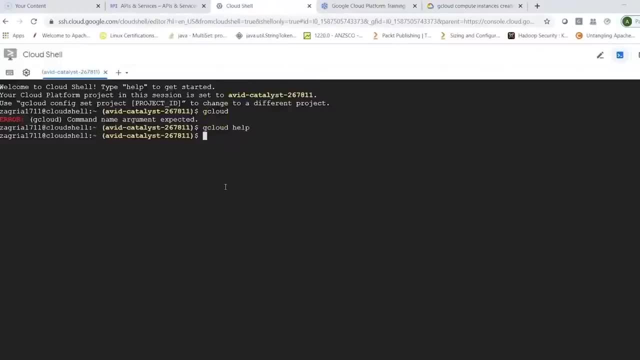 And you can straight away start working from command line. However, I would suggest using console in the beginning, and when you are well experienced, then you can start. Okay, So you can start using cloud shell to do things from command line, And when you are fully experienced you can always switch, and certain things are usually. 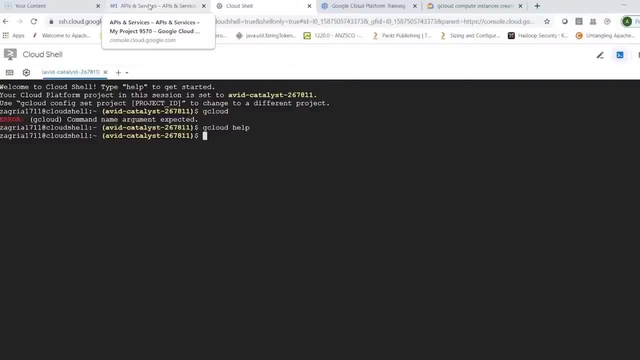 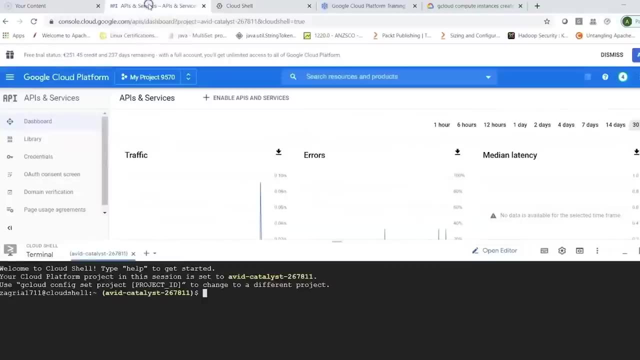 useful or easier when done from command line, And some are easier when you do it from the console, and you can use any one of these options. Now we can go to Google Cloud console. Now, as of now, I can close this one. I still have my cloud shell open. 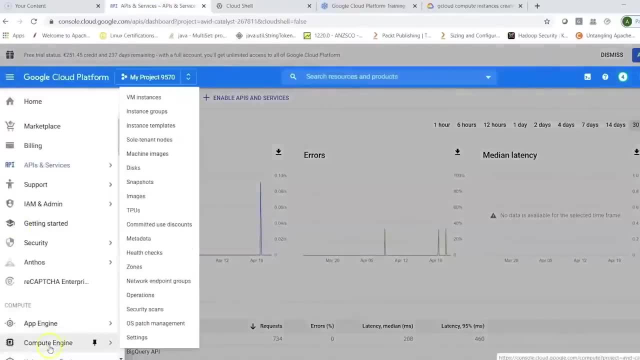 If I would want to look into it, I can click on this one and I can straight away go to compute engine, Where I would want to work on creating some instances on Google Cloud platform using the compute engine service and then basically connecting to those instances and basically 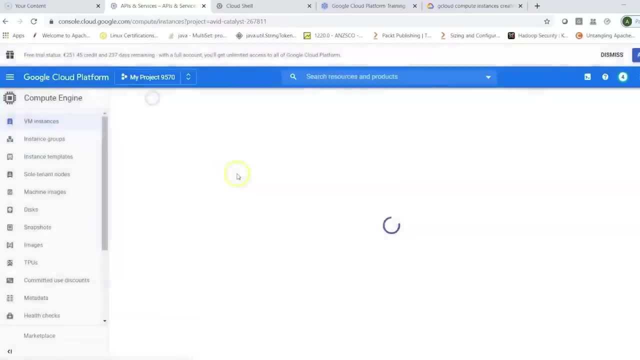 trying out some basic things So you can click on VM instances and then, once this comes up, I can always create some instances. Now, if you see here I have some instances already created, right, And I can continue working on those. I can create new instances. 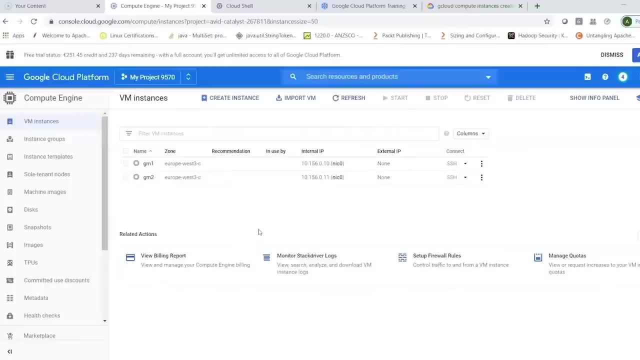 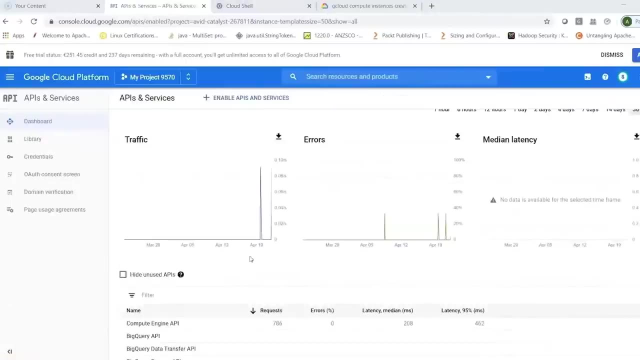 I can use different options while creating instances and I'll show you that in a demo in quick seconds. So let's have a quick demo on setting up GCP instances Now. before that, let's have a quick recap. So when you talk about instance or a virtual machine, it is hosted on Google's infrastructure. 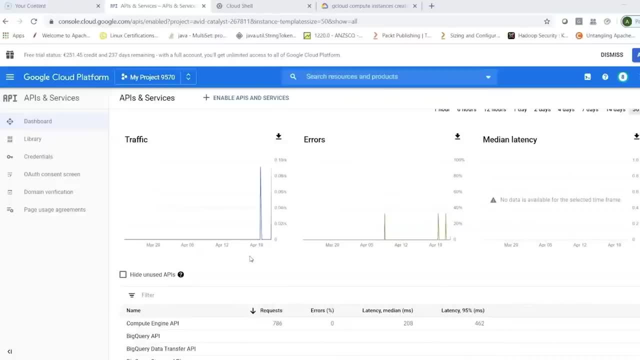 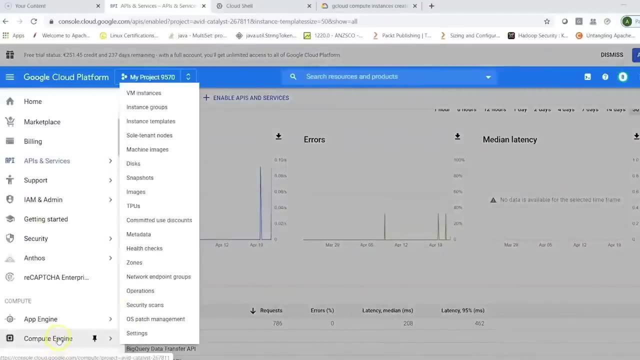 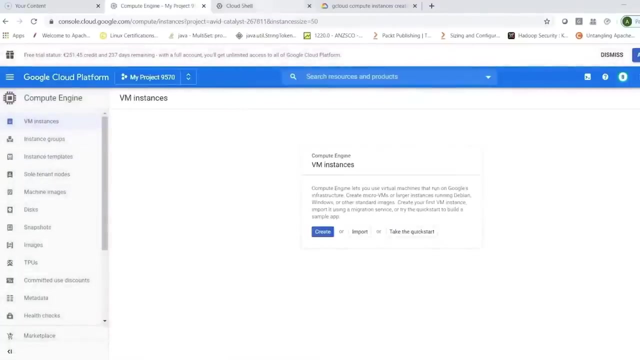 right, And you can create your Google Cloud instance using this Google Cloud console, That is, by clicking on this and then going to compute engine and clicking on VM instances. Now you can also do that from Google Cloud command line tool, that is, Cloud Shell, and 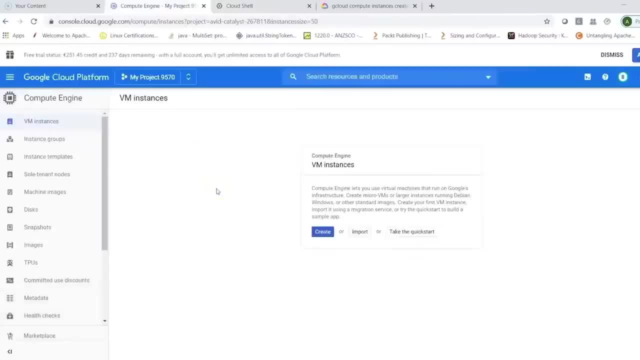 you can be doing that using compute engine API, So compute engine instances can run the public images for Linux or Windows servers that Google provides. You also have option of creating or using custom images that you can create. You can also create custom images that you can create. 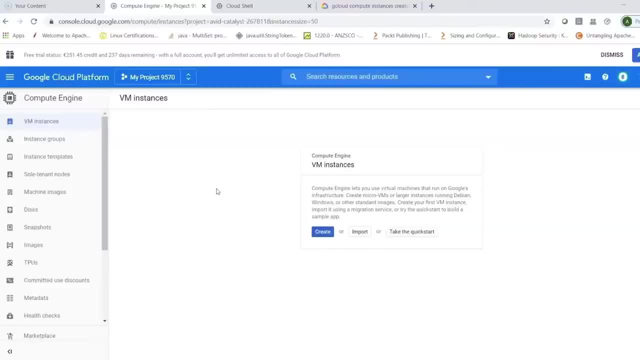 You can also create custom images that you can create. You can also create custom images that you can create and import from your existing systems. You can deploy Docker containers which are automatically launched on instance running containers optimized OS. Now, when you talk about instances and projects, always remember that in each instance belongs. 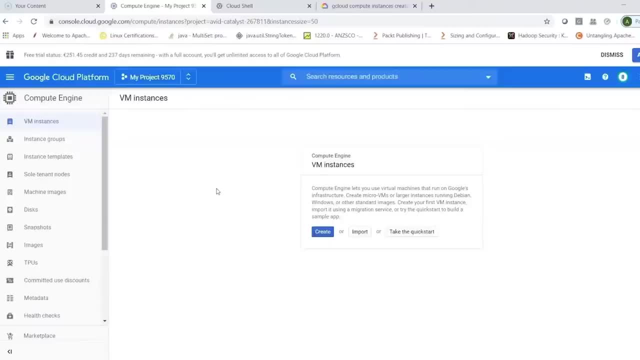 to a Google Cloud console project, and a project can have one or more instances. When you talk about instances and storage options, each instance has a small boot persistence. So let's say you have a boot persistence disk, which I will show you in further screens. 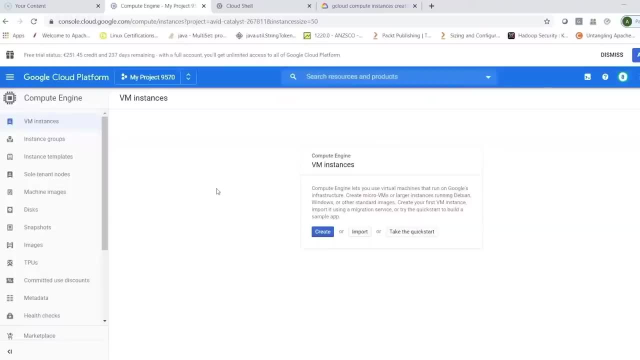 that contains the OS. you can add more storage space if needed. When you talk about instances and Network, a project can have upto 5 VPC network. So VPC Network is Virtual Private Network, wherein you can have virtual private cloud networks where you can have your resources within your own subnet. And each instance belongs to one VPC network. We are going to say that each instance has 5 VPC networks. We are going to say that each instance has 5 VPC networks. We are going to say that each instance has 5 VPC networks. 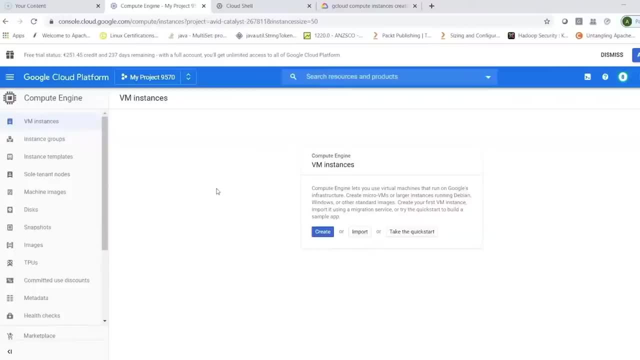 And each instance belongs to one VPC network. So if we do this, we are going to be able to access all the VPC networks which are part of Microsoft VPC network. Now instances in same network can communicate with each other through local area. 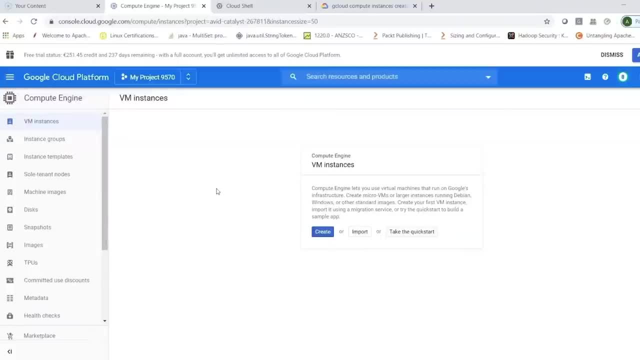 network protocol. An instance uses internet to communicate within any machine, So that could be virtual, physical or outside its own network. When you talk about instances and containers, you should remember that Compute Engine instances support a declarative method for launching your 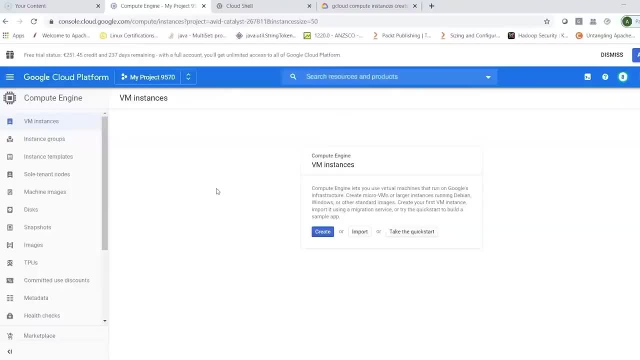 application using containers. Now you can create a VM instance or a VM instance template. You can provide a Docker image and launch the configuration. So there are different ways in which you can create these instances. And once you create these instances, you can say, for example, 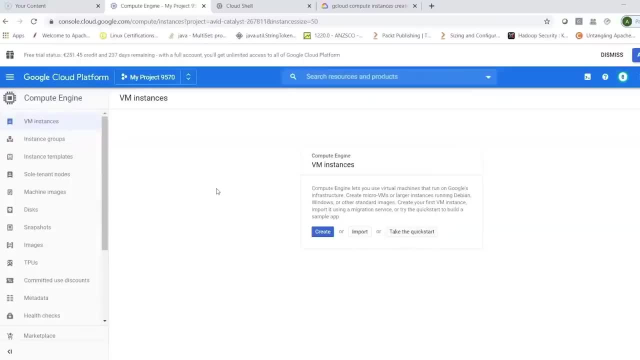 you're creating a Linux instance, You can associate SSH keys with your Google account or your G Suite account and then manage your admin non-admin access to the instance using IAM roles If you connect to your instance using G Cloud or SSH from console. 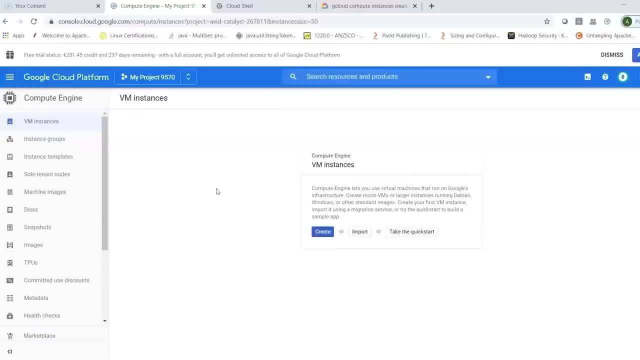 which we will see later. Compute Engine can generate SSH keys for you and apply that to your Google Cloud or G Suite account. Now what we can do is we can see how we can create your Google Cloud instances from your console or from the command line. Let's have a look in creating. 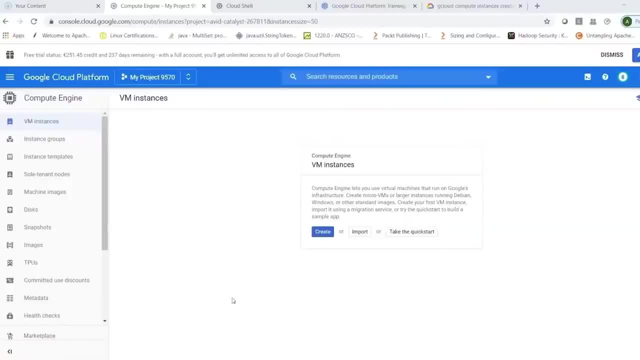 from your intra-magnet console or Cathodehtml. Add some a few cover, condemn as see if that works. Let's also see what are the different options which are when you would want to create the virtual machine instances here. So when you click on your drop, 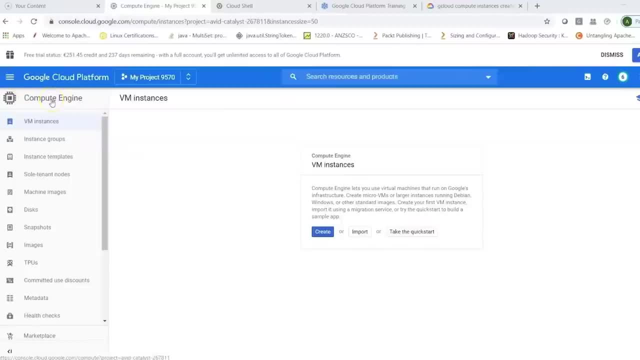 down from the top left and choose compute engine. so it brings you to this page. So I can show that again. So you can click on compute engine, click on VM instances and that basically brings you to this page. Now, here it tells you compute engine lets you use virtual machines that run on Google's. 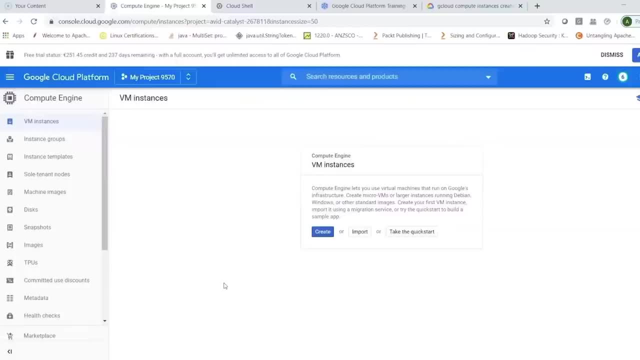 infrastructure. So we can create micro VMs or large instances running different distributions of Linux or Windows using standard images, that is, public images, and you can also have your own image. So let's create a VM instance by clicking on create Now. that's basically helping me to. 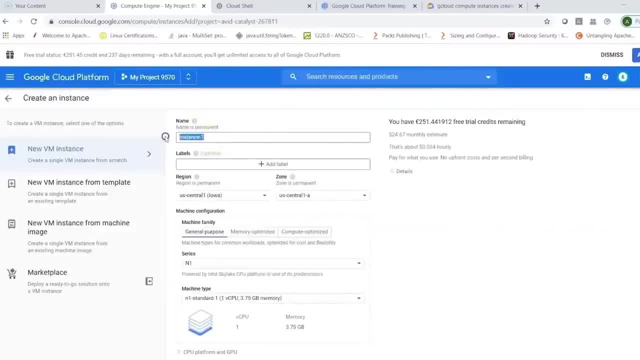 create an instance here. So it shows me the instance name. I can give it something. So let me say C1. Now I can add labels. So what is label? It basically allows you to organize your project. add arbitrary labels as key value pairs to your. 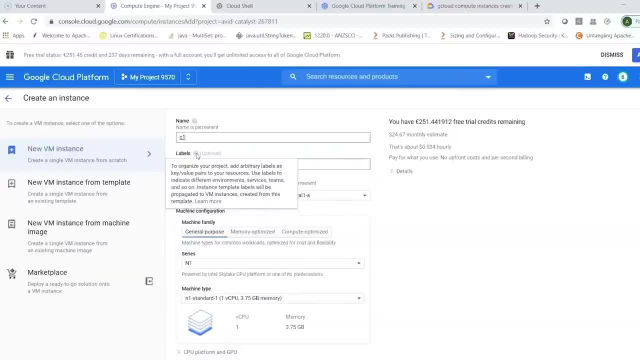 resources. So this is basically categorizing your labels and projects. if you have multiple projects Now remember if you have your cloud console and if you have created your free trial account, it will allow you to do these things. If not, you may have to go back to the billing. 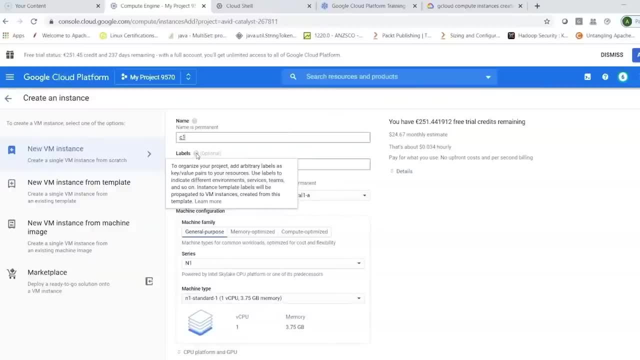 section and see if the billing is enabled, which also means that when you are creating your Google Cloud account, it will ask you to create a free trial account. So, if you have a free trial account, it will ask you to create a free trial account. So, if you have a free trial account, it will ask you to. 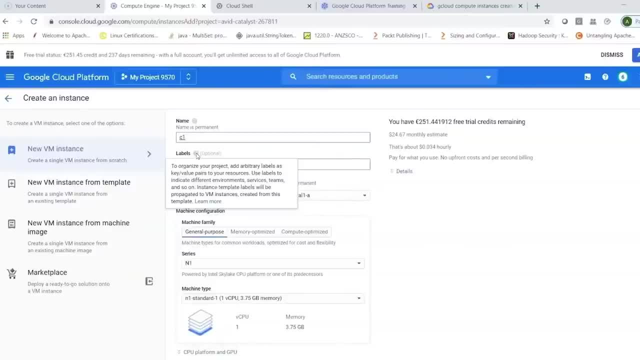 key in your credit card details, but they do not charge anything, or they might charge. might be one dollar or one rupee, depending on your location, and that's also refunded. but that's just to verify your card Now. once I've given the name, I can choose a region, So I would basically choose. 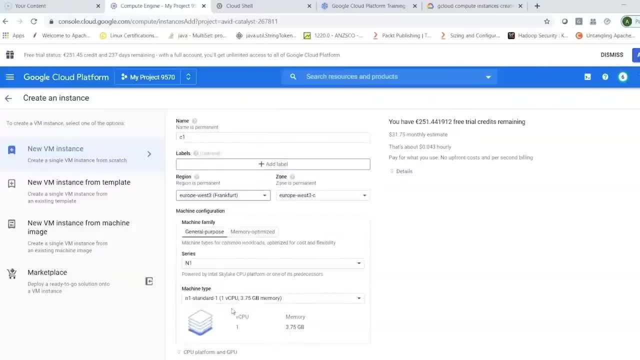 Europe. Since I'm in Europe, I would be clicking on Europe West 3 and here I can choose an availability zone. Availability zone is basically to make your services or instances or any other resources highly available. So you can choose one of the availability zones. Now I would choose save as three. Now this one, we can scroll down and here 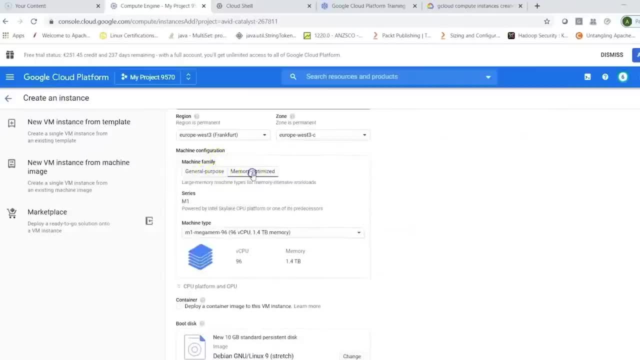 it says machine configurations. You have general purpose machines, you have memory optimized machines, which is M1 series, and you can always go back to the Google Cloud page and see what a particular kind of machine specializes in. So I would click on general purpose and in general. 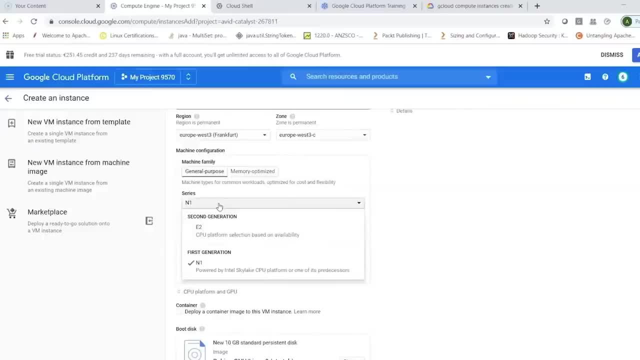 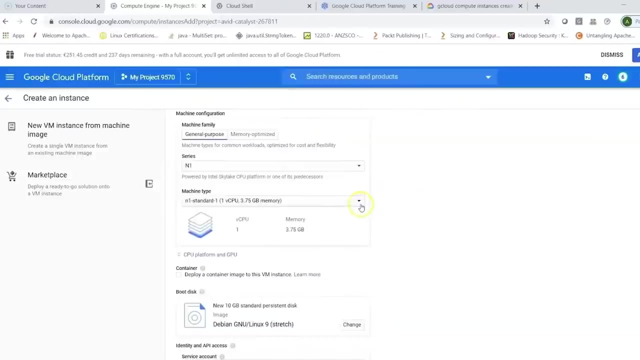 purpose. you have different categories. So you have N1, which is powered by Intel Skylake CPU platform, or you have E2, which is CPU platform selected, selection based on availability. So let's have N1 selected Now. this one shows me the machine type and if you are using your free. 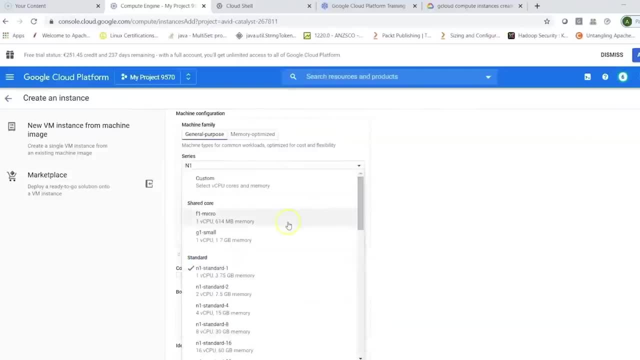 tier account. then you can start with correcting a micro machine, which is one virtual CPU core. You can go for a G1 small, which is one virtual CPU core, and 1.7 GB. You can even go up to a high end machine and then you can basically see if you are using. 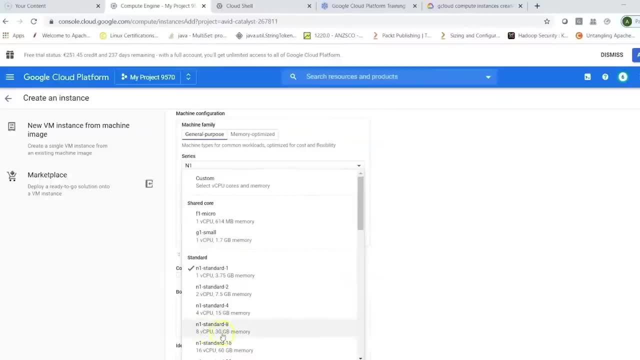 a free account. how many of these machines you can use? If I would be selecting eight virtual CPU cores and 32 GB of memory, then it would allow me to create at least two instances by this configuration. We will use N1 standard, which is one virtual CPU core, 3.75 GB memory. 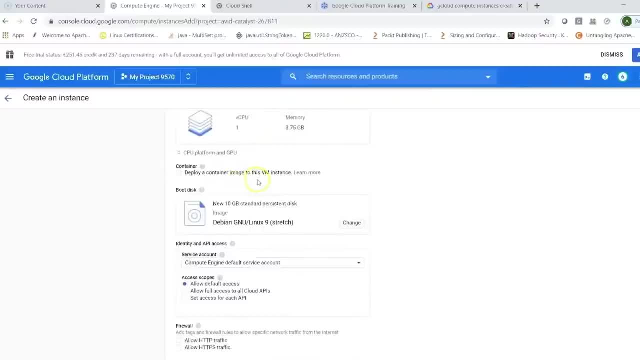 Now. then we can also deploy a container. We can deploy a container image to this VM instance. If you would be interested in deploying a container image, let's not get into that right now. Here it shows you the boot disk and it shows you DBN, GNU 9, Linux 9.. What I would do is I can go for this distribution. 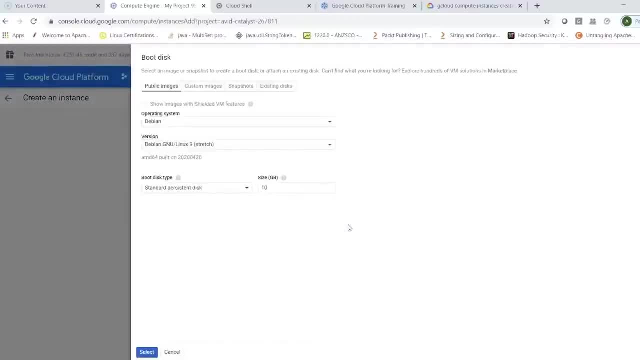 or I can choose a Linux distribution of my choice. So here you have public images, you have custom images, You also have snapshots, if you have created backup of your previous images. here I can choose, for example, Ubuntu and then I can choose a particular version. So let's go for Ubuntu 18.04.. You 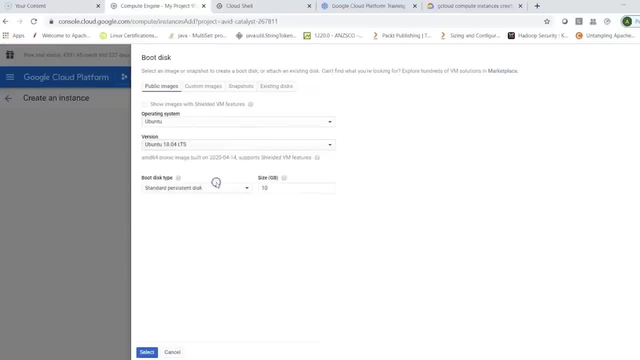 can go for the latest one also. 18.04 would be good enough. And here it tells me what is a boot disk. So you have SSDs or you have standard persistent disks. Now SSDs are little expensive in comparison to your standard persistent disks or your SDDs, but then SSDs are faster. 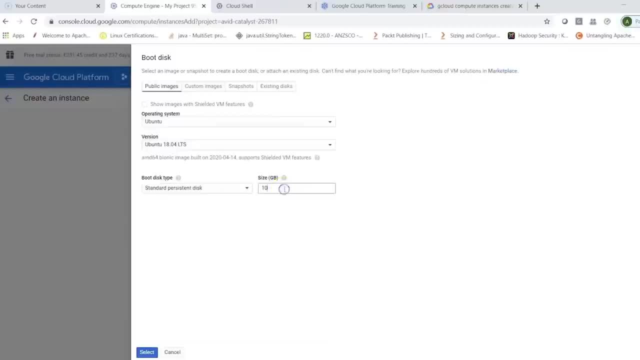 So as of now, we can choose standard persistent disk As it is and we can let the gigabyte be 10.. Now, depending on your requirement, you can increase this. You can even add disks later. That's not a problem. Click on select now. 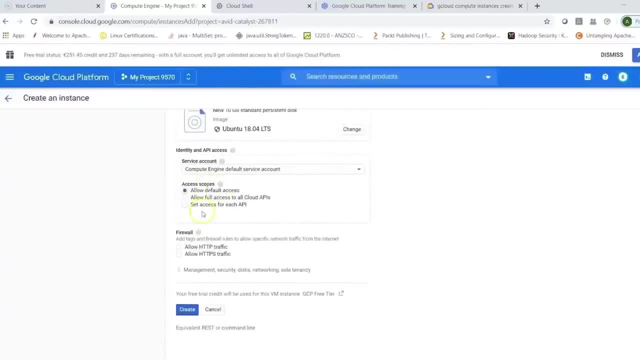 here I have access scopes, So here I will say: allow default access. You can also set access for each API, or you can give full access to all cloud APIs So that based on your requirement you can any time change later. also say: allow HTTP traffic. and we can also choose: allow HTTPS traffic. that basically allows me to 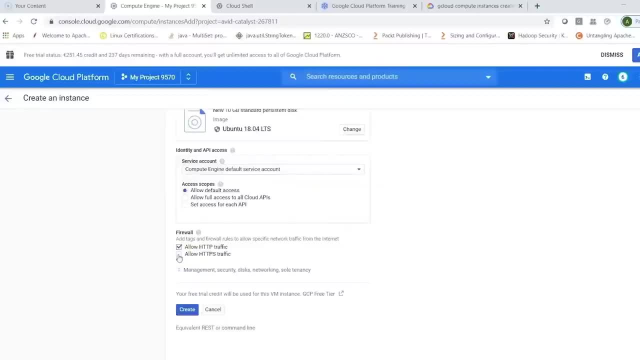 access this machine or services which are HTTP based accessible from this machine. Now I can just click on create. however, it would be good to basically enable connectivity to this machine Now. we can do that in different ways. one is: when you bring up your machine, it will have an SSH. 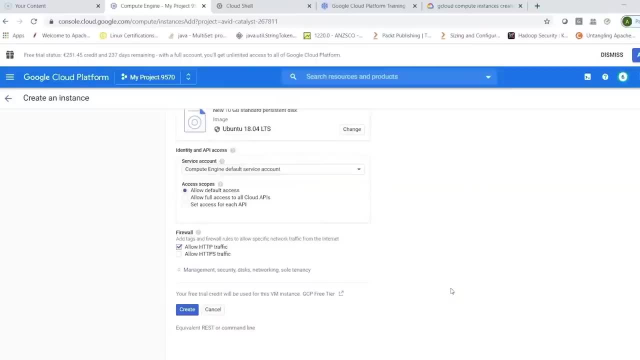 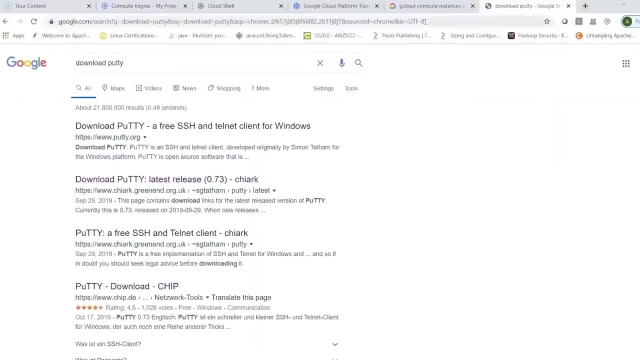 access which you can log in from the cloud platform here itself. or what you can do is you can create a private and a public key using some softwares like putty or putty gen. So, for example, if you do not have that on your machine, you can download. you can just type in download putty. 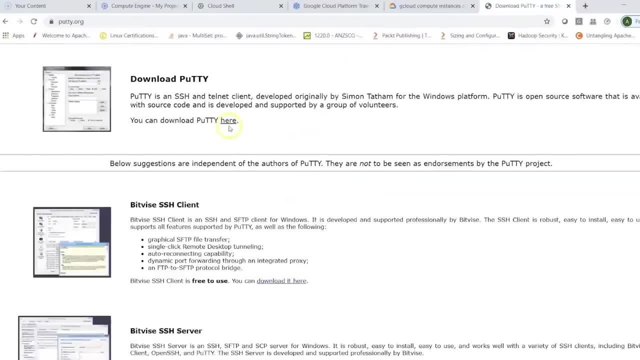 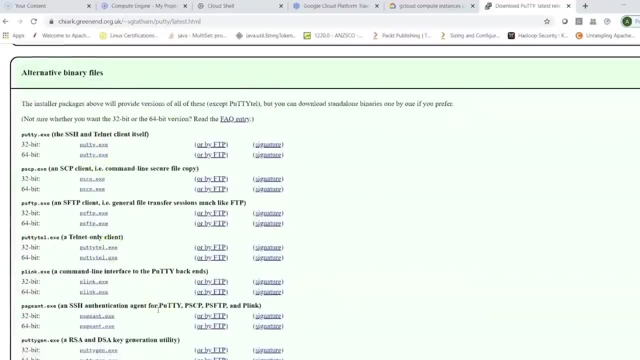 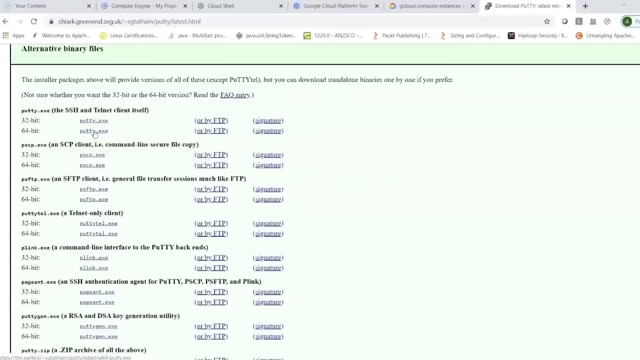 that takes you to the puttyorg page and here you can click on download putty and scroll down, which shows you. for your 64-bit machine, which I have in my case, You can download puttyexe, which is basically your SSH and telnet client to connect to your. 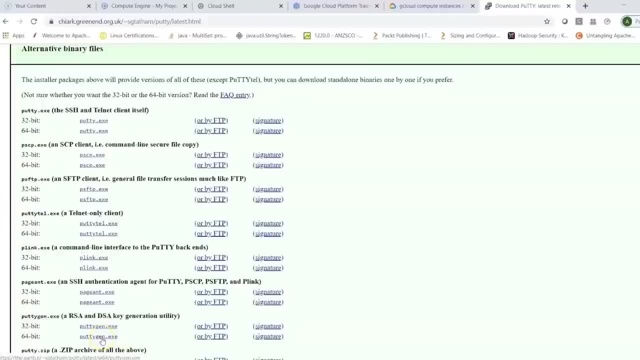 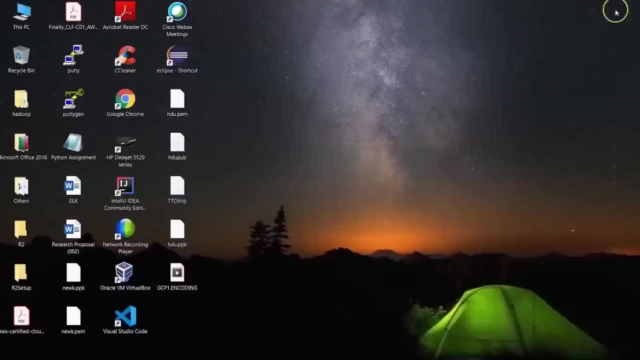 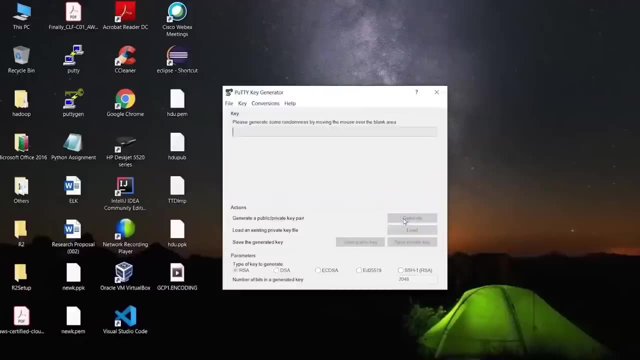 machines. You can also use putty gen, which will be allowing you to create a private and a public key, which I have done in my case. Let me show you how. So what you can do is you can go to putty gen to begin with, and here you can click on generate Now. then, to have this key generated, just move. 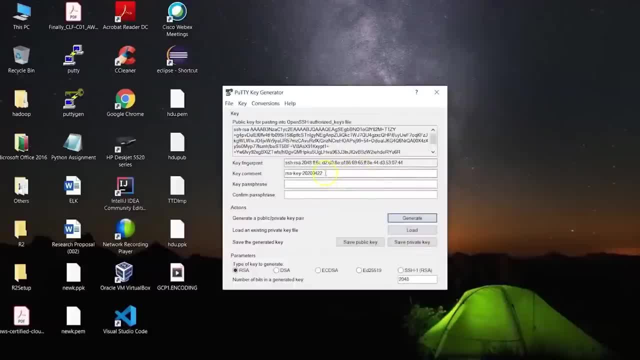 your cursor on the top here in the empty space, and that will allow you to create a private and a public key. So what you can do is you can give it a name. So, for example, let's give a user name. I would give HDEU. Now I can give a password. 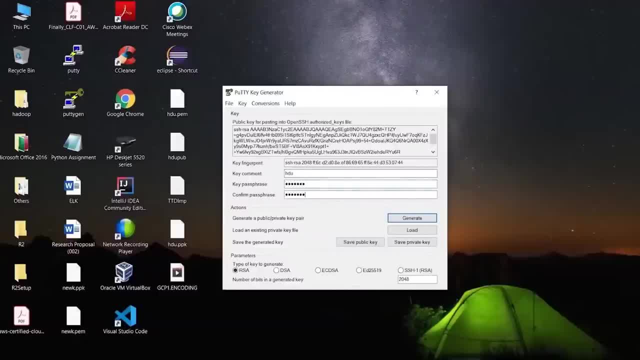 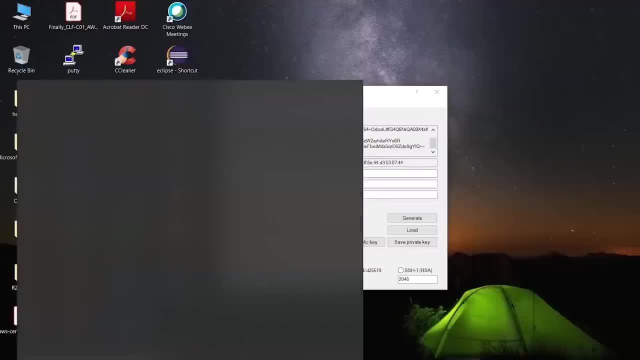 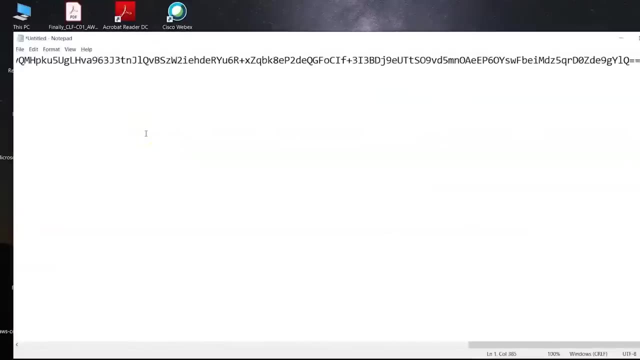 for this one. So let me give a simple password, and what I can also do is I can copy this public key from here and, for my later usage, I can just keep it in my notepad file, which I can use later, and I'll show you when. So now we can save this private key and we can go to putty genorg. 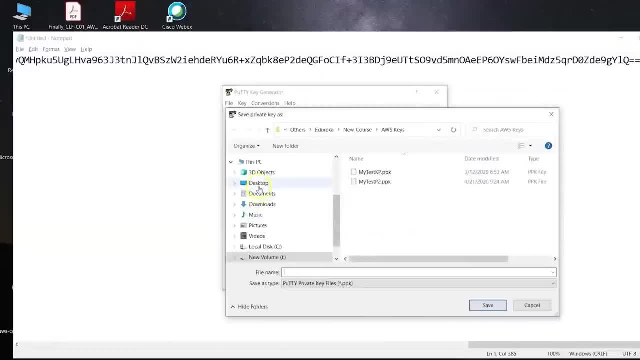 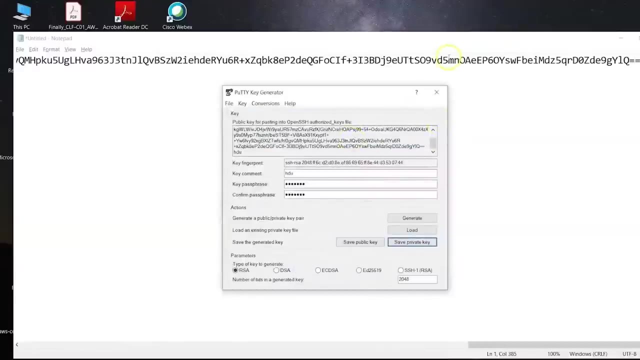 So let's save this private key, and this will basically allow me to save my private key. I can choose desktop and I can give it a name. So let's say new key, new key, and that will be getting saved in a ppk file. So let's save it and that's done. So we also have our public key and we have saved our. 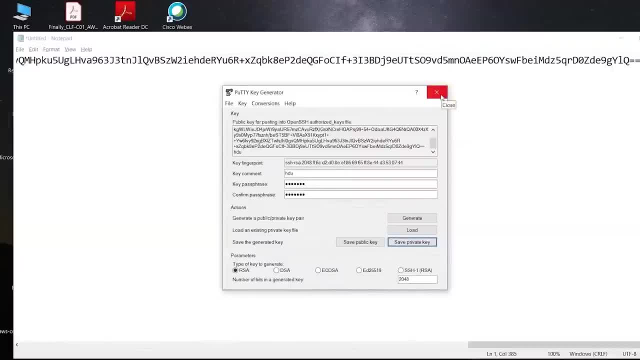 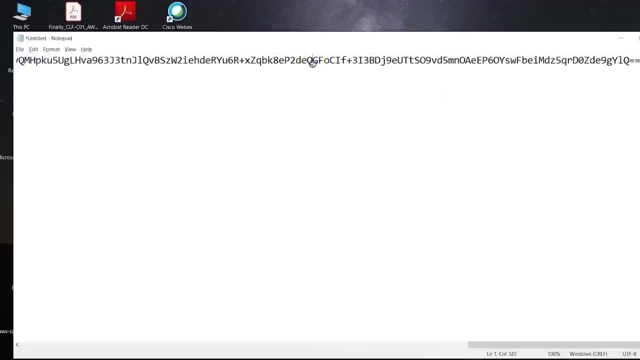 private key. Now we know that when you would want to connect using SSH, you need your private keys to the client and public key also has to be existing. So let's take this public key and we can give it a public key. So let's do a control a. I'm going to copy this and I'm going to come back. 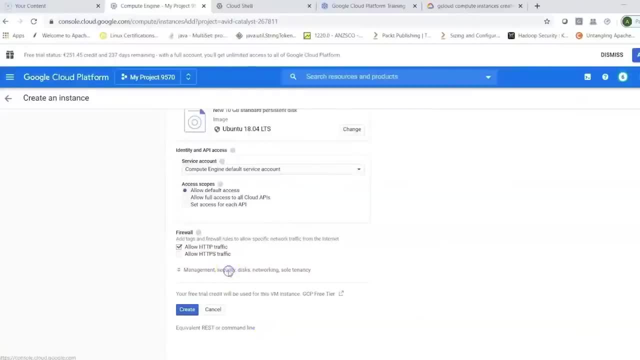 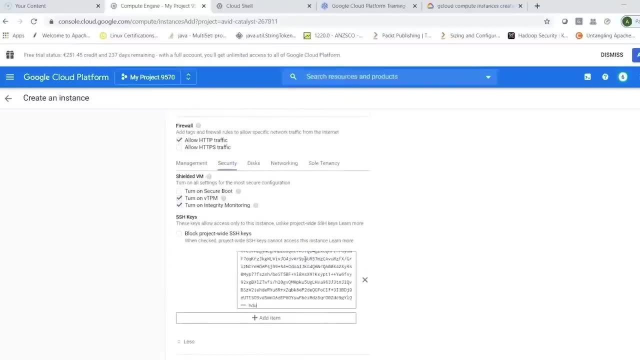 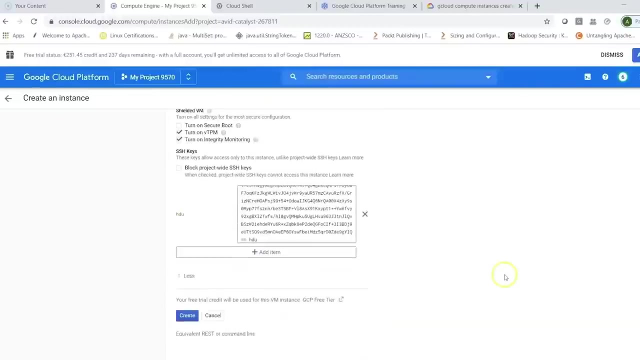 to my Google Cloud console and here you can click on security. So you can click on the security tab here, scroll down and just give you a public key. Once you give that, it resolves and shows you the name. and this is good enough so that I can use my SSH client to connect to this machine. I can click. 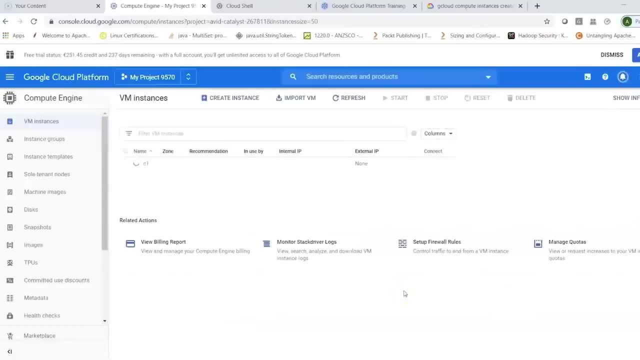 on create and this will basically create my VM instance. It will take some time and then your instance will have an internal IP which will show up here external IP and it will also show you options to connect to these machines. So this is my internal. 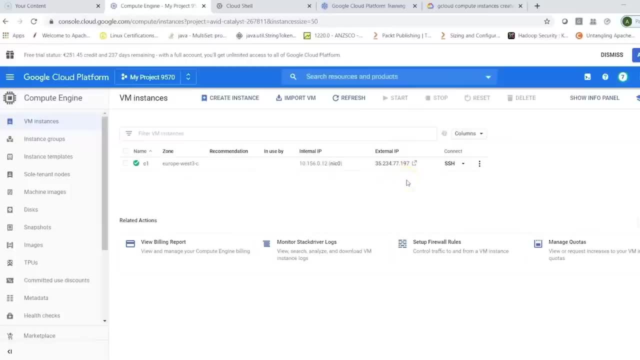 IP. This is my external IP which I can use to connect from a client. I can easily connect from the option here which says SSH and I can say open in a browser window. I can even open this in a custom port. I can look at the gcloud command which you. 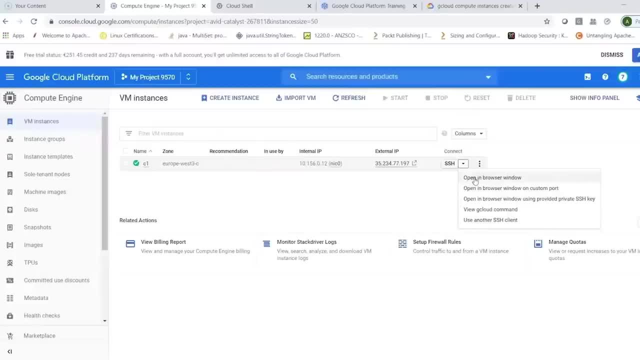 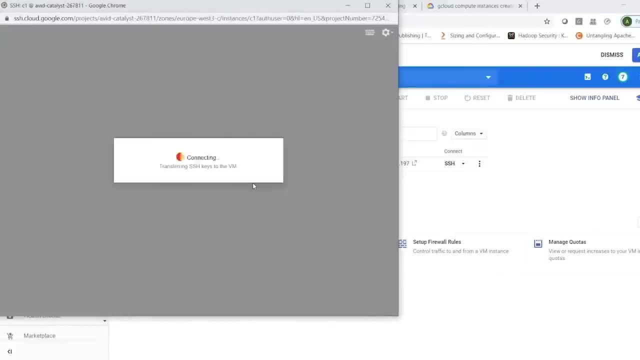 can give from Cloud Shell or you can use another SSH. So let's first do a open in browser window and let's see if this connects, So we can easily connect to our instance, the Ubuntu 18 instance, which I just set up here easily in a couple of seconds. Now this is trying to establish a 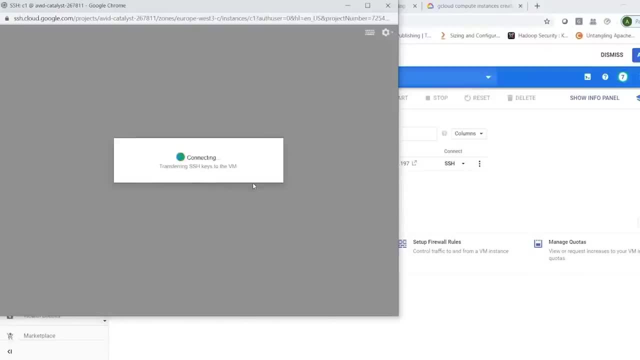 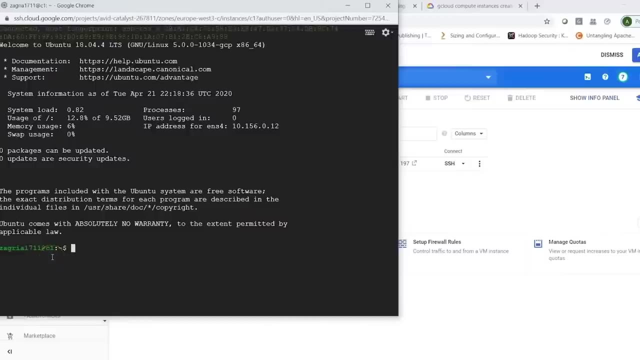 connection using your SSH keys, and when you do that, it also basically brings up this web browser, So I'm already connected. It shows my username, which is my cloud account username, and I have been connected to this machine here using SSH. It did not ask me. 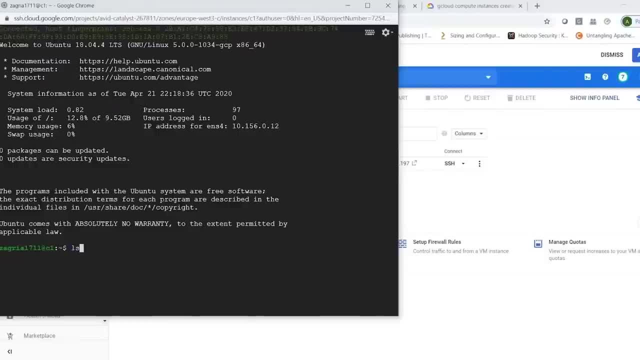 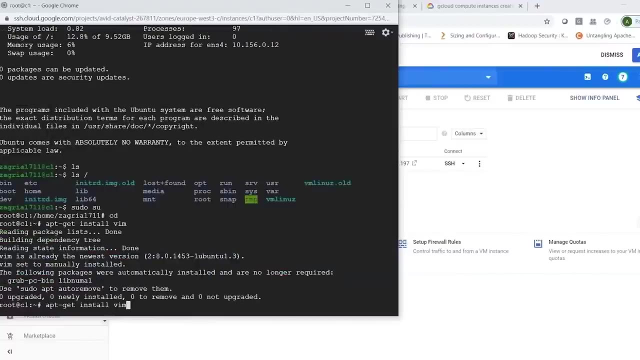 for any password and basically now I can just check what do I have in my Linux file system right, And I can anytime log in as root by doing a sudo su, For example. let's try installing a package and I can say apt-get install vim or apt-get install wget or apt-get install. 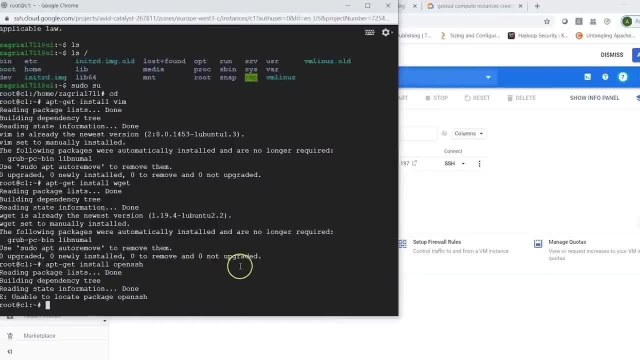 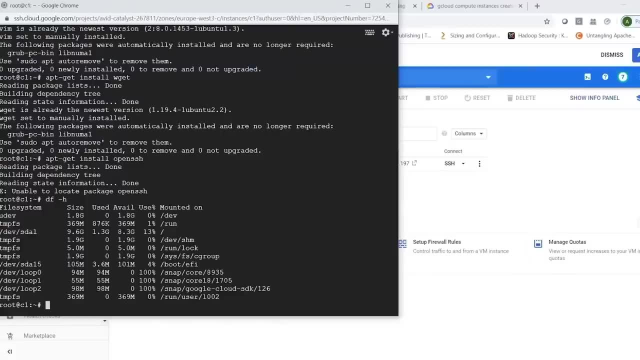 ssh and all these packages are already existing, So not an issue. Now I can start using this instance. I can just look at the disk. what is available? Okay now we gave around 10 gigabyte, out of which we see 8.3 gigabyte here for the dev sda1, and then 1.8 gigabyte available and you can. 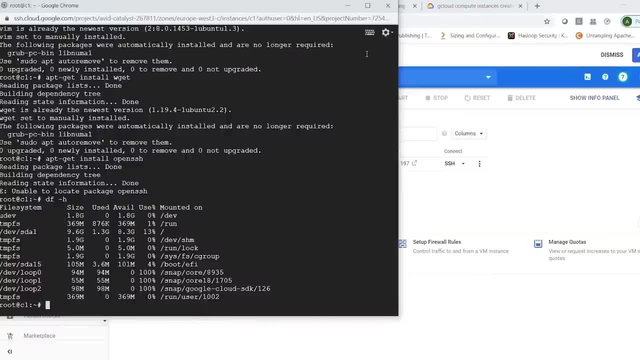 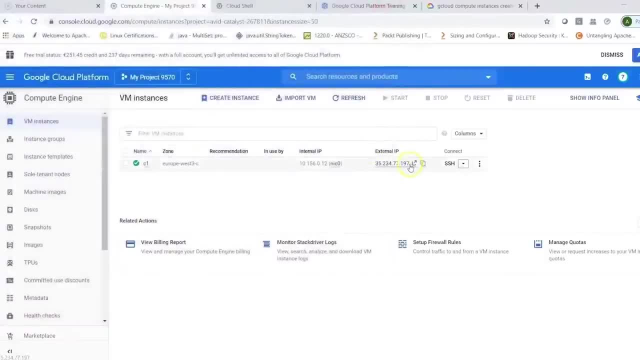 continue using this machine. This was the easiest way of connecting to a vm instance using SSH. Now what we can also do is I can just leave this and I will now try to connect using an external SSH client right, And here you can copy the public IP. So when you want to connect to an instance you will have to get the public IP. 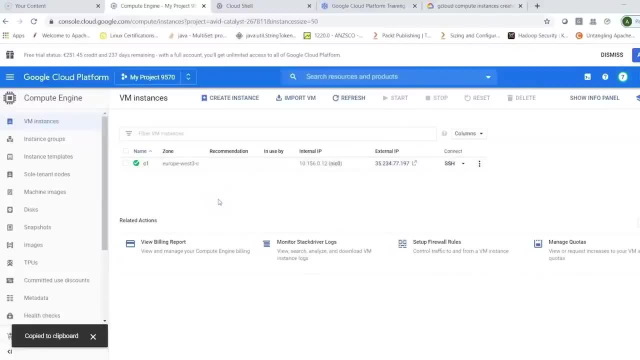 Also remember that if you select and stop this machine, which will stop your billing counter, and if you start it again, the internal IP will remain same, but the external IP is the one which will change. I can obviously select this machine anytime and I can just click on it and it will. 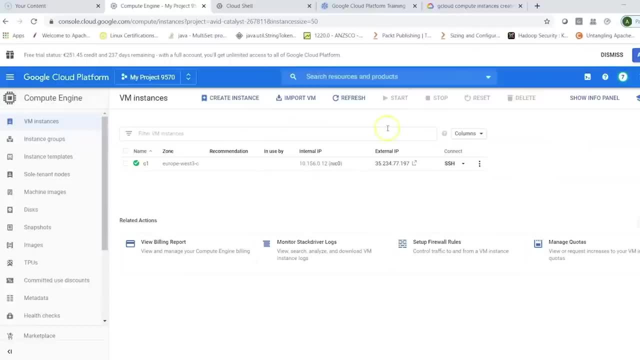 change. I can do a cleanup and I can delete it. I can do a start of the machine if it is stopped, and I can even import the virtual machine to be used later. So there are different options which you can always use. So this is my instance and if you would want to look at the details, 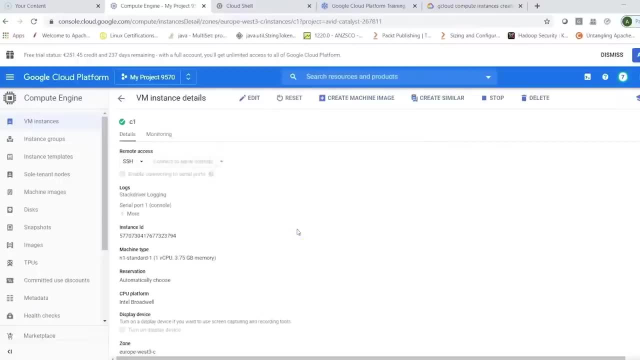 click on this one, C1, and that should basically allow you to look at the details. So it shows you what is the instance ID, What is the machine type, Is it reservation Specific, What is the CPU platform, What's the zone And all the other details At any point of. 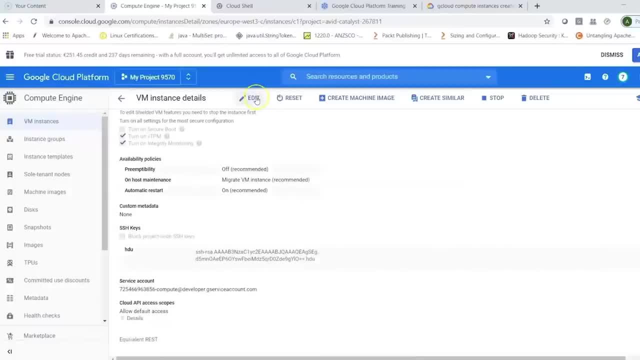 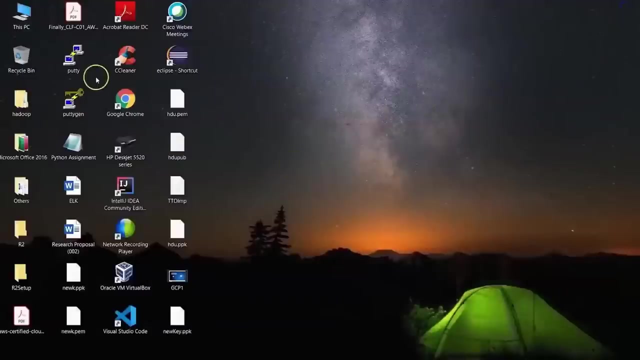 time. if you would want to edit, you can always click on edit and you can change the details as you need. Now you can also look at the equivalent REST command to basically use the REST API to connect to this instance. For now, I have copied the public IP and I would want to connect it using 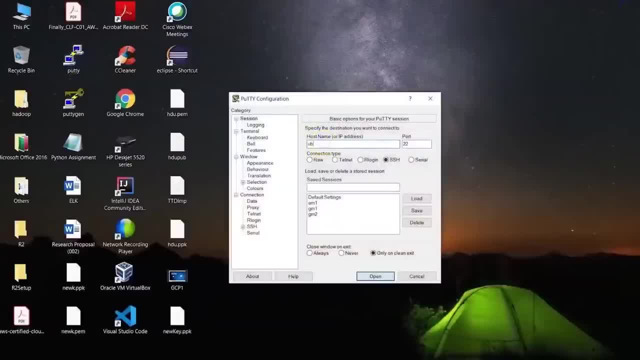 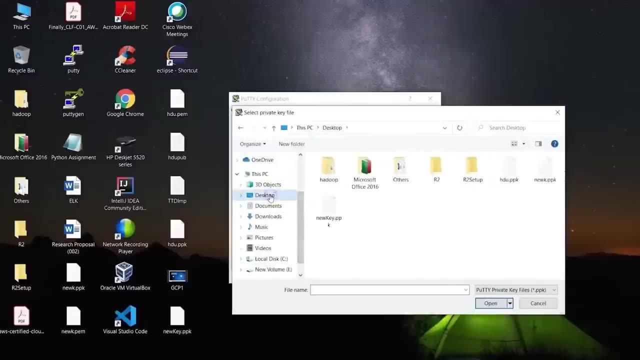 Putty. So let's go in here and let's give it the host name So I can give Ubuntu, I can give my IP address. So that's in my session. Now I will click on SSH, I would go into authentication, I'll click on browse and this is where I need to choose the PPK file. So this is. 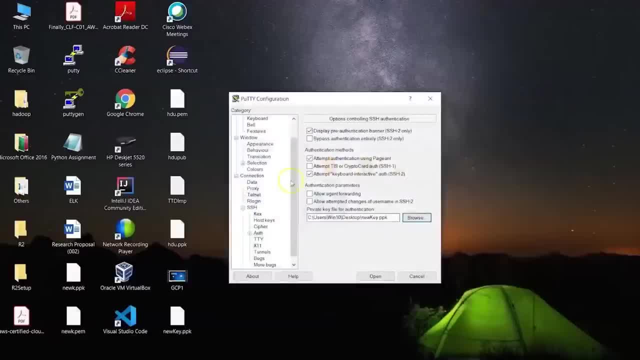 the one which we created new key. Let's select this and then I can come back to session. I can even save this and I can call it as my instance one. Let's save it and you can create any number of instances. So you see, I have created my instance and I have created my IP address. So 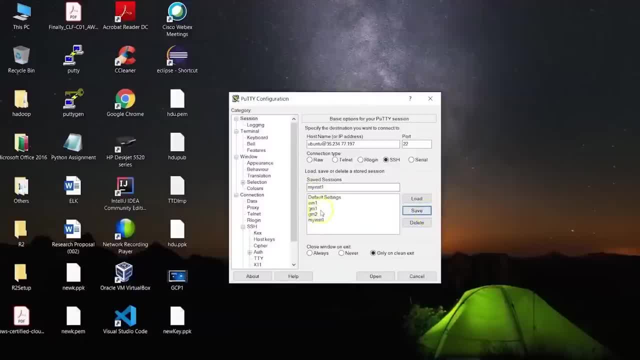 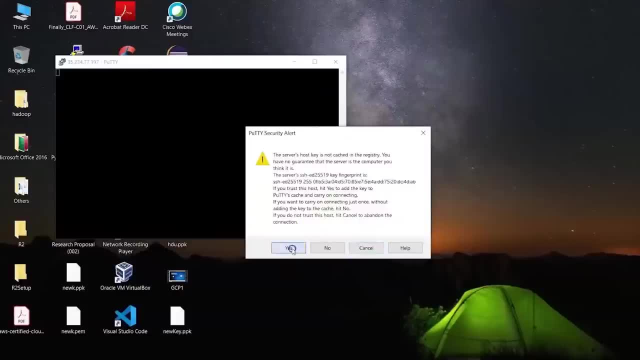 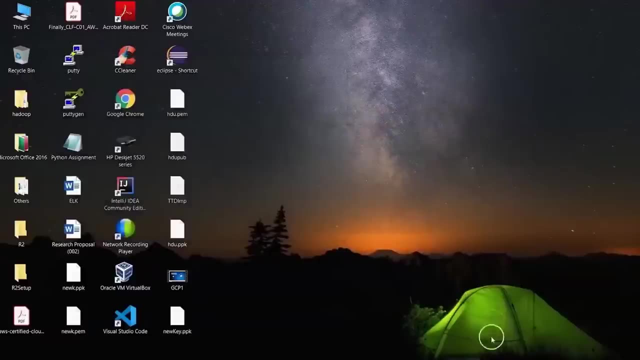 I have created different instances here for my Google Cloud or Amazon related instances and I can click on open. It says the server's host key is not cached in the registry. That's fine. Just click on yes and basically it says no authentication method supported. Now this could be because we 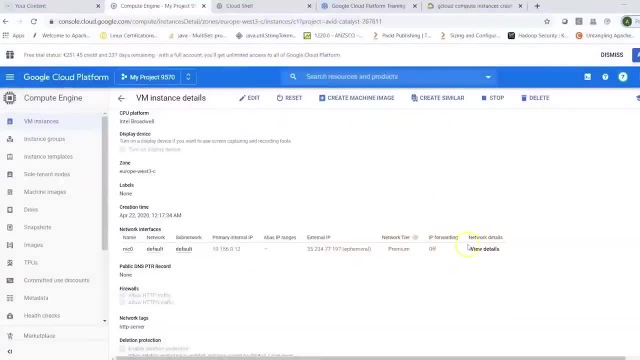 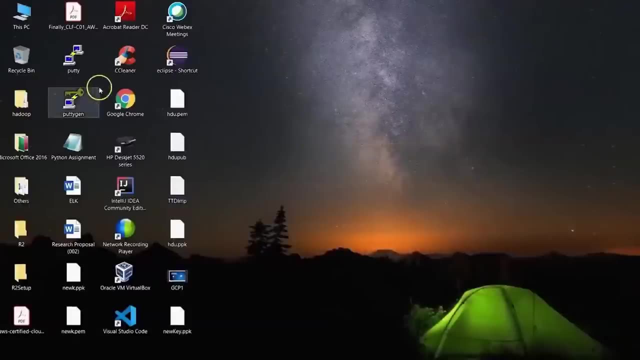 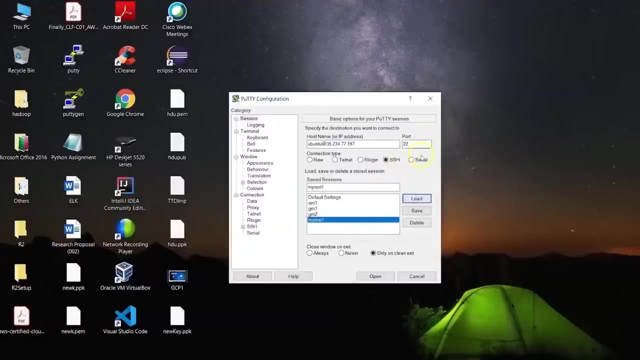 have not enabled your SSH access. So let's look at that. So now let's see if we were trying to connect using Putty, What was the issue here? So if I go to putty, I can see that I have a network connection. So I can go back to my Putty, select my instance, load it. It says port 22.. I'm 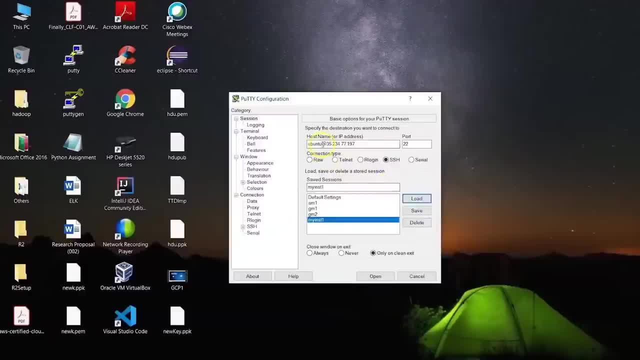 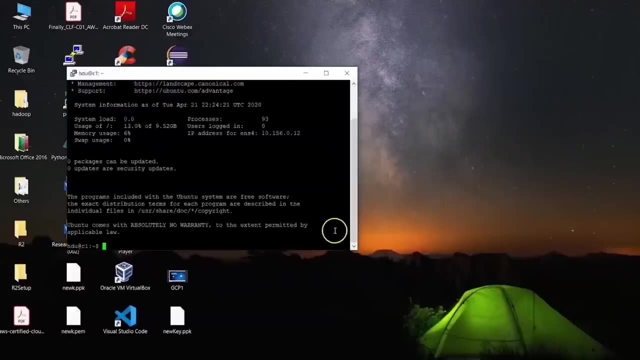 giving the username, which is Ubuntu, or? sorry, that's the wrong username we gave and that might be the reason we had set up the user as SDU. So let's save this again. and now let's try connecting to this one, and it asks for my password and you are able to connect this right Now, if there was. 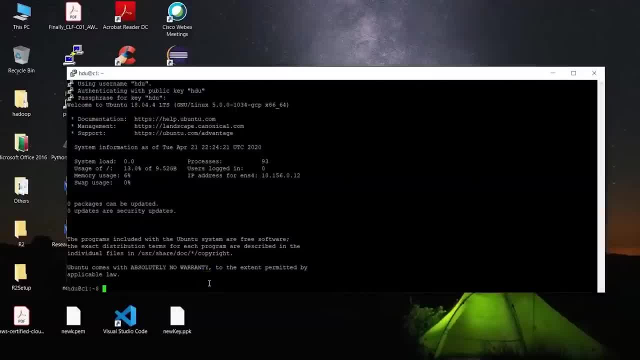 any other issue related to network connectivity, you can click on yes and then you can connect to the call and your DNS bulking out for a zero cache activity. Then we could look at the rules- the inbound and outbound rules- which allowed us to look into the machine. Now we are. 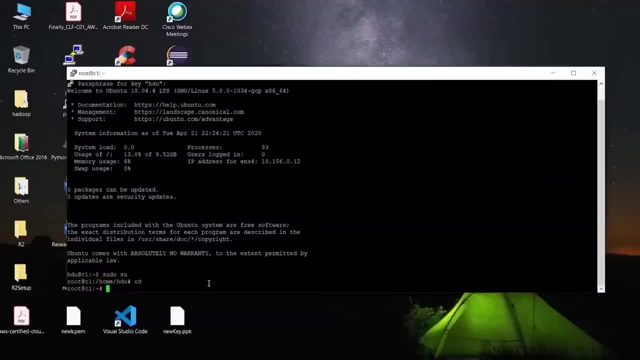 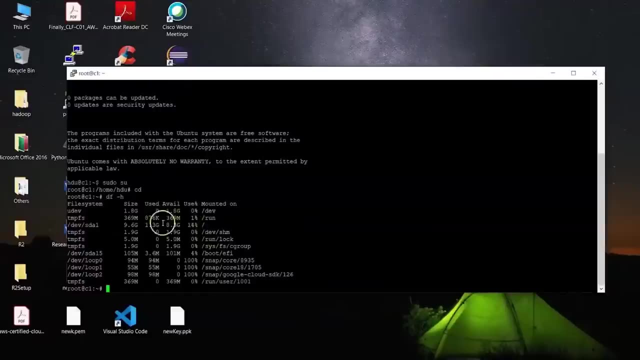 connected to our machine. here, using HDU user, I can log in as root and I can continue working. So not only from the SSH within the cloud console, but you can use an external SSH client and connect to your machine. So this is your Ubuntu machine and we. 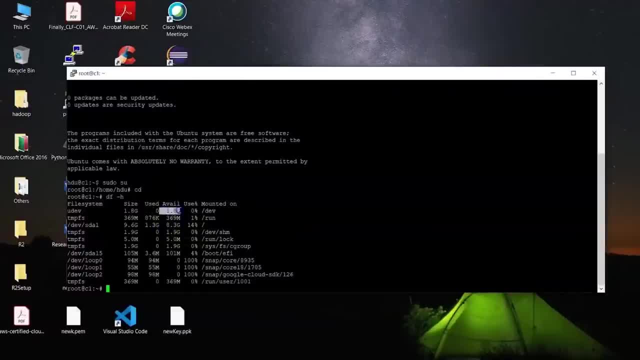 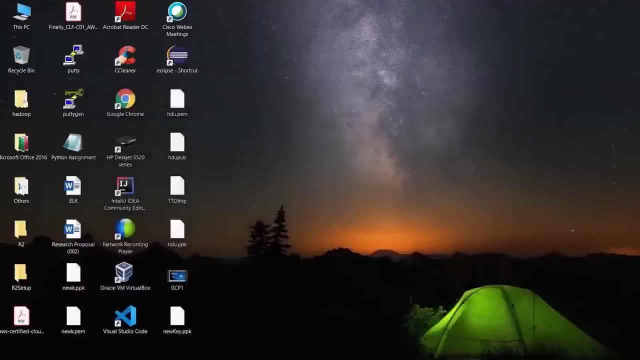 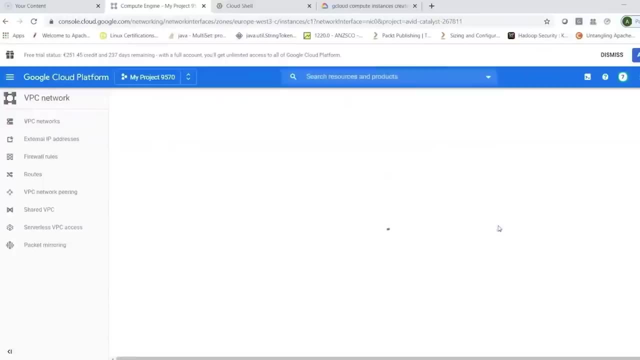 to the same machine which shows 8.3 gigabytes here and 1.8 gigabytes here, which we were seeing from the ssh in the browser. now let's close this and let's go back to our instance page. now here you can always look at the network details and this will show you your different kind of rules. that 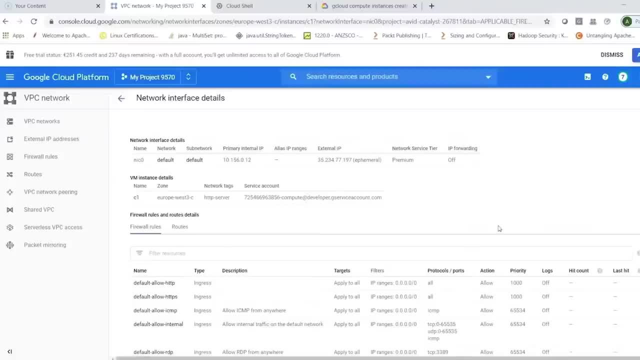 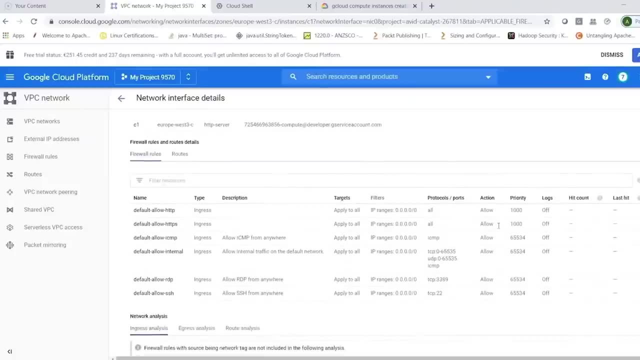 is ingress or egress rules, which basically allows to connect to this machine from an external network or for this machine to connect to an external network. so here we have different firewall rules. which shows default allow http. that's your ingress rule and it tells you apply to all. it shows me. 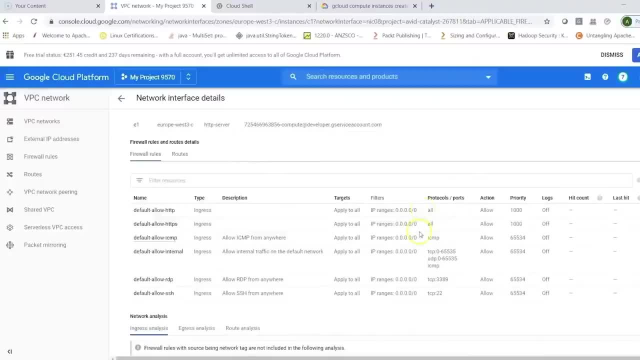 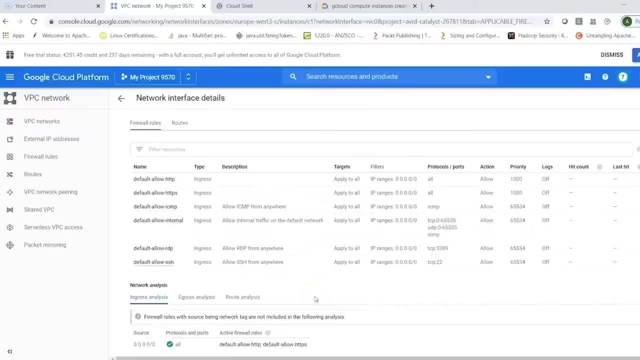 what are the ip ranges where i can specifically give the ip of my machine. it shows the protocols. it shows what are the different ports which you have used for these services, for example rdp or ssh, which shows 22. you have icmp, http and http gdps. now, anytime, if you would want to make a change to these rules, that can be done by going. 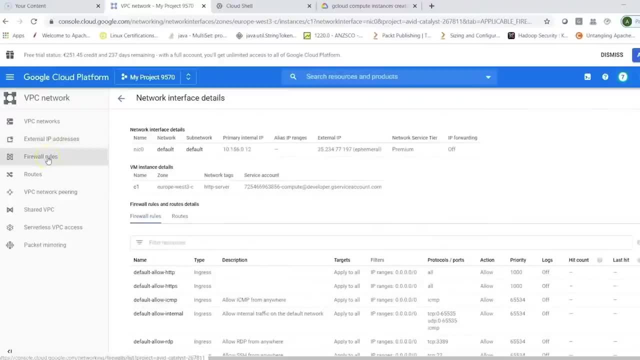 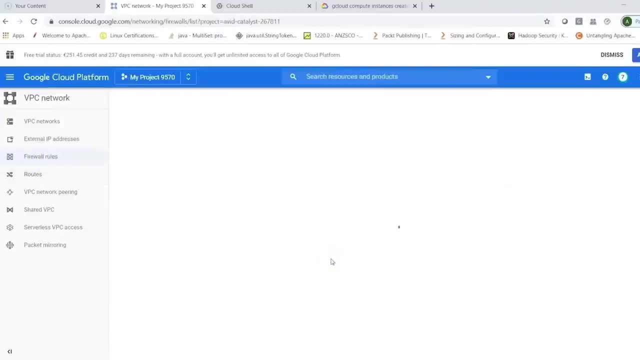 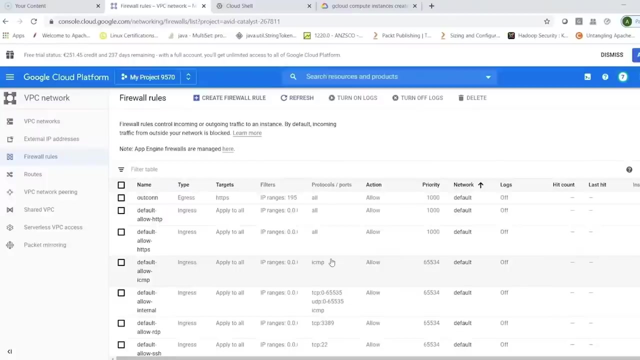 into your network details and say, for example, you would want to work on firewall rules, so we have these firewall rules here, you can click on this one. so right now we are looking into the network domain and we are looking into vpc network. right, and this shows me what are the different rules we 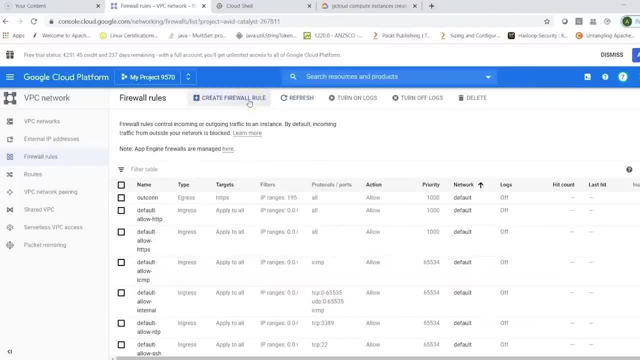 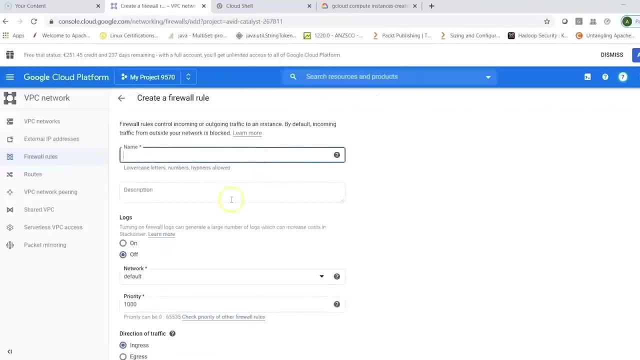 have. now. if i would want to create a different network, i would want to create a different firewall rule for a different protocol. i can always click on create firewall rule. i can give it a name. okay, i can say what. if you would want to turn on the firewall logs, you can basically say: 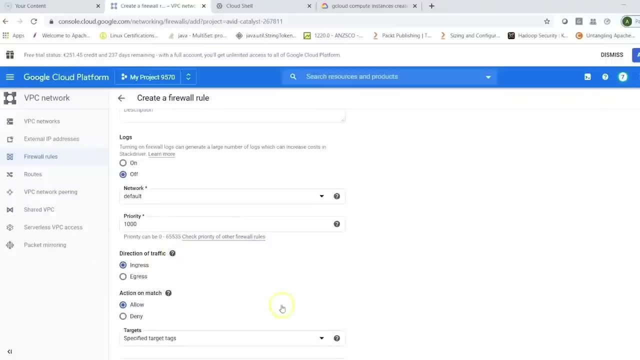 what is the kind of traffic. so ingress applies to incoming traffic and egress applies to outgoing traffic, and you can then basically choose what are the ip ranges, from where you want that connection to be, coming in or to going out. you can choose the genre you want that connection to be. 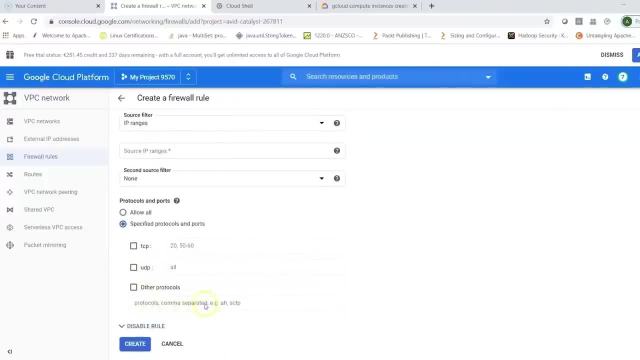 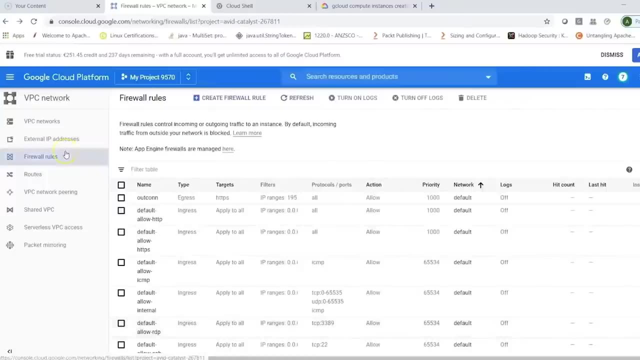 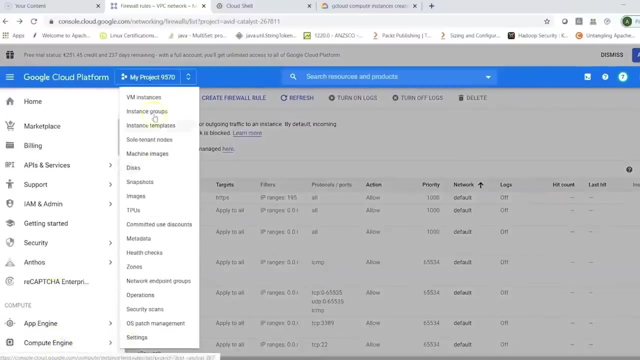 a particular protocol. you can give a protocol here with comma separated values and you can create a firewall rule. so this might be required depending on the services which you are running wherein you might want to enable your access to your machine from an external service or to an external service. so you 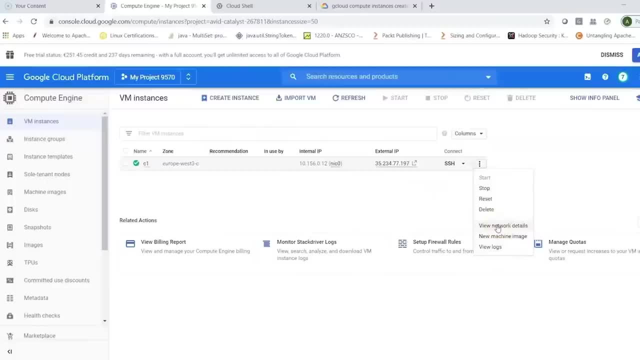 can always go to network details from here. you can then go into firewall rules, create a firewall rule, apply that to your instance and restart your instance. so as of now we don't need to create any network details here, because my ingress or egress rules are already available right now. I can basically then have my 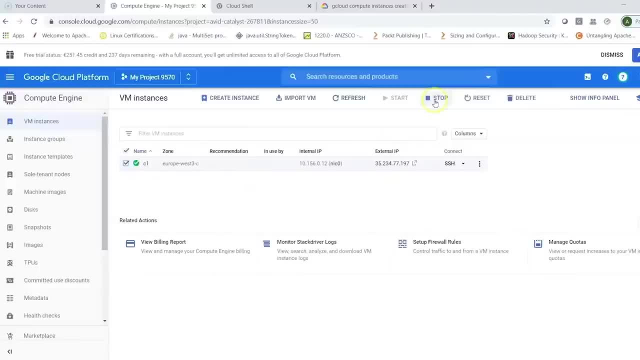 instance, stopped and removed so I can just do a stop. or, since this is running, the ideal way would be to do a stop- I could also do a reset. now, what does reset do? reset does not basically delete the machine. what it does is it does a cleanup of the machine and it. 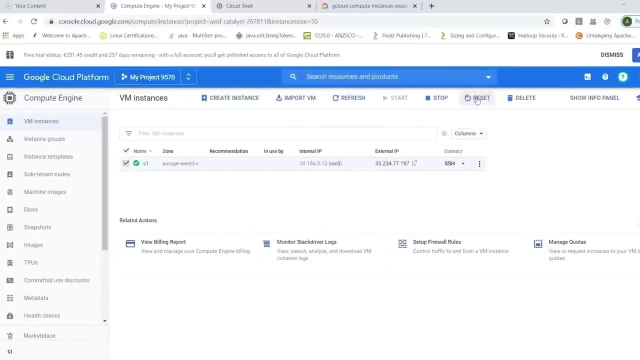 brings it to the initial state. so sometimes we might have installed certain things on our machine. we would want to clean them up and at that time reset can be useful. I can basically click on delete right and I can select this and I can do a cleanup. and this is good. always when you are using a free. 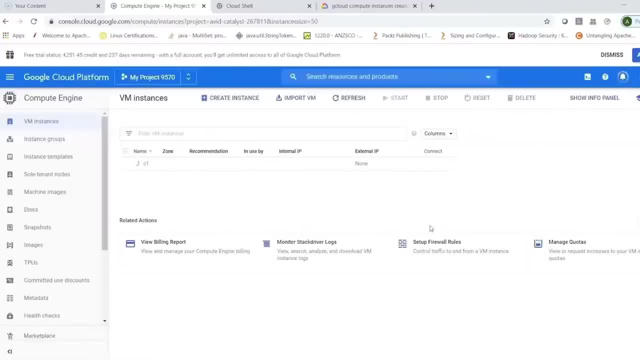 trial account. try to use different services, play around with them, and then you can clean up so that you do not. you can clean up so that you do not waste your free billing credit right and you can use it for meaningful stuff. now I have clicked on delete and, within a few seconds, my instance, which I had 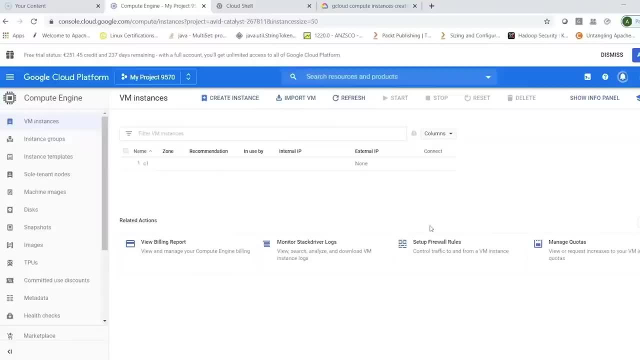 created will be deleted. also to remember is if you are creating multiple instances, then you can connect from one machine to other machine using SSH, by using the private file. so for that we can learn in detail later. so this is just a simple example of using your compute engine, creating your instances, connecting to it from an internal SSH or 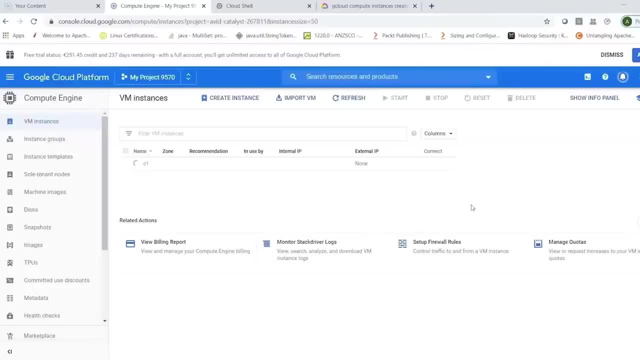 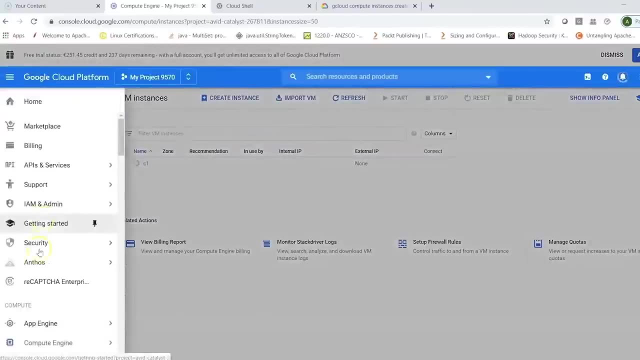 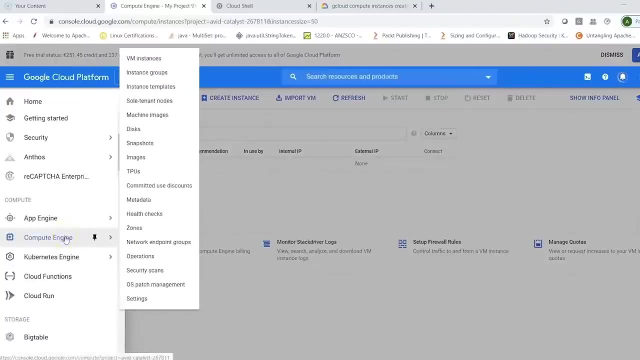 from an external SSH client, such as putty, where you have already created your private and public keys. now I can click on the browser here and then I can basically come out and I can basically be looking into any particular service. so we just looked into compute engine. right, you have different, other options. you. 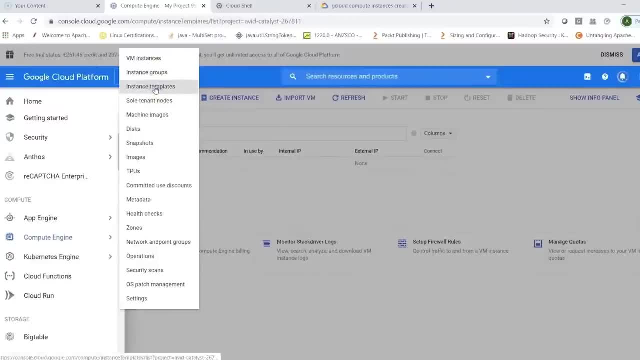 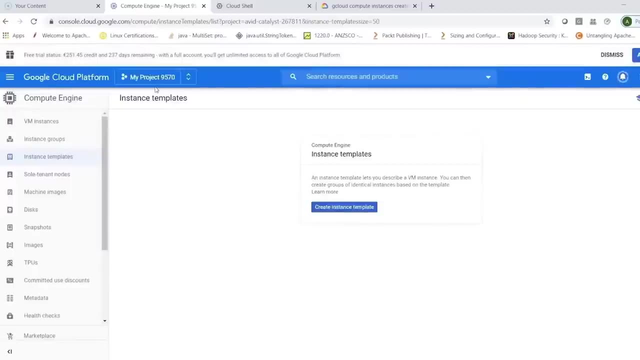 have instance groups. you have instance templates, for example, let's click on instance templates here and that basically shows you that you don't have any instance template and this basically facilitates. say, for example, you are working as a admin and you would want to create an instance template. so 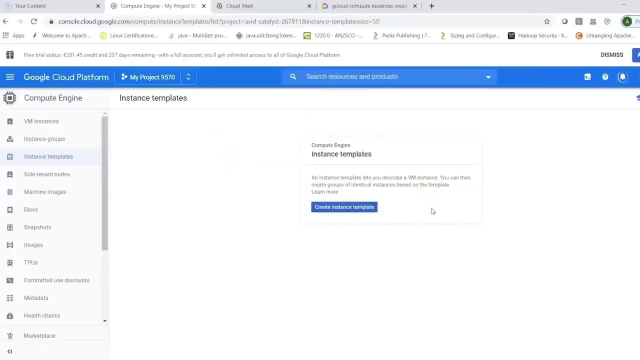 that using that, you can describe a VM instance, and then you can basically use this template to create different instances. you can go for sole tenant nodes, you can look for machine images, you can also look at your tests, you can create a snapshots and you can look at different options here. now let's come. 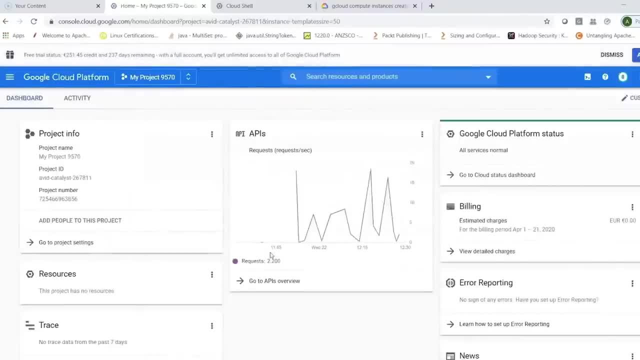 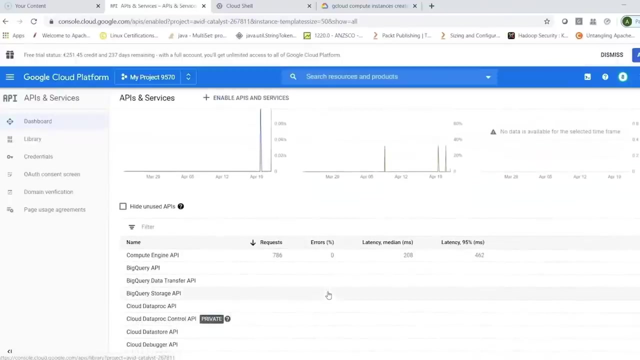 back here and let's click on home and that should take you back to your home page, which basically shows you if a particular API which you have used recently, which shows me in the graph here so I can go to the API's overview- right, and that basically shows me if there were any errors, if I was using the. 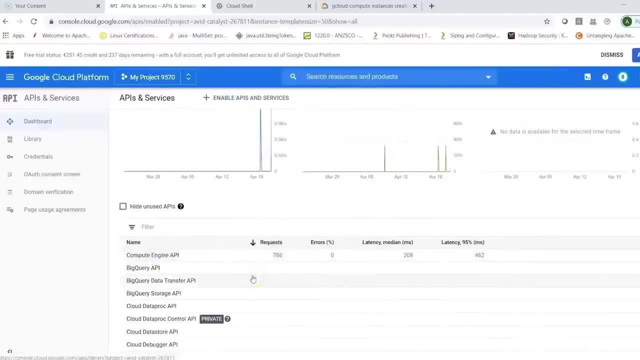 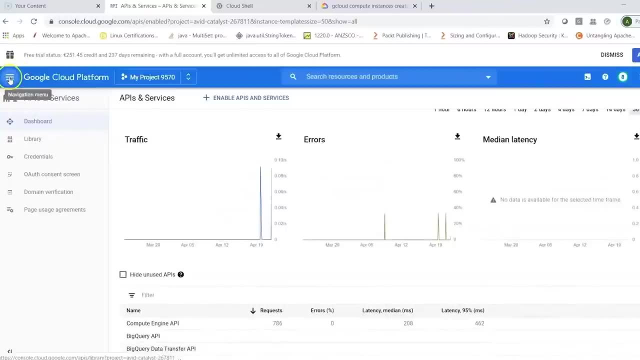 compute engine API to basically create a VM instance, and that's why we were seeing some spike in that instance and that's why we were seeing some spike in that instance and that's why we were seeing some spike in the graph. so this is a quick demo of using your compute engine service. 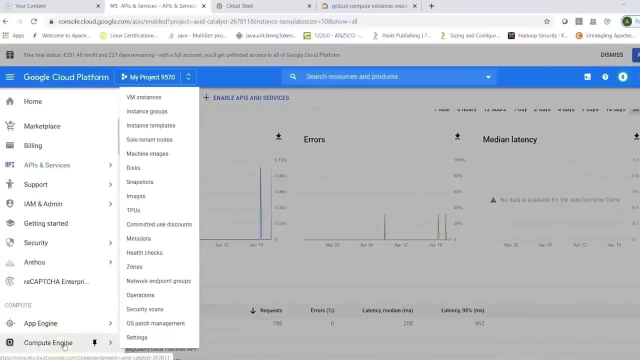 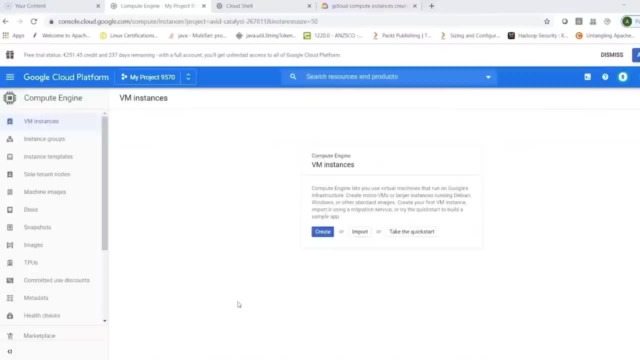 provided by Google Cloud, wherein you can create VM instances and use those VM instances for your application installation for any other purpose. now that we have seen how you use your cloud console to create an instance and also clean it up, let's also understand how you can do using your command line. 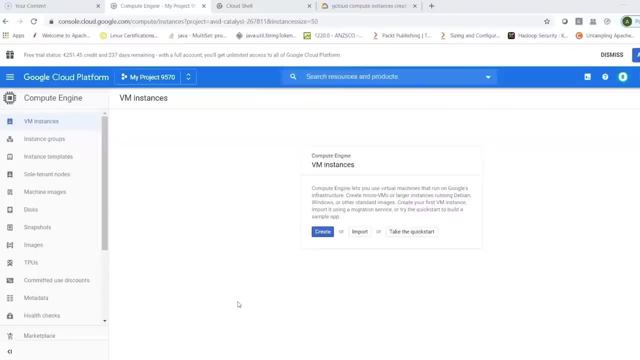 options and let's see what it takes, or what are the different commands which you can use to create your instances. now, you can always win. when you are creating an instance, you can use compute engine which provisions resources to start the instance. so instance basically has different states which we can see when. 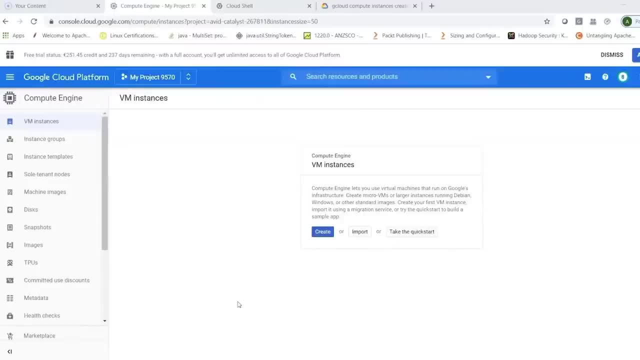 we are creating the instance, so you basically start the instance instance moves into staging, that is prepared for your first boot, finally in boots up and then it moves into running. so when you look at instant states, which we will create instance and see it will basically have different states, such as provisioning, where the sources are being allocated. 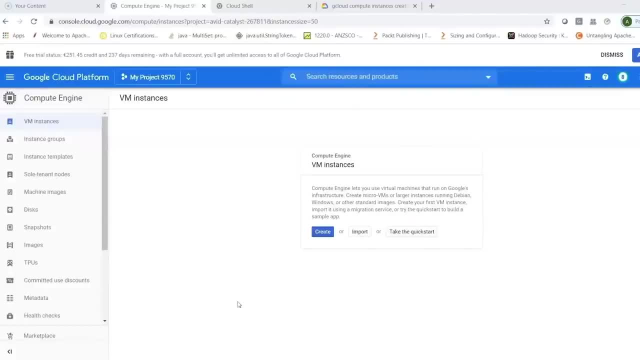 for instance, but instance is not yet running. then it goes into staging, where resources have been acquired and instance is being prepared for your first boot. then instance is booting up and running and if you are stopping an instance it goes into being stopped status and it would be moved to the. 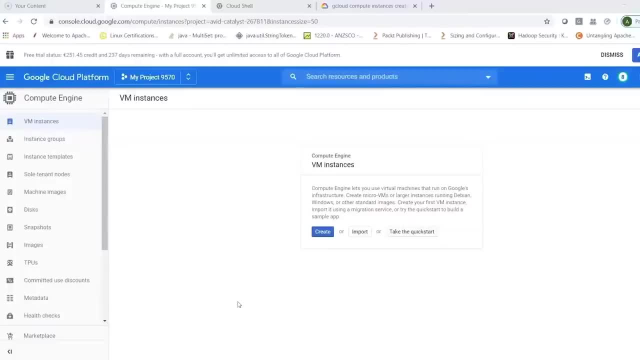 terminated option. You can also do a repairing of instance and finally, you can terminate your instance or clean it up by stopping and then deleting it. Now, when you say stopping and resetting an instance, you can stop the instance, as I showed earlier, if you no longer need it. but 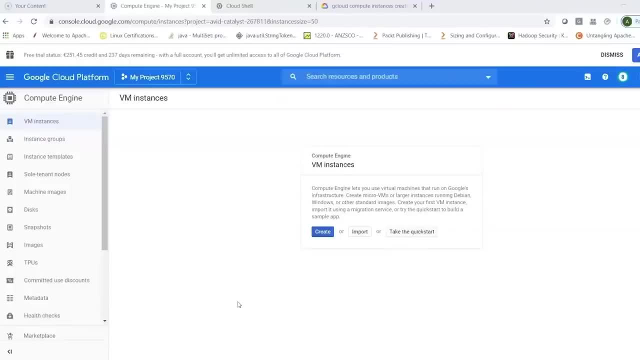 if you need for future use, you can just use the reset option, which will basically wipe the contents of instance or any application state, and then, finally, you can stop it and have it terminated Now, when you would want to do that using your cloud console. we have seen the options. 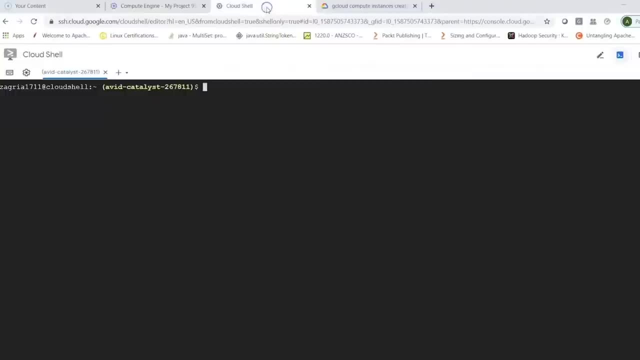 now let's also see from the command line tool how you can do it. So here I have the cloud shell which I brought up from here and I basically opened it up. and now I have the cloud shell which I brought up from here and I basically 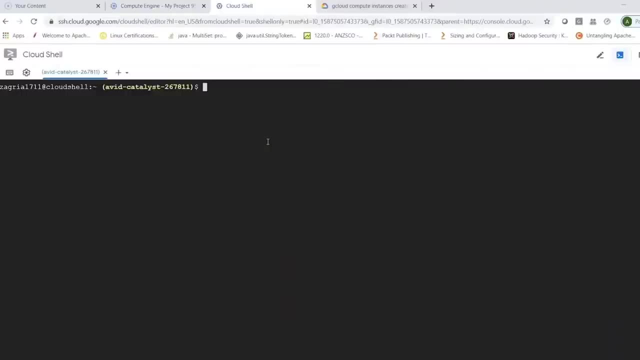 opened it up and now I have the cloud shell which I brought up from here and I basically it in a new window. So command line tool enables you to easily manage your compute engine resources in a friendlier format than using your compute engine API, Now gcloud, which is part of cloud. 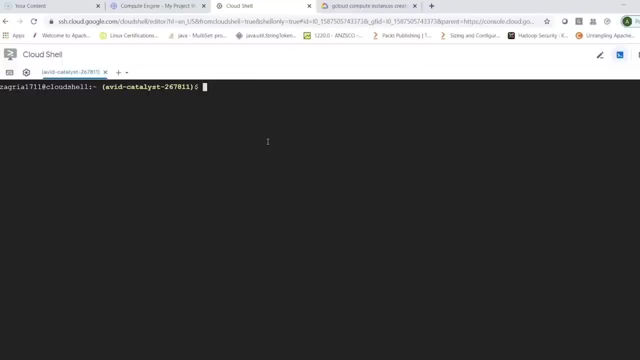 sdk is the main command here and then you can always auto complete the different options here. So when you would want to create or work on gcloud, you can just type in gcloud here and then for example, I could just say: help to see different options of gcloud which will show me different. 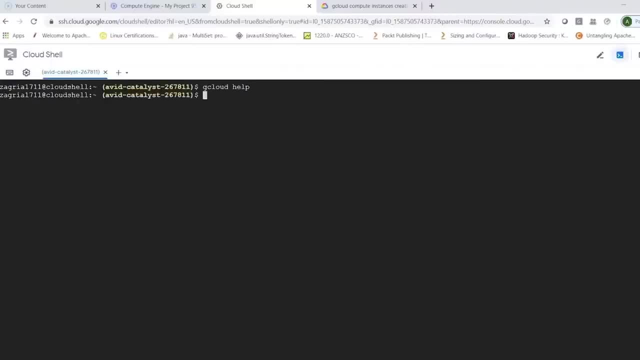 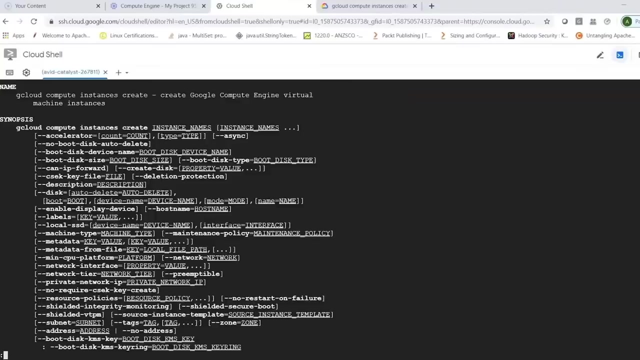 options which you can use here. Now we would be interested in compute instances so I could also do a gcloud compute compute instances and then I can basically say create and then I can do a help. Now that should show me different options which work with gcloud compute instances: create command. 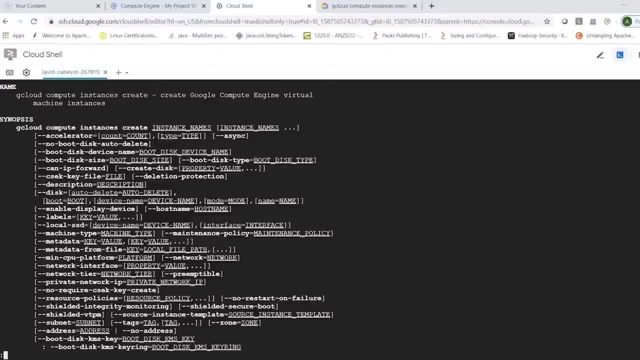 which is a command that I can use to create a gcloud compute instance, and then I can also do a gcloud compute instance create command, which is expecting an instance name. So your google cloud sdk, which we can set up on our windows machine or even on your linux machine, is set of tools that 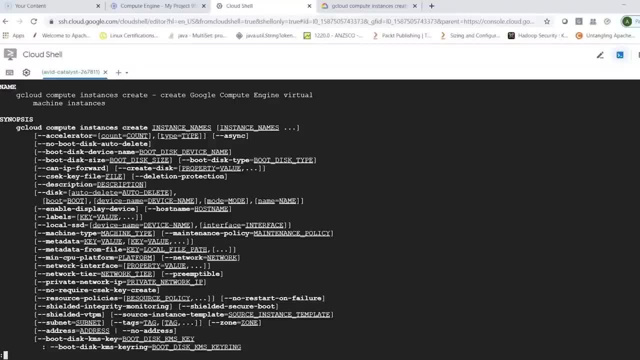 helps you to manage resources and applications hosted on your gcp. that is your google cloud platform. Now, here you have options such as gcloud, which I'm showing you right now. you have gsutil, and then you have bq, so that also can be used, So you can. 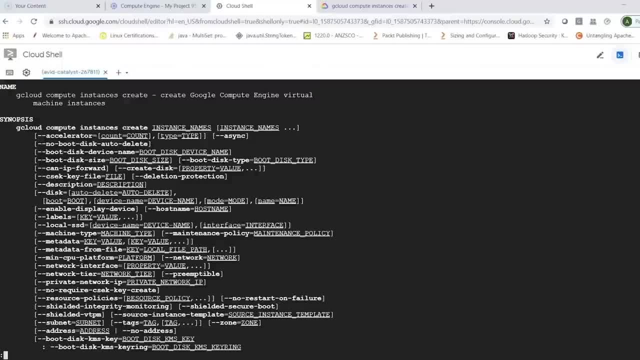 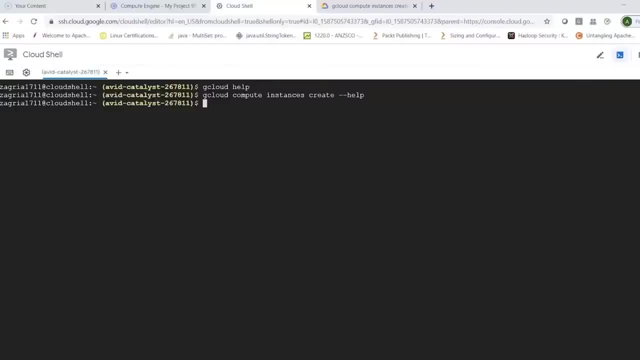 set up a google cloud compute if using gcloud. now what we can do is if we are setting up our sdk on our windows machine, then we would have to do a gcloud init which basically initializes your configurations for gcloud. Now here we are, using a cloud shell which was started from the console. 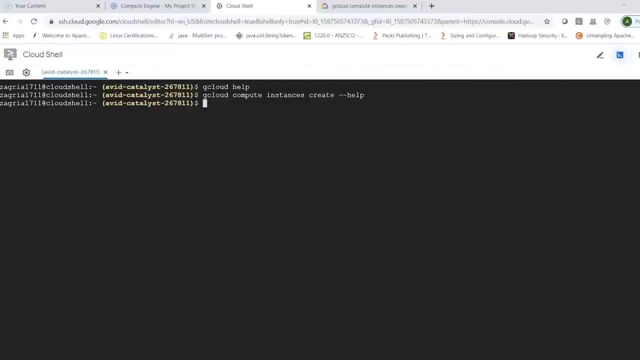 and we don't have to basically give your gcloud init command because it's already initialized Now. you can always look at your default zone, you can look at your region, what is being used? all those things are coming from the metadata which is being used. So, for example, 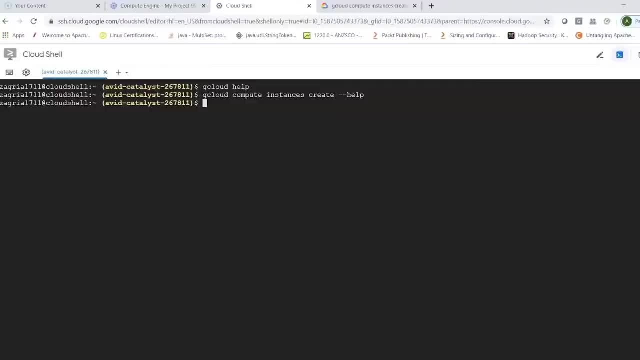 I could be looking at the metadata for my particular project by just doing a gcloud and then I can say compute, and I would be interested in project info. so I can do it can just do a project minus info and then I can do a describe and then I need my project ID. so I 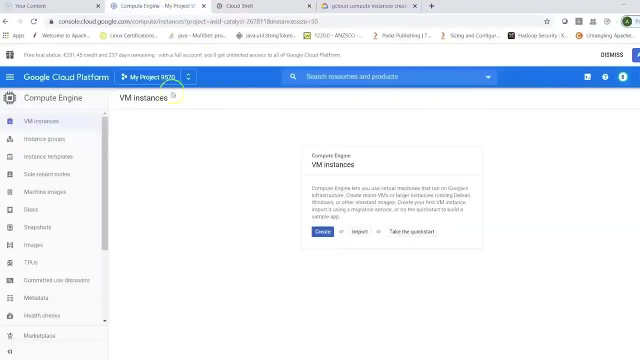 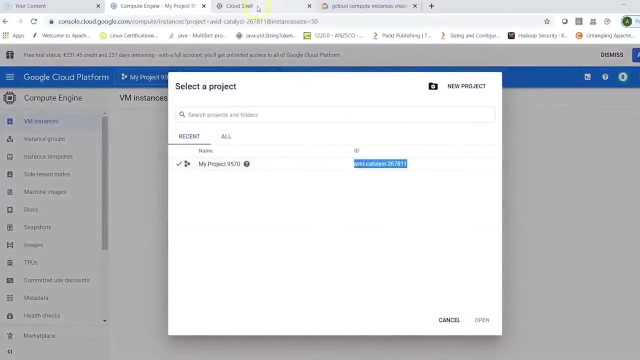 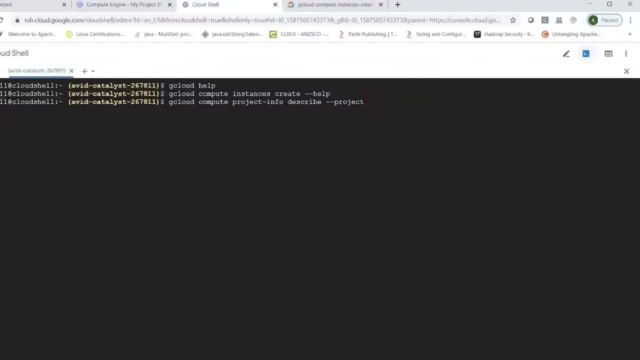 can say minus, minus project, and I can get my project ID from here. so you can click on this one and that's my project ID, so I can click on this one, and here I can just do a right click, and if it does not paste, then you can do a ctrl v and then I can try to look at my project info. so this: 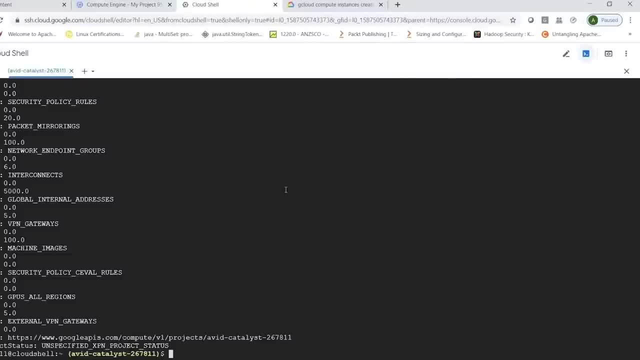 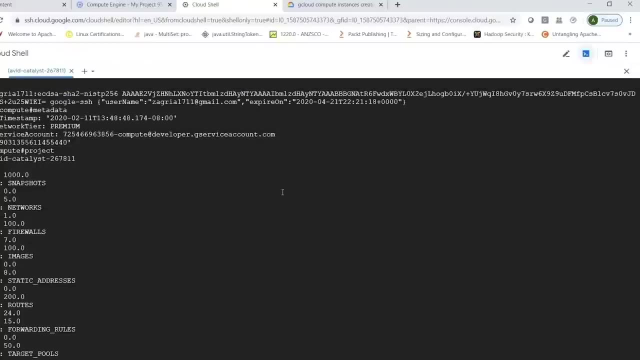 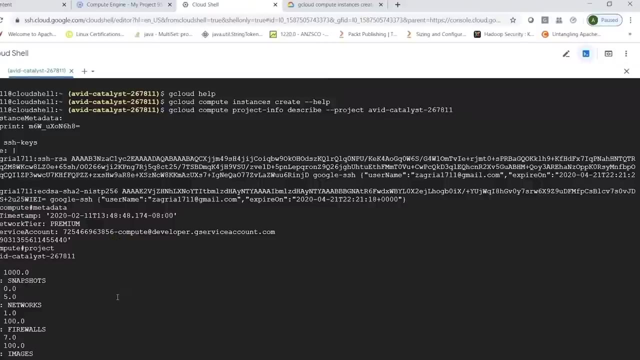 basically will give me the metadata which is by default set and we can always look at what are the regions or what is the zone which has been set. so if it has been set, so I'm looking at my details, it is showing me my ssh keys and then it can be using your default region and your default. 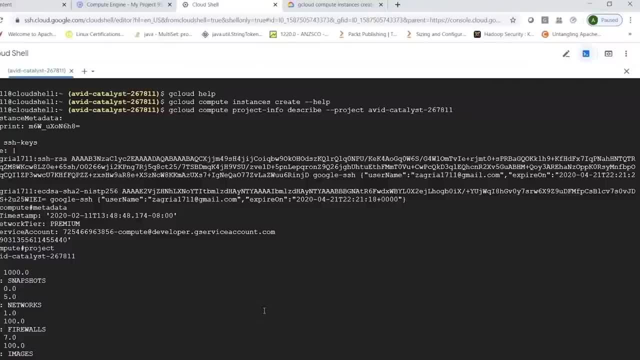 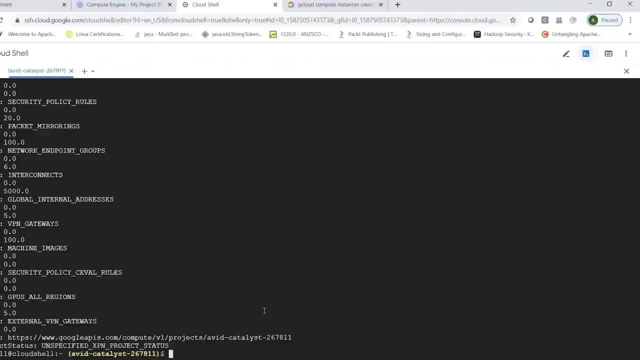 everything Available zones. it also shows my username and other details. so this is basically to look at the metadata which is available now. at any point of time, I can basically say add metadata. I can basically choose metadata option and I can say my default region should be Europe, which I was. 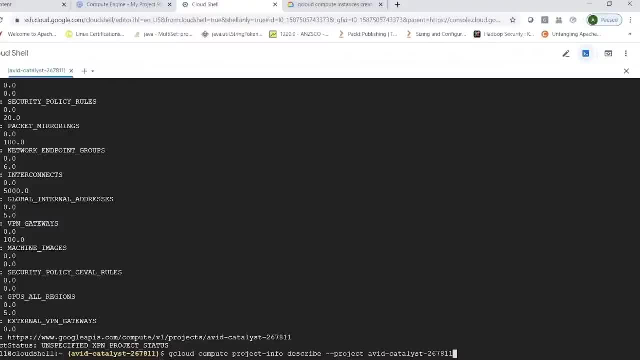 choosing earlier. so I can just bring up this command again, and what I can do is I can say here, where I have gcloud compute project info, Where I did it describe earlier. now, what I could also do is I can just say add metadata and then I 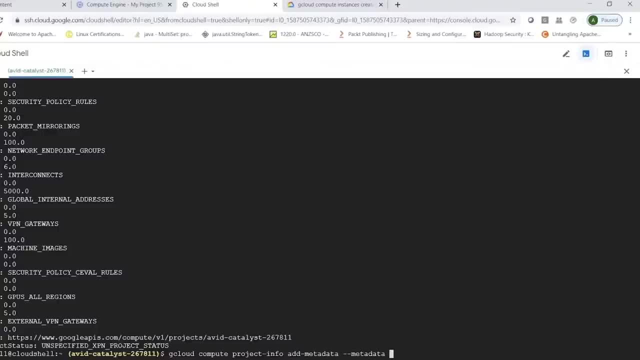 can specify what is the metadata. I would be interested in adding. I can then say google compute default region and then I can basically give a region, for example Europe, and then I can say west three, and if you are not Well experienced, you can always do it from console or you can be doing it from here. so I'm giving 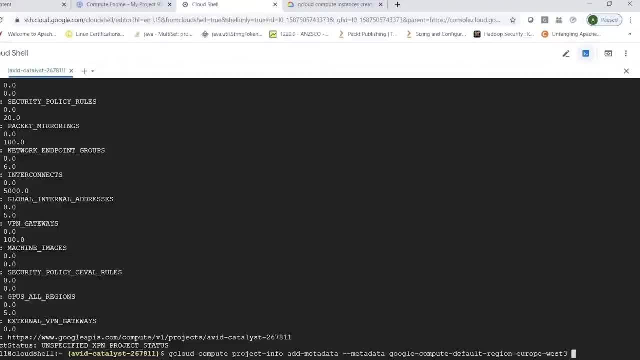 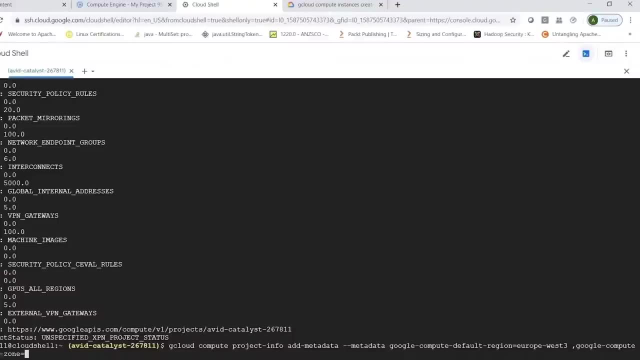 google cloud compute, google compute default region, then I can also give a google compute default zone and then I can pass in a value for default zone so I can say Europe west three and then basically I can give an availability zone. so if it is basically giving me some error where I'm trying, 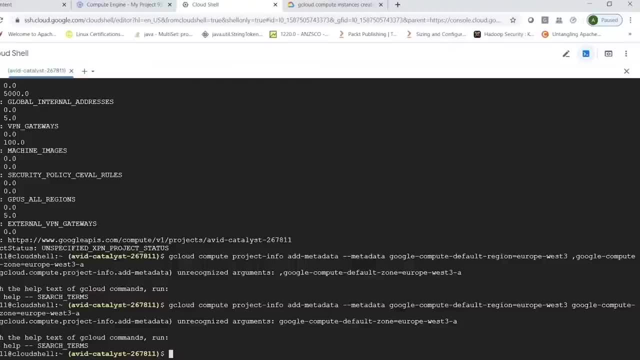 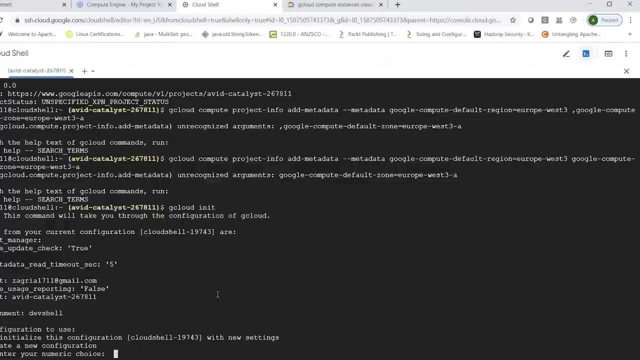 to pass in the These values. so I can just give it this way. and then it basically says that if you can look into particular help to see what is the command which you would have to do now, I can basically do a g cloud in it here: initial configuration. and this basically says that it is initializing my default. 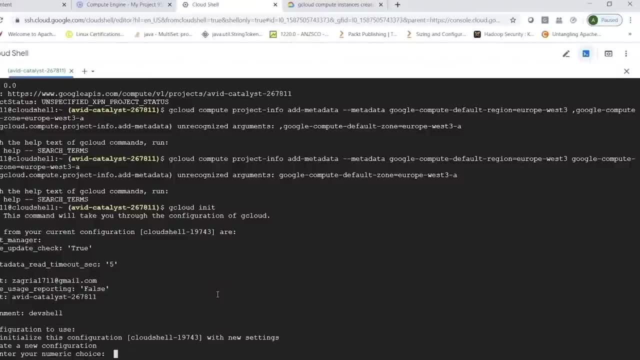 configuration. it says: reinitialize this configuration from cloud shell. you want to create an new configuration. so if I had updated my metadata then basically I could just do a cloud in it and I could be reinitializing my default configuration or properties which I have passed in. so as of now, I 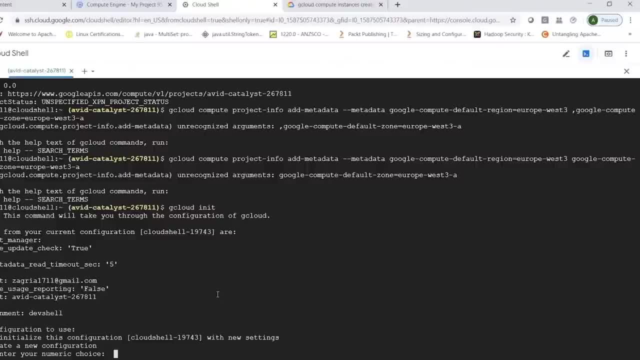 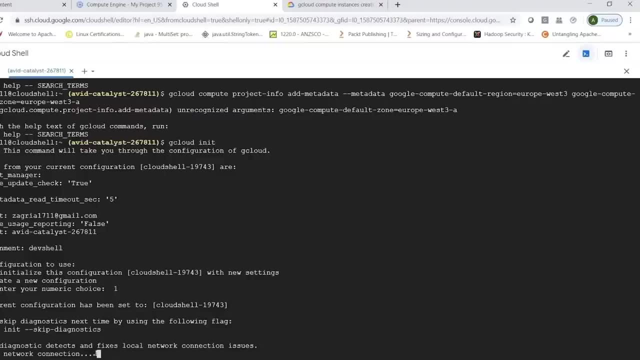 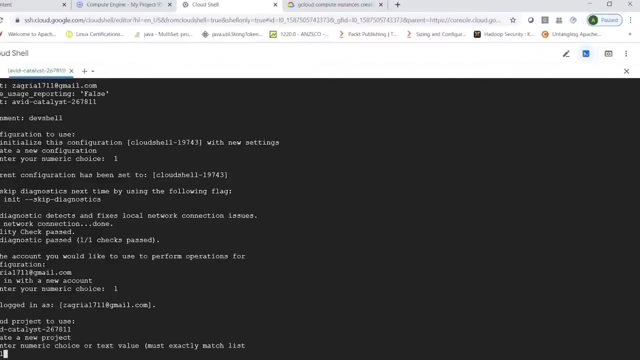 will not activate or change the default region. let's go for a simple way in which you can create your compute engine. so, for example, I'll just say one, and it is reinitializing. it asks me what is the username, and let's select that. it says what is the project, and let's select. 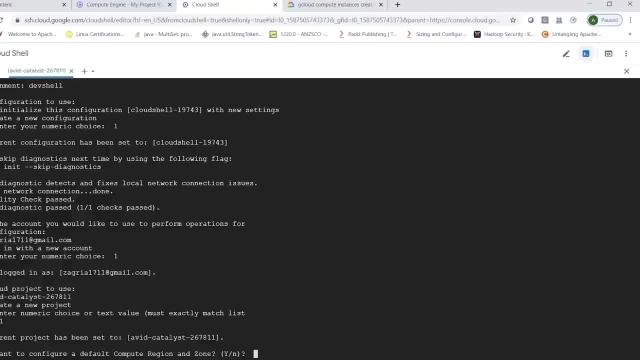 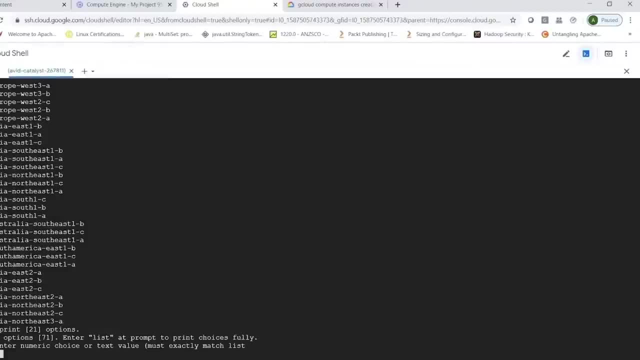 that and do you want to configure a default compute, region and zone? right, and I will just say yes, and basically then it shows me different options which we have here. so there are too many options here. and then here we were interested in Europe west three, so let's choose twenty one, right? 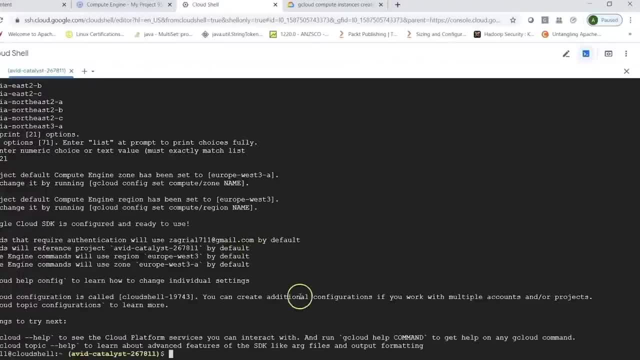 And then that basically allows me to choose my region and my zone. So it also gives you some specifications. So it says your project default compute zone has been set to Europe S3A. You can change it by running gcloud config set and you can give a compute zone. 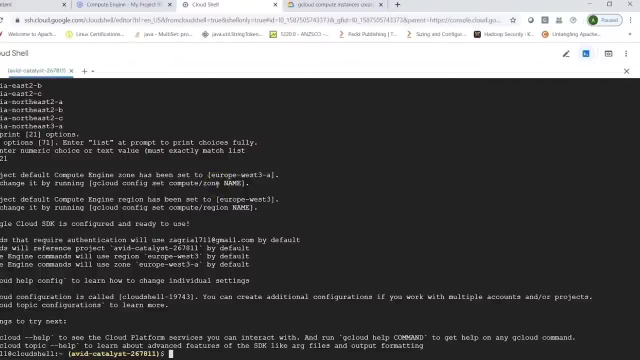 Right, So I can always give these commands. I can get help information here. So I can just say gcloud config set and I can be specifying the compute zone. So I can say compute slash zone and I can give a zone. I can say compute slash region and I can give a region name if I would want to do it. 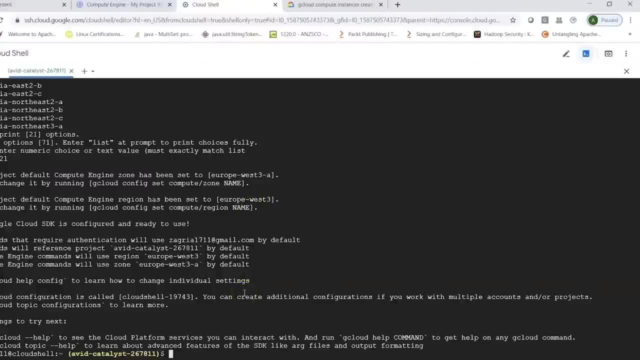 Or the easier way is like what I did right now. So you can basically do a command, gcloud init, and then basically it allows you to change your configuration or set default things. here You can all the times you can say gcloud config unset to basically remove a compute zone or a compute region. 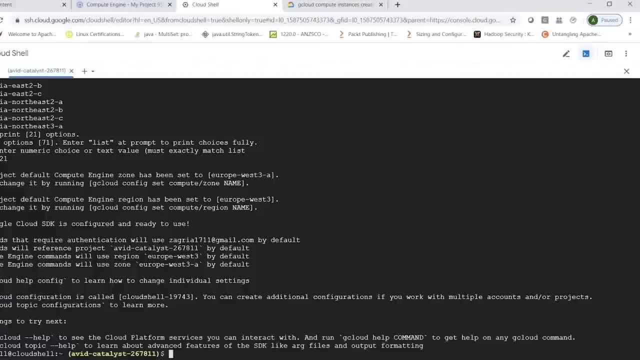 Now there are different ways. So if you were working on a Linux machine, you could always use an export command, something like this, So you could do: export compute- sorry, cloud SDK. And then you can say compute underscore zone and then give your zone. 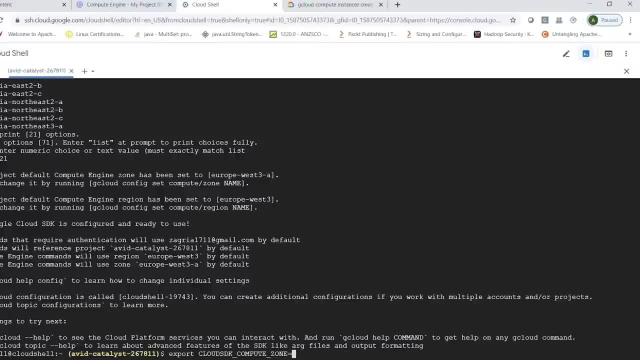 Name or compute underscore region and give your region, or you could add it in your bash RC file. Right now, that is when you have your cloud SDK set up on your Linux machine or on Windows machine and you would want to specifically set a zone and a region for all your compute related resources. 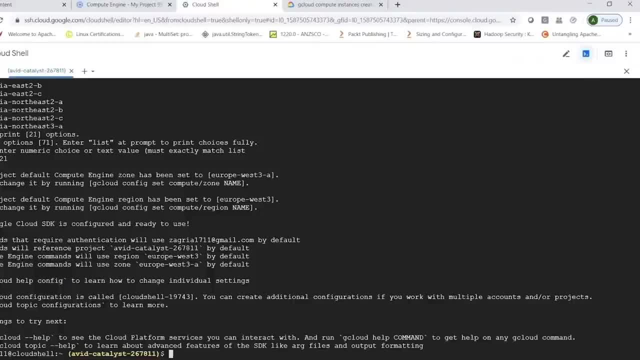 So we don't need to do that. The default settings are already given here, Right, And what we can do is we can start by quickly looking into G cloud compute instances options. So I can say g cloud compute instances and then I can just do a list at any point of time. 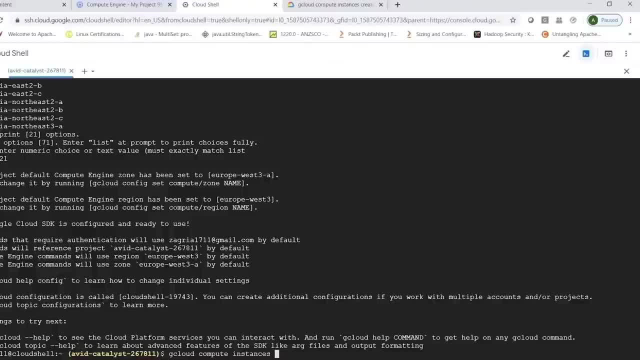 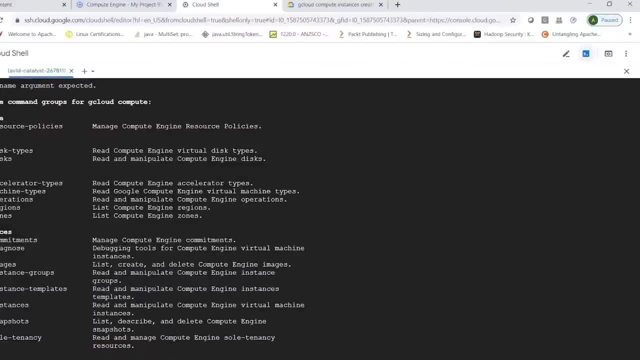 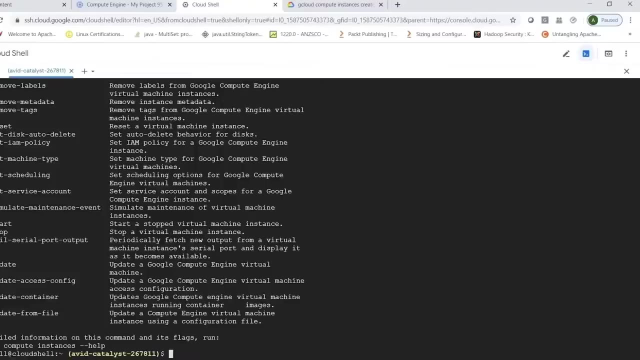 If you would need help, you can just do a g cloud compute and then say minus, minus, help. or I could just do a g cloud compute and that shows me different options which I have here, from which I use instances. I can always type instances and again hit enter and it shows me different options. 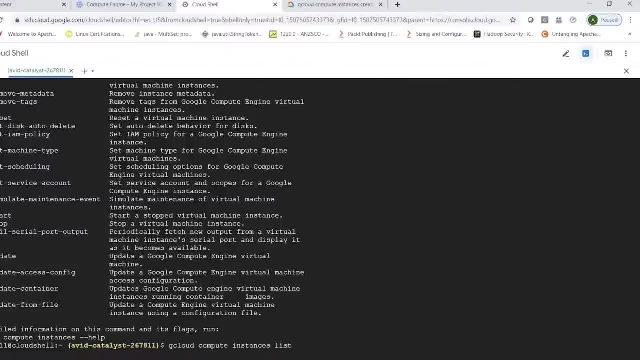 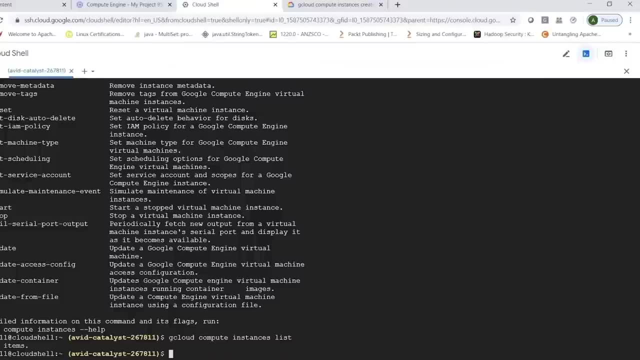 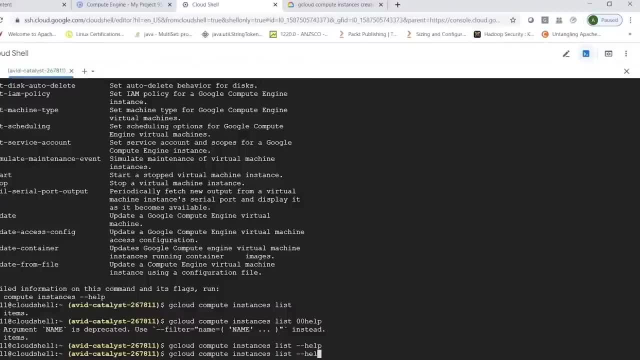 So, for example, if I do a help and it shows me with list what are the things you can do, so you can give a minus filter, So�E can then go back to our console and see what has it done, so I can say here: Create. 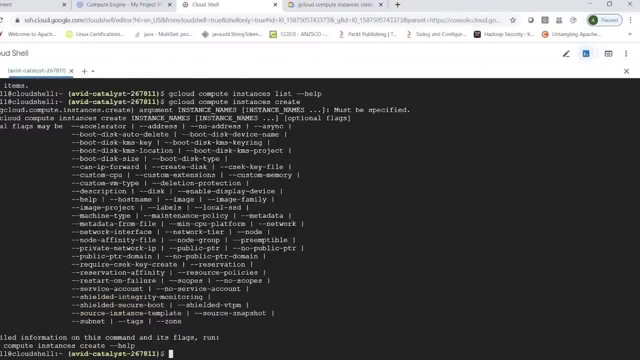 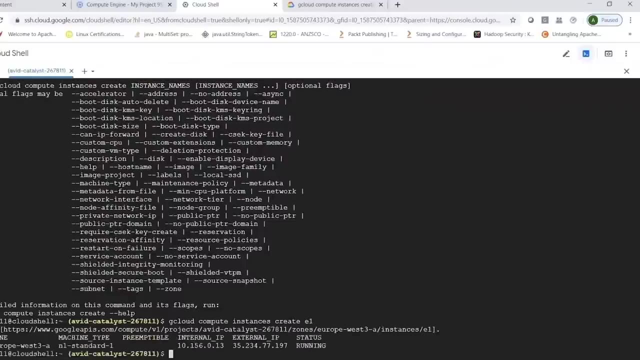 Let' see what does the create do? so it says, okay, you are giving a create option, but you would have to give a name. So let's say, let's call it e1 and that will be the name of my instance. and this one is an easy command from your Cloud Shell which basically creates an instance. 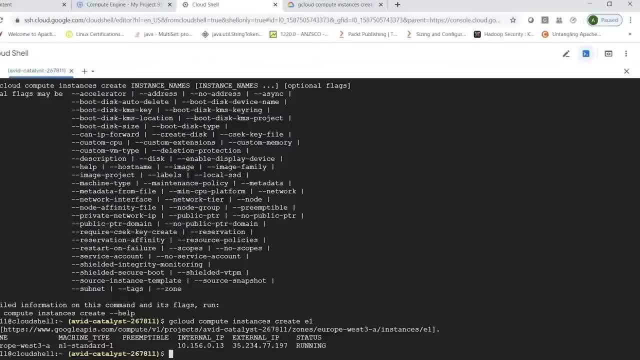 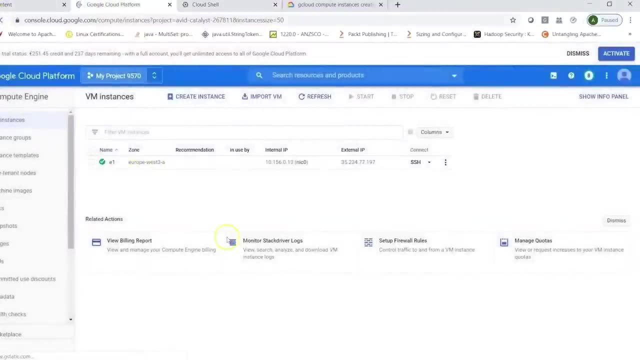 You see the zone which has been set. It is the standard number of inventory machine type. it is not preemptible. it has an internal IP and it has an external IP. Now I have created an instance and here I can just go back and then I can just do a refresh on this. 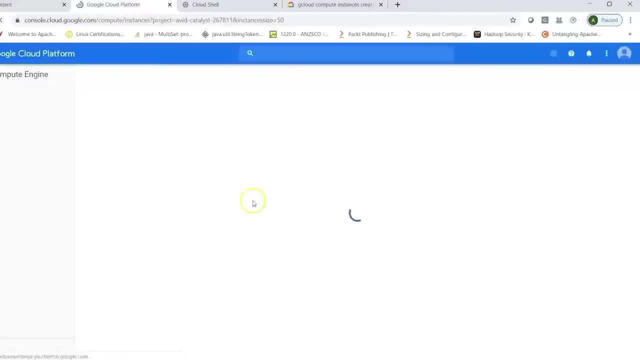 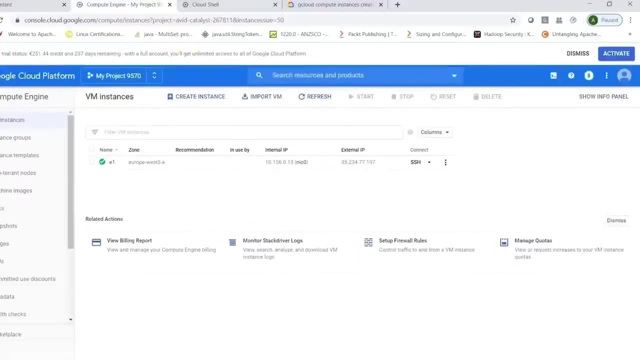 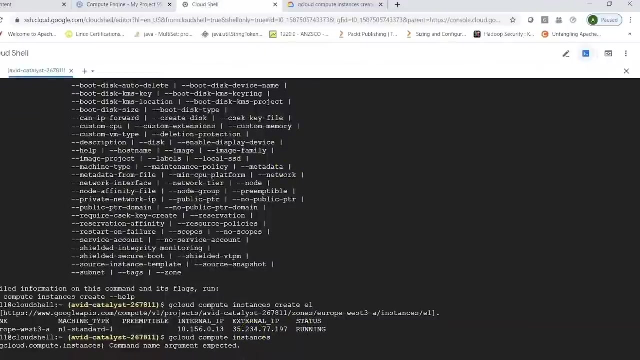 page and that already shows me the instance which I have created, and then you can use the same method to connect to it using an SSH. So I have an instance created from my cloud shell and what I can do is I can basically look into instances and see what are the different options with instance. 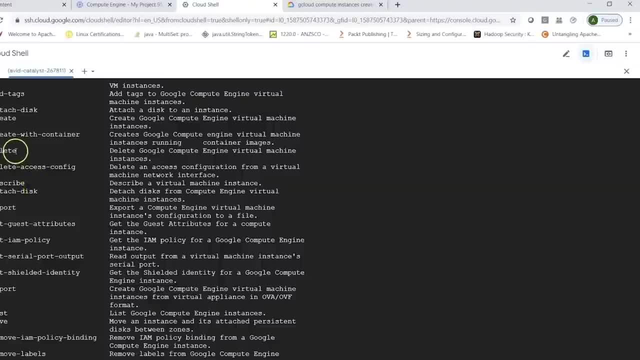 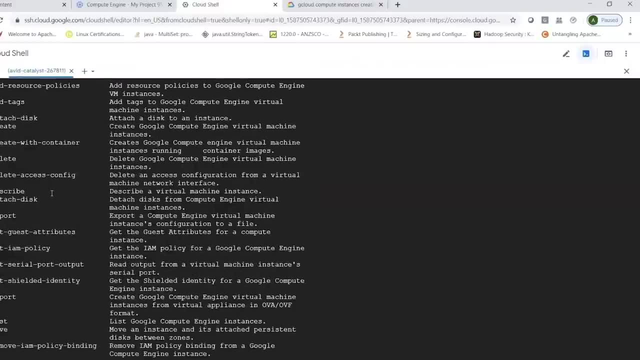 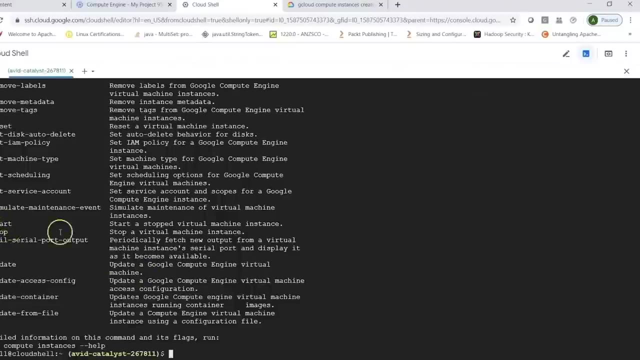 so if we did a create, right, you have an option delete. we did a create, you have an option delete. you can be in deleting the instance from the command line or you can use other options so you can do a list, you can do a stop, you can start. so I can basically do a stop and let's say even let's. 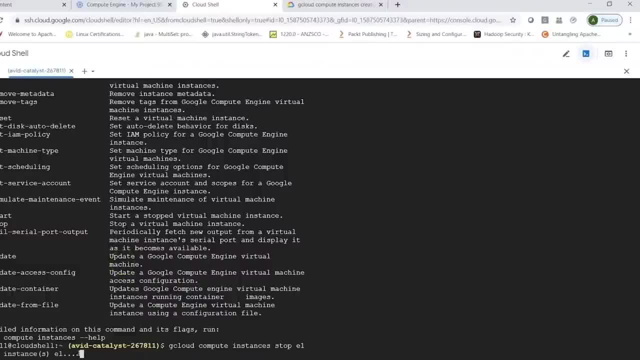 go ahead and do a stop- Commands are pretty easy here to remember- or you can always use the help option- and now I'm trying to stop the instance and then basically I can go ahead and delete it. So this is a simple way where I created a instance from the command line or from the console which I showed earlier and similarly. 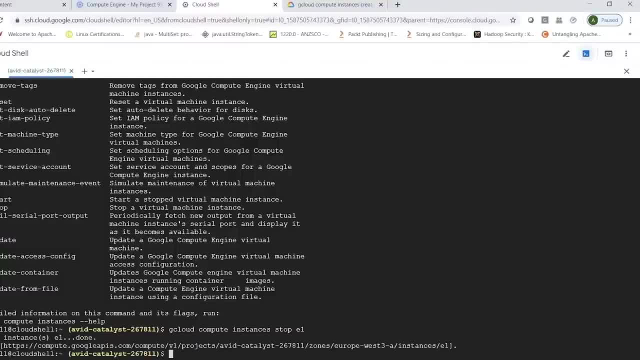 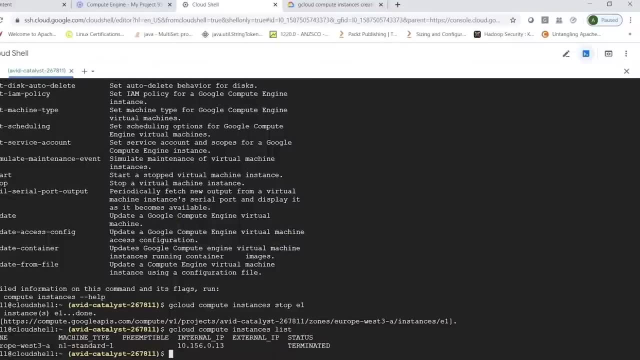 you can be working with other options. So now I've created stop the instance, let's do a listing to see if my instance Shows up. it shows up right, and it says the status is terminated. so you have stopped it. it's in the terminated status and now what I can do is I can go ahead and delete it. 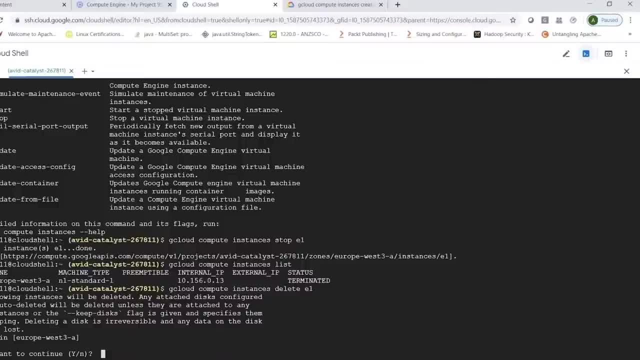 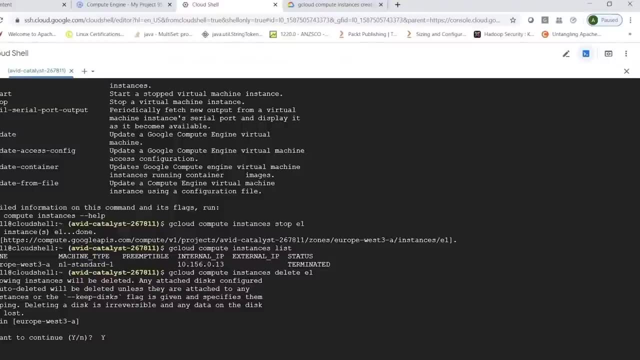 So it says this will be lost. are you sure you would want to continue? just say yes, and that should take care of deleting your instance. So this is a quick demo on creating your instance. we have already seen how you can connect to these instances using SSH. 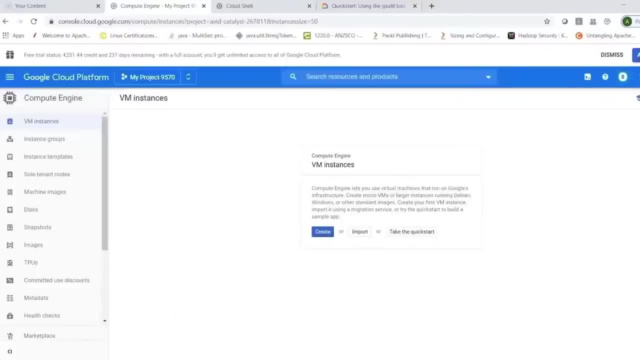 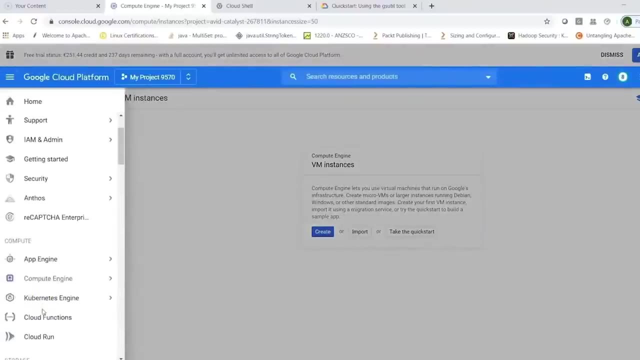 Now that we have created instances, let's also see how to use Google Cloud's storage service, which can be used to load data or upload data. so for this we will have to look into your Google Cloud storage options, and here you can look in cloud storage. so let's go back here on the top, which 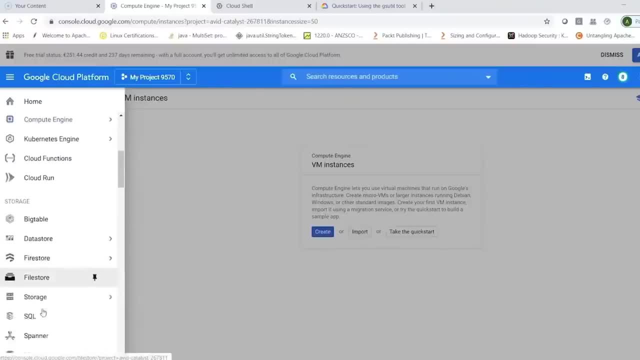 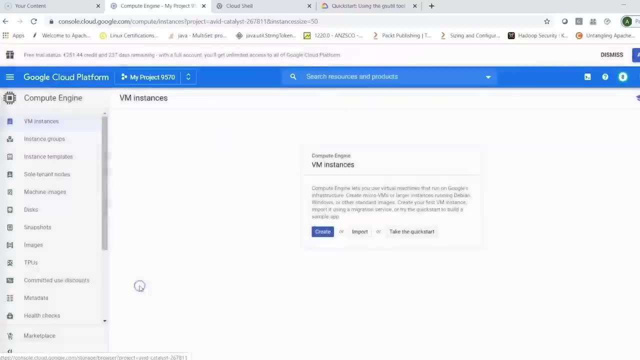 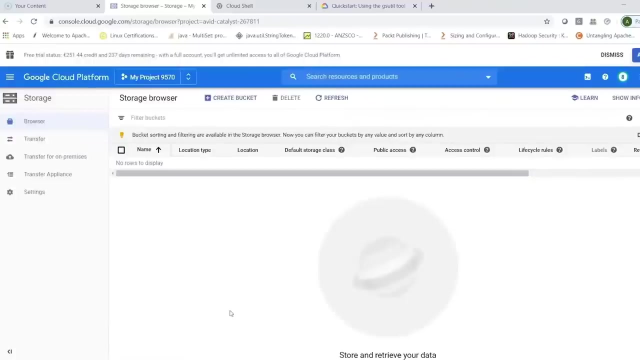 shows me different services which we have here, and let's look into storage. So this one shows me your storage option. now you can click on browser and that basically shows me your storage browser, which shows me on the top you have options for creating a bucket. 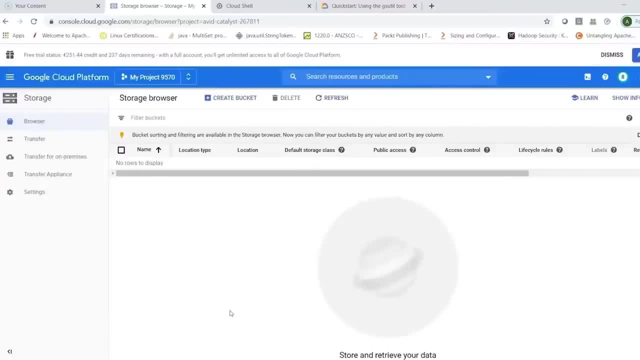 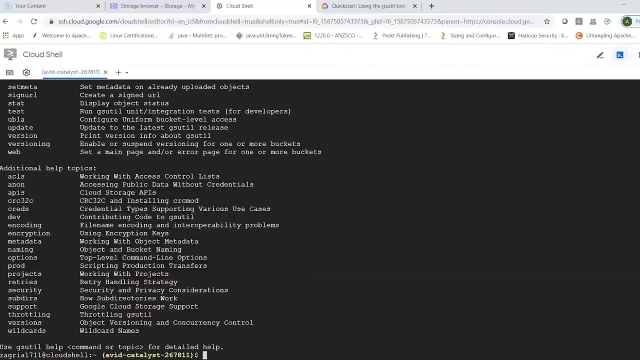 Now Google Cloud storage allows you to store any kind of data. here, the easiest and the simplest way would be by using cloud console, although you can again use cloud shell, and in that you can use your gsutil command, and gsutil basically has different options where you can be using, say, for example, I: 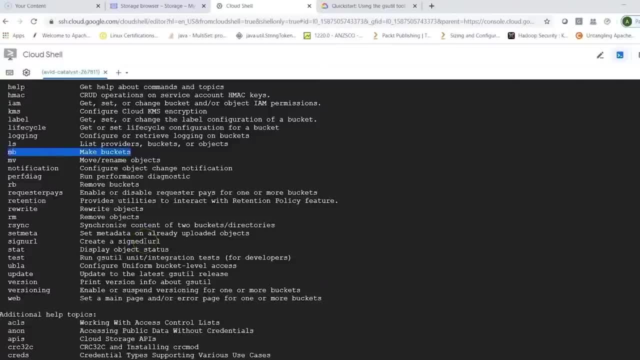 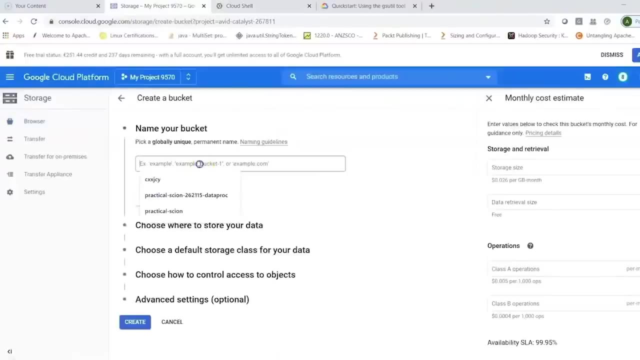 would want to work on buckets so I can be using MB and then I can use my command line option to create buckets. I can put in data there, I can browse it and I can access the data from command line. So let's create a bucket here, let's click on this, let's give it a name. so let's say my data. 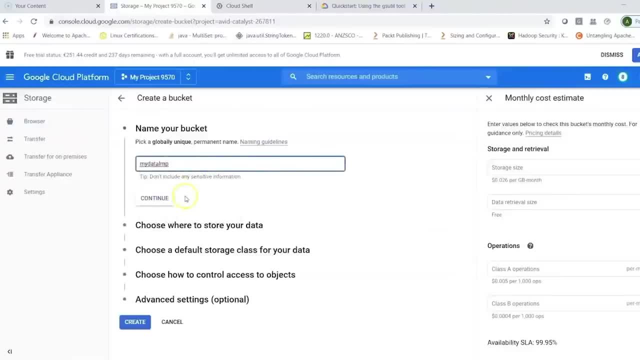 important. that's the name. now I can click on continue straight away. I can look into all of these options if I'm interested in, so you can basically be looking at your monthly cost estimate in the beginning. now I can click on continue. or you can say: choose where to store your data, and this one 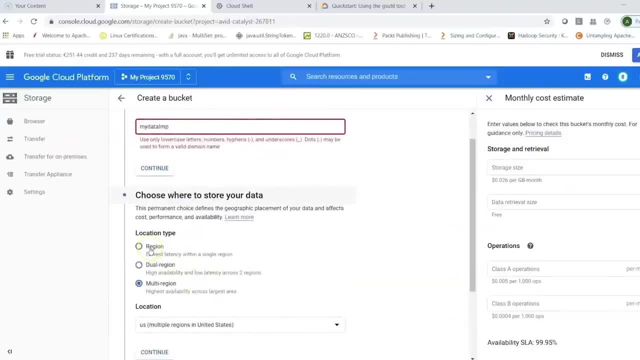 shows you different options. so you have region specific. so let's also give the bucket name with all lower case. that's what is required. Yeah, So coming back to the location type, you can choose multi region, which basically allows high availability, so your bucket or your storage option will be accessible across regions. you can also 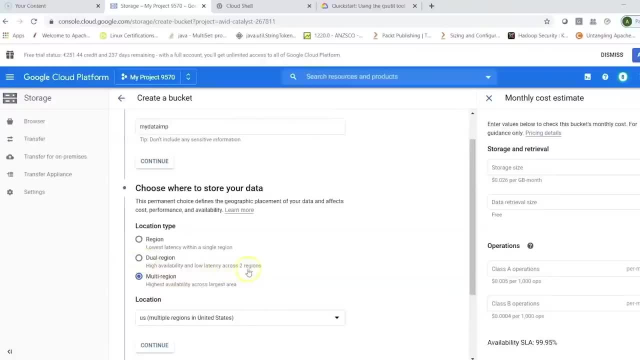 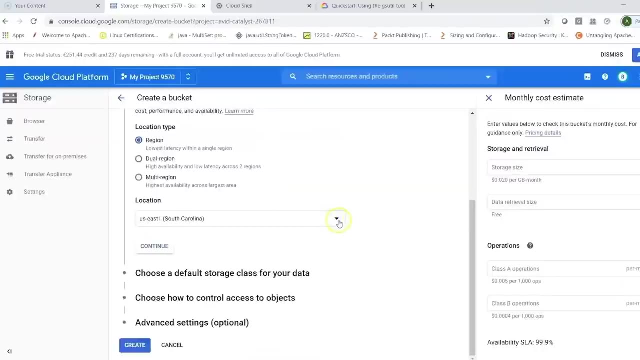 give dual region and high availability and low latency across two regions. I can also say region specific. so for our use case we can just give region specific which can keep our cost low. but in business use cases you would be going for multi region. Now here you have location and I would again go for, say, Europe, and let's choose Europe West 3, Frankfurt. 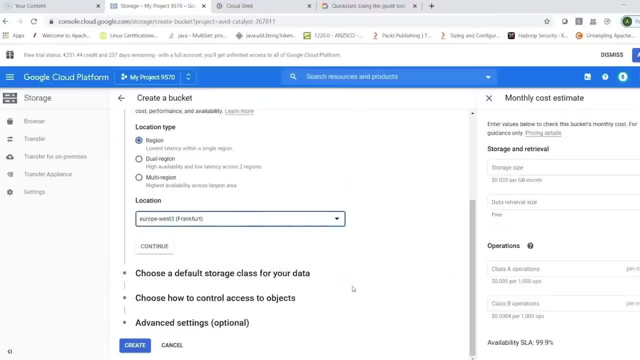 it is always a good practice that when you create your instances, when you create your storage or you use different services, try to have a geographical region chosen and then you would try to put things or your services within the particular region, within a particular zone, unless you would want to make. 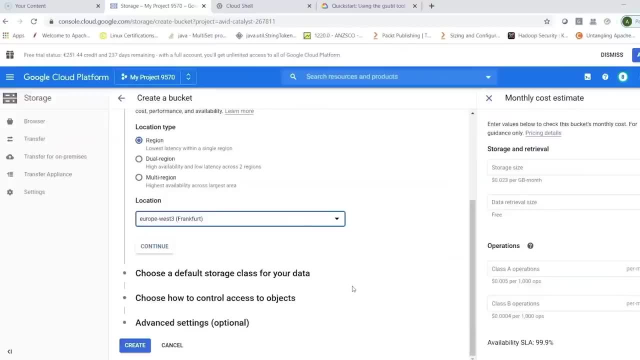 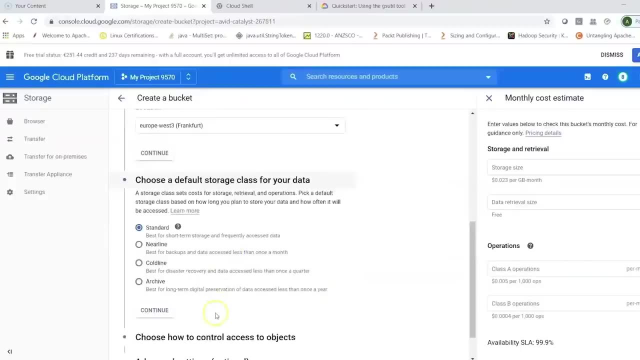 it accessible and available Across regions. now I can then choose a default storage class. So when you say default storage class, there are different storage class and each one is for a different use case. So you have standard, which is best for short term storage and frequently access data you have near line. 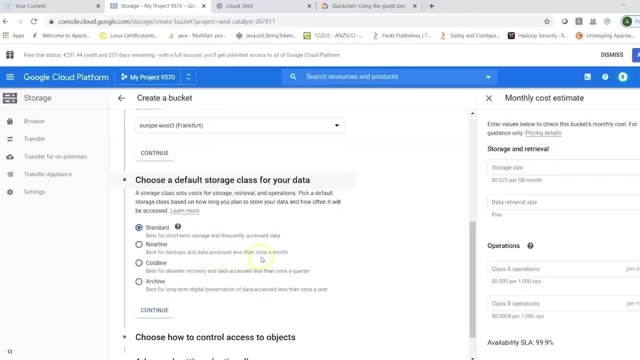 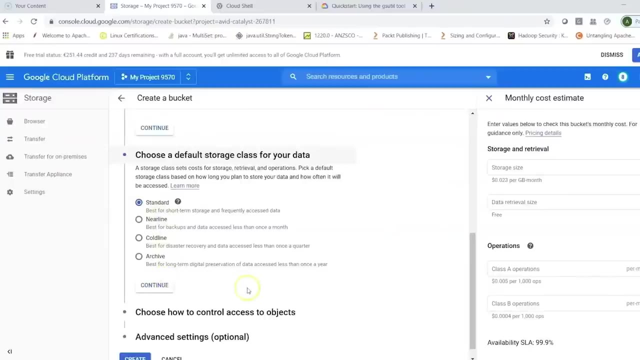 So this is basically best for backups and data access less than once a month. You can also have cold line, so these are basically like your cold storage or freezing storage, which you might have heard Generically as terms. So you can choose one of these storage classes depending on what will be the use case for this particular storage bucket. 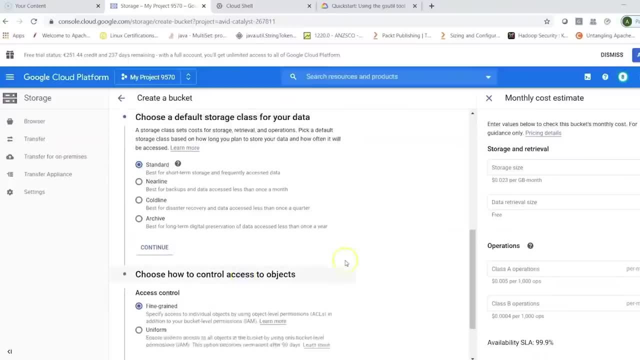 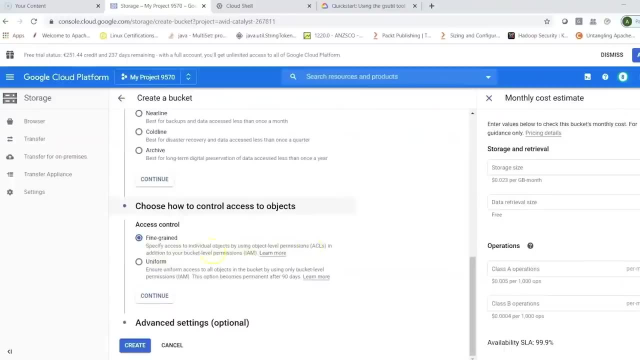 So let it be standard Now how to control access to objects. So you can basically say: specify access to individual objects by using object level permissions. Now you can give permissions to the bucket. You can just say uniform access to all objects in the bucket by using only bucket level permissions. 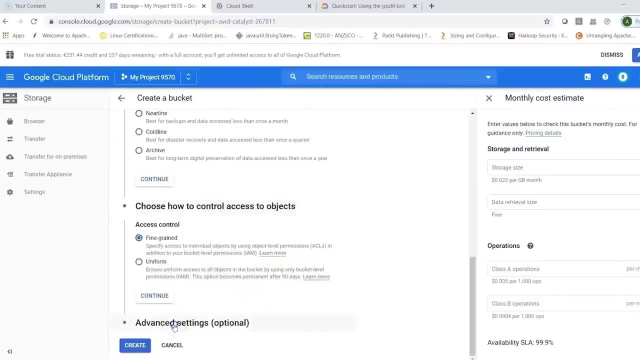 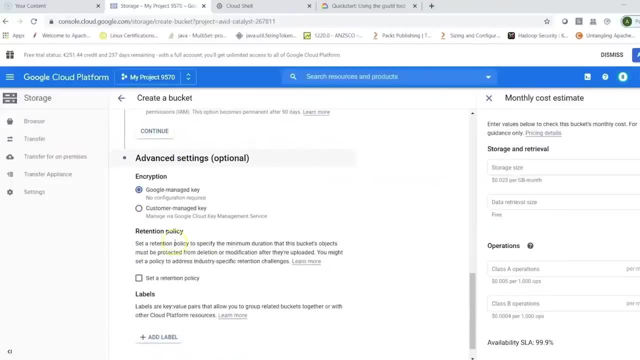 So you can choose that. You can also go into advanced settings, and here you can see different ways in which you can have configuration set up. Now you can also have a retention policy to specify the minimum duration where that this buckets object must be protected from deletion. 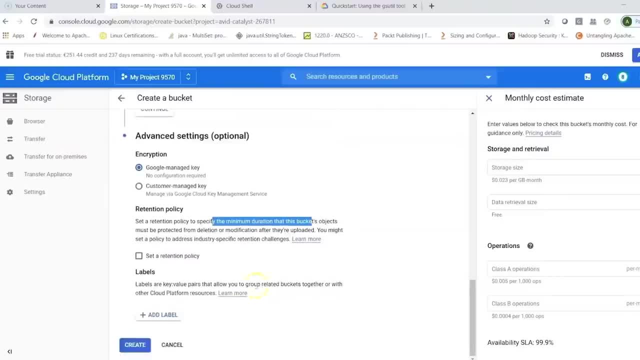 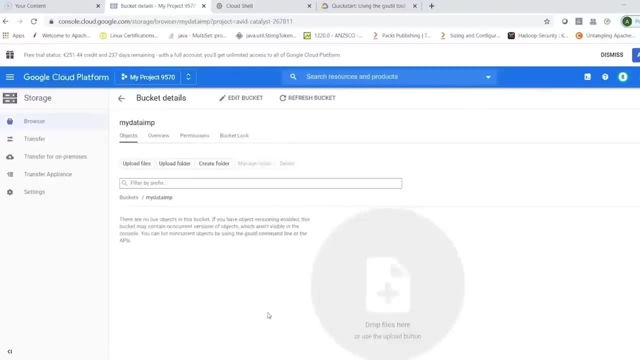 And you can set a retention policy. We will not get into all that, We will just first try creating a bucket. So just click on create and that should create your bucket, Your bucket wherein I have my bucket. Now I can click on overview to see the details. 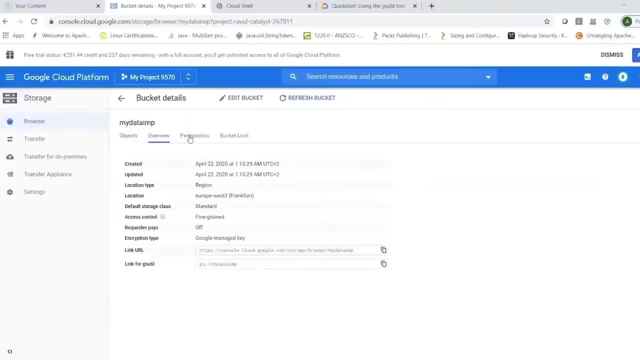 What is the region? Which region it belongs? What is the storage class? Anytime, you can always click on edit bucket and make some changes. here You can look at the permissions. So bucket uses fine-grained access allowing you to specify access to individual objects. 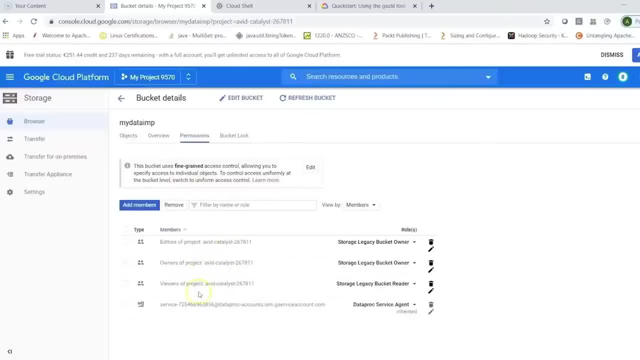 And then you can basically look at who has access to this. So in my case, Editors of the project- They basically are the bucket owners, Owners of project, Viewers of the project Right- And you can basically choose what kind of access you need. 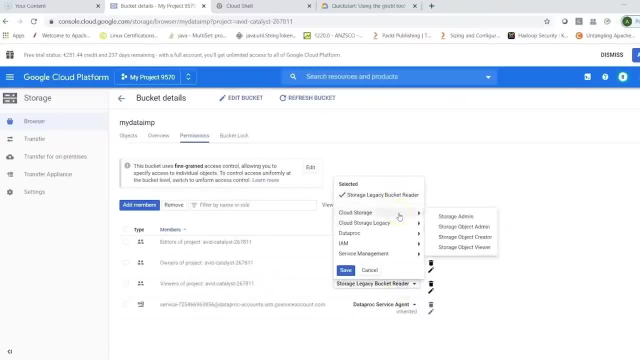 So for this you can always go into cloud storage and then you can decide what kind of access you would want to give. Whether that's a storage admin, It's an object admin, object creator, object viewer and so on, You can always look at storage legacy. 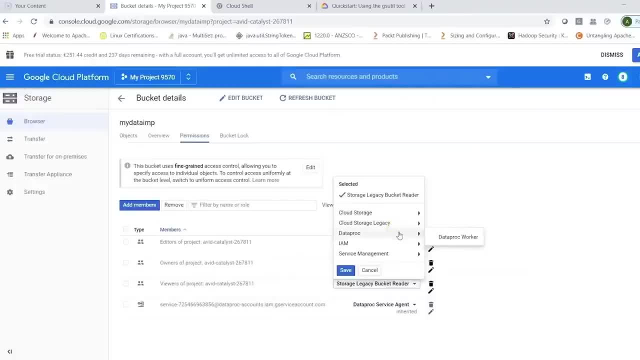 And for any other service. Depending on what APIs you have enabled Right, You can always control your permissions. So right now it is storage legacy bucket reader, And that's fine, And this one is bucket owner, And then might be. I was using some other services, like data proc, which uses cloud storage. 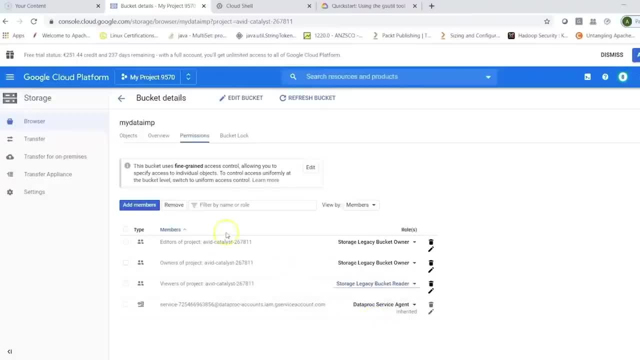 And that's why I've given data proc service agent also. So these are some of the members you can remove. You can view by specific members, You can view by roles. So what are the different roles Which have access to this? So it says storage legacy bucket owner. 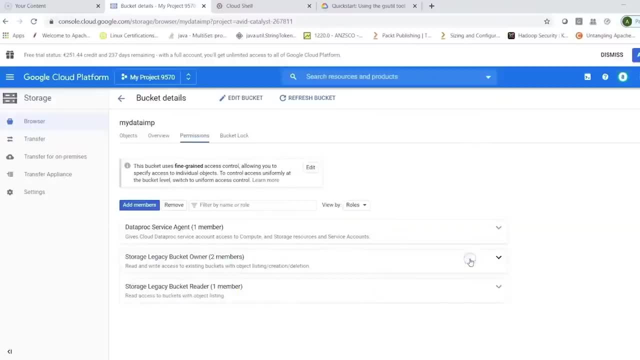 There are two owners based on this particular project, So these are auto controlled. But then you can add or remove machines. You can save storage costs by adding a lifecycle rule to delete objects after the duration of current retention policy. So you can add different policies. 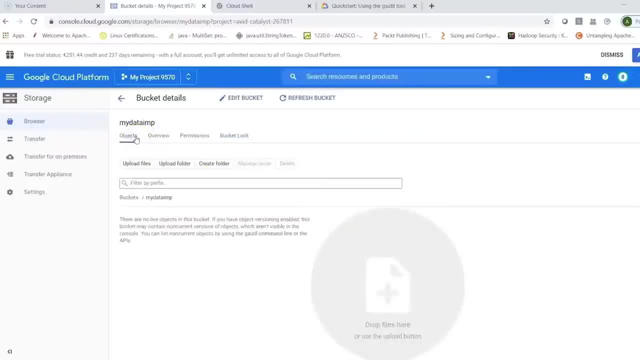 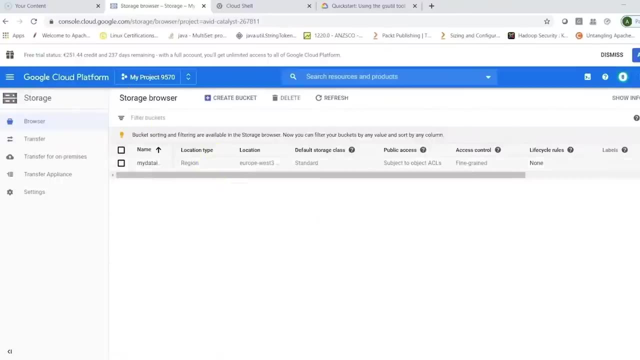 And you can basically control your bucket. Now my bucket is already created, Right, So I can go back. And then I see my bucket is already here. I can click on this option And you can anytime edit the bucket permissions. You can edit the labels. 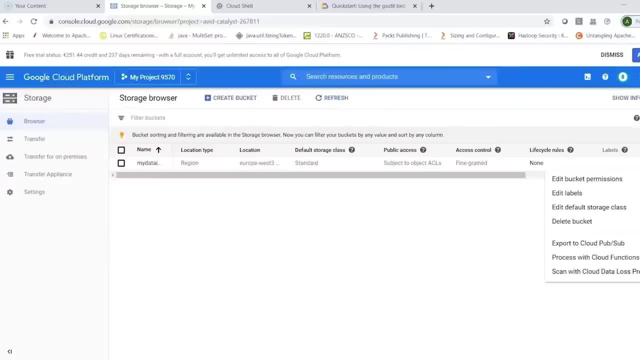 The default storage class. You can just go ahead and delete the bucket. You can export it to cloud pub sub. So basically, if you would want to have the content from this bucket being accessible in a message queuing system, You can go for pub sub. 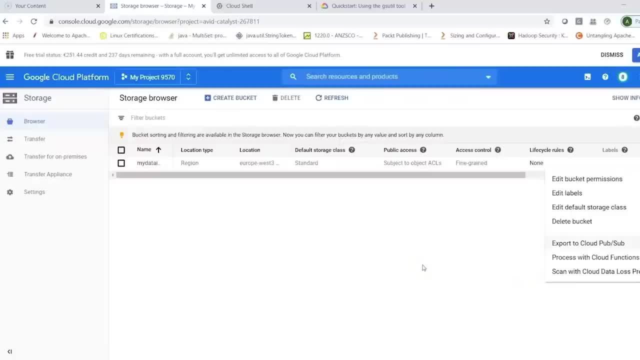 You can process with cloud functions And you can scan with cloud data loss prevention. So there are different options which are available. We can always select this bucket and delete it. Now I can click on the bucket And that basically shows me different ways in which I can upload some data here. 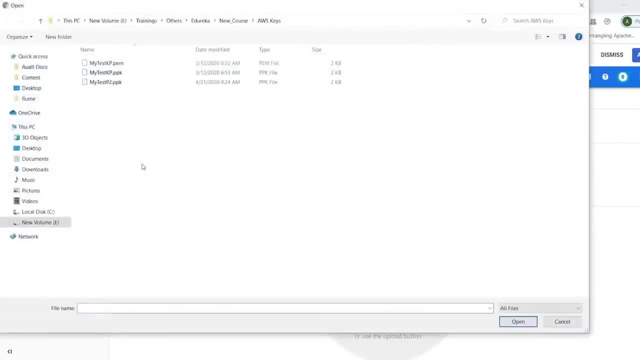 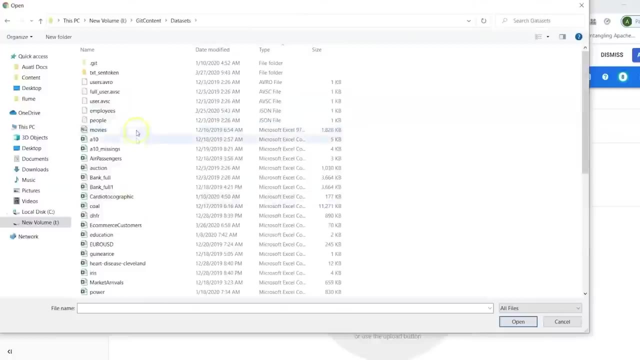 So I can just click on upload files And here then I can choose some files. So, for example, I'll go in here, I'll go into data sets And I have different data sets. So, for example, let's choose this one Which is a CSV file. 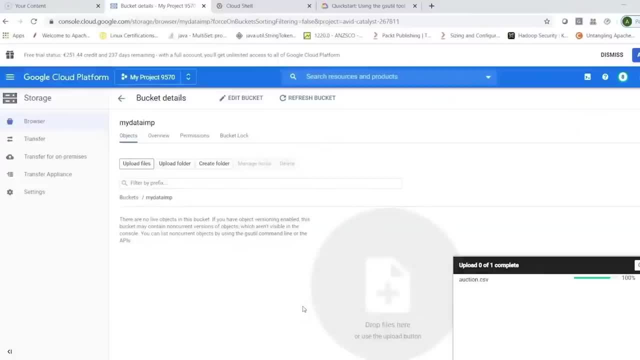 And then I'm just uploading this To my cloud storage. It's as simple as this. So you can drag and drop your files, Or you can just upload your files And my file is uploaded here. Now I can basically edit permissions for this one. 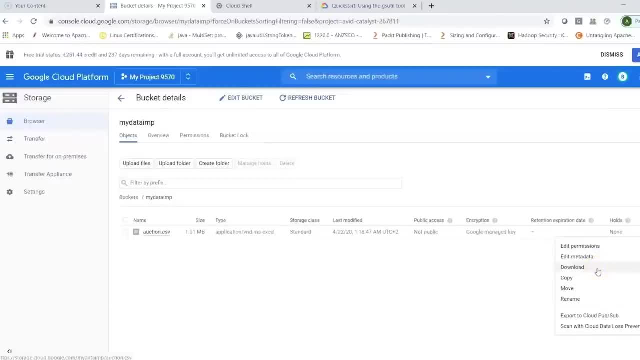 So this is in the bucket, So anyone who has access to this bucket Can basically download this file. They can copy, move or rename this, You can export it And you can look at the permissions of this file. So let's look at edit permissions. 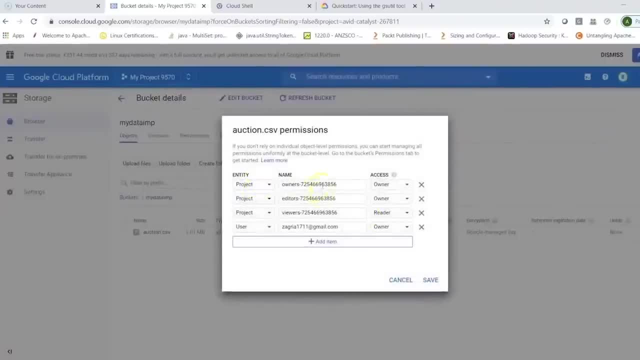 And it says: For this project, Whoever is the owner It has access. I've also given a specific user my Gmail ID And I've given access. So at any point of time You can just say add item And then you can start giving different kind of accesses. 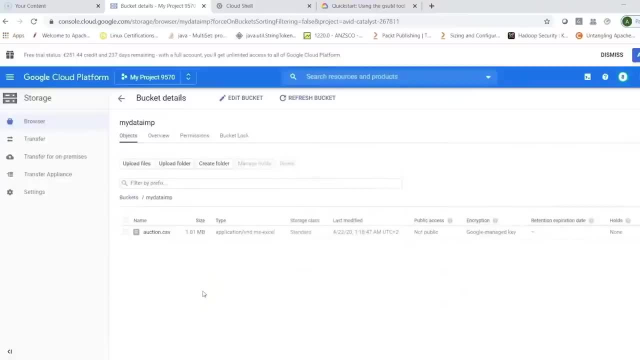 So let's click on cancel here. Now my data is already uploaded Into this particular bucket, And that's a simple usage of your cloud storage. Now what we can also do is I can basically select this And I can delete it. 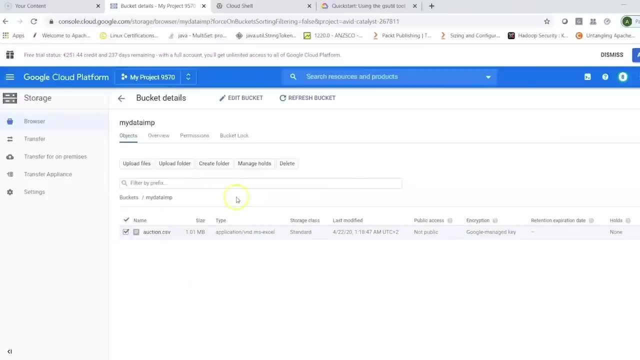 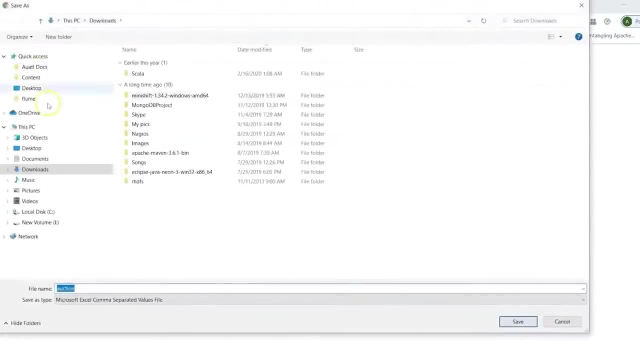 I can also create specific folders And then basically Load data into it. I can click on this one, I can just do a download, And then I can download it anywhere on my machine. So let's go to desktop And let's download this file. 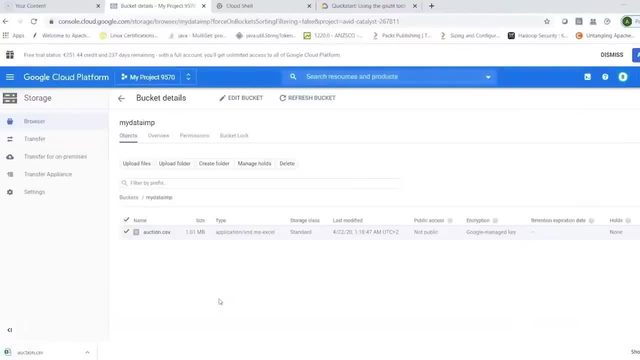 So we not only uploaded some content in the bucket, But we also downloaded that In a different location, Which will be accessible. Now, what I could have also done Is I could have created a folder here And I could have specified, Say for example: 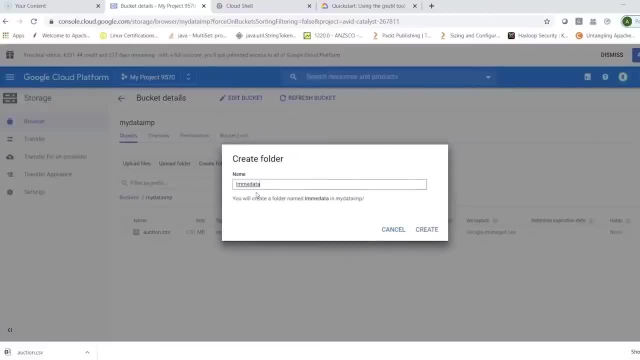 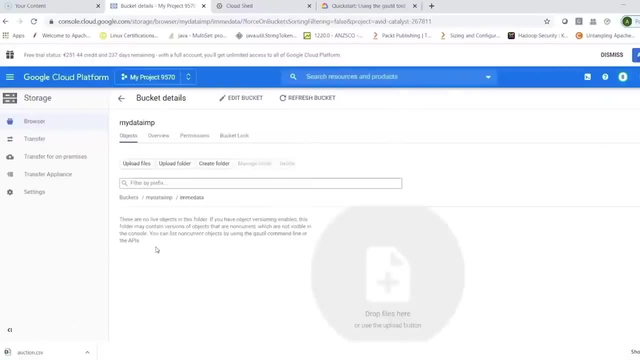 Immediate data. Okay, And I'm clicking on this one. So that's my immediate data. I can click on this one And now I can upload my data specifically To this particular folder By using the same mechanism. You can just do upload file. 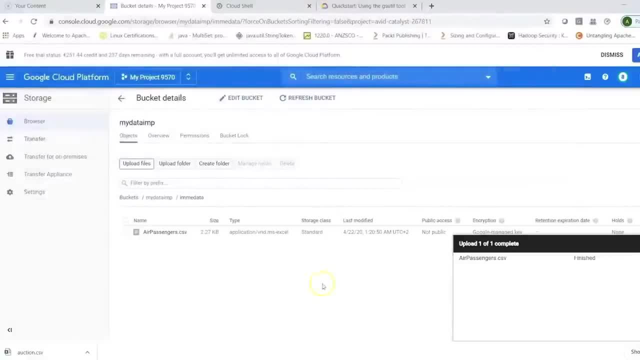 Let's choose air passengers, Let's do. a open File will be uploaded So you can always choose What is the retention Expiry date for this one. So, as of now, there is nothing, But you can be deleted. Objects can be deleted or modified. 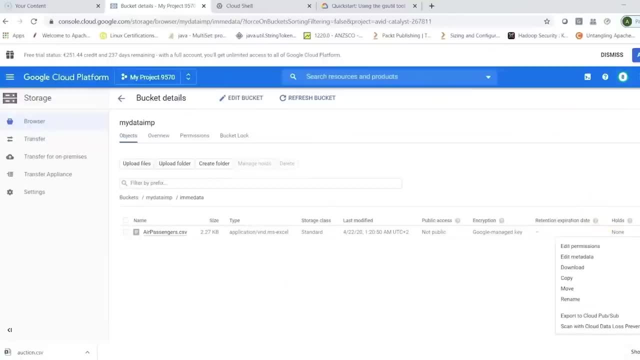 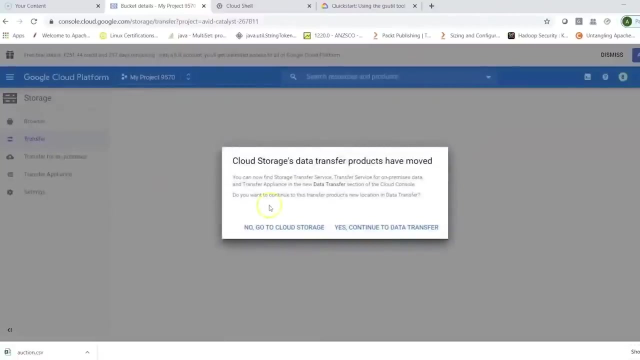 Until they reach their minimum duration. You can control all of that. You can basically download it, You can copy it And you can move it And rename it. So this is a simple example Where I created a particular bucket. For example, you click on this transfer. 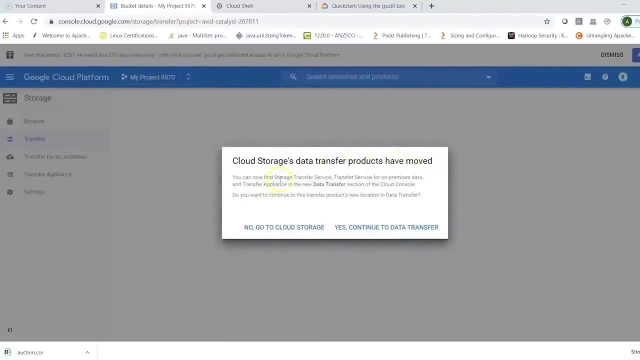 So it says: cloud storage data transfer Products have moved. You can now find storage transfer service On premise data and transfer appliance And new data transfer section, So you can always go back To cloud storage. You can also look at transfer options. 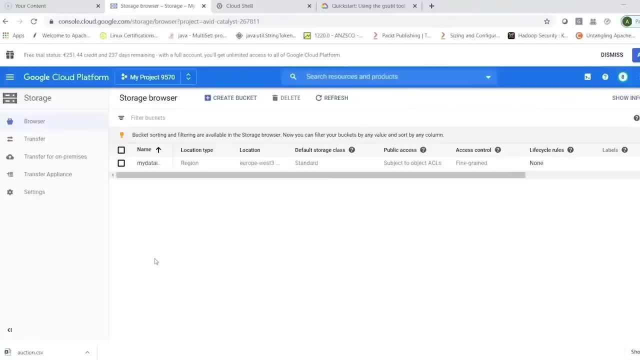 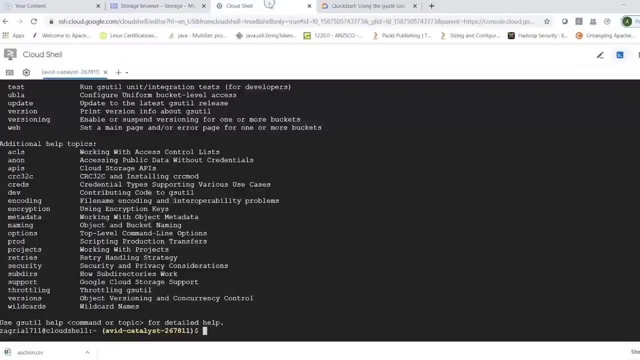 Which are mainly when you are Using an on premise service And you would want to upload data In a Google cloud. So this is my bucket here. Now I can go to cloud console And here what I can do is If I would be interested in working. 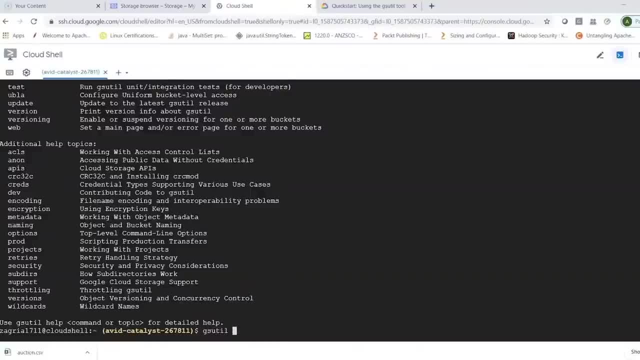 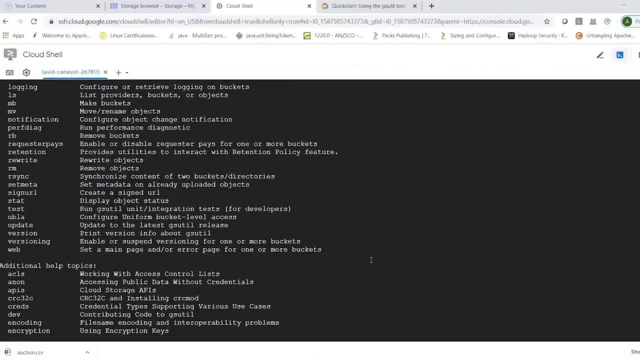 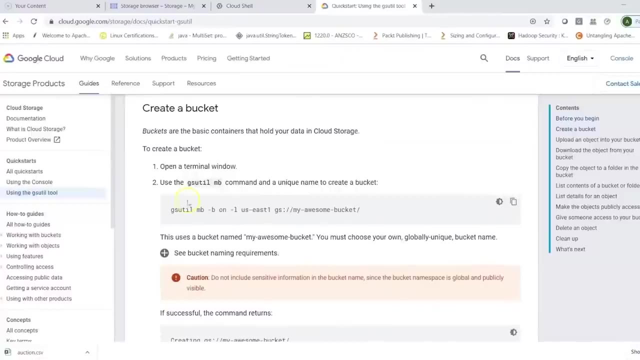 So I can just say gsutil, And then we have, For example, Let's try a help. And that basically shows me My gsutil. Now you can always go to quick start gsutil tool. And this is one more way. 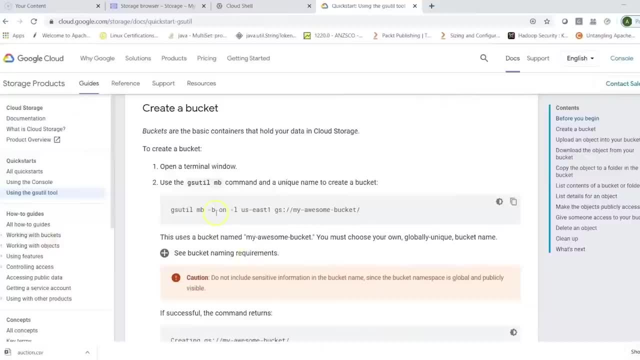 Where in. basically you can do it from the command line, So working with buckets, So you can do a gsutil mb Minus b On a particular zone If you would be interested in, And then you can say gs, colon And give a name. 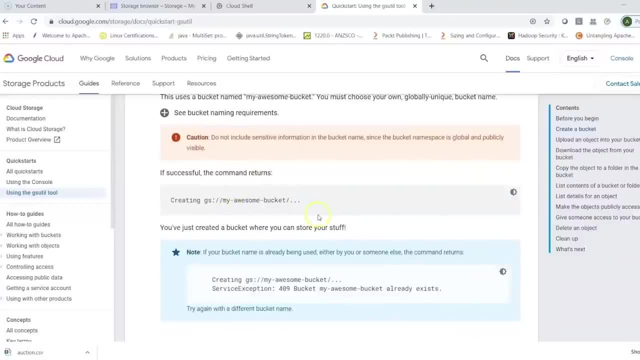 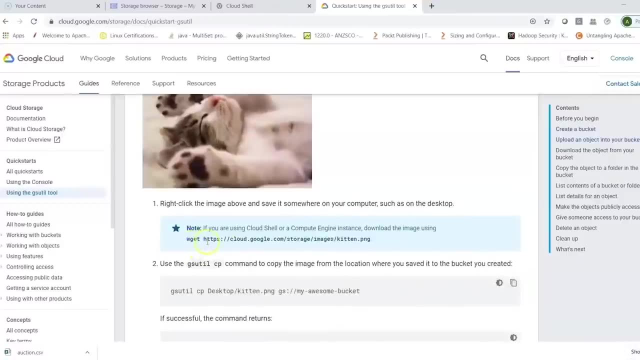 So my awesome bucket. This is how you will create a bucket Which will show you It is creating a bucket And then, basically, you can upload an image Or some data from internet. You can just do a wget: Download the file. 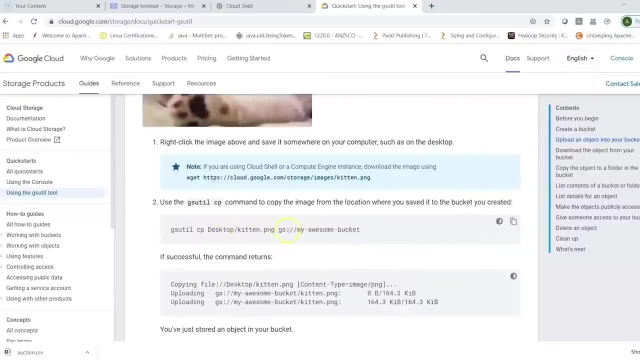 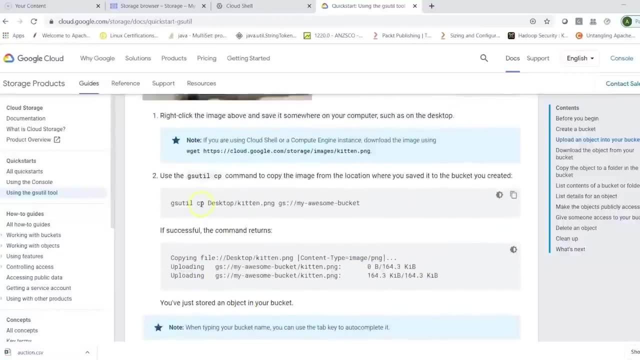 And then you can just do a gsutil copy command And that basically will pick up the file From your cloud shell location. Once you have done that, You can always do a copy. So here you are doing a copy From your local machine. 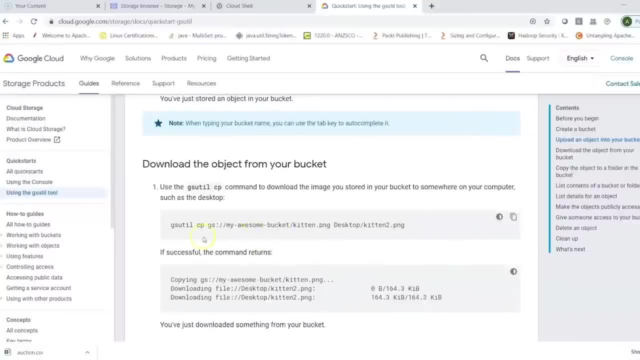 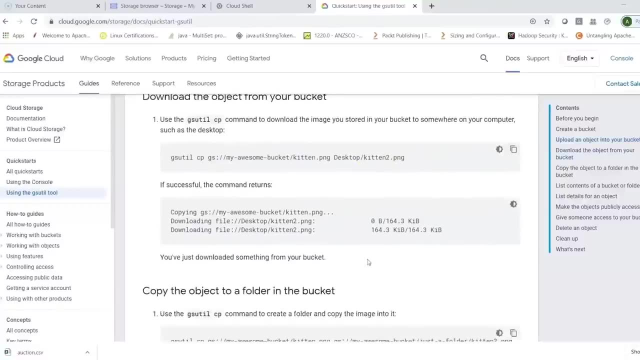 That is your cloud shell machine To your bucket And you can do the reverse of that, That is, you can do a copy And you can point your bucket And the file And download it to your desktop, So you can just download that. 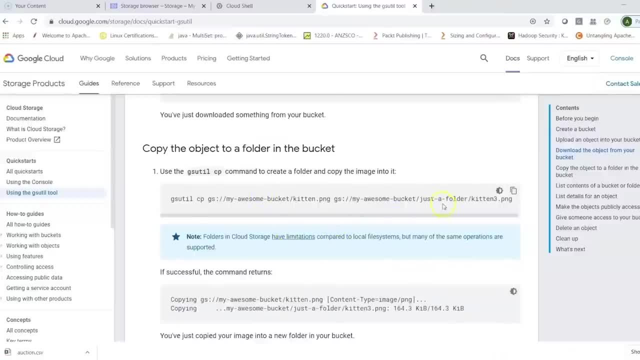 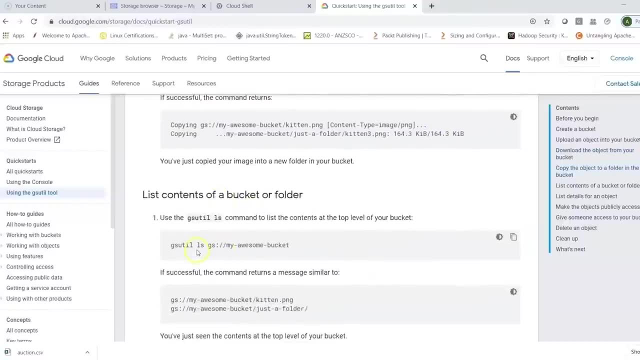 Using the command line, And you can copy the object to a folder in the bucket. So that is, by creating a particular folder, You are pushing the file into a particular bucket. You can list the contents of a bucket Using ls And then give your bucket name. 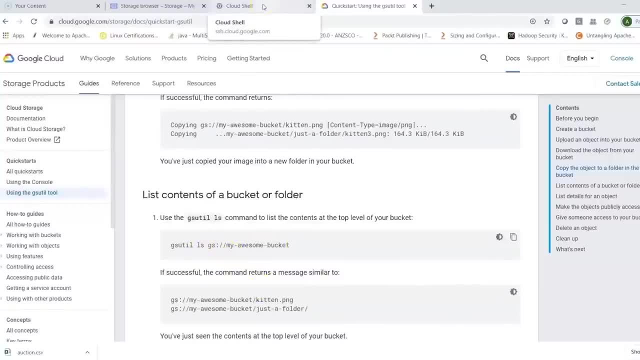 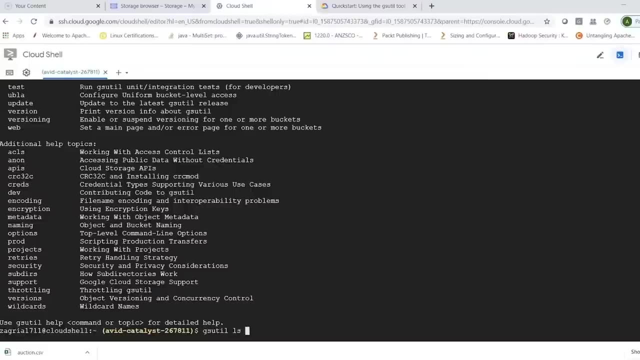 So gs, colon, So we can just try this one to be simple And rest you guys can try. So here you can just do a gsutil, You can do a ls, gs, colon, slash, slash, And then I need to give my bucket name. 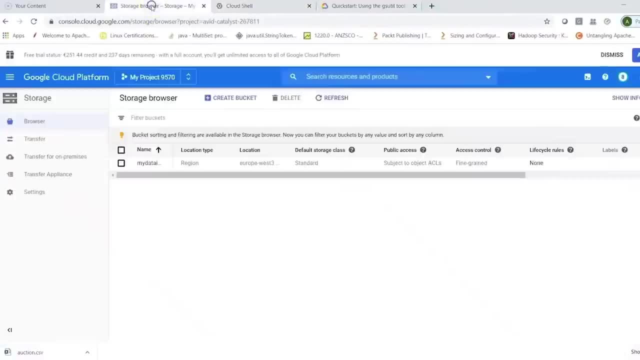 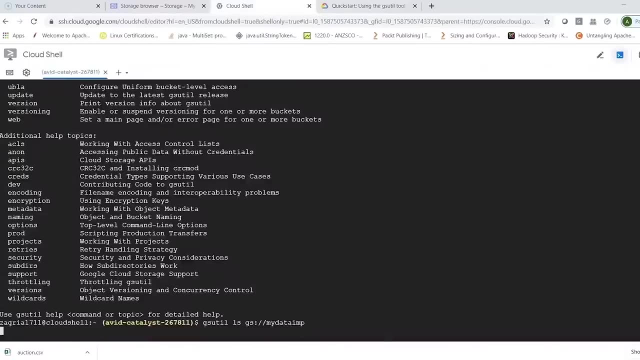 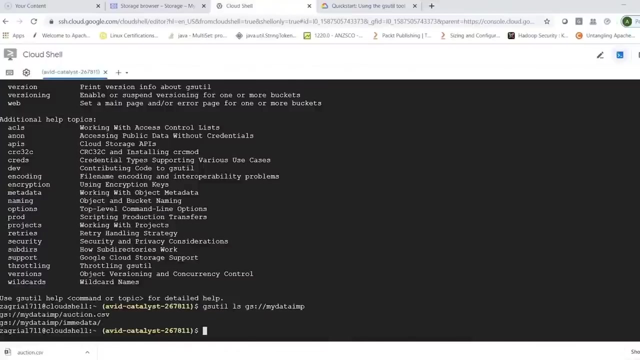 So in my case The bucket name was My data important. So let's try that. So let's say My data important And I am trying to list the bucket And the content it has, And then you have a folder. 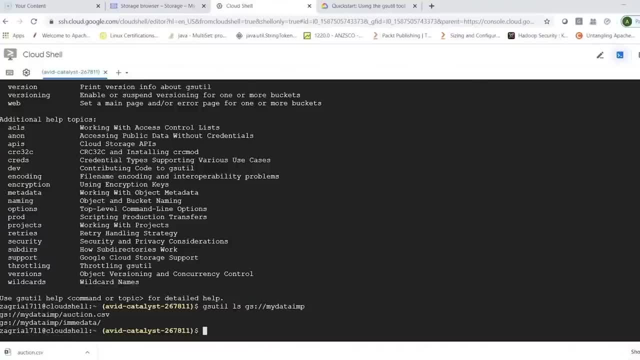 And then you can look into the folder And look into the files. So this is a simple, quick option Where in you can use your cloud shell. You could be using your google cloud sdk From your local machine Or you can be using cloud console. 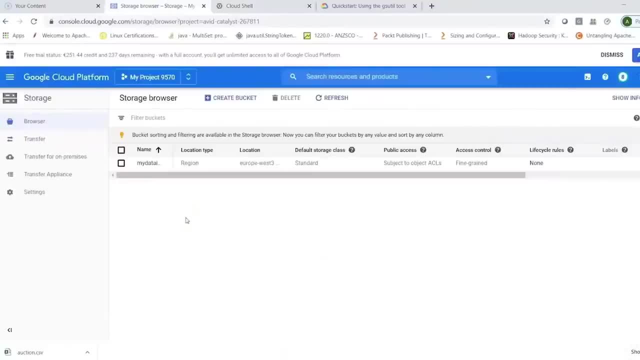 To create a bucket, Upload some data on it, Load the data, See if the data is accessible, And that basically shows you the power of cloud storage, Where you can easily Upload any kind of data. Now, what we can also do is: 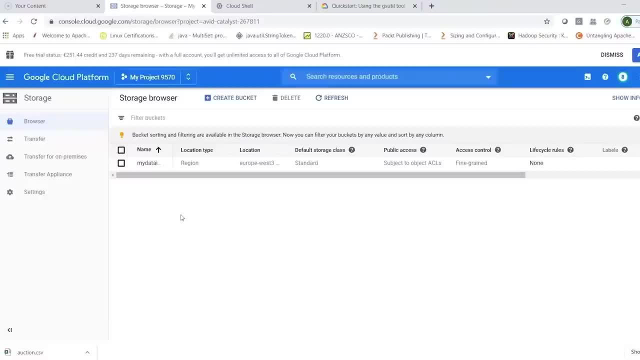 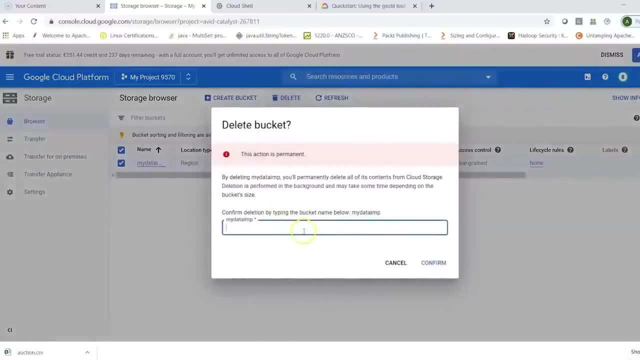 As you are using a free account Or even a paid account, Unless and until you would want to keep the bucket, You can select it And you can just go ahead and delete it. So this will basically ask you to key in the bucket name. 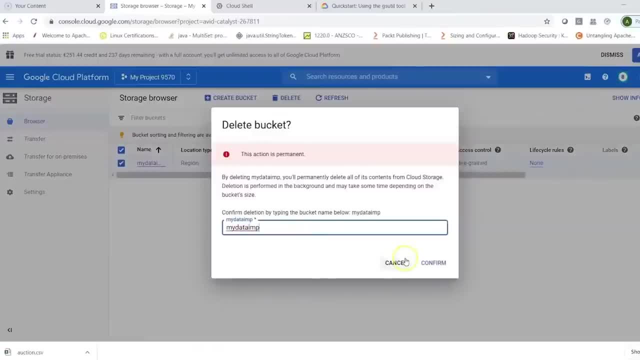 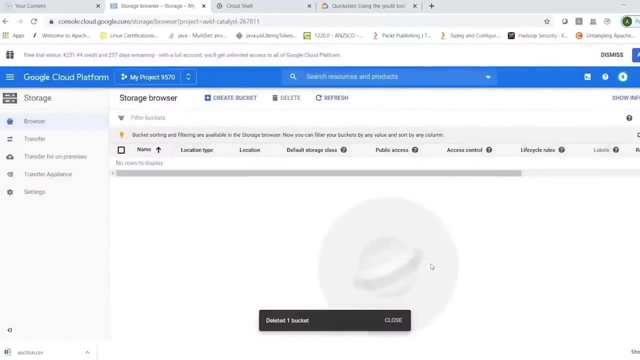 And let's say My data important. You need to confirm your bucket name And you could have done that using gsutil And a delete command From the command line, That is, from cloud shell. So we have now created a bucket. 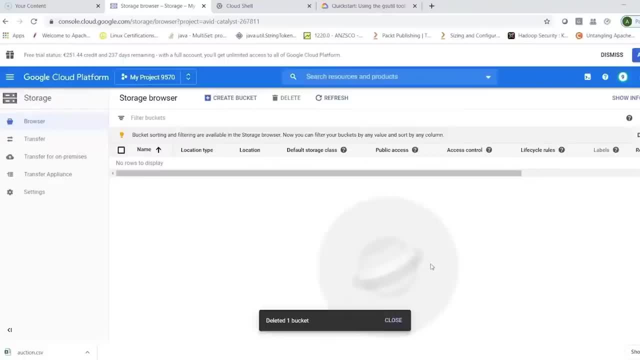 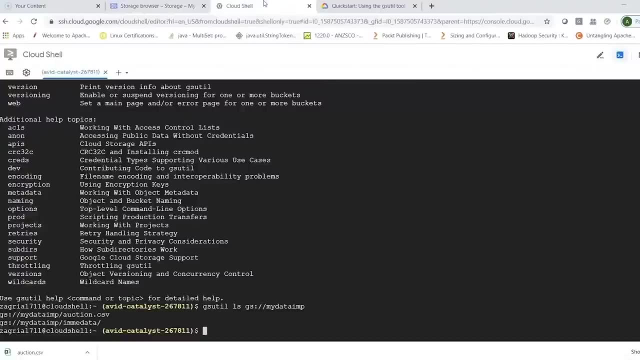 We have uploaded some data into it. We saw how you can download it Or create a folder And upload some specific data into it, And also you can do the same thing Using gsutil tools, Where in you can list your bucket. 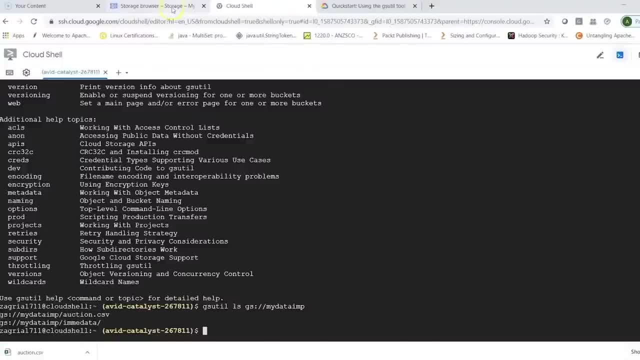 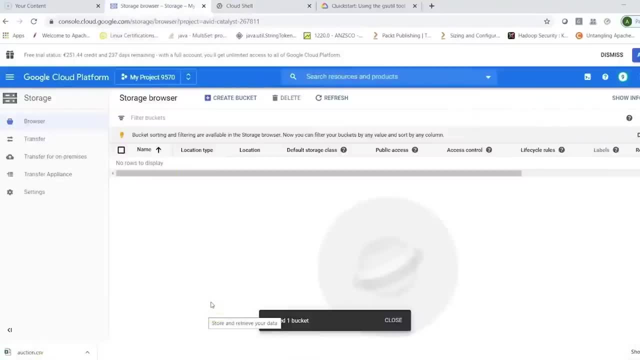 Create your buckets, Delete it, Create some folders into it. So this is in simple way. You can use your gcp, Where either you can spin up your machines Or you can use cloud storage To basically use a storage Or a easy to use instance. 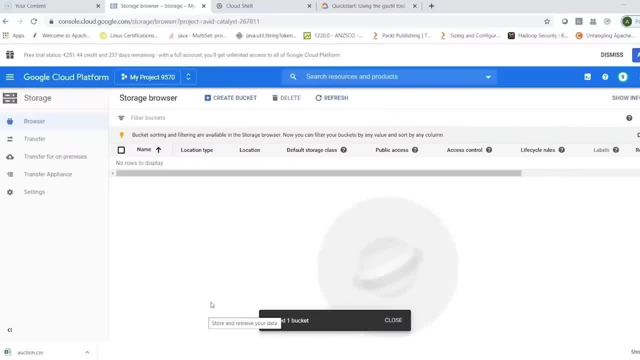 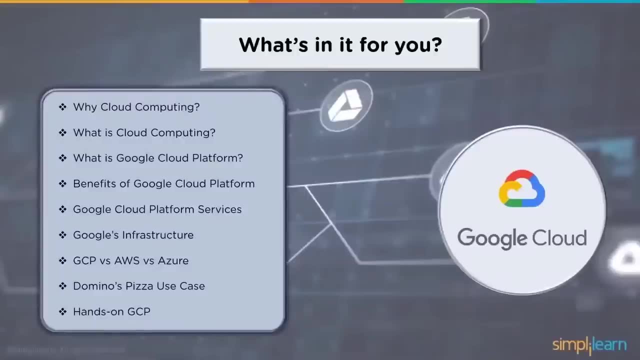 On google cloud platform. Welcome to this tutorial About google cloud platform, And here We will learn about cloud computing. What is cloud computing? What is gcp? That is, your google cloud platform, And here, What are the benefits Of google cloud platform. 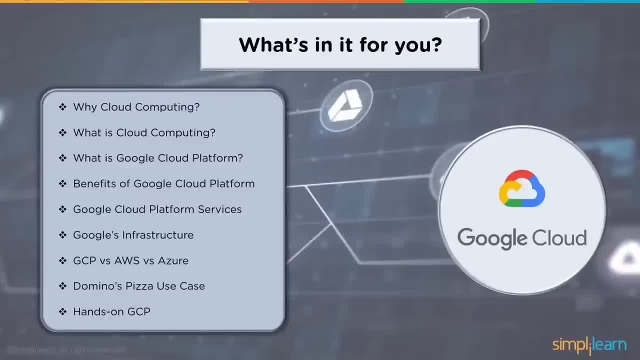 And what are its different services. A little bit about google's infrastructure: A comparison Of different cloud providers, Such as google Offering gcp, That is, google's cloud platform, Amazon offering amazon web services, And microsoft, Which offers azure. 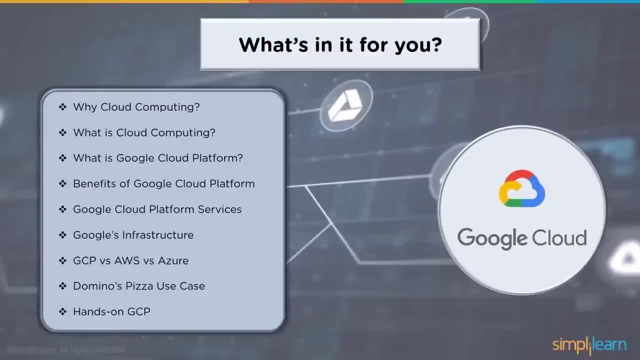 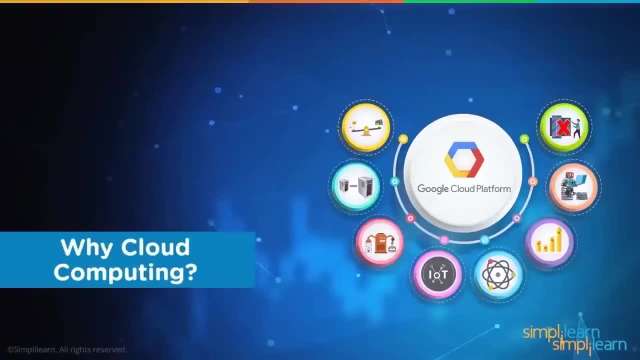 We will also learn about domino's pizza use case And then have a quick demo On using services on gcp. Before we begin, Let's understand Why cloud computing, And it would be always good To learn about cloud computing. 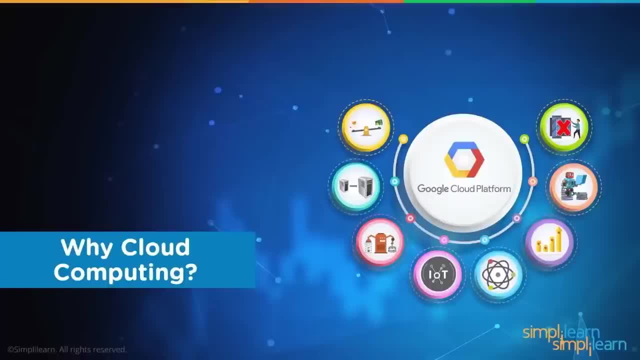 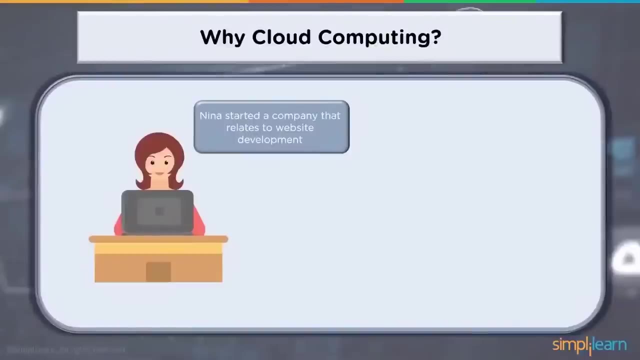 Based on a use case. There are varied use cases Where organizations are adopting Or moving their solutions Or their infrastructure Into cloud, Or I can simply say Integrating with cloud. Now here is one use case That relates to. 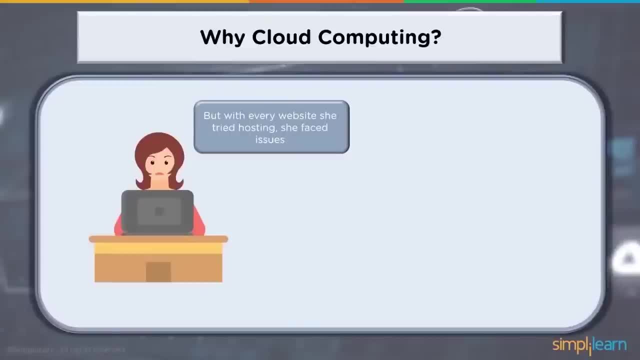 Website development. The challenges Which nina was facing Were: low memory space Whenever required For processing Or for any other kind of application Related work, High traffic to website That crashed it, And also less number of servers. Now, with these challenges, 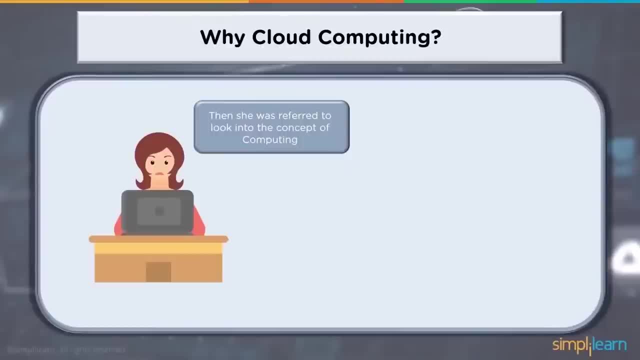 She was then referred to Concept of cloud computing So that could benefit And help her in solving her issues. Most of her issues Were solved When she started using cloud computing And with cloud computing She could increase her memory space. 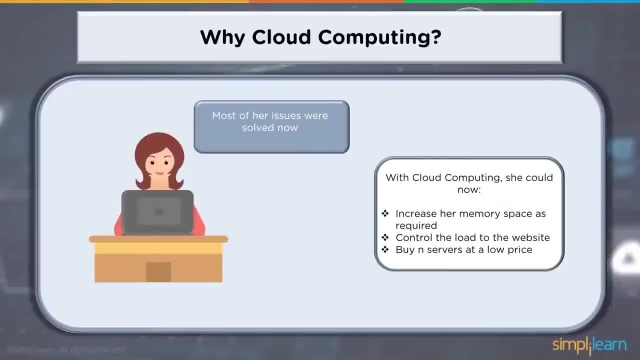 As required, That is, on demand. Control the load to the website. That is basically load balancing And handling more requests on the website Or requests per minute. Buying servers at a lower price. That is, Scaling up or down Based on the requirement. 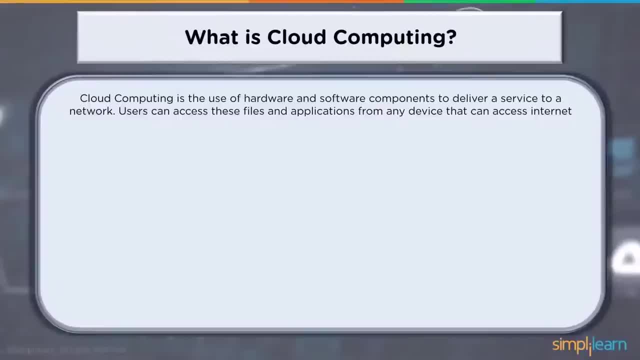 When we talk about cloud computing. Cloud computing Is use of Hardware and software components Which a cloud provider offers As a service Which can be accessed over network. Cloud computing is use Of these resources, Which could be either dedicated resources. 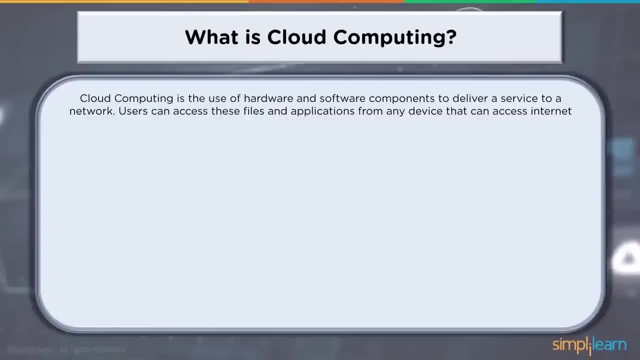 Or coming from a pool of resources Which cloud provider offers To deliver a service To clients. Users can access These different services, Applications, Files- from any device Which can basically access internet. Cloud computing allows Automatic software integration. It allows backing up. 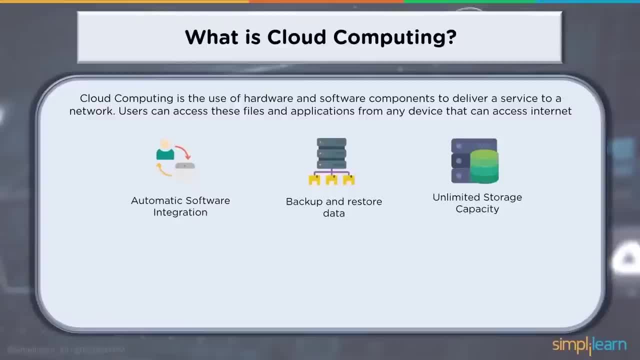 And restoring of data. It basically offers unlimited Storage, memory Or computation capacity. It gives Access to reliable sources Which usually the cloud provider Themselves are using For their use case, And it is A cost efficient model. 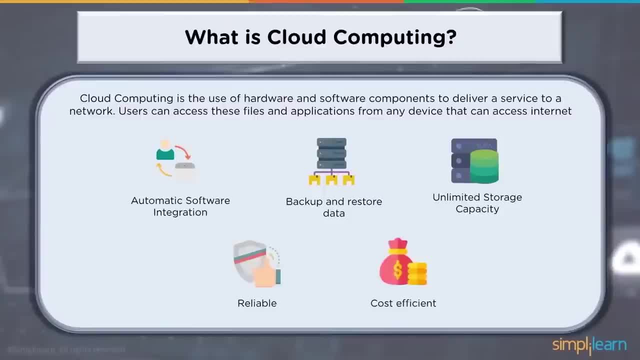 Which helps organizations To quickly Integrate or Basically modernize their Infrastructure. Cloud computing is usually Used with IT Or within IT space, Where in There are five traits: If there is a Requirement of resources As the business dynamically. 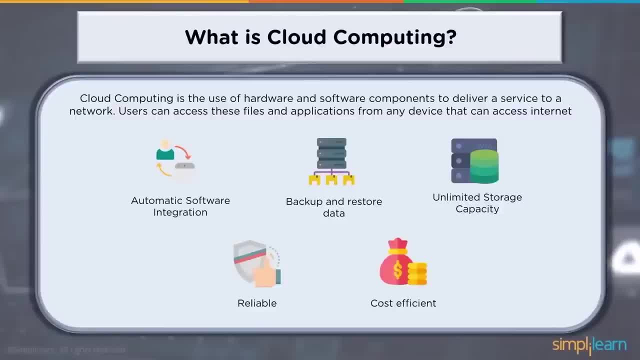 Changes or grows. So for this, cloud computing offers On demand self service, So users Could be using on demand Computing resources Or memory resources, Storage network and so on Provided by cloud provider And also do a self service. All this is possible. 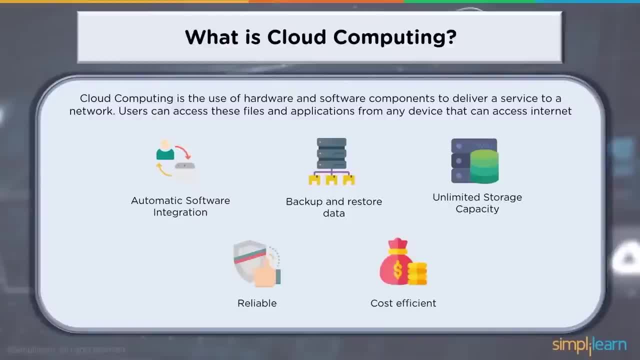 Using a simple interface And users can be Using processing power storage Network as they need And pay as they go. So there is least or no human intervention Required When it comes to projects Which might need scalable Network access. 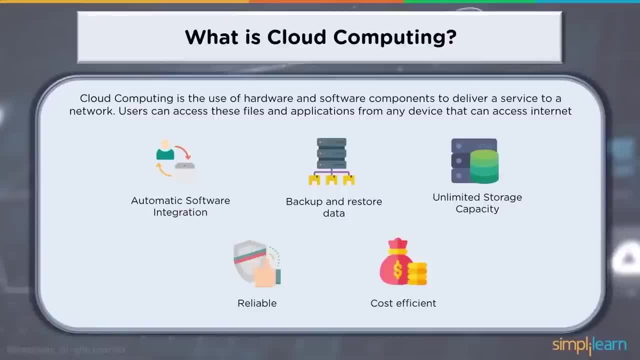 Cloud computing offers broad network access, That is, accessing resources Over network Across geographical regions, Or what we call as Zones, Which might be multiple sites Within a particular geographical region. Cloud providers also have What we call as resource pooling. 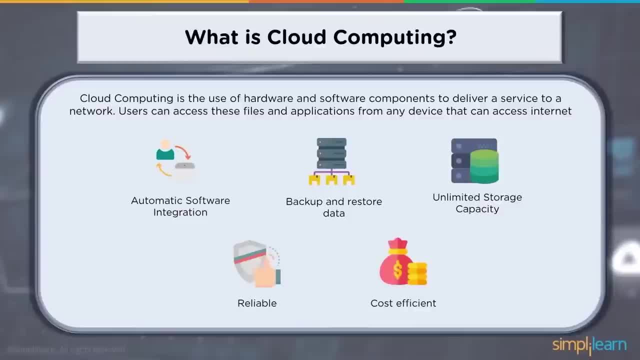 So this basically provides A huge pool of resources Which are shared And can be accessed by customers At a lower cost. Now there might be customers Which are interested in not sharing the resources And would be interested in dedicated resources, And in this case, 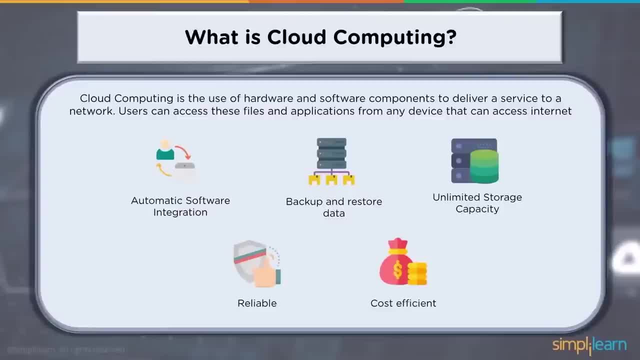 Cloud provider also have Sole tenant offerings Which help such customers. If an IT business Or any other business needs Rapid elasticity, Then cloud providers Also have resources Which are offered Which are elastic. You can get more resources rapidly. 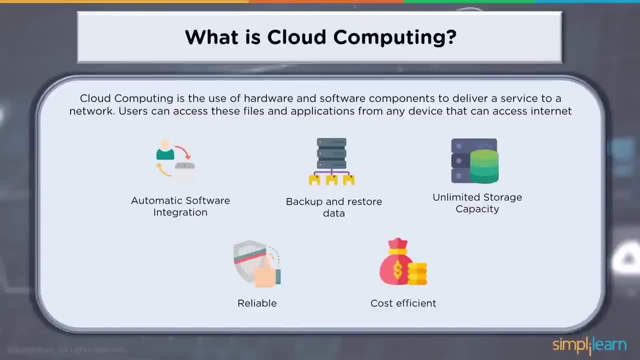 As needed, And thus you can scale up and down. Think of a gaming company Which would be interested in launching a new game And they would have predicted The number of users Which would get on to the portal Playing the game. 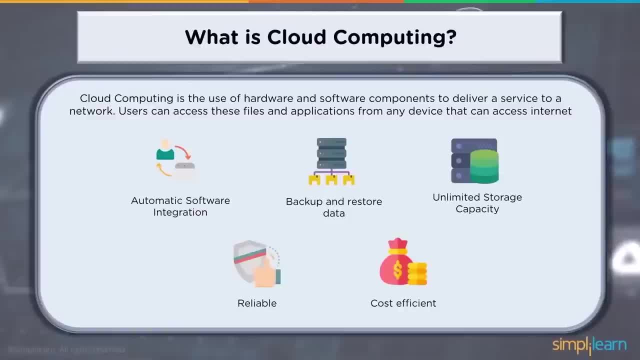 And what happens if The request per minute Or if the number of users who are joining in Might increase. Now, in this case, Organization would want An underlying solution Which handles this dynamism Scales as needed On demand. 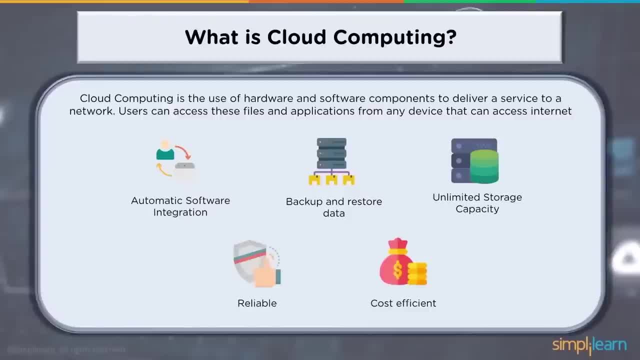 And once the demand is done, Scales down. Then cloud providers Also include measured services, That is, pay as you go model For the usage Or for the reservations Which a user or organization Would have made For resources offered by cloud computing. 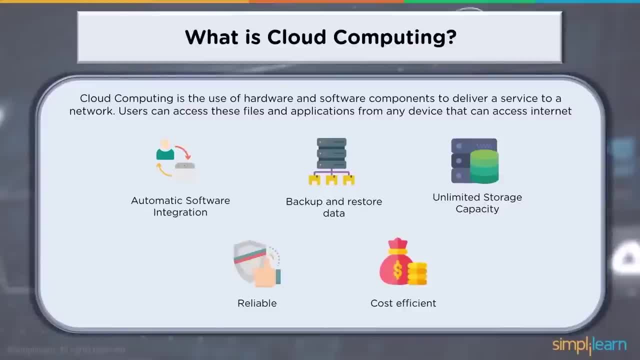 So when we talk about cloud computing, One of the question which always arises is: Why is this model so compelling? Why is this so interesting For organizations or users Who would want to use one Or many services? The first trend Which brought storage- cloud computing. 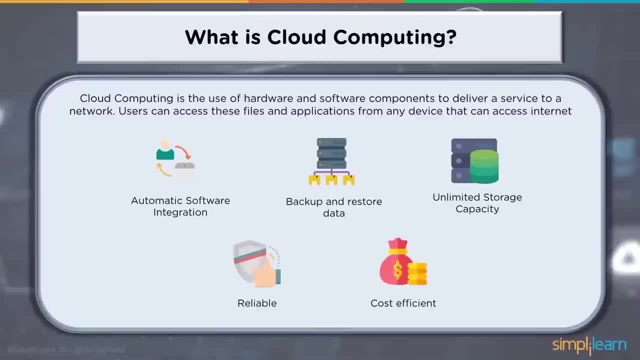 Was what we call as colo. That is, colocation. IT shops That have been using Or managing huge amount of data From decades Basically wanted to build Their infrastructures To handle their business needs. Now, instead of building, 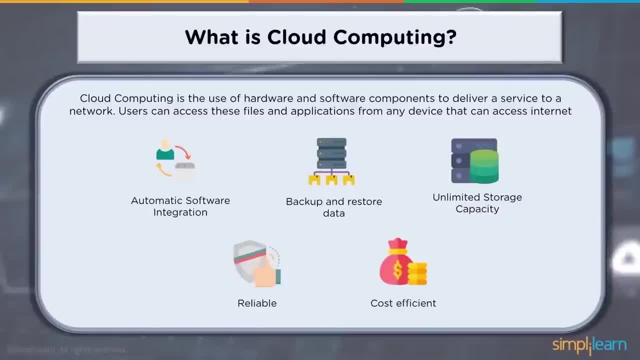 Costlier data centers. They would rent space Or share facilities. Even in past. Thus they would free up The capital for other use cases. Now this was More of user configured, Managed and maintained By them. Later, organizations started thinking. 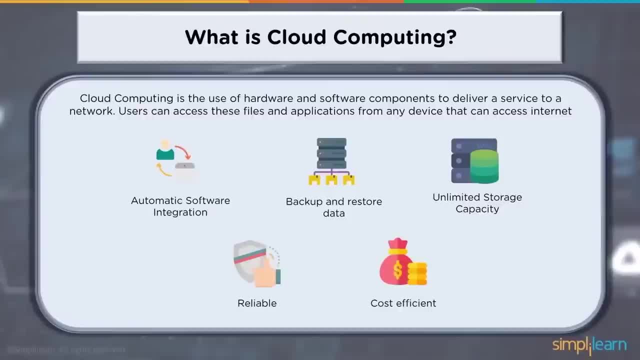 Of virtualization. So that was again user configured But provider managed And maintained. So components of a virtualized data center Matched that of a physical data center And Organizations would have Virtual devices Separately managed from Underlying devices. 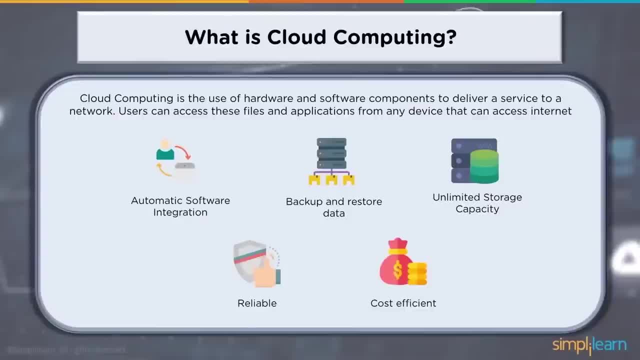 Then later came container based architectures Or basically Automated services. So within Google, Services are automatically provisioned And configured, Letting your infrastructure scale On demand. There are various reasons why An organization would think of Integrating with cloud. 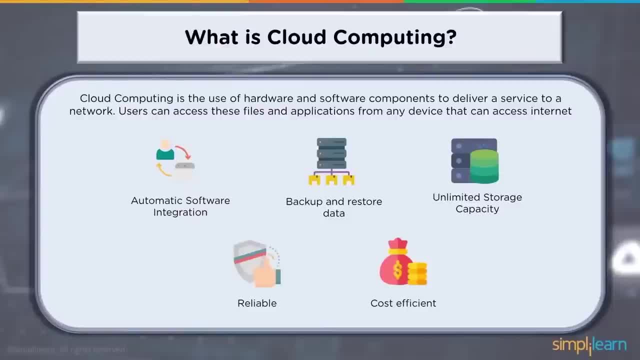 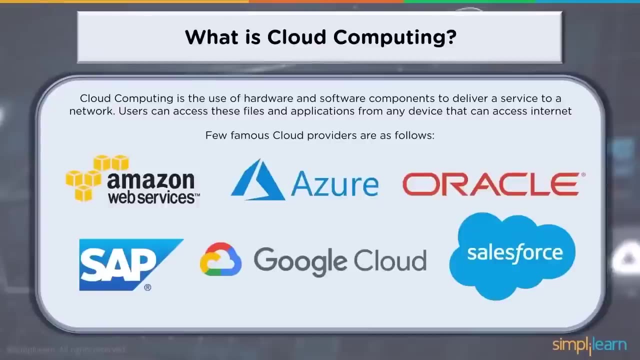 By using cloud And thus Instantaneously Reaping the benefits of modernizing Their infrastructure. Now, few famous cloud providers Are here, So you have Amazon, Which offers Amazon web services, And a huge list of services Which come in with this. 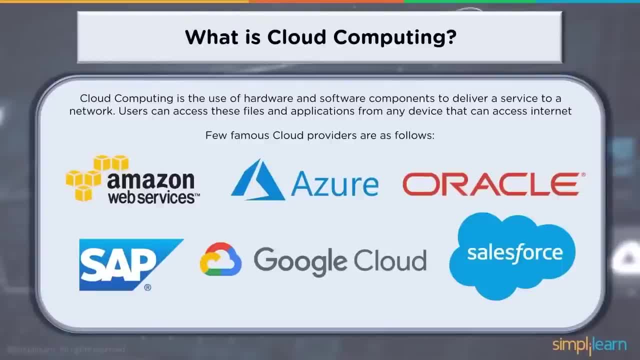 You have Microsoft's Azure, You have Oracle's cloud, You have SAP's cloud solutions, GCP, which is offered by Google, Salesforce, and so on. There are many other small players Which are also providing Different services which are cloud based. 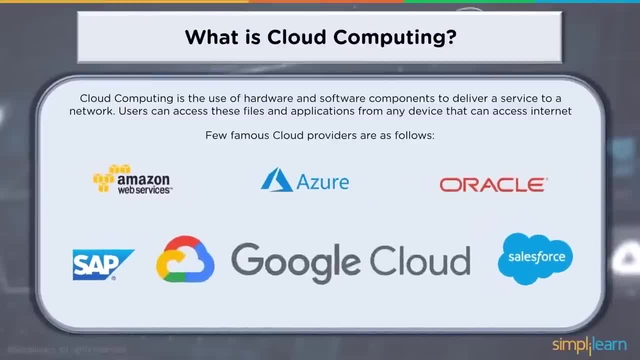 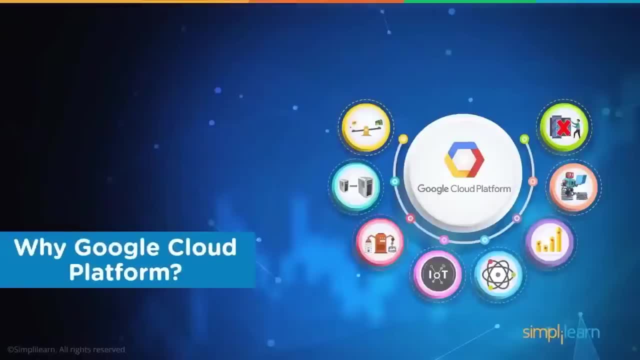 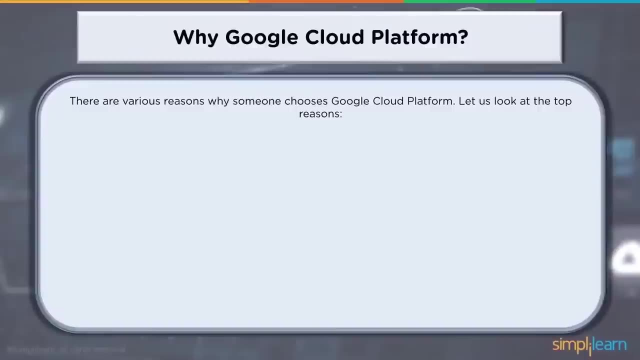 Or organizations Which are partnering with these Main cloud providers, Thus offering cloud services to their customers. When we talk about Why Google cloud platform, There are various reasons Why someone would choose Google cloud platform. GCP has better pricing Compared to its competitors. 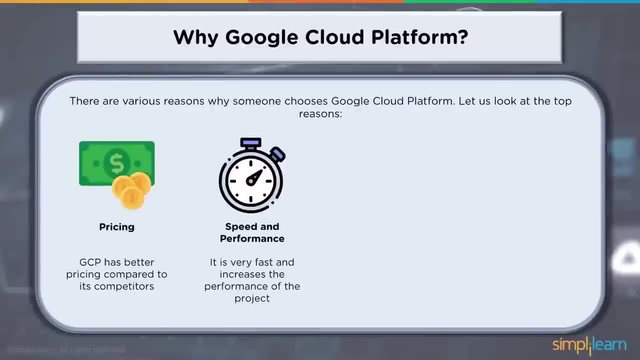 When it comes to speed And performance, It is very fast And increases the performance Of the project. Live migration of apps And there are huge number of solutions, Which I will show you further In further screens, Which help an organization to adapt. 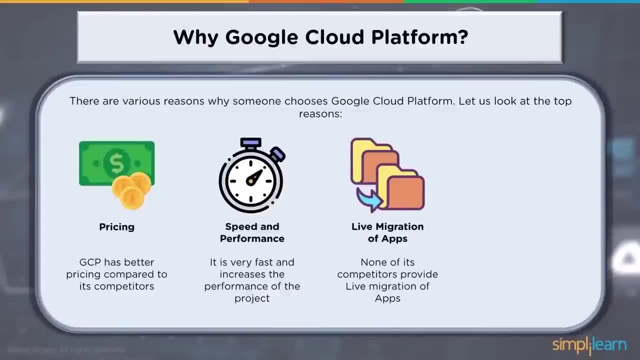 To a cloud platform Or integrate with cloud platform Or even completely migrate Into a cloud platform. None of Google's competitors. When we talk about big data, AI, Machine learning kind of solutions, GCP provides Lot of innovative solutions. 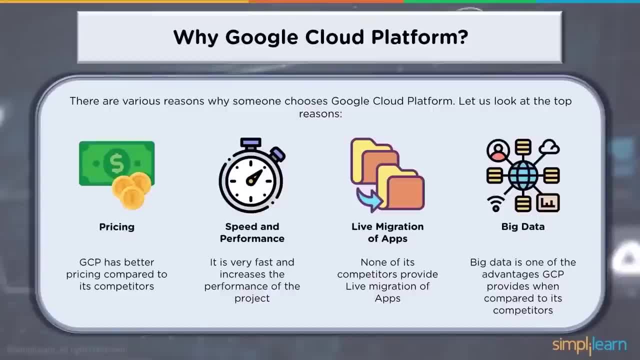 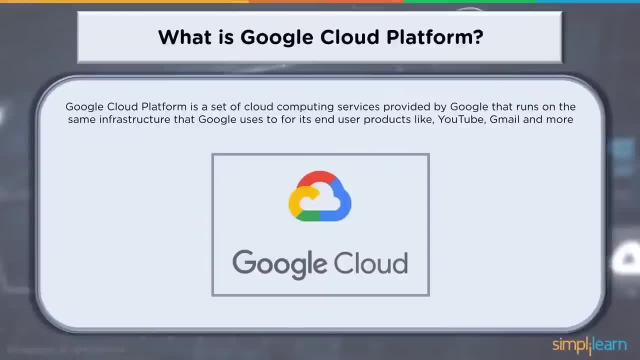 In comparison to other cloud providers Such as AWS, Azure and so on. So What is Google cloud platform? It is a set of cloud computing services Provided by Google That runs on the same infrastructure That Google uses To and from. 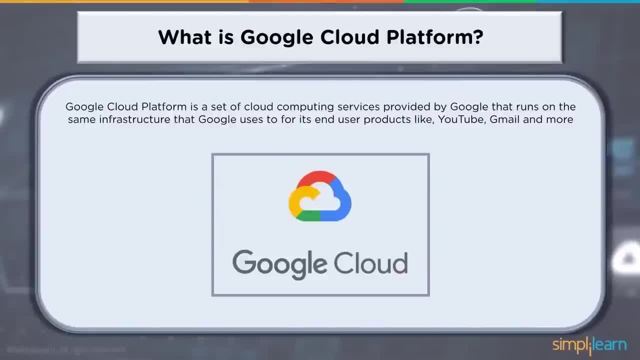 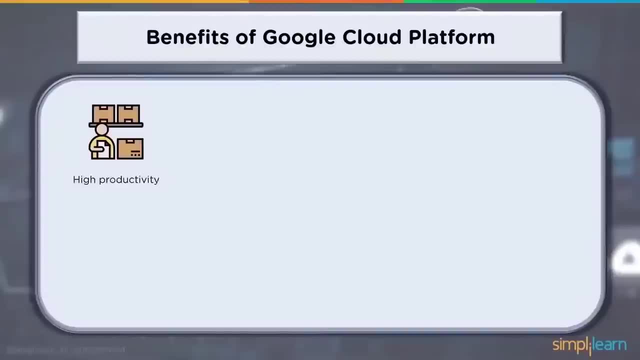 For its end user products Like YouTube, Gmail And so on. Let's learn about benefits Of Google cloud platform, Such as high productivity, Working from anywhere, Quick collaboration, High security, Fewer data stored on vulnerable devices, Reliable resources. 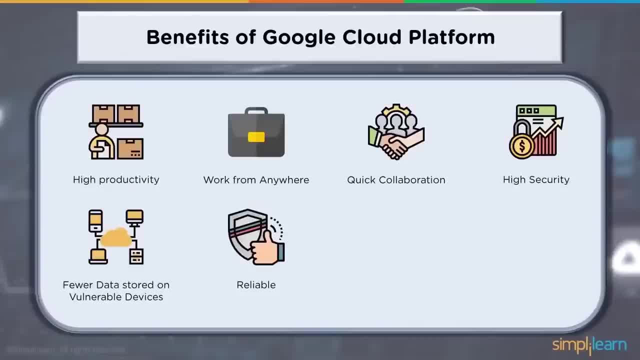 Which can be used across organization, Across geographical regions, Across countries. And flexible, Which allows organizations to scale up and down As the demand rises Or as the demand declines, And cost effective solutions For various use cases. These are some of the benefits. 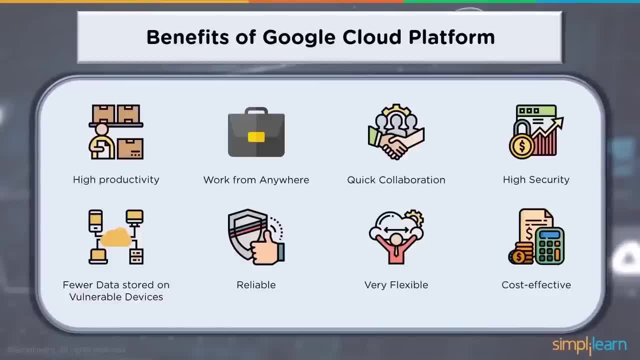 And if we look into different services Which Google cloud platform offers, We could look into Detailed benefits Which each service offers In a different use case, Which basically helps Organizations In different domains Handling different kind of small, Mid or larger businesses. 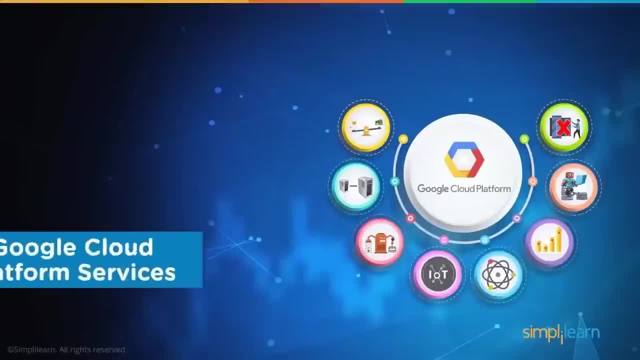 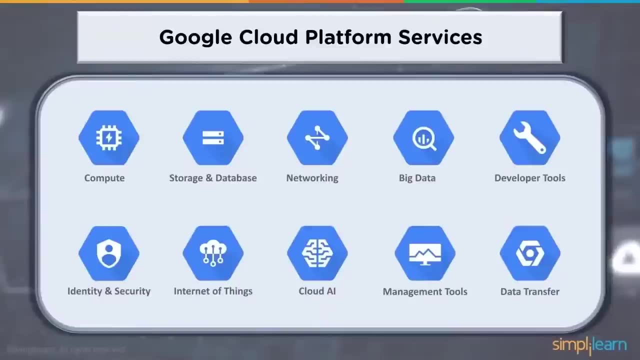 And with different business goals. When we talk about Google cloud platform services, Here is a list of services, Or I could say high level Domains or categories of services. So you have compute Related services, You have storage and database. 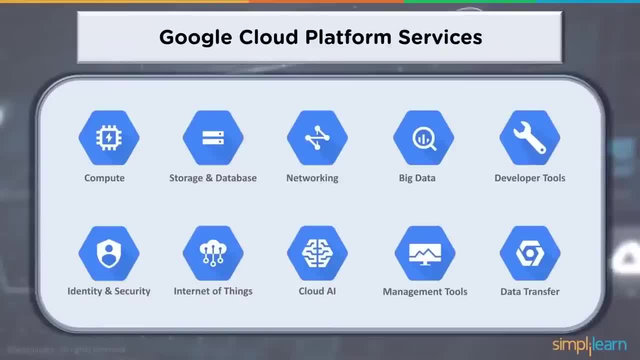 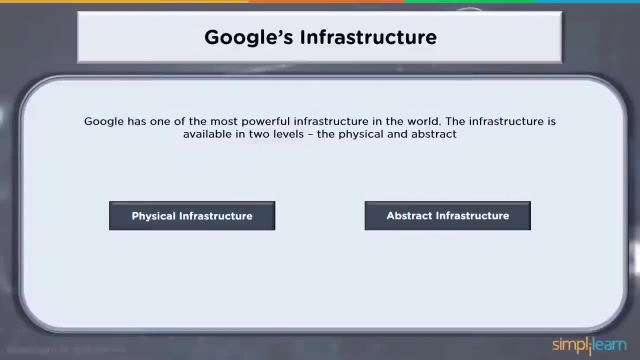 You have networking, Big data, Security management, Internet of things, Cloud, AI Management tools And also data transfer solutions. When we talk about Google's infrastructure, Google has one of the most Powerful infrastructure in the world. The infrastructure is available in two levels. 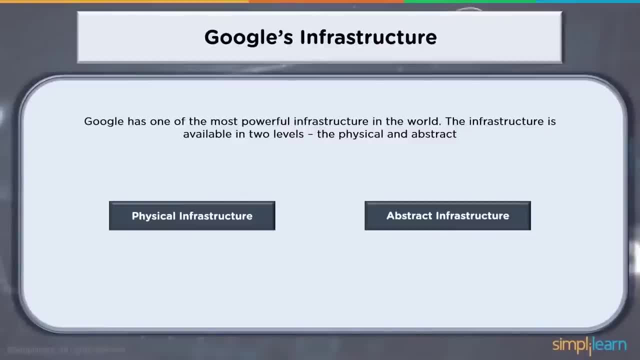 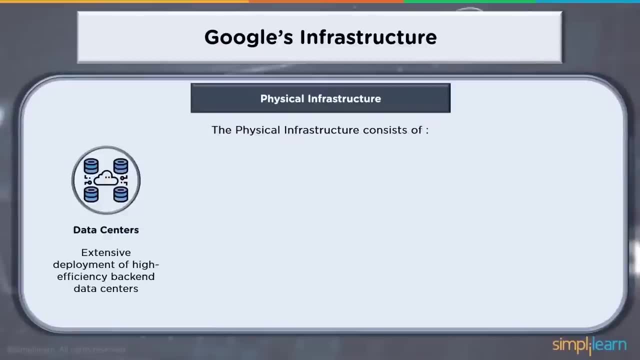 The physical and the abstract layers. You have physical infrastructure And then you have the Abstract infrastructure. Physical infrastructure And then you have Data centers: Extensive development of high efficiency Back end data centers. You have a very strong backbone network. 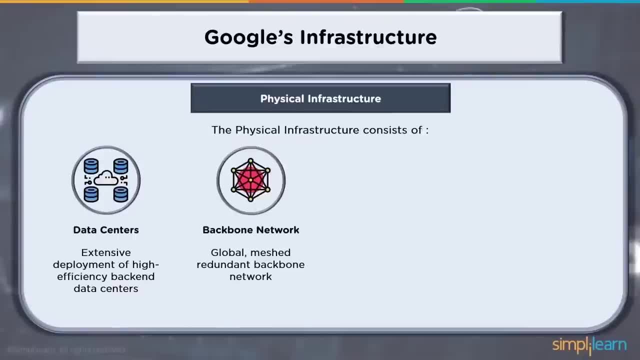 Which is used by Google itself And also offered As services to customers Via GCP platform services. So you have global, Meshed, redundant backbone network Points of presence. When we talk about Google Data centers, You have multiple points of presence. 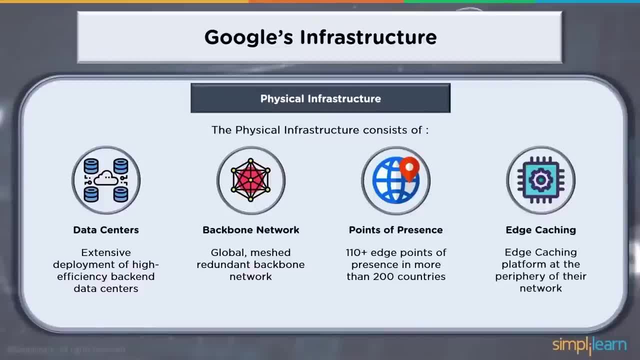 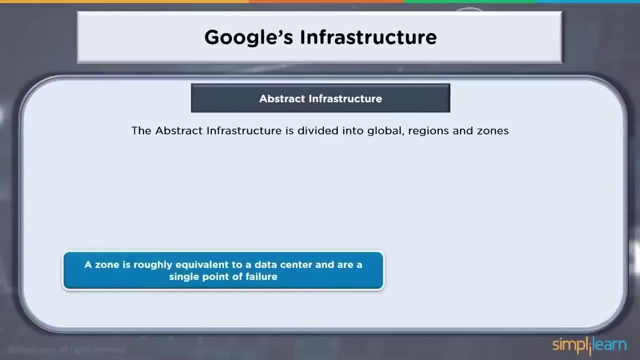 In more than 200 countries And when we talk about edge caching, Edge caching platform- At periphery of their network. So this is What defines the physical infrastructure Of Google. Now, there is much more to it, Rather than just these four points. 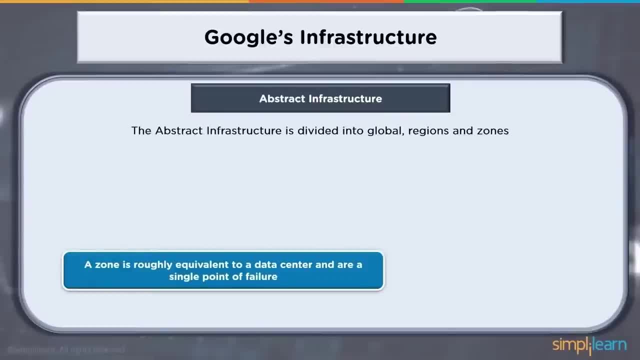 When we talk about abstract infrastructure, That is divided in global Regions and zones, When we talk about Data center And a single point of failure. So you could have your compute engine Which is within a zone, Or you could say compute engine. 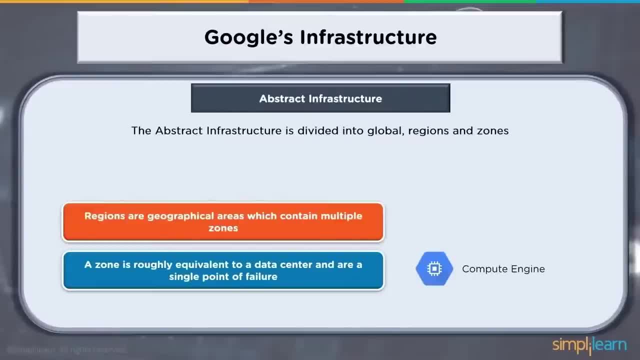 Is a zonal resource. You have regions which are geographical areas Which contain multiple zones, So you could have a region For US central Or Europe central, Europe west and so on, And within a region You would have one or multiple zones. 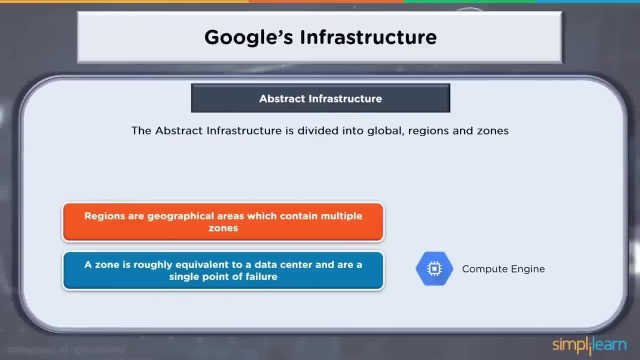 And zones basically Allow high availability Of resources. So you have cloud- Load balancer is an example- Which is regional resource. Then you have global resources And they are available and shared Across the planet, So you have various global resources. 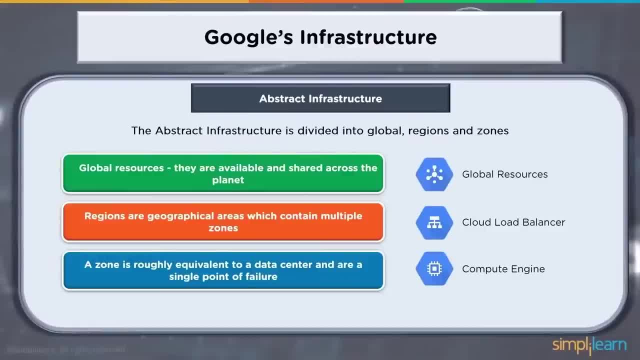 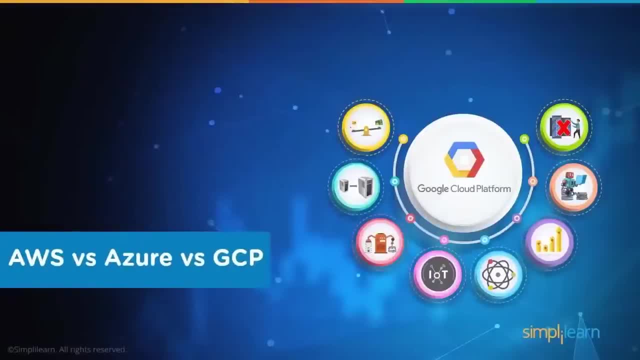 Such as network, Which could be even your IP addresses, and so on. Now Let's do a quick comparison Of AWS, GCP And let's look at What each cloud provider offers. Later we will also look into different services. 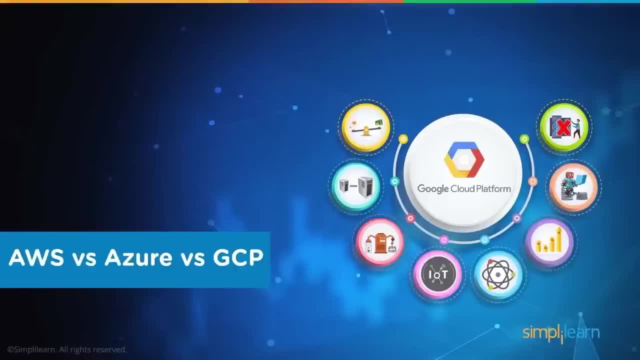 In detail When it comes to Google cloud platform, What each service does, What you can benefit from, Which service should you use In what case. We will learn about those in later slides If I compare Your different cloud providers When we talk about. 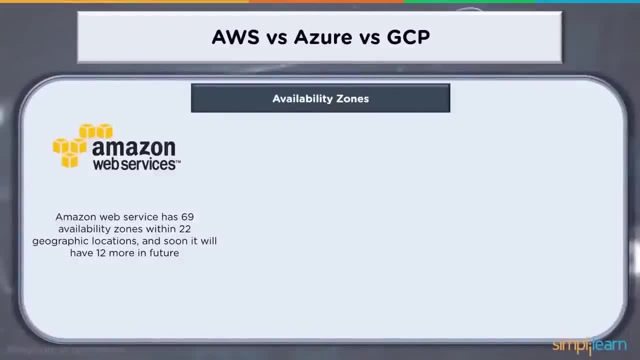 Amazon, It's cloud offerings, That is, Amazon web services, or AWS As we well know it. Amazon web services has 69. Availability zones Within 22 geographical locations, And soon it will have 12 more in future, So this number keeps growing. 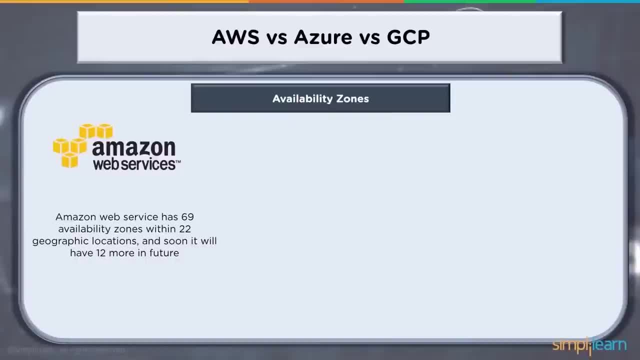 Based on the spread Of the services which A particular cloud provider offers. Here we are talking about Availability zone, specific information. When we talk about Microsoft's Azure, It has 54. Availability regions worldwide And is available in 140 countries. 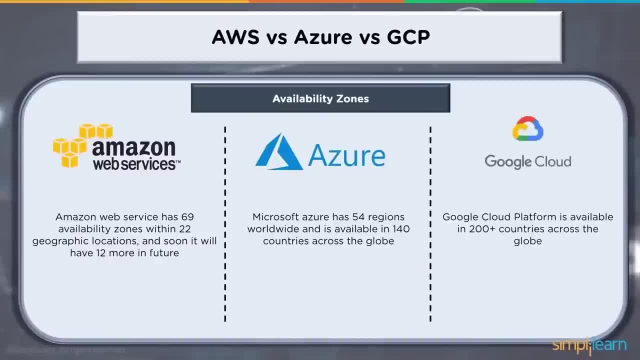 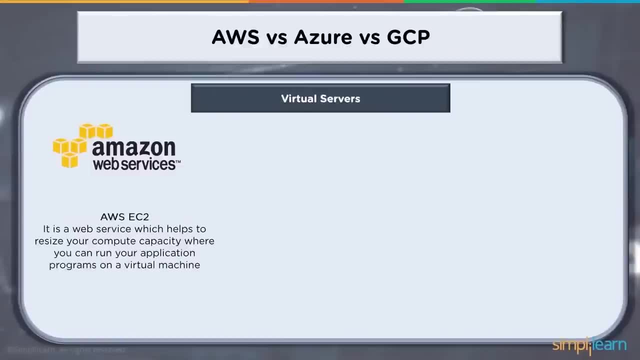 Across the globe. When we talk about Google cloud, Google cloud platform is available In 200 plus countries Across the globe. When we talk about virtual servers, Amazon's EC2.. That is elastic compute cloud. It is a web service. 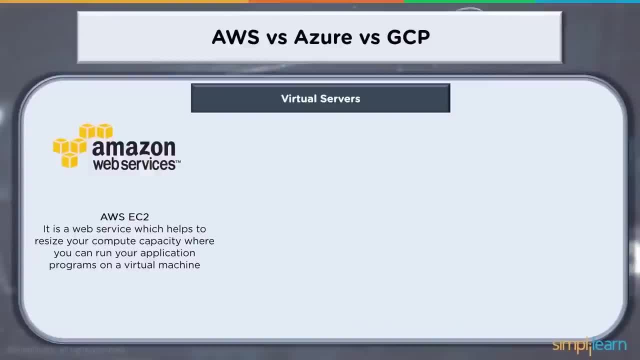 Which basically helps to resize Your compute capacity, Where you can run your application Programs on a virtual machine. You could launch Virtual instances that could have Any distribution of Linux, Windows. You could have different specifications When it comes to RAM or CPU cores. 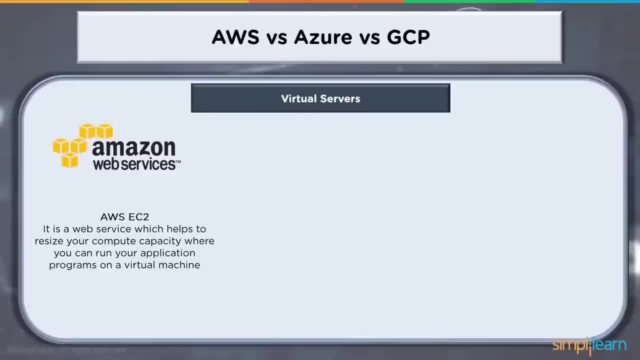 Or disk. You could also decide on What kind of storage A particular instance should use, Whether the storage should be local to the instance, Or whether that should be Elastic file system Or even an object storage. When it comes to 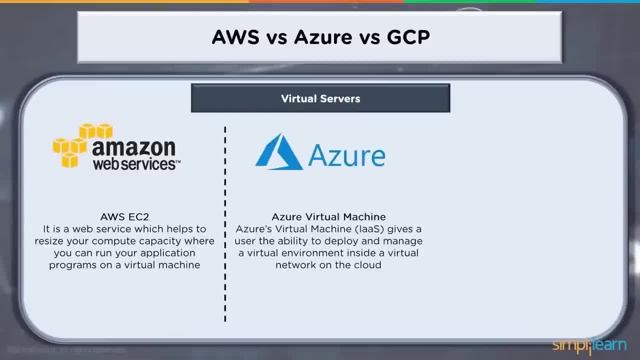 Azure or Microsoft's offering. Azure virtual machine- That is, infrastructure As a service- gives a user The ability to deploy And manage a virtual environment Inside a virtual network On the cloud, And this virtual network on the cloud Would be managed by cloud provider. 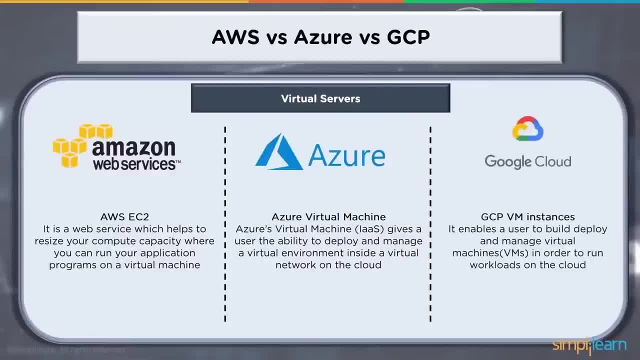 Google cloud Or the offerings From Google cloud platform, That is, GCP VM instances- Enables users to build And deploy And manage virtual machines In order to run Different kind of workloads on the cloud. Now, when we talk about compute engine, 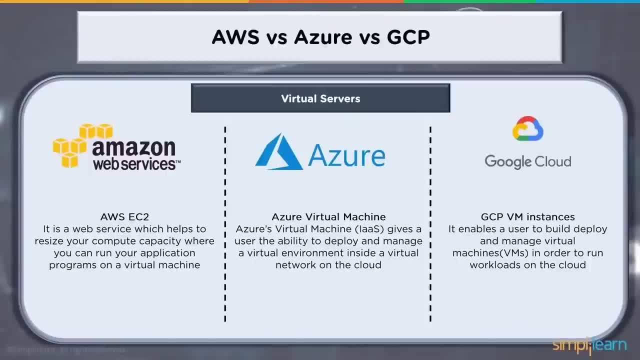 Here it would be good To discuss a little bit More about compute engine And what are the different options Which Google cloud offers. So when you talk about Your compute engine, You have scalable, High performance virtual machines. Compute engine delivers. 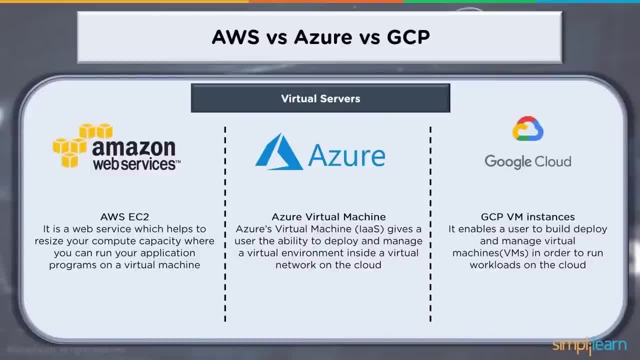 High performance virtual machines In Google's data center With access to high performance Networking infrastructure And block storage, And you could select VMs for your needs. That could be general purpose Or workload optimized. And when we talk about workload optimized, 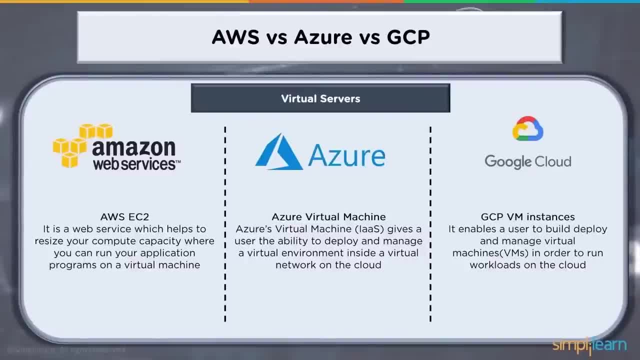 You have predefined machines Or you have custom machine sizes. You can integrate compute With other Google cloud services, Such as AI or ML. You have, when we talk about Your GCP VM instances. Just to expand on that, You have general purpose instances. 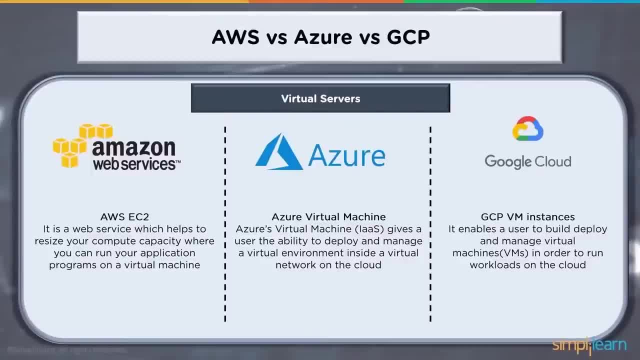 Which we call as N2.. Which provide a balance Between price and performance, And they are well suited For most workloads Including line of business applications, Web servers and databases. Google cloud also offers Compute optimized instances, Which we call as C2 instances. 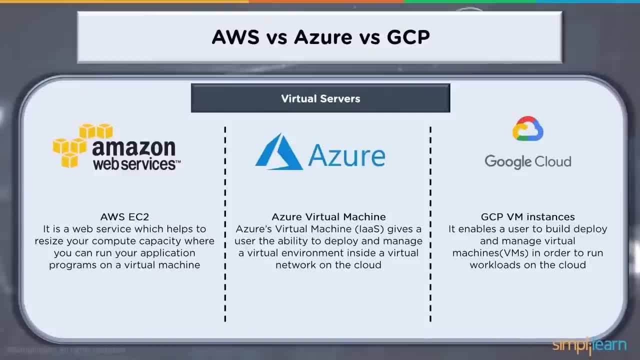 Which offer Consistent high end Virtual CPU performance, Which are good for AAA, gaming, EDA, HPC And other applications. Now, when we talk about compute optimized Or general purpose, How would we leave memory optimized instances? Those are M2 machines. 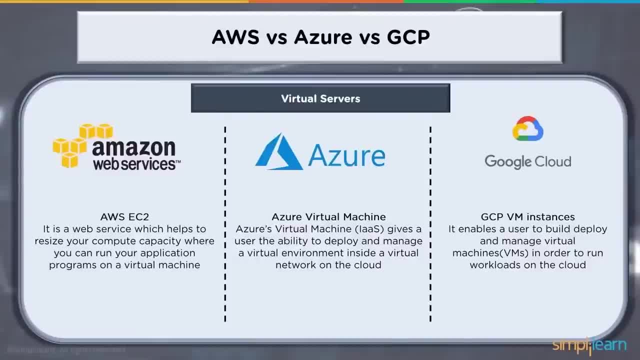 Which Google offers, So these offer highest amount of memory. These VMs are well suited For in memory databases Such as SAP HANA Analytics, And in memory caches. So if I would summarize this, When we talk about different instances, 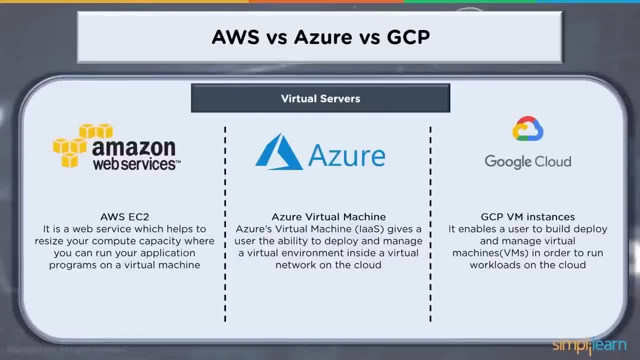 AWS Also offers different kind of instances, Which are memory Or compute Or disk optimized. You have general purpose And each category of machines Has a different pricing model. You can always go to an AWS website, Look for the pricing models. 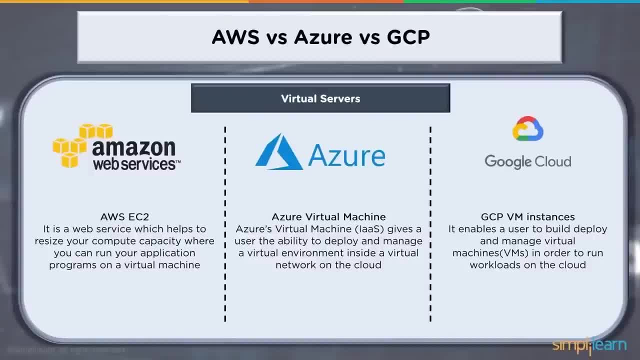 And that will give you an idea of Reserved instances or dedicated instances, Reserved instances and so on. Similarly, If you talk about Google cloud, Google cloud also has instances With various options, Which become the key features Of why customers would choose. 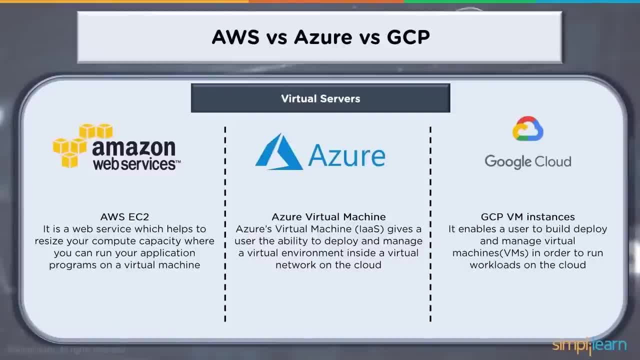 Google cloud platform, Such as live migration for VMs, So compute engine Within your GCP Can live migrate Between host systems, And when I say live, migrate without rebooting, which keeps your application running even when the underlying host systems require maintenance. you also have preemptible virtual machines wherein you can run bad jobs. 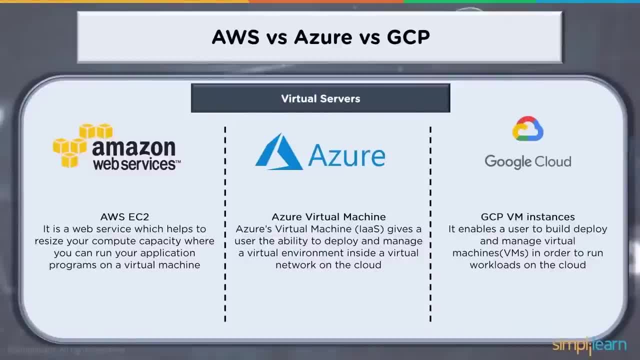 and fault tolerant workloads on preemptible bms to reduce your virtual cpu and memory cost by up to 80 percent while getting the same performance. so these are your preemptive or preemptible virtual machines. the only demonet is these can give you a really cost efficient resource usage. 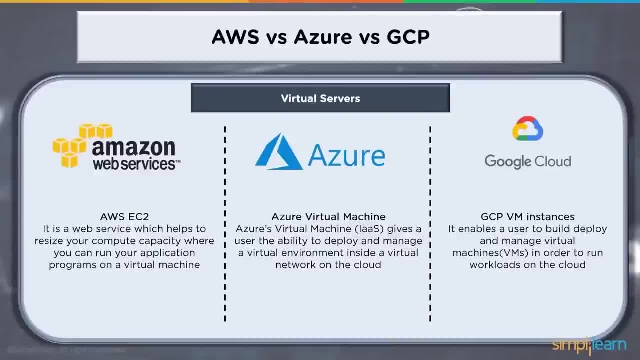 however, can be taken off the shelf anytime, and that's why we call them preemptible virtual machines. you also have sole tenant nodes, which are physical compute engine servers dedicated explicitly or exclusively for users use case, and when we talk about sole tenant nodes, these are usually good when you are dealing with or when you're working with your applications, which we 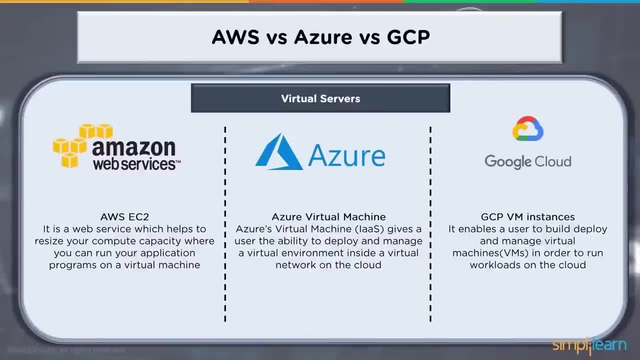 call as bring your own license applications, so sole tenant nodes give you access to same machine types and virtual machine config options as regular compute instances. so there are different options which google cloud offers when it comes to these instances which we are talking about and it takes care of different use cases in comparison to other. 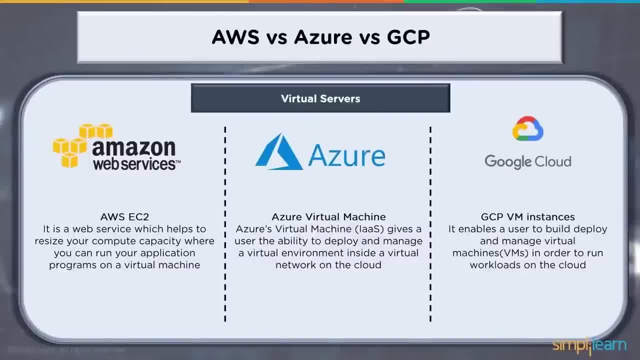 cloud providers which are also offering these services, such as: you can have predefined machine types. you can have custom machine types, preemptible vms- as i said, live migration of vms. you can use persistent disks, which could give you durable, high performance block storage. you have local ssds. you 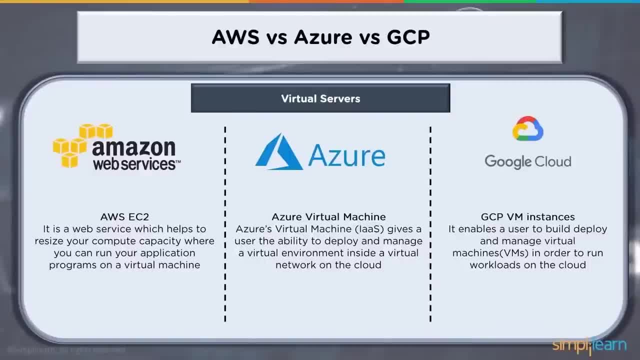 also have gpu accelerators, which can be added to accelerate computational intensive workloads such as machine learning, simulation, medical analysis and so on. and you have features such as global load balancing, which makes google cloud a unique choice when we talk about platform as a service amazon has. 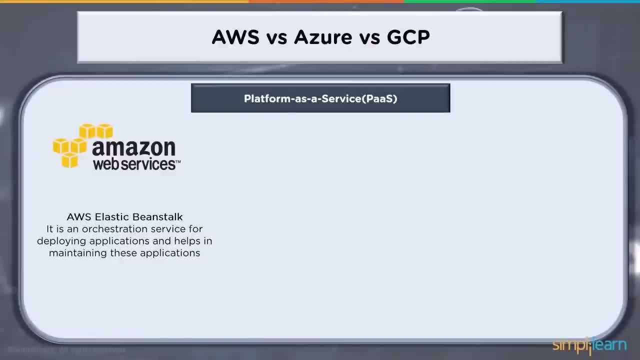 platform as a service offering which we call as elastic beanstalk. among one of its services, it's an orchestration service for deploying applications and helping in maintaining these applications. azure cloud service provides a platform to write the user application code without worrying about the hardware resources. google app engine is a service used by developers for building and hosting applications on google's 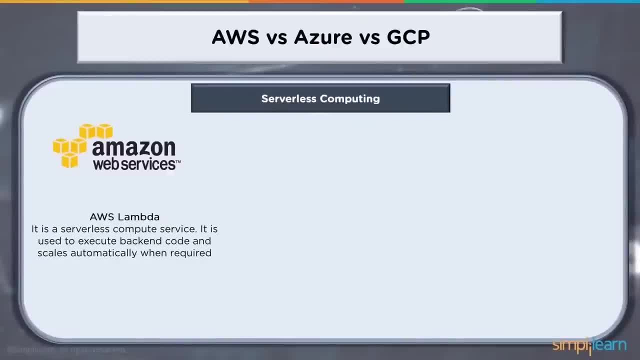 data centers when we talk about serverless computing. so amazon's aws lambda is a serverless compute service. it is used to execute back-end code and scales automatically when required. when we talk about azure, you have something called as functions, which allow users to build applications using serverless, simple functions with a programming language of their choice. when we talk about google, 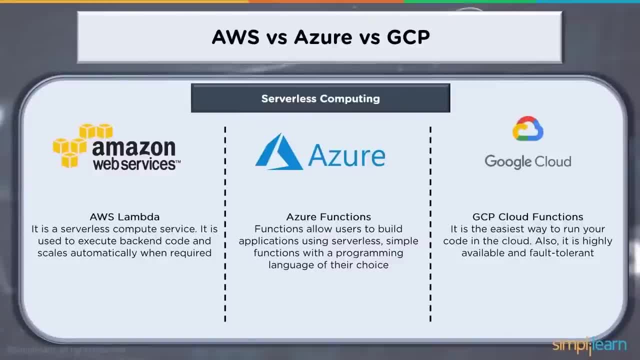 cloud. gcp has cloud functions, which is easiest way to run your code in the cloud, and it is highly available and fault tolerant. so, in these days, when we are talking about microservices architecture which organizations are preferring, when we are talking about organizations which can scale, which can dynamically change their underlying architecture, organizations would be interested. 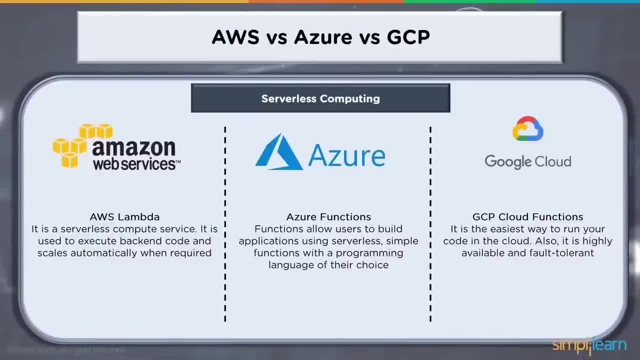 in serverless computing, where they do not have to have a infrastructure setup a planned in advance before going for their use case, and this is where monolithic applications are really not a preferred choice. a lot of organizations are decomposing their applications into microservices based on. 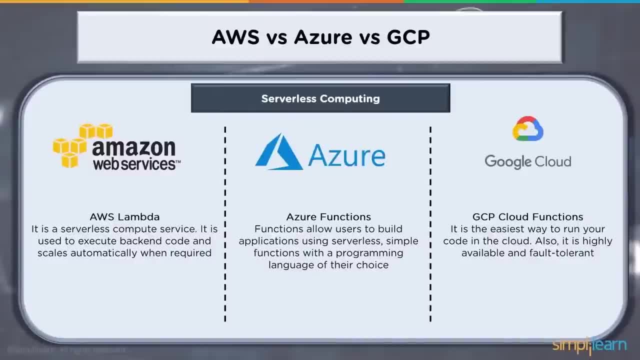 business capability or decomposing based on subdomains. we can learn about microservices architecture later, but just to know that, serverless computing, which basically helps any organization if, for example, if you have a web application that receives non-linear traffic and you cannot keep an eye on your 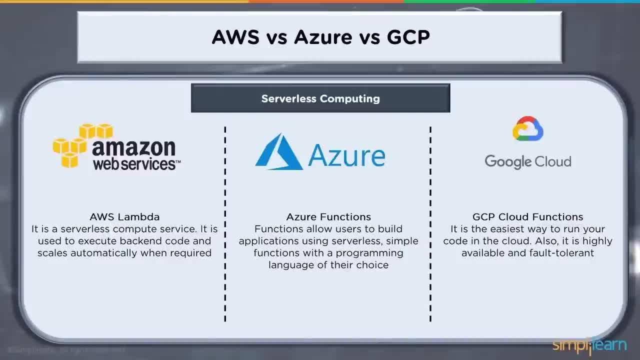 serverless computing, which basically helps any organization. if, for example, if you have a web application that receives non-linear traffic and you cannot keep an eye on your server always, it would be good to have someone to auto scale your application. serverless is basically a computing model where cloud service provider is responsible for managing the piece of code without the 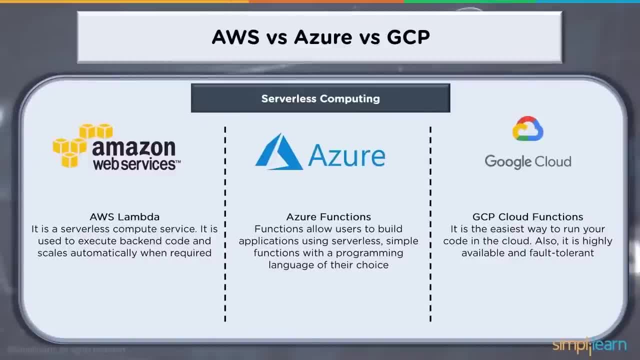 developer having to bother about infrastructure setup, management, maintenance and so on. now, when we talk about applications being serverless or benefiting from serverless computing, one of the key things that we need to know is that, when we are talking about applications being serverless, key things would be: zero administration, so deploying application without any provisioning, and 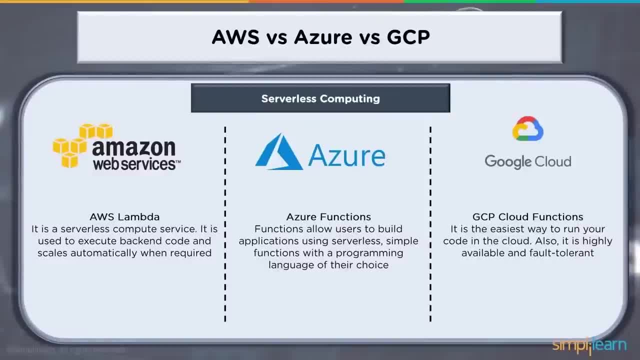 management auto scaling capability, that is, let the service provider worry about scaling the application up and down. you have pay-per-use model, which any customer would want to benefit from. that is, pay only for the resources that you have used or that you are continuing to use. right, shorten the time between idea implementation and 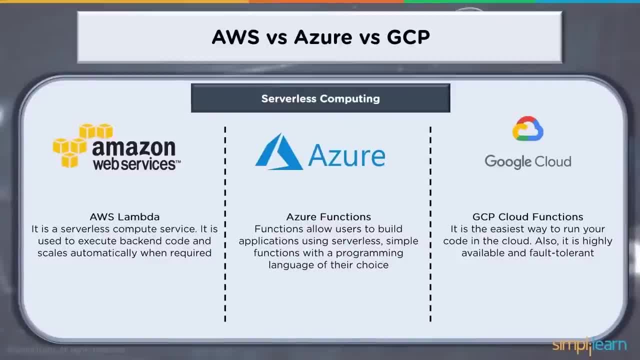 implementation, and then you have to pay for the resources that you have used or that you are going to use. in terms of the deployment- and this is something which any organization would want- that you would want a faster bring to the market solution timeline in comparison to getting 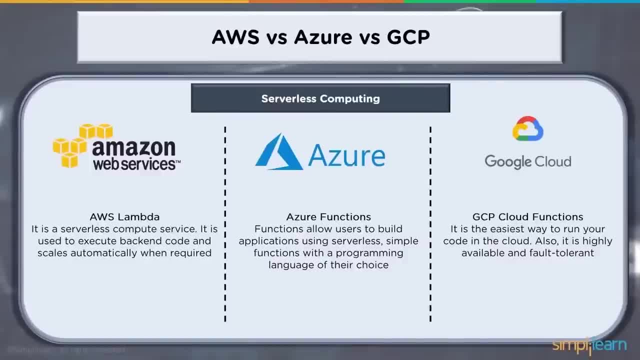 entangled with deployment, management and maintenance of your underlying infrastructure when your applications are facing a high demand. so when we talk about serverless, it is a function as a service, because each part of your application is divided as functions and can be hosted over multiple service providers. You have serverless apps which are usually divided. 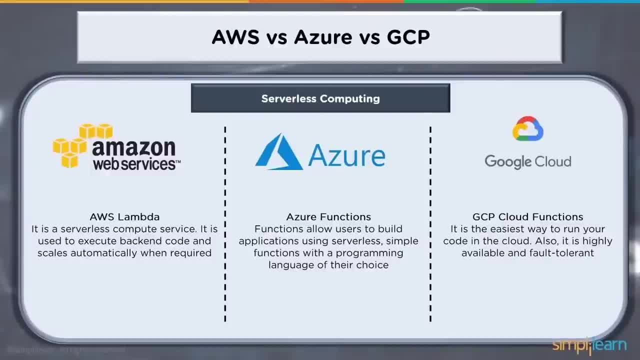 as separate units or functions based on functionalities or domains and so on. So serverless computing is gaining quite popularity these days, in comparison to the traditional three-tier architecture where you had a presentation layer, you had an application layer, you have a database layer. Now that kind of infrastructure is not really preferred in. 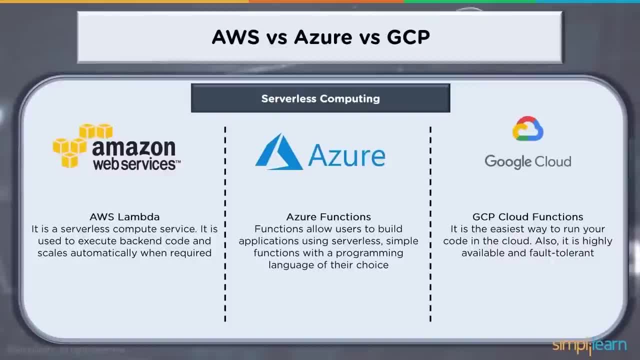 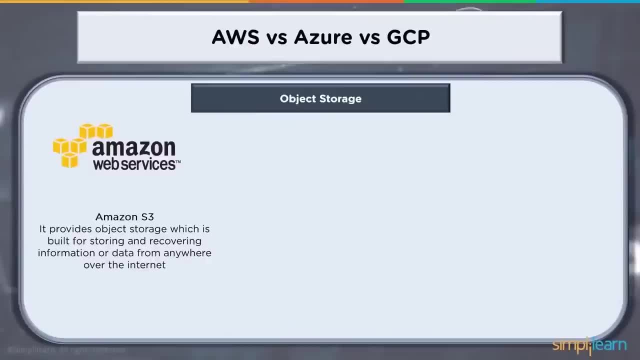 today's modern times, when organizations are working on different kind of newer applications. When we talk about object storage, Amazon has simple storage service. that is S3. It provides object storage which is built for storing and recovering information or data from anywhere over the internet. Azure comes up. 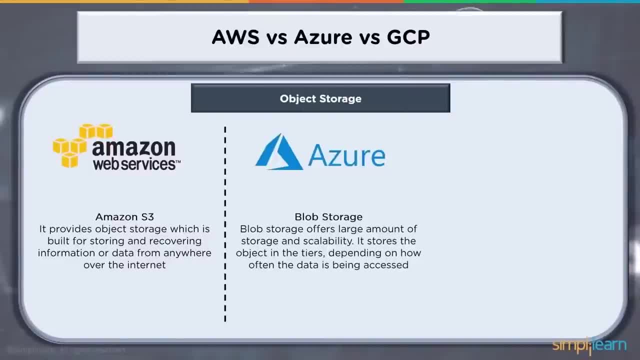 with blob storage, that is, binary, large objects storage. It offers large amount of storage and scalability. It stores the object in the tiers and depending on how often the data is being accessed. Now same thing applies to even S3, which is from Amazon, So S3 also. 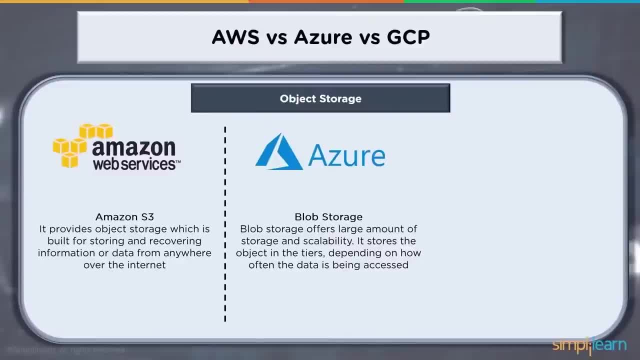 has different kind of storage classes which can be selected when a user or an organization intends to use a storage service. And when I speak about storage classes, it basically means having a frequent access storage or a infrequent access storage, or what we call as just an archival solution. Google Cloud has cloud storage and it provides unified object storage. 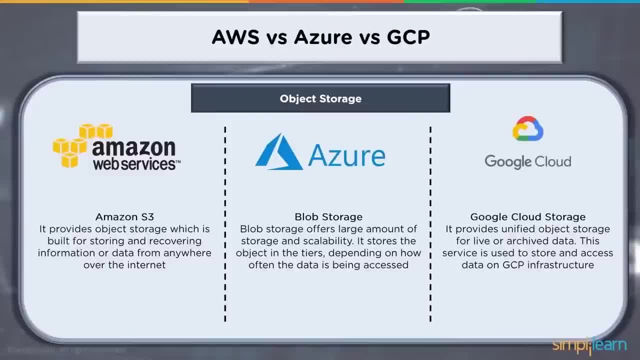 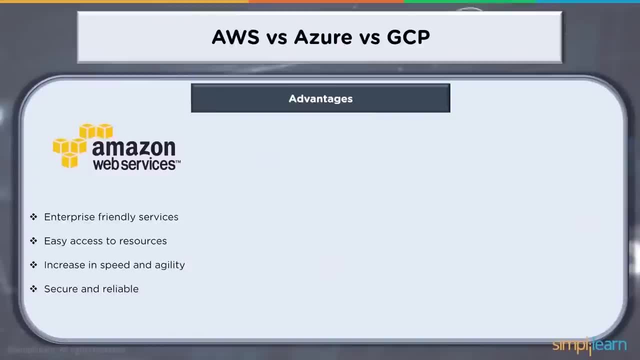 for live or archive data. The service is used to store and access data on GCP infrastructure. When it comes to advantages, Amazon Web Services has enterprise-friendly services, easy access to resources, increase in speed and agility, and that too, on demand and takes care of. 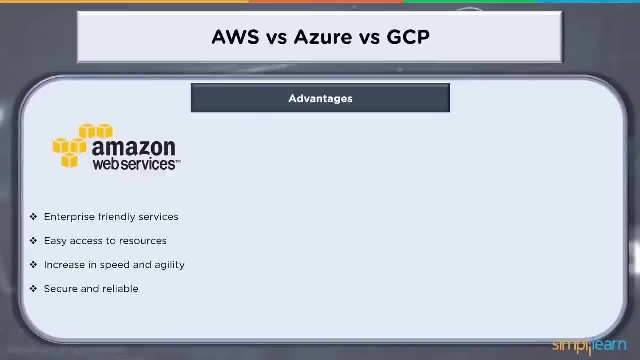 your security and reliability of resources which are offered. When it comes to Azure, it has better development operations. strong security profile, provides a lot of cost-effective solutions and operation execution Friendly. When we talk about Google Cloud, one of the key features here is better pricing than 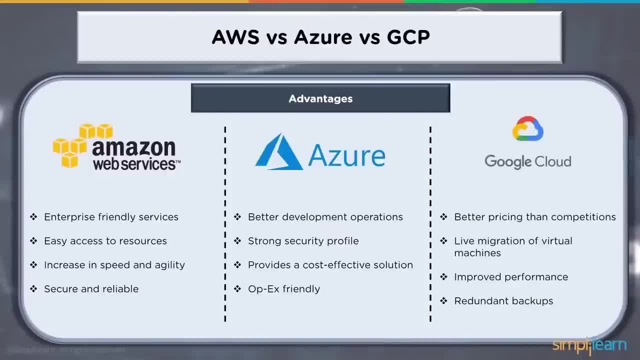 competitors. live migration of virtual machines, which really interests a lot of organizations would want to modernize their infrastructure without having any kind of disruption in their existing services: improved performance, redundant backups, and so on. When it comes to disadvantages in AWS, you have limitations. 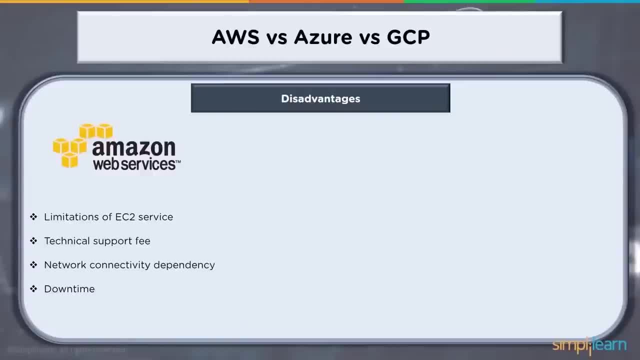 when it comes to EC2 service. well, there are different options in the kind of machines which you can choose, which you can work on. You have a technical support fee which is incurred, network connectivity and then also downtime, which might be in case when you're migrating. 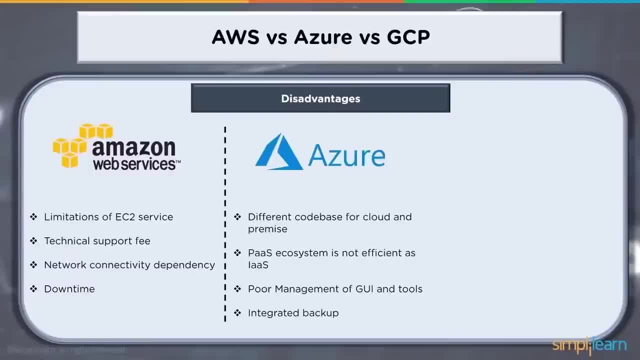 Azure. it has different code base for cloud and premise. platform as a service ecosystem is not really as efficient as infrastructure as a service of GUI and tools. integrated backup. When we talk about Google Cloud, support fee is quite hefty. It depends on what kind of solution or support you would or organization would be. 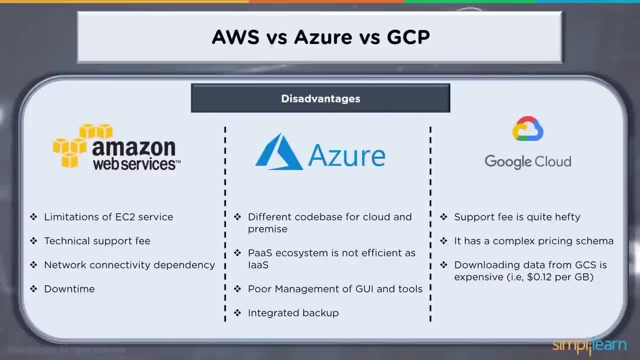 interested in. It has a complex pricing schema, although it has different use cases for which any user or any organization can benefit from. Downloading data from Google Cloud services is an expensive option. Storage might not be, However, uploading data or downloading data. 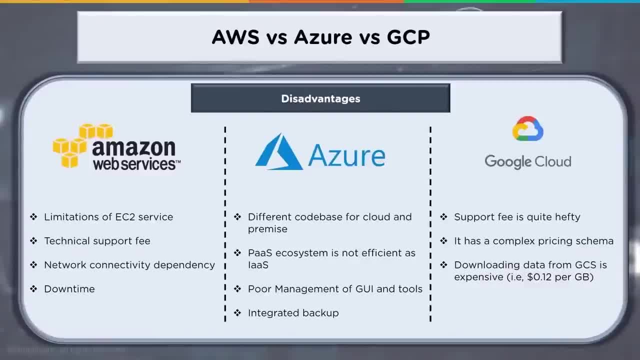 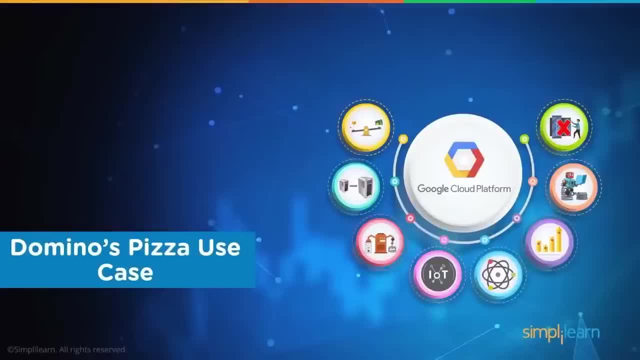 would be an expensive option. When we talk about Domino's Pizza use case now, while we were discussing about these features, I would really want to spend more time in discussing each of these features or services in detail, such as: you have compute engine, you have storage. 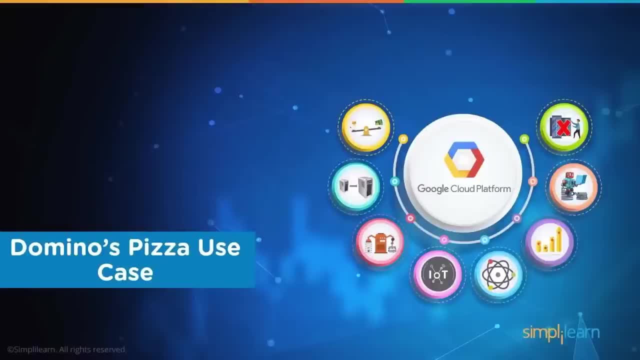 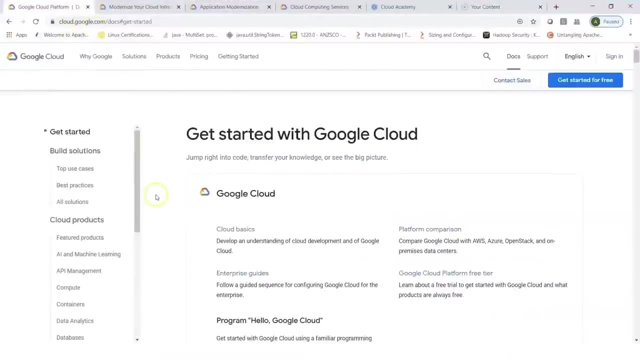 you have big table, you have data proc and so on, So there are a huge list of services. Now, before we get into your Domino's Pizza use case, let me show you this page on Google Cloud where you can look at different services. So if you go to cloudgooglecom and if you look at, get started, 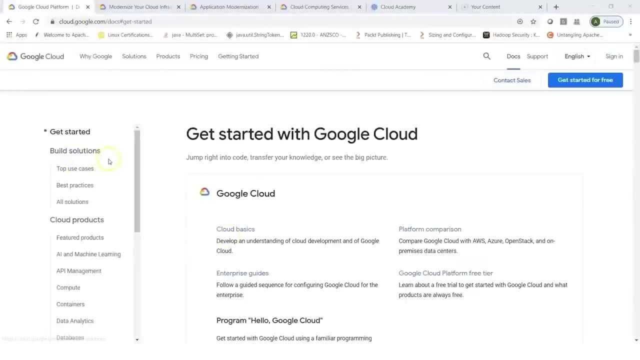 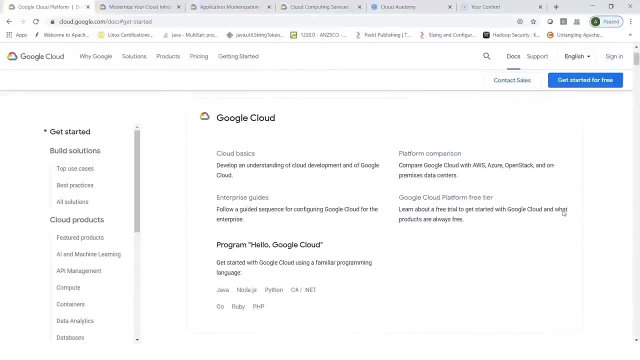 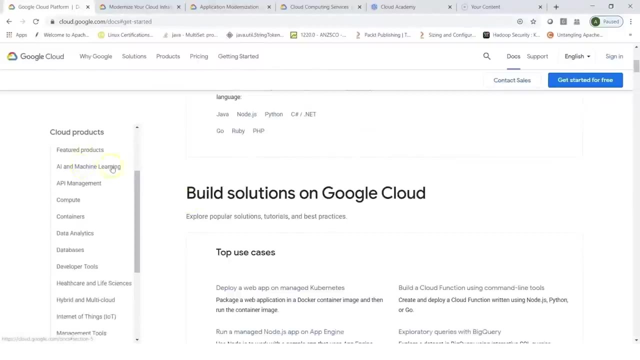 option under docs. so here you can find build solutions, look at different use cases, learn from cloud. what are cloud basics? Then you can look at different cloud products. So here you have products in different categories, such as AI and machine learning, API, management compute. 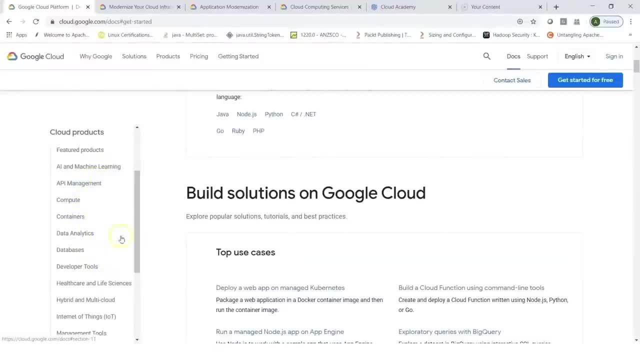 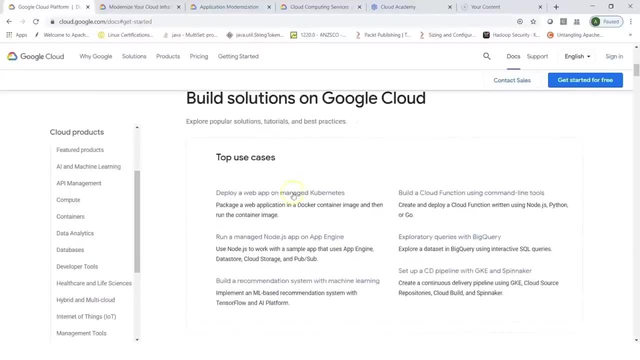 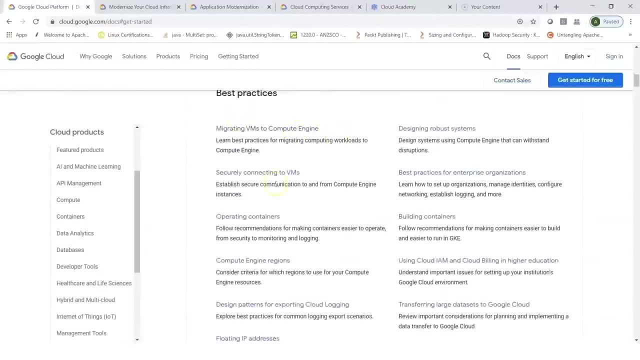 containers, data analytics, databases, developer tools and so on, And you can always click on any one of these to look into different solutions which are being offered. what are the different use cases? what are the best practices when it comes to migrating VMs to compute engine? 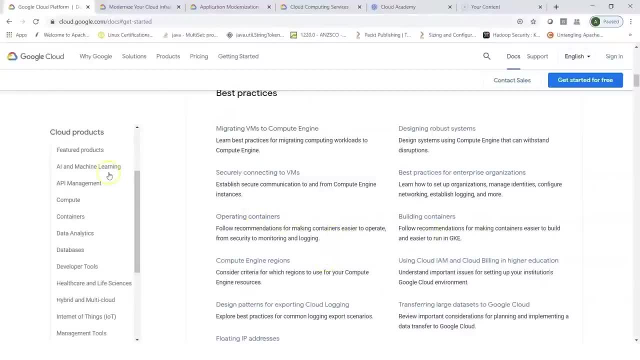 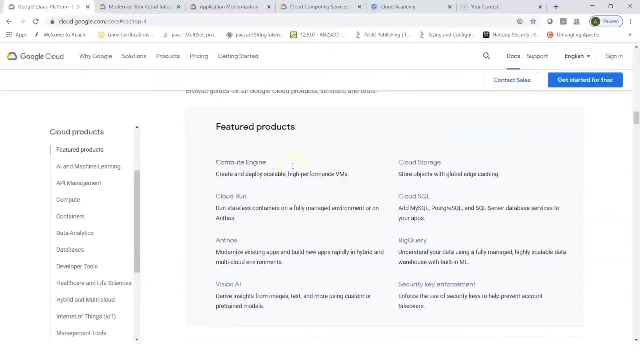 Or operating containers, or building containers and so on. You can always look at featured products and that gives you a quick snapshot of what are the different products, such as you have compute engine, you have cloud run big query, which is a data warehouse. you have cloud SQL, which is a 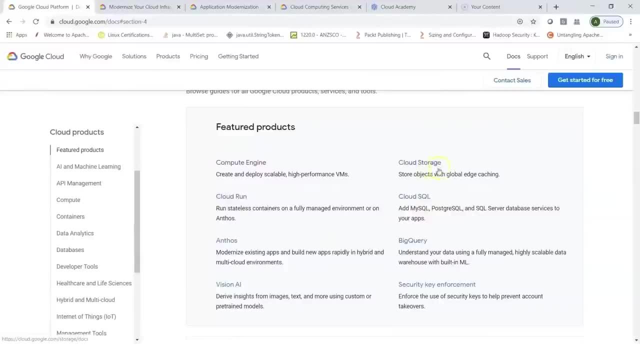 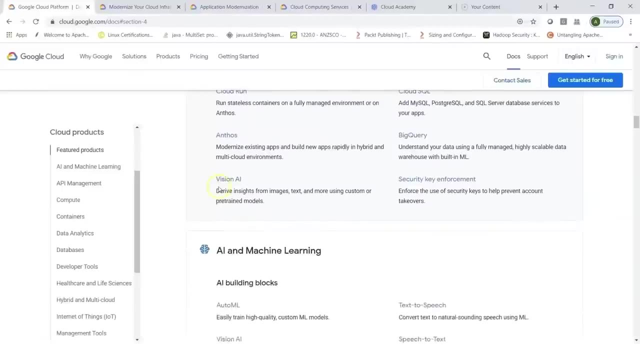 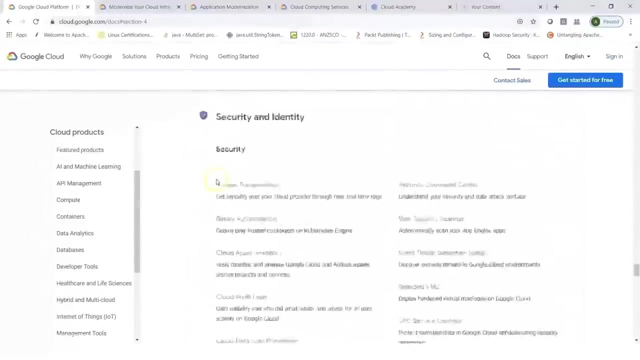 managed MySQL or Postgres. you have cloud storage to basically push in any kind of data there. you have security, key enforcement, AI and machine learning and so on. So you have different featured products. Now, if you scroll down to the lower end of this page, you can again look at. 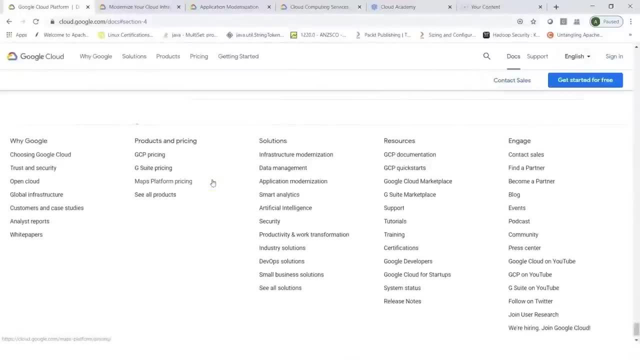 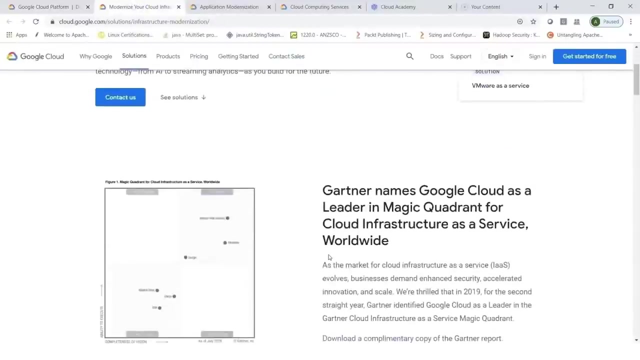 different solutions and that would be really interesting to read and learn from. So you have infrastructure modernization, you have application modernization, you have data management and so on. So if I look at infrastructure modernization, you could basically look at the solutions which. Google Cloud offers and what it does when it comes to migrating VMs to compute engine. So you can really look at different solutions and that would be really interesting to read and learn from. So you can really look at different solutions and that would be really interesting to read and learn from. So you can 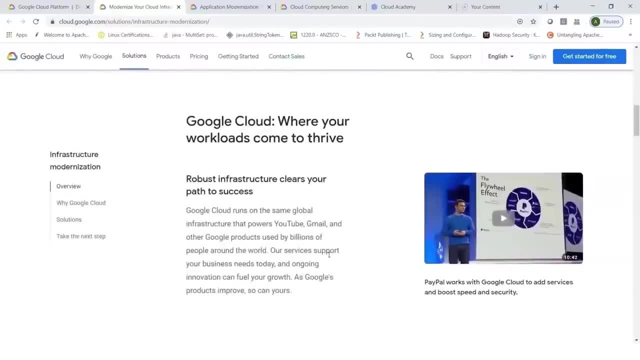 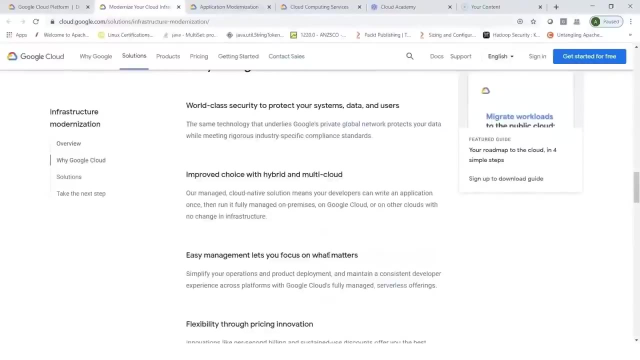 to having your infrastructure modernized or benefiting by integrating with cloud and having immediate benefits of infrastructure modernization. You can look at different use cases, what they are doing, how Google Cloud really helps when it comes to migrating the workloads to a cloud and how 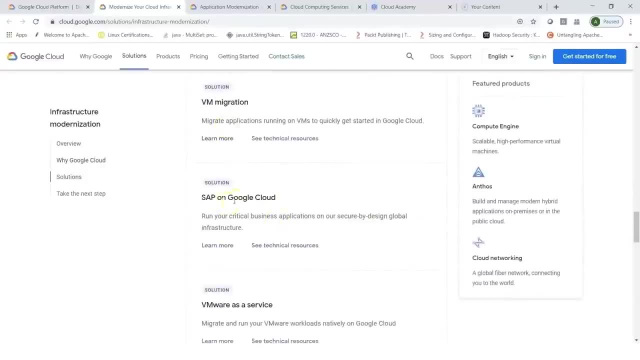 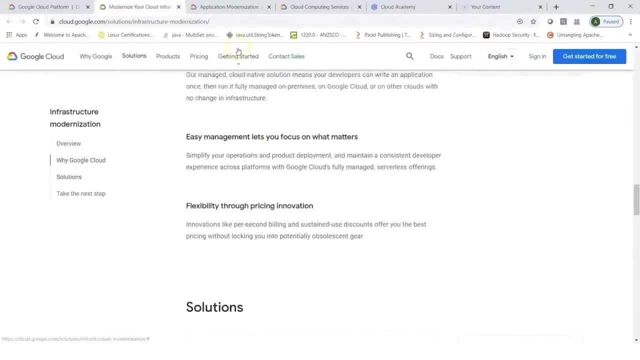 your different cloud solutions, such as VM migration. you have SAP on Google Cloud, VMWare as a service, and so on, And you could learn from these different solutions which are offered. You can also look at application modernization, So not only infrastructure modernization. 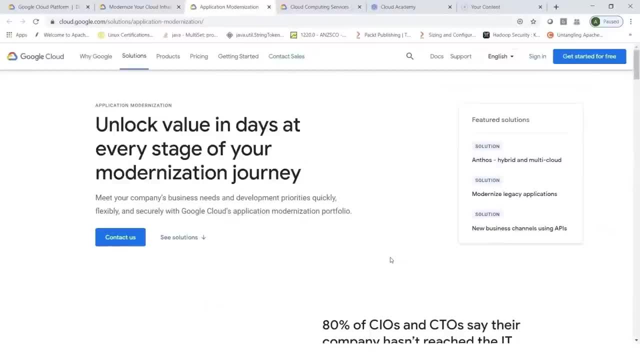 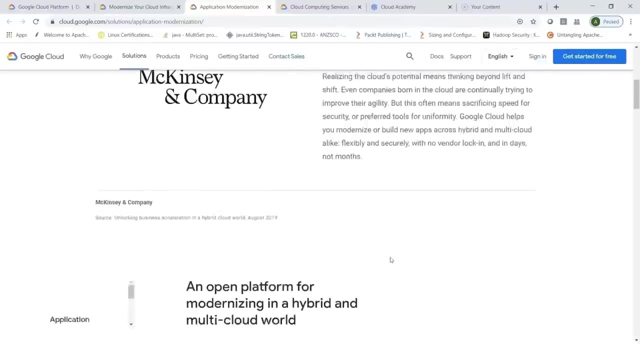 but organizations would also be interested in re-looking at their applications, re-looking at how these applications could be moved from monolithic to microservices architecture or how applications can benefit from modernization and cloud computing offerings. So you have again different use cases, what they are doing, what they are doing what they are doing what they are. 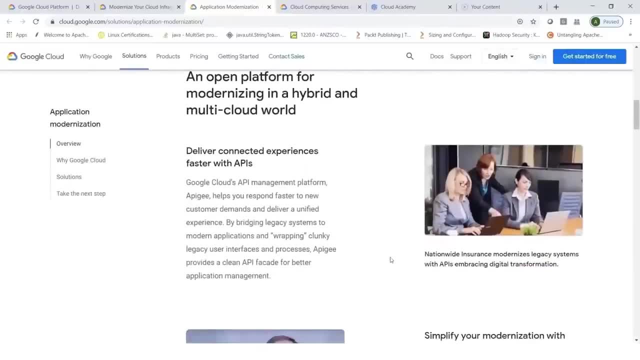 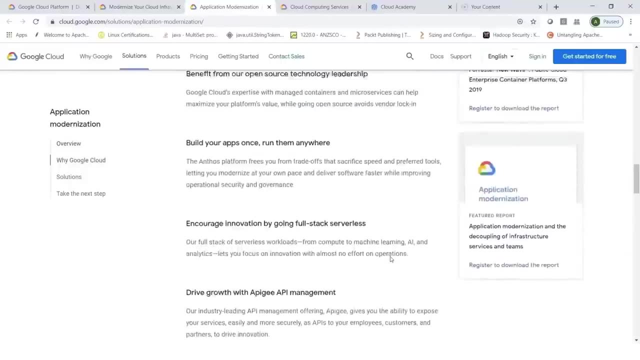 offering. So there are some different uses cases here, which talks about different ways in which Google Cloud can help, how you can modernize your applications, how you can use different solutions which Google Cloud is offering. Now, when we talk about cloud computing services, you 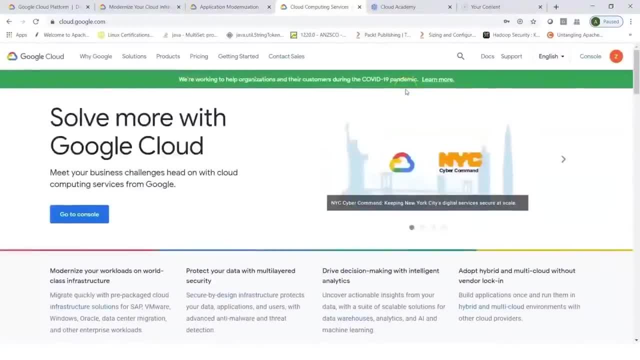 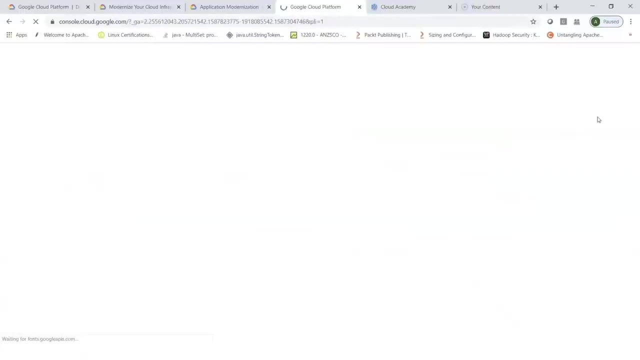 can always go into cloudgooglecom. If you have created a free account, then you can just log in and every user by default gets a $300 free credit. they can try out different products where they can use different services. so here, if I click on console where I am already logged in with my gmail account, 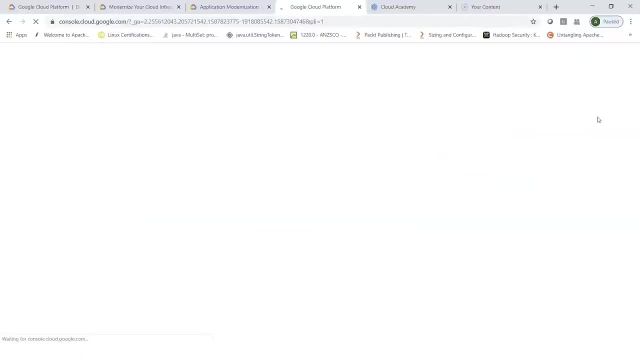 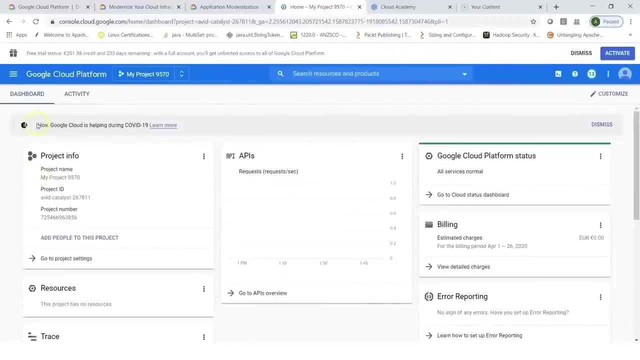 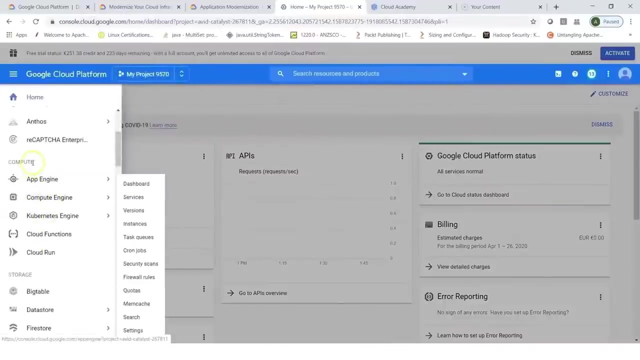 or my Google Cloud account, wherein I have $300 free credit, out of which some is being used. you have a Google Cloud console and here, from the hamburger menu, you can click and you can look at different services within different domains. so you have compute domain, which has different services, such as app. 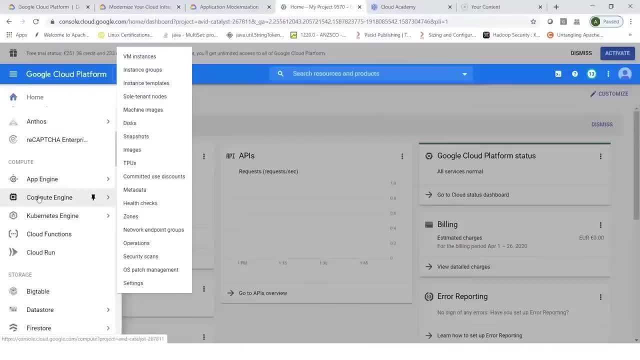 you have compute engine and that basically allows you to use your VM instances, which we were talking about previous slides: different instance groups. create your templates, use sole tenant nodes. create snapshots or backup of your data. use different zones. you can go for kubernetes, which is containerized. 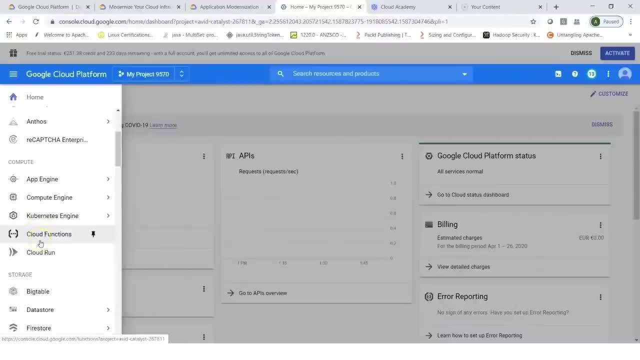 based engine, you have cloud functions, you have cloud run, and then you have storage related different options, such as big table, you have data store, fire store, file store, storage and so on, and for each of these services you can read about from the Google's documentation, or anyways, I will. 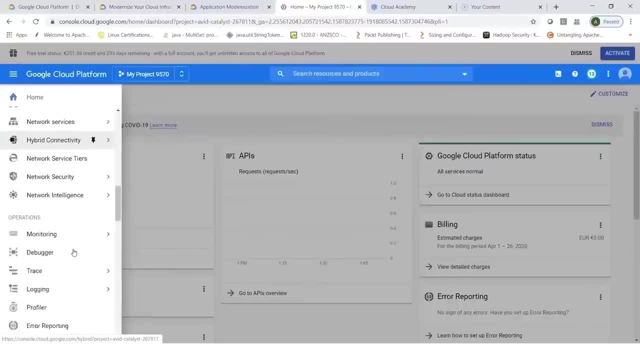 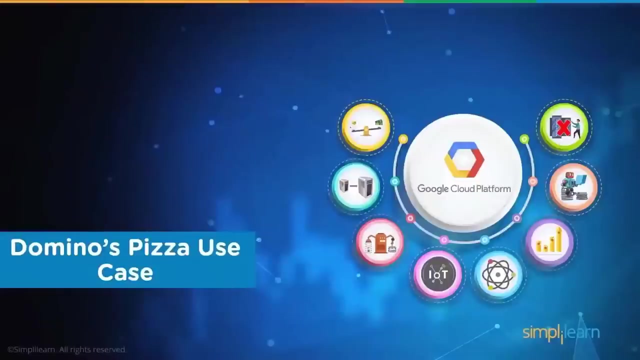 be explaining that later. you can also look at networking related, operation related and other tools which are offered by Google Cloud. so these are huge list of services which Google Cloud platform offers in different ways for different use cases. now let's look at this Domino's pizza use case and see what it 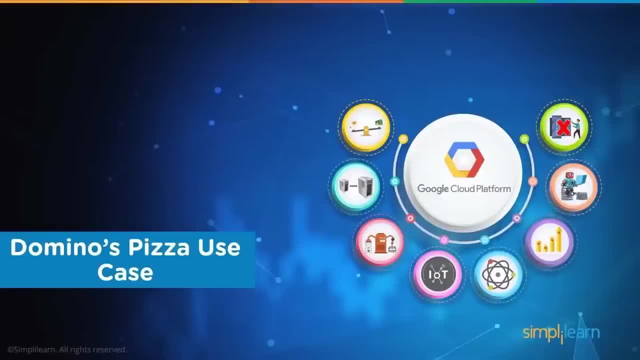 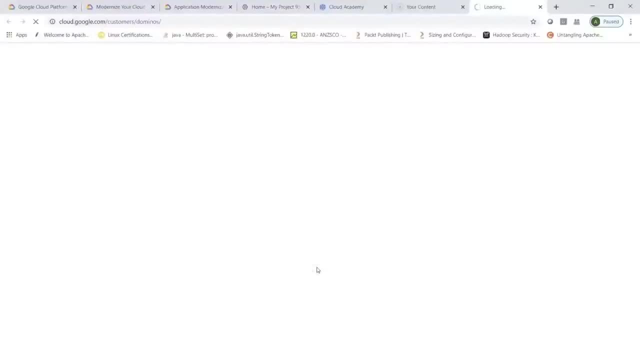 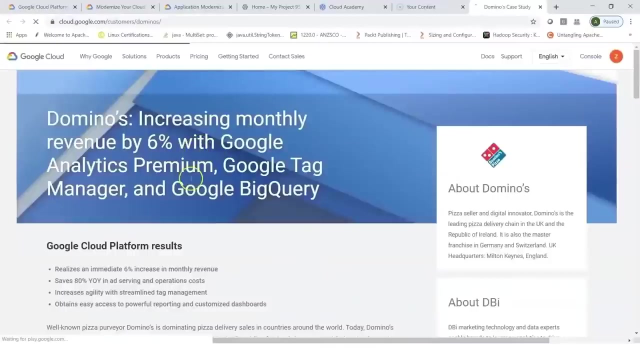 helps us learn about. so you can always access this page by going to this link which talks about customers and then which shows you different use cases. so Domino's increasing monthly revenue by six percent with Google Analytics premium, Google tag manager and Google bigquery. so this is. 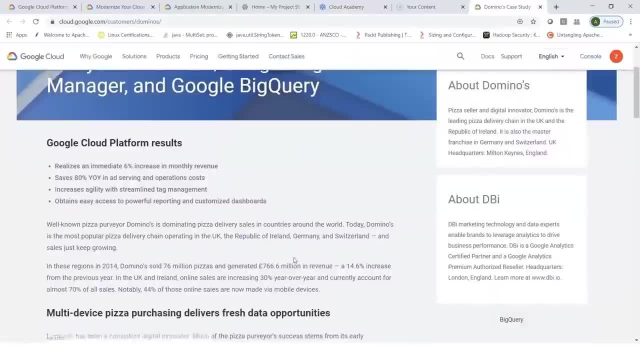 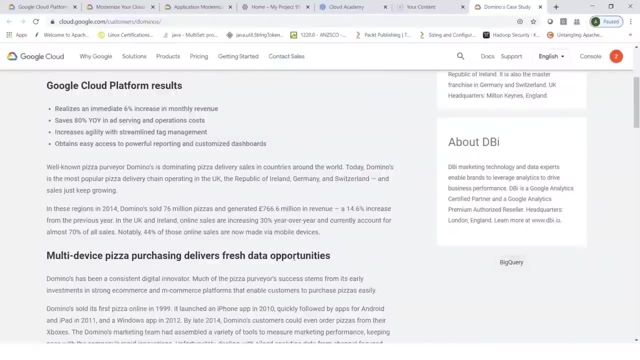 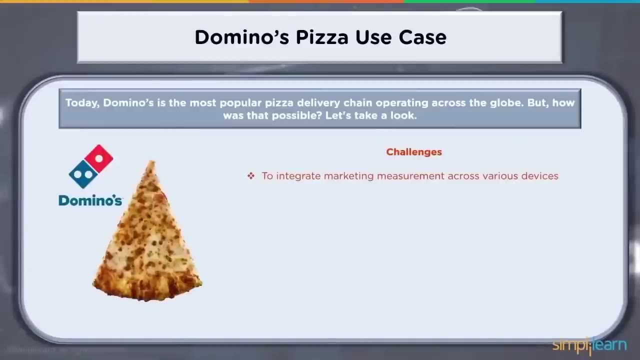 basically when Domino's started using GCP, and what was the result of that? now let's look further into this. so we all know that Domino is most popular pizza delivery chain operating across the globe, but how was that possible? let's take a look. so the challenges were: they wanted to integrate marketing measurement. 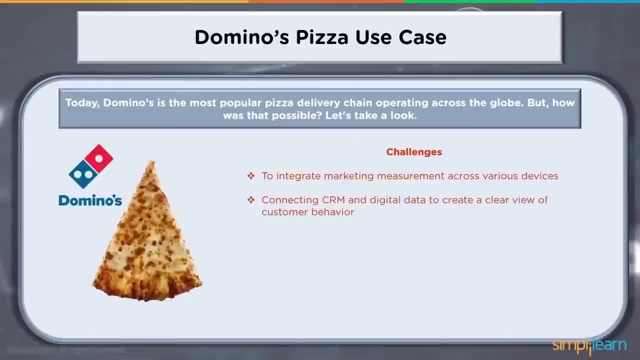 across various devices, connecting software to device across the globe and therefore making it sort of an wished-by scenario for a business. CRM and digital data to create a clear view of customer behavior. to make cross-channel marketing performance analysis easy and efficient. Now for these challenges which Domino's was facing, the solution was using Google. 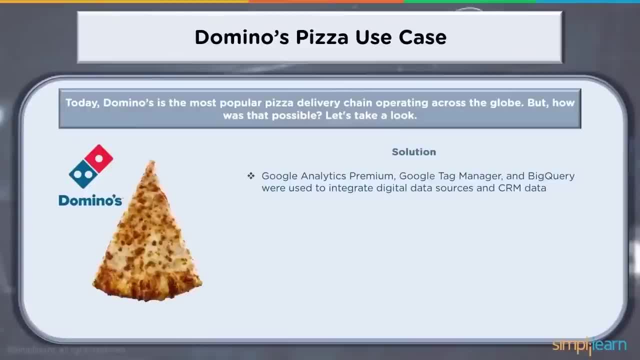 Analytics Premium, Google Tag Manager and BigQuery, which were used to integrate digital data sources and CRM data. The reporting was made easier and more efficient by implementing Google Analytics Premium because it had the ability to access a single Google Analytics account to evaluate web and app. 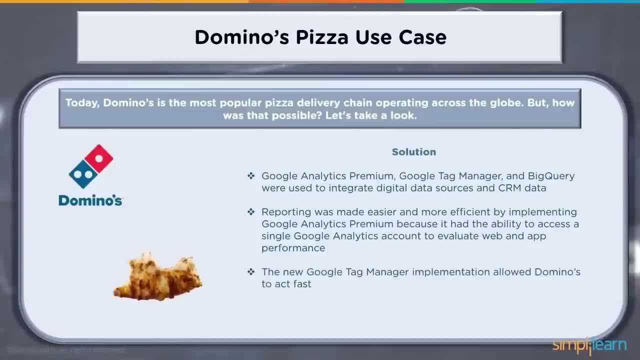 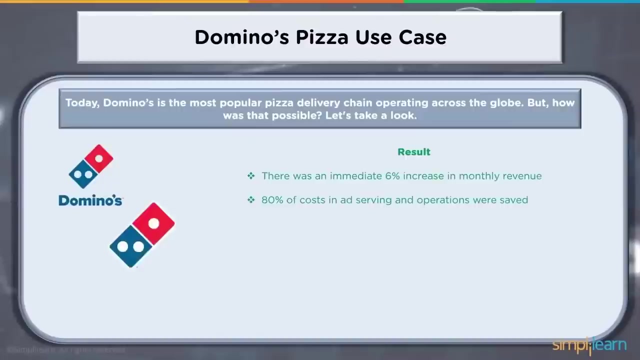 performance. By using the new Google Tag Manager implementation, Domino's were able to act fast. They were able to connect CRM data with digital analytics, which basically provided Domino with greater visibility on. What was the result? There was an immediate 6% increase in monthly revenue, 80% of costs in ad serving and operations. 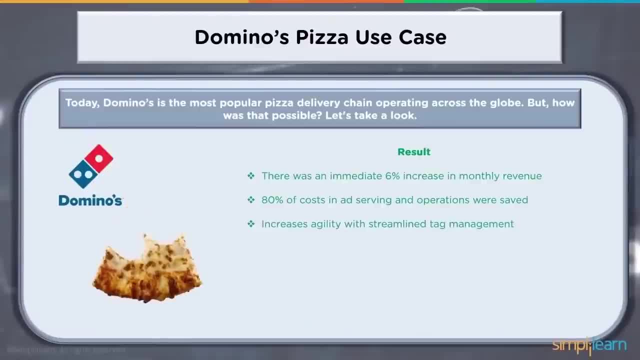 were saved increases agility with streamlined tag management. They obtained easy access to powerful reporting and customized dashboards. Now that was just one simple use case. Before we go on to hands-on, we can also talk a little bit back about the services. 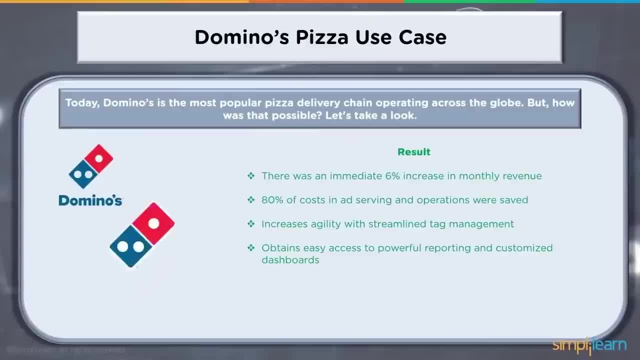 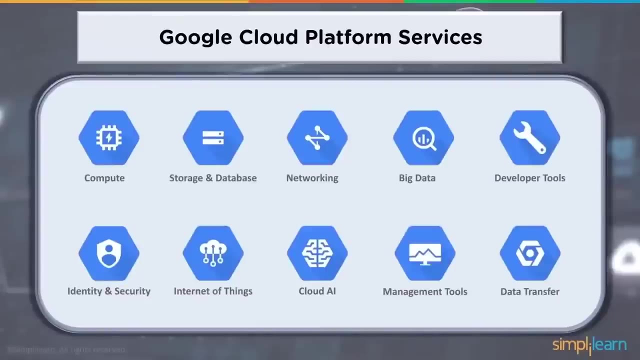 that Domino's was using. There are a few services which Google Cloud offers, as we discussed, and some of these services which can really make you think: why not Google Cloud Platform? So, when we talk about your different cloud platform services, let's learn about some. 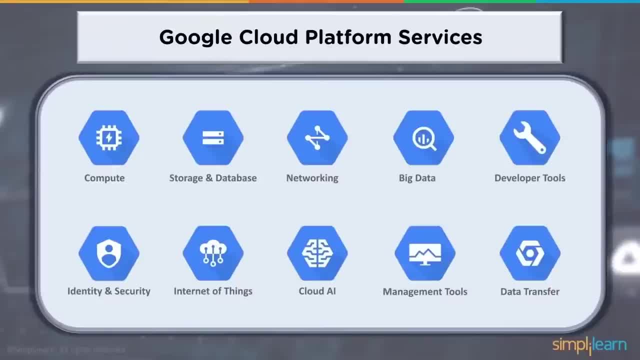 of these services in brief, in what each service is, what it does and how it can help us in handling our use cases or working with different products. So let's learn briefly about different services which Google Cloud Platform offers. Now. one of the domains is compute, and then let's look at the compute services which GCP 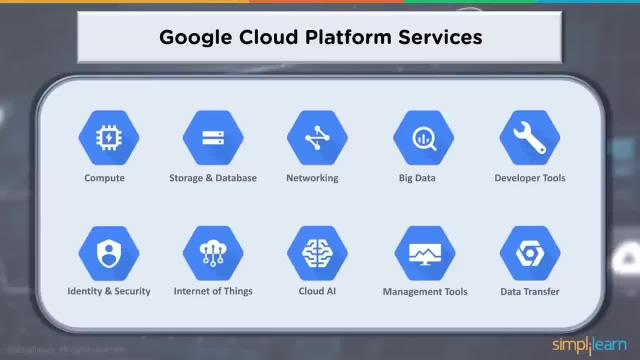 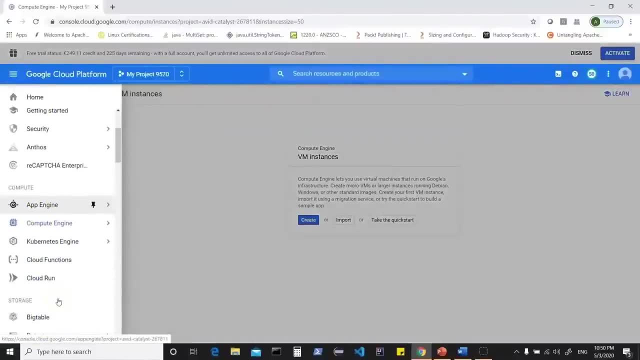 offers. Now here I can log into the console and this hamburger menu on the top left corner. I can click on this one and go into the compute engine section. So this is the compute domain, which has App Engine, Kubernetes, Engine, Cloud Functions. 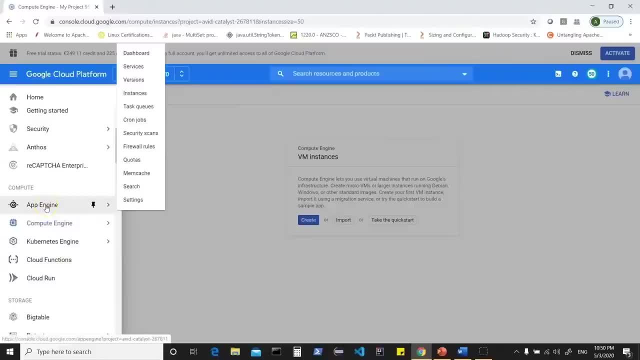 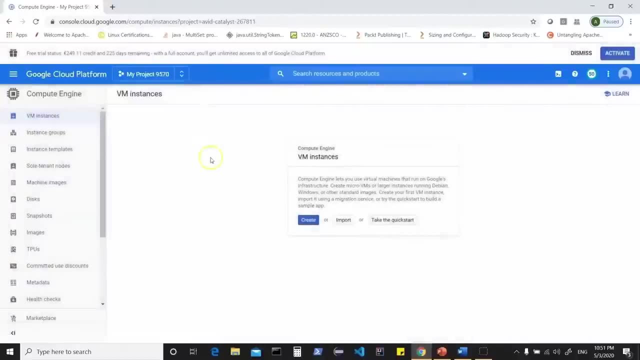 and Cloud Run. So these are your different services which are offered within the compute domain, and here we can get into compute engine by clicking on this one and then basically going to VM instances. So before we see how we can use this compute engine, let's understand about some of the 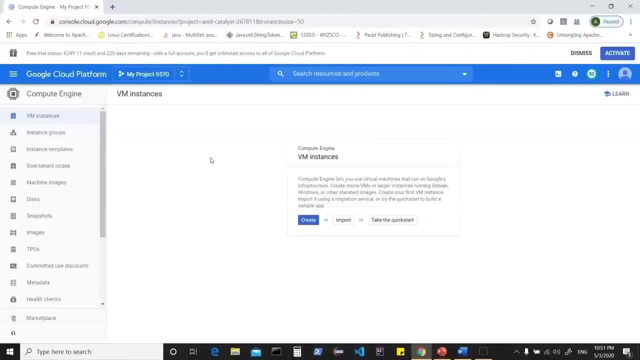 features of compute engine which basically offers scalable, high-performance virtual machines which are configurable, and which runs in Google's data center with access to high-performance networking. So from here you can select VM for your needs, for your general purpose or workload. 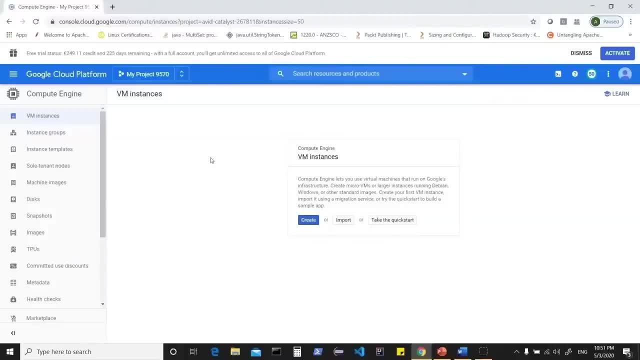 optimized, predefined or custom machines. Now, here you can integrate compute with other Google Cloud services, such as AI, ML and other data analytics services. You have different machines which are offered here, such as general purpose, which provide a balance between price and performance, which are well-suited for mobile. 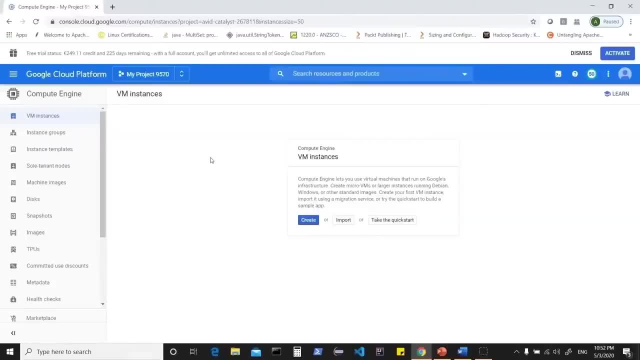 So now we can see the different applications which you can use to configure compute engine and compute machine. You also have compute optimized machines which offer consistent high-end virtual CPU core performance and which are mainly good for gaming, EDA, high-process computing and other. 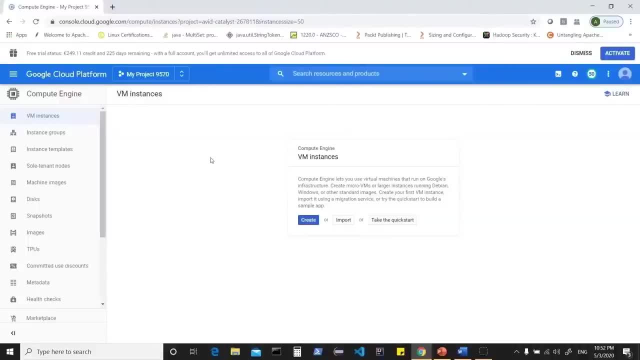 such applications. Apart from general purpose compute optimized, you also have memory optimized machines which offer highest amount of memory, and these VMs are basically well suited for in-memory databases such as SAP HANA, real-time analytics and in-memory cache. Now we can see these options here. You can click on. 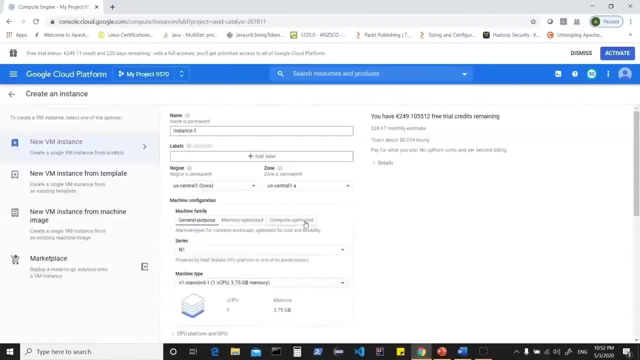 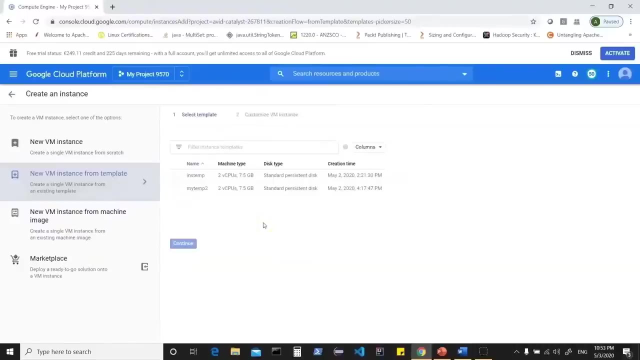 VM instances while you are logged in into your Google Cloud console. Here you can even create an instance template which can be used to spin up instances, For example, if I click on new VM instance from a template. there are some templates which I have already created for my usage. 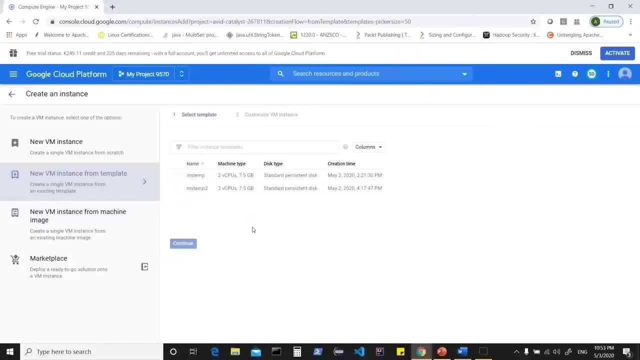 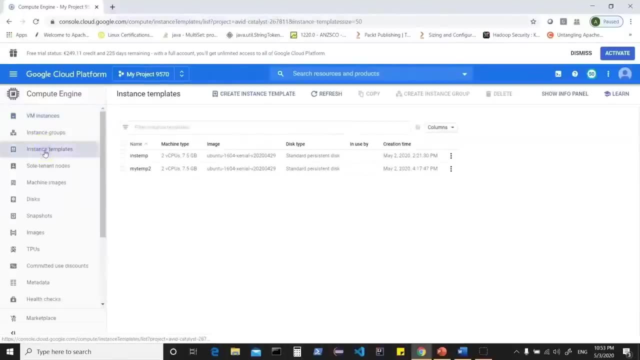 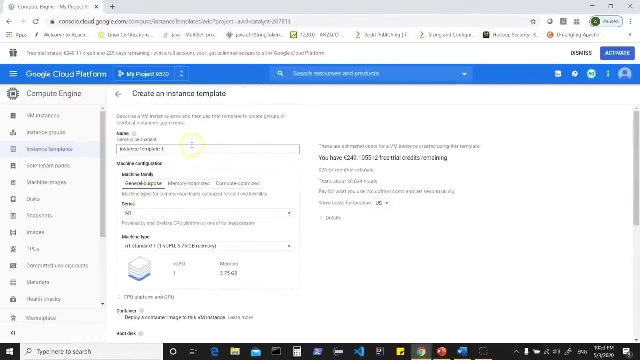 Now here I can basically use one of these templates, or what I can do is I can go back, I can go into instance templates and this basically allows me to create a template. So you can click on create instance template, which basically allows you to create templates which can. 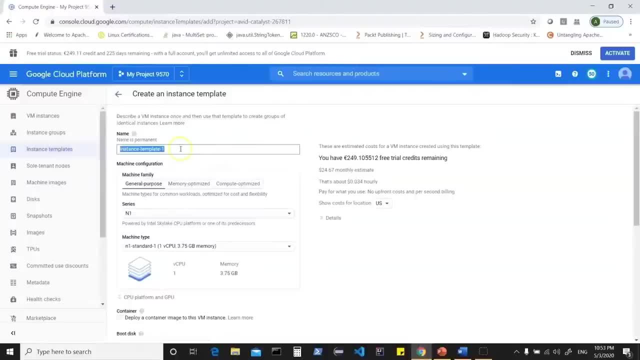 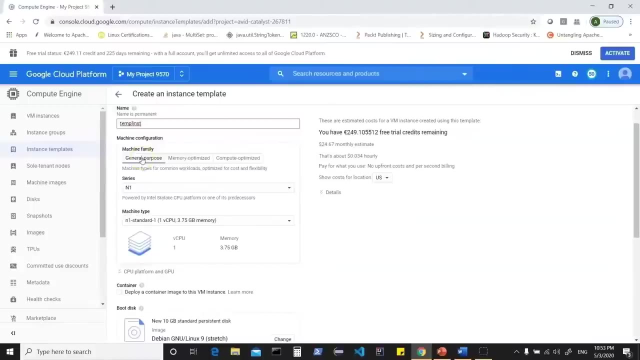 be used to spin up different instances. We can give a name to the template. For example, we can say templatehtml- Instance. Now here I can choose machine configurations and this is where you have different options. So you have general purpose, as I mentioned, which provide a balance between 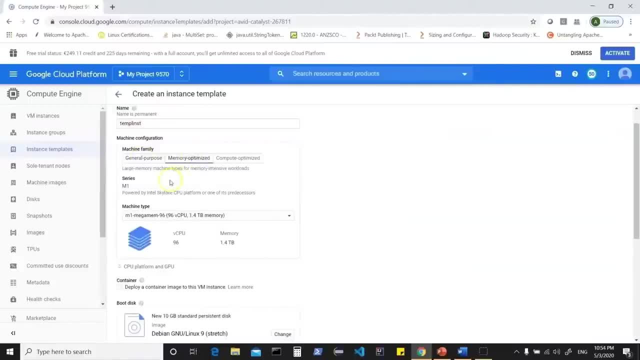 price and performance. You have memory optimized, which are large memory machine types for memory intensive workloads. You also have compute optimized, which basically give you high performance machine types for compute intensive workloads. So you can choose any machine configuration which is available here based on your requirements. Now, if you click on general purpose, 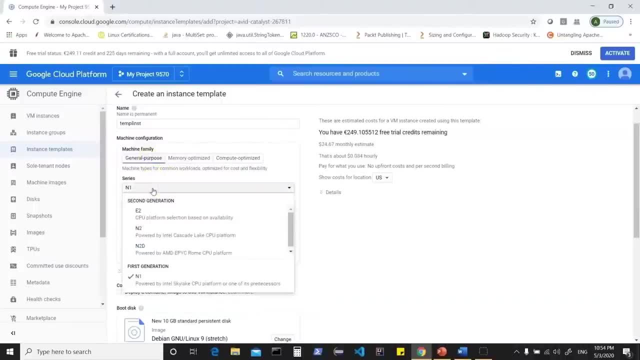 that has different options here. So you look into the series. where you have N1 series, you have e2, which is CPU platform selection based on availability. You have N2 and N2d, So let's just have N1 selected. Now you also have here which talks about machine types. 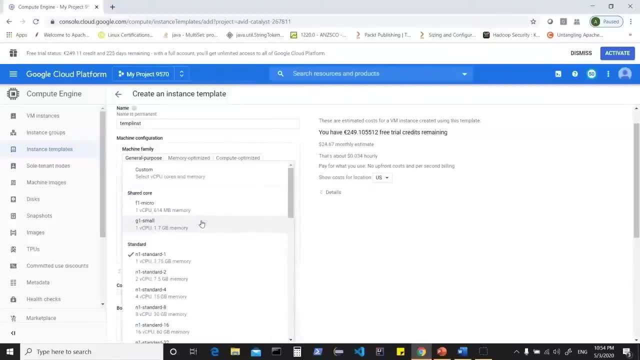 and here we can choose the configuration which we are interested in, Depending on the applications which will run within the machines. we can choose a machine, so by default it shows one virtual cpu core and 3.5 gigabyte of memory or ram. you could choose a higher end. 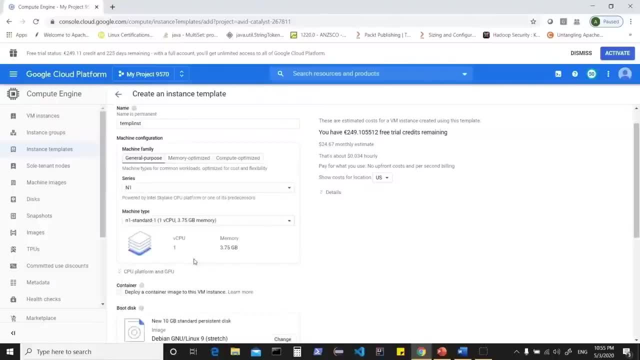 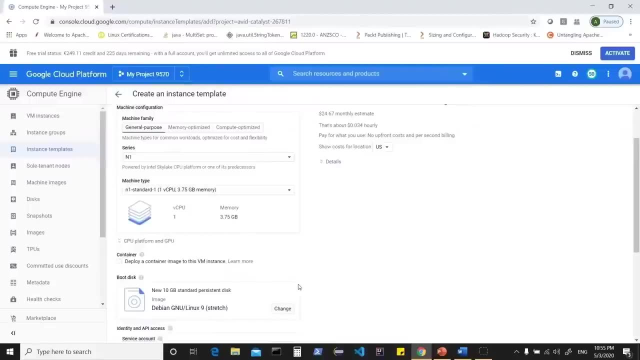 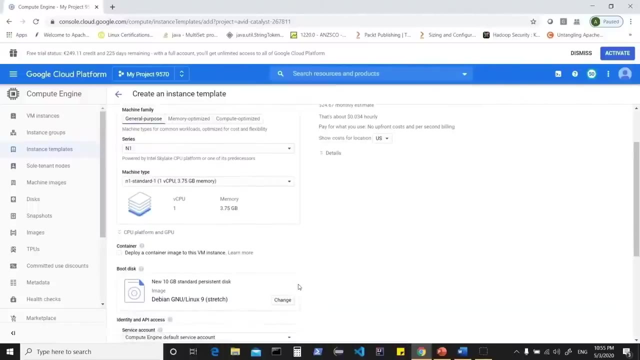 machine. so as of now i'll just say n1 standard. now that basically allows me to choose these machines. so there are different features which your compute offers, such as: you have live migration for vms, you have preemptible virtual machines, you have sole tenant nodes, and all those options can. 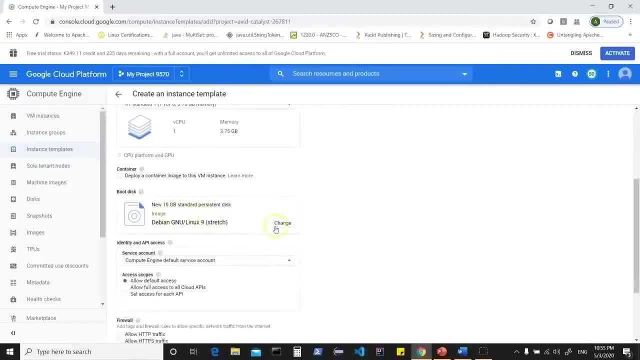 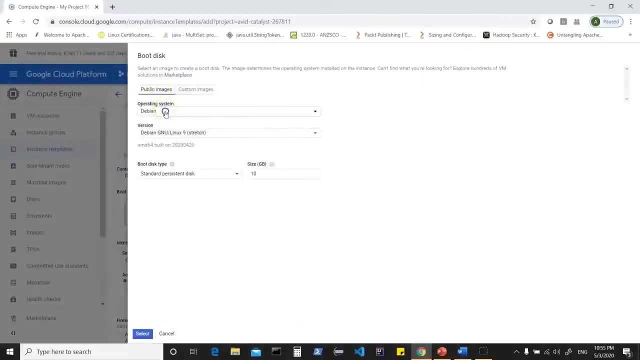 be seen here now. in this machine for my boot disk, i can select a distribution which i would be interested in. for example, i could be going for public images and i can choose, for example, ubuntu, and then i can choose a version. so it shows me 16.04 and you also have latest versions, such as. 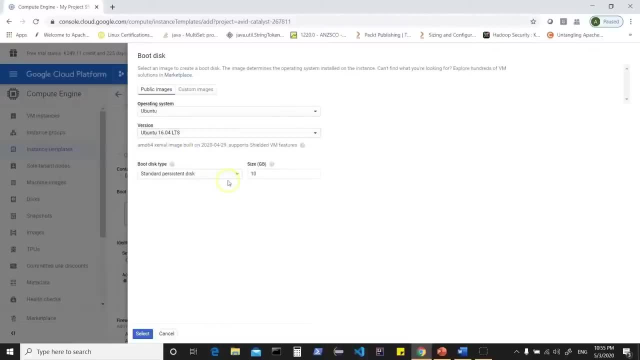 ubuntu 20 you can choose one of these and here it asks you to choose the boot disk type, so that could be standard persistent disk, which is HDDs, which are low in performance and you can say low in cost in comparison to SSDs. So SSDs give. 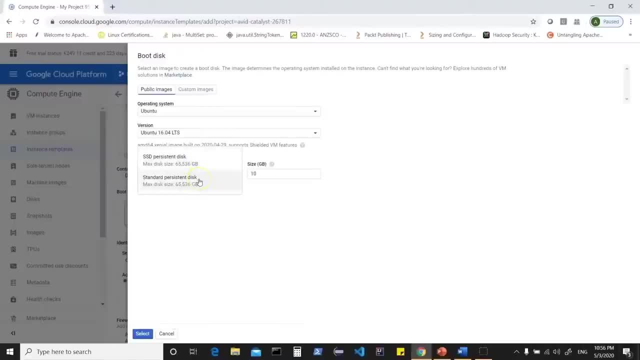 you better performance, but then they are little expensive than using standard persistent disk. We can choose this and we can give a disk size, for example 20 gigabyte, and I can click on select. Before clicking on select, I can click on custom images and that shows me if you have any other. 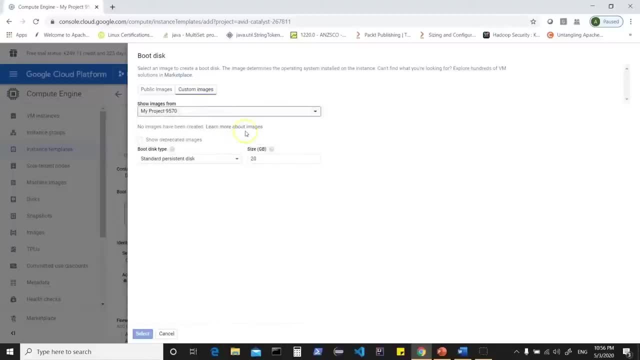 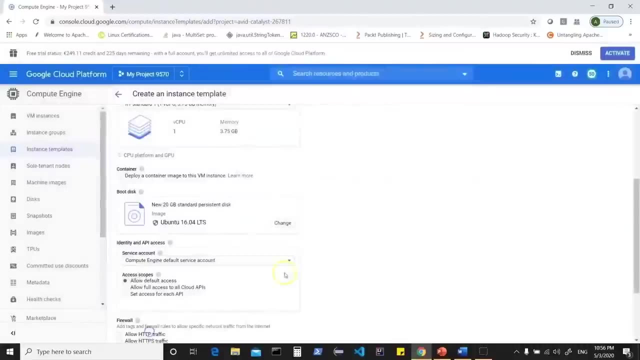 images created in your project. you could use those. You could also learn about images by clicking on this link, So we'll click on public images. We have chosen this distribution. Let's do a select. and now here you have identity and API access management, So let this be default. 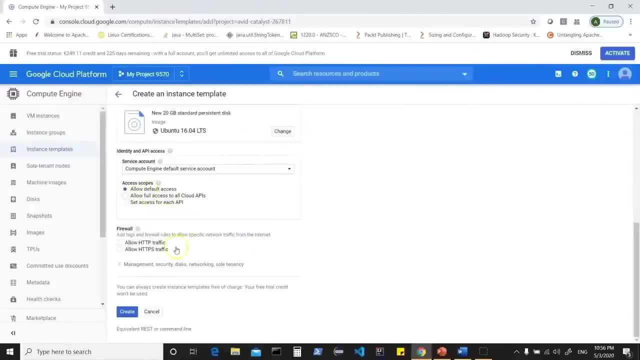 You can say: allow default access and what you need is, depending on the services we can choose, it allows HTTP and HTTPS traffic. Now we would also need some way to connect to these machines, So when you set up an instance by default, you can do SSH into it. 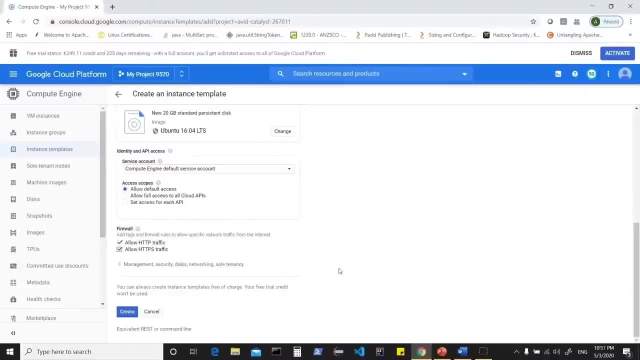 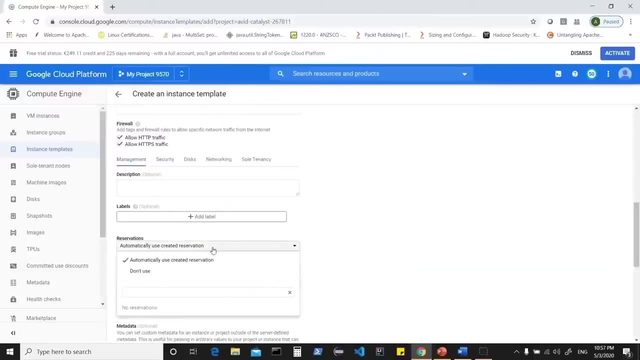 using the Google Cloud console or from Cloud Shell. You can also give a private and a public key. So here you have the option where you can give all these details. So, when it comes to management, it tells you: would you want to go for reservations and you can say: automatically use. 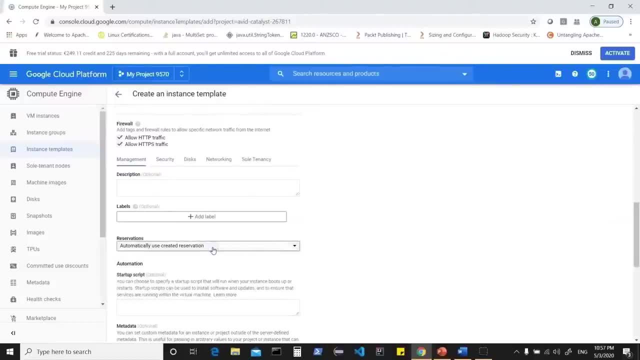 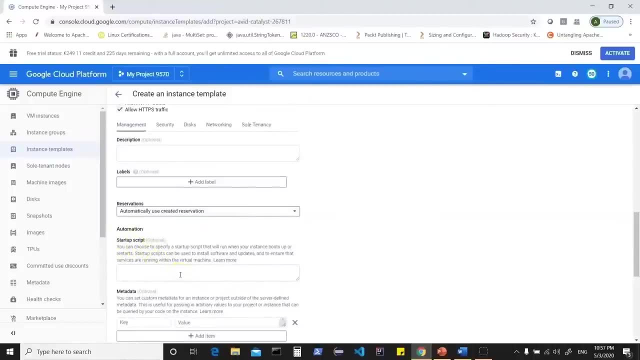 created reservation. You could also say no, you would not want to use a reservation. You can also say no, you would not want to use a reservation. You can also say no, you would not want to use a set up or provide a startup script which you would want to give whenever your machines come up. 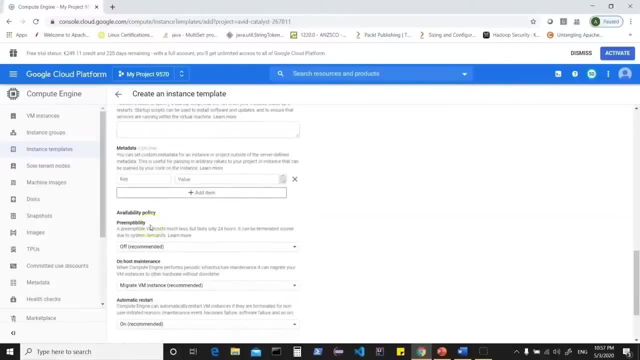 And here you have the options of preemptibility. So compute offers preemptible virtual machines. So that is mainly when you would want to run bad jobs and fault tolerant workloads on these machines and you can benefit with a reduced cost for your virtual CPU and memory. 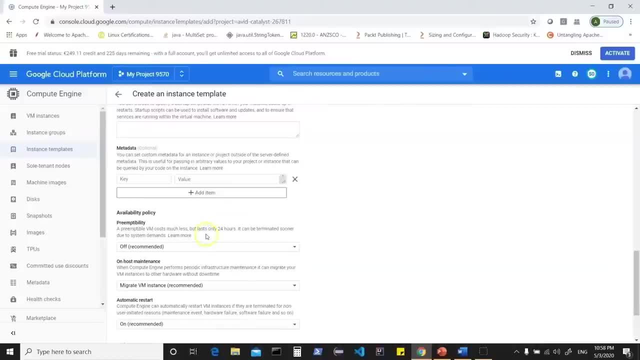 by 80 percent. So these are virtual machines which would be lasting less. Now, by default, this is off and it purely depends on your workload what you would want to run on these instances. I could just go ahead and select preemptible- being on that, and use this feature of. 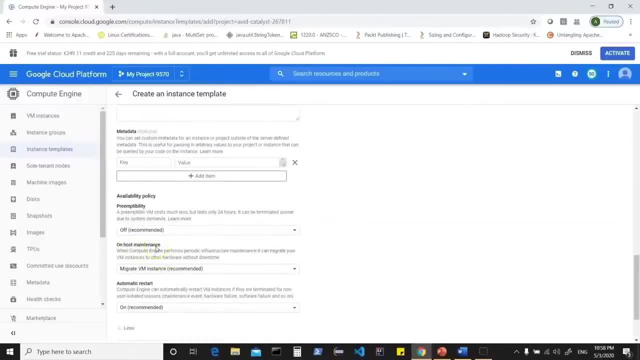 compute You also have on host maintenance which talks about what would be happening with this compute engine instance. So when compute engine performs periodic infrastructure maintenance it can migrate your VM instances to other hardware And this is one of the features which you can do. So let's say you have a VM instance which compute engine offers, which we call as live. 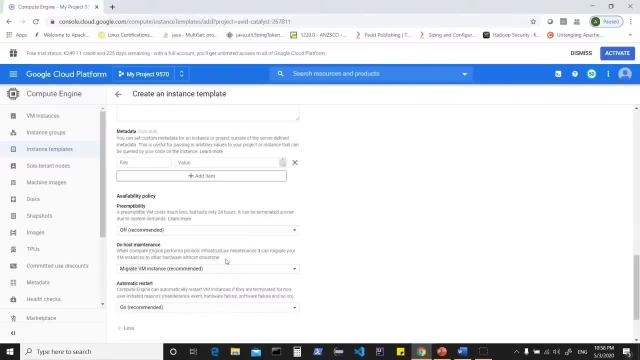 migration for VMs. Here your compute engine can live migrate between host systems- that is, the underlying systems on which these VM instances are based on, without rebooting, which will keep your application running even when host system require maintenance. And here it says: migrate VM instance recommended and let that be as it is. You can also say that if there is a maintenance. 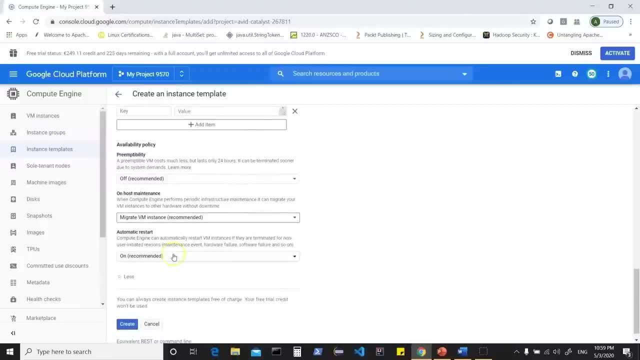 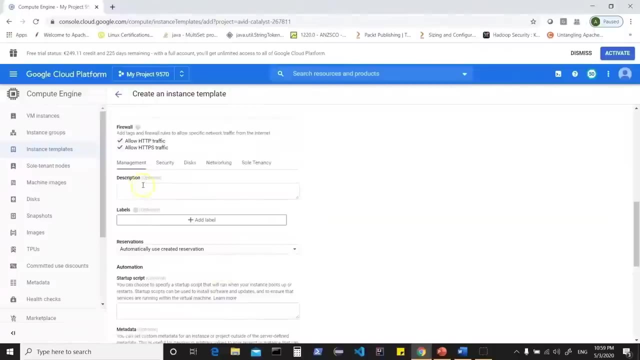 happening, you can terminate the VM instance. Now it also talks about automatic restart, which is on, which basically means compute engine can automatically restart VM instances if they are terminated from non-user initiated reasons. So these are all the settings which are available in management, and it also tells us the different 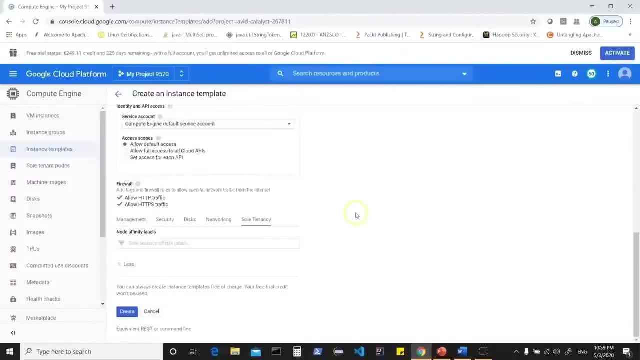 features which we have. There is also a feature called sole tenancy, which basically means sole tenant nodes which can be chosen So you can have physical compute engine servers dedicated exclusively for your use, And this is usually good when you're talking about bring your own. 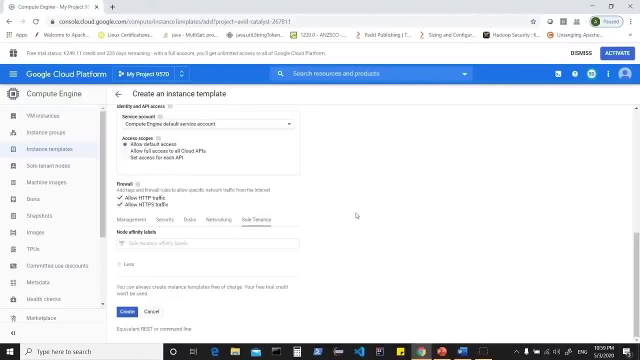 license applications. So sole tenant nodes give you access to same machine types and VM configuration options as regular compute instances. However, these might be a little expensive. We can choose this one. We can also look into networking, which basically shows the default setup which goes for. 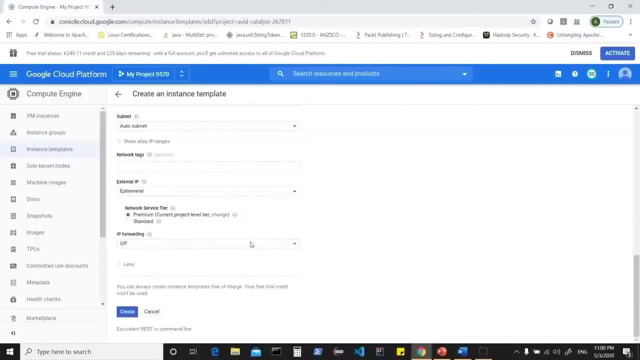 auto subnet. You can also choose a particular IP if that is required, But that would cost more. You can click on disks which talk about: what do you want to do with the boot disk when the instance is deleted? What is the encryption mechanism you would want to use? 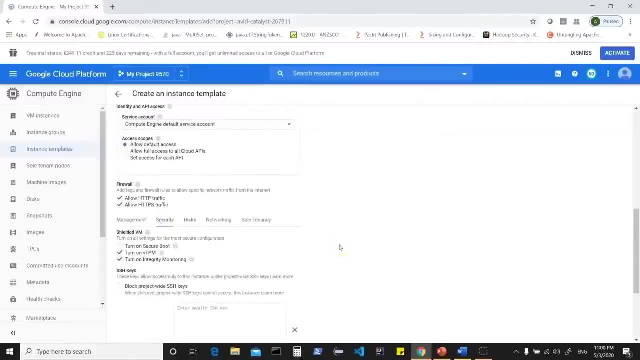 And here, finally, you have security. So basically, as I said, you can SSH into instance using the cloud console option and you can also provide a public SSH key, So one way of doing that if you intend to use an external SSH client, such as Putty, to connect. 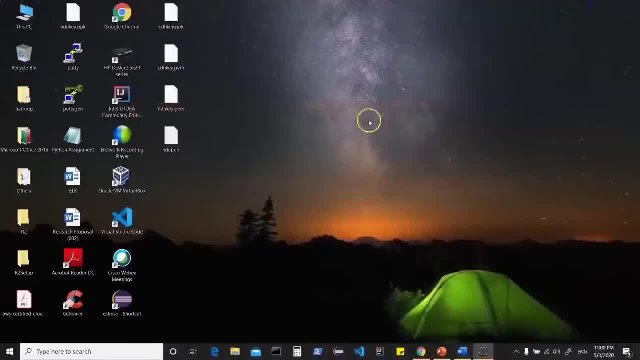 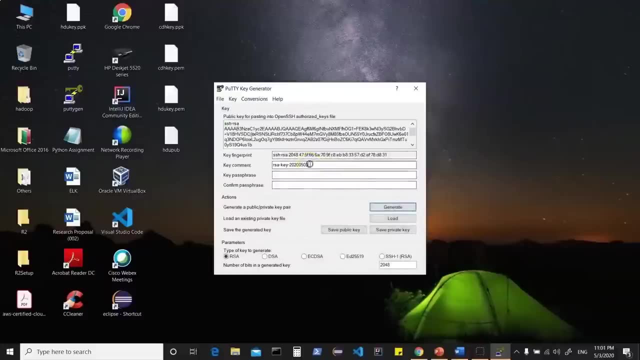 can create a key. so, for example, I can go into puttygen and here I can say generate, just move my cursor over here and that will create a key. I can give a name to this one, so I will say HDU will be username. I will give a simple. 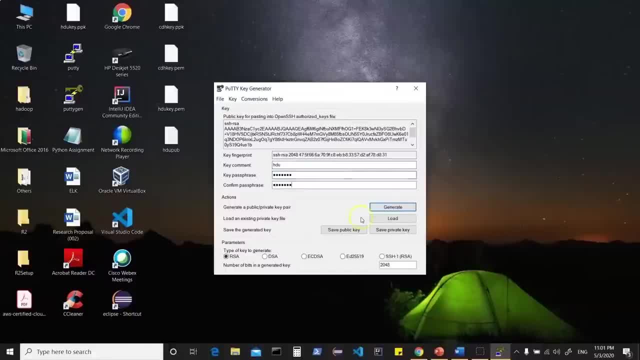 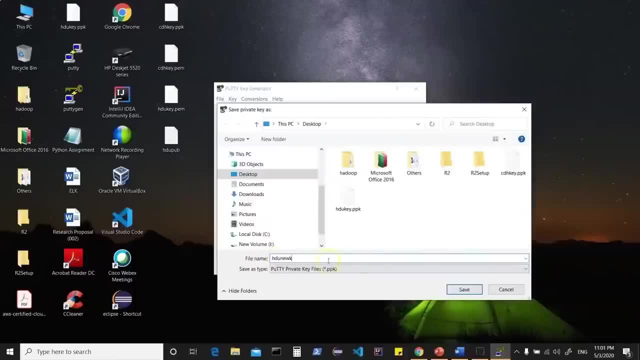 password which I will use to login to this machine, and then I can save this private key which will get saved. so let's say HDU new key, and this gets saved in a dot PPK file which is usually used when you use an external SSH client to connect. so save this one and that saves a PPK file on your desktop. 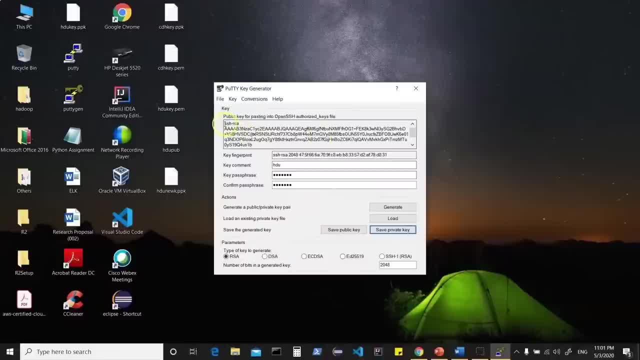 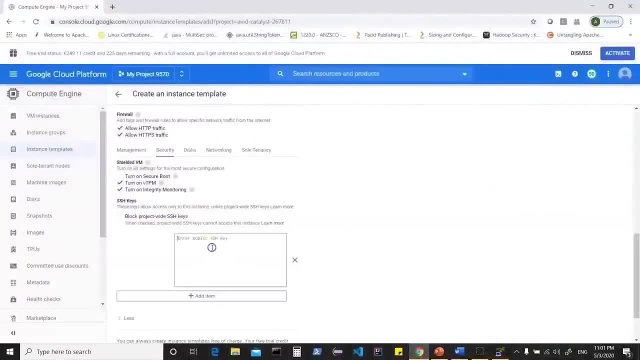 what you can also do is you can copy this public key content from here- and this is what we would want to give in our instance here- so so that the public key gets stored on the instance and private key is what we will use to connect. so, once again, this is what we will use to connect. so, once again, this is. 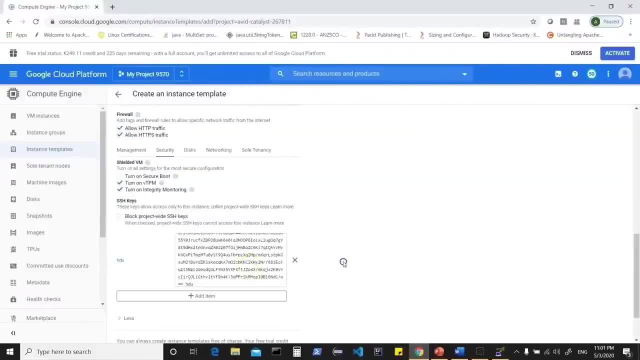 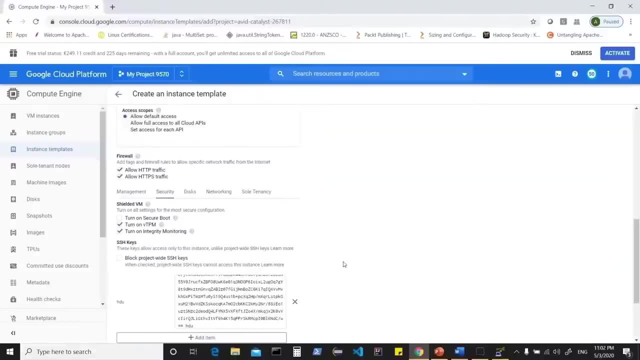 what we will use to connect. so, once again, this is what we will use to connect. so once I paste it here, it resolves the name to HDU and we have given the public key. now, in certain cases, you may want to use a software which uses SSH to connect to the machine and that software might not. 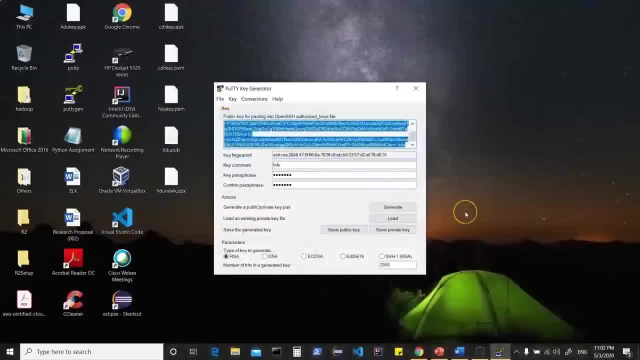 be such as your putty. so in that case you may want a PEM file or a private key which is saved as a dot PEM file. so you can also do that by going to conversions and do export, open SSH key and then save it. so I'll say: HDU new. 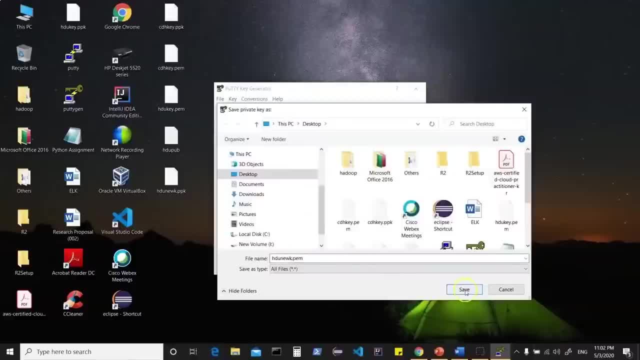 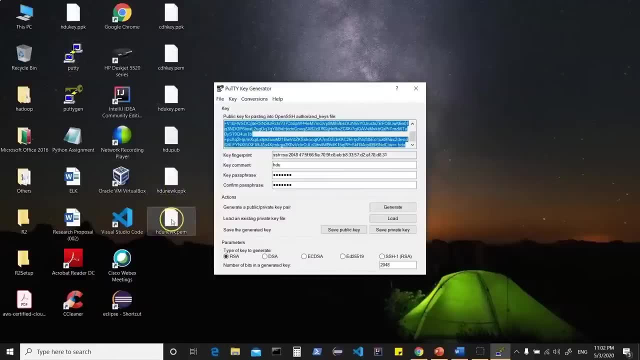 key, but then this one will be saved as a PEM file on my machine. so you have PPK file which allows you to use putty to connect to the instance. you have a PEM, in case a software needs directly SSH to these machines. you also have the 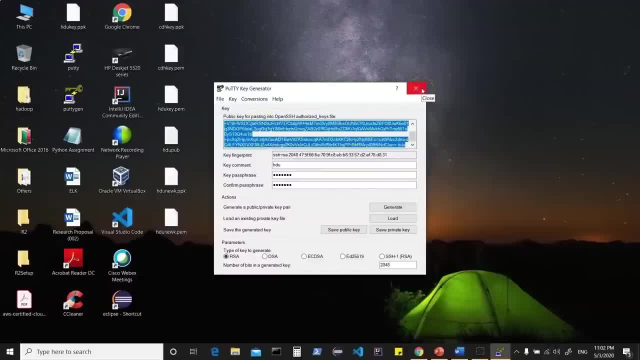 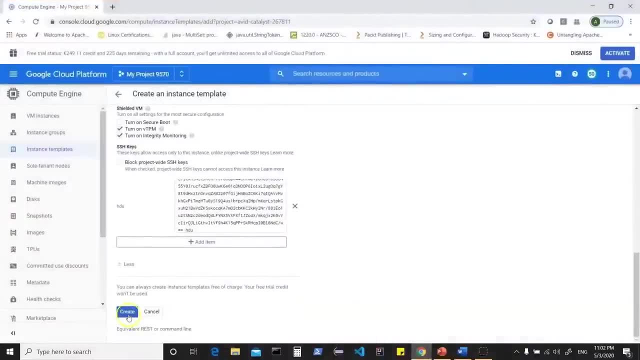 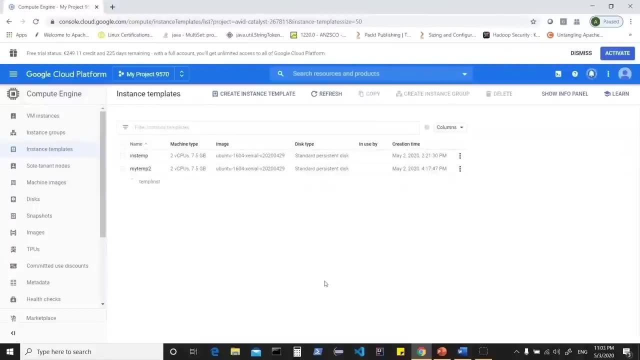 public key which we have already provided in the machine. now, once this is done, I can close puttygen. I can go back to this page where I'm creating an instance template, and then I can just click on create. so this has created a instance template which I can use to spin up my instances. any number of 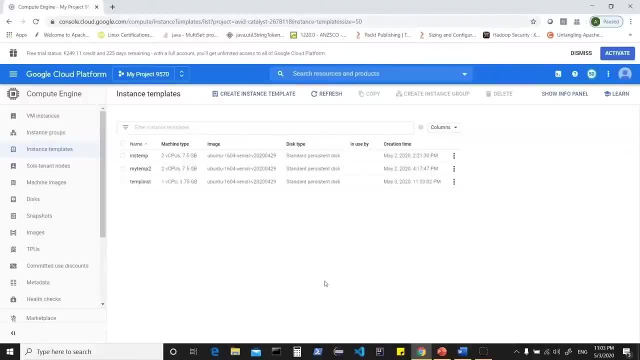 instances using the same template. only thing which I would have to do is change the region where I would want the instance to run. so now that we have created instance- and that's my this one. the third option- I can go back to VM instances. now I can click on create, and here I can either create an instance, 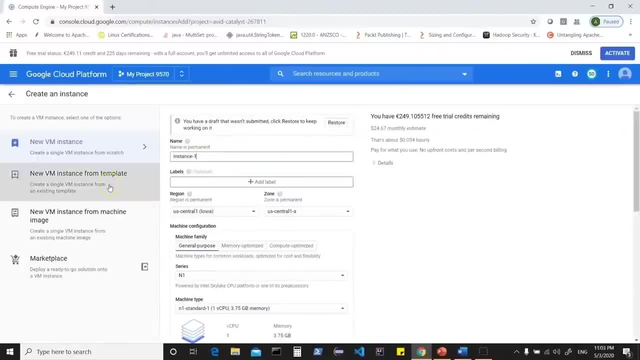 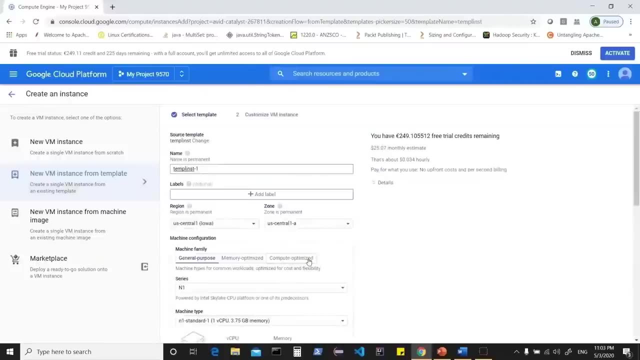 from scratch by giving all the details again, or I can just use my template so I can click on new VM instance from a template. choose my template, click on continue and once this is done, I can give my instance name, so let's say c1. I can choose the region, so I will choose Frankfurt and then rest. everything is. 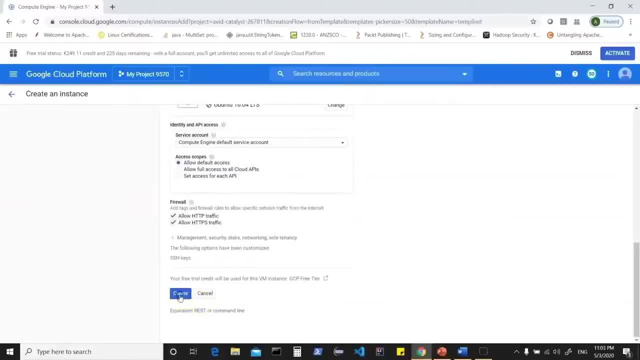 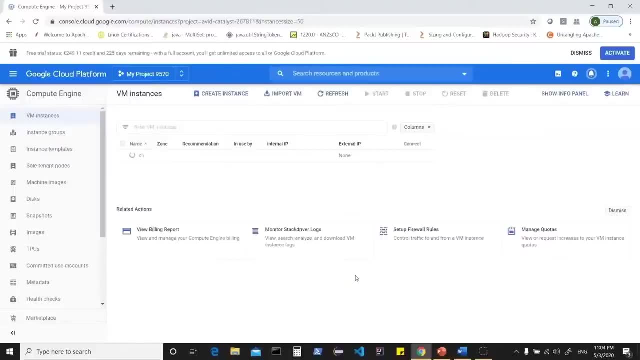 auto populated based on the template, what you have given, and you click on create now. this basically allows you to spin up an instance and you can create any number of instances using your template. you could have already created instance right from scratch. now, once the instance is created, this has a public. 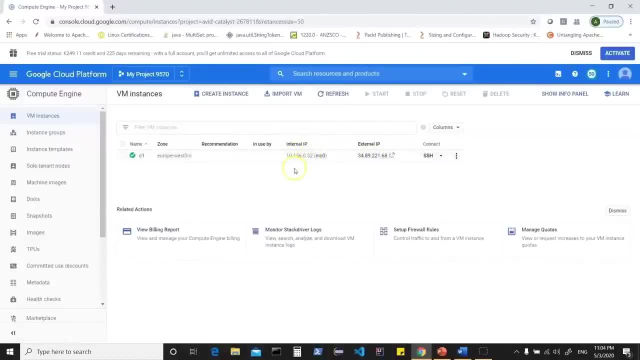 IP and a private IP. private IP will not change, unless you would want to set up a new machine, but public IP will change every time you stop and start the machine. now this is what we need to connect to this machine. I can also do a SSH from here by doing this and open in a browser window. let's click on this so. 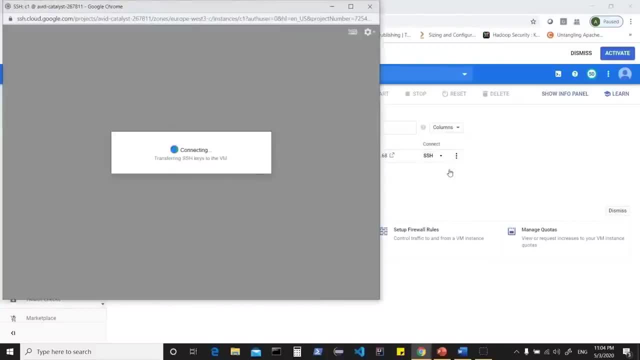 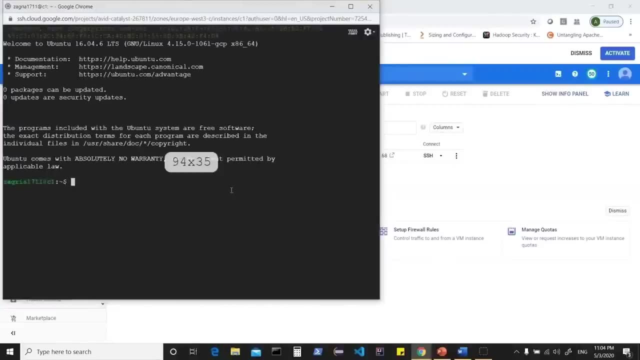 this is an internal way of connecting to your instance using SSH. let's wait, because it would be transferring the SSH keys to the VM. it establishes a connection and I am connected to my machine. what we can easily do is to confirm if we are in the right machine. we can just do a LS to. 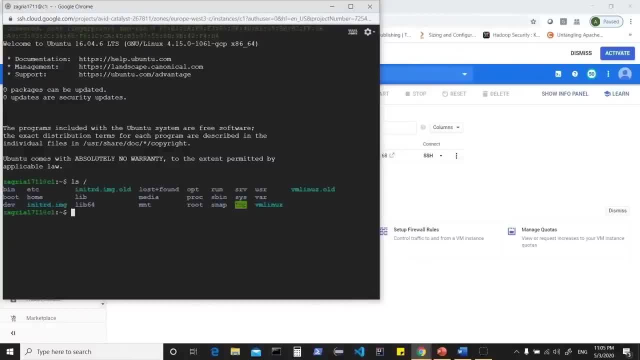 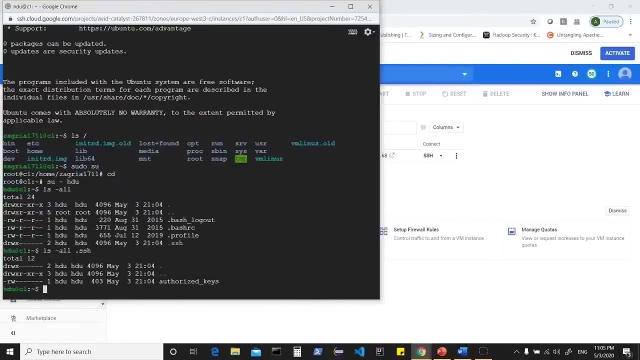 look at the file system. what we can also do is we can basically log in as root by doing a sudo su and that allows you to get into the machine as root and from here I can switch to HD you user, which will have a dot SSH directory in home and that basically has authorized keys. and if we would want 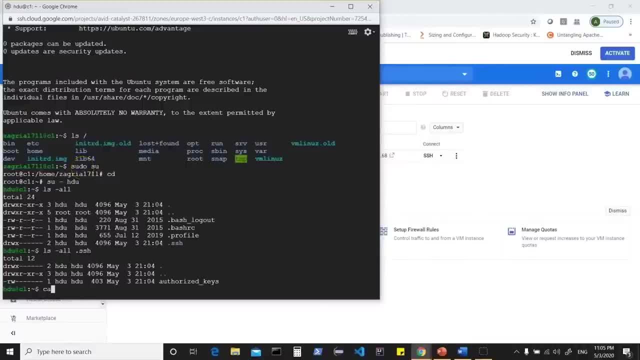 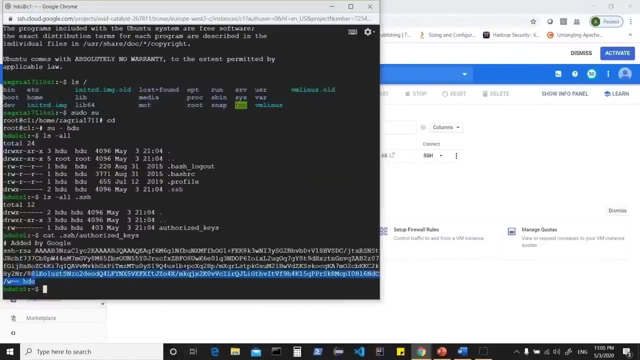 to see if this one contains my public key. I can just do a cat dot SSH and then look into authorized keys and this shows me the public key which we had initially added to our instance. so this confirms that we are logged into the machine which we created. now I can close this, and what I can also do is I can copy. 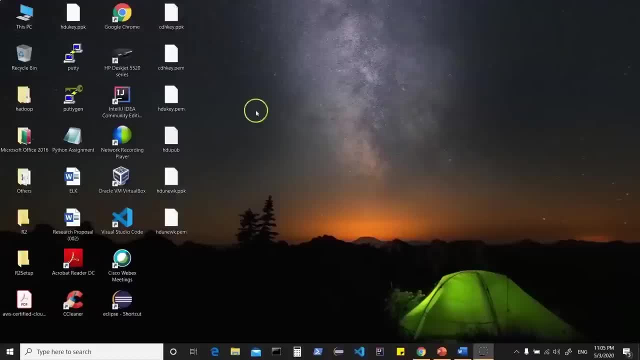 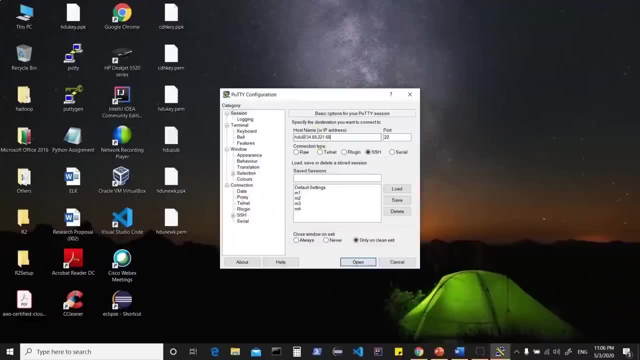 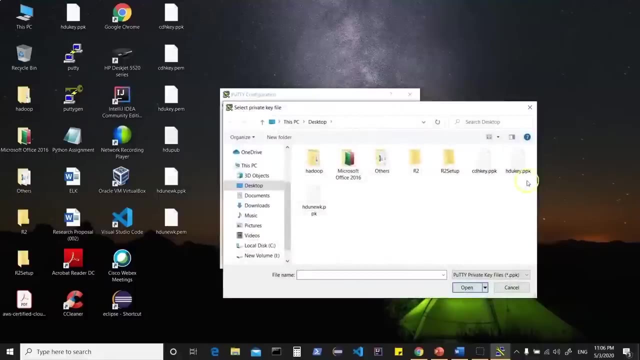 this public IP. so let's do a copy to clickboard. now go to putty and here I will say hostname, where I'll say HD, you give my public key, I'll click on SSH and in SSH I'll go to authentication. now, here we need to give our PPK file. so the PPK file was HD. you new key, select this one. 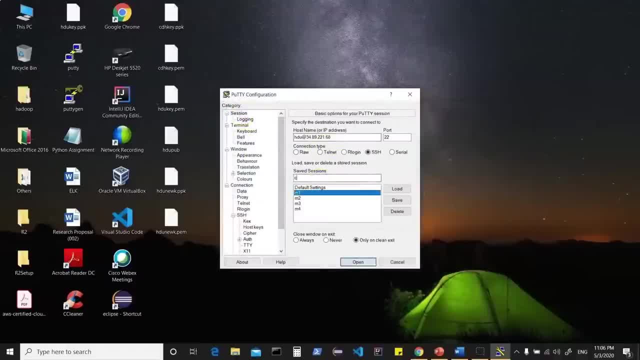 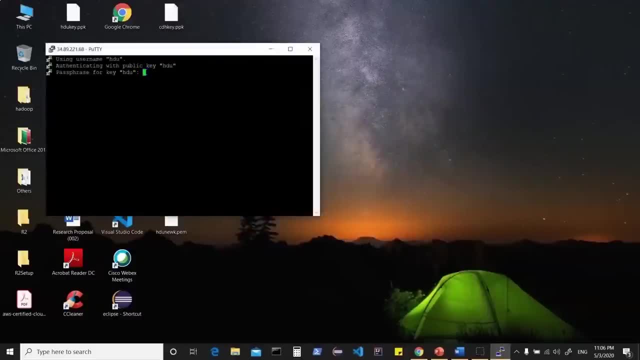 come back here, come to the session, give it a name, for example c1, save it, and then you can just say open and say yes, and you are logged in to your machine. now, once you're logged in, you can always do a minus SSH and that shows you the file. so this is how you have just used the Compute Engine to 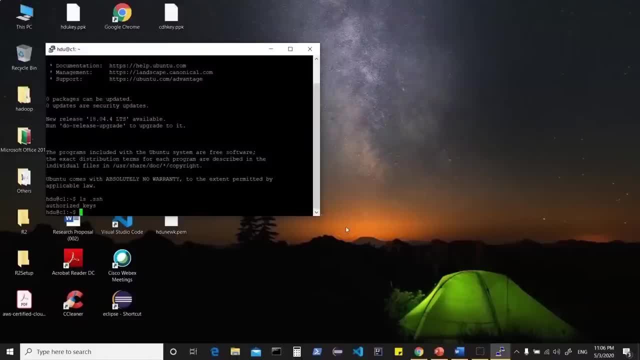 spin up an instance, but we used a template which basically allowed me to create this instance and then I can connect to this instance and then I can start working on this. so when we talk about features of Compute Engine, it has predefined machine types, as we saw. so Compute Engine offers. 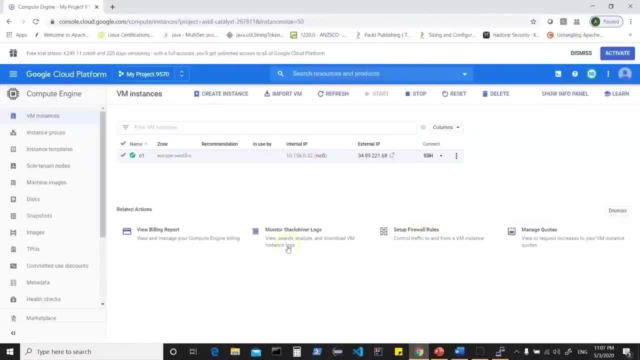 different types of machine types. so we can see that we have predefined machine types, as we saw. so Compute Engine offers different predefined virtual machines and this they have configurations for every need, from small general-purpose instances to large memory optimized instances with up to 11.5 terabytes of RAM. you can have fast compute instances, optimized up to 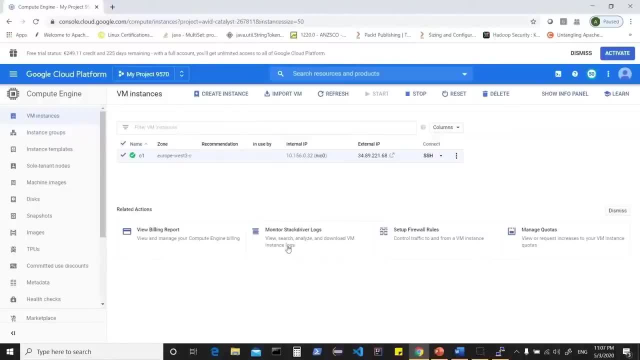 60 virtual CPU cores. you also have custom machine types, so you can create a VM that best fits your workload, and by tailoring a custom machine type to your specific need, you can realize significant savings. there are preemptible VMs, which we saw. there is also a facility which 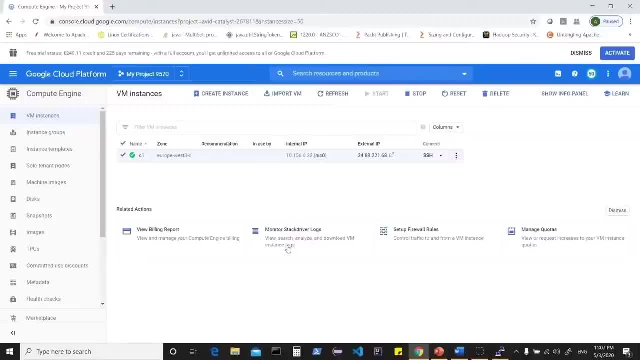 allows you to take the benefit of live migration for VMs. you have durable, high-performance block storage for virtual machine instances in the form of persistent disks where data is stored redundantly for integrity, flexibility and to resize storage without interruption, and you could be choosing HDDs or SDDs for your instances. now you also have a lot of options for your 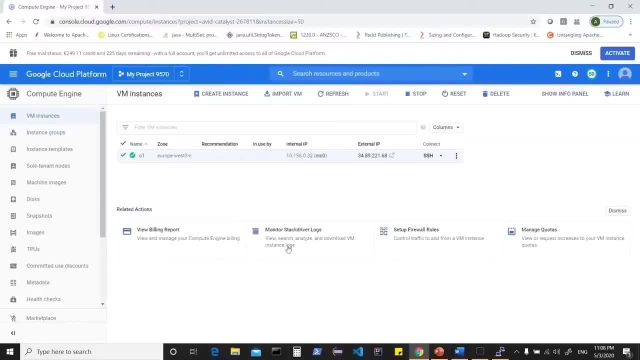 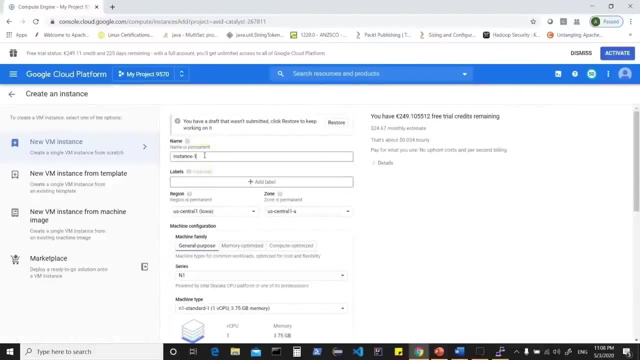 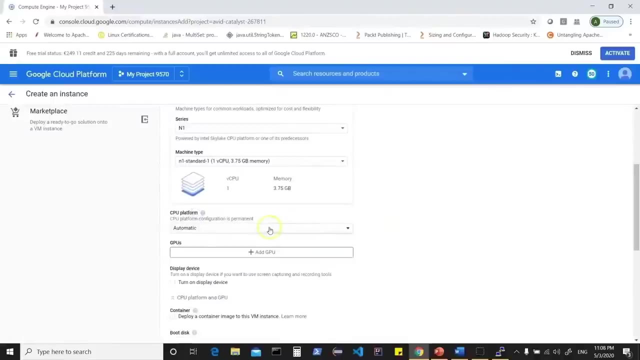 option, such as GPU accelerators. so, for example, if I just click on create instance and I can look into that. so here, let the instance name be instance one and what I would be interested in looking at, this one which says CPU platform and GPU. so CPU platform configuration is permanent. you can also 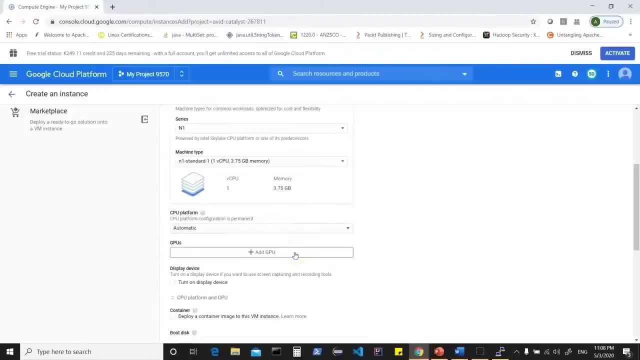 do add GPU. so GPUs can be added to accelerate computationally intensive workloads like machine learning, simulation, medical analysis and virtual workstation of applications. so you can add and remove GPUs to a VM when your workload changes and pay for GPU only while using. so these are some of the 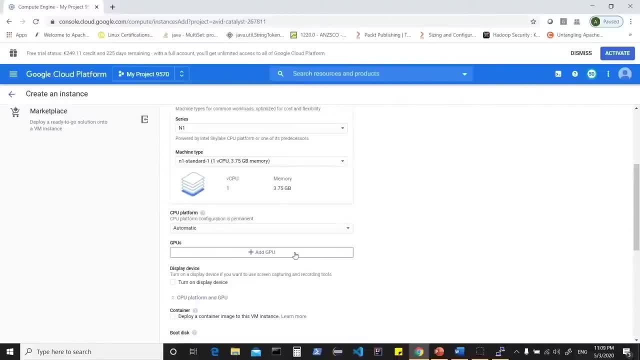 features which basically Compute Engine offers, and we already know that Google builds in second level increments, so we only pay for the compute time. now there are different savings which are possible, so you can add some of the features like machine learning, simulation, medical. you have commitment savings which basically means you can save up to 57 percent with up upfront cost. 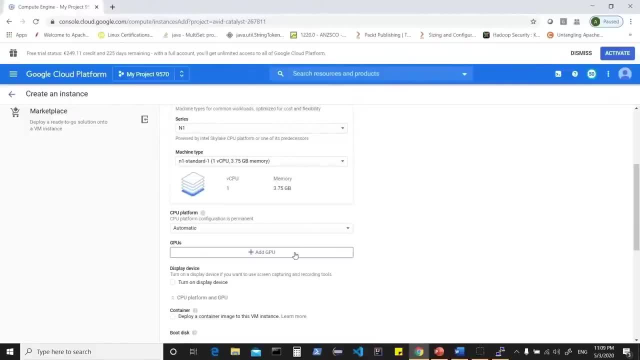 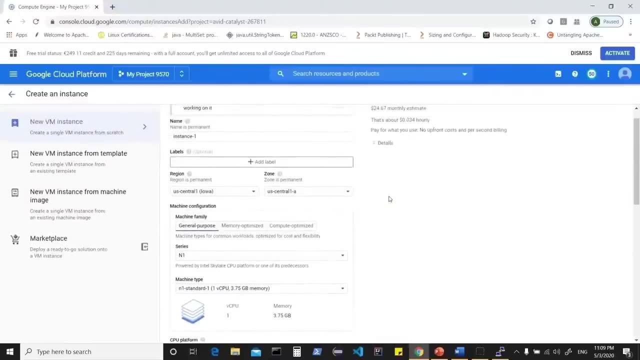 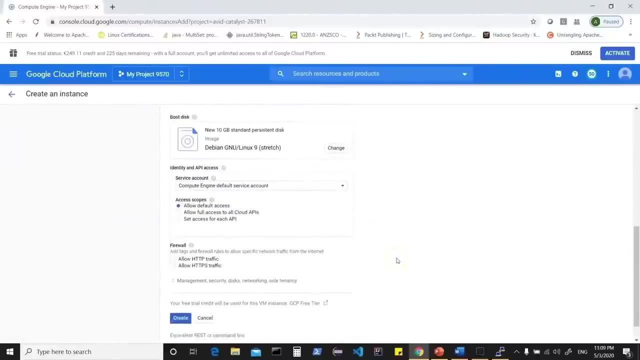 per instance, type lock-in, You have container support so you can basically run, manage and orchestrate docker containers or compute engine instances. So here, when we are setting up our instances, there is an option which basically allows you to use or deploy docker images. Now 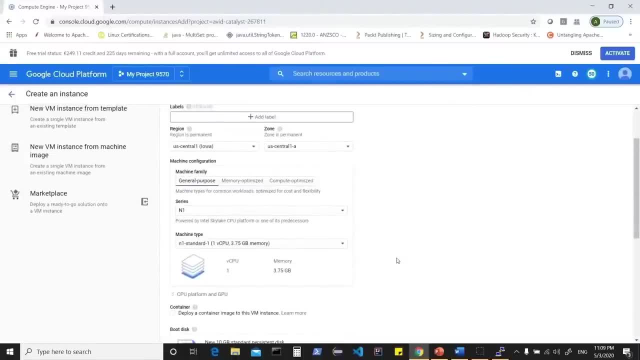 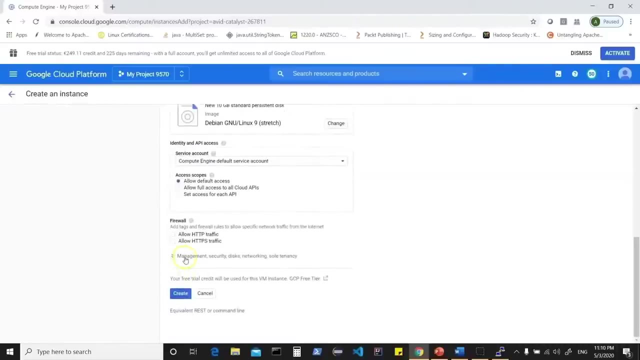 that can be done. you can also benefit from sustained use savings, that is, sustained use discounts, which are automatic discounts for running compute engine resources for significant portion of the billing month. You can create a reservation for VM instance in a specific zone, which is basically seen under your management section here, and you can ensure your project. 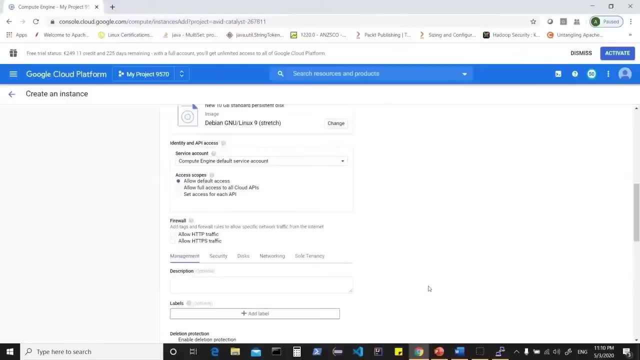 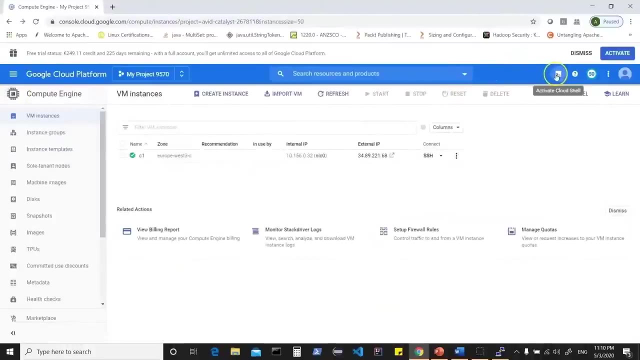 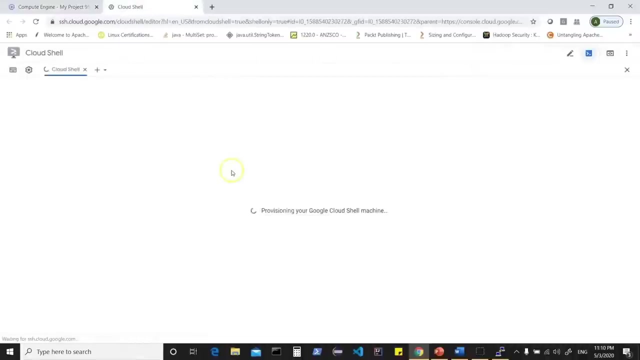 has resources for future increases in demand and, if no longer needed, delete the reservation. So these are some of the features of Compute Engine. What we have done is we have created Compute Engine using the console. Now you can go back. You can also do that using Cloud Shell, and you can click on this one which activates Cloud Shell. You could also have the Cloud SDK support on setup on your machine which can be used. Now I can just open this in a new window and from here I can start giving commands. if I would be interested in setting up an instance from 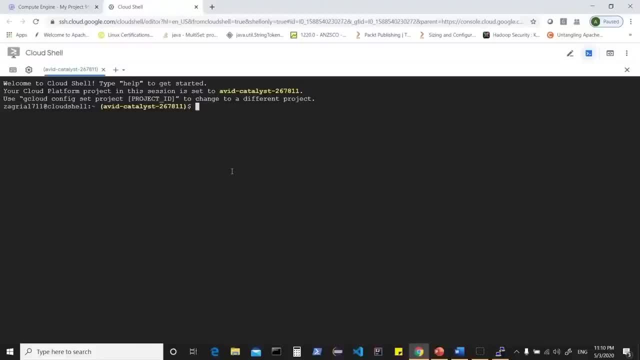 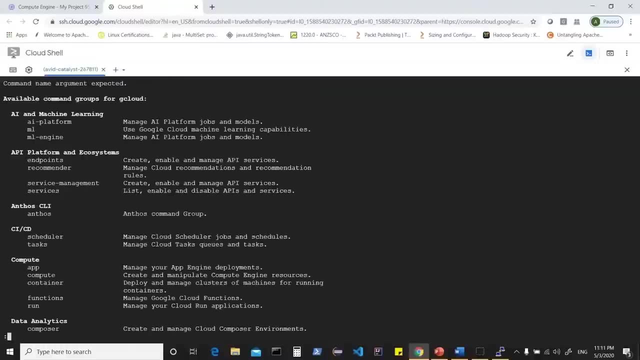 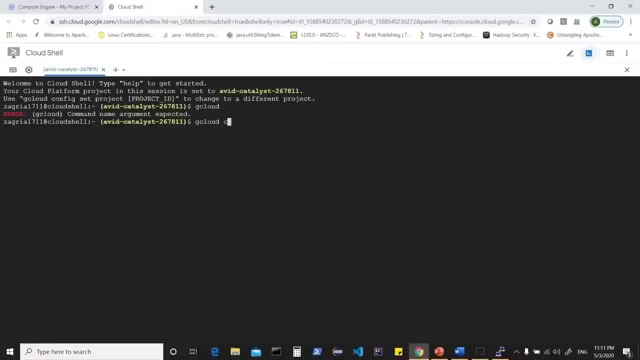 my, which shows an option to create and manipulate compute engine resources. Now I can just do a queue to quit, I can do a G Cloud Compute and that basically will again show me different options which are available if you would add spaces to several company offerings. 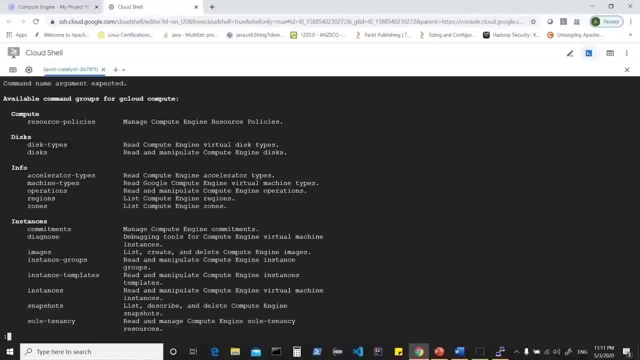 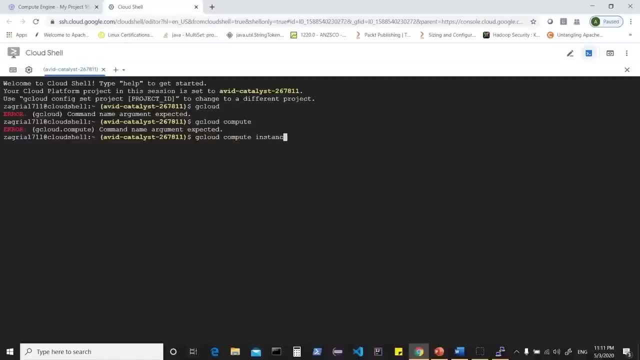 be interested in setting up instances from the command line. so here I can say G cloud compute and then go for instances. and if you do not know the commands you can just hit enter. that will show you all the different options which we have. so here we have different options such as list or create or start. 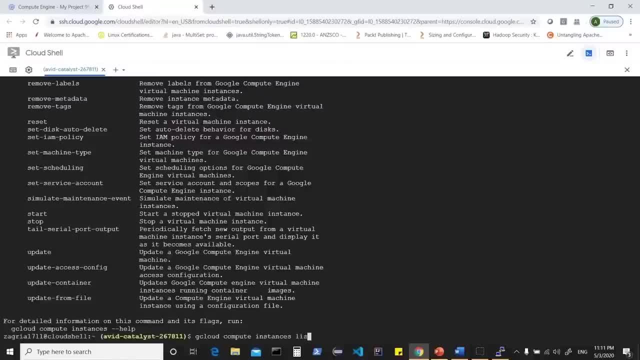 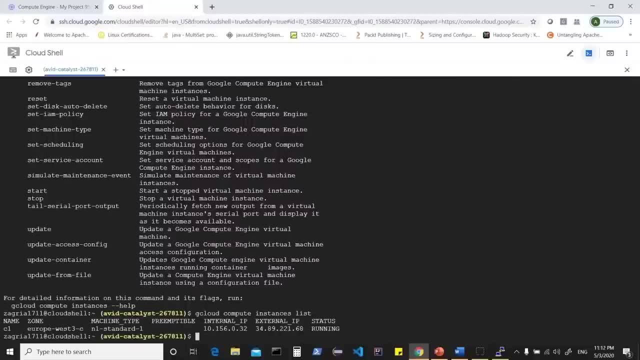 or update. for example, I can just do a list here to see what instances I have, and the instance which we just created shows up here. it says that status is running. I can just stop this instance. I can delete this instance. I can even create an instance by using a create command here and you can just do a. 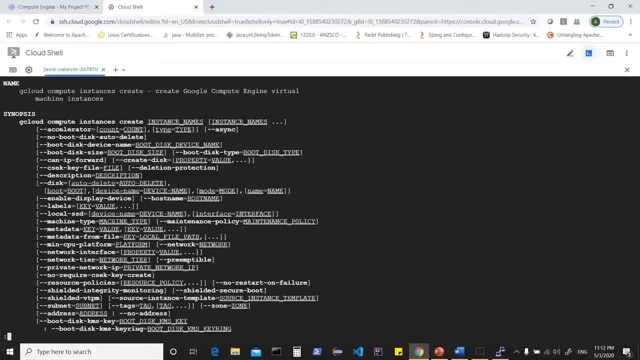 create help which will show you what are the different options you can give. so it says: instance name is what you need. you can choose an accelerator, you can choose the boot disk and various other options. so I can just say create and then I can just click on create and then I can just click on. 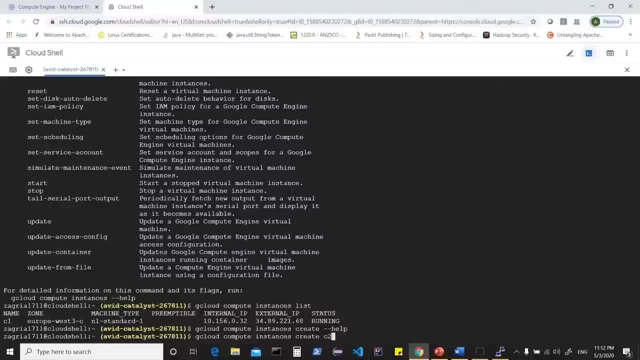 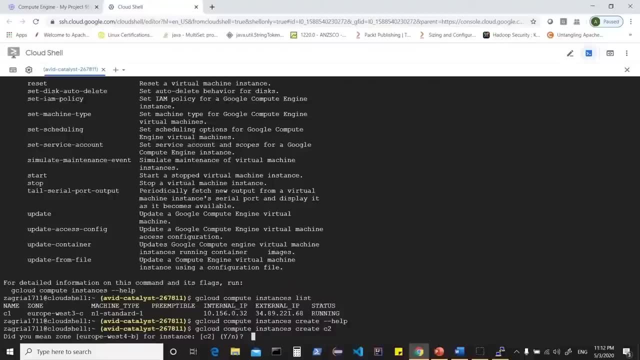 create and then I can give a name, for example c2, and once I click on this one it says: did you mean Europe West for zone? so it is asking me for the region and the zone and I can say yes, and these settings are coming from my default. 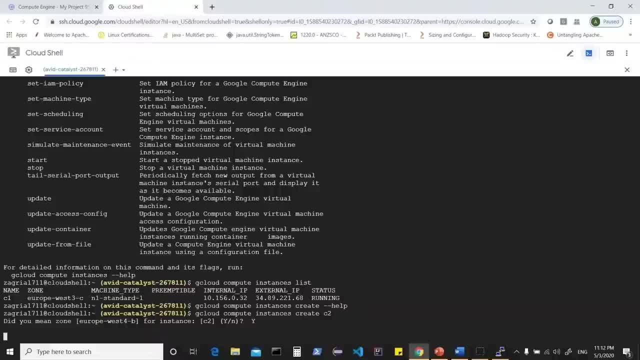 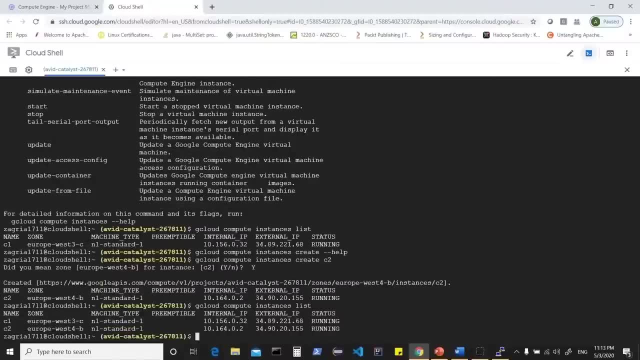 profile. I can always change those by changing the metadata. so now we have created an instance, it says running. if we do a list again to see, we see two instances created. one was in Europe West, three. one was on in Europe, yes, West. for both of them have internal and external. 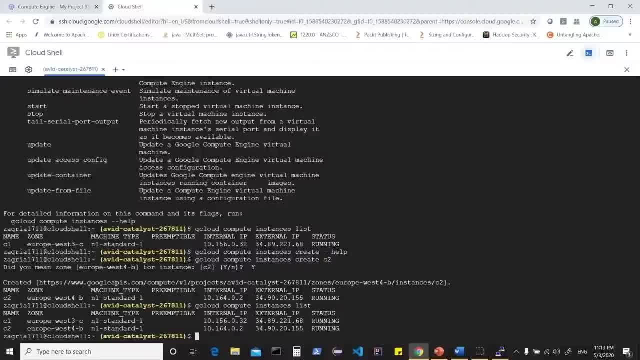 IPs. now you can do a describe to look at the different options here. so G cloud basically allows you different commands which you can use to work with your instance: to create instances, to change the metadata if you would want to change the region, if you would want to add a startup script. all those options are. 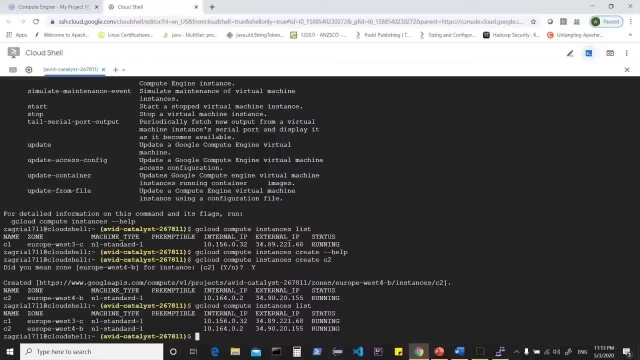 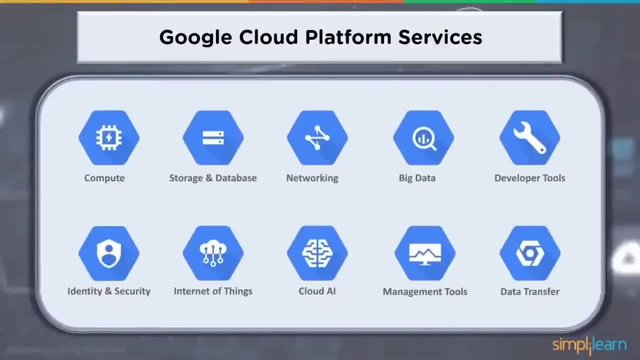 possible from the command line, which we can learn in detail in later sessions. so this is your compute engine as a service. now that we have learned about the compute domain and G compute services, which is offered by GCP, let's also learn about storage and databases. that's again within the 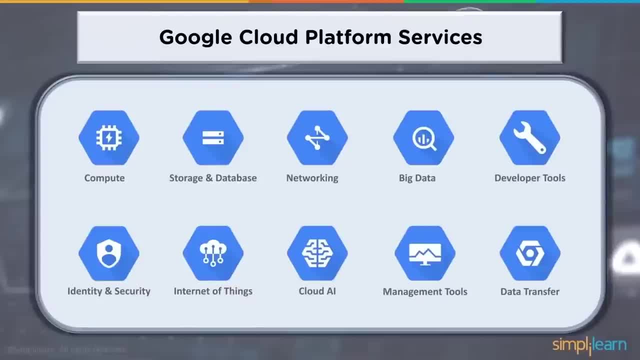 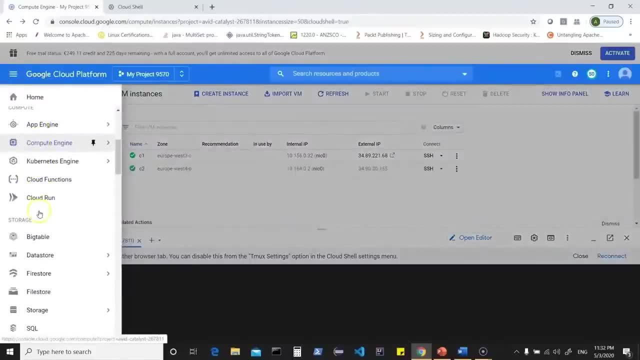 storage domain and the services which are offered by Google Cloud Platform. now you can go back to console and here you can click on this one and here you can just scroll down to see what are the different options in storage. so you have options such as bigtable, you have datastore, firestore. 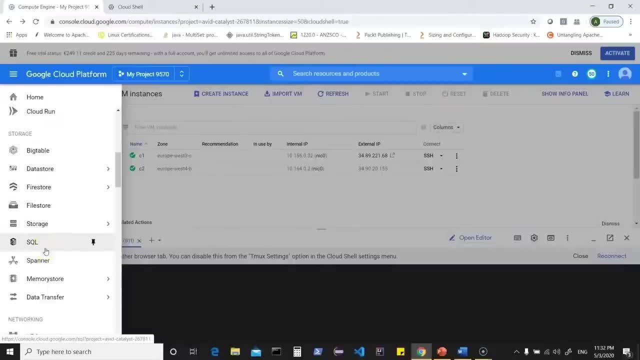 file store, you have SQL based services, you have storage which is object storage, and then you have other options which are available. so Google Cloud Platform offers different storage based services, out of which storage which is your object storage is quite popular. one click on storage and that basically. 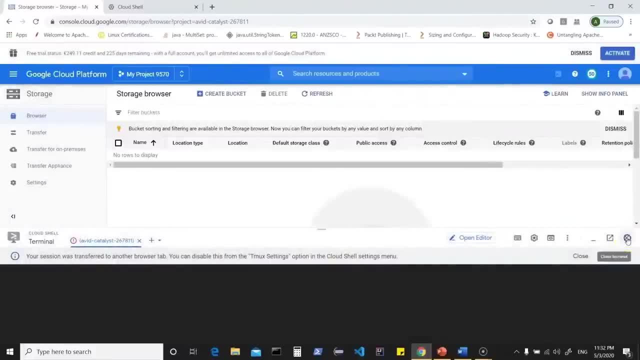 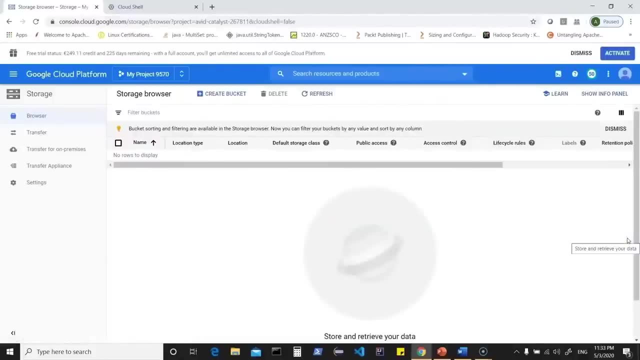 shows you an option which talks about storage browser. so this is your Google Cloud's object storage. so when we talk about object storage, it is basically a storage where you could store any kind of data, and when we talk about object storage, it is a bunch of bytes which we address, wherein every object will have a 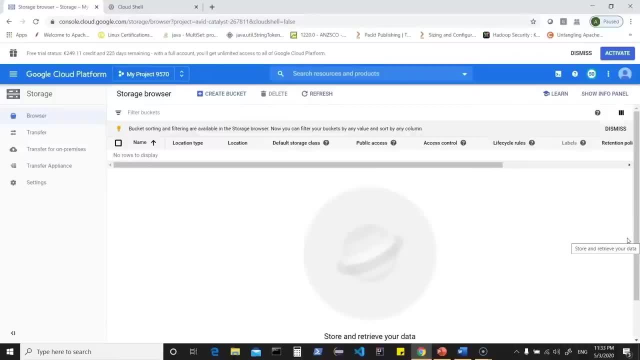 unique key. these unique keys are in the form of URL which allows you to access the object. so storage is comprised of what we call as buckets, which are used to store and hold your storage objects. the storage objects are immutable and every change creates a new version. now you can also have control access via IAM. that is identity. 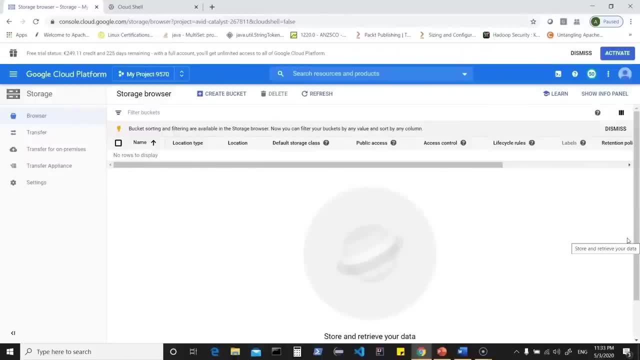 access management or via access control list. so there is also an option called object versioning, which basically says, if it is on, every time you try to store the same object, a new version of the object would be created. otherwise, newer option will override old one, as we cannot archive the old version. so let's see how we work. 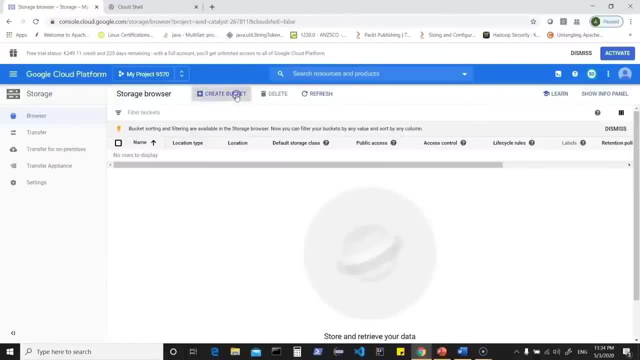 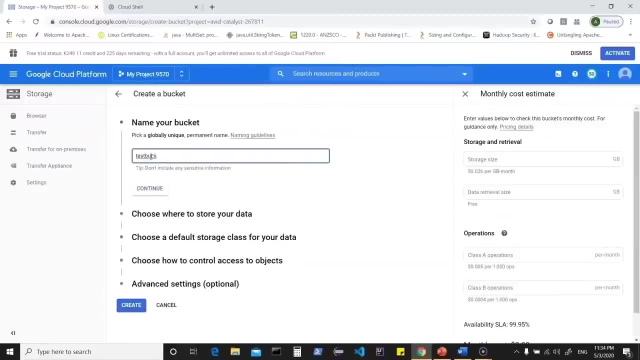 with this object storage. so here you can click on create bucket. now, once you click on create bucket, it needs a name. so let's say test bucket and here I can just give, say number one so that says this is the name of my bucket. now I can. 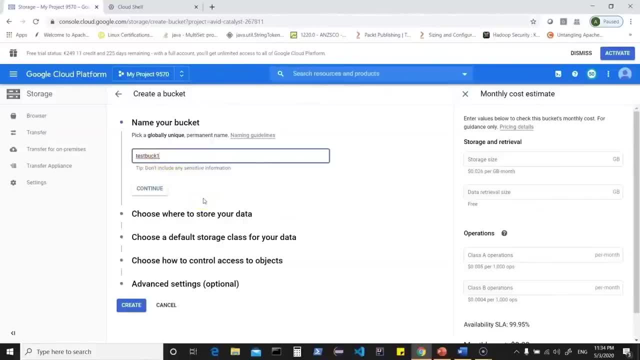 directly click on continue, or it would be good to look at different options which are available here. so when you click on choose where to store your data. so it already gives me an option. it says the bucket name is already taken, so let me give it a unique name. so let's say: 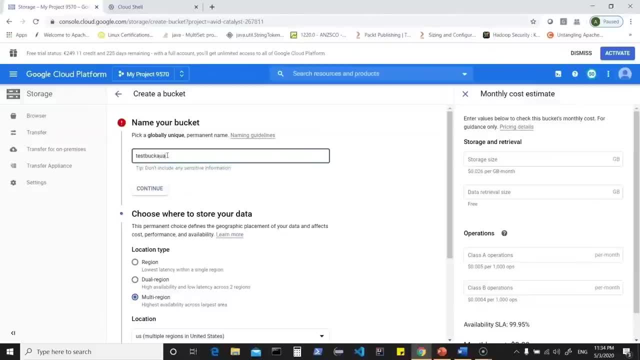 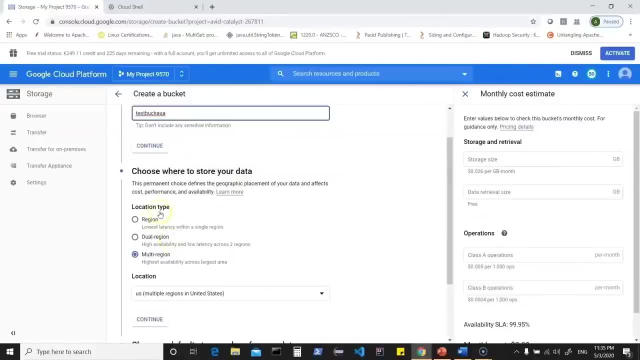 test buck and let's call it aua, so that should be unique. now here it says: choose where to store your data. so this one gives you location type, so you can have region specific buckets which give you lowest latency, that is, fastest response time within a single region. however, it does not make your storage highly. 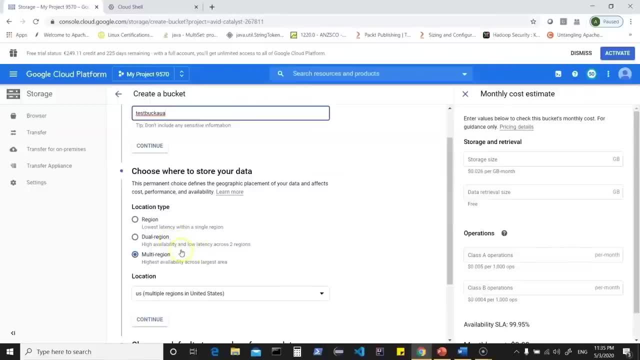 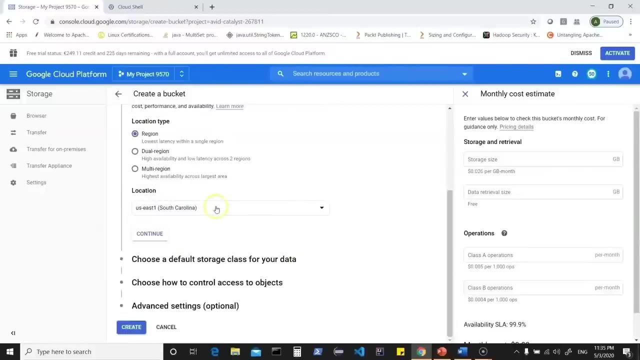 available. you can make a dual region, which is basically allowing your bucket or storage to be accessible across regions. you can also make it multi region, which is highest availability offered as of now. we can choose region specific and now it asks you to choose a location now as. 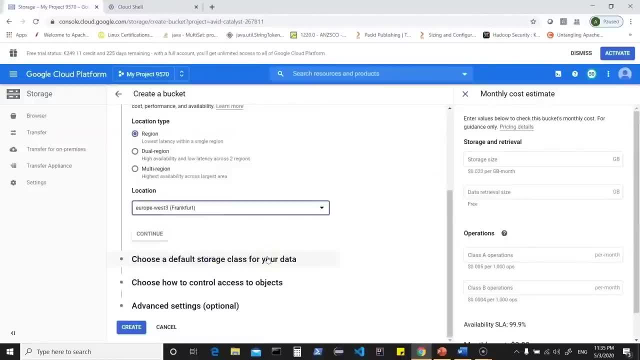 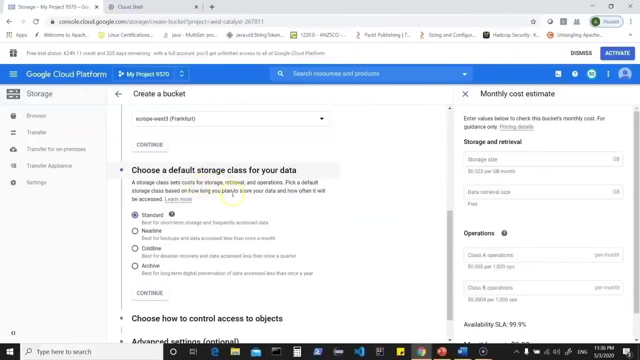 always I will choose Frankfurt. now I can click on continue and rest all the rest. let all the storage options be default. or you can click on a default storage class. now that tells you, based on your storage class, there are variant costs when it comes to storing, retrieving or doing any kind of operations. so you have 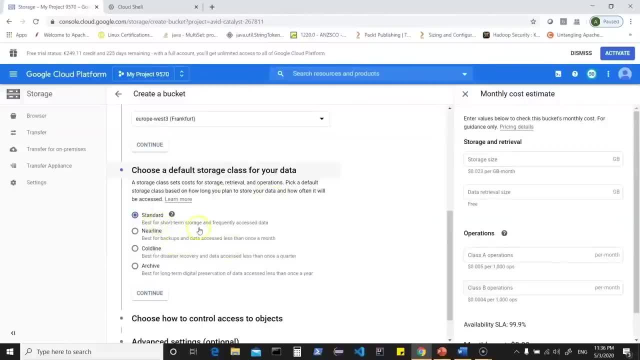 a standard option, which says best for short-term storage and frequently access data. you can also go for cold storage, such as near line, which is best for backups and data access less than once a month. you can go for freezing storage, such as cold line, best for disaster recovery and data. 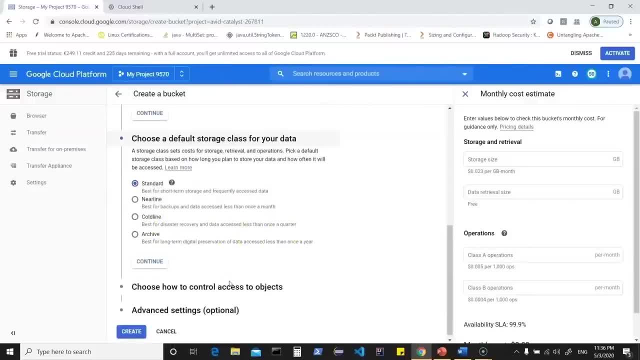 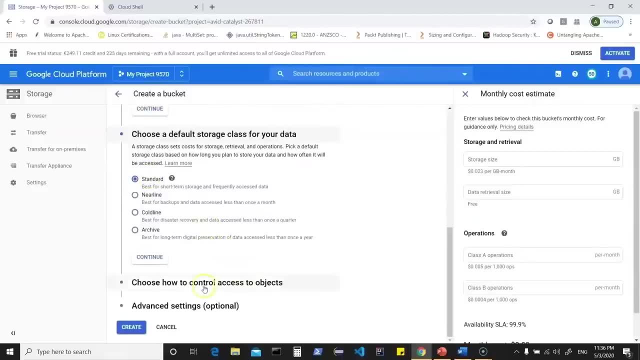 accessed less than once a quarter, or you can go for archiving where the data is accessed less than once a year. let's go for standard as of now, and now you can choose how to control access to objects, so you have fine-grained or uniform let. 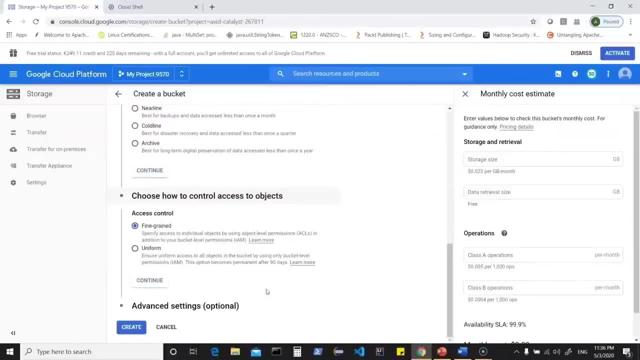 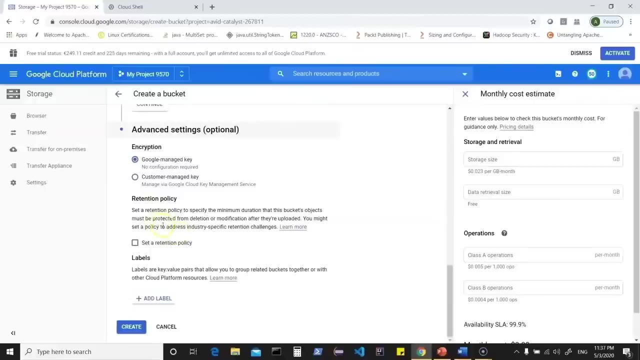 it be fine-grained, wherein you can give additional permissions at bucket level using IAM or object level permissions using access control list. in advanced settings you can choose the encryption and you can also choose a retention policy, so a retention policy to specify the minimum duration that this buckets. 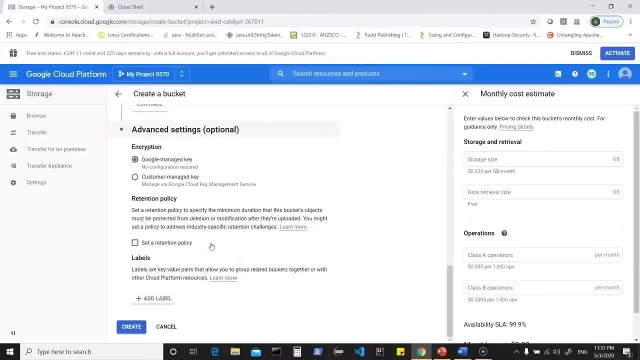 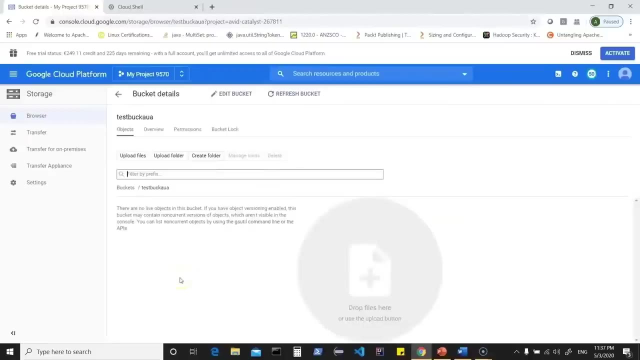 objects must be protected from deletion or modification after they are uploaded. you can always learn about this more by clicking here. now, once I have chosen all the relevant options, I can click on create and that, basically, will create a bucket by the name I have given. I can click on. 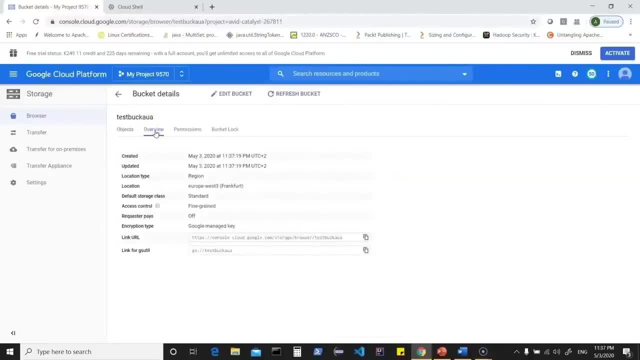 overview to basically see brief details about my bucket, such as region, what is the default storage class, and it also shows you the link URL which can be used to access your bucket. it also gives you the link for GS util. GSU tell is a command which can be used in your cloud shell to basically work with your 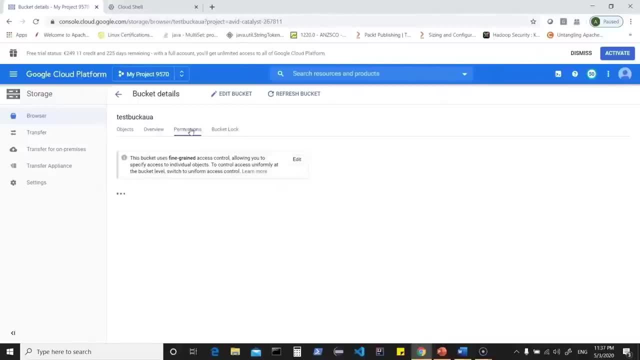 bucket, click on permissions to basically see what kind of permissions are already in place and you can then make changes. you can basically add members. you can view by different roles. so for example here by default it shows other services, such as data proc or your bucket owner or bucket reader related. 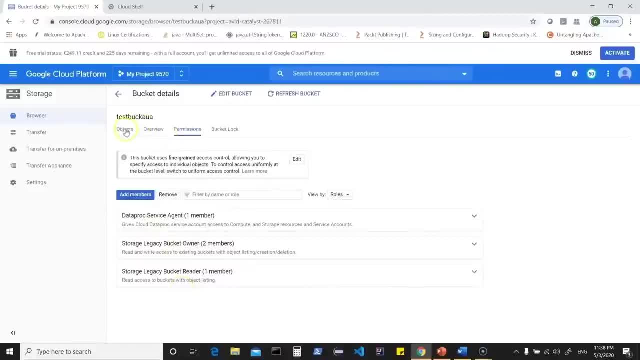 permissions which have been already granted. now, once i have looked at my bucket, i can start using it. i can drag and drop and push in files here. so as of now, there are no live objects in my object storage. that is in my bucket. what i can do is i can click on upload files and then 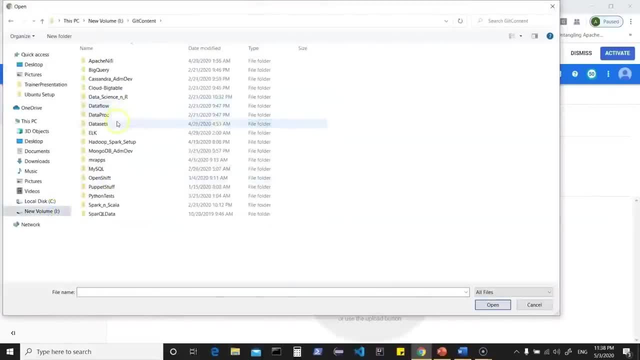 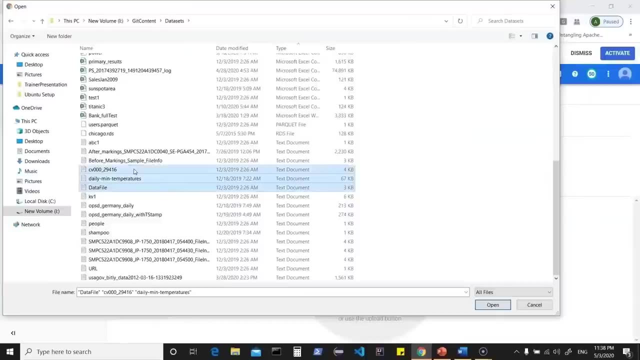 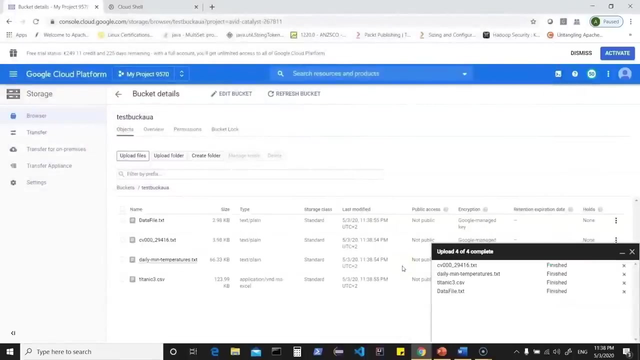 i can choose a location from my machine. for example, i'll go into data sets and what i can do is i can choose some of the files here in any format- let's choose csv or text- and just to open it up. this one is my custom file, so this one will basically upload my data sets here. now, once i've 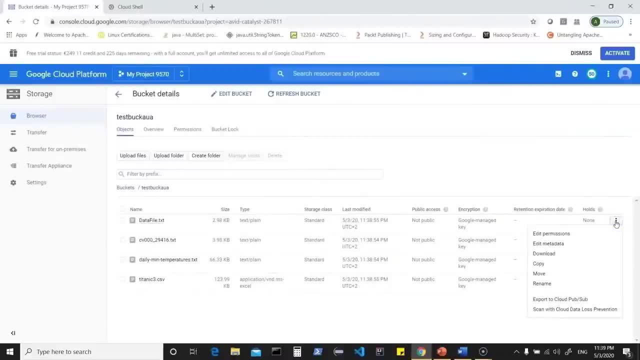 uploaded the files. i can basically close this one- i can look into options here- which says edit permissions and edit metadata. if you would want to download it, if you would want to copy, move or rename it, if you would want to export to a different service called cloud pub sub, which is 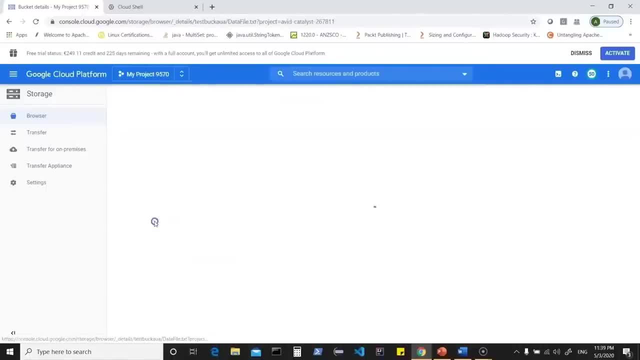 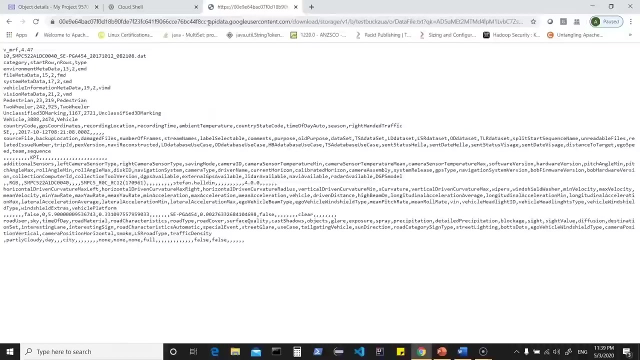 publish subscribing messaging system. you can scan the data on a particular file and that basically shows you the URL which basically allows you to access this file. You can try copying this. You can click on download and download this file. You can even try accessing this from public and that basically shows you the content of this file, based on the. 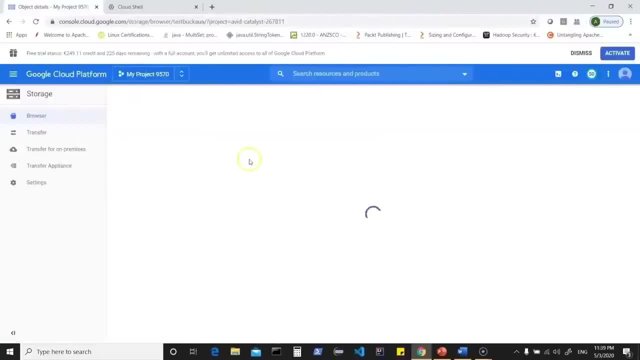 permissions. So this is basically your object storage, which is one of the service which is offered. What you can also do is you can create folders, and within folders you can then upload your data. So this is your Google Cloud storage option, which is for your object storage, That is. 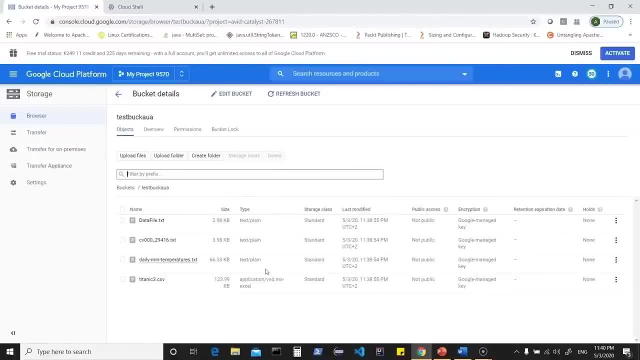 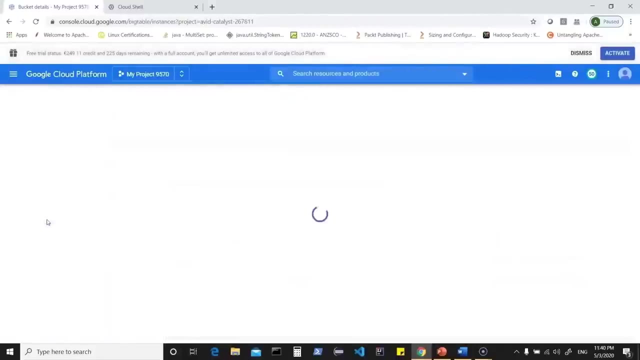 you can add different items, You can give different permissions and you can use this Google Cloud Platforms storage service offering. Now you also have other options, such as big table, and we can go into that By clicking here and click on big table. So big table is one of the service which kick-started. 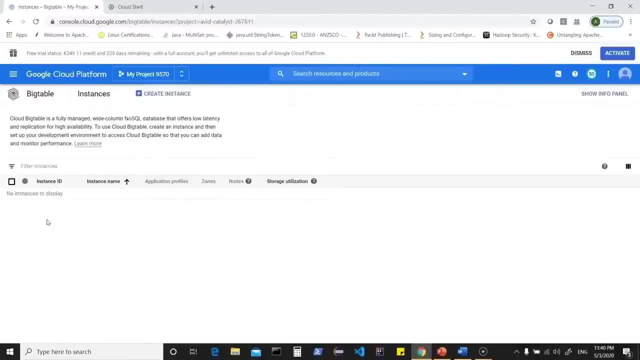 NoSQL databases. Today in market we see different NoSQL databases, such as Cassandra, HBase, MongoDB, CouchDB, Neo4j and many others, So you can basically use big table, which was the pioneer when it comes to your NoSQL databases, or not only SQL databases. So the problem 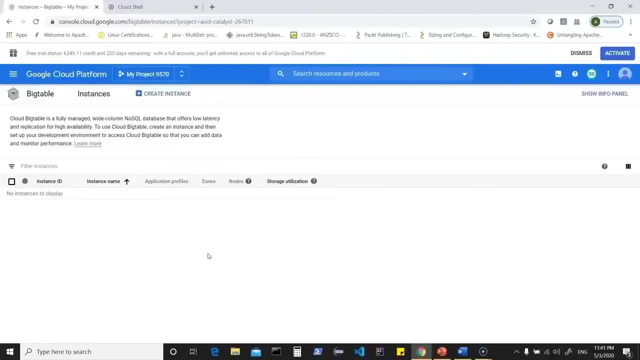 here is that you have to go to your NoSQL database and you have to go to your NoSQL database and you have to go to your NoSQL database. So the problem initially faced by Google was that the web indexes behind search engine were taking too long to build. So company wanted to build. 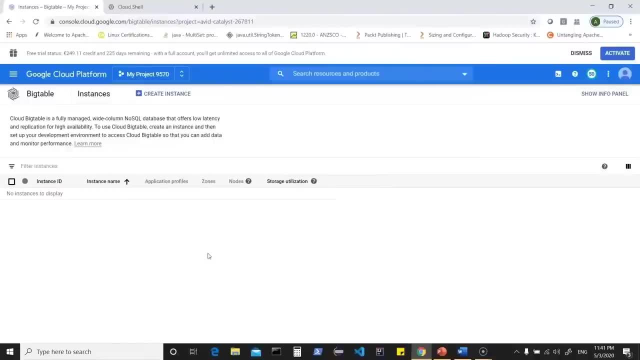 database that would provide real-time access to petabytes of data, and that's where big table began. So big table powers different other Google services, such as Gmail, Google Maps and other services, and in 2015, it was launched as a service for customers. So, when it comes to scalability, 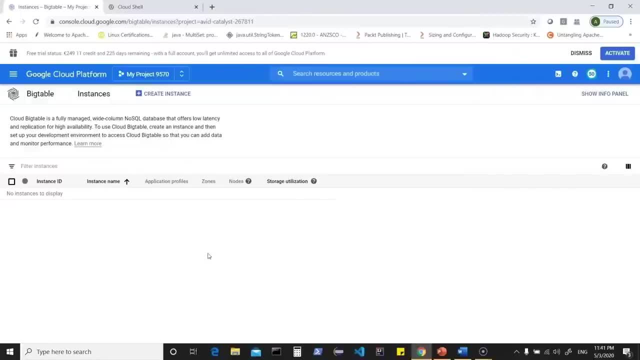 with use of big table, you can increase your machine count without any downtime and you can handle admin tasks like upgrades, restarts and so on, which are basically taken care by the cloud provider. Data present in cloud big table is encrypted and you can use IAM roles to specify. 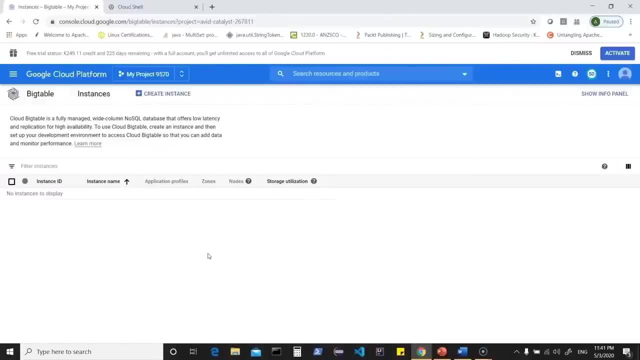 access. So data written to or from big table is through data service layers such as managed virtual machines, HBase REST server and so on. So if you want to use big table, you can use HBase REST server, HBase REST server and so on. So if you want to use HBase REST server, you can use HBase REST server. 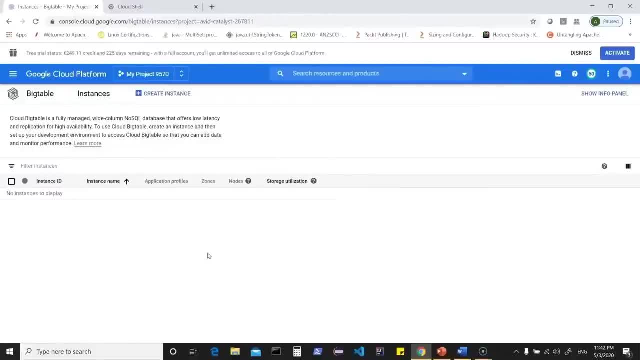 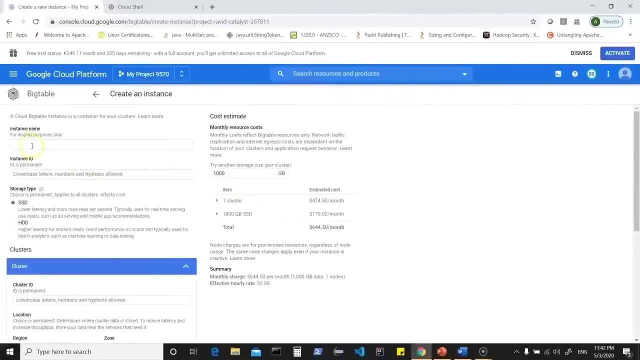 HBase REST server, Java services, HBase client and so on. Here, if I would want to use big table, I can click on create instance and that basically tells me cloud big table instance is a container for your clusters. Now here you can give a instance name. So, for example, I will say a, u, a. 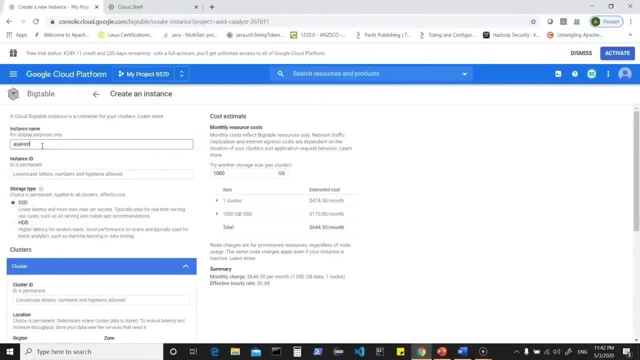 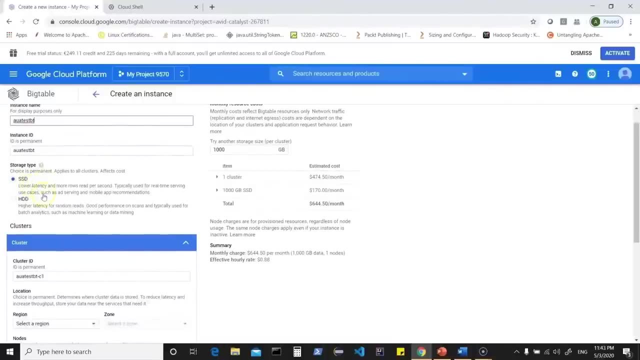 and then say, for example, test, and let's say big table, So that will be the name of instance. This will be permanent. You can choose the storage type again. You can go for lower latency, more rows read per second, typically used for real time serving use cases, or you can go for 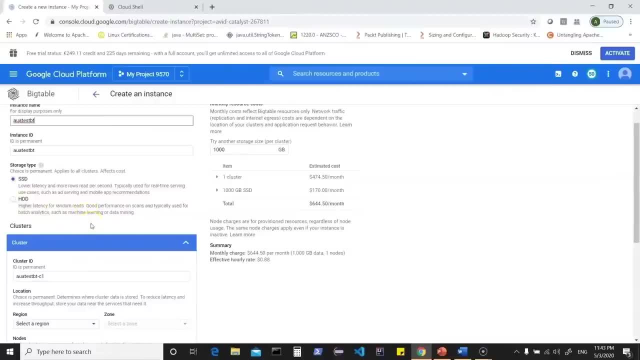 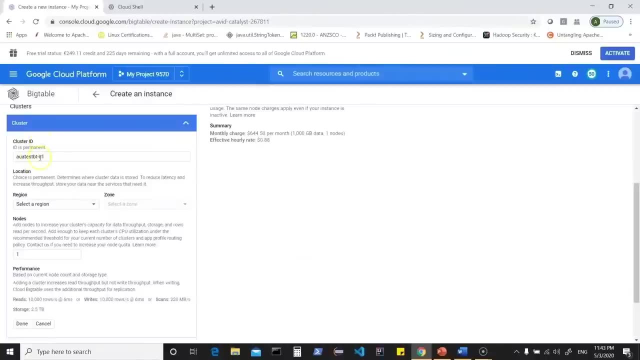 SDDs, which have higher latency for random reads, good performance on scans and typically used for batch analytics. So let's go for SSDs as of now. Here you have cluster ID which is auto populated. You can choose a region, So let's go for our favorite one here, where I can say Europe. 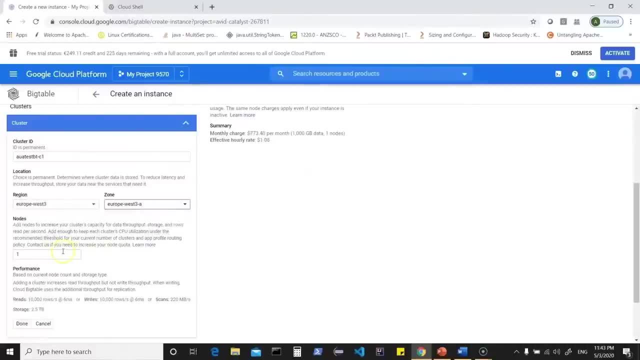 West three. I can choose a zone here and I can then choose how many nodes would I want to use for my big table. So when you talk about big table service, it will have a cluster underlying which will have various nodes which will control your data. 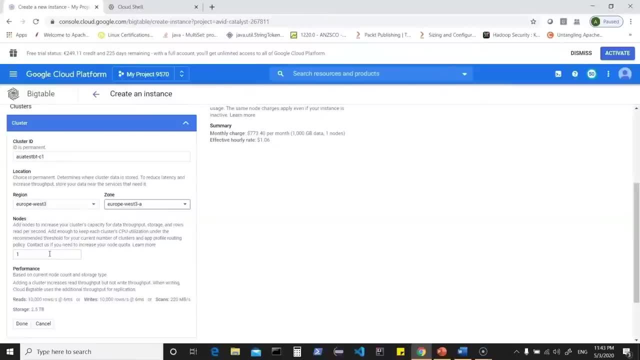 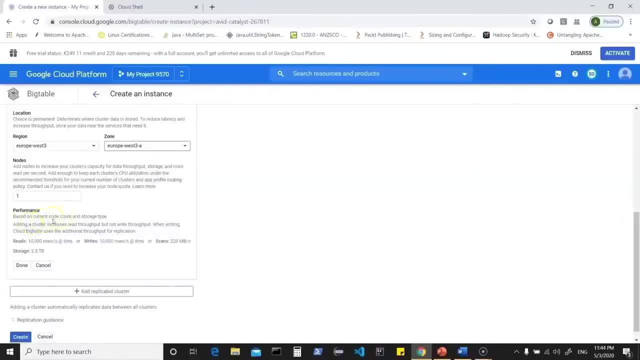 throughput storage and rows read per second. So as of now, let it be just one node and that's enough for our demo. When we talk about performance, it basically tells you, based on the current node and storage type, it tells you how many reads can happen at milliseconds. So it says 10,000 rows. 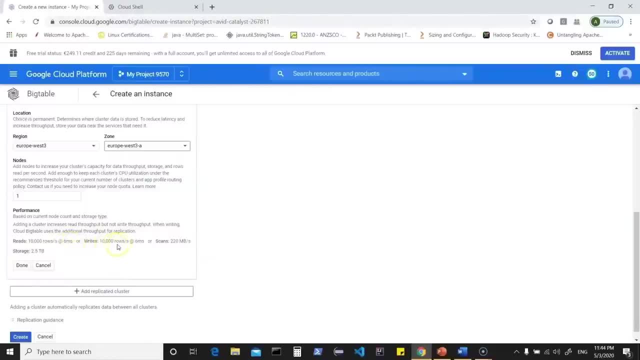 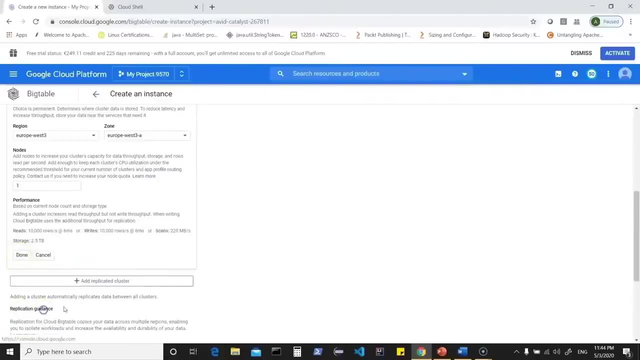 per second at six milliseconds. You have writes which are 10,000 rows per second, or you have scans which are 220 megabytes per second. Storage which is taken care here would be 2.5 terabytes, and I can then basically click on create. Now there is also some option called replication. 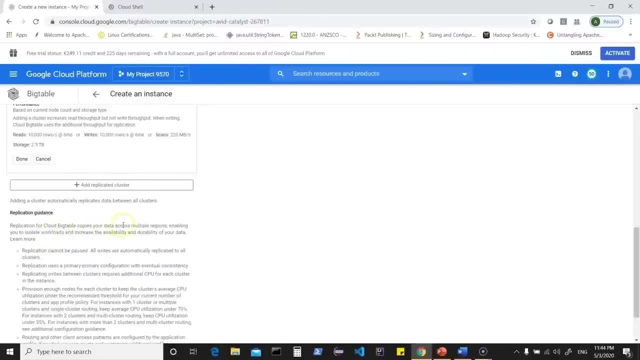 guidance which basically says replication for cloud table. big table copies your data across regions, enabling you to isolate workload and increase the availability and durability of your data. Depending on your use case, you can have big table which can be used to have your 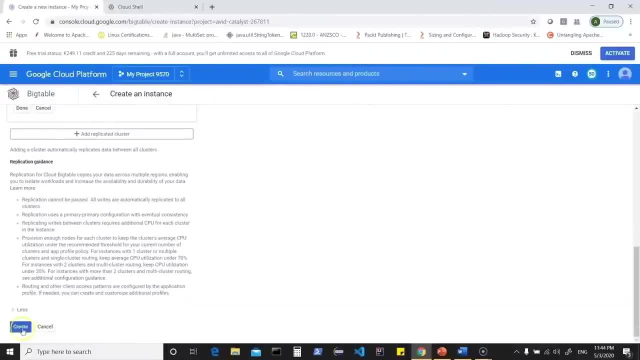 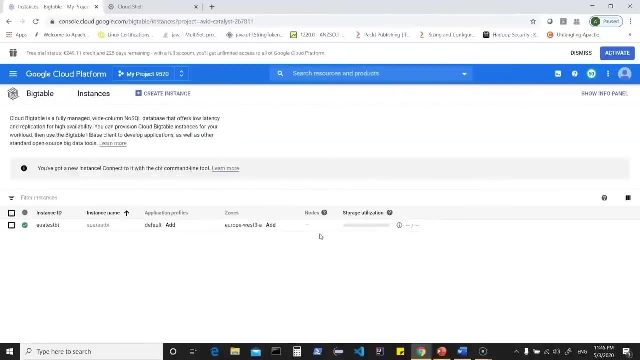 data across regions. Now you can click on create, with all your specifications chosen, and that's going to set up a cluster, or you can say a fully managed NoSQL database, which will give you low latency and replication for high availability. Now, once we have 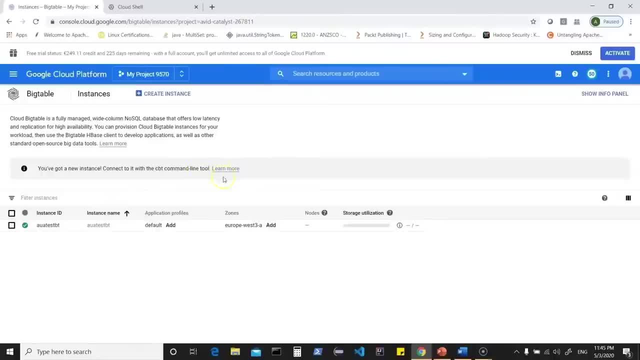 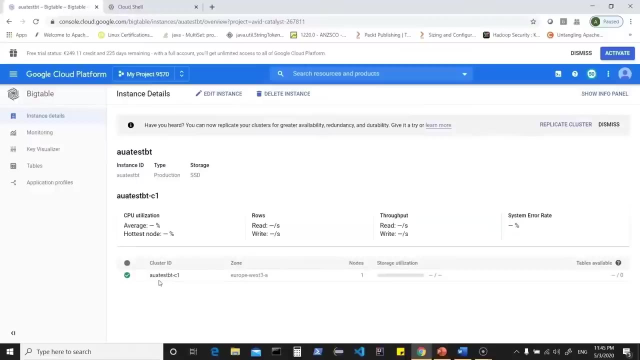 a new instance. you can connect to it with the CBT command line tool and for instructions you can click on learn more here. You can just click on this instance ID to see the details again if you would want to look into your big table setup. So it tells me here that we have one. 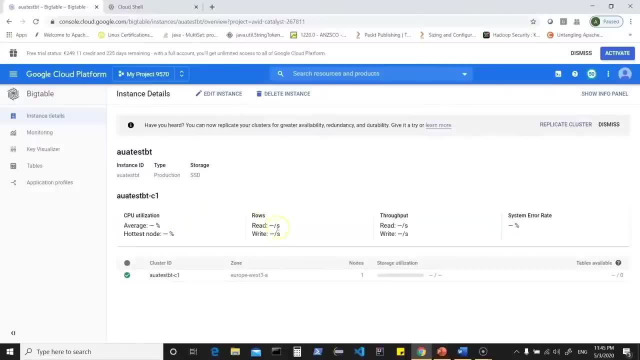 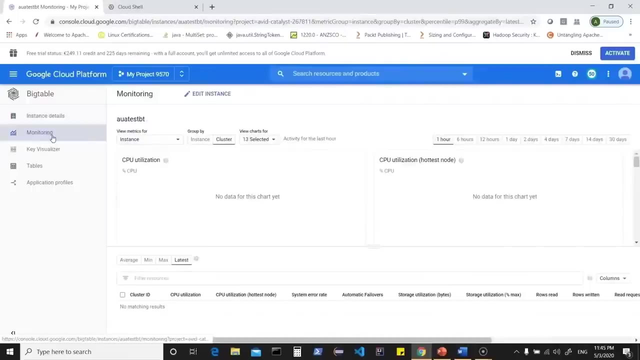 instance, What is the CPU utilization time, How many rows were read or written, What is the throughput- And this is auto populated based on your usage. You can click on monitoring and that, basically, will give you different widgets which will display information for your 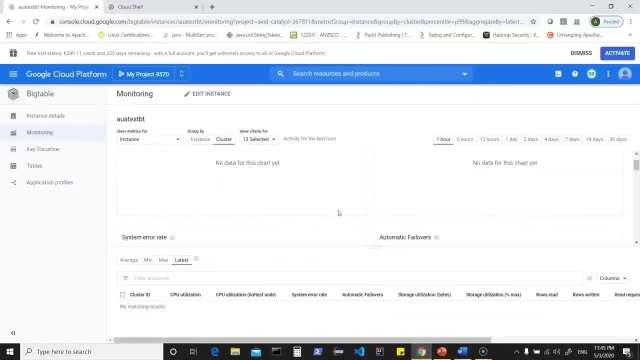 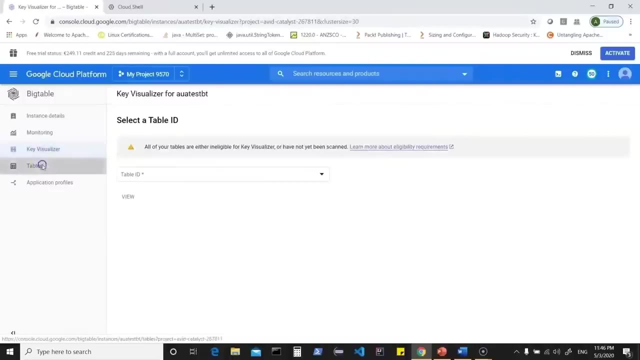 CPU utilization. What is your hottest node, depending on how many nodes you have, system errors, automatic failovers, storage utilization and so on. You can click on key visualizer, which will allow you to look into your table If you have already created some data here and you can. 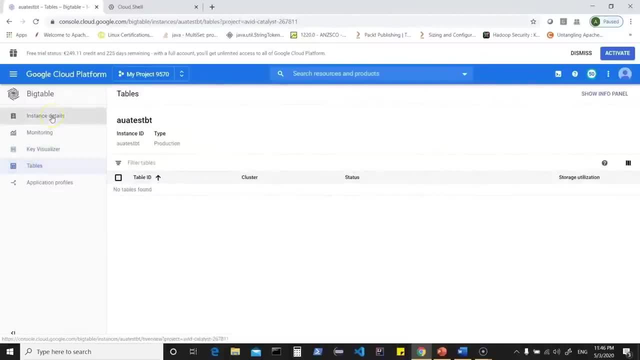 click on tables to see how many tables you have added here. So that's, in brief, about your big tables, Which is one thing which we need to remember is it's not good for all use cases, So should be used for low latency access, that is, fast access and good if at least data is greater than one terabyte. 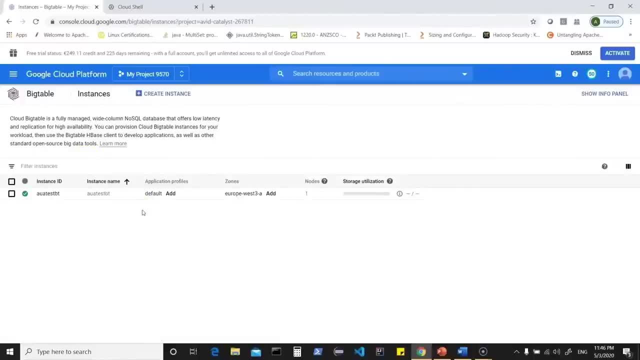 For smaller amount of data, the overhead is too high. So big tables performance will suffer if you store individual elements larger than 10 megabytes. If you want to store bigger objects, such as images, video files, then go for object storage and that would be a better option. So always remember big table is. 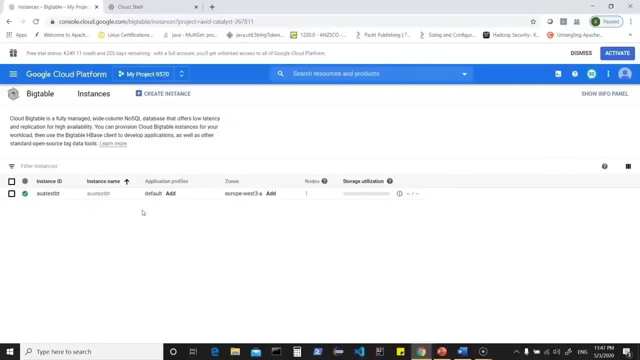 not a relational database. It's a NoSQL database and when you talk about multi-row transactions or online transaction processing, big table is not the right choice. So it can be used for wide range of applications, especially when you talk about your OLAP, that is, online analytical. 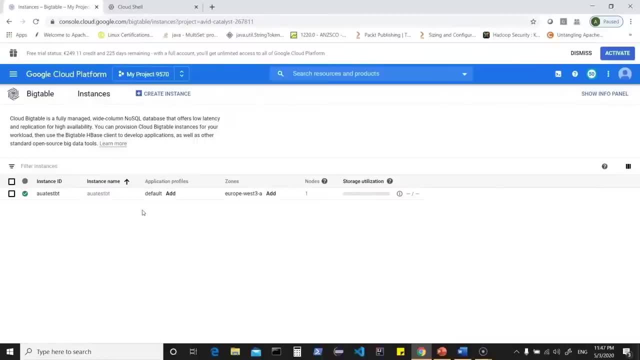 processing. So it is designed to store key value pairs and there can be different use cases. So, for example, if you are using something like cloud data flow or cloud data proc, where you would want MapReduce kind of operations, big table can act as a good storage because it has 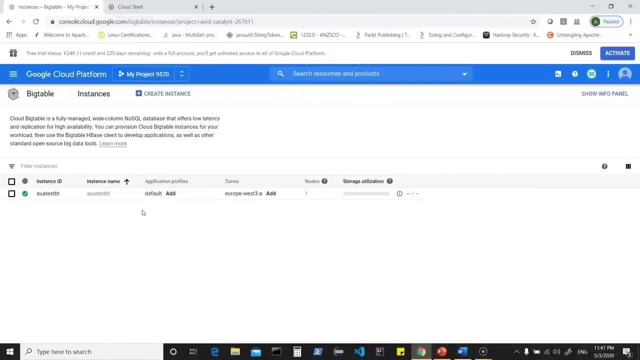 very high throughput and scalability. And the best thing is that it supports HBase API, thus allowing easy integration with Apache, Hadoop and Spark clusters, which you can bring up using one more service. So big table is a good choice for real-time analytics. It's commonly seen in financial 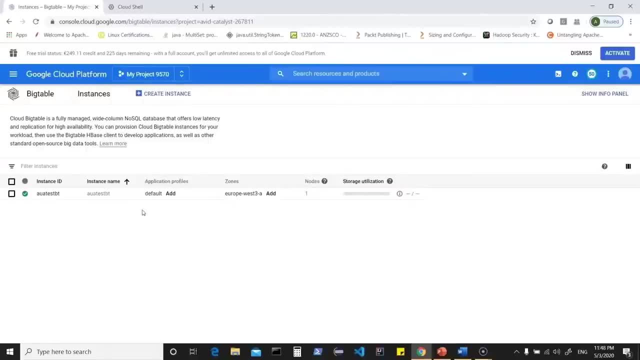 services, IoT and others, And if you are thinking of running interactive SQL, then big table would not be the right choice, but the other choice would be BigQuery. You should also remember that this has a cluster running and you would be charged if this cluster runs, If you are running a cluster. 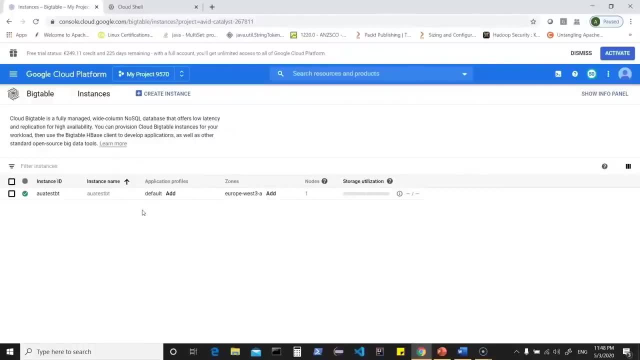 this cluster kept on running. So you have to be very careful in your free account when you are using such services. Now we have clicked on this one so I can select this one and basically I can look at the permissions, I can look at the labels, I can look at inherited permissions. here I can. 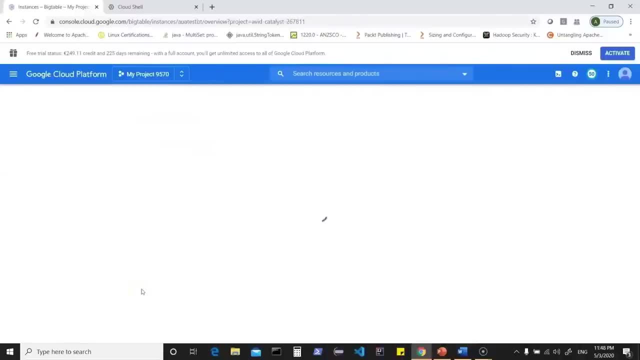 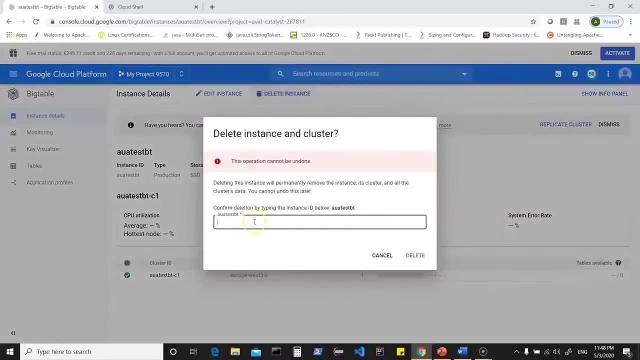 also click on my instance, which we created, and either you can edit or you can just do a delete. So, as of now, we will just delete this, which needs you to give in the name. So as of now, we will just delete this, which needs you to give in the name. So, as of now, we will just delete this, which needs you to give in the name. 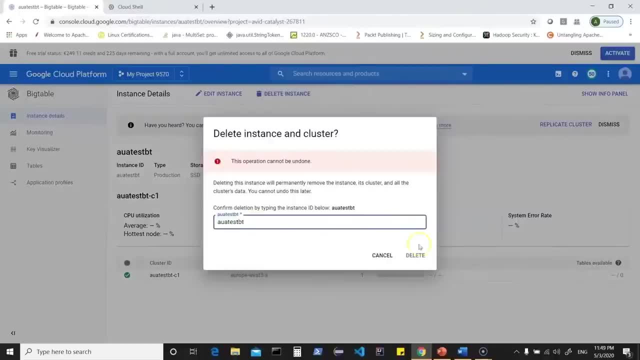 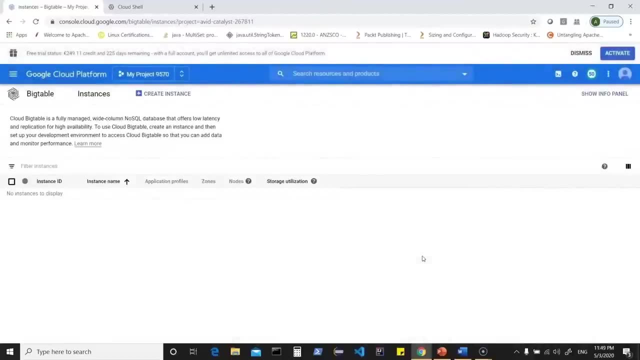 So we'll say AUATestBT and then click on delete. So whenever you are trying out different services, the first approach should be setting up these different services, seeing how they work, basically trying connecting to them And, once you are satisfied with the initial test, 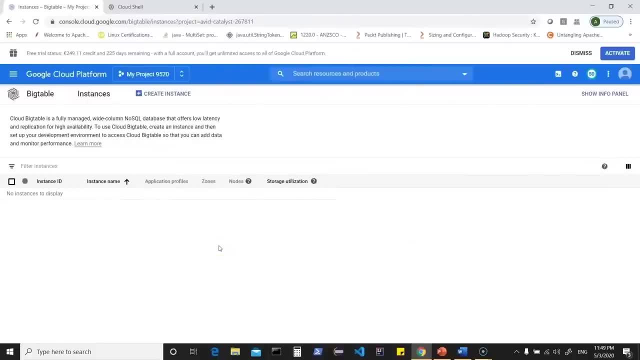 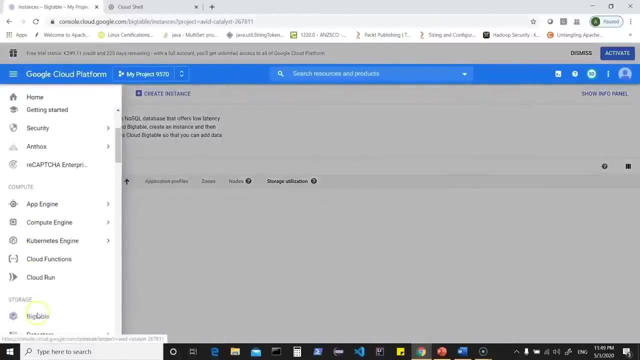 then you can plan your actions and come back and use the service for a longer duration. Now that's your big table, which is one of the offerings. We can go back into storage, and here you have other options which are available. So, for example, we were in big table. 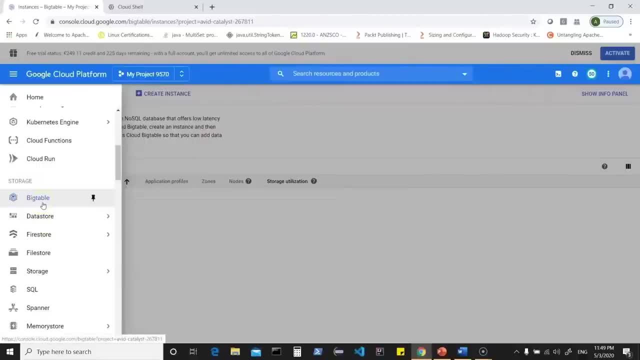 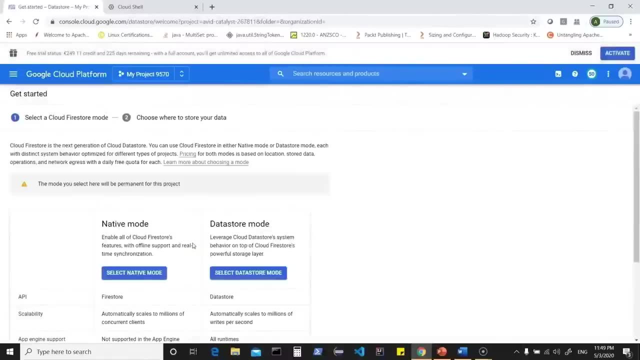 You also have an option such as cloud data store. Now, that's one more service which is offered by Google cloud platform when it comes to storage domain. So Google added software on top of big table which supports more than simple key value pairs. When you talk about secondary 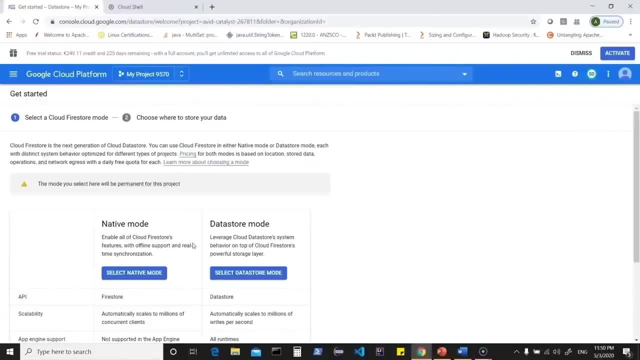 indexes instead of just having one primary index when you talk about asset properties, for reliable transactions such as SQL query, like language. So these features or these services were added to or on top of your big table, which gave birth to a new service which was released. 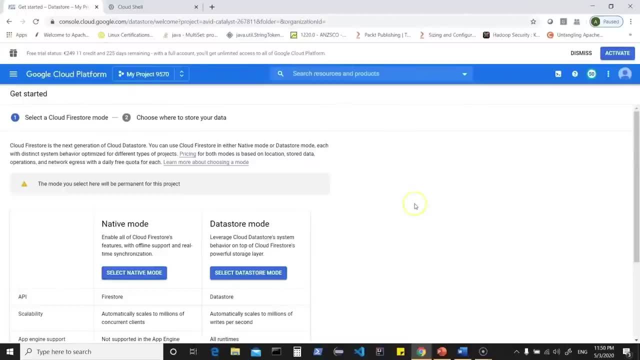 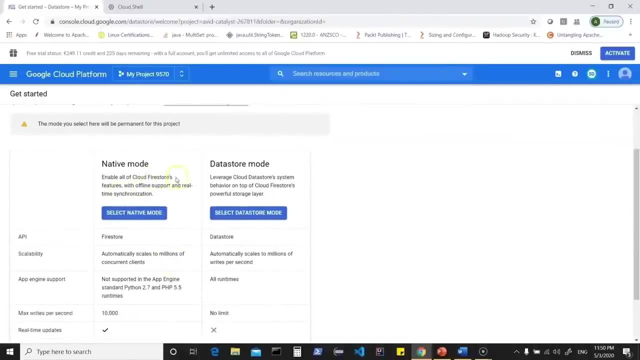 as cloud data store. So this is where you have cloud data store and you can select a cloud fire store mode. So you can go for a native mode, enable all cloud fire stores features with offline support, or you can go for Clouds data store system on top of clouds fire store. So these are different options here. 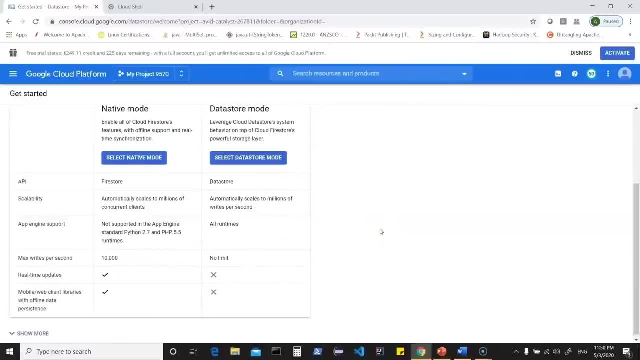 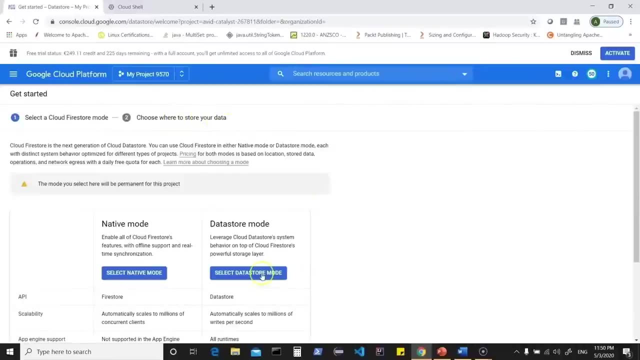 And here we look at the API or scalability engine support, how many rights it supports and so on. You can choose one of these and then you can choose where to store your data. So, for example, if I click on this one, then it choose- asks me to choose a location- So it says: 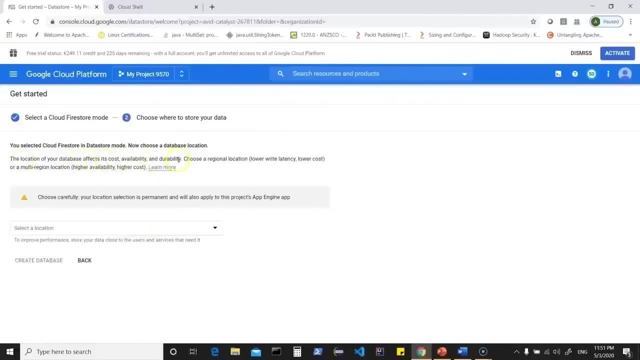 the location of your database effect its cost, availability and durability. choose a regional location, lower right latency, lower cost Or multi region location. here I can basically choose, for example, Europe, and then I can go ahead and create a database. So it says: initializing cloud fire store in data. 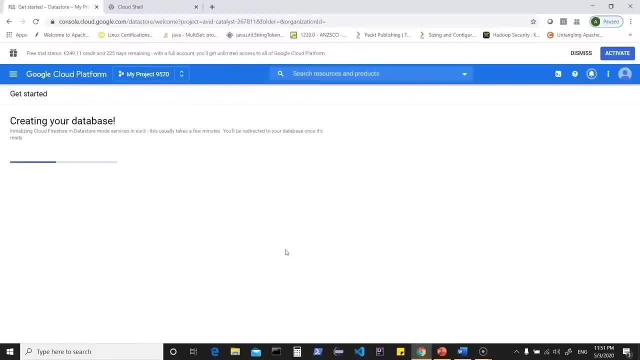 store mode services in EU three. This usually takes a few minutes. You'll be redirect to your database once it is ready. So if we compare the pricing structure between cloud data store and cloud big table, always remember cloud data store You pay for monthly. 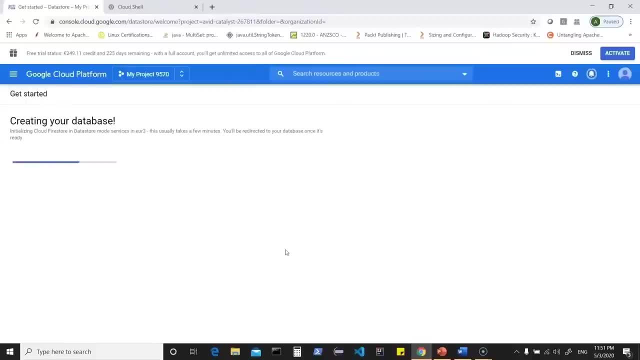 storage, which is also in the case of Bigtable. However, here you are paying for monthly storage for reads and writes, But in case of Bigtable you are paying for cluster when it is running. So cloud data store is a good option for small data, infrequent access and it acts cheaper. 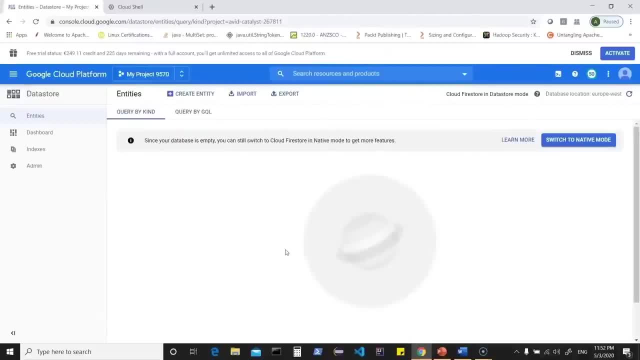 When you talk about large amount of data or big data and frequent access, then you are talking about cloud Bigtable, So Bigtable is cheaper. when you talk about larger amount of data, So here it says: since your database is empty, you can still switch to cloud fire. 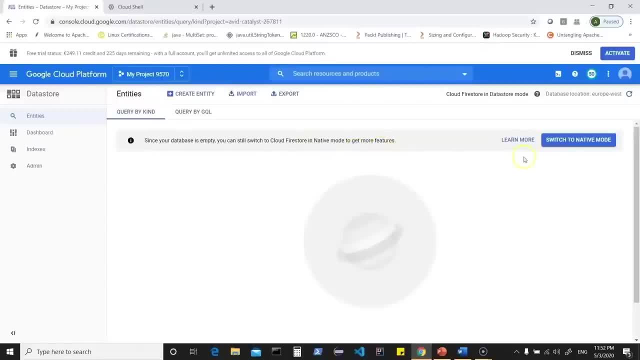 store in native mode to get more features. You could do that, You could learn, You could say: query by GQL. As of now, we don't have any data here. Let's look at the dashboard. It says: since your database is empty, you can still switch to cloud fire store in native. 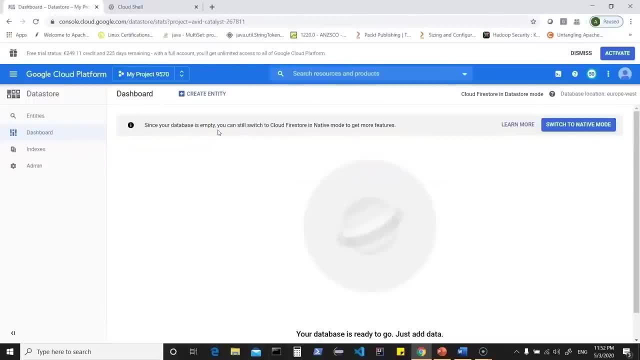 mode to get more features. So this is your cloud data store and it has many features which help you to work with your data. However, some features or important features of our DBMS were still missing, and that's where Google created yet another Bigtable based service called Cloud Spanner. Now we can continue. 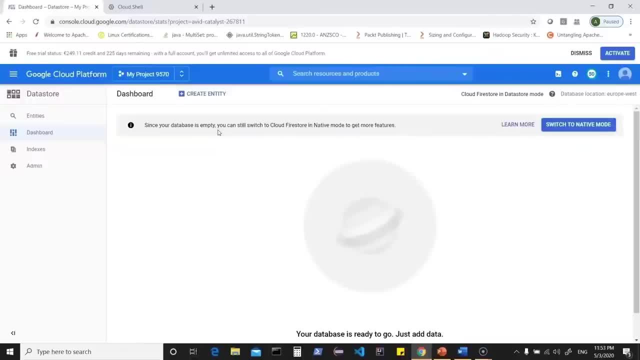 working on cloud data store, which basically gives you one option to work with your data. You can create an entity Here by clicking on create entity and that basically gives you options such as default namespace, You can give a kind, You can give numeric ID and you can start adding properties. 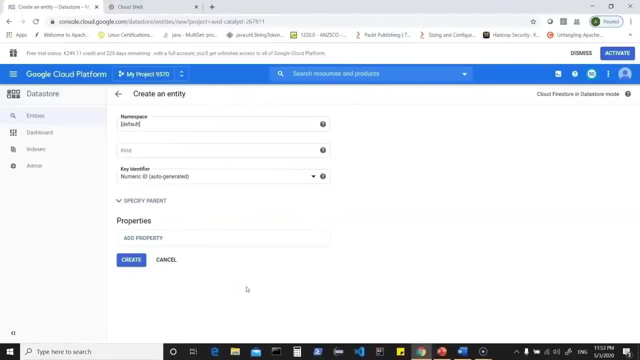 but to learn more about data store. we will learn about this in further sessions. So, as of now, I'm going to click on cancel, I'm going to go back to my data store and this basically Let's go to data store option, or I can go into admin here, which basically 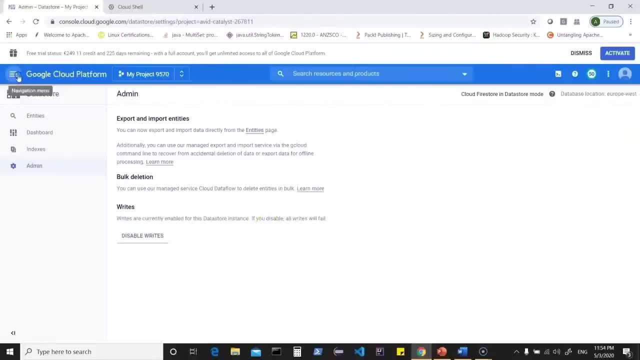 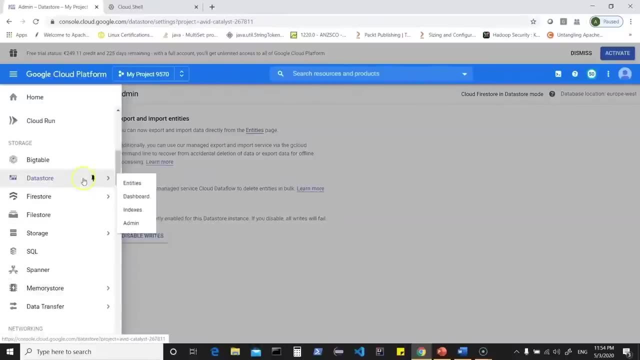 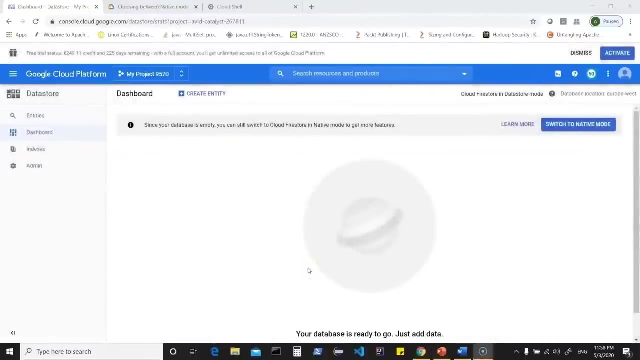 says: if you have entities, you can import or export them. so let's go back and let's again look into storage options. so, as of now we were in data store, let's click on this one. so, as i mentioned, your cloud data store, which basically gives you some additional features on top of your big table. 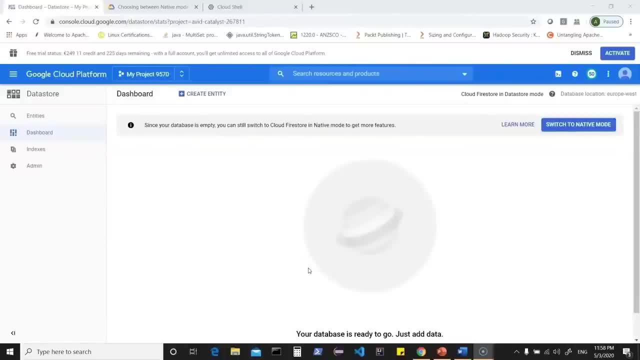 but what google also did was it realized that there was a need for rdbms feature support, that is, there were a lot of features. now, here we have created a data store and it says: your database is ready to go, just add data. you can create entity, start putting in data and then you can go ahead. 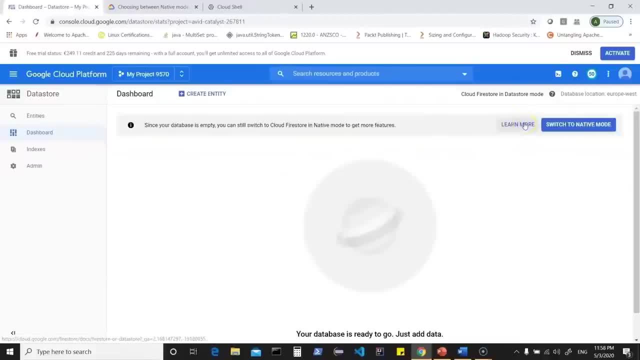 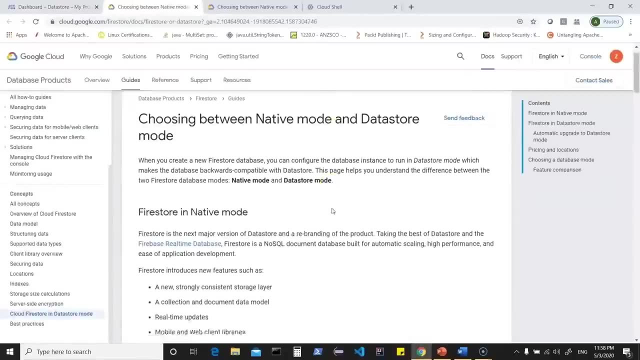 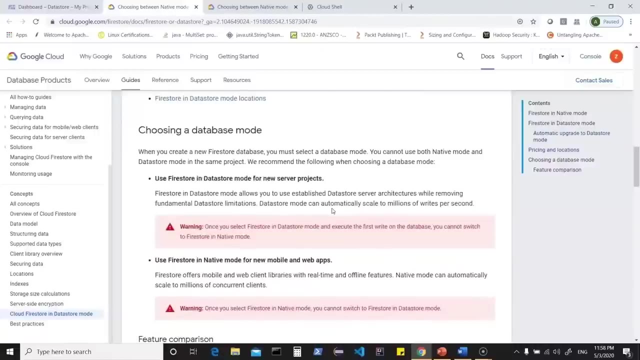 and query this. so if you would want to learn more about your data store, you can just click on this one, and that takes you to the complete documentation of native mode and data store mode. what is fire store in native mode? what is in data store mode? what are pricing and locations, how you choose a. 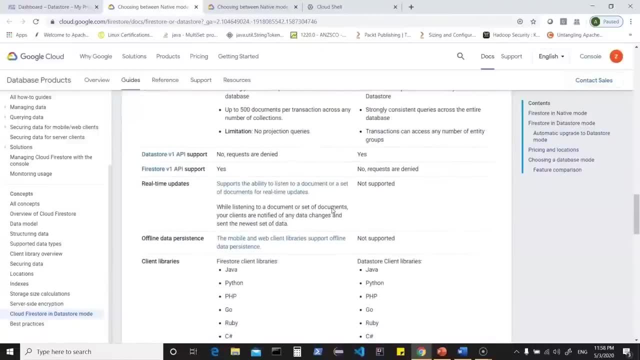 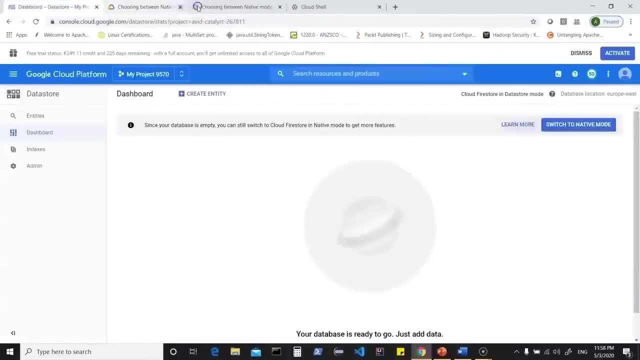 database mode and what are pricing and locations. and what are pricing and locations and what are mode, what are the feature comparisons, what you can do, what you are allowed to do here, what programming languages can be used, different regions, pricing and so on. as of now, we'll click. 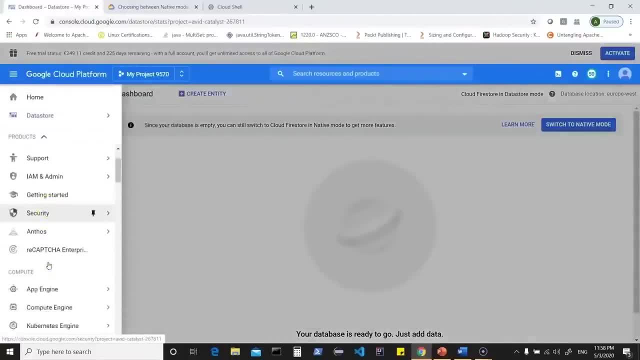 on this one and let's look at one advanced service which google cloud came up with when it comes to your additional features of rdbms. so google created yet another big table based service called cloud spanner. now that you might not see here, but if you scroll down you should. 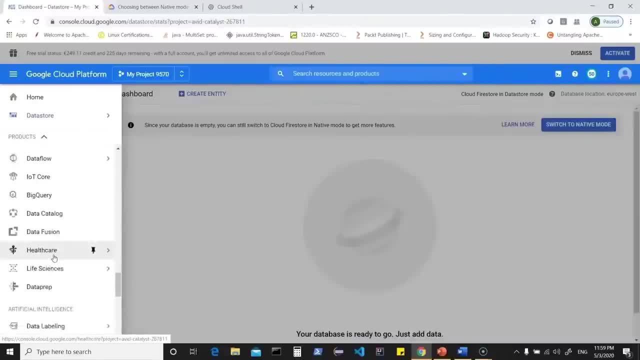 be able to see that you have a big table based service called cloud spanner. now that you might be able to see your cloud spanner in the options here, or did we miss it on the top, so let's again look here? yeah, so it is here and you can click on spanner. so cloud spanner was released in 2017. 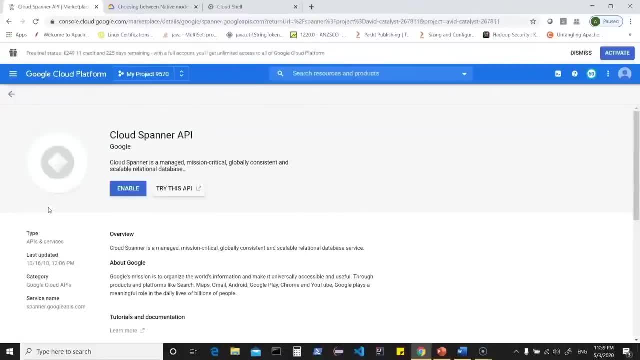 it basically supports relational schema, so it offers strong consistency for all queries which can be sql based. you can have multi-region deployment. now, when it comes to massive scalability requirement and strong consistency, cloud spanner is a good option. so it says cloud spanner is a managed mission critical globally. 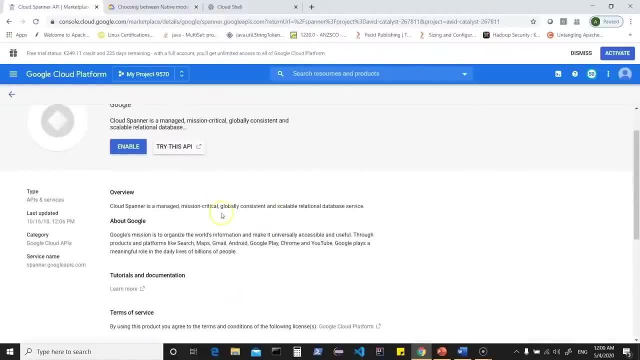 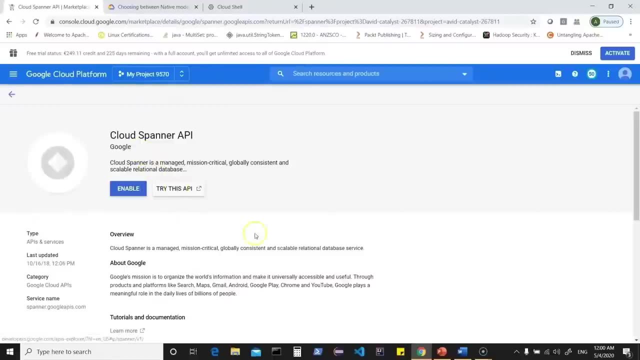 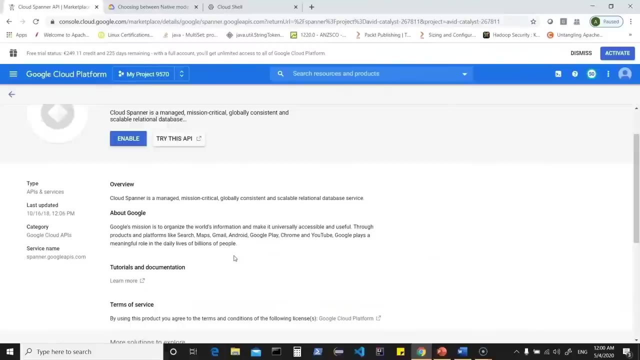 consistent and scalable relational database. so if you would want to use this, then you will have to enable this api, which shows you an option here. it says: try this api. so it's a managed service. so it is one of the google's most expensive database services. there is also one more. 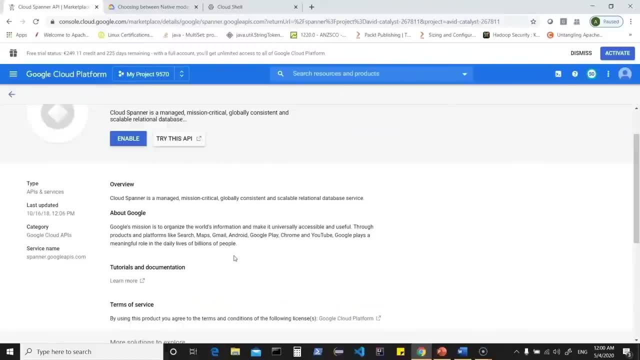 database service, which is cloud sql, which can be used, so it is one of the most expensive database. so when we talk about your cloud spanner, it is fully managed relational database service. it is massively distributed. you can have millions of machines across hundreds of data centers with support, automatic sharding and synchronous replication. it gives you low latency and schema. 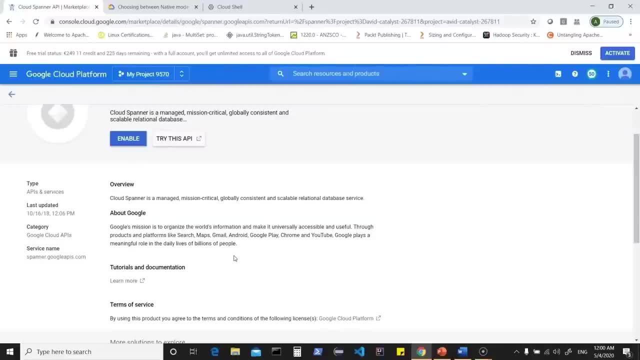 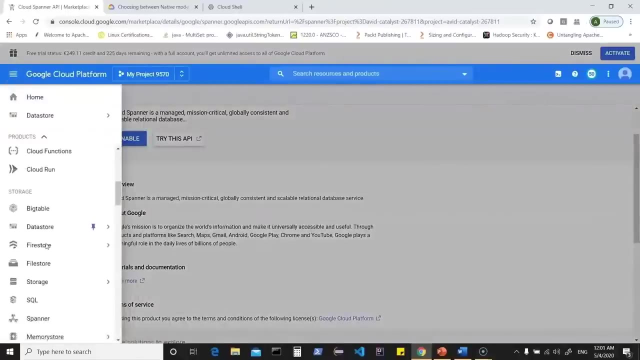 updates without downtime, making data high availability and reliability. so we learn about cloud spanner with more details later in other sessions. now we can also go back to storage and we can look at the different options which we have here. so you have object storage, you have spanner, you also have your sql based service, which is yet another. 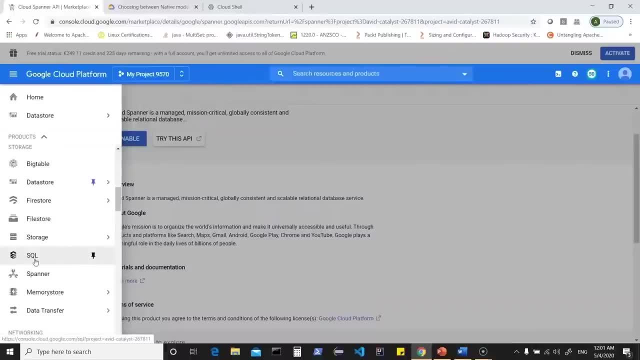 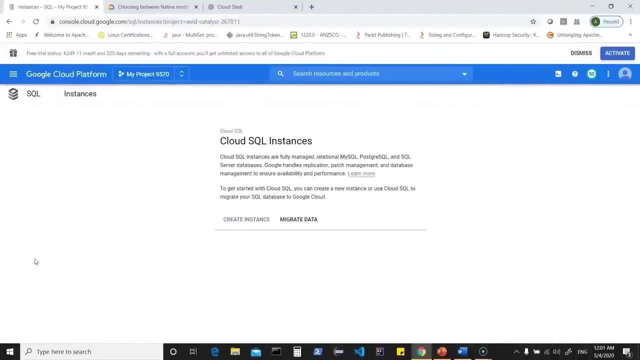 managed service offered by cloud- or google cloud, i would say. so that's called cloud sql. so this is basically a service which allows you to have fully managed relational mysql, postgres and sql server databases. so this is a service which allows you to have fully managed relational mysql, postgres and sql server databases. 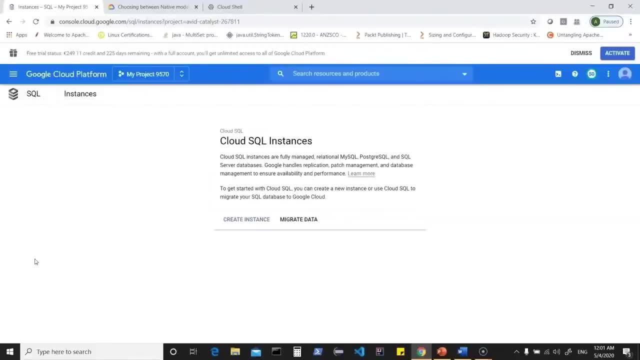 Google handles replication, patch management, database management and other things which are related to this managed or fully managed database service. It can allow you to handle terabytes of storage capacity with 40,000 IOPS, with huge amount of RAM, per instance, So you can click on create instance here and then you can choose one of the database which 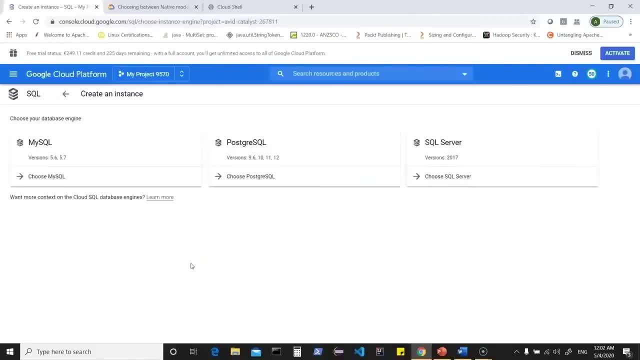 you would want to use. So Cloud SQL is a managed service. You can choose one of your MySQL or Postgres and SQL server. Say, for example, I choose MySQL. Now that basically tells me what is the instance ID. It sets up a password. 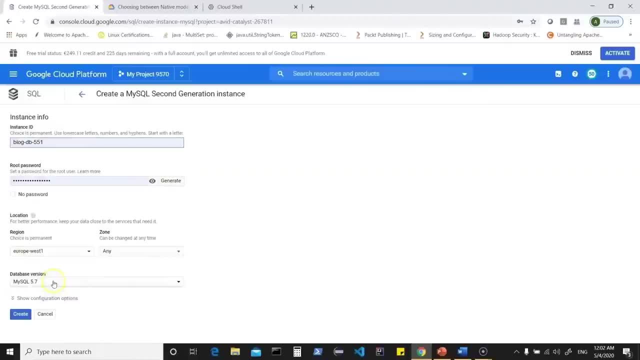 You can always change the password, You can change the region, You can choose your database version and then you can also look at other configuration options which talk about machine type which will be used. what is about your backup and recovery, maintenance And all that? 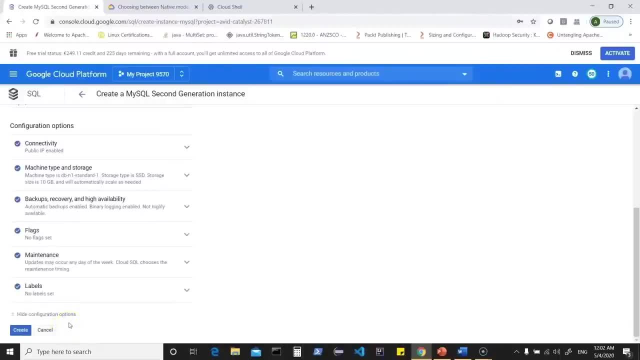 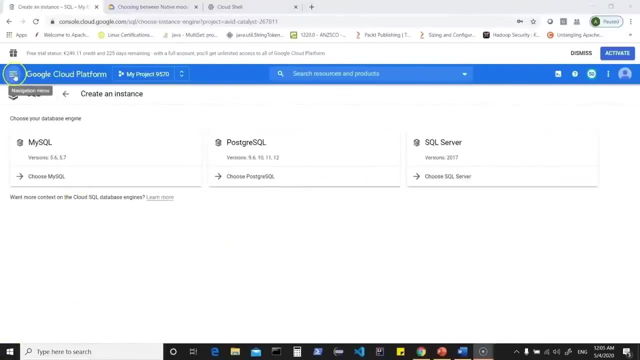 And if you click on create, this will basically create a fully managed SQL service which can allow you to straight away start using MySQL on cloud, thus allowing you to store your relational data. When we talk about storage options, how can we not talk about a data warehouse solution? 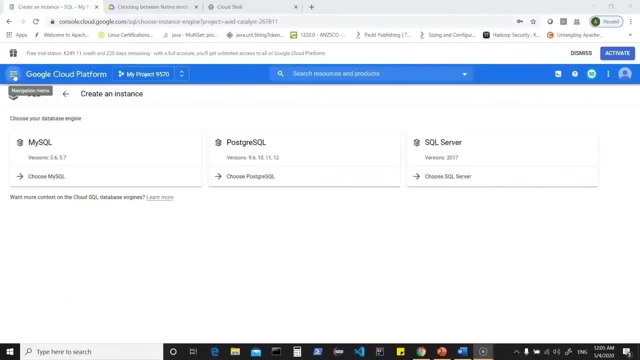 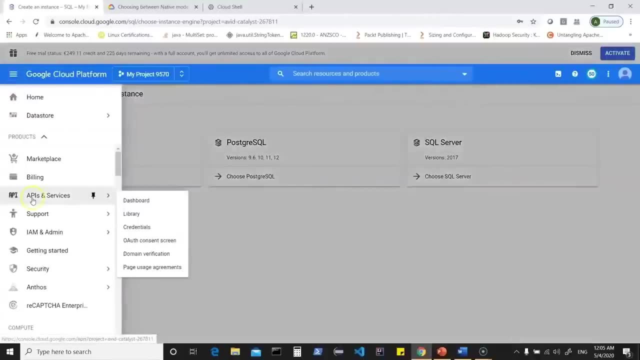 or basically an option which allows you to run your queries by directly updating data. So you can use a database, You can use a data warehouse service which Google Cloud Platform offers and that's called BigQuery. So basically, you can be looking into the big data section here and here you have an option. 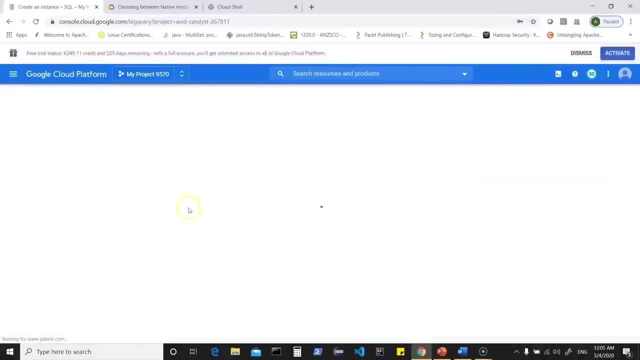 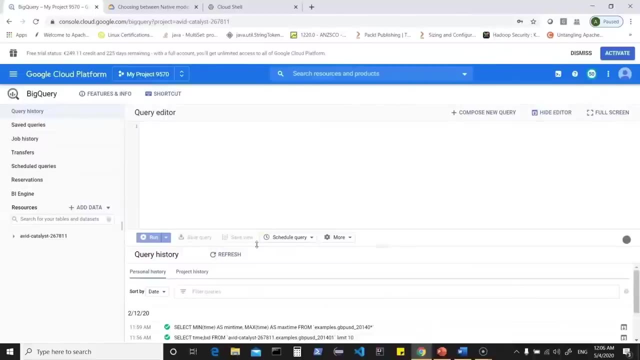 called BigQuery, So this basically brings ease of implementation and speed. So building your own data warehouse can be expensive, time consuming and difficult to scale. So with BigQuery you just load data and pay only for what you use. So You have features such as capability to process billions of rows in seconds. 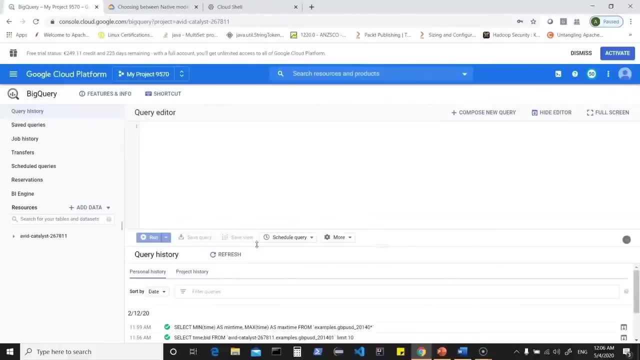 And if you would want to do real time analysis of streaming data, that is also possible here. So here we have clicked on BigQuery, which basically shows you the option where you can start typing your query and test your data access. For example, if I have uploaded some data, so it shows me there are some queries which 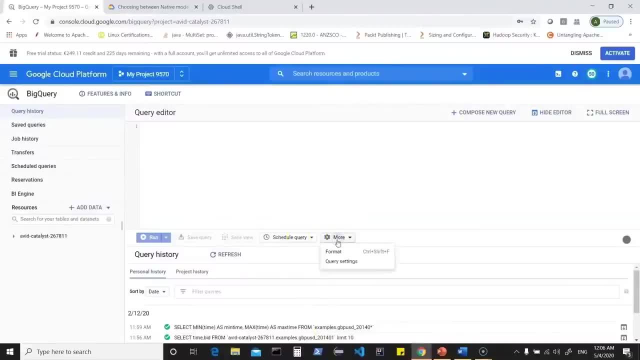 are saved here. Now I can schedule your query. I can basically choose the format of a particular query by clicking on this more. Here I have an option which says add data, so I can pin it to a particular project. I can explore public data sets. 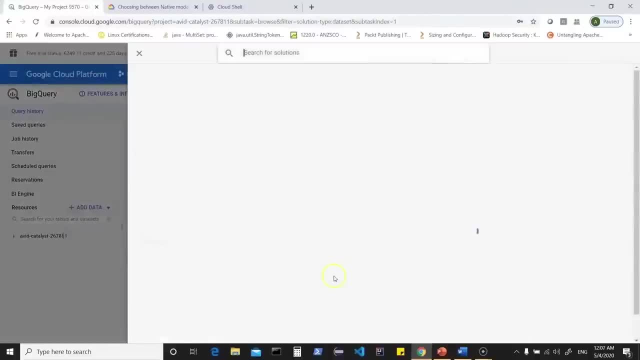 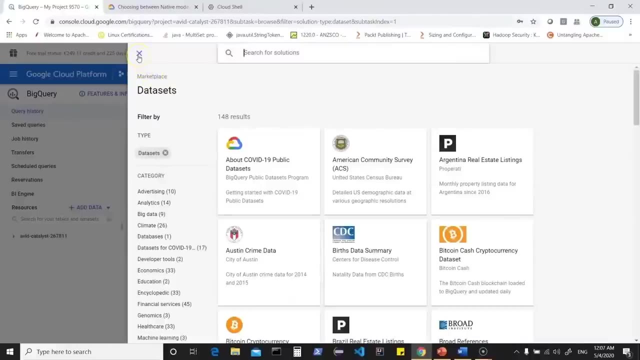 I can create a connection. So if I click on explore public data sets, then it takes me to a page from where you can get different kind of data sets which are already available, which you can put into your BigQuery and start querying your data. 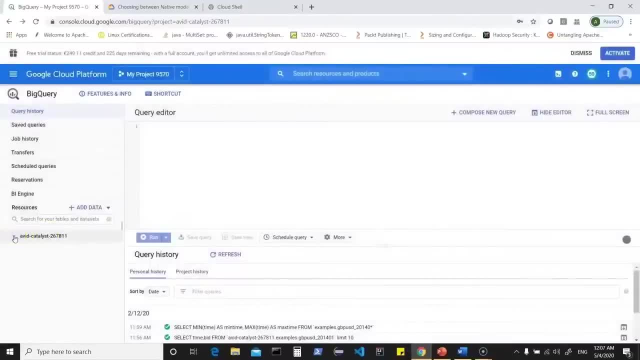 By default. It shows that it is aligned to my project and I don't need to worry about it. I can look at saved queries- if I have already saved a particular query. I can look at job history. I can look at transfers, scheduled queries and reservations. 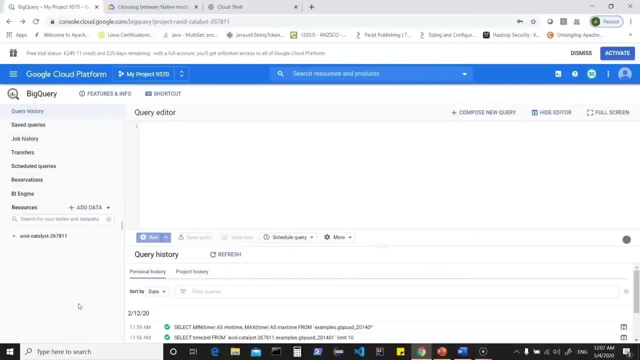 So BigQuery basically initially had its own version of SQL, which was slightly different from standard SQL, But in 2016, BigQuery 2 was released that supports SQL 2011 standard. You can always select standard SQL, Now BigQuery. when it comes to pricing, we need to remember that the storage costs is. 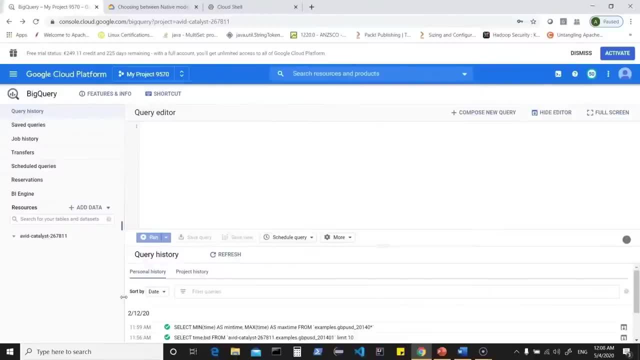 very less here, approximately 0.02 cents per GB per month. It is almost similar to Nearline, where you can also have low cost. that is, 0.01 cents per GB per month. There is no charge for reading data from storage. 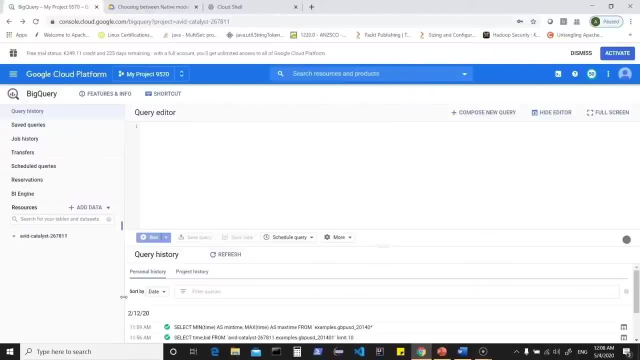 When it comes to querying, And that's where the cost is incurred. So one terabyte per month is free, and after that it costs few cents per GB. So this is mainly for high volume customers. There is a flat rate by pricing which can be used. 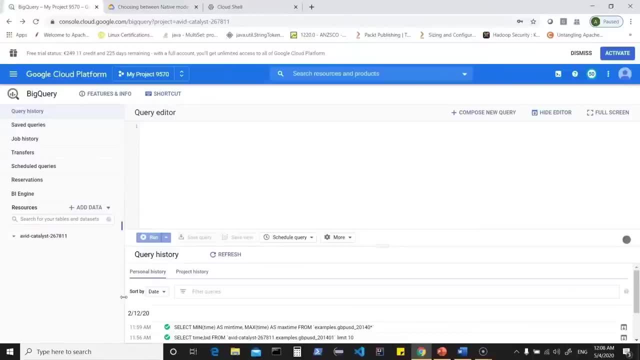 So when you talk about querying, you can save your query results. You can create data set to store the results. Now results are put in a temp table in cache and after you're done with that you can delete data set and delete all the data. 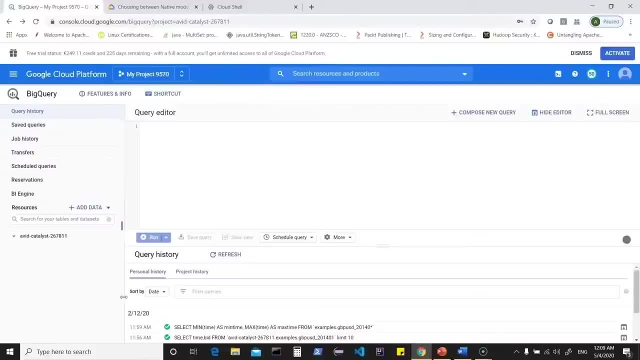 So, when you talk about loading data into BigQuery, you can get the data from cloud storage: Google Drive, cloud data store, stack driver, stack driver, other options. You have cloud big table or other web interfaces So you can download from URL such as CSV, JSON, Avro. 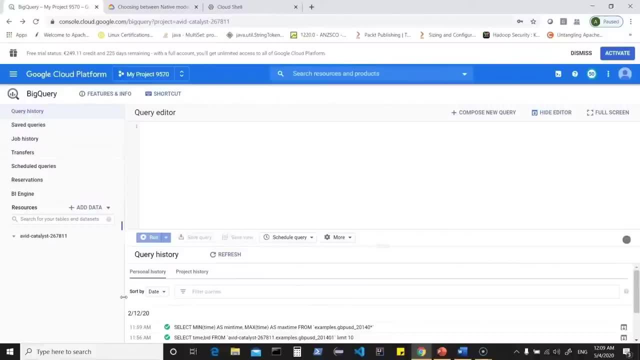 You can create data set, create table and create from source By doing a file upload, So 10 megabyte or less files can be uploaded using web interface. as an option, You can also use command line and then you can start working with your BigQuery. 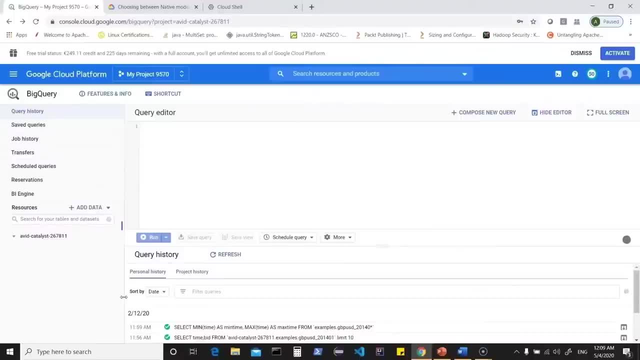 So here you can also work with streaming data by basically pushing in streaming data into your BigQuery, which allows you to add one record at a time. Now you could use something like cloud data Flow, which allows you to use a particular pipeline about cloud data flow. 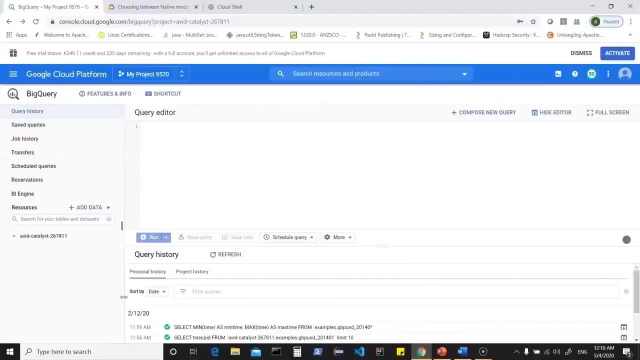 We will learn later, So you can benefit from different features of BigQuery and does use Google's offering to work on your structured data, or, I would say, data which suits well in data warehouses. Now, these are some of the storage related services which Google cloud offers, although 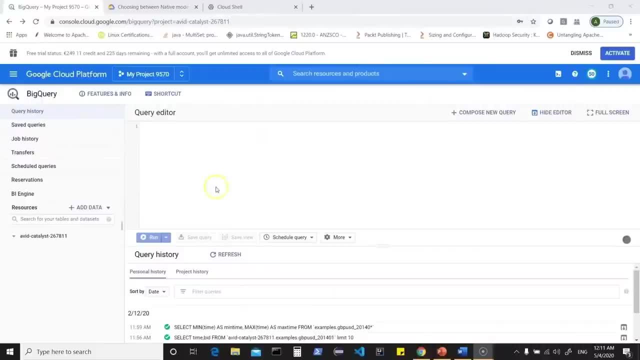 we will Learn about using BigQuery and running or uploading some data by creating add data set here, by, say, creating connection or using a public data set. So as of now I have this. You can also access the command line to work with this. but we will learn in detail about. 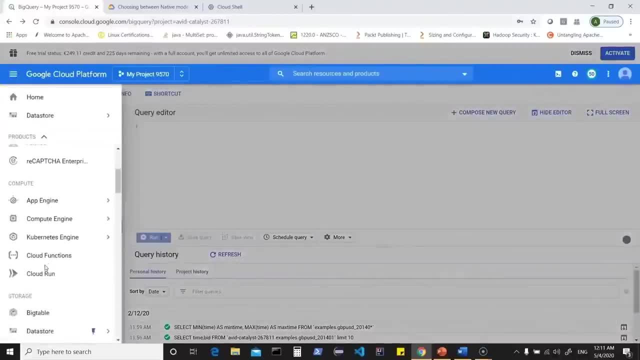 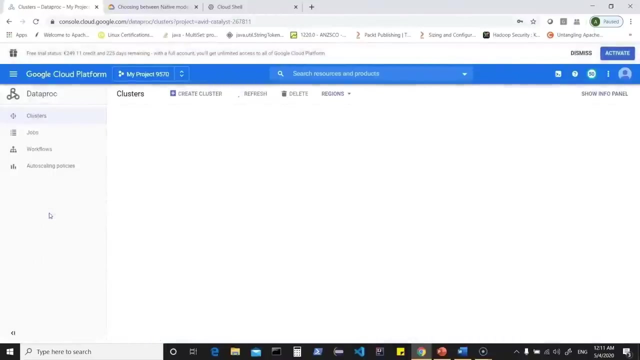 BigQuery in later sessions. Now here you can scroll down and you also have an option within big data space. I'm going to click on it And that is your data proc. So when you talk about data proc, this is again a managed service which allows you to run. 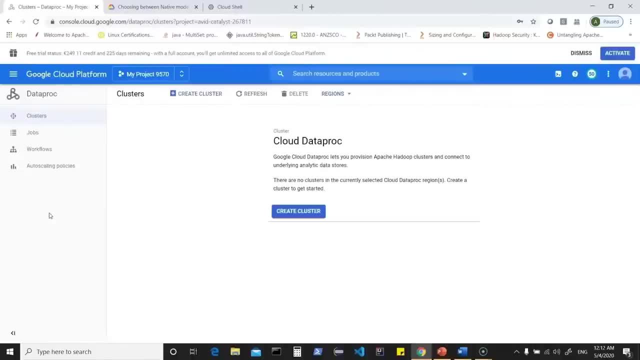 spark or Hadoop jobs, So especially if you are interested in big data workload. So for big data processing, for machine learning, you can always use cloud data proc. This uses compute engine instances under the hood but takes care of management of these instances. 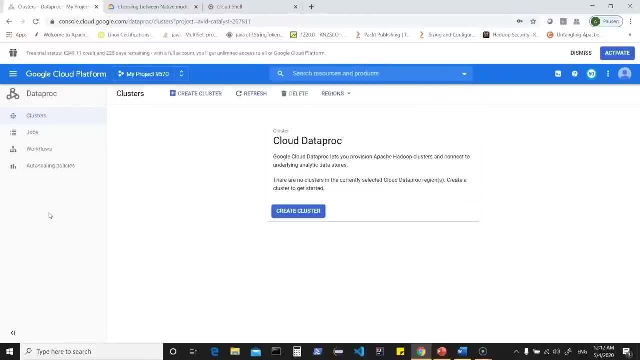 So it's a Top to spin up clusters. It's a managed service. It's cheaper Pay when the jobs are running. only It's fast because it is integrated with other Google cloud services. You have open source components pre-installed and data proc is integrated with yarn to make. 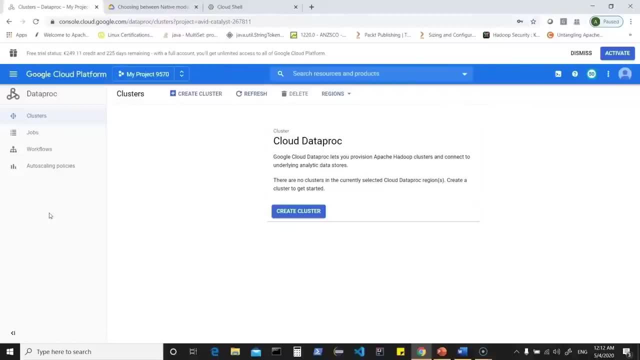 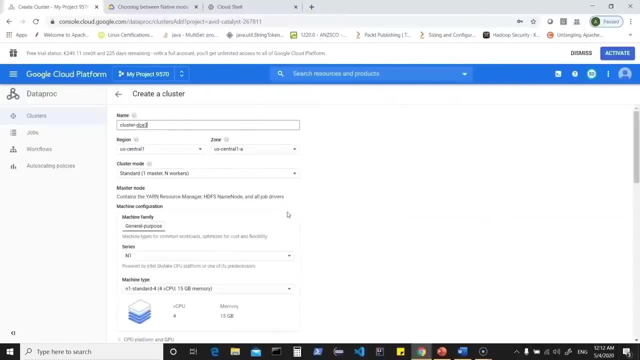 cluster management easier When you talk about data proc. you can click on create cluster and that basically allows you to set up your cluster by choosing a particular Region which you would want to use. For example, I'll choose Europe West for here. 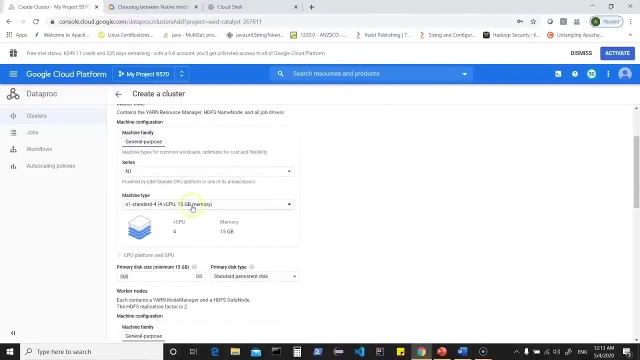 It tells what kind of machines you would want to use And by default it has populated as the machine here, which is for CPU and 15 gigabyte. Now, since you might be using a free account, let's not go for the high end machine. 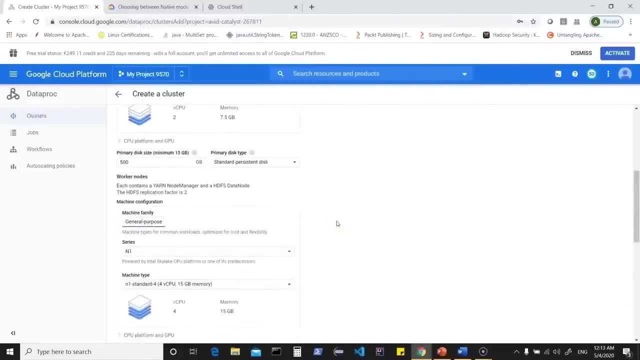 Let's go for N one, standard two, and then you can scroll down. It says what is the primary disk, What is the disk type, And this one was for your master machine, That is, machine Which will have the master processes running. Then you have your worker node configuration which tells: 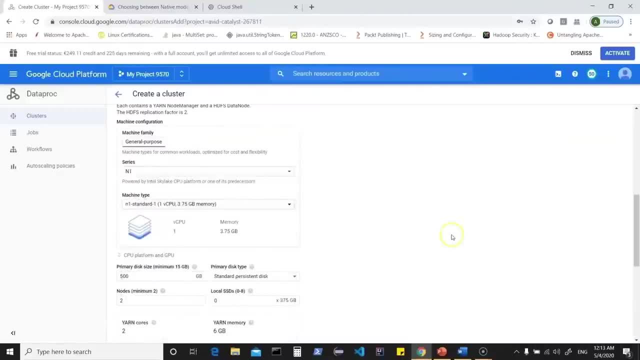 This will be. let's choose a lower end machine and we can choose how many worker nodes you would have. So it says minimum two. You can choose the SSDs and their capacity. It talks about yarn cores and yarn memory which will be allocated. 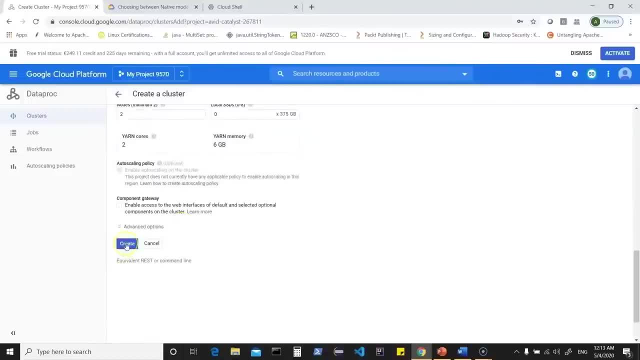 And here we have then option of clicking on create. So once you click on create, This will basically spin up a cluster wherein you can straight away start submitting jobs to this. You can basically go ahead. Once your cluster is ready, you can go into the cluster. 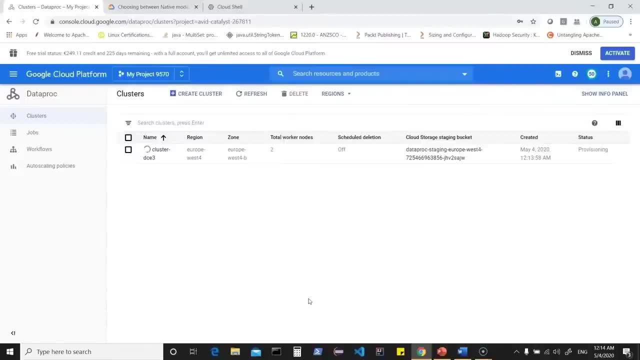 You can submit a job, You can choose a type, which is spark or any other application which you would want to run, And then, basically, you can use this fully managed service which allows you to run your big data clusters. You can obviously control. 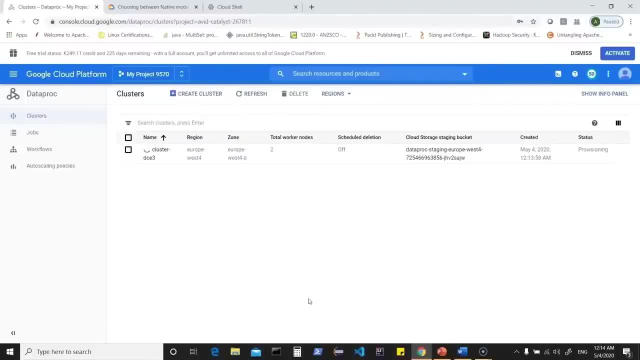 Access. we are roles or access control list and you can have access as it is, at project level or based on your data proc cluster or even at your worker nodes. So we'll learn about data proc in later sessions. So as of now, you see here, the cluster is getting created. 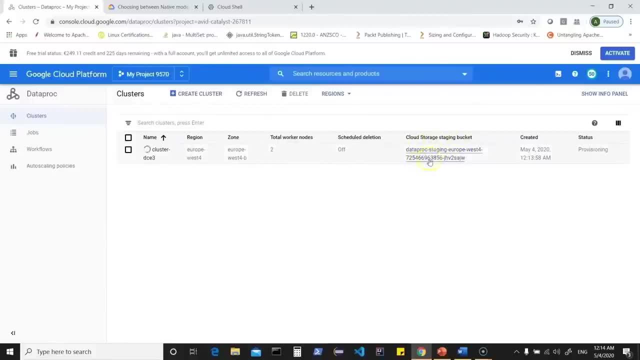 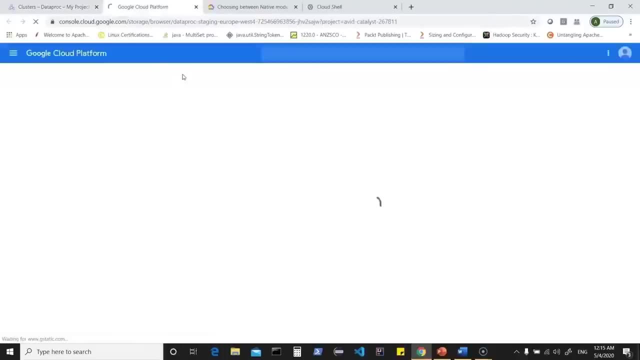 It says the cloud storage bucket which it is using is this one. Now I can click on this and open link in a new tab. It still takes me into console, but now it is showing me the bucket which is being used by your data proc cluster. 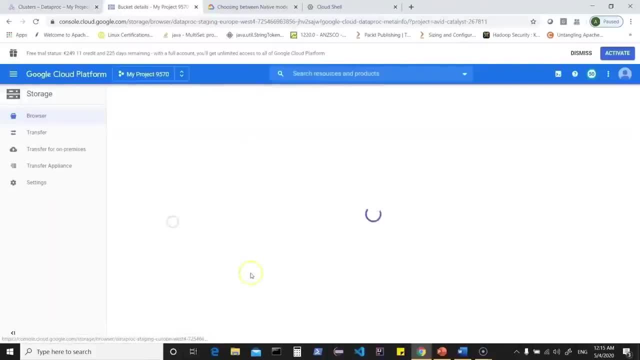 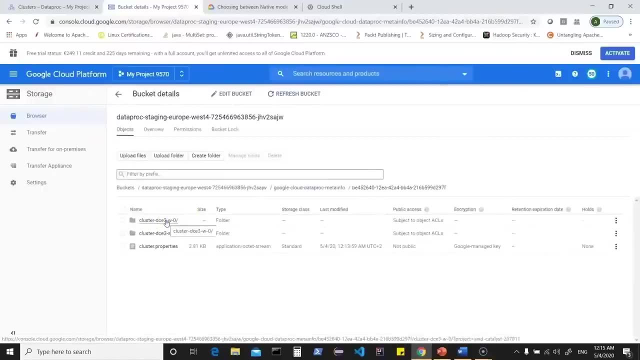 This is the bucket which is being used, and it is being used for an underlying metadata which gets stored here. So you look at the cluster related folders, You can click in these folders and then it gets see what is the script output, what it is doing, and so on. 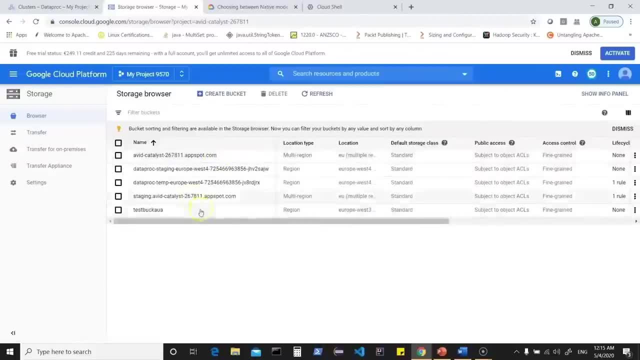 Now I can come back here to my bucket, Which will basically show me what kind of buckets have been created. So you see, data proc service automatically created some buckets which will be holding some data. You also have some other buckets which were created based on other services which we used. 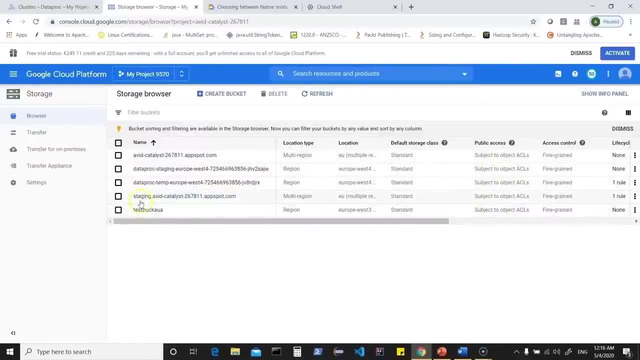 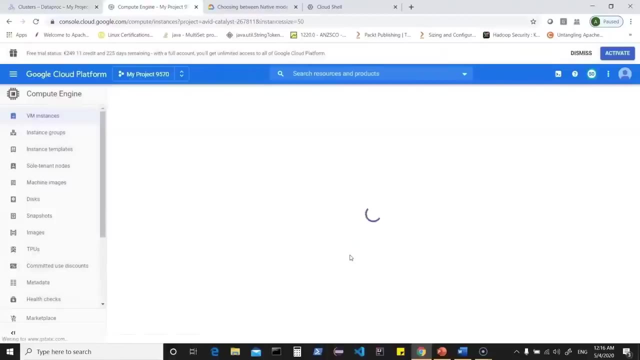 The access control is fine grained in all cases. plus, it also shows our bucket. So underlying it is using compute instances. It is basically using: let's go here And let's go to compute instances And let's look in to VM instances. 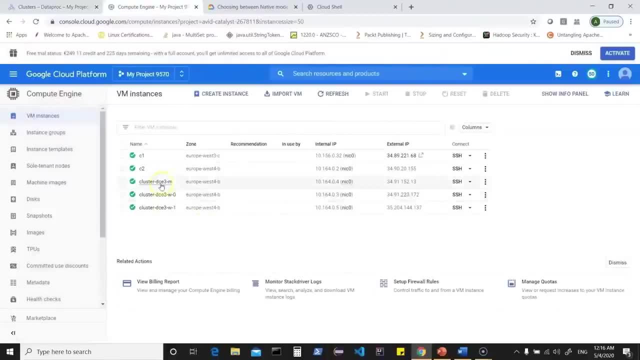 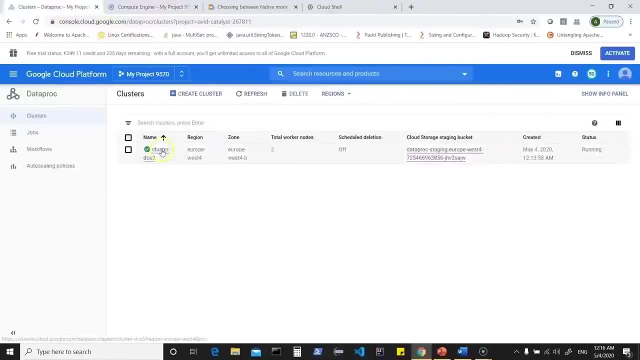 So data proc, which has spun up a cluster, is also using the VM instances which we see here are running. It is using the buckets and it has made a cluster ready to use. So you can click on this cluster and that shows me my cluster related details. 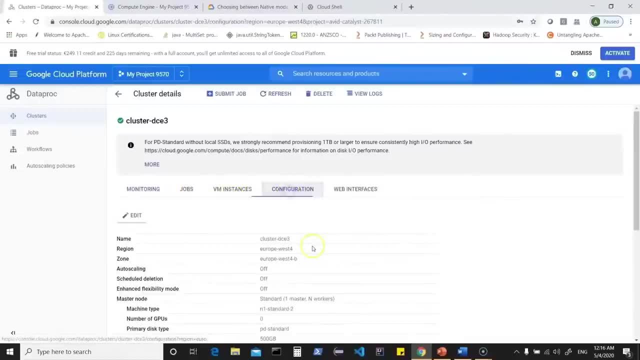 If there are any jobs running, what are VM instances, what kind of configurations it has used and you can look at different details here. You can look at the logs, You can click on jobs and that will show you if you have basically run a job on this ready. 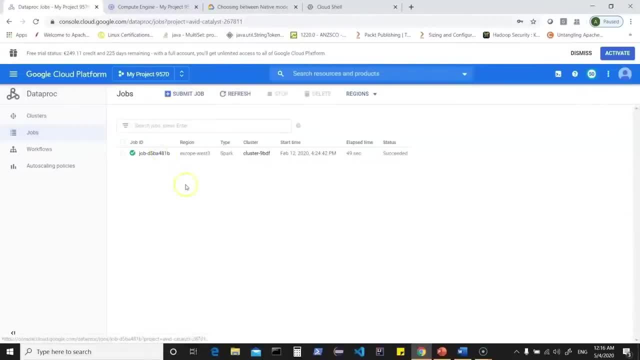 to use cluster. So it says there is this particular job which was run, which was a spark job. You can click on submit and this one tells you what is the job ID, what is the region you would choose, For example. we will again choose, for example, Europe West 4.. 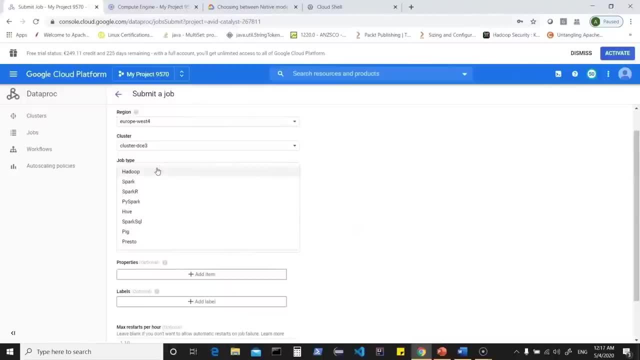 It tells what is the job type, So you can run all these type of jobs in this cluster, Such as Hadoop, Spark, PySpark, Hive Pig, Presto. You can give your jar file, So if you have packaged your application as a jar, you can mention that here. 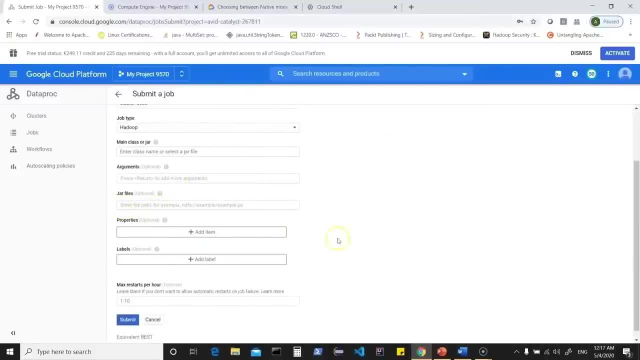 You can pass in some arguments. You can also say some other jar files, add some properties and then click on submit, which will run your job on this. ready to use cluster? Now, since we have tested it, I can basically go ahead and do a delete. 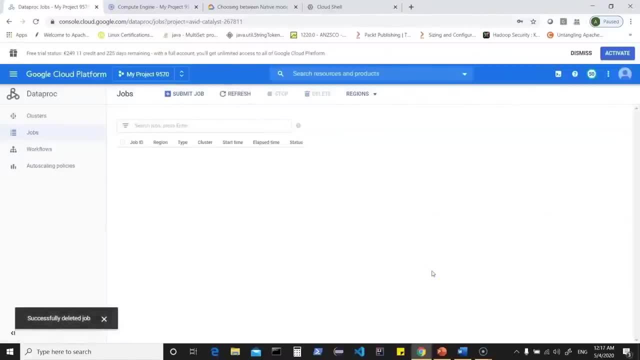 I don't want to incur any cost on these managed services which are running. So there are a lot more information about using these services which Google Cloud Platform offers, and we can continue learning about these services as we explore your Google Cloud console or even your command line option. 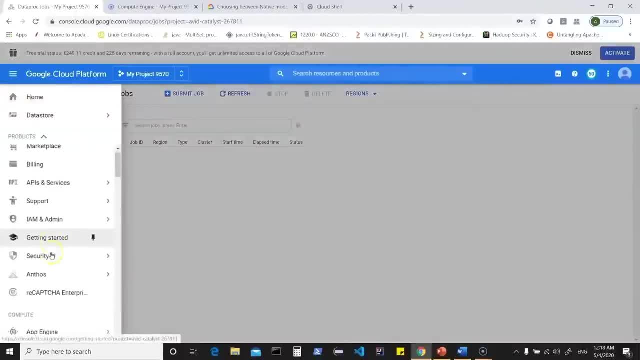 Now we can come out of this one by clicking on this menu, and then we have other options, such as Kubernetes. You have cloud functions. You have your networking related services. You have monitoring related services, Different kind of tools, what you have. You have other big data specific services which you can learn about. 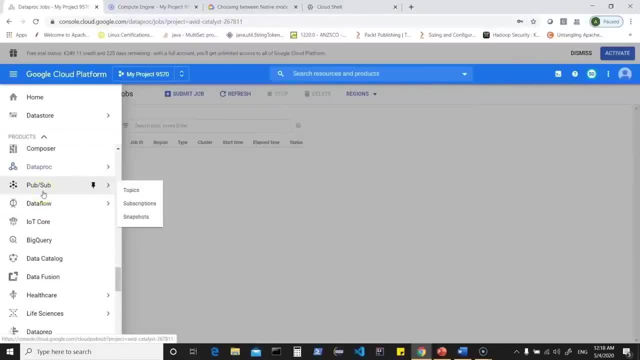 And for each of these services, Google has a very good documentation available. For example, when you talk about publish, subscribe messaging system, it is a real time managed service which basically is a pioneer, which was used, and now you have a famous service such as Kafka, which is being used for your cloud. 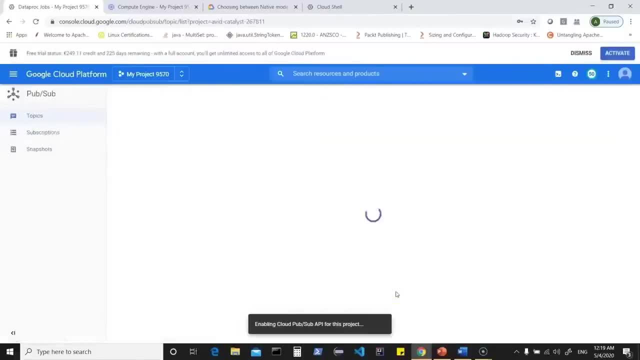 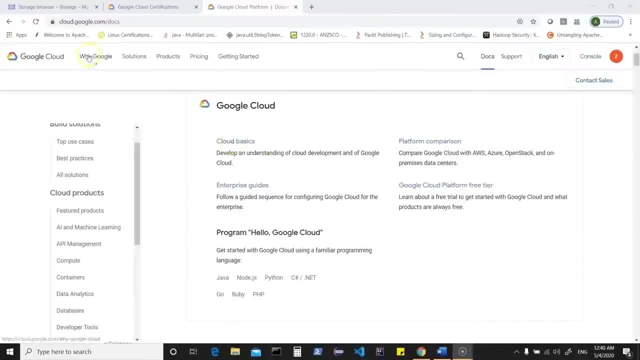 Publish, subscribing or messaging system kind of requirements. So to conclude about Google Cloud Platform services, you can always go to cloudgooglecom and look into the document section. Now, here you have list of different featured products. You also have list of your different domains and services which Google Cloud offers, and 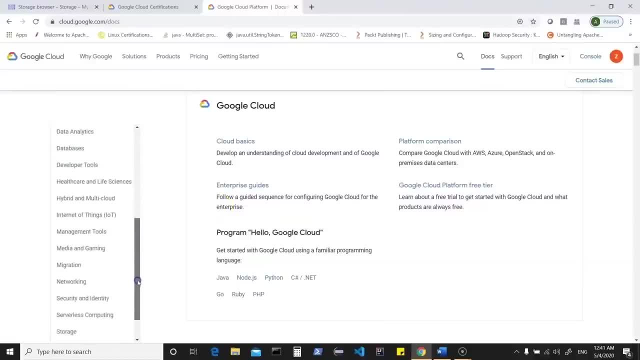 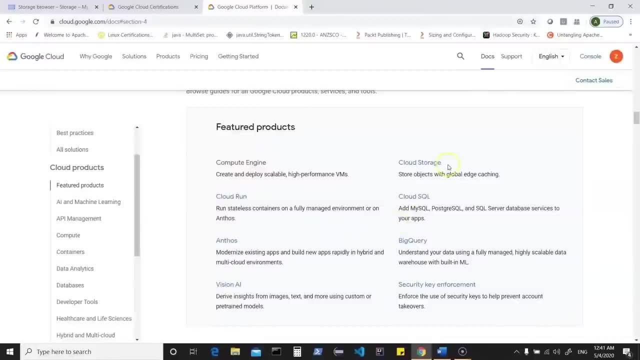 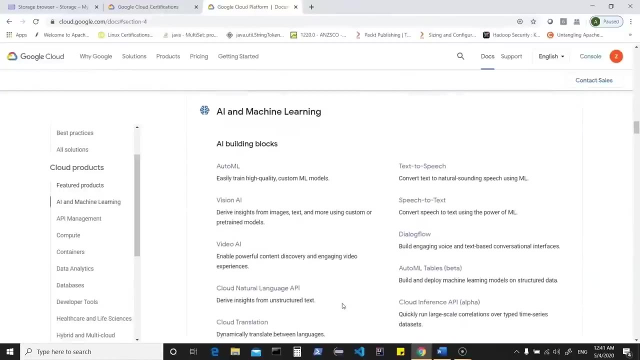 you can learn about all the different services which are offered by Google Cloud. Here you can click on featured products and that basically shows you compute engine. cloud run, cloud storage. You have cloud SQL, BigQuery, Vision, AI. You can scroll down and look at your artificial intelligence and machine learning related. 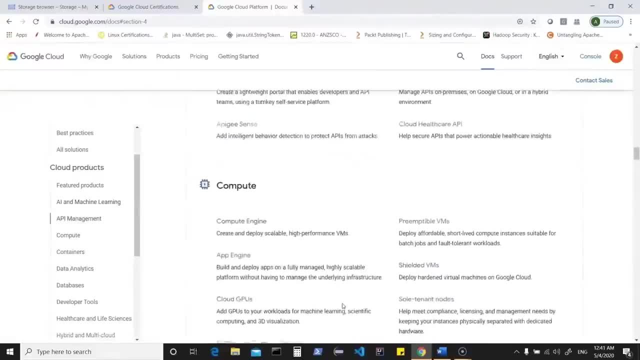 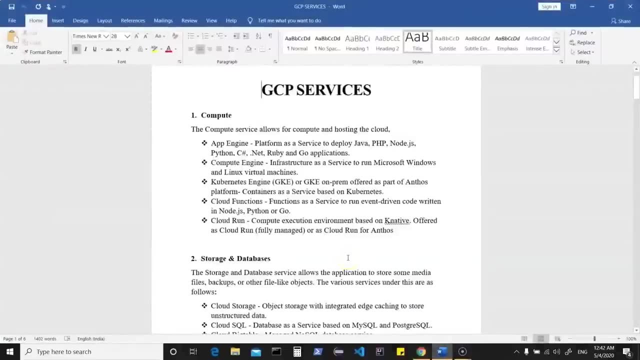 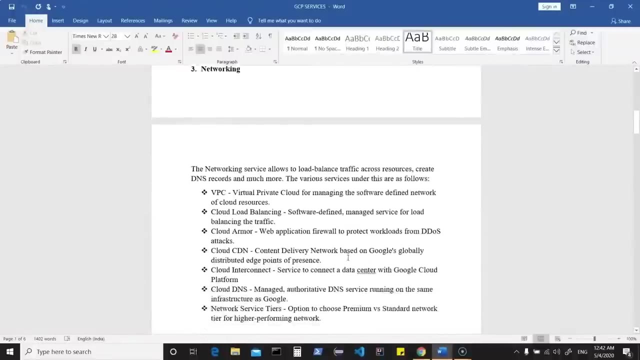 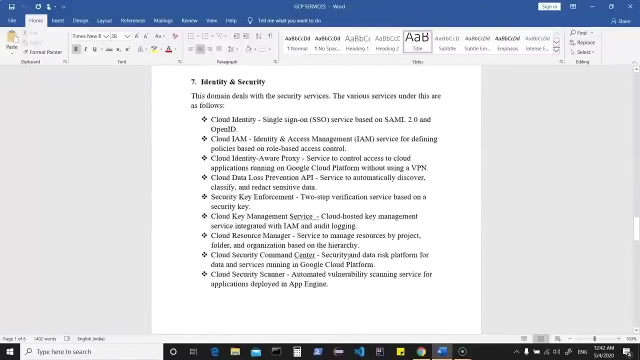 services platform and accelerators, API management. So Google Cloud Platform offers different services. in mainly in your compute storage and databases. You have networking related services, big data, specifics, developer tools, cloud AI, identity and security, IoT management tools, API platform and so on. 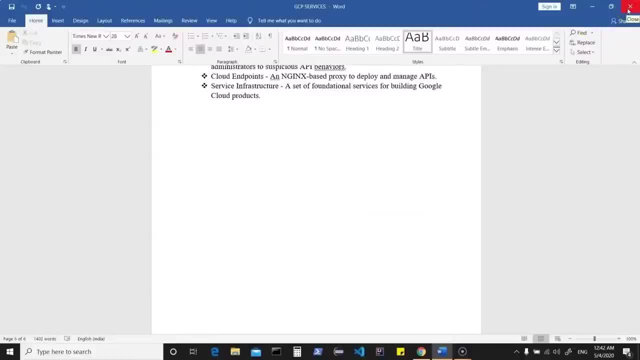 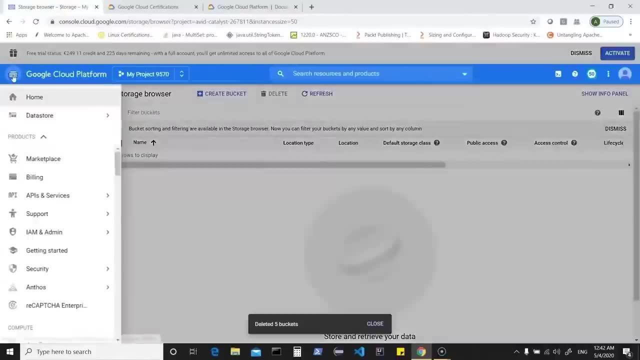 So basically learn about the GCP services which Google Cloud Platform offers, and in detail. you can play around with different services which are offered by creating a free account And, as I demonstrated in the previous video, you can play around with different services which are offered by Google Cloud Platform. 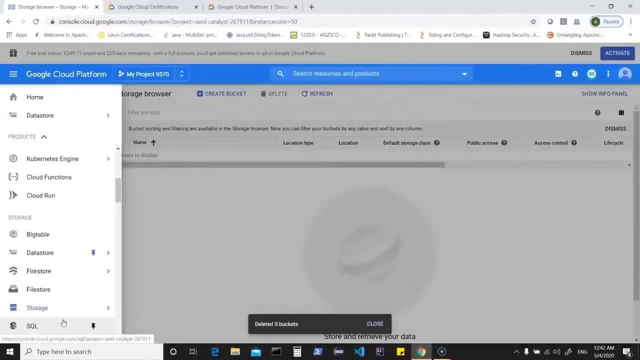 You can use any one of these services quick: start them, basically connect to them, put in your data, or use a managed service to manage your data and benefit from Google Cloud Platform, thus having modernized infrastructure for your different use cases. Hi guys, today we've got something very special in store for you. 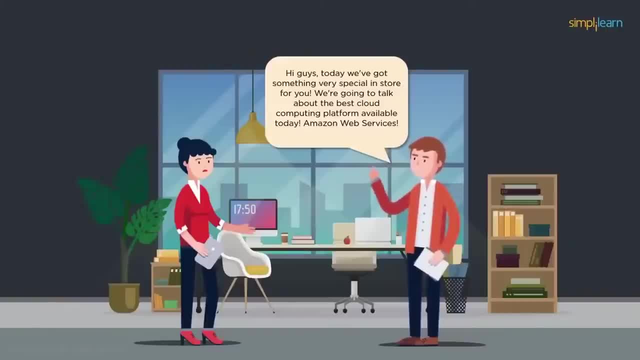 We're going to talk about the best cloud computing platform available: Amazon Web Services. Uh, Rahul, Rahul, I think you said something wrong here. The best cloud computing platform is obviously Google Cloud Platform. No, it isn't. AWS has more than 100 services that span a variety of domains. 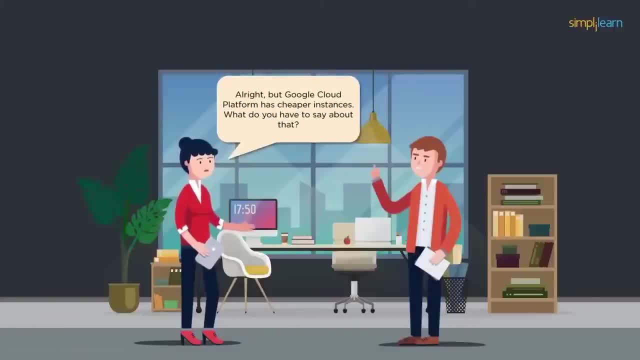 Alright, but Google Cloud Platform has cheaper instances. What do you have to say about that? Well, I guess there's only one place we can actually discuss this: A boxing ring. So, guys, I'm Apeksha and I will be Google Cloud Platform. 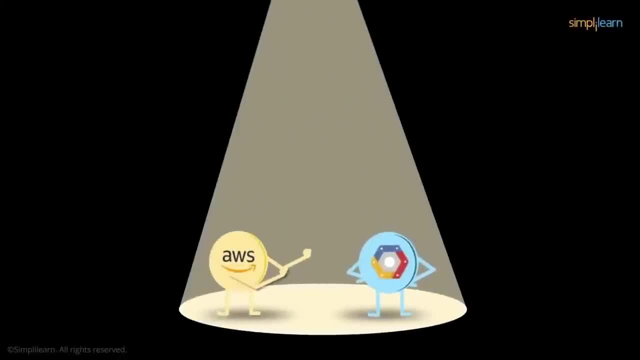 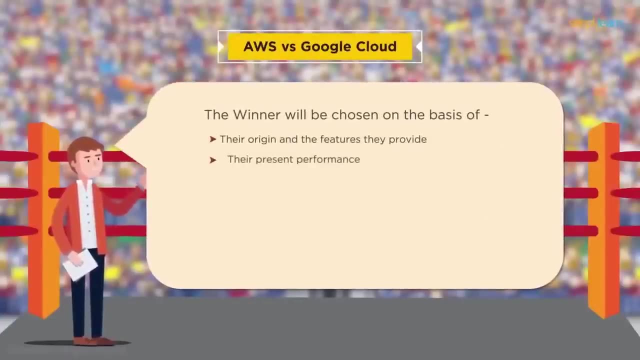 And I'm Rahul. I'll be AWS, So welcome to Fight Night. This is AWS vs GCP. The winner will be chosen on the basis of their origin and the features they provide, their performance in the present day and comparing them on the basis of pricing. 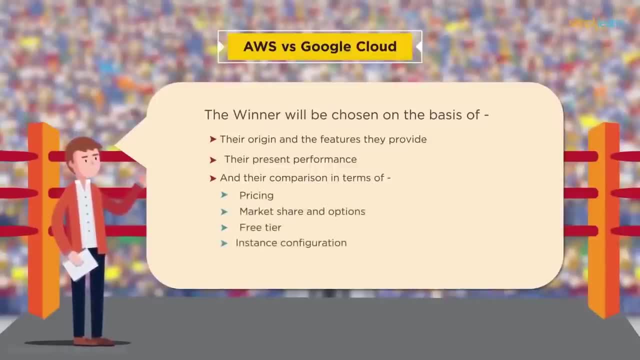 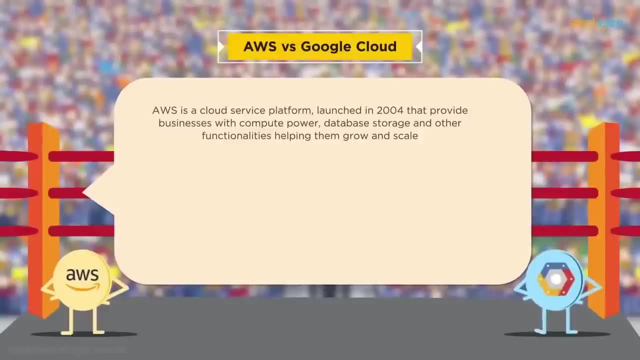 market share and options- the things they give you for free- and instance configuration. Now, first let's talk about AWS. AWS was launched in 2004 and is a cloud service platform that helps businesses grow and scale by providing them services in a number of different domains. 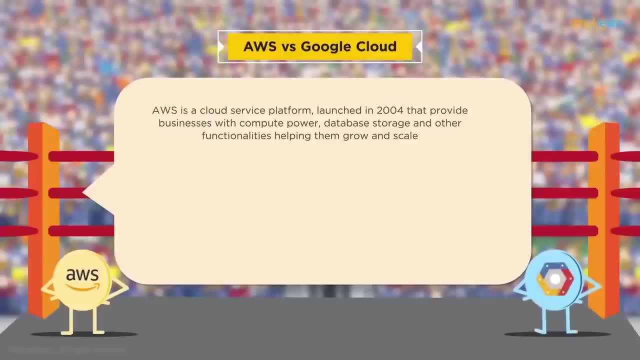 These domains include compute, database storage, migration, networking and so on. A very important aspect about AWS is its years of experience. Now AWS has been in the market a lot longer than any other cloud service platform, which means they know how businesses work and how they can contribute to the business growing. 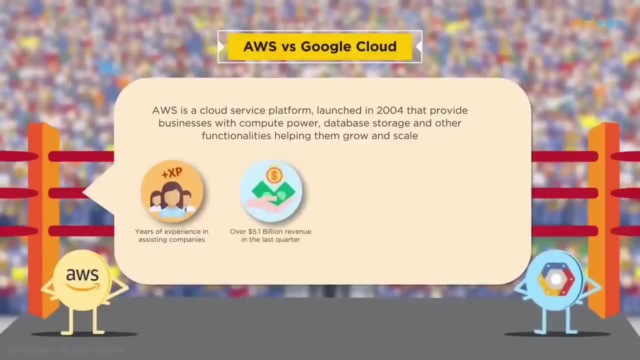 Also, AWS has over $5.1 billion of revenue in the last quarter. This is a clear indication of how much faith and trust people have in AWS. They occupy more than 40% of the market, which is a significant chunk of the cloud computing market. 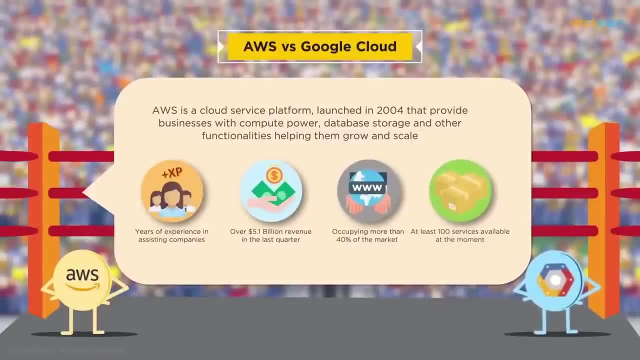 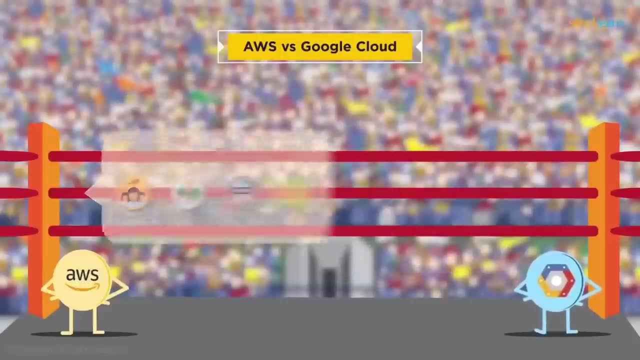 They have at least 100 services that are available at the moment, which means just about every issue that you have can be solved with an AWS service. Now, that was great, but now can we talk about GCP. I hope you know that GCP was launched very recently, in 2011, and it is already helping. 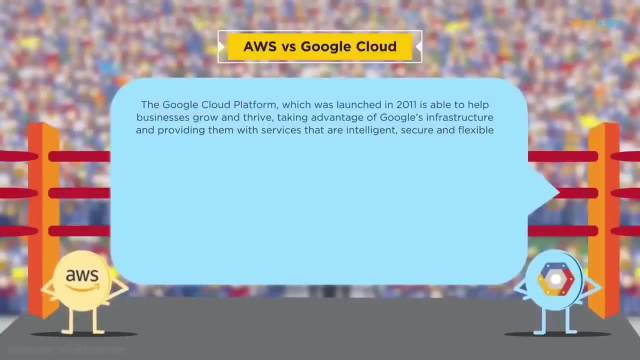 businesses significantly with a suite of intelligent, secure and flexible cloud computing services. It lets you build, deploy and scale applications, websites, services on the same infrastructure as Google. The intuitive user experience that GCP provides with dashboards, wizards, is way better in. 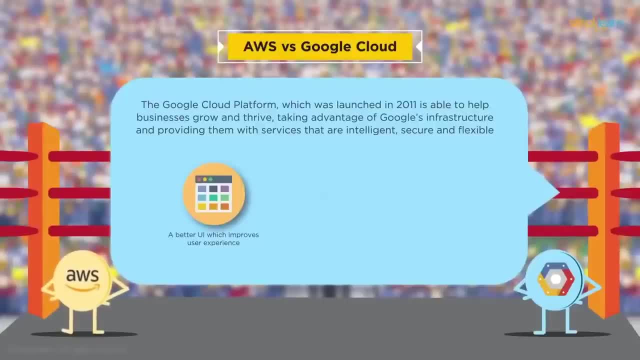 all the aspects. GCP has just stepped in. It is already offering a modest number of services and the number is rapidly increasing. And the cost for a CPU instance or regional storage that GCP provides is a whole lot cheaper, And you also get a multi-regional cloud storage. 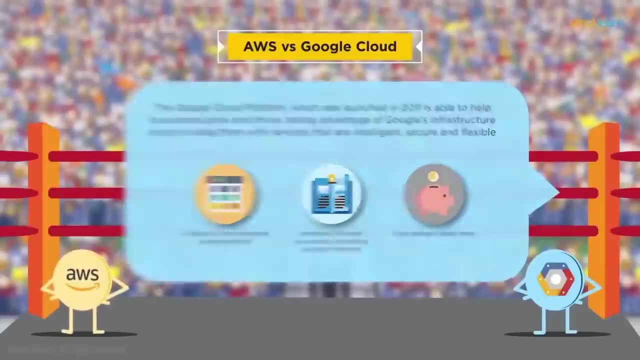 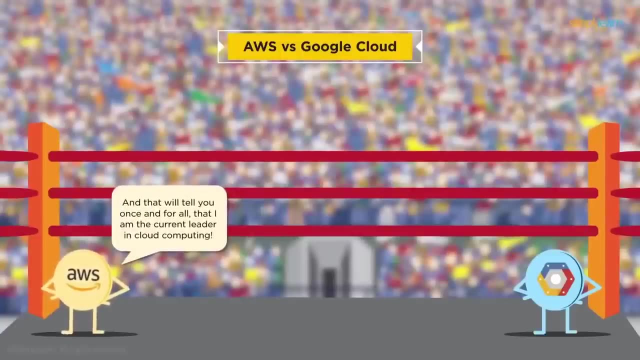 Now, what do you have to say on that? I'm so glad you asked. Let's look at present day, In fact, let's look at the cloud market share of the fourth quarter of 2017.. This will tell you once and for all that AWS is the leader when it comes to cloud computing. 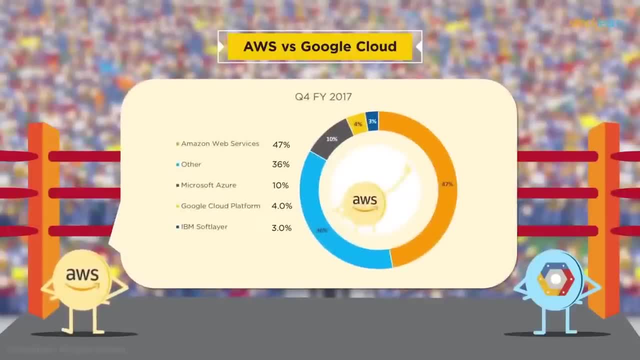 Amazon Web Services contributes 47% of the market share. Others like Rackspace or Verizon Cloud contribute 36%. Microsoft Azure contributes 10%, The Google Cloud Platform contributes 4% And IBM Software contributes 3%. 47% of the market share is contributed by AWS. 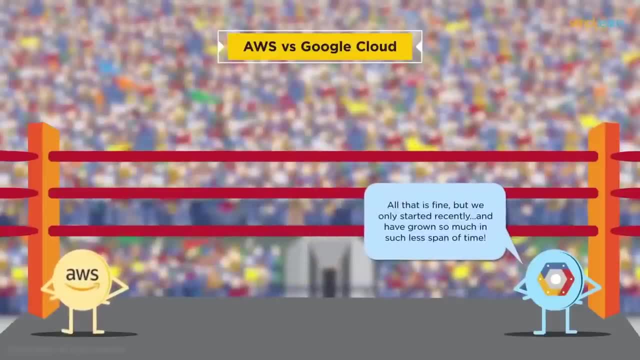 You need me to convince you any more. Wait, wait, wait. All that is fine, But we only started a few years back and have already grown so much in such a less span of time. Haven't you heard the latest news? Our revenue is already a billion dollars per quarter. 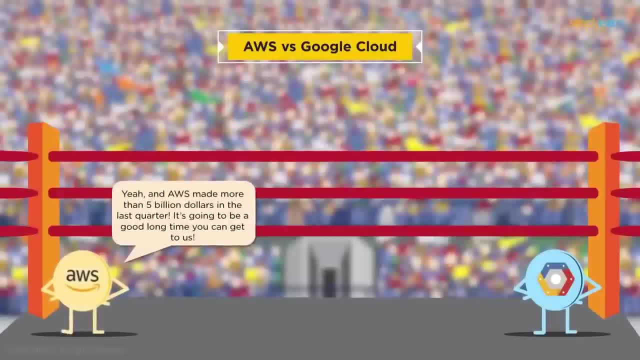 Wait for a few more years And the world shall see. And AWS makes 5.3 billion dollars per quarter. It's going to take a good long time before you can even get close to us. Yes, yes, We'll see. 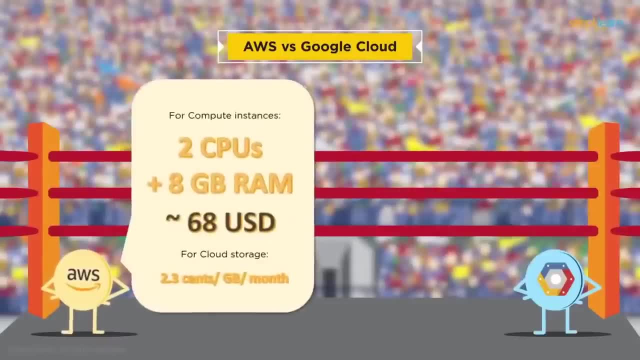 Now let's compare a few things. For starters, let's compare prices. For AWS, a compute instance of two CPUs and 8GB RAM costs approximately 68 US dollars. Now, a compute instance is a virtual machine in which you can specify what operating system 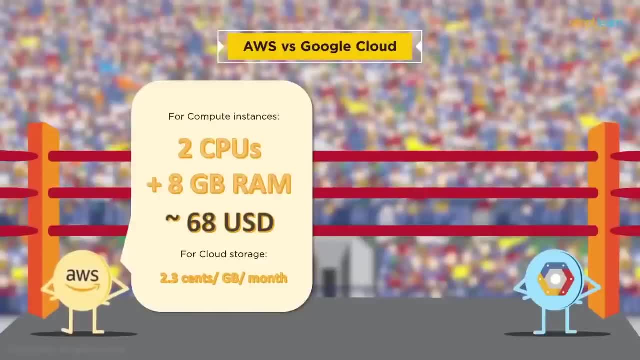 RAM or storage you want to have For cloud storage. it costs 2.3 cents per GB per month with AWS. You really want to do that Because GCP wins this hands down. Let's take the same compute instance of two CPUs with 8GB RAM. 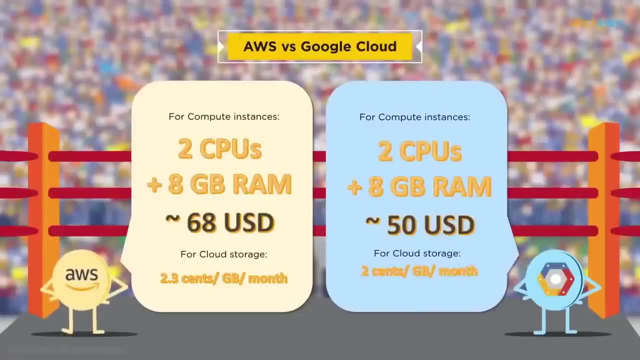 It will cost approximately $50 per month with GCP And, as per my calculations, that's a 25% annual cost reduction when compared to AWS. Talking about cloud storage costs, it is only 2 cents per GB per month with GCP. 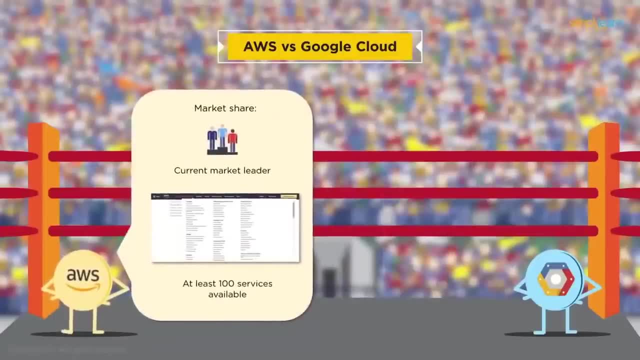 What else do you want me to say? Let's talk about market share and options. Now, AWS is the current market leader. It's the biggest market leader in the world When it comes to cloud computing. Now, as you remember, we contribute at least 47% of the entire market share. 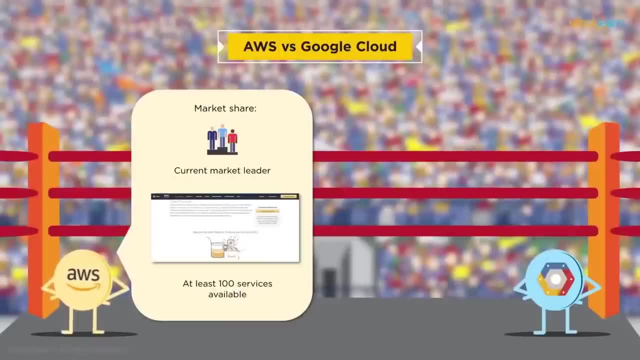 AWS also has at least 100 services available at the moment, which is a clear indication of how well AWS understands businesses and helps them grow. Yeah, that's true, But you should also know that GCP is steadily growing. We have over 60 services that are up and running, as you can see here, and a lot more to come. It's only a matter of time when we will have as many services as you do. Many companies have already started adopting GCP, So let's talk about the things you get for free. With AWS, you get access to almost all the services for an entire year, with usage limits. 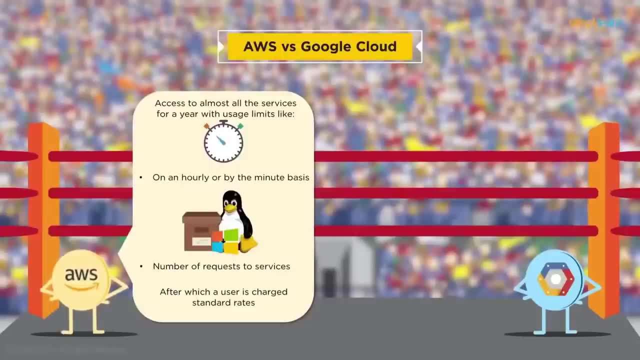 These limits include an hourly or by-the-minute basis. For example, with Amazon EC2, you get 750 hours per month. You also have limits on the number of requests to services. For example, with AWS Lambda, you have 1 million requests per month. 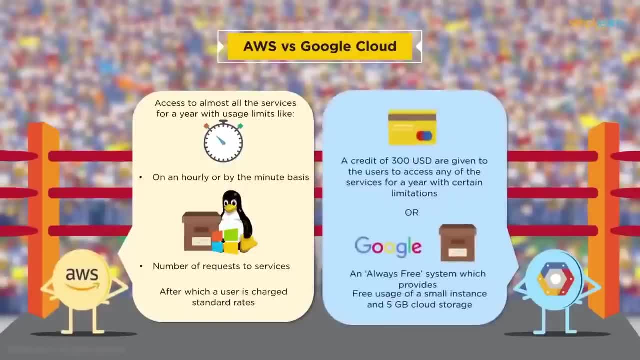 Now, after these limits are crossed, you get charged standard rates. With GCP, you get access to all cloud platform products. You also get access to the cloud platform services. You also get access to the cloud platform services. You also get access to the cloud platform services. 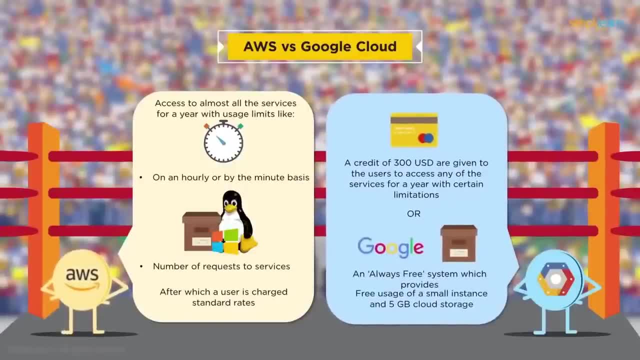 You also get access to the cloud platform products. Finally, with GCP, you get axes-high access to the various cloud platform products, Like such as Firefox, Google Maps and so on. You also get $300 in credit to spend over a 12-month period on all the cloud platform. 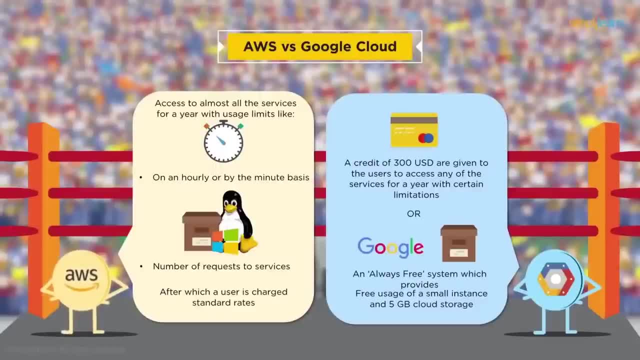 produces. Now, interestingly, after the free trial ends, you won't be charged unless you manually upgrade to a paid account. Now there is also the AWS free version, for which you will need an upgraded billing account. Here you get to use a small instance for free and 5 GB of cloud storage. 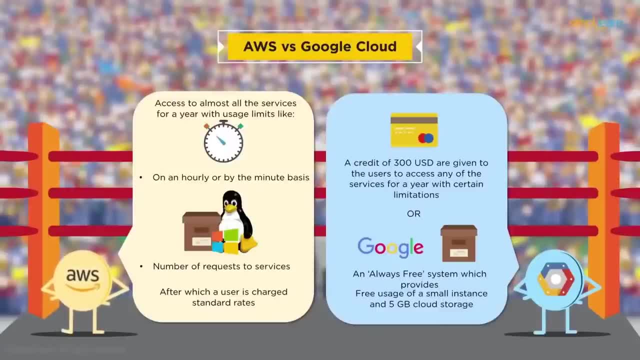 Any usage above the AWS free usage limits will be automatically included in GCP. With AWS emails, you get to go into Google store, download videos and use the stores on your computer. Uh, but begin for free. before buying today, build at standard rates. Now let's talk about how you can configure instances. 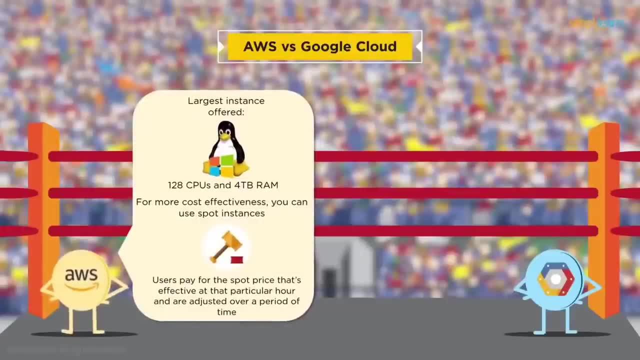 with AWS, the largest instance that's offered is of 128 CPUs and 14GB of RAM. Now, other than the on-demand method, like I mentioned before, you can also use spot instances. Now, these are for situations where your application is more fault-tolerant and can handle an interruption. Now you pay for the spot. 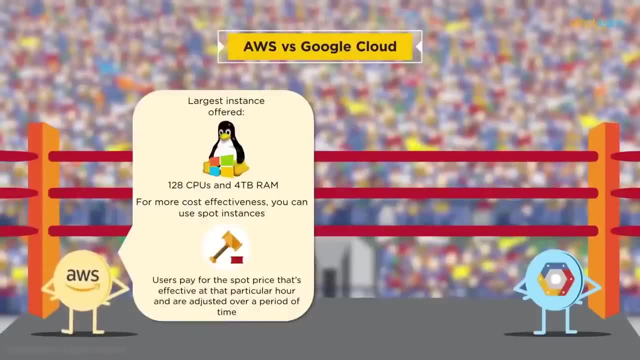 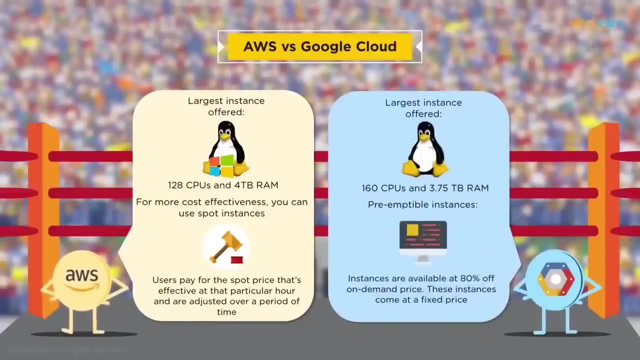 price which is effective at a particular hour. Now these spot prices do fluctuate but are adjusted over a period of time. The largest instance offered with Google Cloud is 160 CPUs and 3.75 TBs RAM. Like spot instances of AWS Google Cloud. 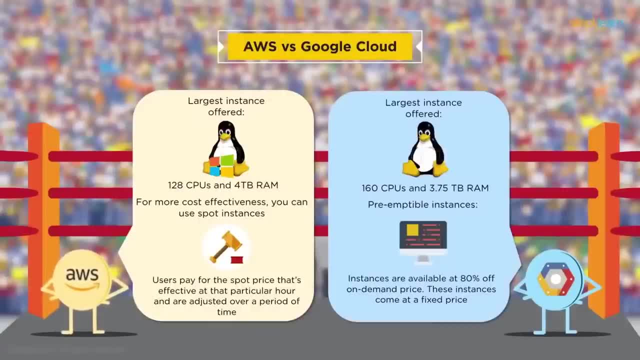 offers short-lived compute instances suitable for back jobs and fault-tolerant workloads. They are called as pre-emptable instances, So these instances are available at 80% off on on-demand price. Hence they reduce your compute engine costs significantly and, unlike AWS, these come at a fixed price. 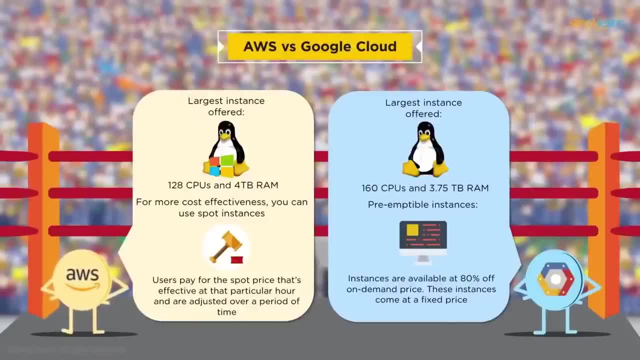 Google Cloud platform is a lot more flexible when it comes to instance configuration. you simply choose your CPU and RAM combination. of course, you can even create your own instance types this way. Before we wrap it up, let's compare on some other things as well. Telemetry, It's a process of 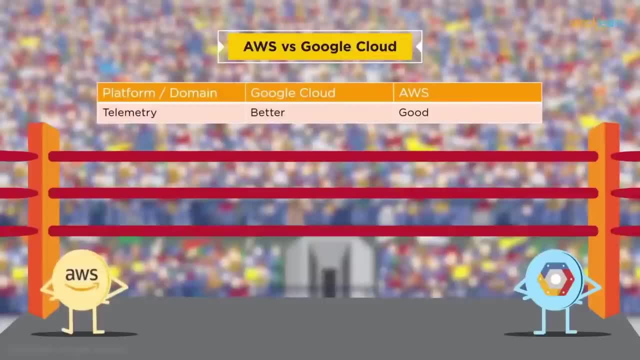 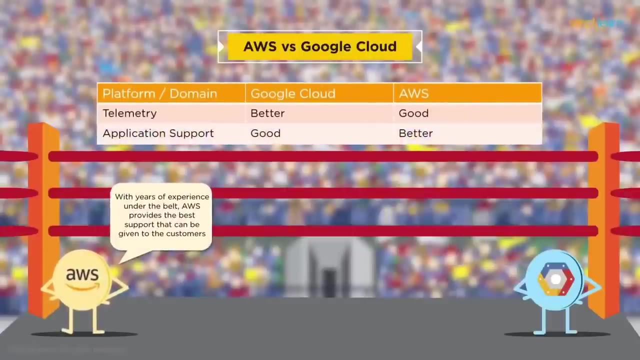 automatically collecting periodic measurements from remote devices, for example GPS. GCP is obviously better because they have superior telemetry tools which help in analyzing services and providing more opportunities for improvement. When it comes to application support, AWS is obviously better. since have years of experience under their belt, AWS provides the best support that can be given to. 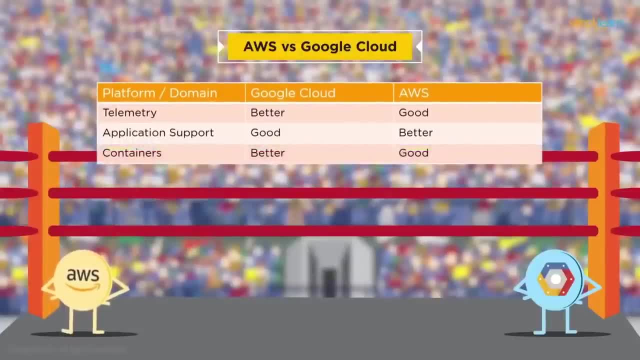 the customers. Containers are better with GCP. A container is a virtual process running in user space. As Kubernetes was originally developed by Google, GCP has full native support for the tool. Other cloud services are just fine-tuning a way to provide Kubernetes as a service. 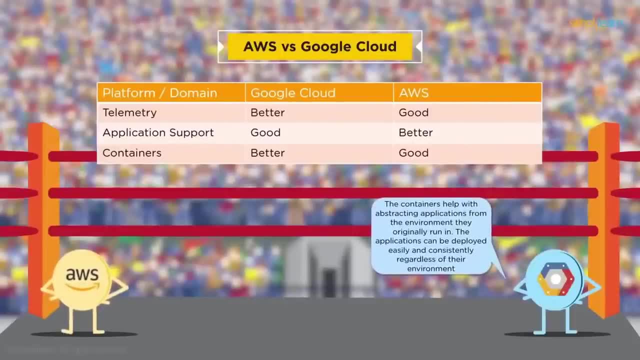 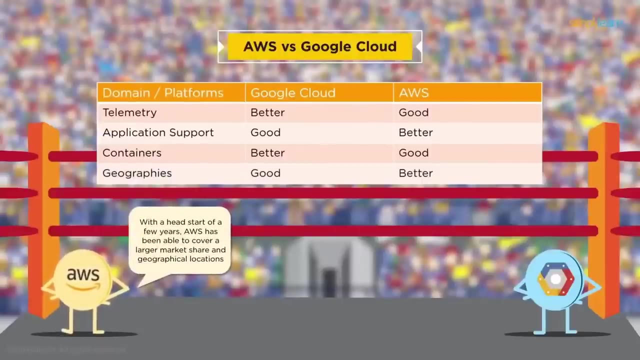 Also, the containers help with abstracting applications from the environment they originally run in. The applications can be deployed easily regardless of their environment. When it comes to geographies, AWS is better, since they have a head start of a few years. AWS, in this span of time, has been able to cover a larger market share and geographical locations. 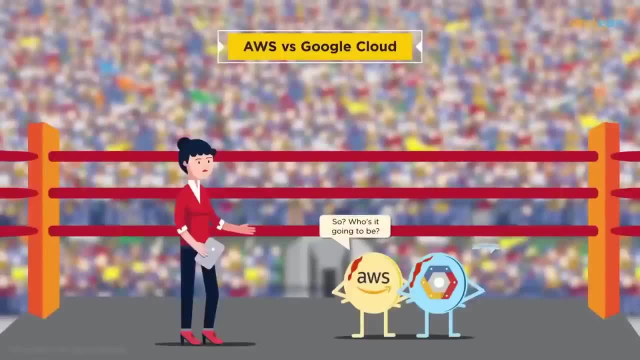 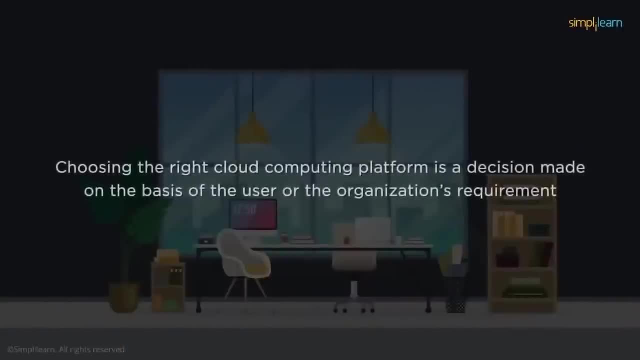 Now it's time for the big decision. So who's it going to be? Yeah, who is it going to be? GCP or AWS? I think I'm going to go for. choosing the right cloud computing platform is the decision that's. 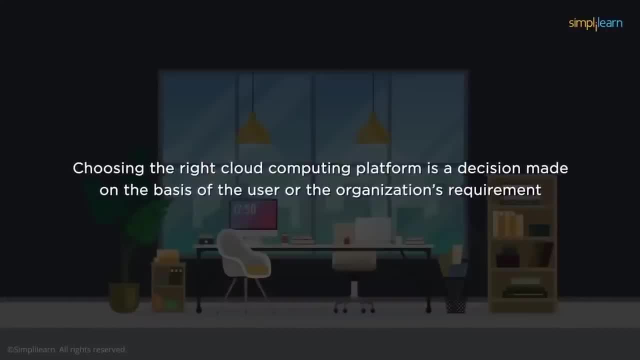 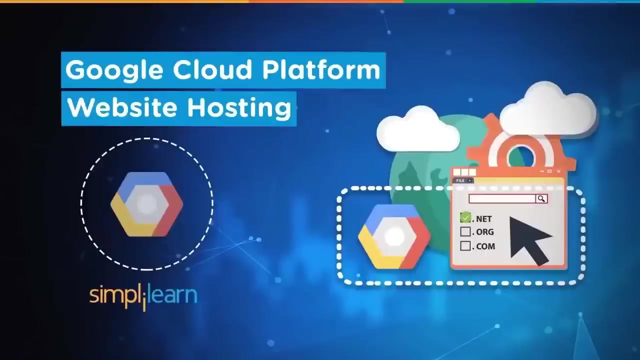 made on the basis of the user or the organization's requirement. On that note, I believe it's time for us to wrap this video up. We hope you guys enjoyed this session. We'll see you in the next video. Bye, Hello, everyone. Welcome to this session on Google Cloud Platform website hosting. 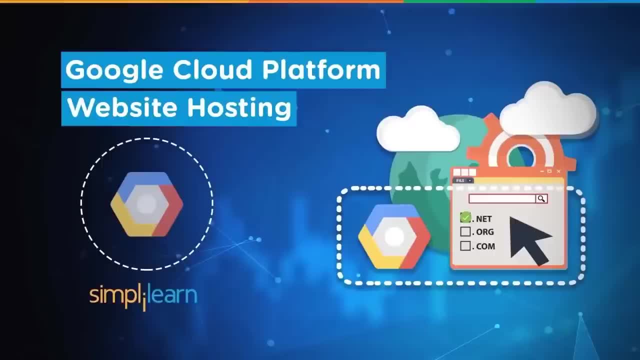 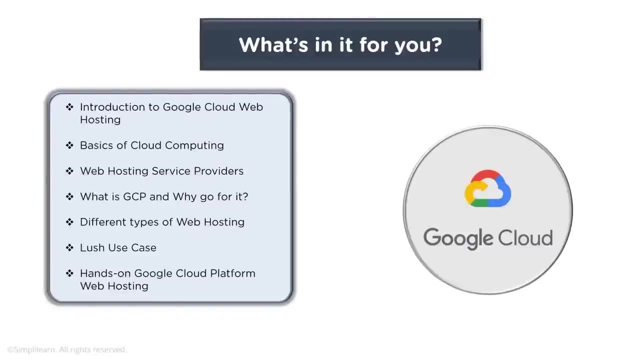 and let's understand what Google Cloud Platform offers when it comes to your web hosting requirements. Here we will learn about Google Cloud web hosting. some basics of cloud computing. web hosting service providers. what is GCP and why go for it? different types of web hosting which are possible. 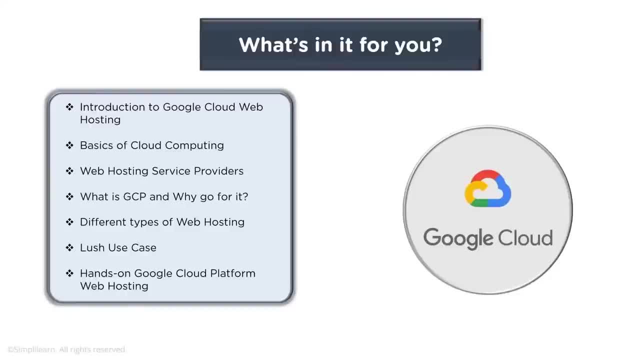 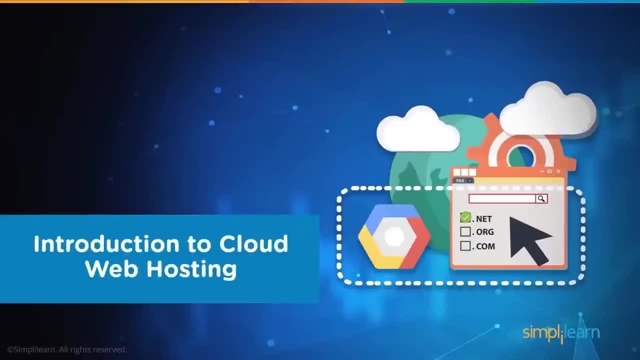 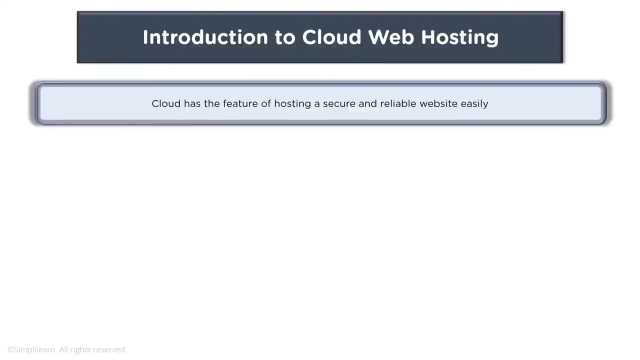 a use case such as Lush and a quick hands-on on using GCP for web hosting. When you talk about cloud web hosting, Google Cloud has the feature of hosting a secure and reliable websites easily. It ensures customers' and sites' protection. The website is. 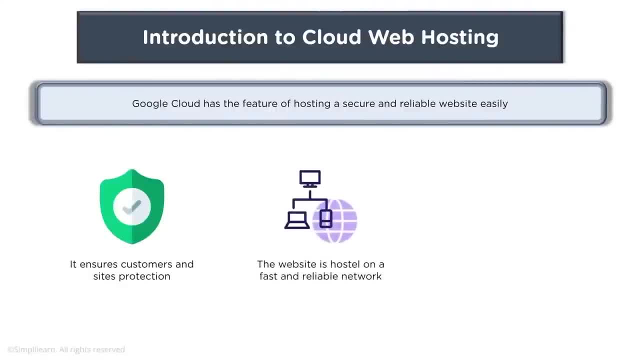 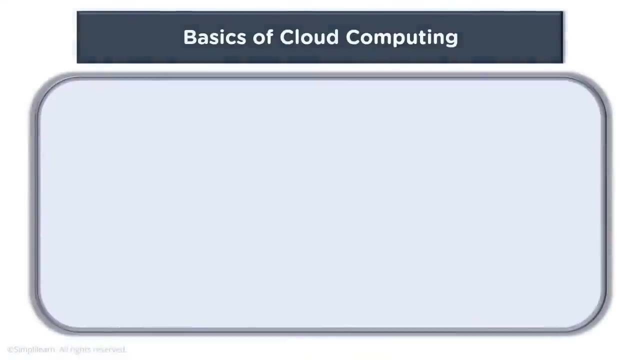 hosted on a fast and reliable network. You can do more work for less price with Google Cloud. Now, when we talk about Google Cloud, it is always good to know some basics of cloud computing. Now, when we talk about cloud computing, cloud computing is basically using resources. 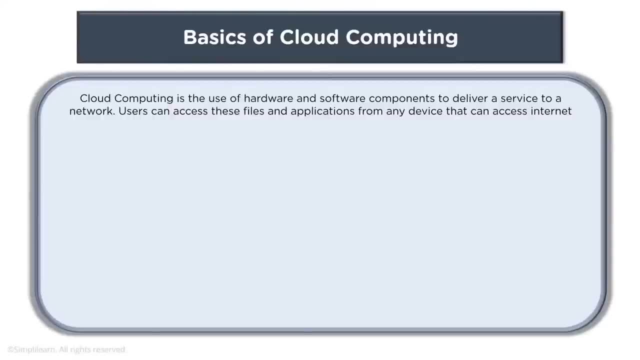 which are provided by your cloud service provider, such as Google Cloud, and cloud computing basically means using hardware and software components to deliver a service on a network. Now, here users can access files, applications from any device that can access internet. 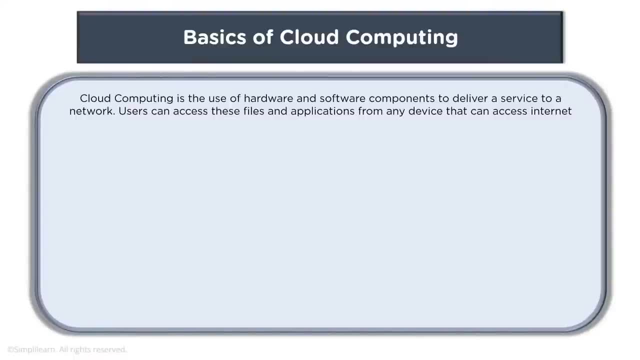 So when we talk about cloud computing, this is basically using services which are hosted on the infrastructure managed by cloud provider. When we talk about resources which can be used, that may include big data services, storage options, your computing options, networking options. 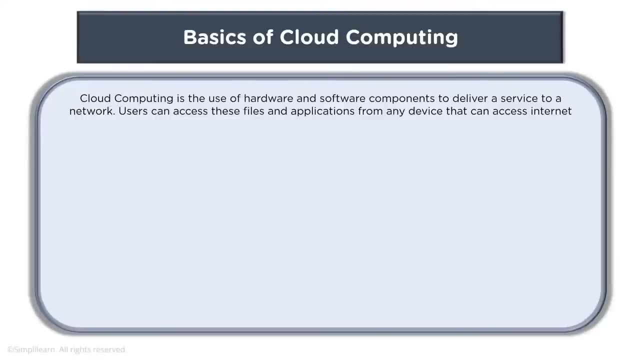 and various other services which a cloud provider offers. Cloud computing has various different service models, such as you have platform as a service, software as a service, infrastructure as a service. Also, these days we talk about containers as a service, and these are your different computing service models which are being 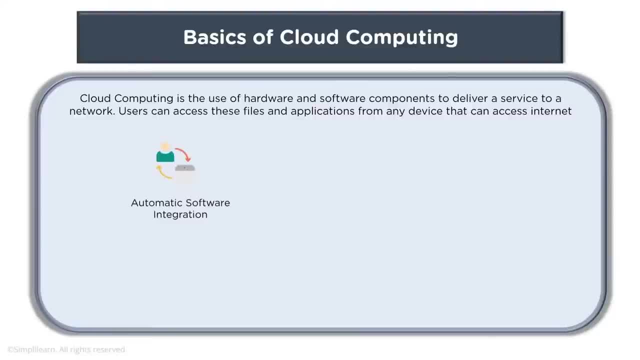 offered by cloud service providers, which allow you for automatic integration with your existing environment or if you would want to benefit from modernization by using a cloud provider's infrastructure. You have different services which are offered. Some of them are for auto software integration or migration, backing up and restoring data, scaling your storage. 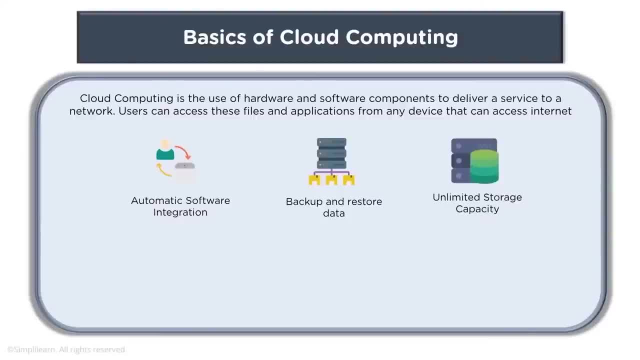 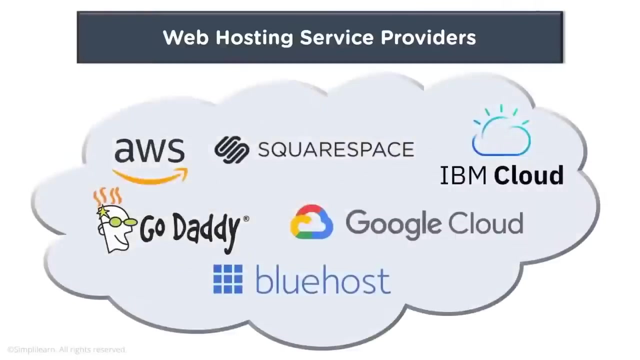 or mounting your system with a cloud is the other, and multi-task splits with a cloud service provider which offers a type of integration process so that you can have large storage capacity. that is, going for unlimited storage capacity and using a resource provided by cloud service provider, benefiting from reliability, cost efficiency, which is offered by 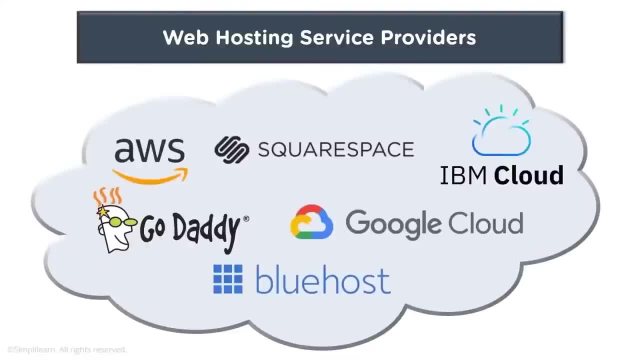 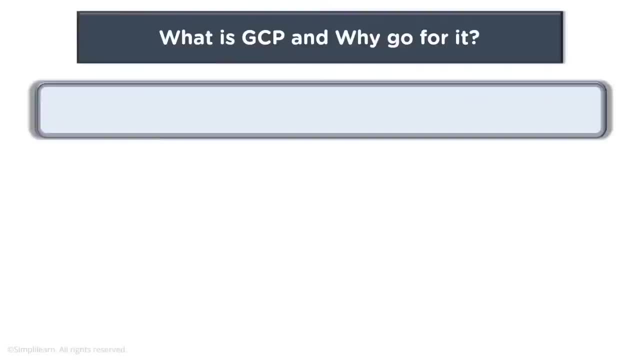 a cloud provider. In this case, we are talking about Google Cloud host and Google Cloud. So what is GCP and why go for it? When you talk about GCP, or as we call it, as Google Cloud Platform, it is set of cloud computing services provided by Google that runs. 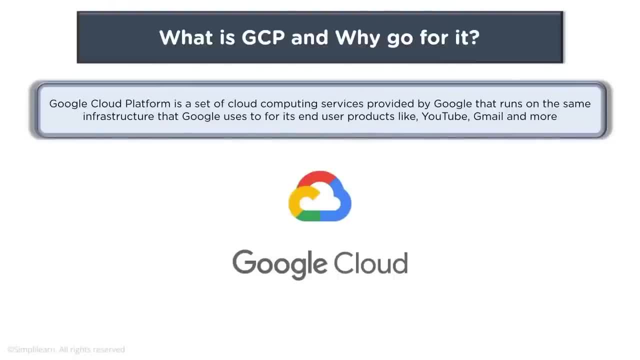 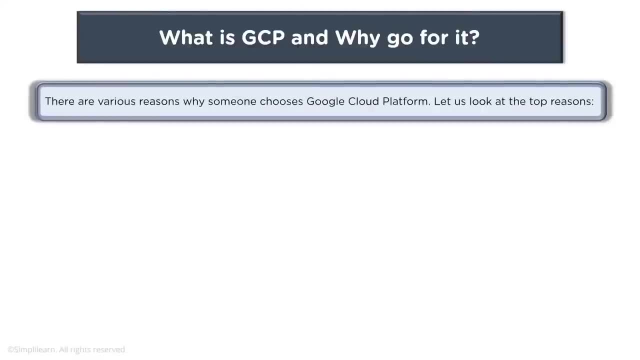 on the same infrastructure that Google uses for its end user products like YouTube, Gmail and much more. When you talk about GCP, there are various reasons why anyone would choose it for their use cases. Now let's look at some reasons. When you talk about pricing, GCP has better pricing. 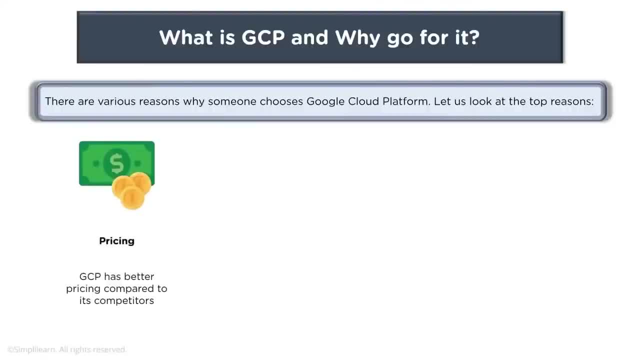 compared to its competitors, depending on the services which you would use, whether that would be infrastructure as a service, such as using compute engine instances and running your applications on them, or might be a managed service, Such as data proc or big table or your big query, where you can have your Hadoop clusters running. 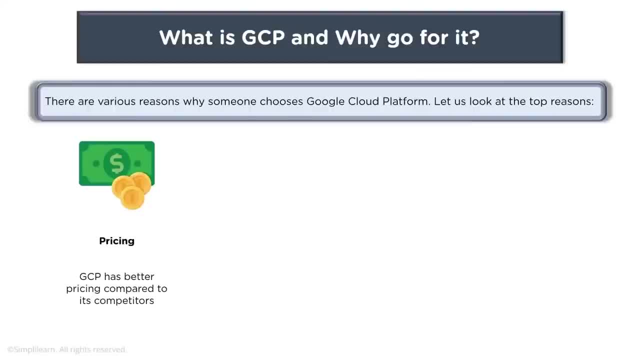 or store huge amount of data, or even build your data warehouse wherein you can store structured data. So there are different services which GCP offers, and pricing has been a better option in case of Google in comparison to other competitors, When you talk about speed and performance, 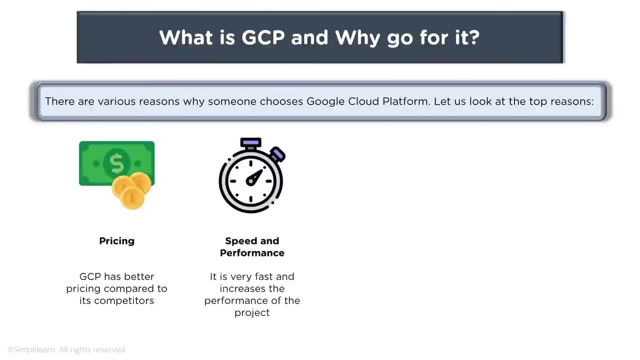 it's very fast and increases the performance. When you talk about live migration of apps, this is one of the features which organizations usually like, which none of other competitors are offering when it comes to live migration of apps. So there are specific features. For example, when you talk about compute engine, there is a feature. 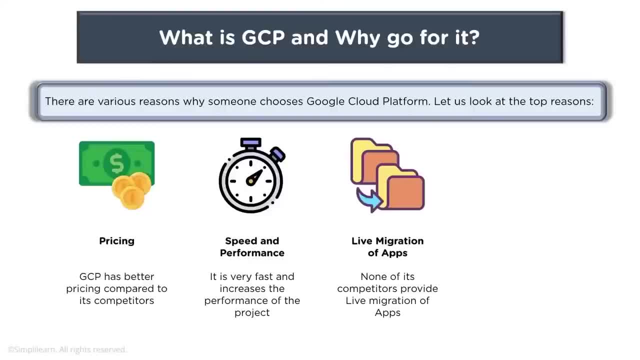 stating live migration, wherein your resources or your instances, which you can use to migrate the services which are running applications, would be migrated during, say, maintenance from one underlying host to another underlying host without affecting your applications performance, and you can benefit from that. When you talk about big data, Google Cloud has various offerings and big data space, and that's. 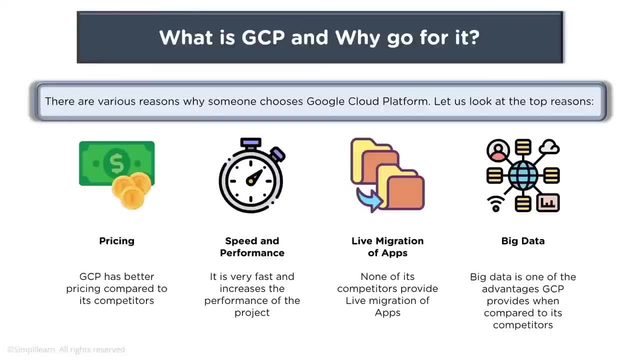 one of the advantages of GCP In comparison to other competitors. you have different services for your big data needs: publish subscribing messaging system or going for data proc, which basically allows you to spin up your Hadoop and Spark clusters to run your different jobs and so on. So when we talk about 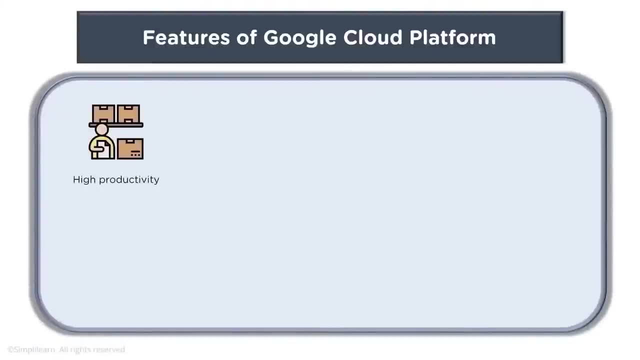 features of Google Cloud Platform. it offers high productivity because you are using the resources which are based on the same infrastructure which Google uses for its own different use cases. You can work from anywhere, provided you have internet connection and you can connect to the cloud platform and use different services offered via web. You can quickly collaborate with different 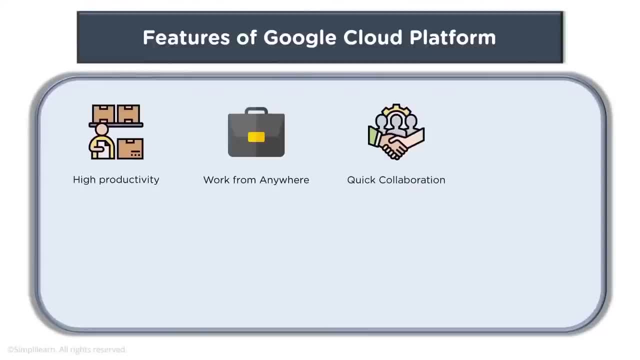 teams or different colleagues working on different projects which might be sharing or using different GCP resources. You are benefiting from high security and different encryption and security mechanisms which GCP offers. Now there are fewer sources, or you could say, data which is stored or vulnerable devices. There is high reliability. 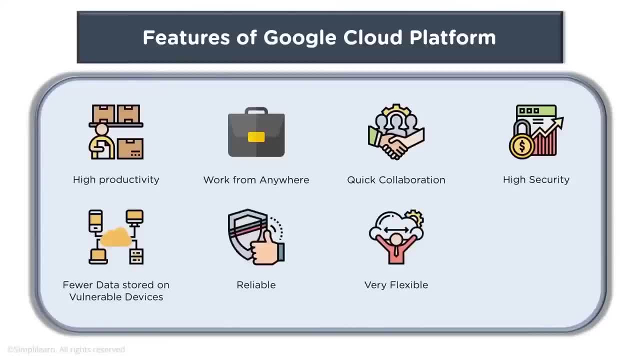 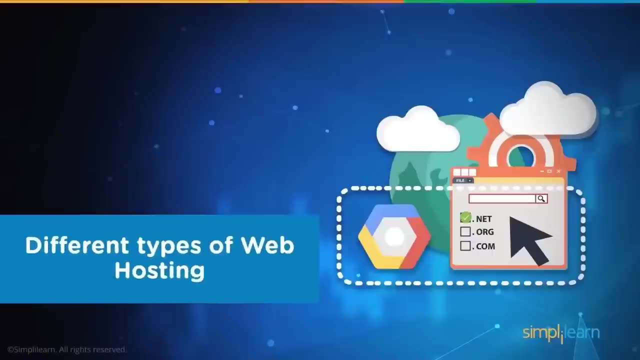 flexibility or scalability which GCP offers, and the cost effectiveness really makes it as a good choice when you would want to benefit from infrastructure modernization and using a cloud platform solution for your use case. Now, when you talk about different types of web hosting, 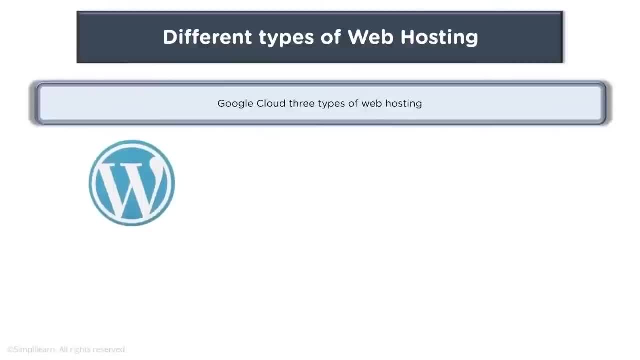 Google Cloud offers three types of web hosting. You have WordPress Now. it is a free and open source content management system. You might have used in past or have heard about WordPress, where a lot of websites are being created. It is a popular web publishing platform to easily set up blogs and websites and thus used by organizations or 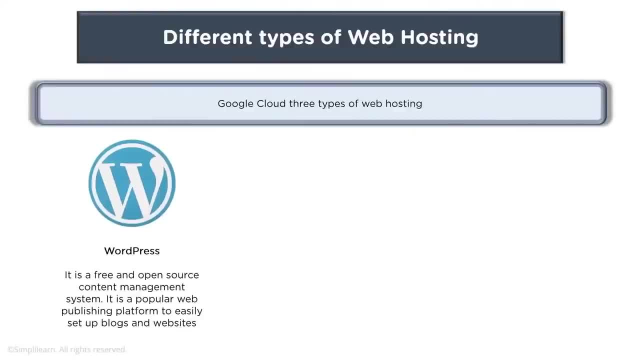 even individual users for having their blogs or running their websites or promoting their products. You have LAMP, which stands for Linux, Apache, MySQL and PHP, And LAMP stack consists of Linux, Apache, HTTP server, MySQL and PHP and is used to. 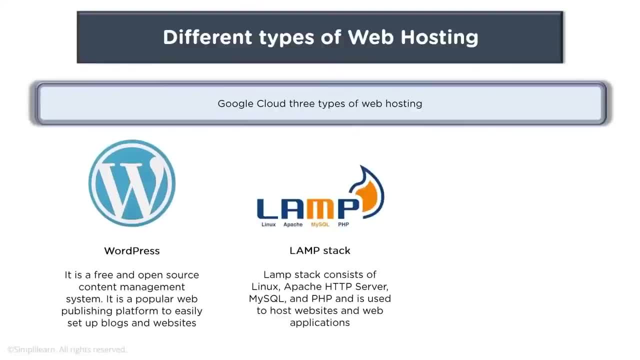 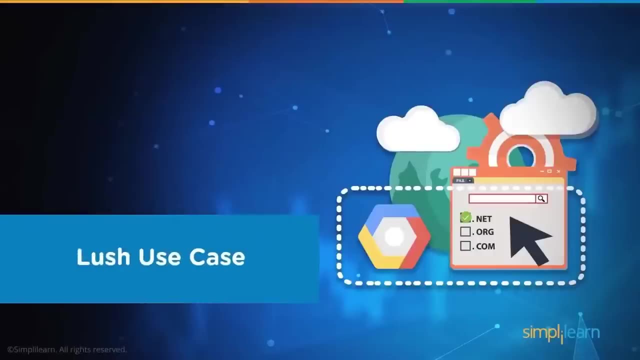 host websites and web applications. You also have your option of building your own website, So you can develop website or web application with your own code directly on Compute Engine. Now let's look at a use case and understand what happened here when we talk about Lush. 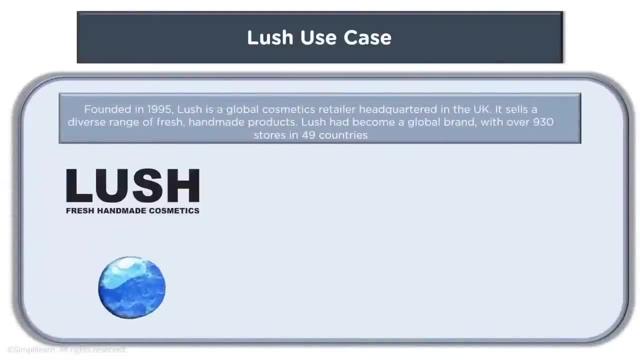 Lush was founded in 1995.. You might have seen this brand somewhere in the streets. It is a global cosmetics retailer headquartered in UK. It sells a diverse range of fresh handmade products. Lush had become a global brand with over 930 stores in 49 countries. So the challenges which were faced. 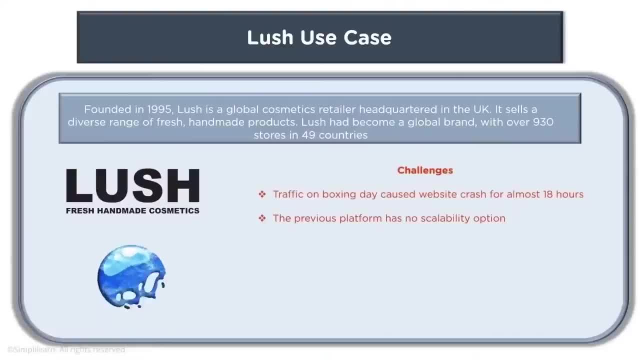 here was. traffic on Boxing Day caused website crash for almost 18 hours, And this is something which had a devastating effect on the website. So Lush was founded in 1995.. It is a global marketing agency based in India, And since then Lush has been a worldwide mobile blogger. 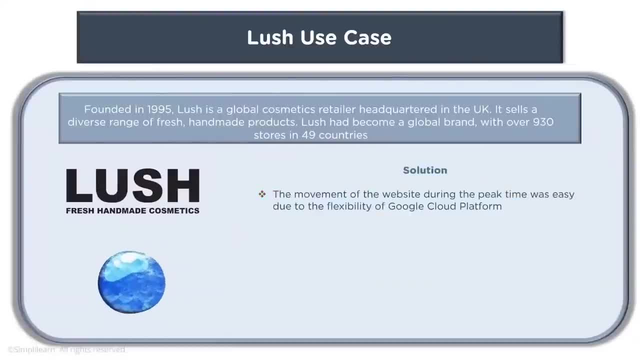 In the meantime, it has been changing markets and has been growing in price and investing in the management of the solution. responsabilization and judicial gravitation are among the major reasons that make Lush a global brand. As a result, it has been an incredibly popular site, So this is a new milestone for the website. 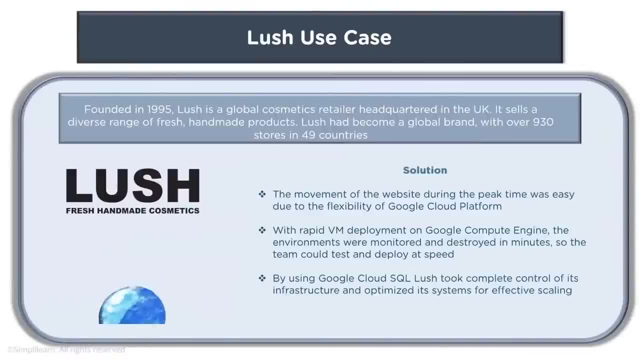 The first platform was called as Zedbox, The second platform was called as Zedbox, The second platform was called as Helptron and the third was called as Zedbox. In the previous platform, its systems for effective scaling. Overall, the platform resulted in lower cost that led to a. 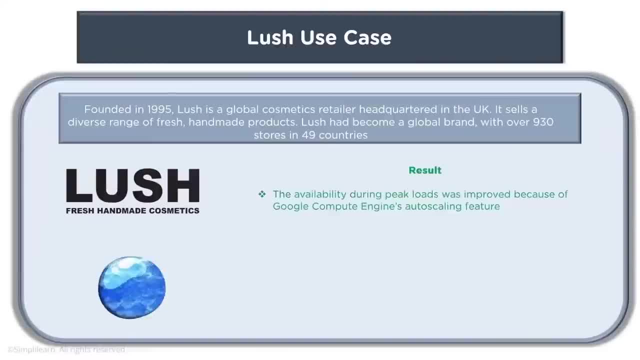 bright future for Lush Cosmetics. Now, what was the result of all this? The availability during peak loads was improved because of Google Compute Engine's auto-scaling feature. The infrastructure hosting costs were reduced by 40%. Streamline data center usage from 5 to 3 with Google's 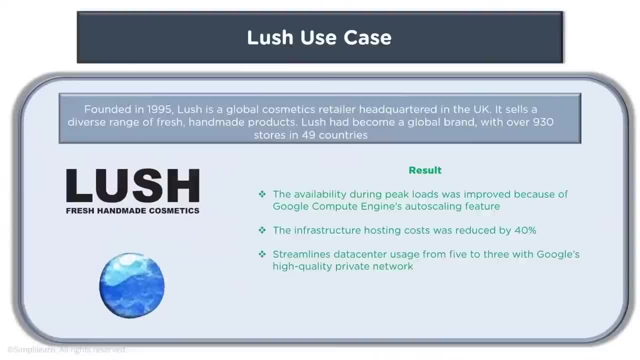 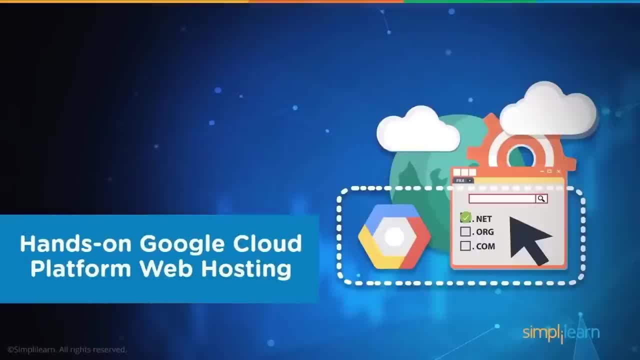 high-quality private network really benefited Lush, and it provided a flexible architecture and scalability for future business growth. Now what we have seen here is that your Google Cloud and its web hosting basically offers users to run their websites or use a web hosting solution that can benefit in more than one way. The simplest approach could be seen is by clicking. 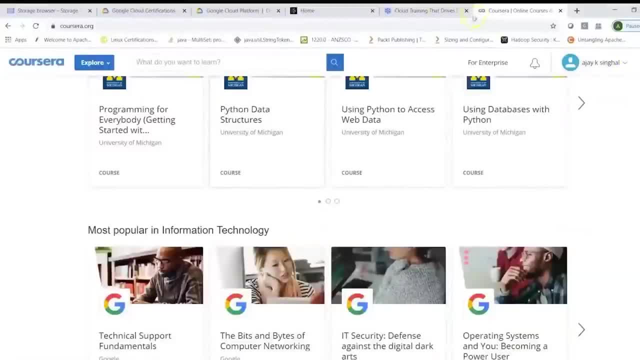 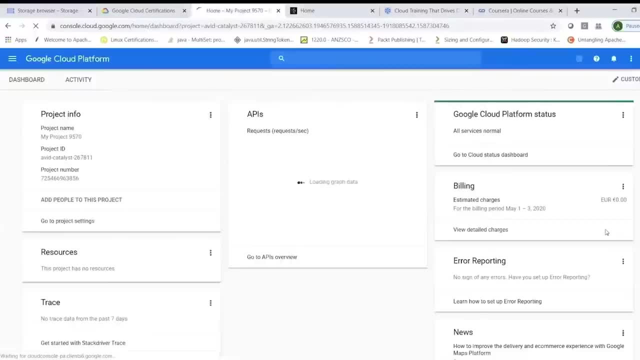 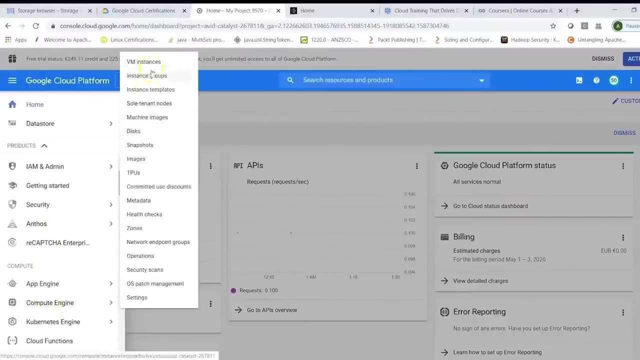 and setting up a VM instance By going to your console. for example, if we go in to the Google Cloud platform clicking on console and here, the easiest way I could test it is by going to my Compute Engine VM instances and here. 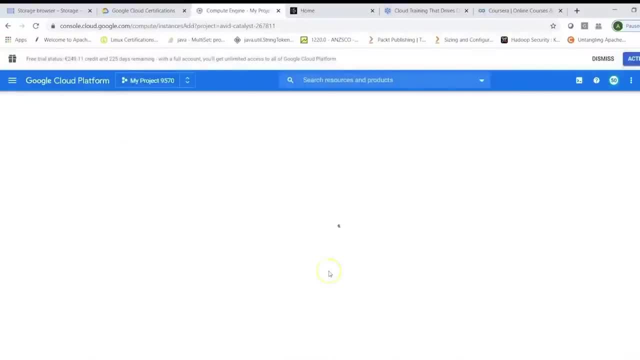 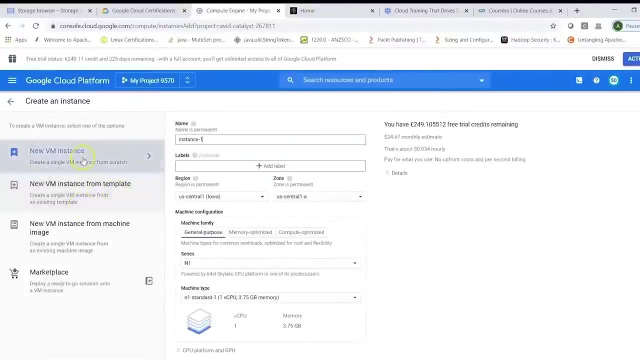 I can spin up an instance. I can click on create Now. in my previous sessions, I have also explained about how you could create a template and run an instance From that. we can also click on new VM instances Now. in my previous sessions, I have also explained about how you could create a. 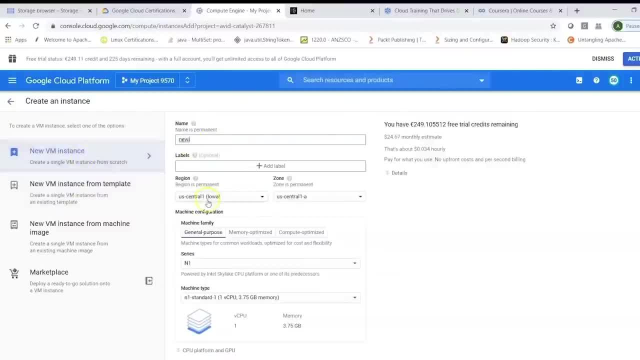 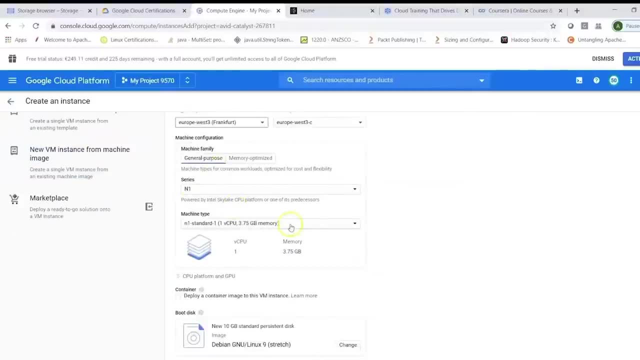 template and run an instance. Let's call it new instance. I will choose a region, For example Frankfurt. I will let it be general purpose machines. Let this machine be one virtual CPU core and 3.75 gigabyte RAM. If I'm looking for a heavier website which might have more users. 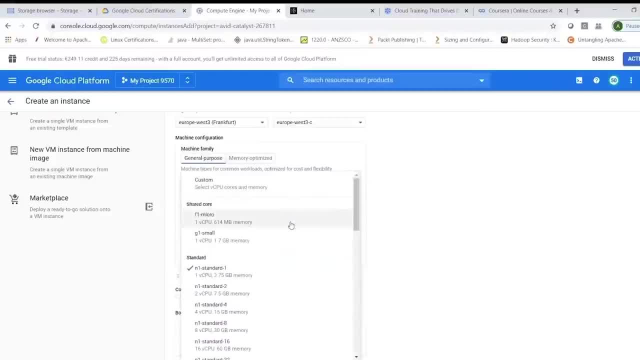 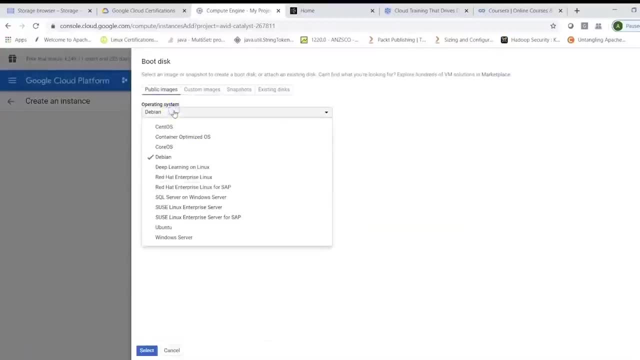 logging in and so on. then I can choose a higher configuration machine. Here we have the option to choose our distribution. So, for example, I can choose Ubuntu and then I can choose a distribution version, So let it be 16.04.. We can choose the. 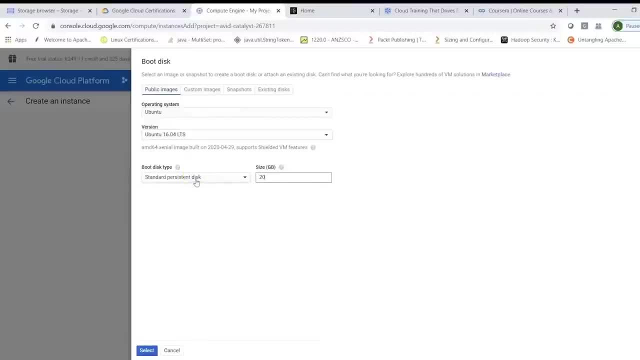 disk size to be 20 gigabyte and we can use SSDs or HDDs. So as of now it is standard persistent disk, that is HDD, and that should be enough. Let's click on select Here I will say allow default. 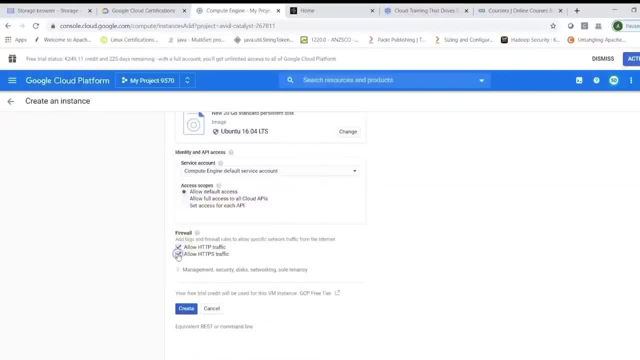 access. I would say: allow HTTP and HTTPS so that if I have a website content hosted on this machine, I can access it over HTTP. Now here you have management options. for your instance, You have security option, which basically allows you to provide a public key, if you are interested. 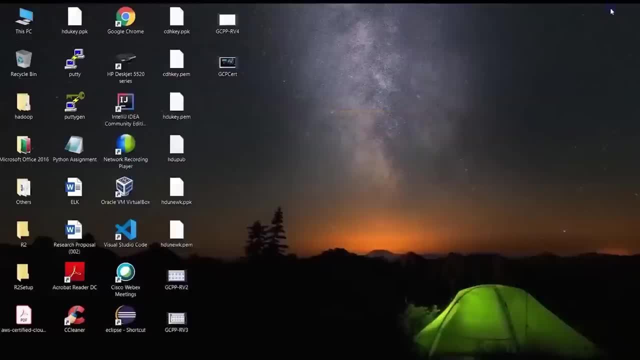 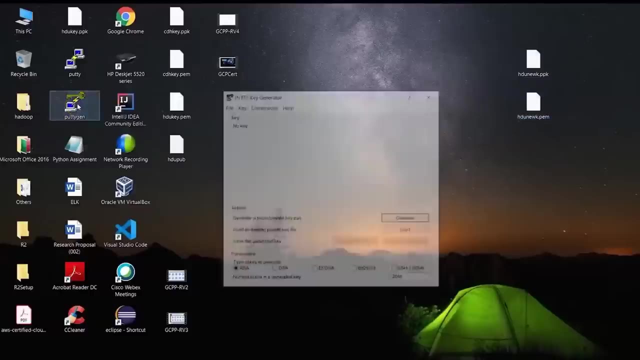 in using an external SSH client to connect. Now I have used PuTTYgen and I have already created a private key, which is here. I have also converted that as a PEM file and anytime if I would want to use this key, all I need to do is click on PuTTYgen. 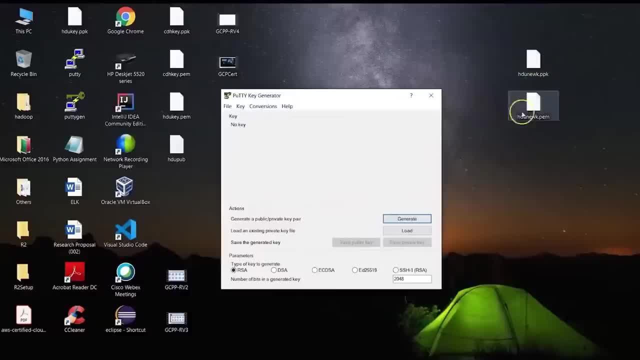 Where I had earlier created this PPK file. Now I can just do a load and I can choose the key which I have here and I can give the passphrase. Click on OK and that shows you the public key. Let's copy the public key from here. Let's go into our instance and I can give this here. 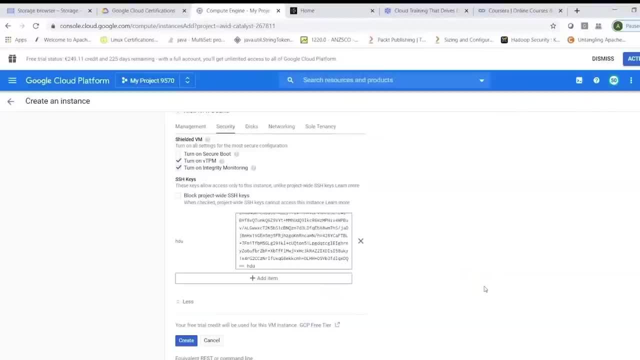 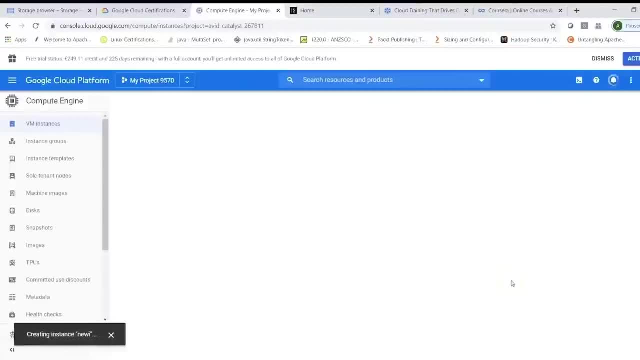 That resolves the name. So I have the private key saved on my machine and public key, which will be pushed into the machine. I can click on create and that should create my instance to which you can connect using SSH from the console itself. 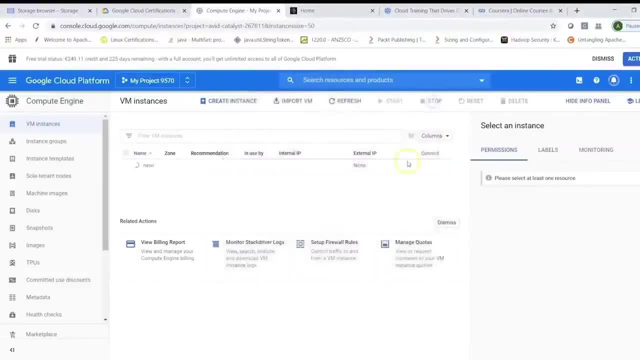 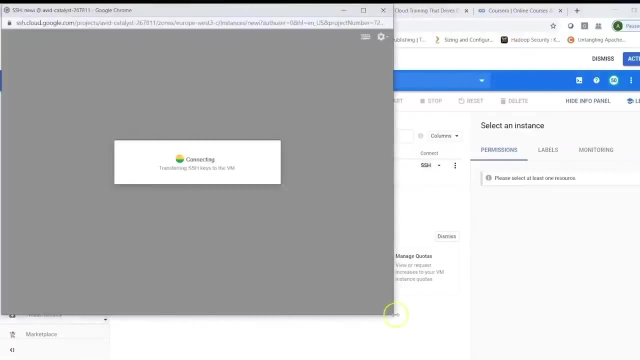 or using a external client such as PuTTY, which will then need the public IP of this instance, the PPK file, what we have- and you can connect to this instance. What I can also do is I can just do a simple SSH from here and that will basically allow me to connect to the instance. What we 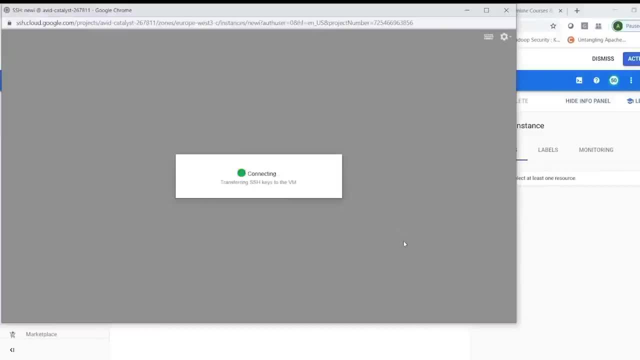 also need to remember is each instance has a public key. So if I want to connect to this instance, I can just do a simple SSH from here and that will basically allow me to connect to the instance. What we create and compute is also having some default firewall rules. Now I have connected to. 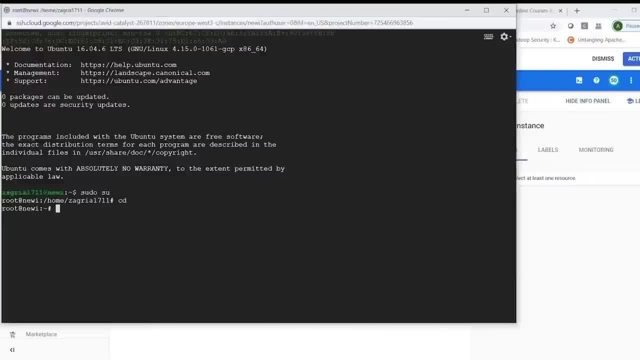 my instance, I can click on sudo, su, I can log in as root and here, if I would want, I can install a particular service. So let's say Apache, Let's say apt-get install, and then I can say Apache 2. 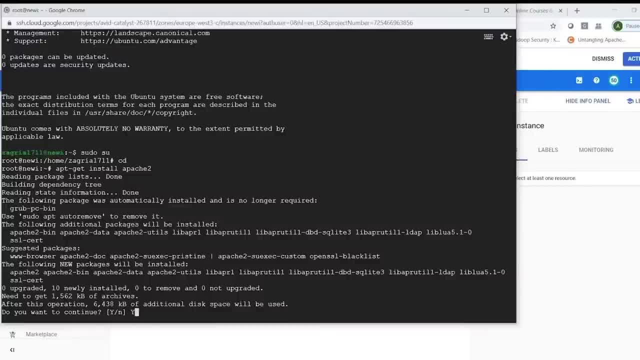 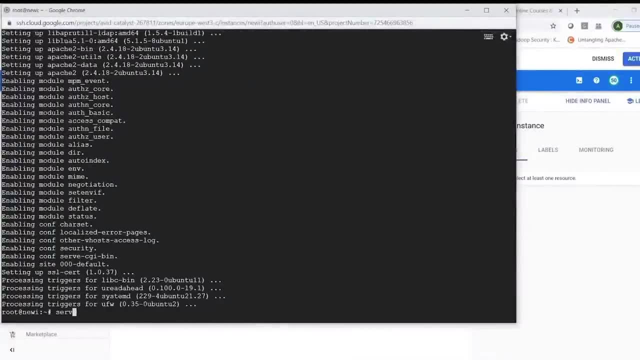 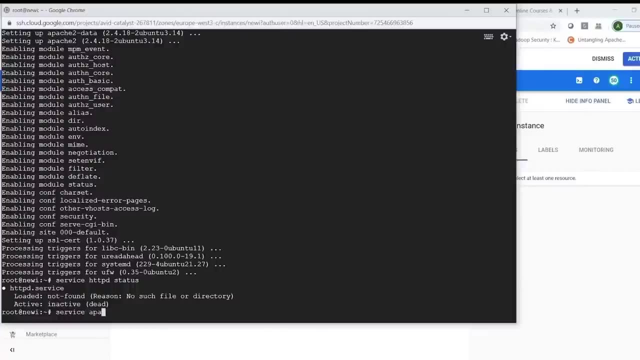 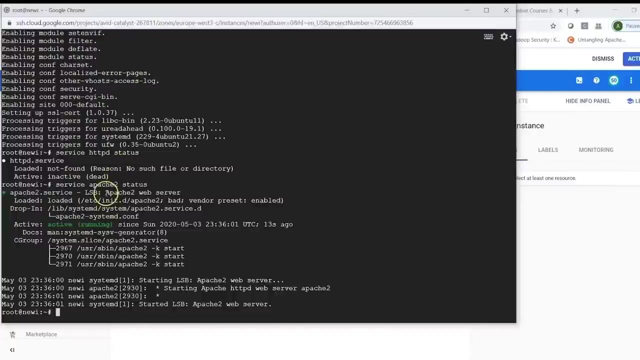 or HTTPD. That is basically to host your web application. So I'm installing the service And here I can check if the service is running by doing a service HTTPD status or I can say service Apache 2 status. It says it is already running. That means the Apache web server page will be. 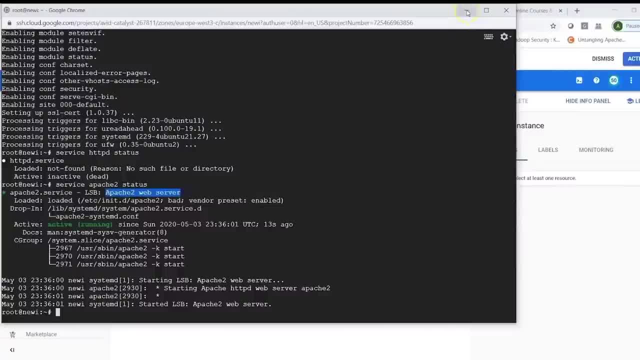 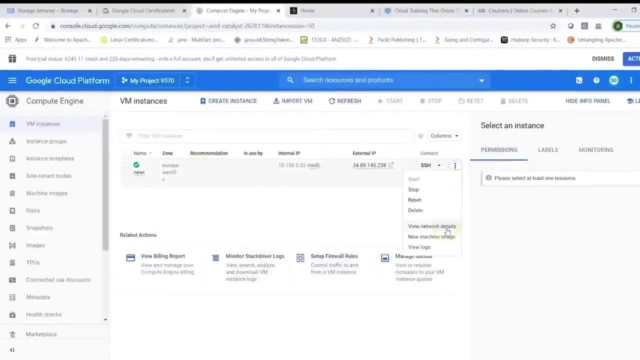 accessible from HTTP, provided my firewall rules allow that. Now, before we look into this, we can also, for our instance, look at the firewall rules. So here you have network details. Now, since we have network details, we can also look at the firewall rules. So here you have network details. 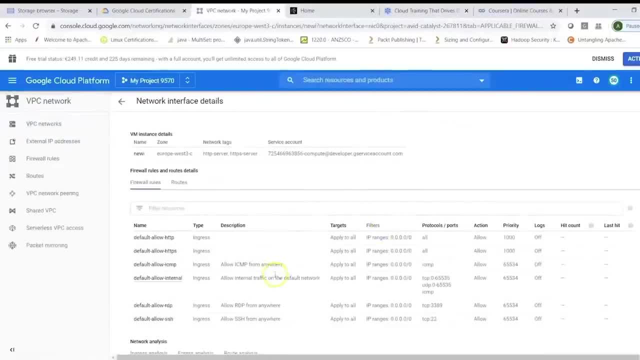 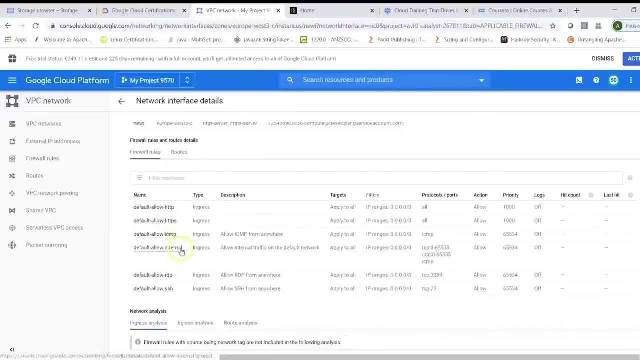 created an instance by default. Google has created some firewall rules which allow default HTTP, HTTPS, ICMP, your default internal access, RDP and SSH access. And here it says these ingress rules which allow incoming traffic are allowed from anywhere. We can customize that. 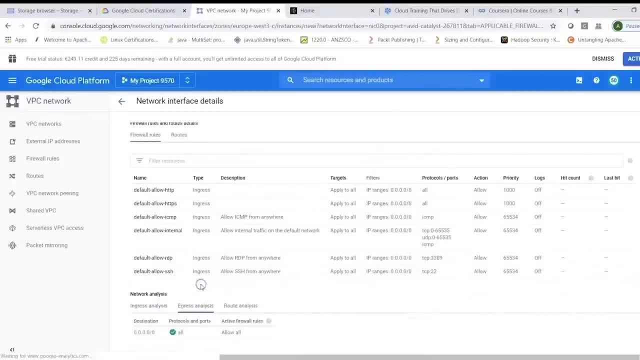 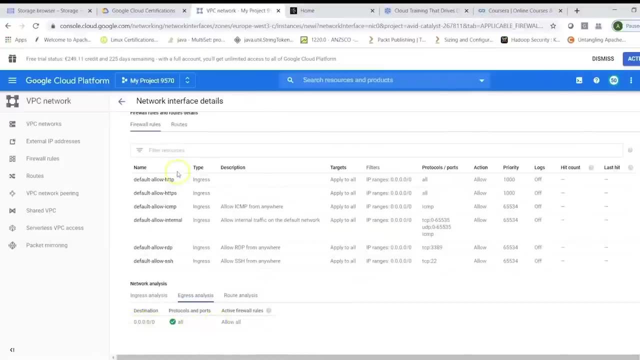 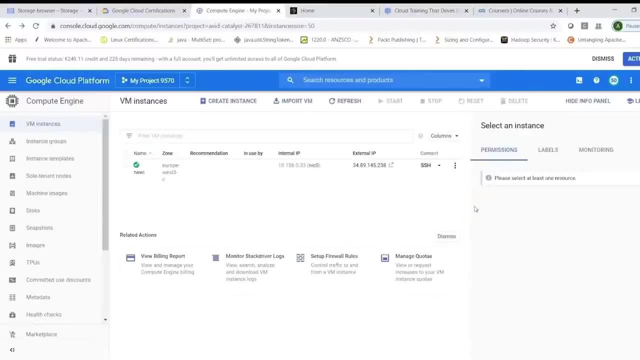 specific IP addresses. We can also look at egress, which is basically outgoing traffic, And this is again saying my machine can connect to the external world in different ways, using different protocols. So you can customize these firewall rules. As of now. I'm going to let it be default. Now we connected to our 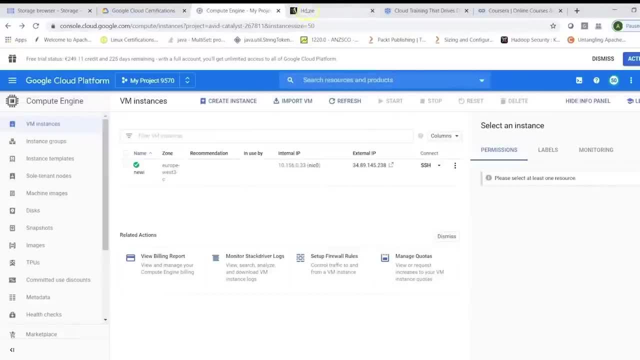 instance from the browser, and we were basically checking how you can use this browser by clicking on this. Now, what I can also do is here I'm logged into the instance. My Apache server is running, So the best way to check if. 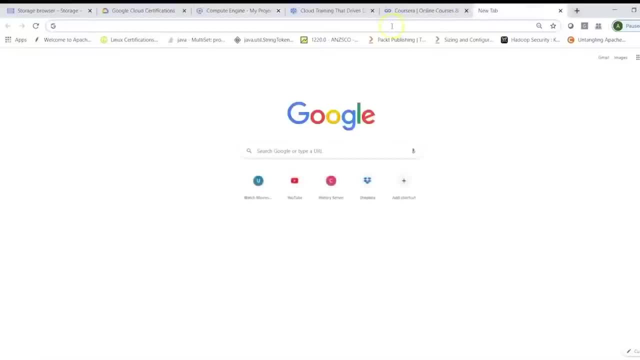 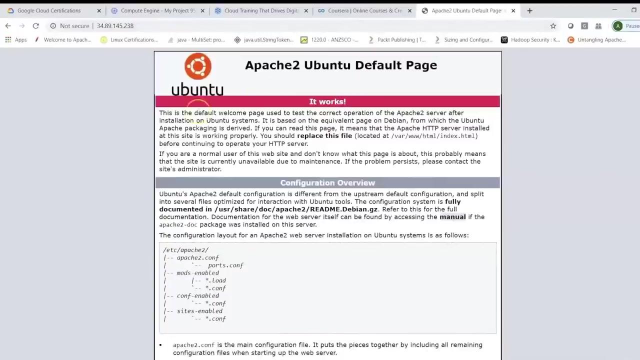 the Apache web server is accessible via HTTP. all I need is my public IP. So let's copy this, Let's go here And I will say: http//. just give you a public IP and that shows your Apache 2 web server page. That means: 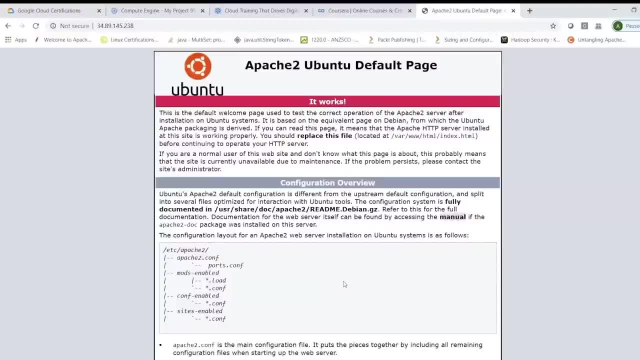 the Apache service has already been run. Now here it tells if you would want to host a particular page. what you will have to do is, as it says here. it is based on equivalent page on dbn, from which ubuntu apache packaging is derived. if you can read this page, it means apache http server is installed. 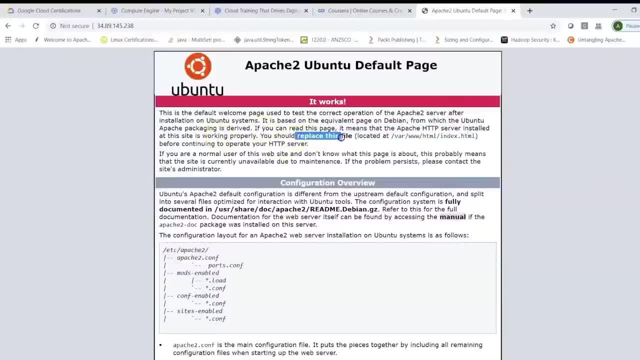 at this site is working properly. now you can replace this file located at var- wwwhtml- indexhtml before continuing to operate your http server. so this is where you can change the particular page and you will be able to host your web site on this particular ec2 instance. 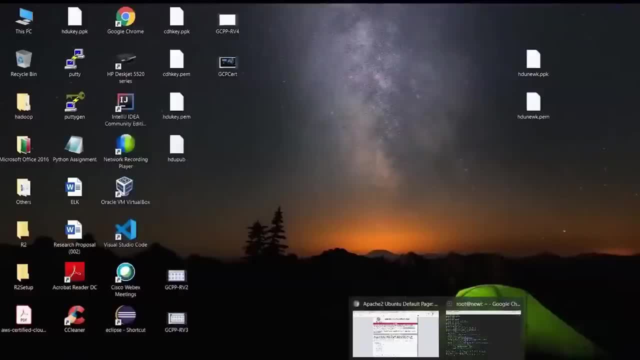 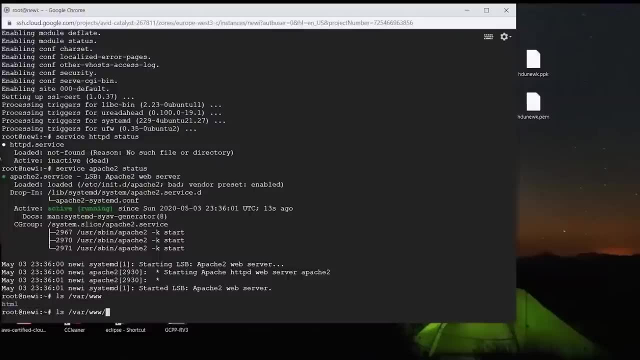 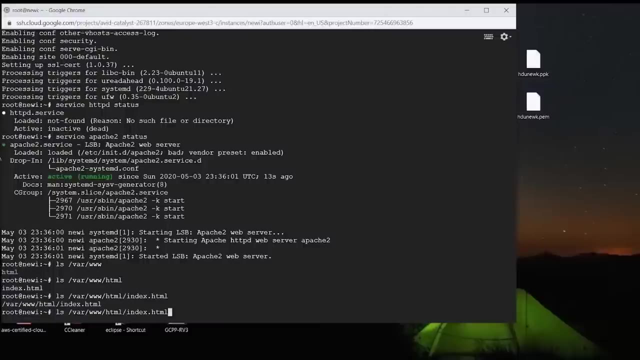 what we can do is we can check this. so we can go into the browser and we can look in var www and that has an html folder. look into this and, as of now, you have a index dot html and that, basically, is the page, what we are seeing. now i can click on this one and i can see. 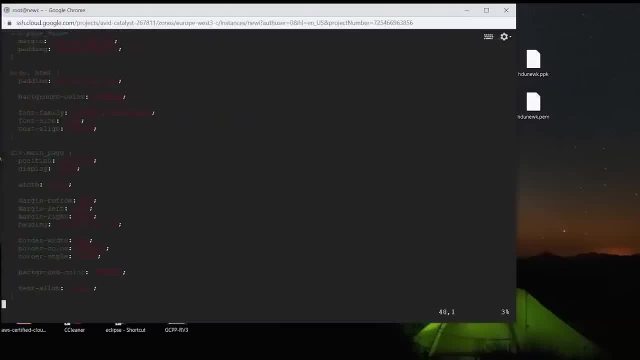 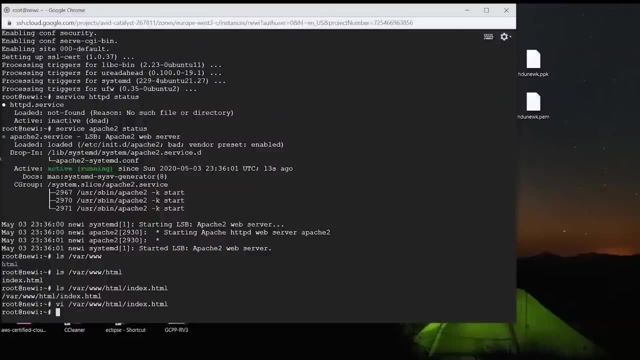 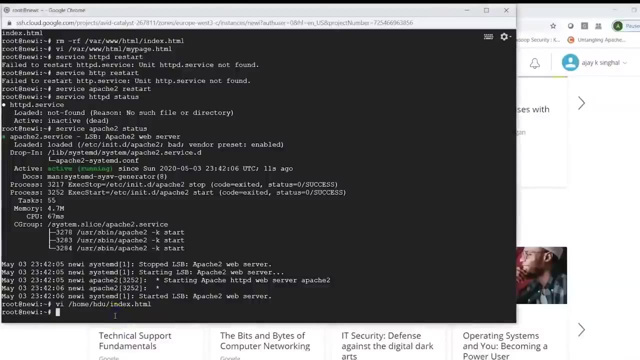 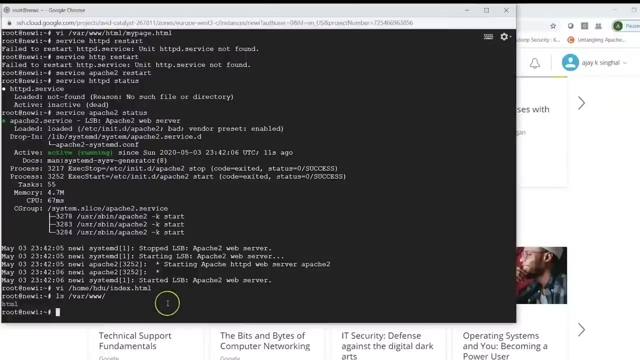 i have a small html page which is basically showing me what we are seeing on our web server. what i can also do is, for now, i can test it out and i can put in a different html page and see how that works. so we had basically the page here in var www and then we had the html folder. 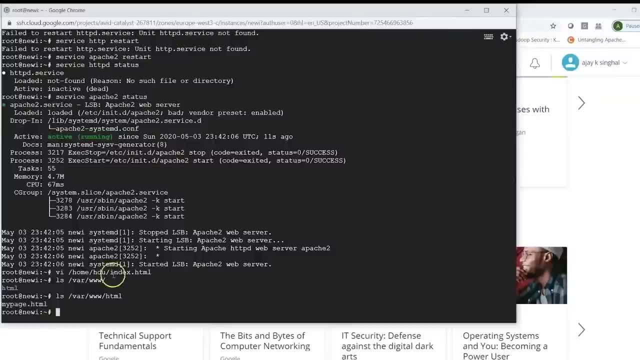 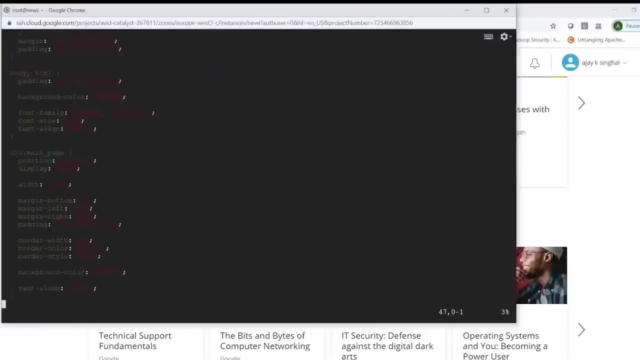 and in html folder what i had was this index file. so as of now, i just moved it and i put it in a different location. so if i look in my home hd you indexhtml, that shows me the complete html page, what we were seeing on our web server. and here it shows you what this page would display if you run it on. 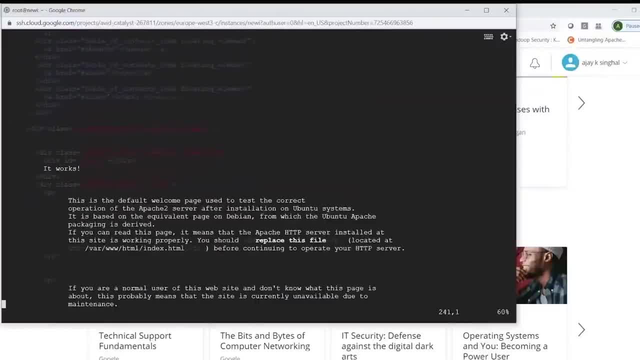 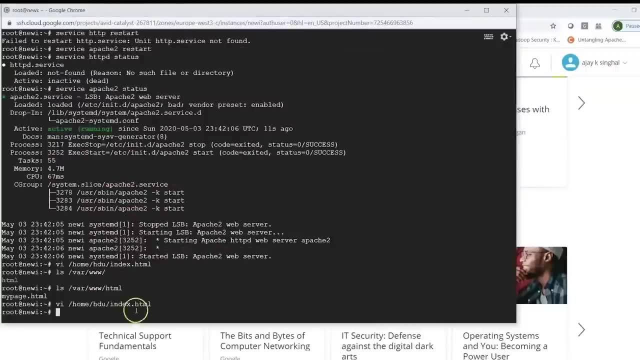 your http. it says apache to ubuntu default page. it shows it works, it shows the content and so on. so for just testing, i moved this page out from this location and what i did was i added a different page here. so that page, if you look in html and then look in my page, dot html section. 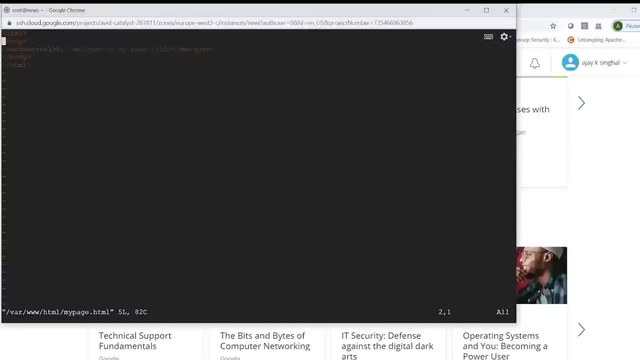 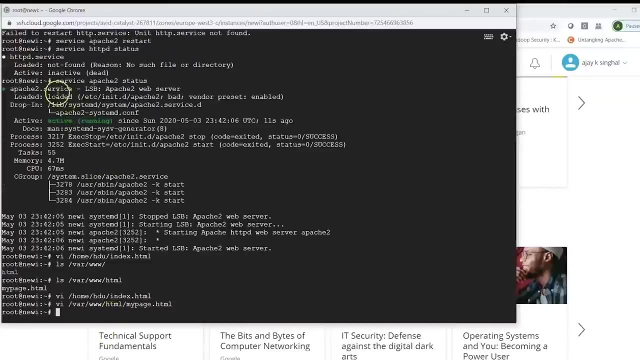 i've just added some basic details of creating html. i'm saying body, i'm using marquee and then i'm closing this with html tag. now, this is a simple html page which i created. what i did was, once i've done this, i basically did a service apache restart. so once you do that, 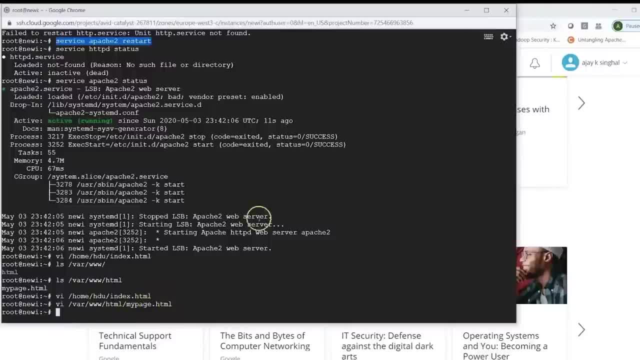 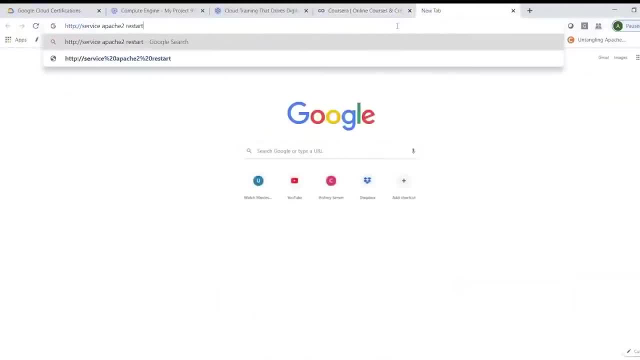 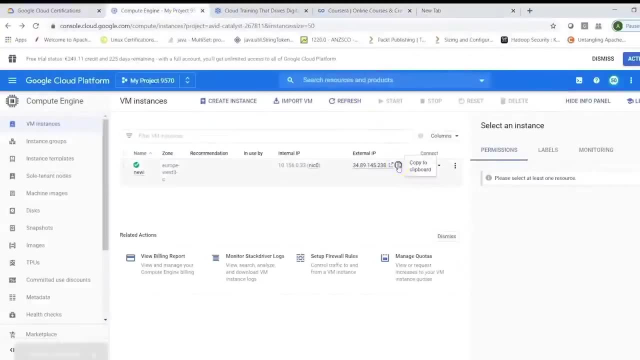 it will take up your new page and once you have done that, now you can access that by going to your http, given your details and then basically give your public ip, which we can get from here and just paste it here now. hit on this so that shows. 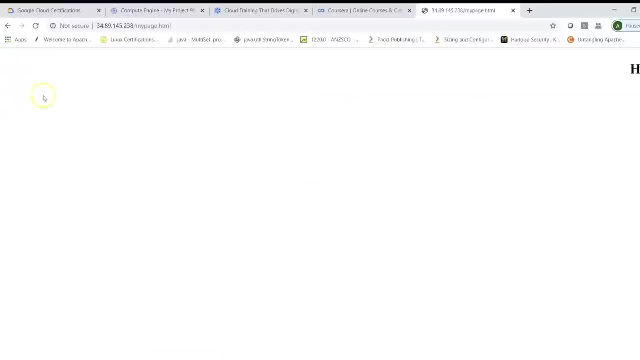 me, there is a my page dot html. i can click on this and that basically shows the symbol page which i created. so, as of now, this is my web page, which i have created, and this is hosted on my compute instance. now, obviously, we can create a more complex website. 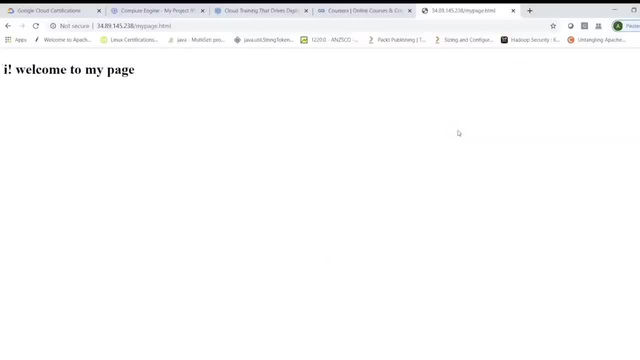 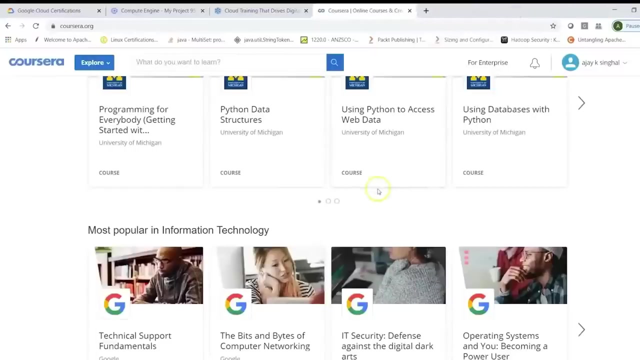 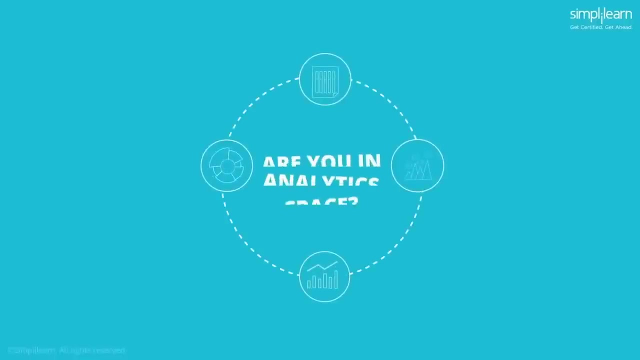 backed up by a database. use php, use mysql to store the data and then host your website on google cloud platform service such as compute, where your actual code is running, so we can learn about your web hosting on compute instances in further sessions. are you in the analytics space? 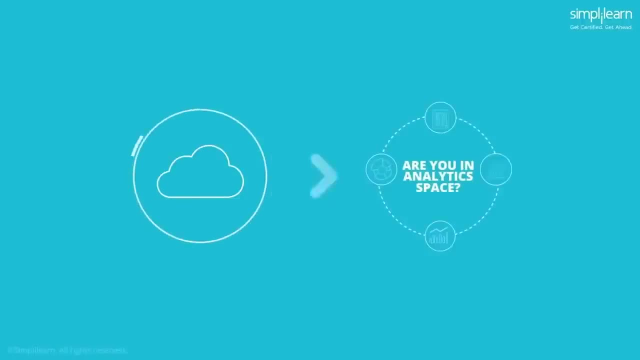 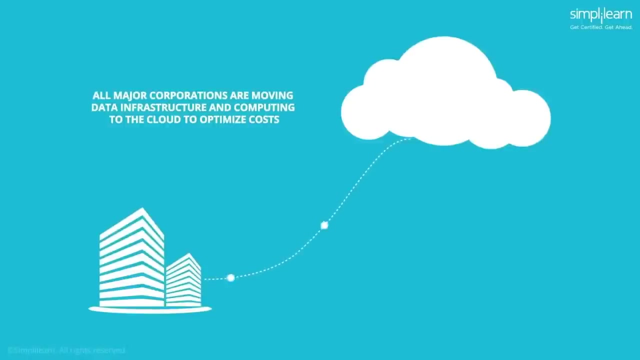 have you ever wondered how data processing in the cloud is changing the analytics space? if the answer is yes, this is the course for you all major corporations are moving data infrastructure and computing to the cloud to optimize costs. to make analyzing data seamless, technology leaders like google and amazon are investing heavily in sas tools on the cloud. 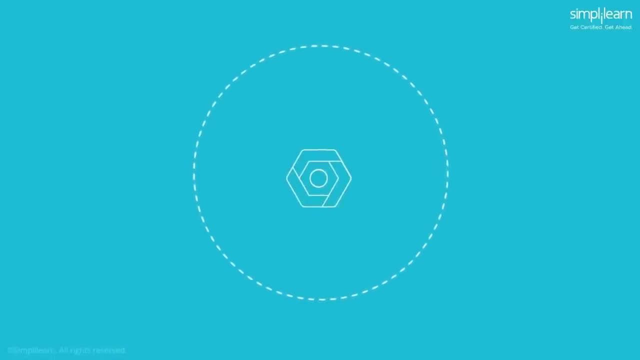 google is a pioneer in this space. the google big cloud data and machine learning platform provides cloud databases, managed hadoop and spark services with tools like dataflow and dataproc. the platform allows for highly scalable and reliable data processing and data processing services and data processing, data processing and reliable data processing, the data lab, bigquery and cloud. 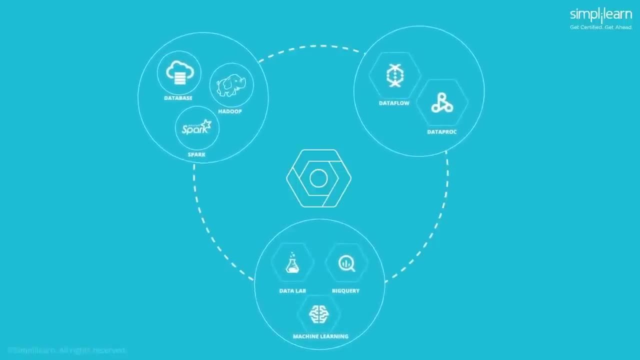 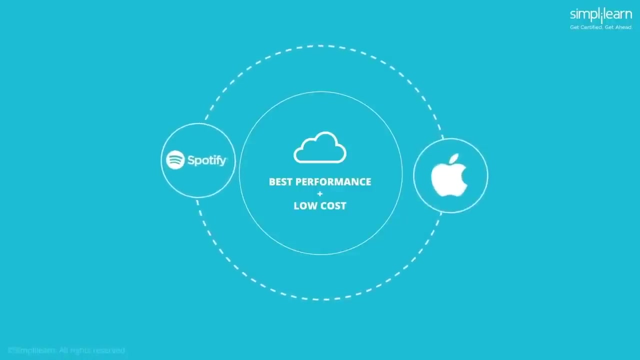 machine learning features make it a great choice for business intelligence, large-scale analytics and machine learning. its best-in-class performance and low cost makes google cloud popular and sought-after. technology giants like spotify and apple have implemented the google cloud platform at their organizations and healthcare and consumer goods leaders like phillips and 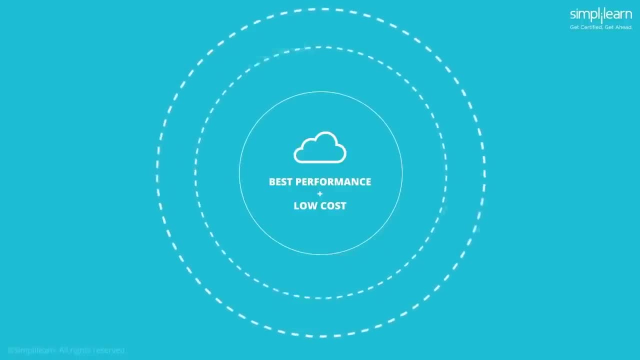 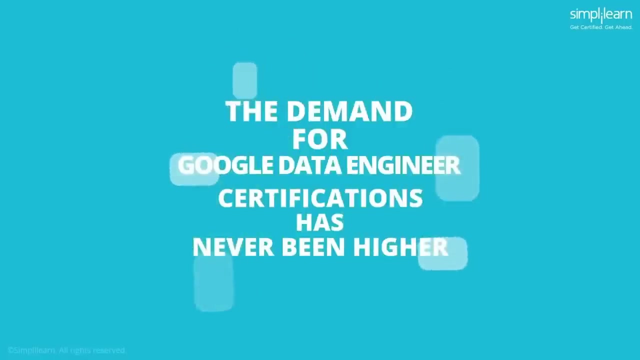 coca-cola are migrating to google cloud for their data analytics needs. a google data engineer with expertise in google cloud machine learning and bigquery earns 102 000 per year on average and the demand for google data engineer certifications has never been higher. simply learns google cloud. 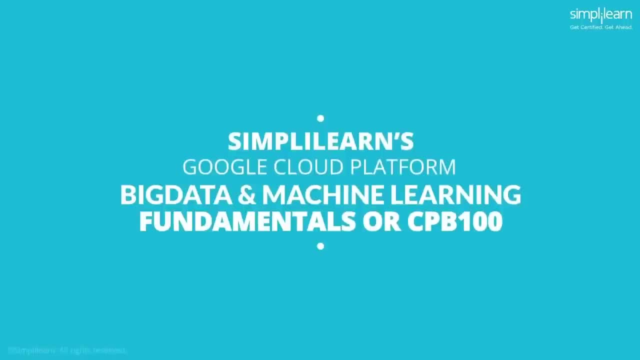 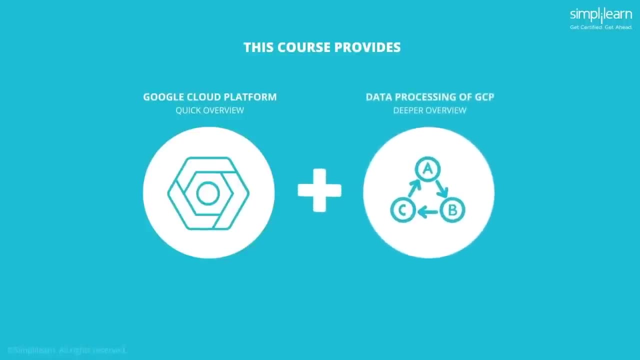 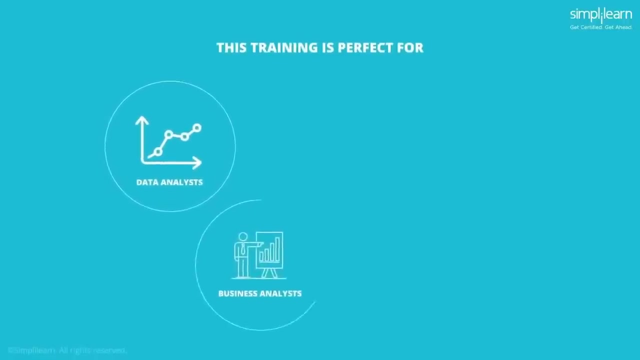 platform, big data and machine learning fundamentals, or cpb 100 course offers a thorough overview of the google cloud platform, covering its data processing capabilities with various use case studies. it's the perfect course for data analysts, business analysts and data scientists with real world experience in querying etl, data modeling or machine learning. it decision makers evaluating 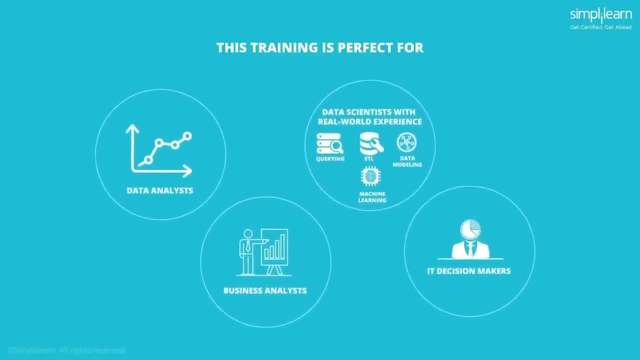 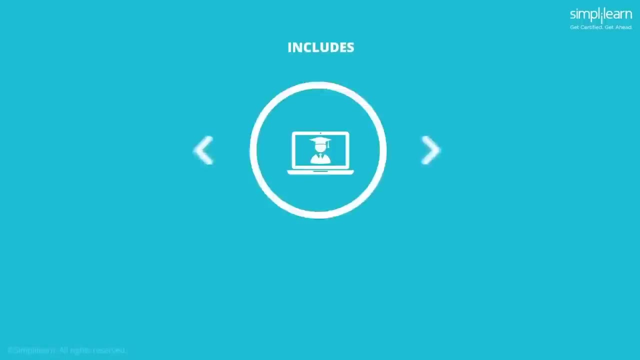 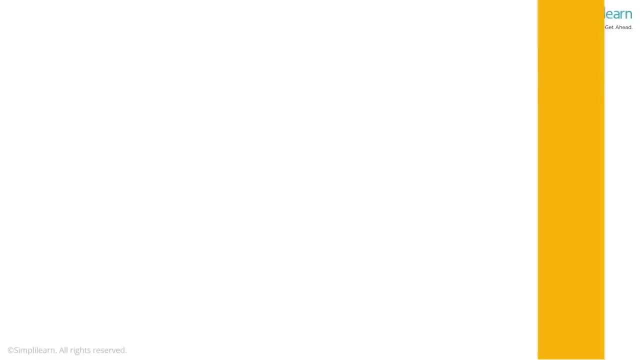 the google cloud platform have also found the training very useful. the course will cover everything you need to know about the google cloud platform and includes the google cloud platform training modules: eight hours of instructor-led training modules on big data and machine learning with the google cloud. hi, my name is randolph kale and i'm the co-author of the google cloud platform. 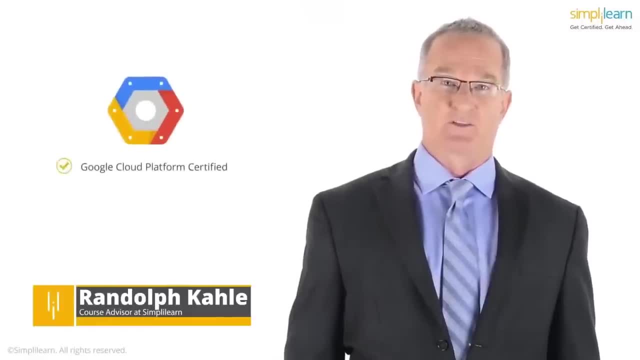 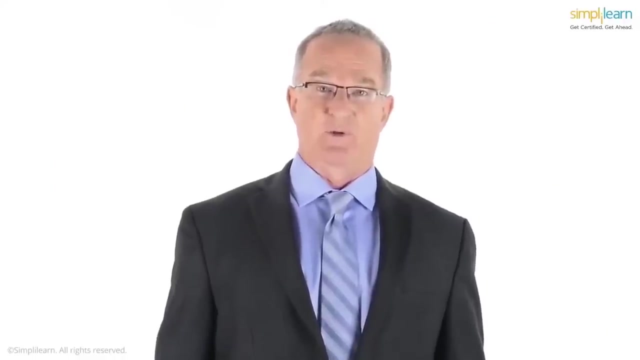 certification courses for google. i'm certified on the google cloud platform, an authorized google instructor and the course advisor at simply learn. i have over 40 years experience in the industry, spanning different roles from development, managing cloud infrastructure to product management. i've partnered with simply learn to ensure that you have the best opportunity to become certified. 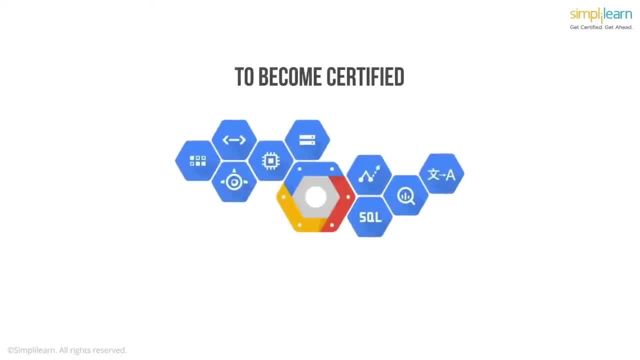 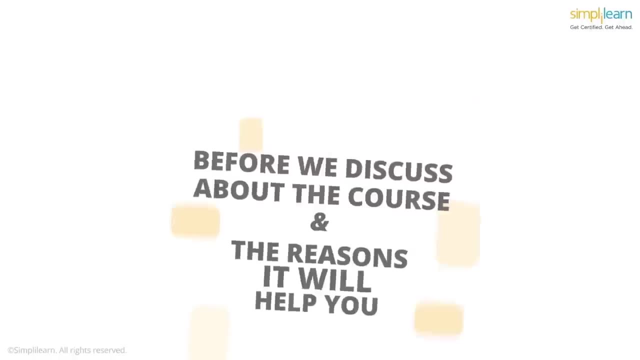 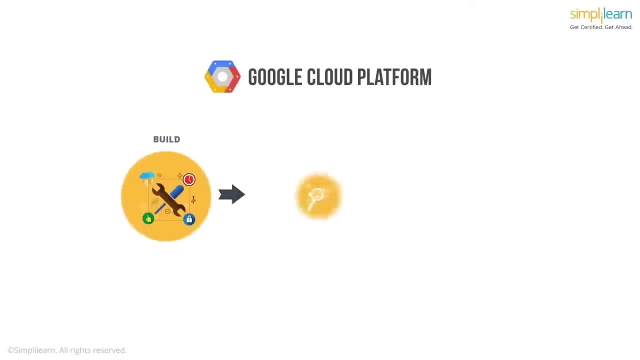 in various google cloud platform technologies, gain hands-on experience on the cloud and make you job ready. before we discuss the course and the reasons it will help you, let me first introduce you to google cloud platform. when you use the google cloud platform, you are empowered to build test. 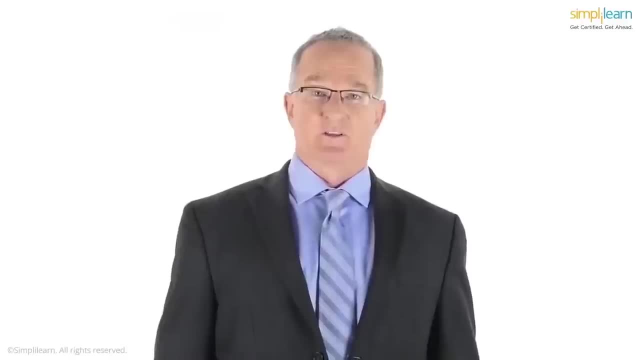 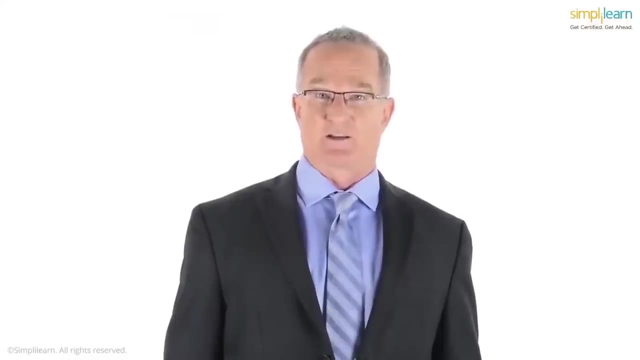 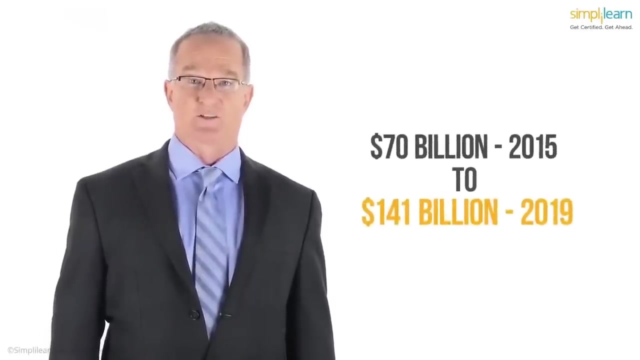 and deploy applications at google scale. the move to the cloud is happening today. there is a broad industry adoption. when i teach classes, i see the pace accelerating across all companies. forbes projects a 19 growth rate to 140 billion us dollars on cloud services by 2019. how can you move to the? 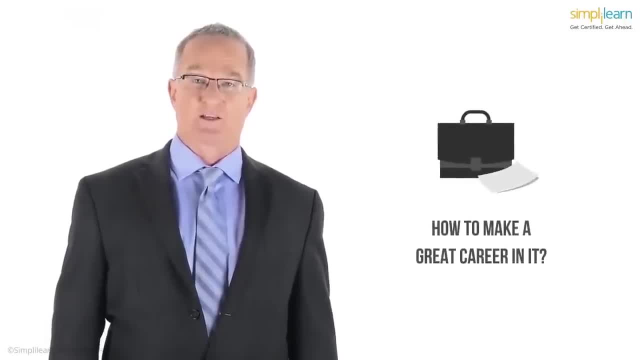 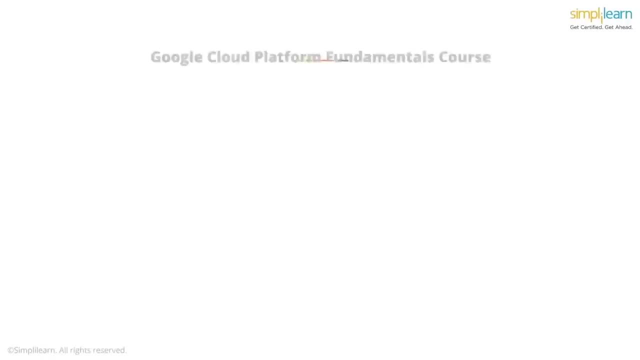 cloud. how can you make a career in this fast growing part of the industry? your first step is establishing your credentials in the google cloud platform domain, and you can do that by getting certified. the google cloud platform fundamentals course introduces you to the google cloud platform and shows you how you can incorporate cloud-based solutions into your business. 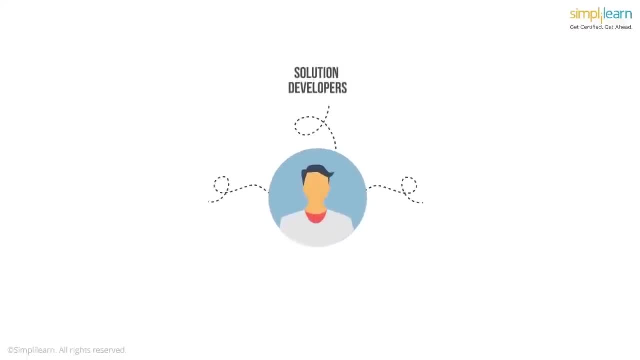 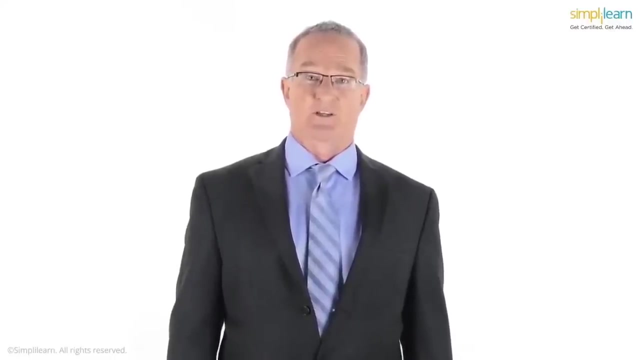 strategies. the course is intended for solution developers, system operation professionals and solution architects planning to deploy applications and create application environments on the google cloud platform. it is also appropriate for executives and business decision makers evaluating the potential of google cloud platform to address their business needs. completing this course will 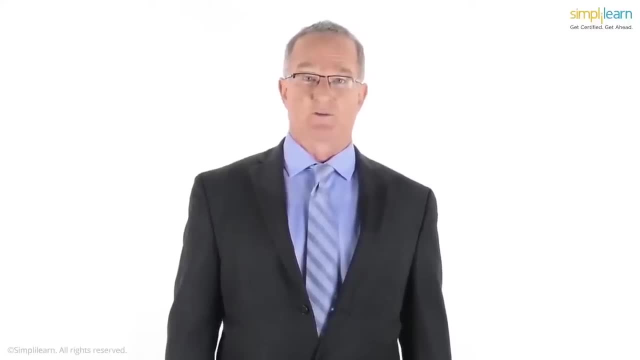 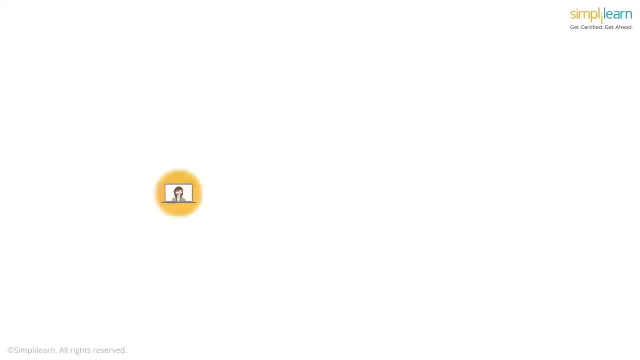 give you the skills and the confidence to take full advantage of the google cloud platform ecosystem. simply learn offers you extensive training to help you understand the platform. you get eight hours of interactive instructor-led live online sessions. along with the course, you receive a free trial account with 300 credit toward the use of google cloud platform for 60. 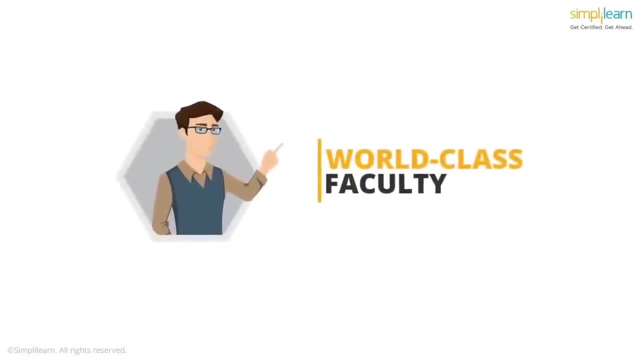 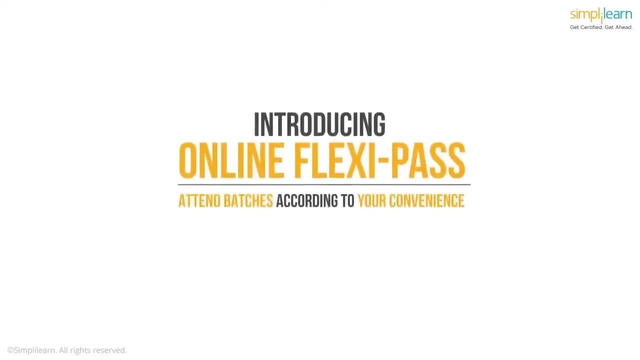 days. the instructors are google authorized trainers, the content is engaging and all the topics are very well explained with simply learn. you'll be enrolling for the online classroom flexi pass, which gives you the flexibility to attend any of the weekday and weekend batches according to your convenience. 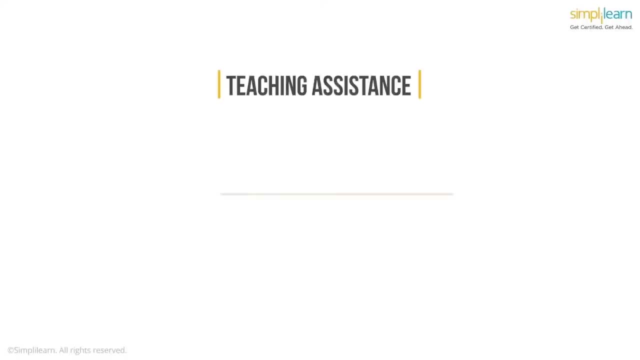 another thing that's impressive is the proactive teaching assistance, where experts resolve all your course related, project related or technical questions while pursuing a course. so if you're looking for the training and guidance, you need to have a deeper understanding about google cloud platform products and services. please visit the google cloud platform website for more information. 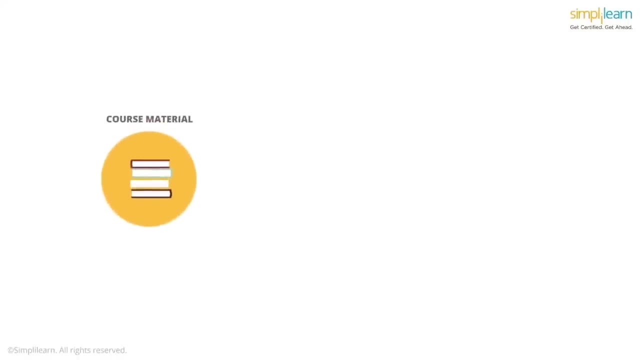 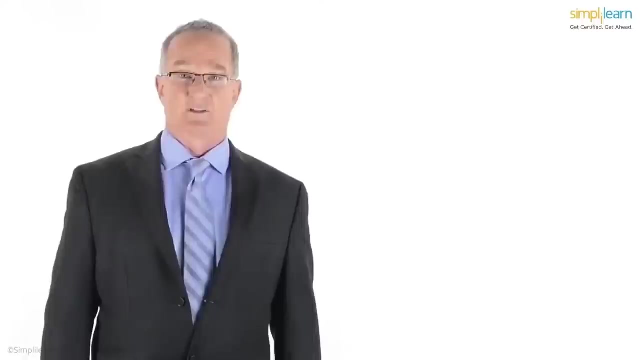 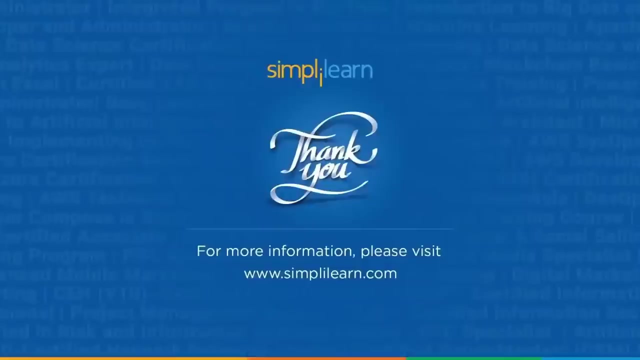 this is the best course for you. with the course material, labs and authorized instructors with extensive experience, i don't think you'll need to go anywhere else. take charge of your career. sign up for, simply learn cp 100a training. all the best to you. and with that we have come to the end of 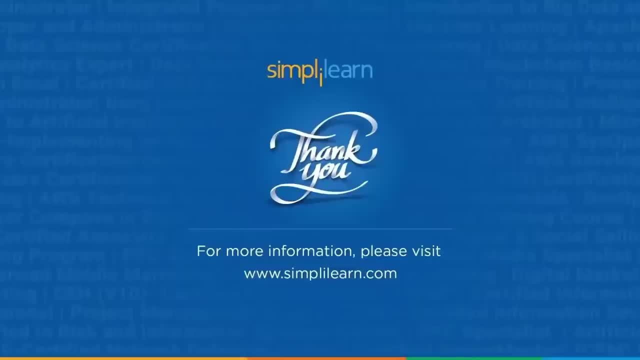 this video on google cloud platform full course. i hope you found it informative and interesting. if you have any questions about the topics covered in this video, please ask away in the comments section below. Our team will help you solve your queries. Thank you for watching. Stay safe and keep learning. 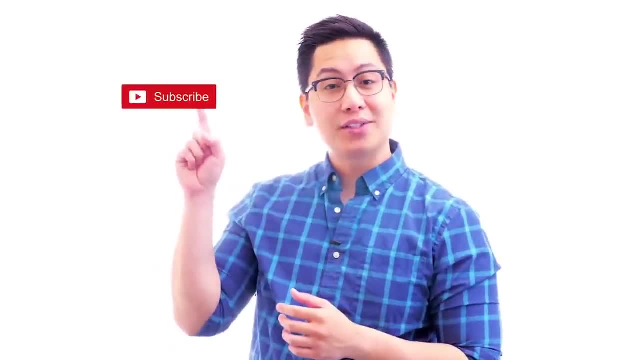 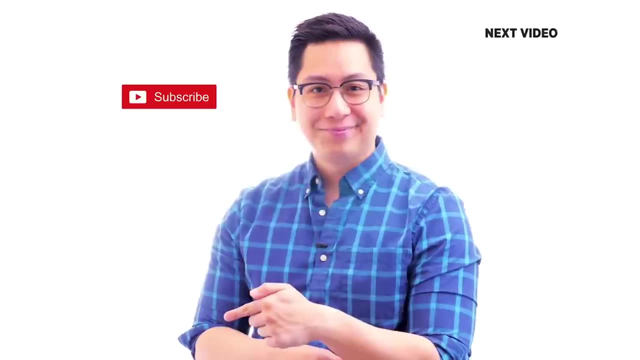 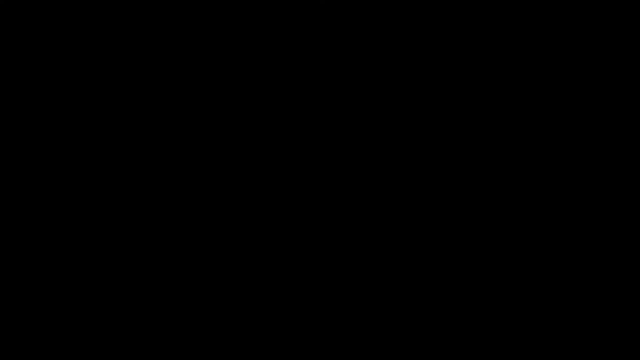